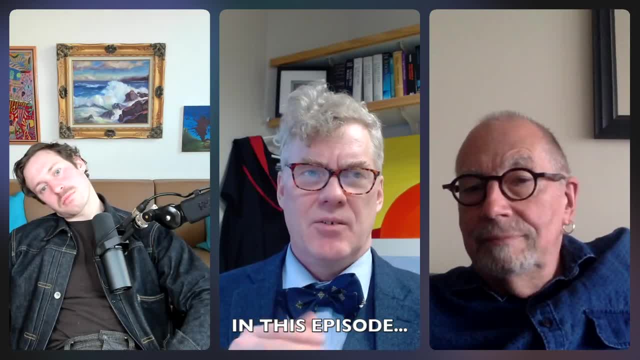 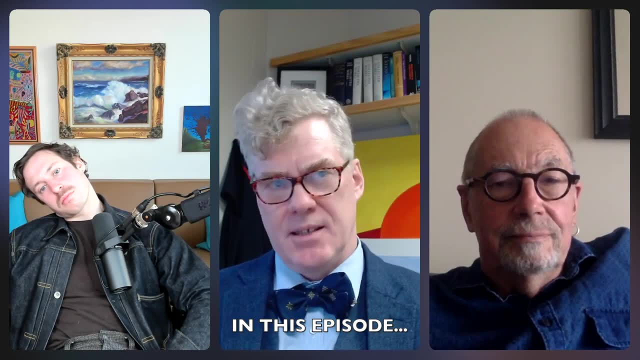 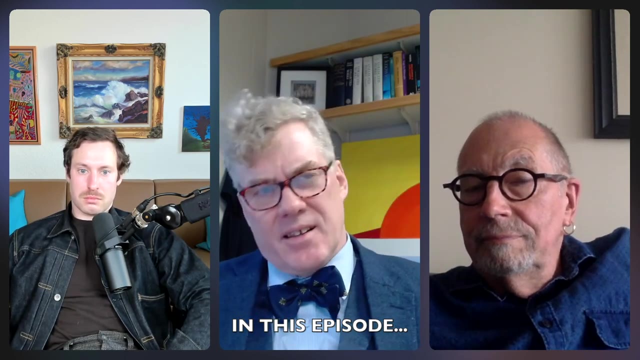 People often talk about, you know, existence in space and time and so on, and physical existence in a manner that suggests that that's the one that we really understand. but abstract existence is the problematic one, And my view is that this is exactly backwards, that actually physical existence is the one that's deeply mysterious. 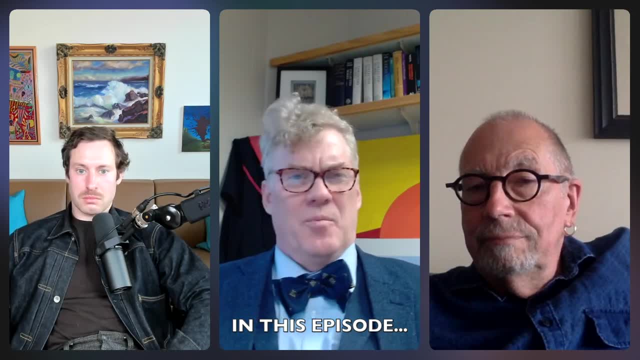 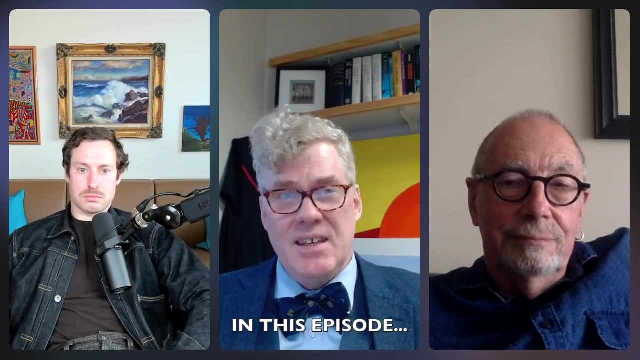 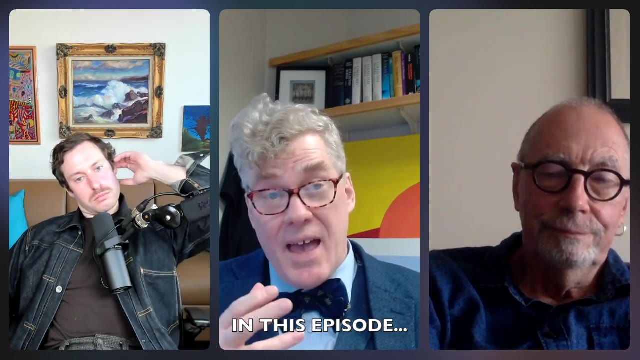 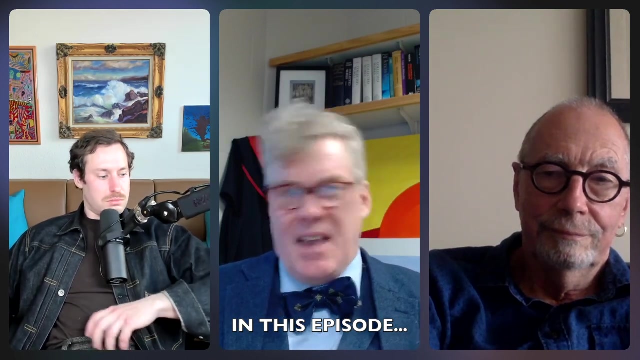 I mean, the more physics we learn, the more strange physical objects are. I'm not even sure, actually, one can give any kind of sensible account of what it means to say that a particular thing exists physically, whereas the existence of the empty set is something that we can seem to say something about, what it means for such a thing to exist. 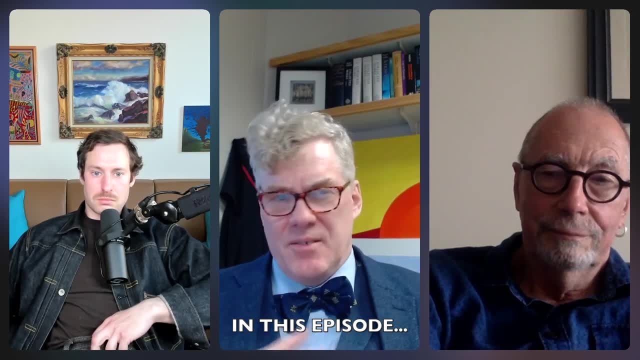 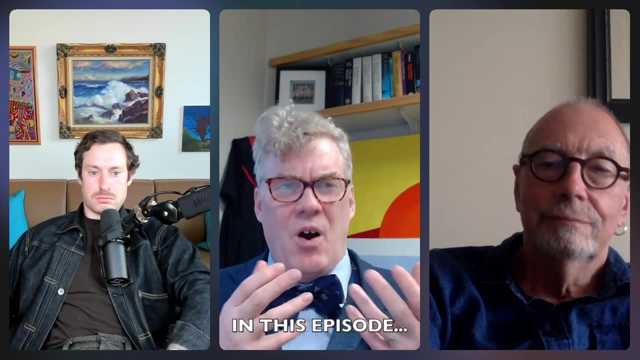 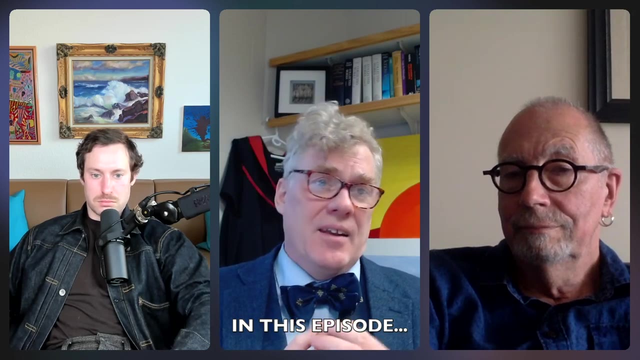 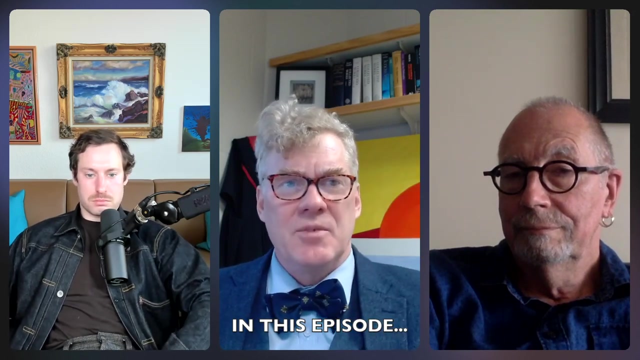 So we can talk about, you know, the instances of contradictory properties and it's the set of instances of contradictory you know. The point I'm trying to make is that that explanation is It's just far more thorough in giving an account of what it would mean to say that the empty set exists than any kind of corresponding assertion or explanation of what it means to say that this cup is a physical object. 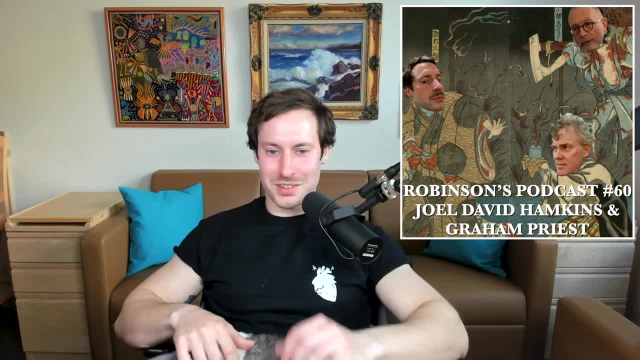 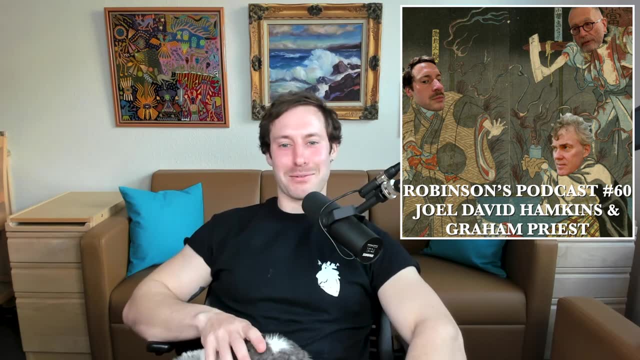 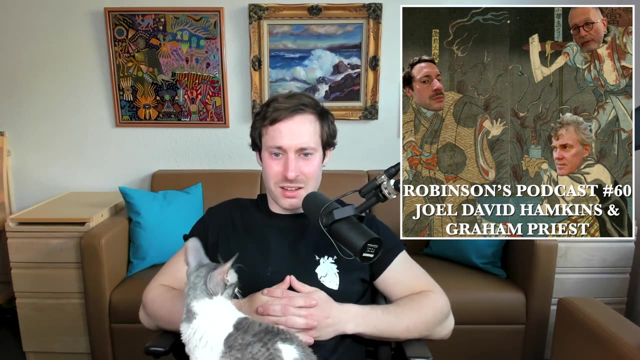 Hello my geeslings. It is Mother Goose Robinson Earhart here with the introduction to an absolute banger, Robinson's podcast number 60. So my two guests on In this episode are prior denizens of the Robinson's podcast universe, which has since split off actually into the Robinson's podcast multiverse. but we'll get to that momentarily. 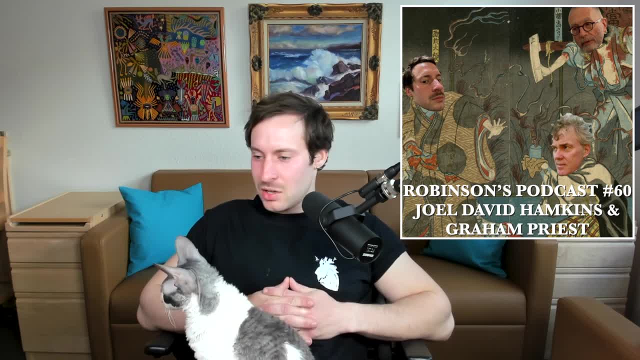 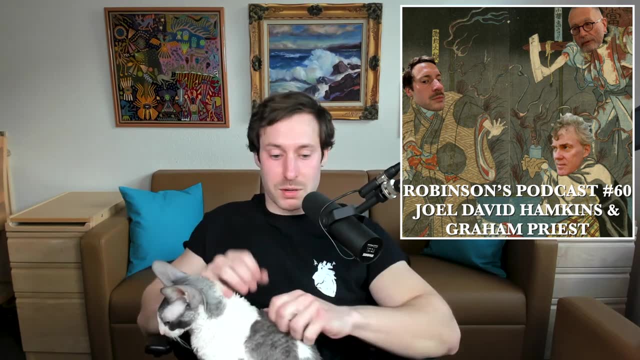 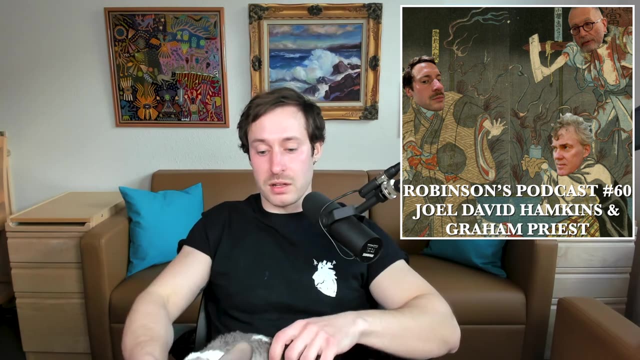 So my two guests are Joel David Hamkins, who is the O'Hara professor of philosophy and mathematics at the University of Notre Dame, where he recently moved from Oxford, And Joel is a top-notch philosopher of mathematics, Also one of the leading set theorists in the world and the reigning king of math overflow. 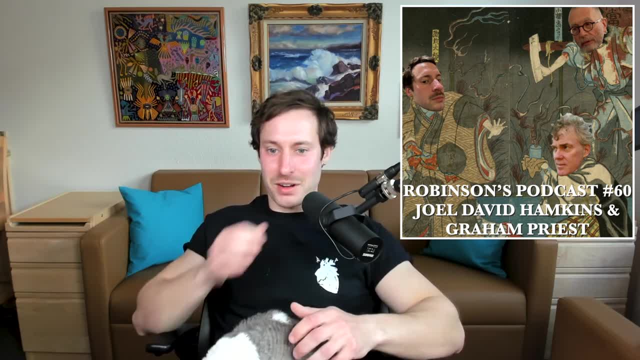 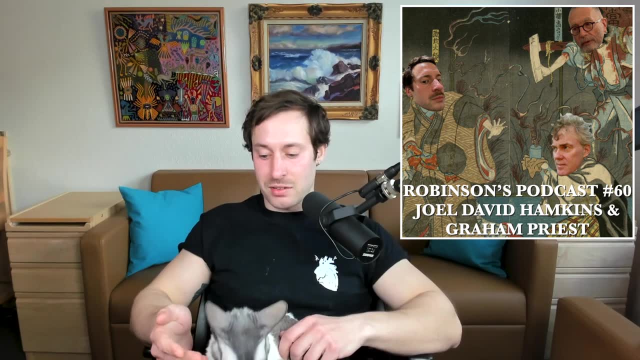 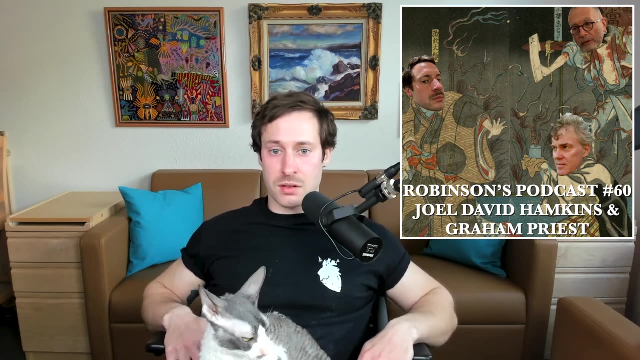 And my second guest is Graham Priest, who is distinguished professor in the philosophy department at the CUNY Graduate Center, And Graham is also, I mean, one of the most widely cited influential philosophers of the past 50 to 100 years or so. 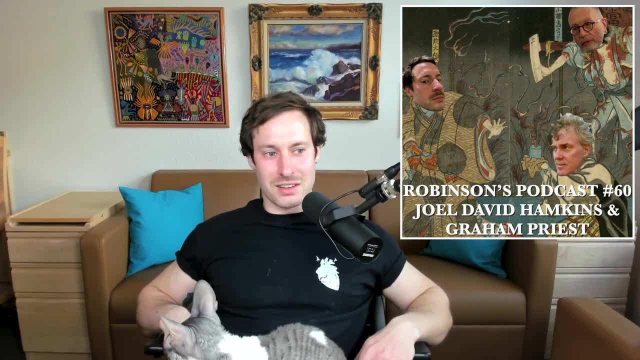 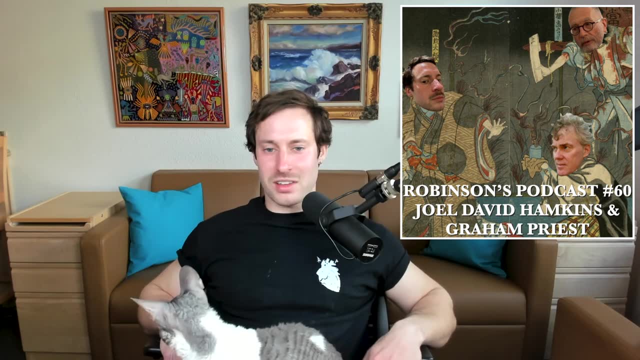 I was looking at his publications A few days ago and I think he's written like 350 papers or more than that, and has plenty of books and on all sorts of wide-ranging topics. It's really extraordinary. I imagine that there are few, if any, people in the philosophical world who have done so much good and wide-ranging works. 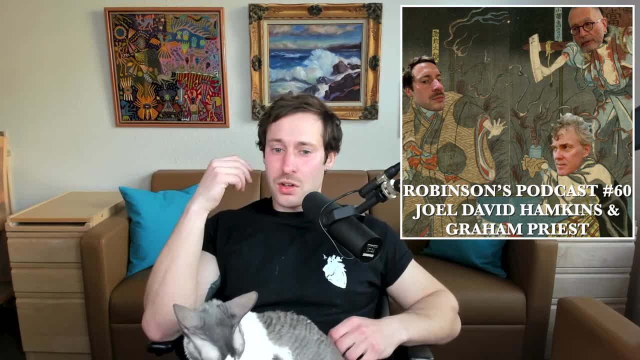 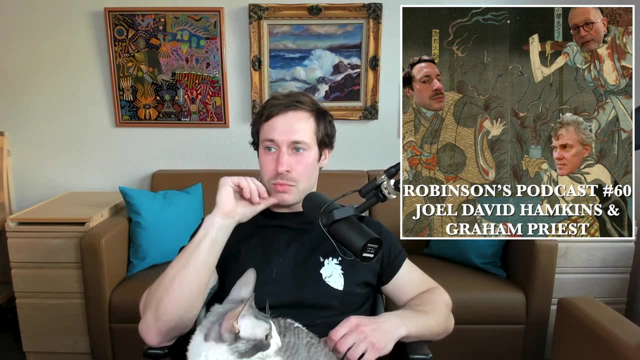 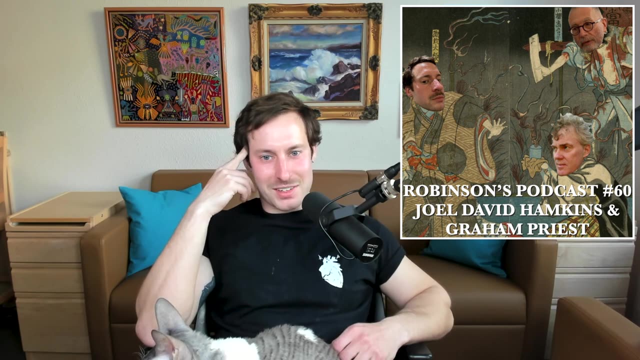 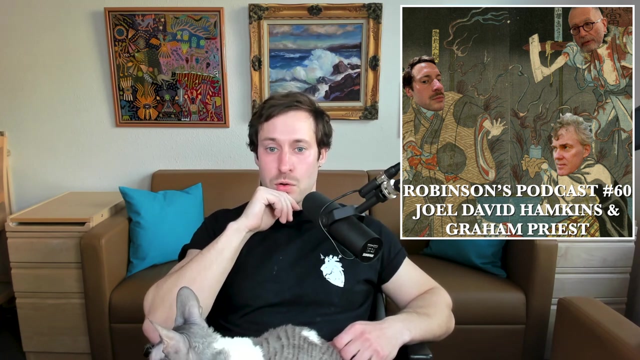 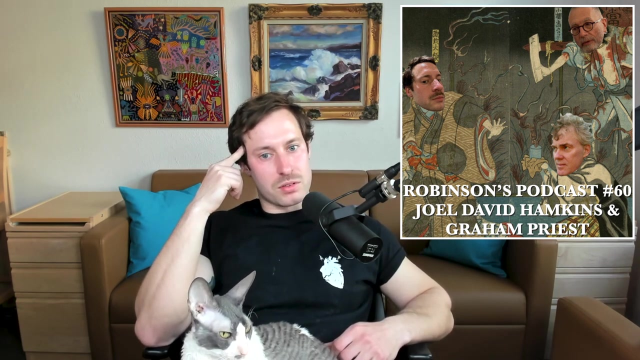 So this episode we talk about two topics primarily, which are the liar Paradox and the set theoretic universe or multiverse, and my sister, who is a listener of the podcast, has pointed out that I really need to do a much better job of motivating the questions that these episodes consider in the introduction, because I don't want these episodes to be appealing only to philosophers or mathematicians or 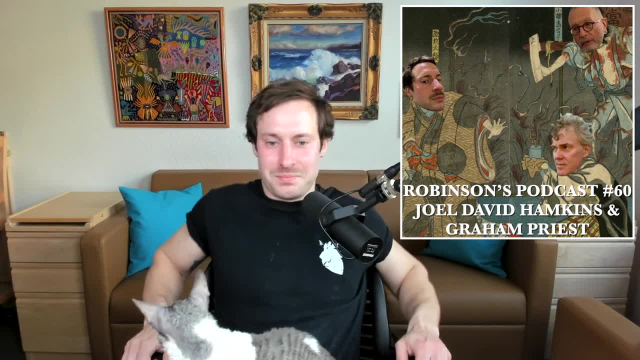 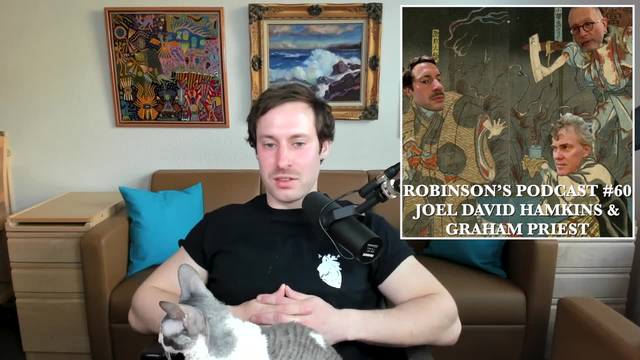 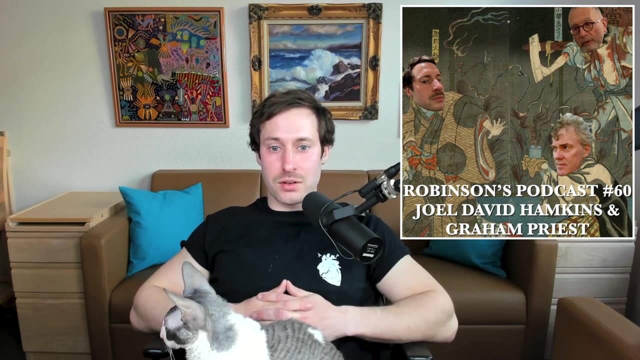 Highfalutin intellectuals. I guess I like this to be appealing to a broader audience, but this is not really the episode for that, because this episode is extremely technical. So what I would recommend is checking out JC Beals article on the liar paradox on the Stanford Encyclopedia of Philosophy, and maybe Joan Bagarias. 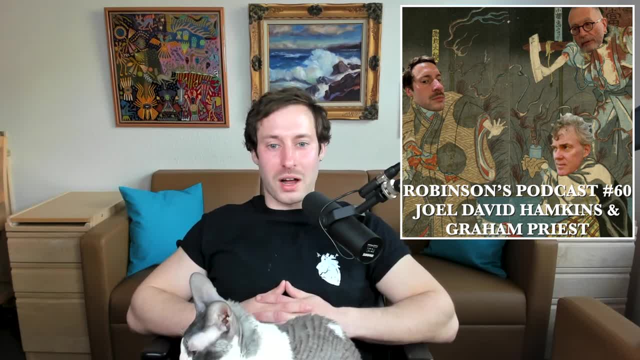 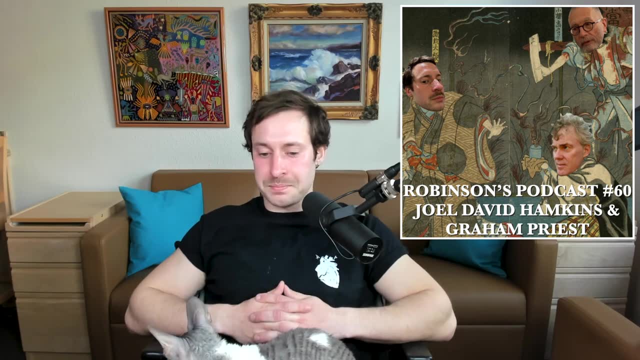 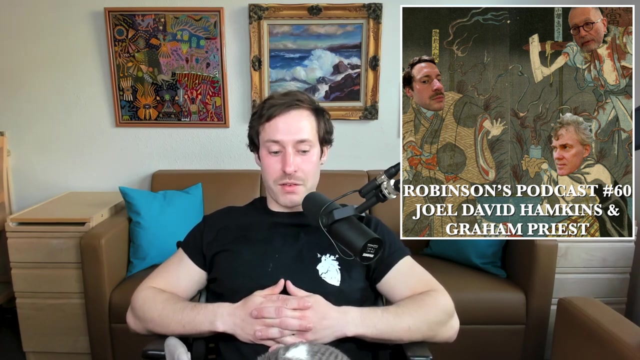 I'm not sure he's Spanish, so I'm not sure if it's Juan Bagarias Article on the liar paradox On set theory in the Stanford Encyclopedia of Philosophy, But at any rate, the liar paradox stems from Ubulides, who is my close friend and mentor, Haim Gaifman's favorite ancient philosopher, about 2500 years ago, and he had all sorts of paradoxes. 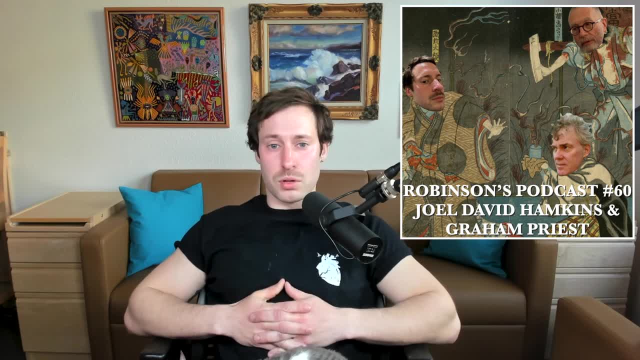 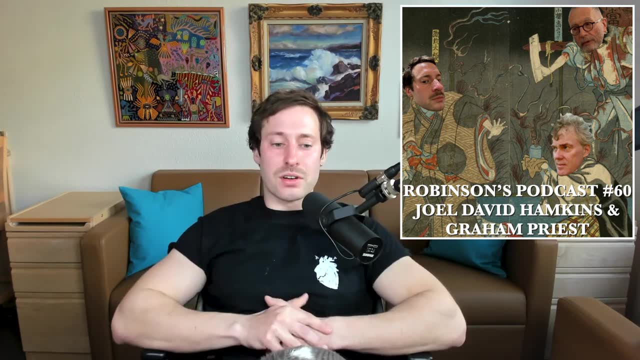 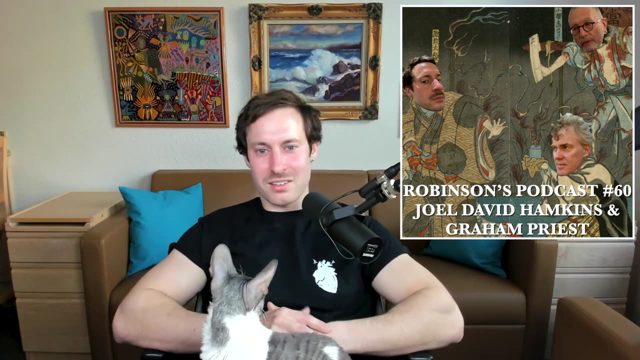 I think the sororities is attributed to Ubulides as well, But the- At least I think the initial version of the paradox is: you have a cretin. a cretin comes up or comes up to you, and he says: all cretins are liars. 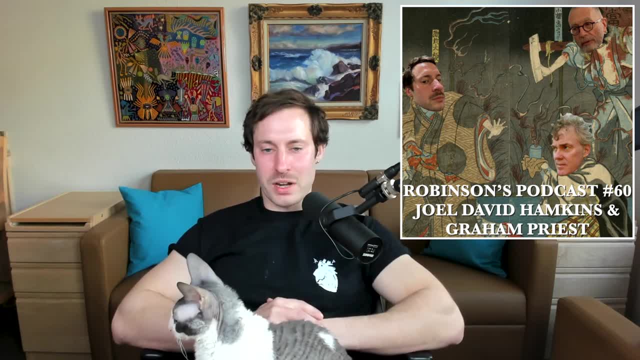 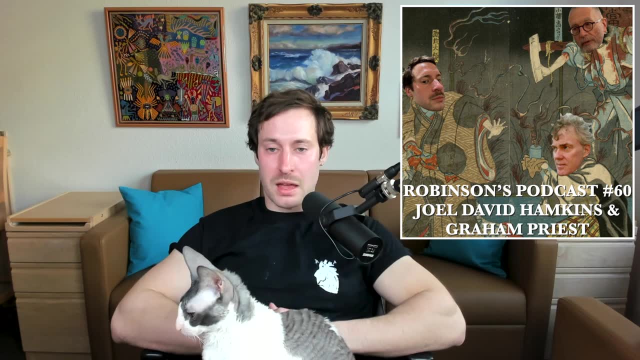 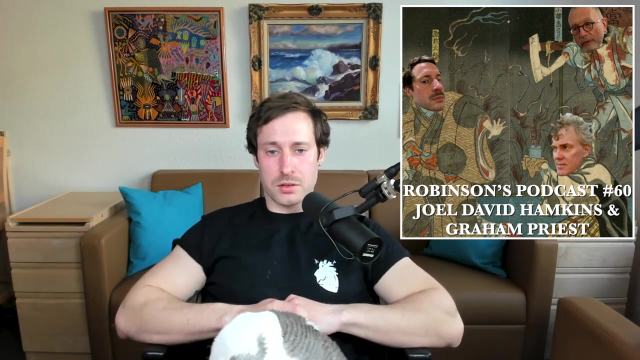 And the idea, roughly, is: what are we to make of a sentence that says of itself that it's false? And Graham has a very notable and important approach to this paradox. So That is the first one, The first topic we discuss, and how answering or responding to this paradox raises questions of logical pluralism. 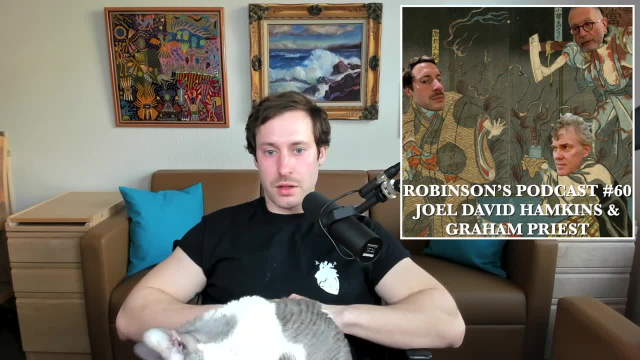 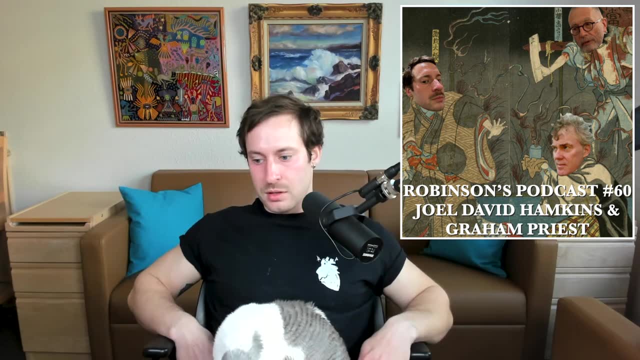 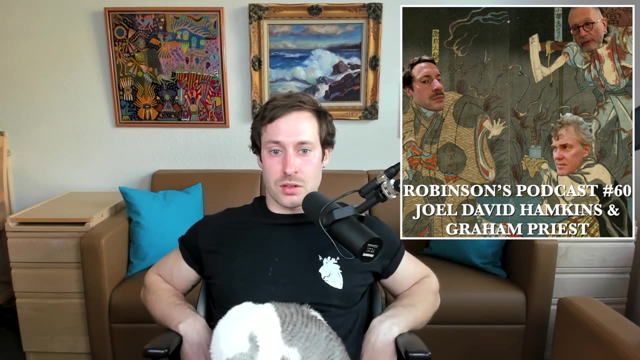 So there are plenty of different logics. There are intuitionistic logic, paraconsistent logic, classical logic, fuzzy logics, Anyway, And There is a question of whether or not one of these logics is the correct logic, Or if all of the logics are equally valuable and which we should choose in various situations. 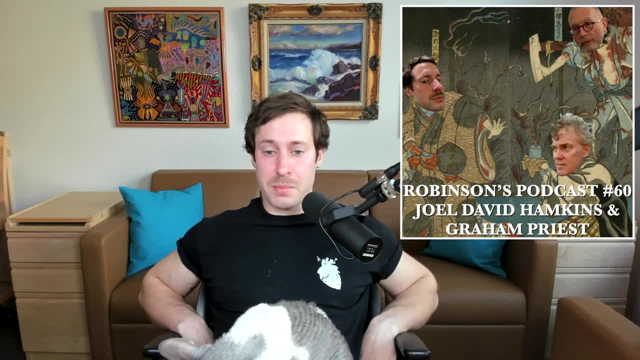 So that is, I'd say, the main point of discussion surrounding the liar's paradox. And then we turn to the set theoretic multiverse, which is the contribution to the philosophy of mathematics that Joel is best known for, And The set theoretic multiverse clearly hinges on set theory. 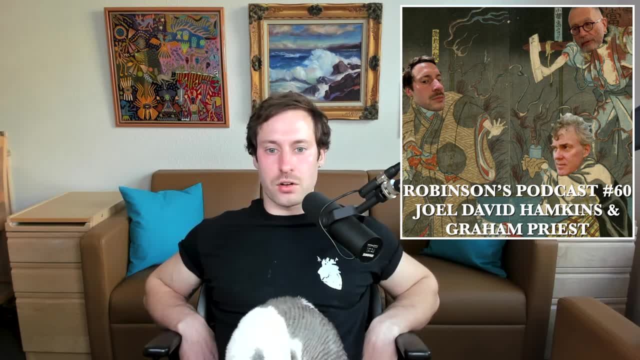 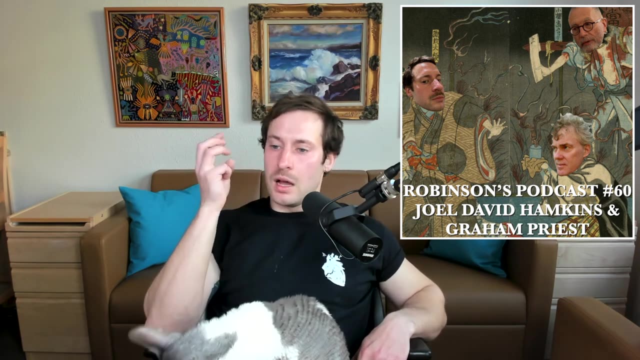 And, as I mentioned, you should check out the article by Joan Vigueria on the Stanford Encyclopedia of Philosophy. But set theory is that branch of mathematical logic of which there are four, depending on who you ask: Set theory, proof theory, model theory and recursion theory. 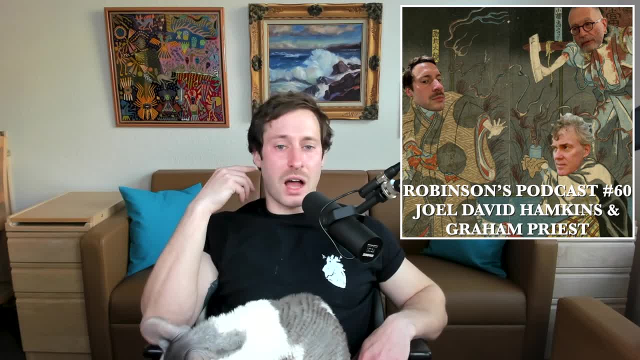 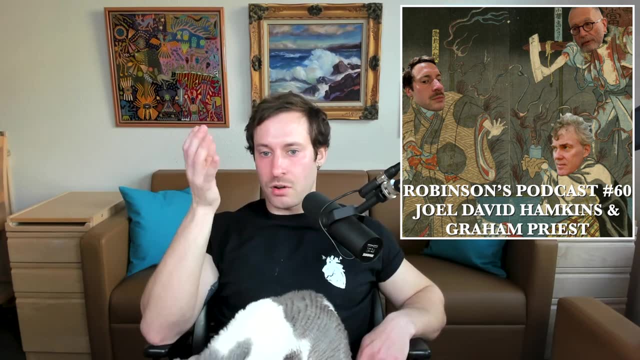 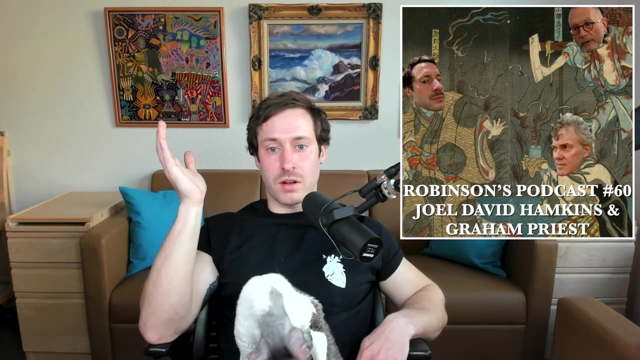 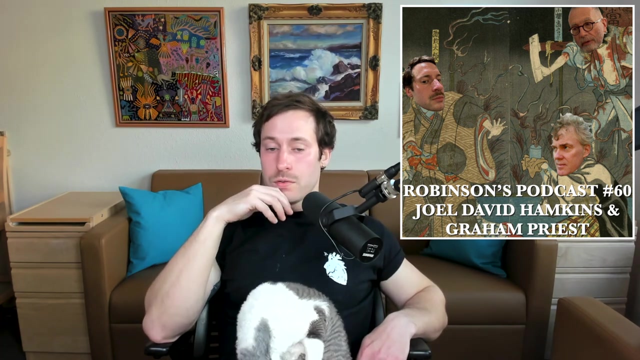 That deals with the objects of Mathematics, At least that's how I think about it, Because all objects numbers, triangles, what have you. they can be construed as sets, which are just collections of objects, And Set theory is of particular interest to philosophers of mathematics, I think because largely of these ontological concerns. 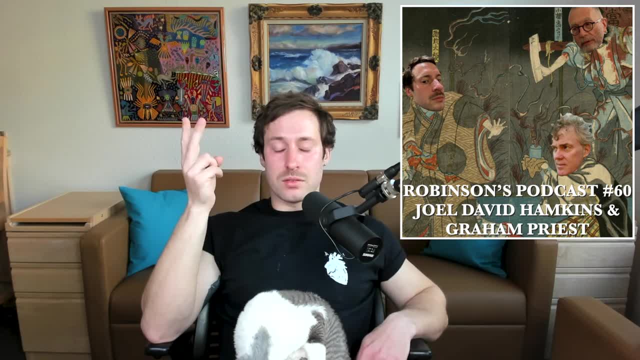 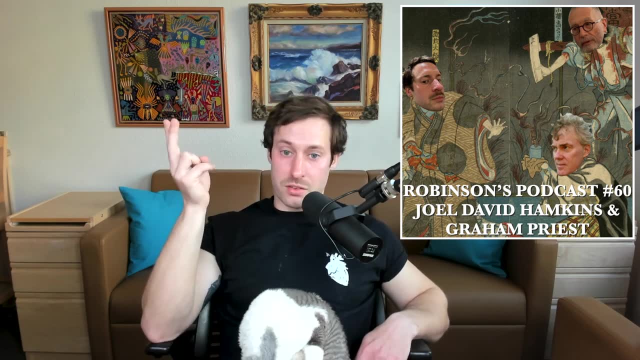 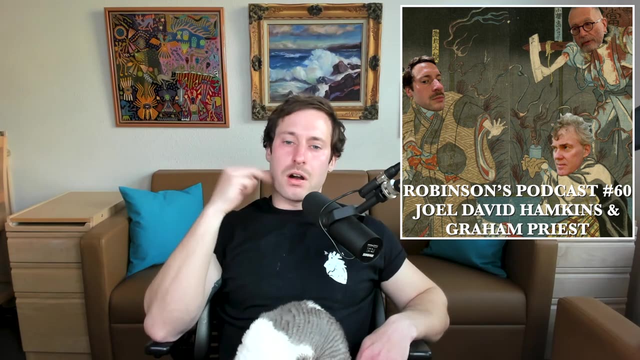 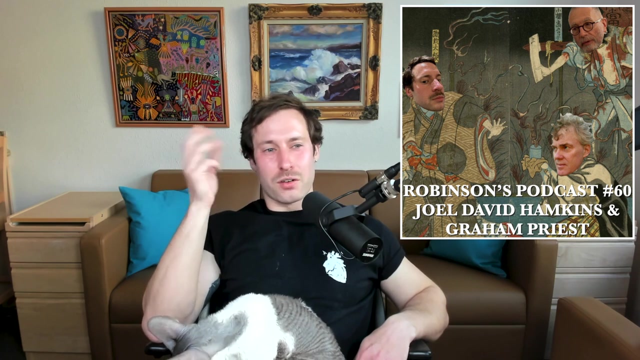 One Set theory is the mathematical discipline par excellence for discussing questions of infinity, which is another major concern of the philosophers of mathematics. But there are also very important questions in the philosophy of mathematics that surround what I'll refer to as objectivity. So is there one correct answer to a certain set theory? 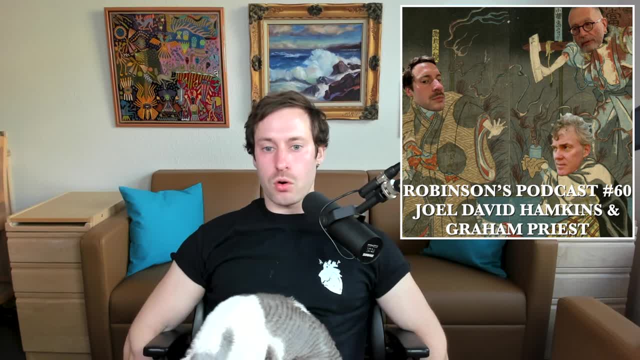 Is there one correct answer to a certain problem? And, Joel, I think one of the primary motivations of the set theoretic multiverse believes that there is not just one answer, For example, to the question: Is there an intermediate cardinality between the naturals and the reals? This question has different answers depending on the set theory in which you're operating. So in discussing this question, so the set theoretic multiverse then is that there are sort of multiple universes of objects about which mathematics is concerned- Stands in opposition to the monist theory that is most closely associated, I think, with Gödel and Hugh Wooden and Peter Colner today. 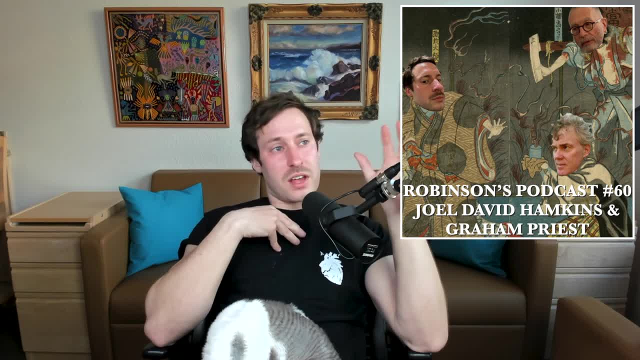 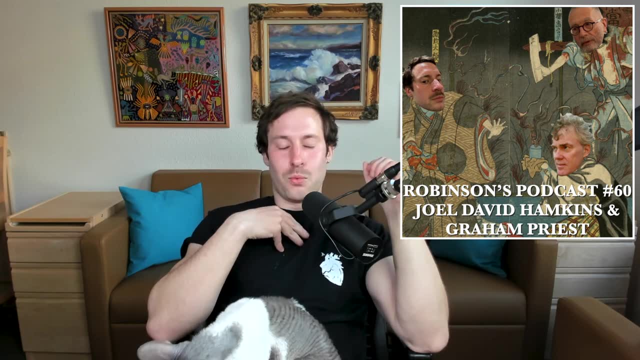 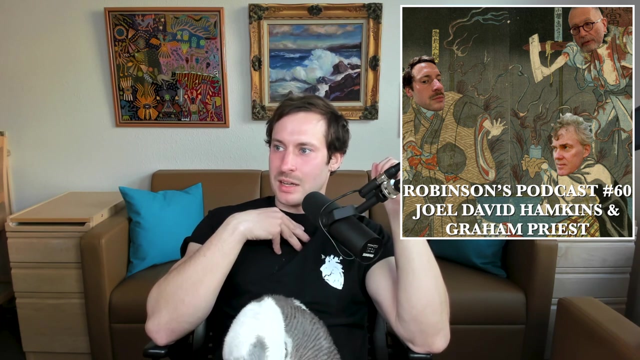 And so we discuss the tension between these two views, We discuss the metaphysics of the multiverse, And then we discuss how all of this relates to the age-old question of whether or not mathematics is created or discovered, And even though that is a sort of trite question that everybody gets, it is a really deep and important question. 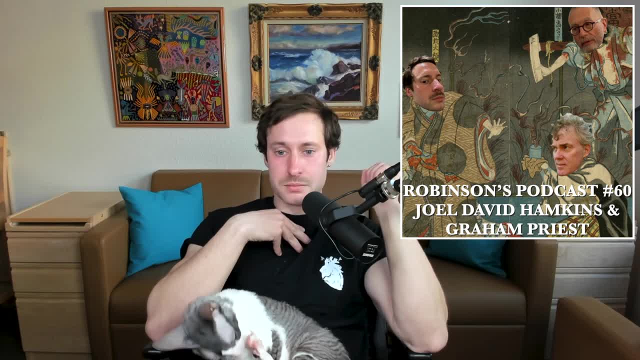 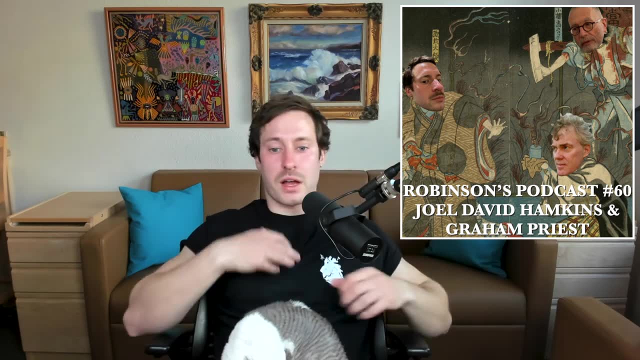 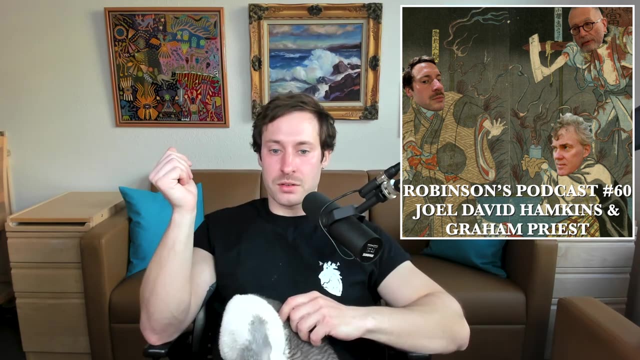 And we actually have a really nice discussion about it. Now, some resources for background information. I've already just mentioned And you should also check out Joel's current project, which is the Book of Infinity, And it's an accessible text on paradoxes and the infinite. 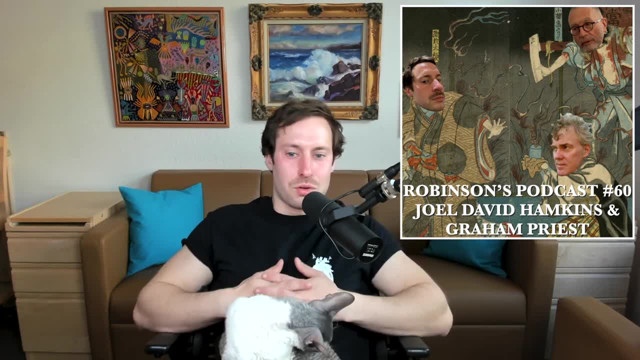 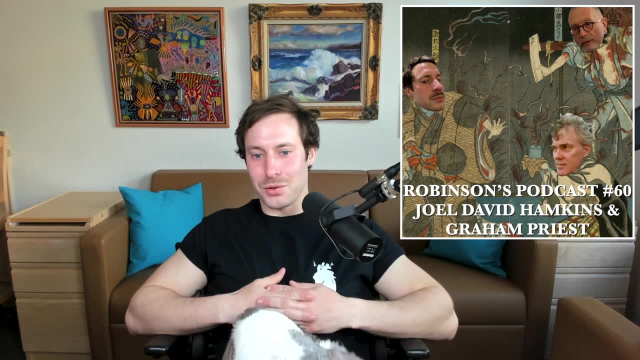 And he's made the very cool move of serializing it on Substack So you can participate in its creation and weigh in through Twitter and read it chapter by chapter, And it's been a really cool project. Then you should also check out Joel's Twitter, his Math Overflow, his blog. 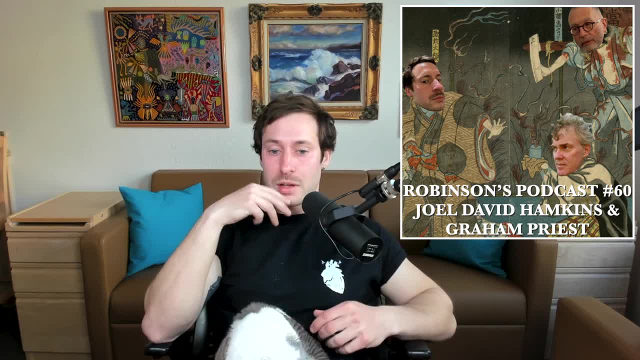 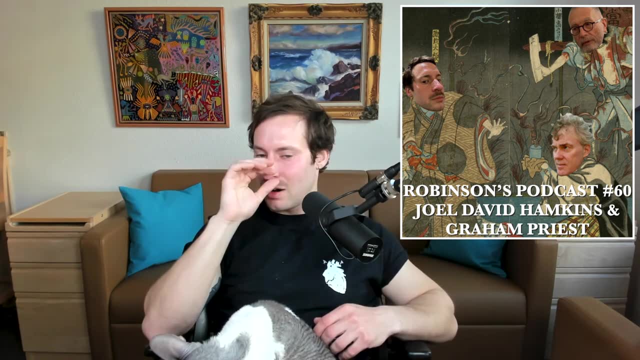 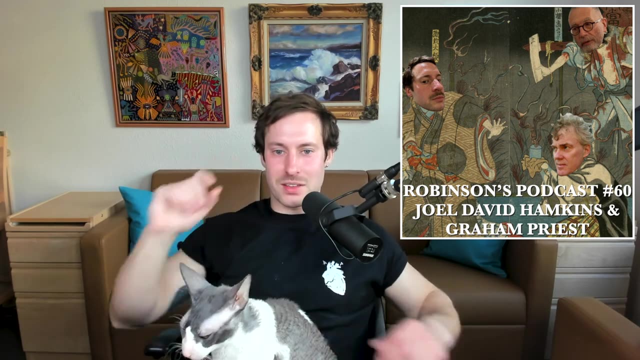 And you can keep up with Graham on his website, grahampriestnet. Though all of these links are in the description, Then the last things I'll mention are following me on Twitter, Instagram, all of these places. That's very helpful. 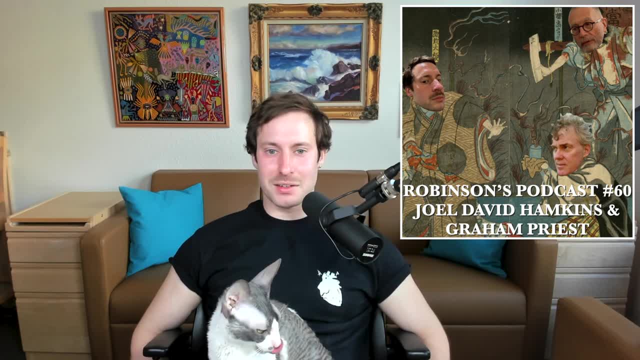 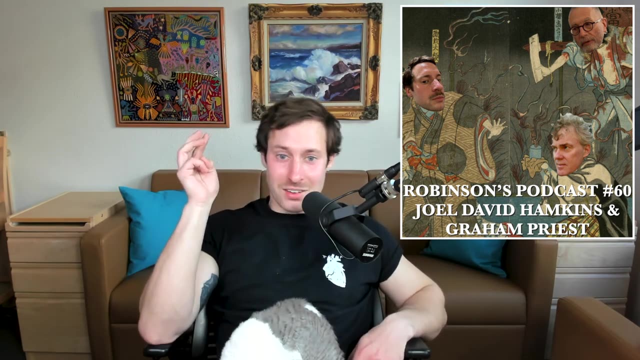 Leaving reviews. I would like more eyes on this podcast And ears And attuned to my guests as well. And then the last thing I'll mention is the Robinson's Podcast Multiverse, Which has now branched in two directions. I have a second show called Robinson Eats. 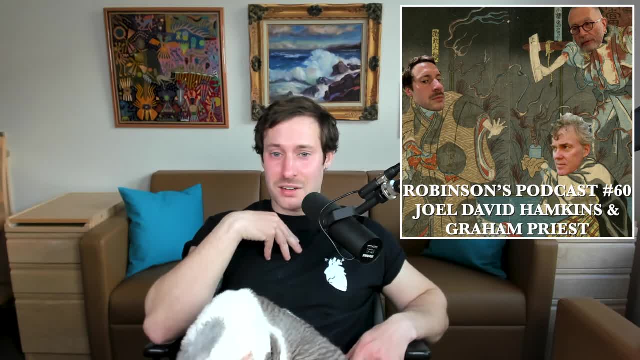 Which is much less philosophically inclined, Though it has its philosophical moments In which I eat a pint of ice cream or something else, I guess, every morning At Palo Alto time, So maybe 9 or 10.. And I do that on Twitch. 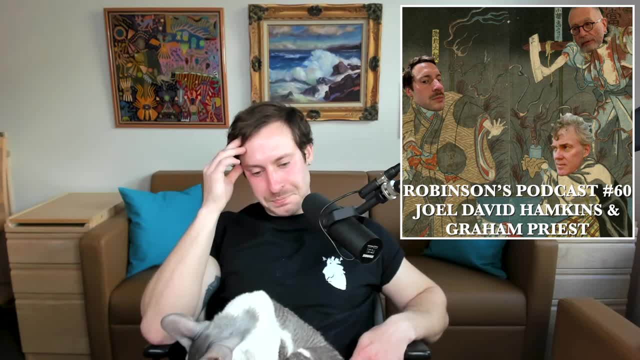 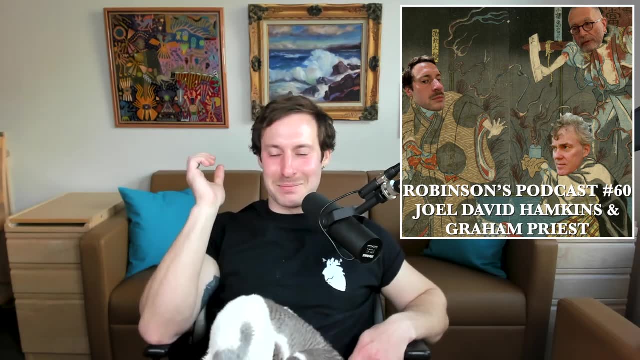 Also on YouTube And I talk with whoever's there. And then I just purchased robinsonsfashionempirecom And maybe I should have called it Le Maison Robinson. But anyway, I have a t-shirt for sale. I designed it. 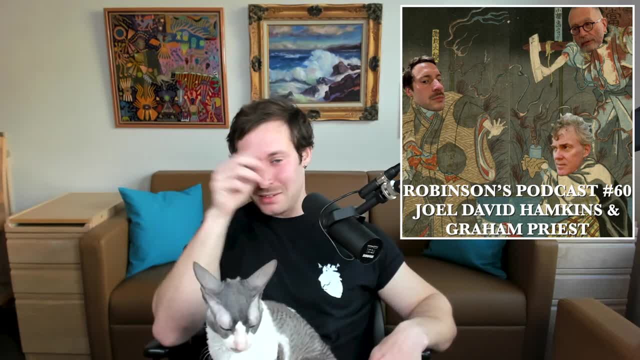 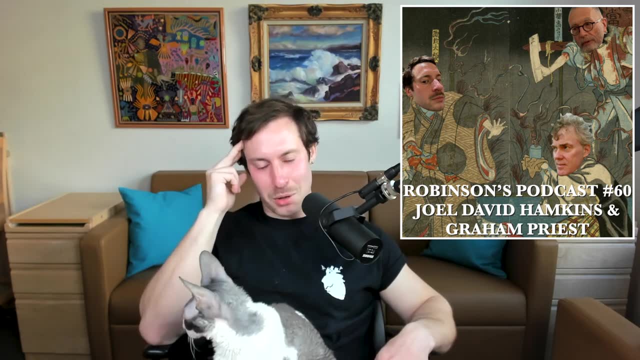 There's an R and a P for Robinson's Podcast And please don't buy it. if you don't want to, You don't have to, But it's a nice way of helping out with the proliferation of the Robinson's Podcast Multiverse. 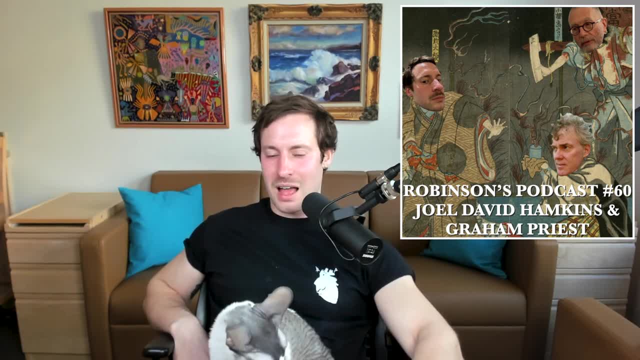 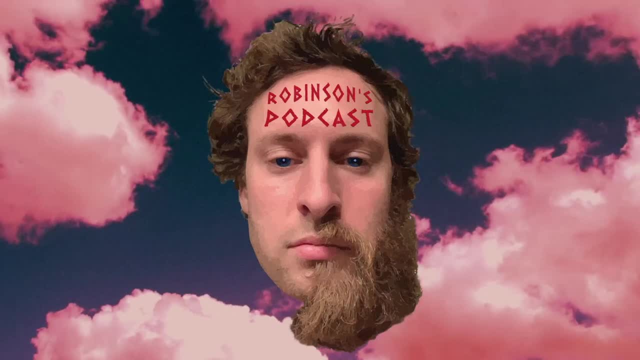 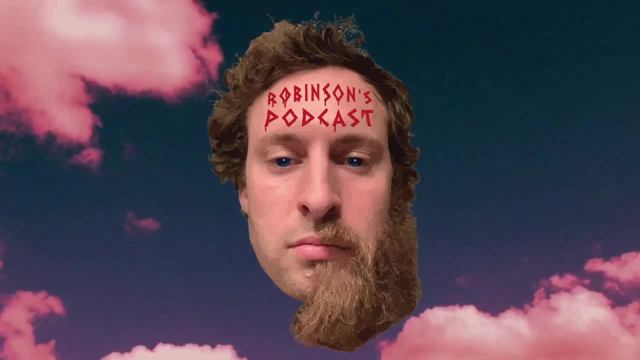 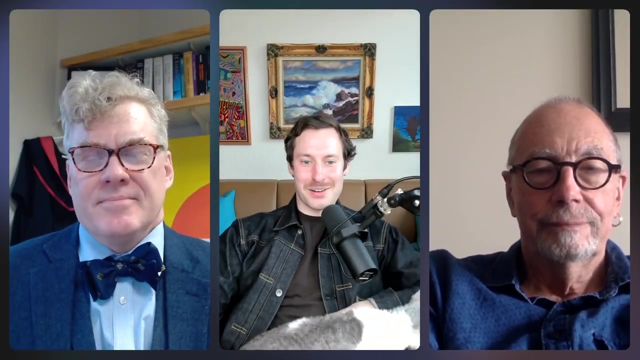 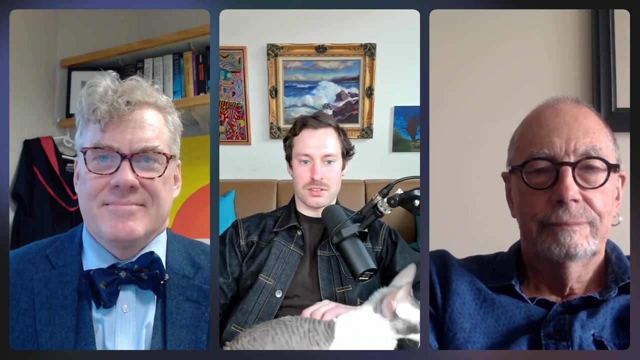 And now, without any further ado, I hope you love this conversation as much as I enjoyed having it with Joel and Graham. Graham, I know this is a very old hat for you, But based on the two of your mutual interests, I thought a nice place to start would be with the liar paradox. 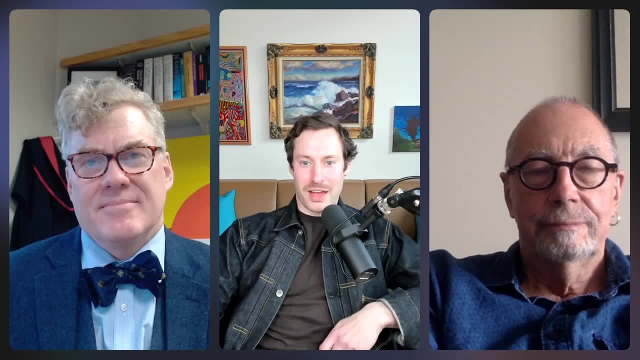 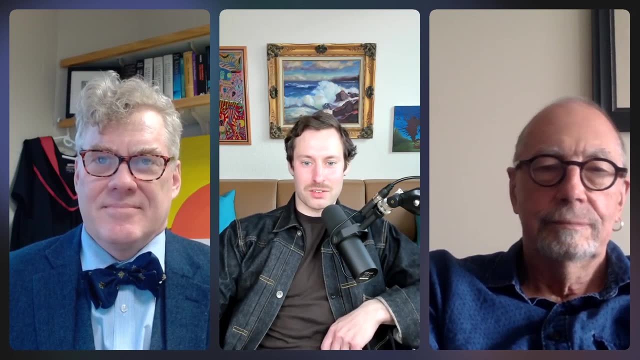 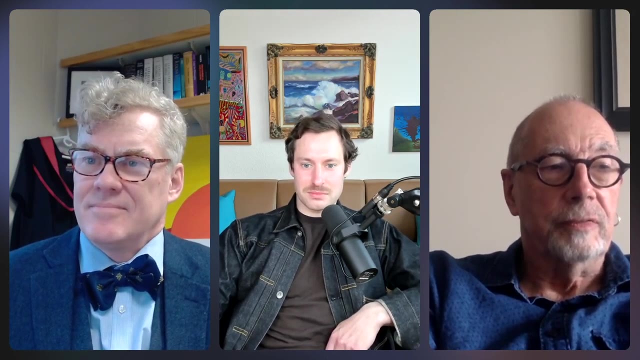 And since you- I mean you both- have your doctorates in mathematics, not philosophy- I'm curious about when it became such an issue, When it became such an important problem for you. Okay, that's easy. When I was a graduate student, I went to a conference. 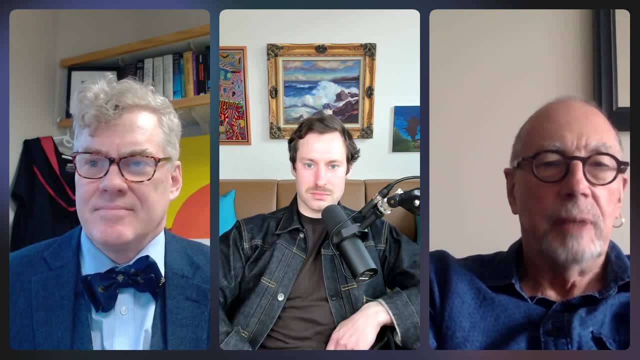 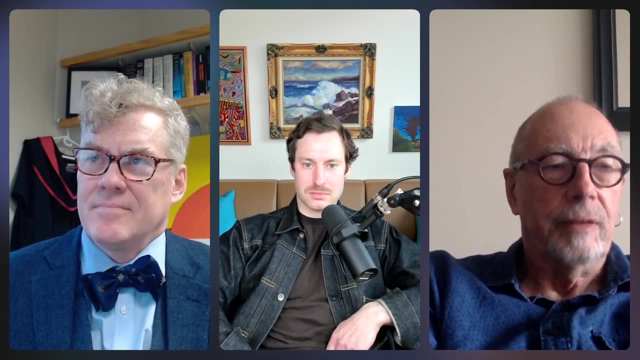 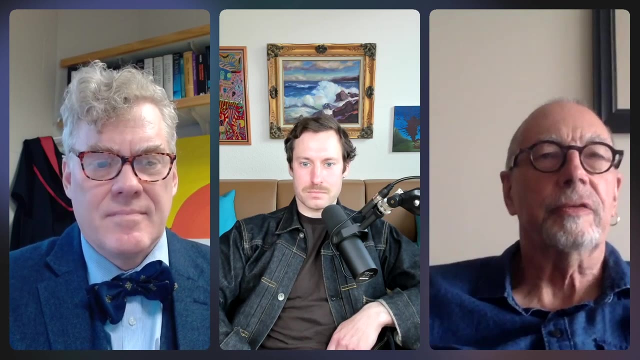 It was the first conference I ever went to And there was a talk by Moshe Makova on Gödel's theorem And it centered around the question of how there can be things which we know to be true which you can't prove. Now, obviously there are all kinds of moves you make in that context. 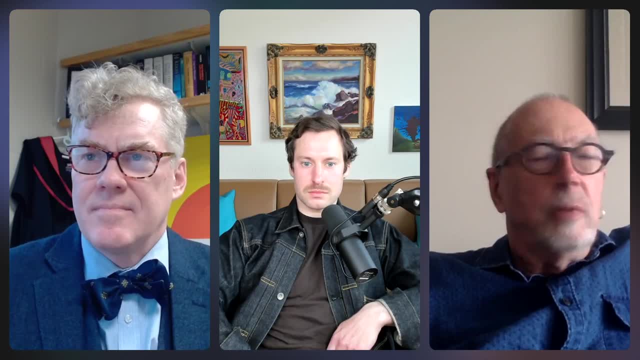 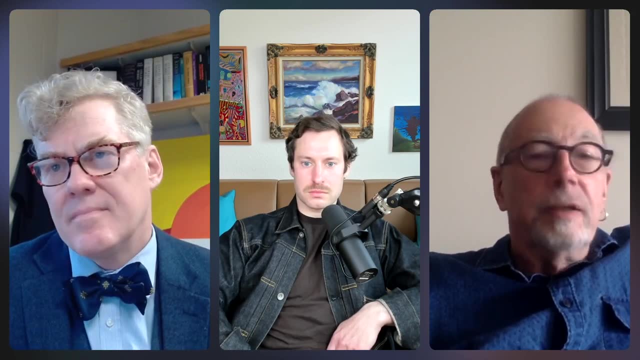 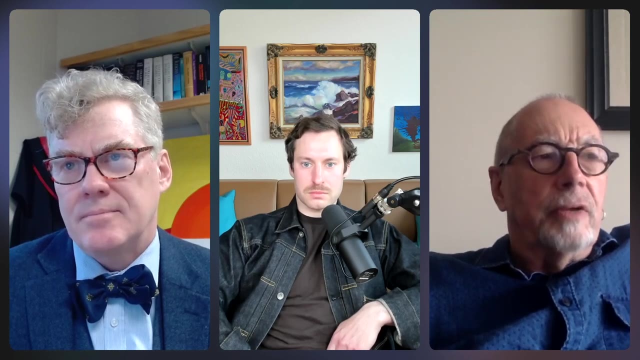 But I started to worry about the fact that we do seem to give certain arguments of a self-referential kind Which seem to break through any consistent axiomatic system. And I started to think that through, And that's when I started to think that an adequate foundation for mathematics should be paraconsistent. 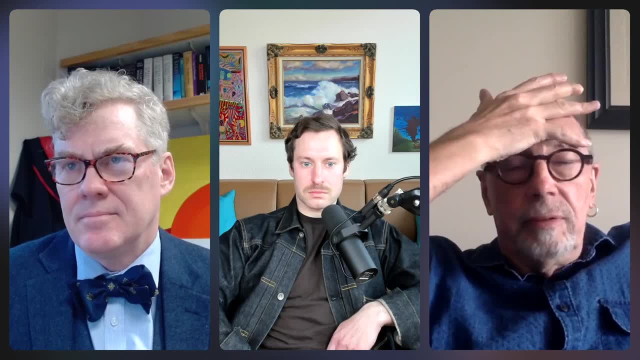 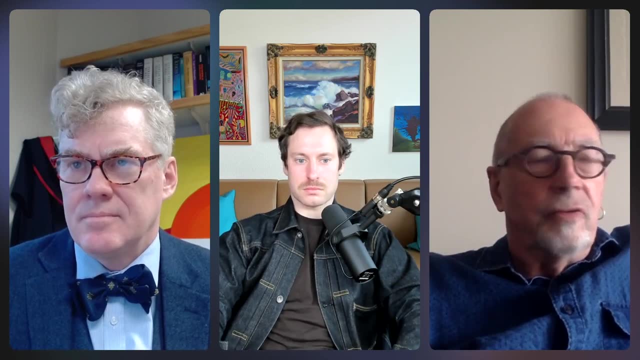 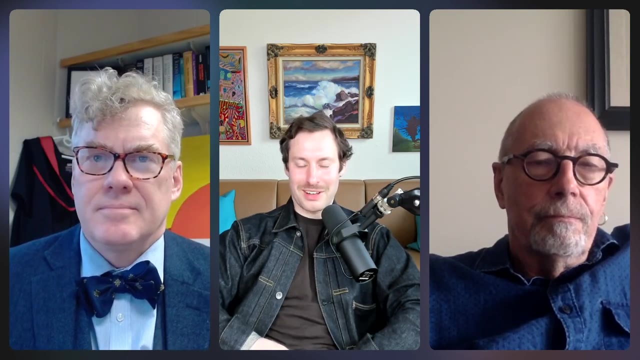 And then, of course, the connections between the original Gödel proof of his theorem And other self-referential constructions like the Lyre are obvious, And so that took me into the board of the main. So it was through mathematics that you came to the Lyre Paradox. 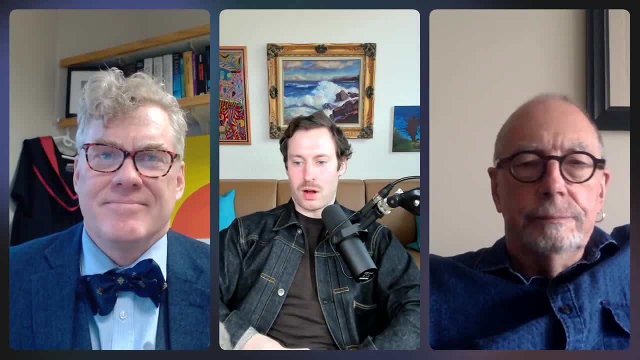 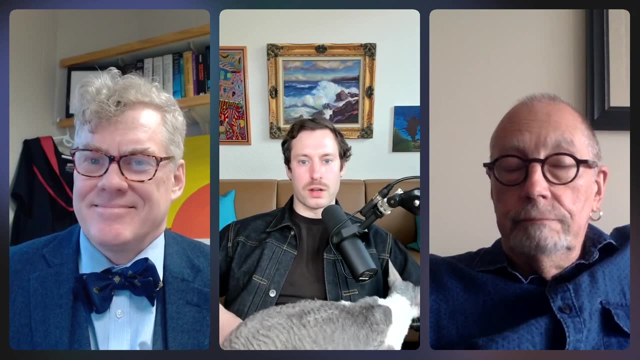 Yeah, it was through Gödel's theorems. Maybe you could walk us through. just to start off, for the audience members who aren't familiar with the Lyre Paradox just what it is. It has many forms, but let's just have one. 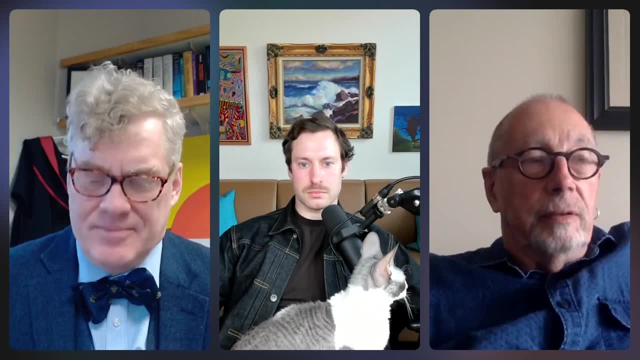 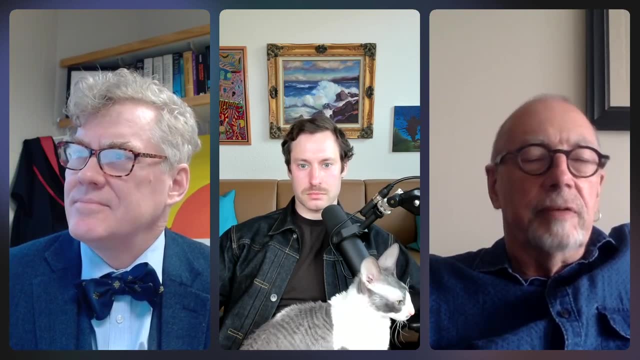 So the paradox goes like this. The paradox goes back, we think, to Eubulides, About two and a half thousand years, Who invented a number of paradoxes or discovered a number of paradoxes. One of these was the Lyre. 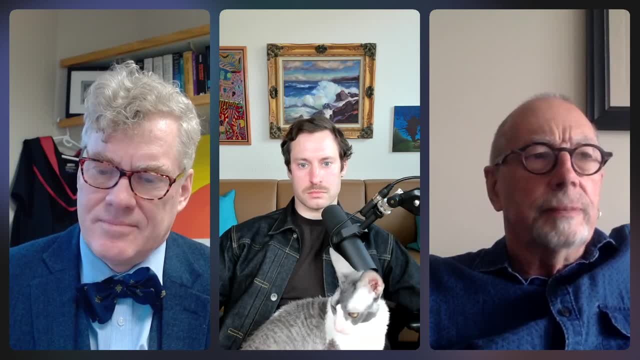 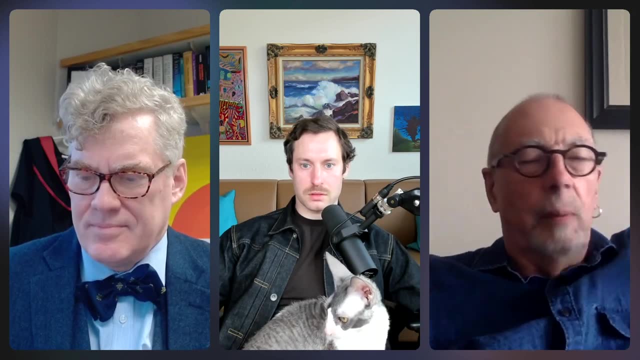 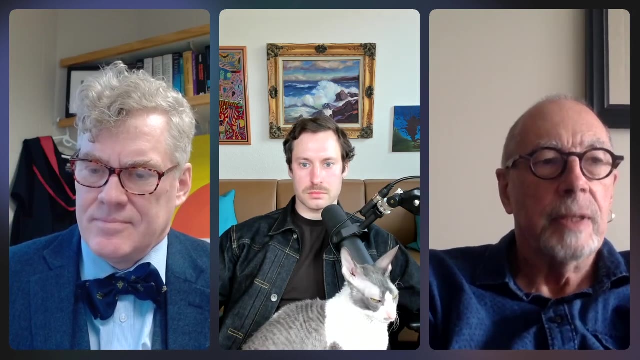 And as a modern logician would formulate it, it goes something like this: Consider a sentence which says of itself that it's not true. I mean, there's obviously some kind of self-reference there. You can arrange that many different ways, But let's suppose you've got a sentence. 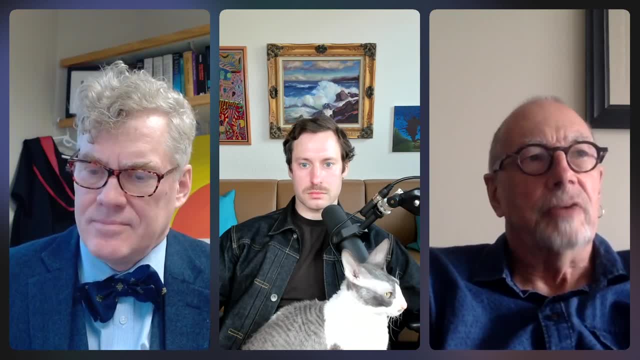 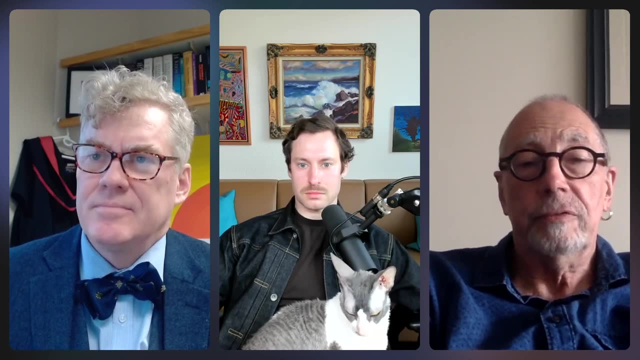 It says of itself that it's not true. Okay, then, prima facie, you reason like this: It's either true or it isn't. If it's true, well, what it says is the case, so it's not true. If it's not true, well that's what it says, so it's true. 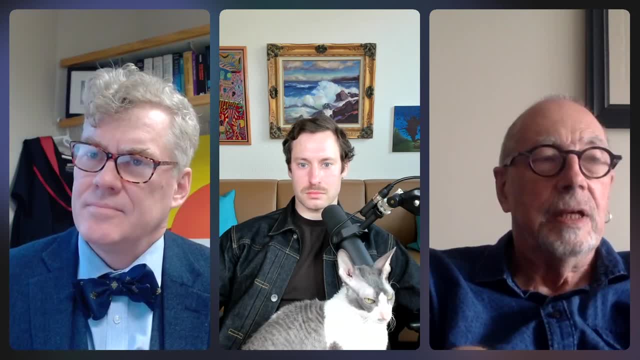 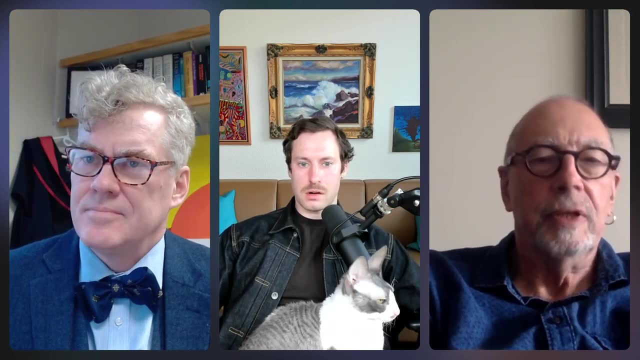 So if it's true, it isn't. If it isn't, it is. So you've got something very puzzling on your hands and there are a multitude of other principles. It's true and it isn't, So you've got a contradiction on your hands. 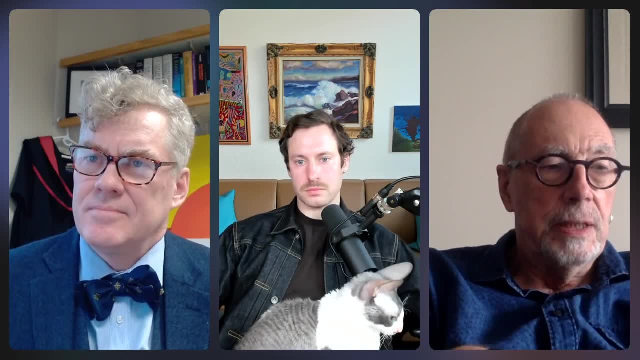 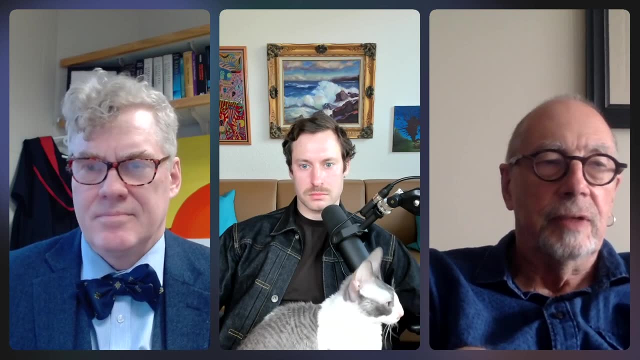 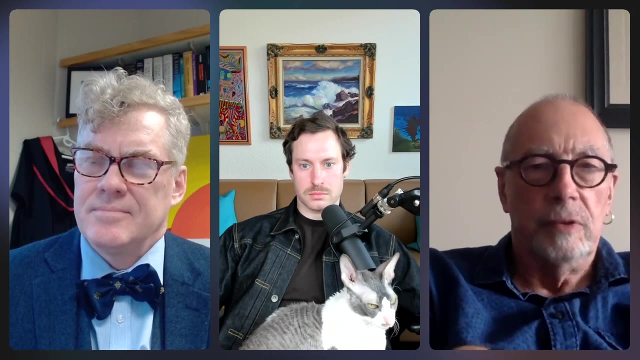 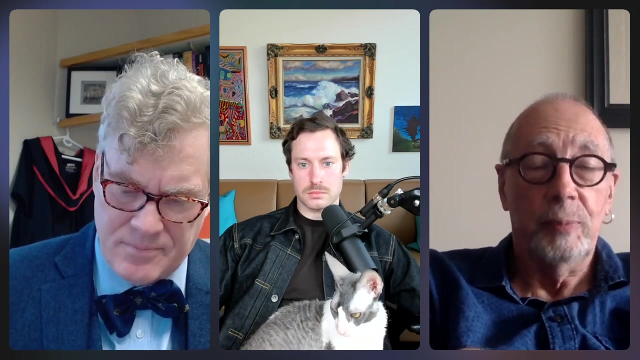 And the traditional response, by which I mean the response of most logicians until at least the second half of the 20th century, including the great medieval logicians, was there's something wrong with the argument, And the name of the game is to figure out what and, more importantly, why. 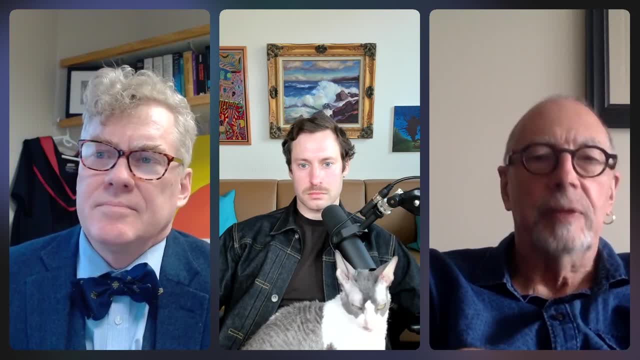 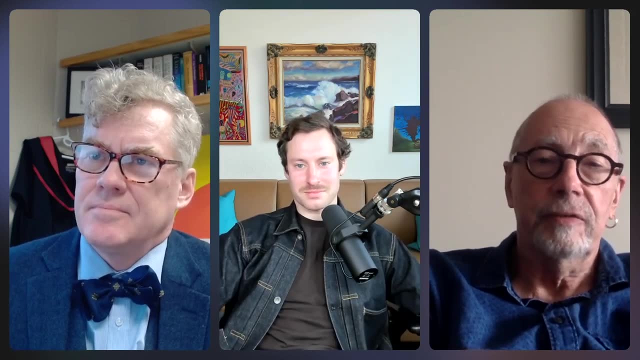 And this hasn't been terribly successful, it must be said. And this hasn't been terribly successful, it must be said, Certainly if consensus is a mark of success, because there still ain't one after two and a half thousand years. So the dialectic move is: well, hey, there's nothing wrong with the argument. 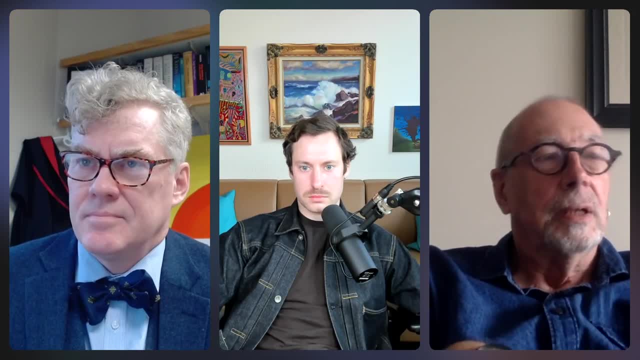 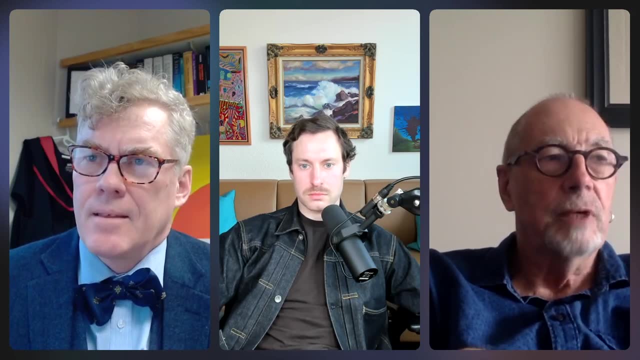 It's veridical, just to salvage its conclusion. Okay, that's only the start of an answer, though, because it means that you've got to have a central way of handling the contradictions, And that's really where most of the action is in this solution. 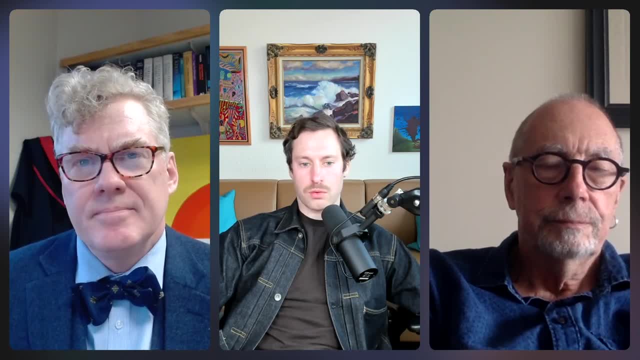 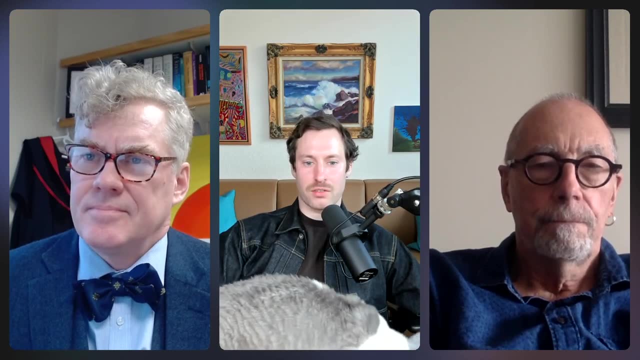 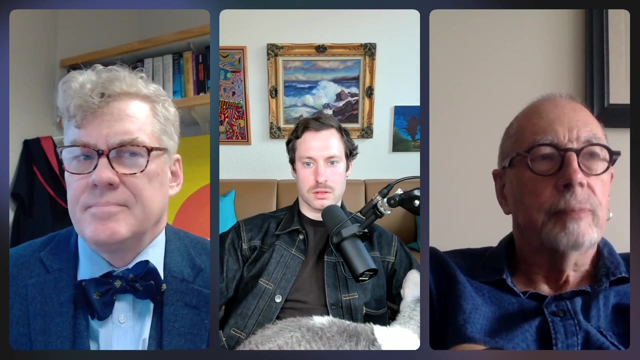 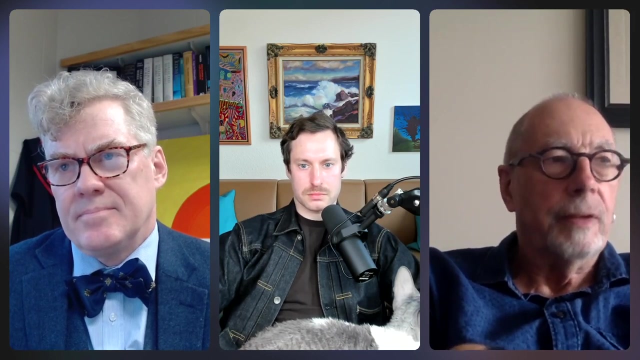 So how does Paris Consistent Logic help us solve the puzzle? And I mean, why does it strike you as the natural or correct way of dealing with it? Well, it's the natural or correct way of dealing with it, simply because you accept the argument at face value. 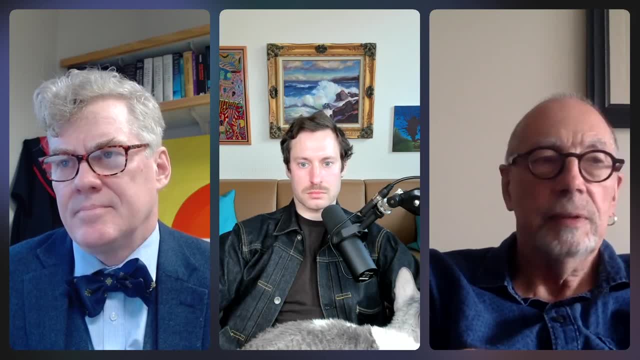 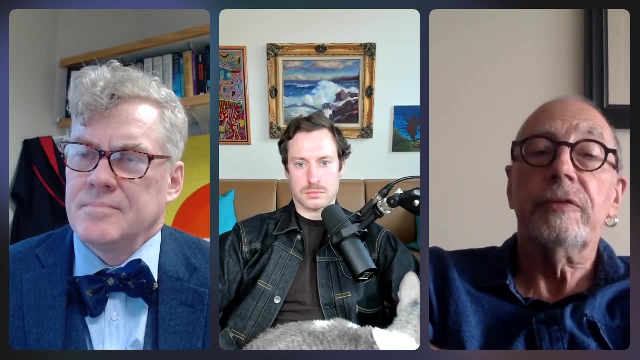 And that's not always the right thing to do. Right, And that's not always the right thing to do with an argument, But it often is. It's you know, to use some terminology from the philosophy of science, it saves the phenomena. 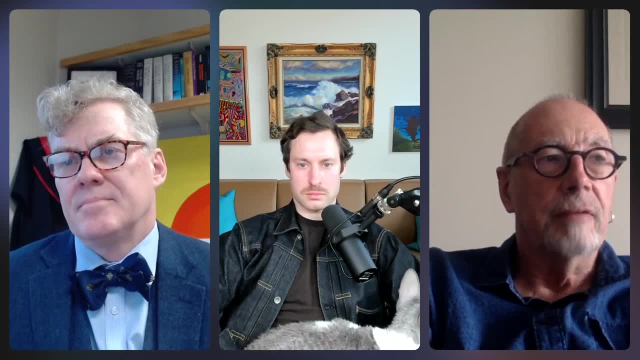 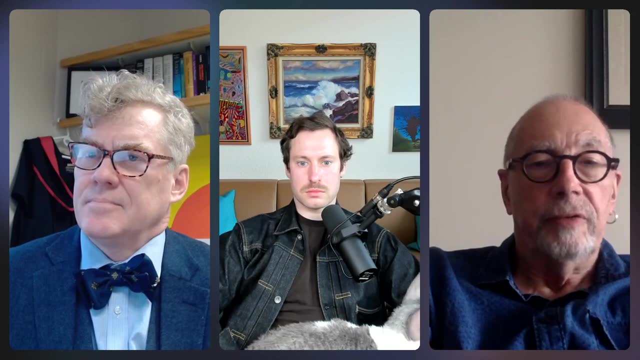 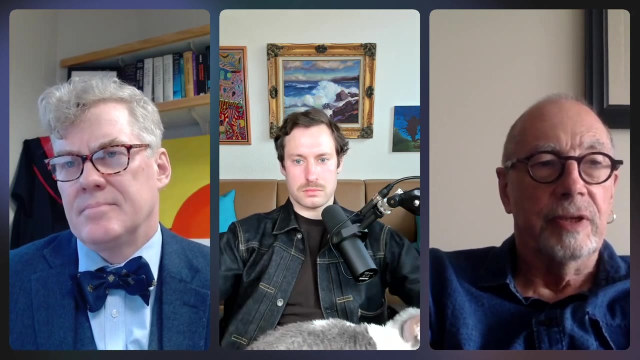 And that's backed up, in this case, by the fact that other approaches have failed for the last two thousand years. Okay, Why is a Paris Consistent Logic necessary? Well, because in so-called classical logic, that is the logic that was invented or discovered by Frege and Russell and company. 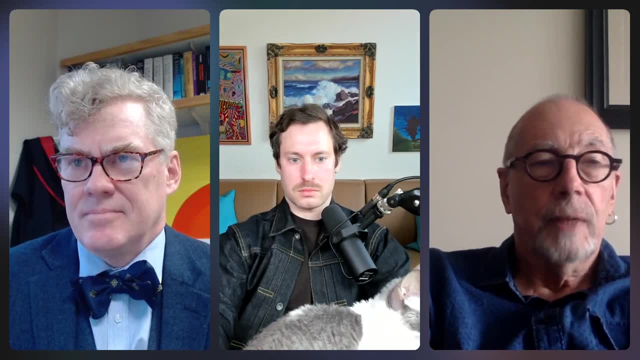 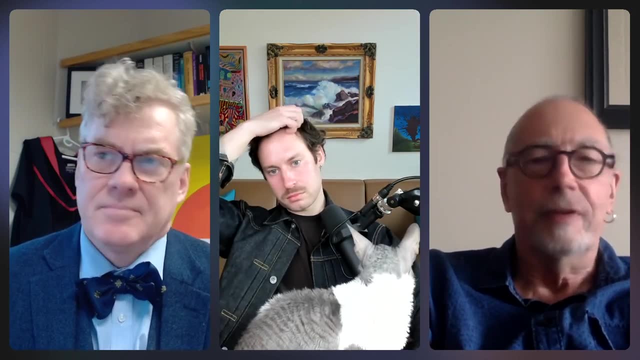 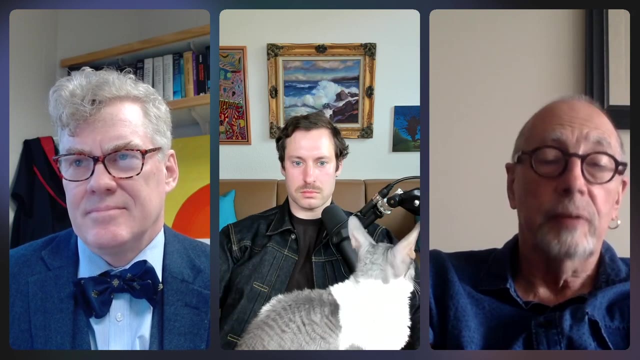 a contradiction will imply everything. So you might think that some contradictions are true, like the Lyre Paradox, but you'd be pretty crazy to think that every contradiction is true. So if you want to be a diluteist about the Lyre Paradox, you've got to reject that principle. 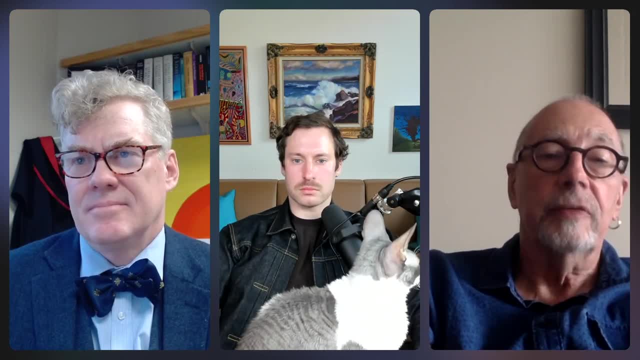 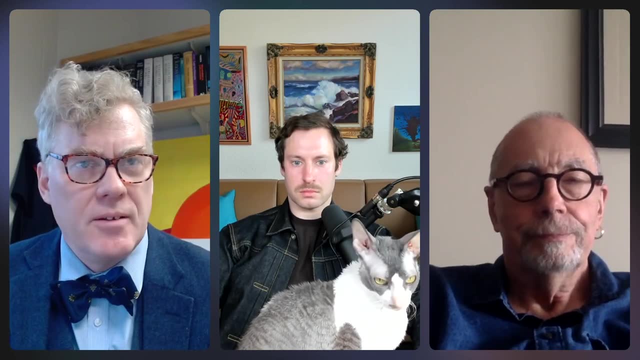 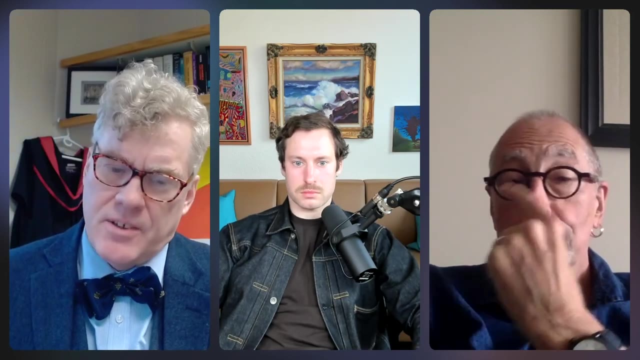 And then you're dealing with, by definition, a Paris Consistent Logic. So let me push against the earlier remark, Graham, that you made, which is that okay, I think I understand your point of view on this. I mean, and I remember when I was visiting at NYU and you and Hartree Field ran that seminar, 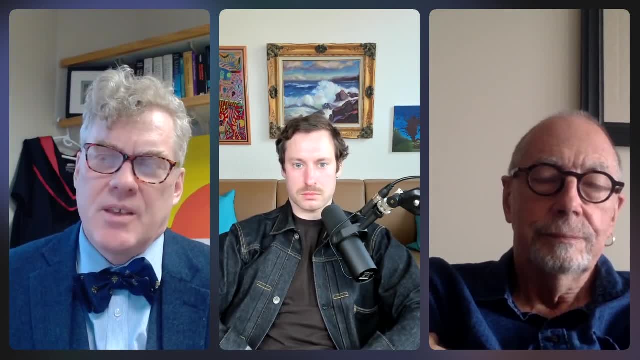 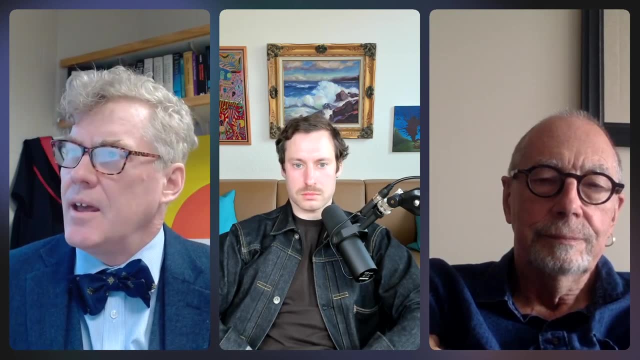 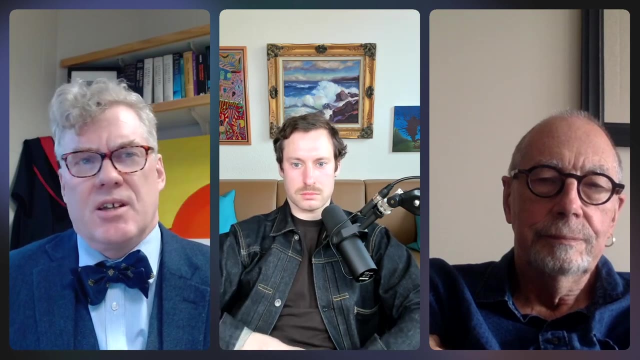 And it was a major theme of the seminar- was about changing the logic in light of the paradoxes arising with the Lyre, And the conclusion, as far as I understand your point of view, is that it was sort of for us to change the logic away from classical logic and to this Paris Consistent Logic. 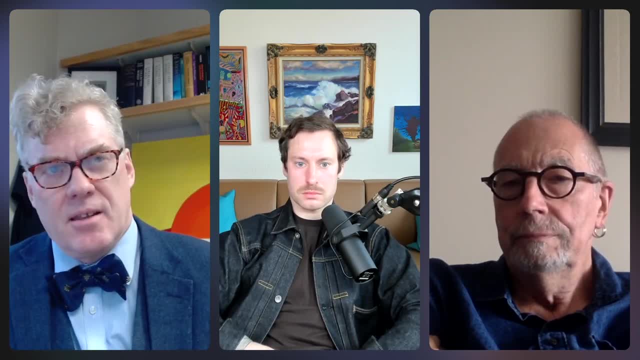 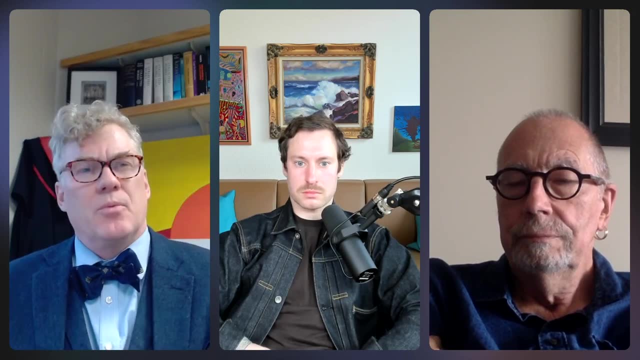 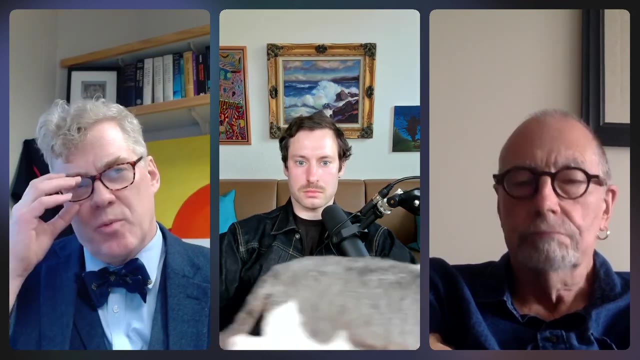 in order to explain and understand the phenomenon of the Lyre Paradox, And I'm completely amenable to that. But what I wonder is whether the solution has actually succeeded in helping us to understand the Lyre Paradox. I mean, what kind of resolution? 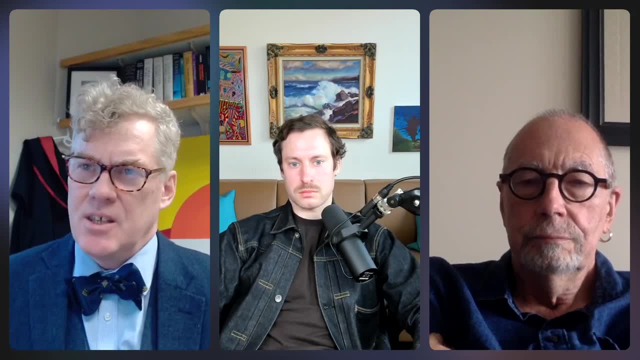 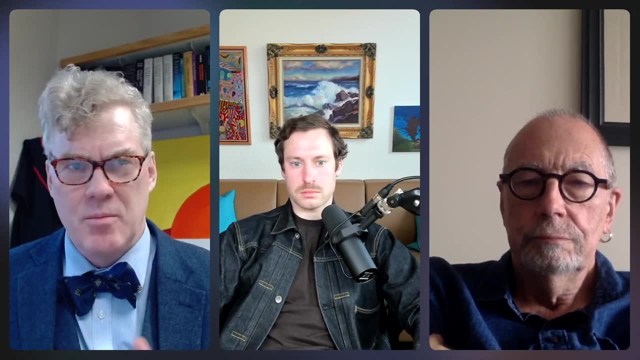 I mean, if one is confused about the Lyre Paradox, then the confusion seems to be based in the idea that, well, the sentence is true if, and only if, it's false. It can't be true, It can't be false. 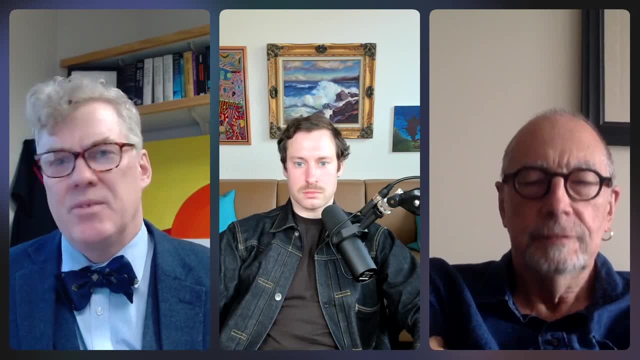 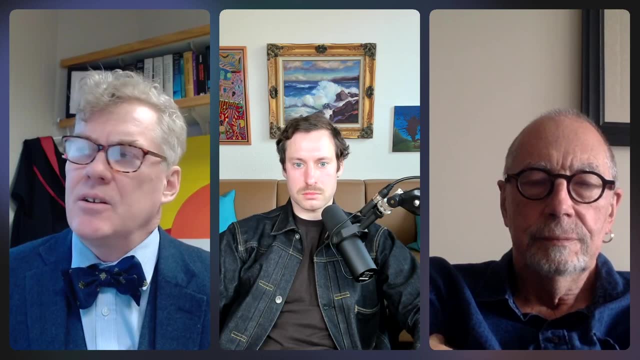 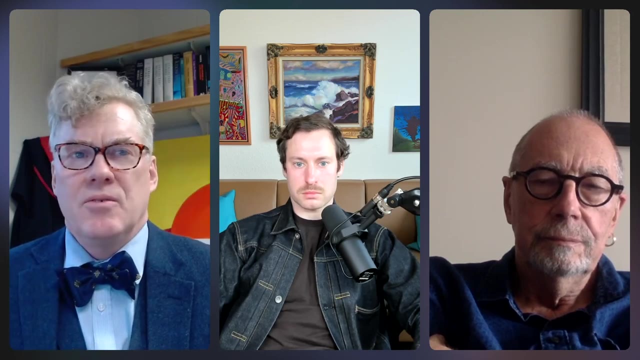 And so I think everyone, I think, is on board with the paradoxical nature of the Lyre sentence. And then to have a logic that just says, well, it's both true and false, How does it solve the paradox? I mean, it just is sort of drawing a line underneath the logic. 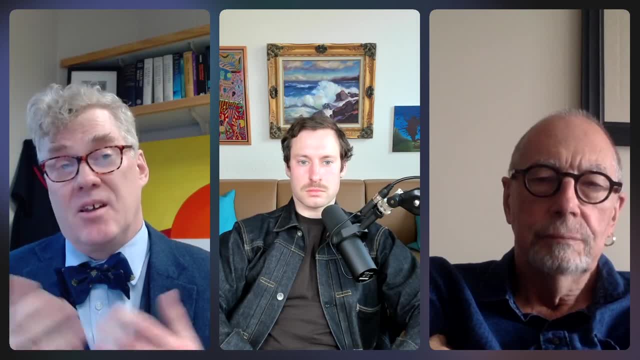 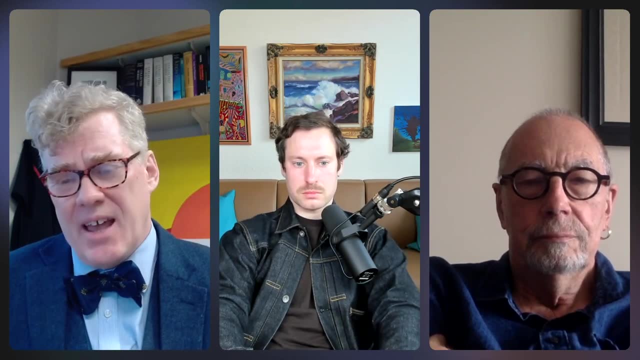 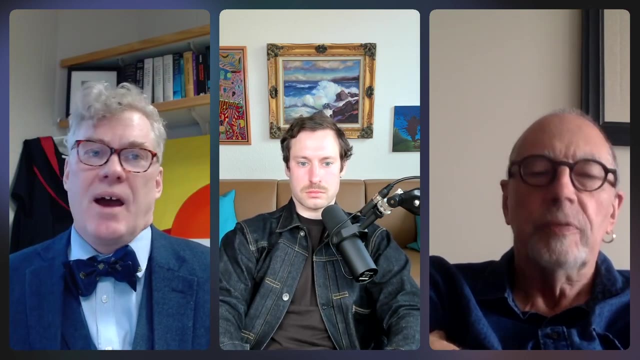 I mean, this is another way of looking at it which makes a lot of sense to me, which is that the Paris Consistent solution hasn't actually given us any explanation of how it could be that there are true contradictions. Rather, it's just kind of pointing it out that, OK, there are these contradictions. 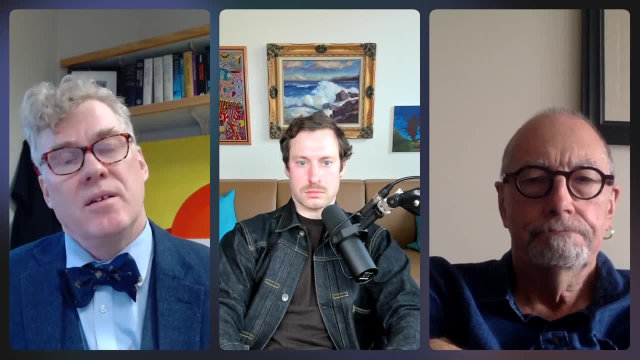 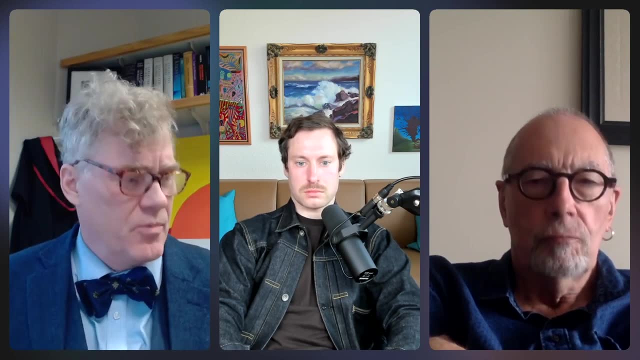 What do you want from an explanation? Well, I would want to come to understand what's. you know what? maybe there's some deeper phenomenon going on, or maybe there's some related phenomenon, or maybe there's some kind of conceptual error that's happening in forming the sentence. 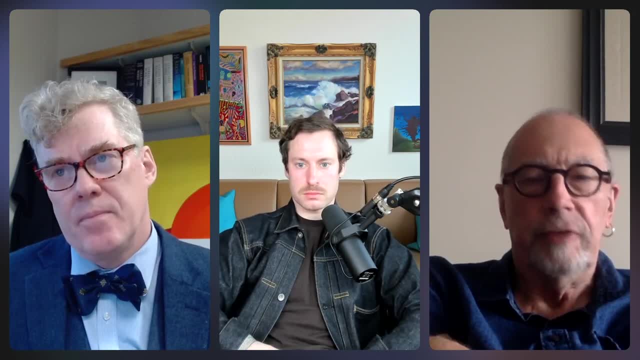 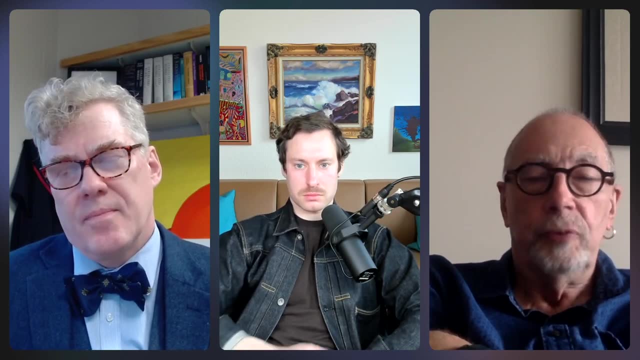 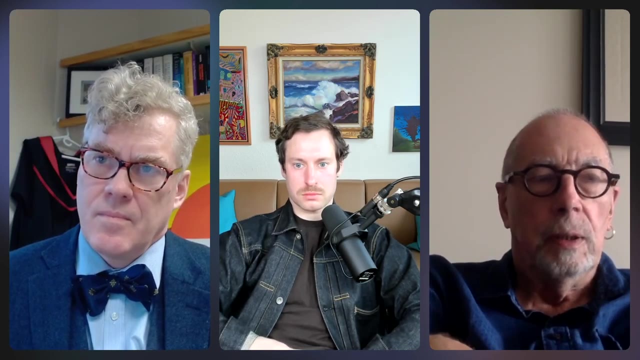 Yeah, I don't think there are any conceptual errors because the argument's critical, But I do think there's a deeper explanation, Namely what produces the paradox is this kind of structural mechanism we have for tearing through the boundaries, And once you see how we have these contradictions, 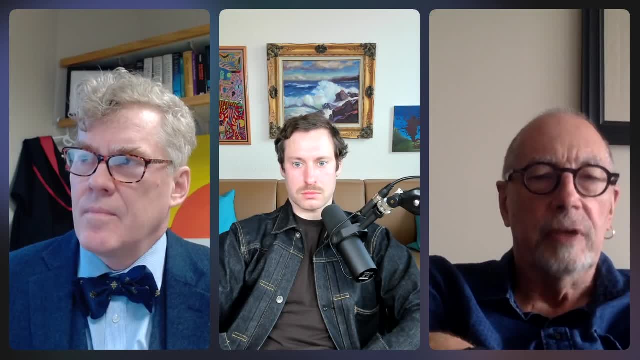 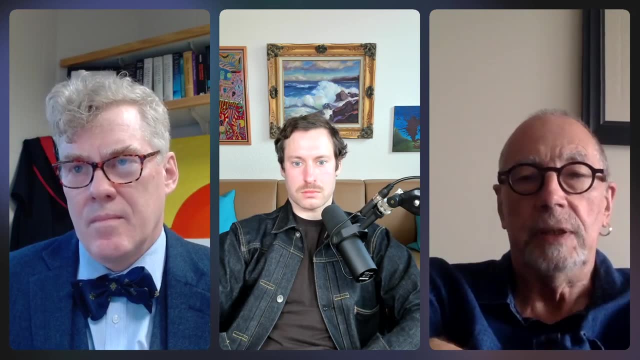 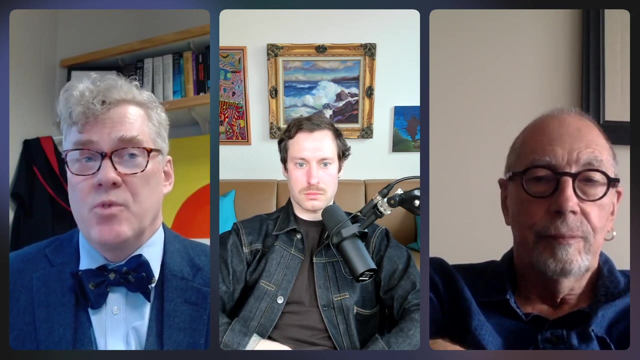 you're always going to get a paradox when you have an absolute boundary, a totality of all sets, totality of all truths, whatever Exactly. But I would say that there are sort of explanations of those phenomena, For example, I mean the sort of standard set, theoretic resolution of the general comprehension principle. 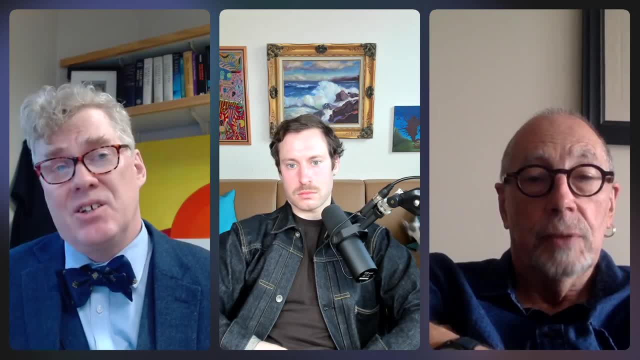 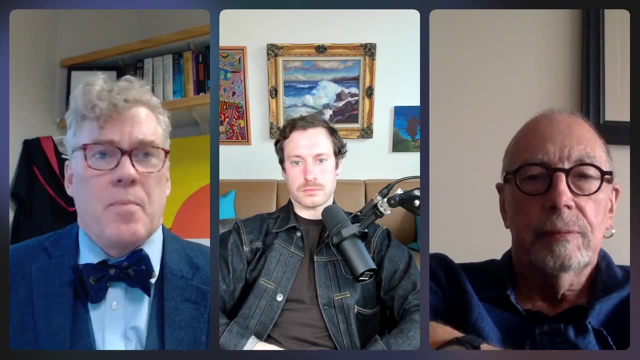 might take to be a kind of explanation of why the general comprehension principle is a logical error. I'm sorry, go ahead. No, no, no, I didn't want to cut you off. So I mean, for example, in the case of the liar sentence. 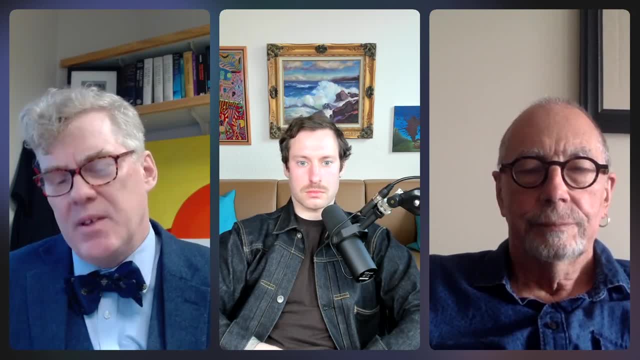 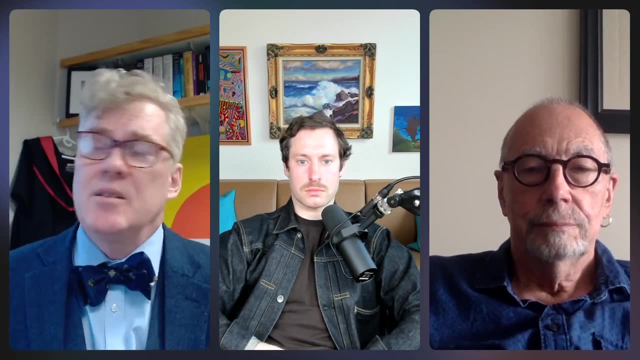 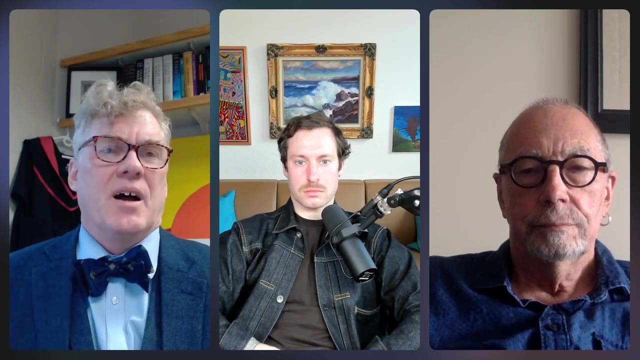 then the underlying commitments that are involved in formulating the liar sentence are about the nature of truth and the theory of truth, And you know what does it mean to make a statement? I mean to say that a statement is true, And it seems like we can say quite a lot about you know. 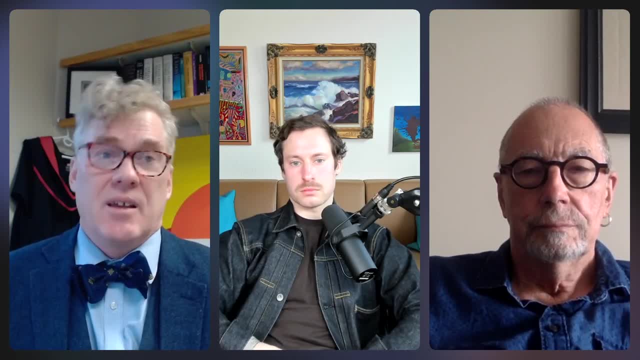 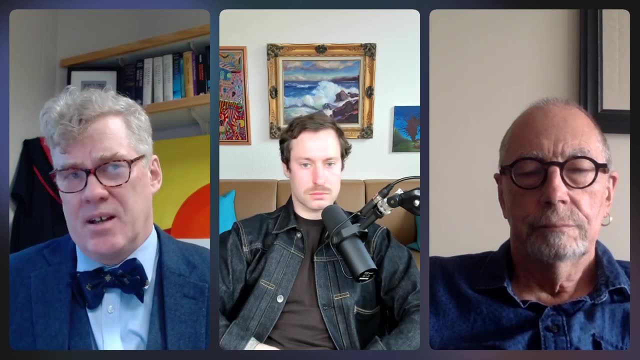 what we expect from a theory of truth or what it's like. Of course it would start not in this self-referential kind of self-applicable truth predicate, but rather in what I would view as a kind of much easier case where you have some kind of base language. 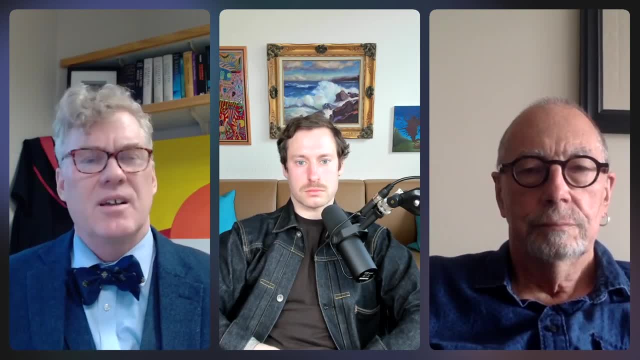 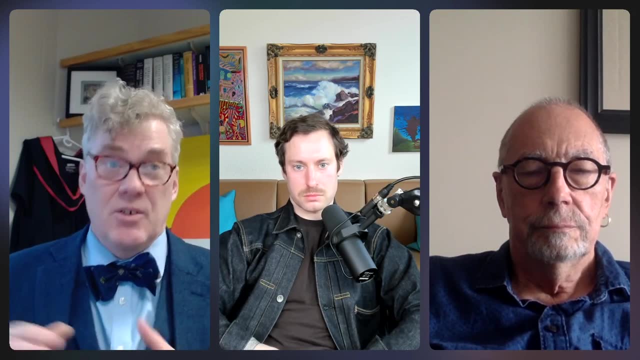 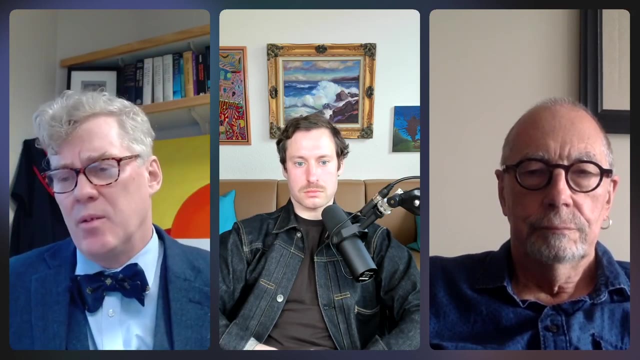 Maybe it's a formal language in mathematics, a first-order logic kind of language or something, And then you want to make truth assertions about assertions in that language. So it's not self-applicable, but only applying to the lower one, And this kind of case seems completely unproblematic. 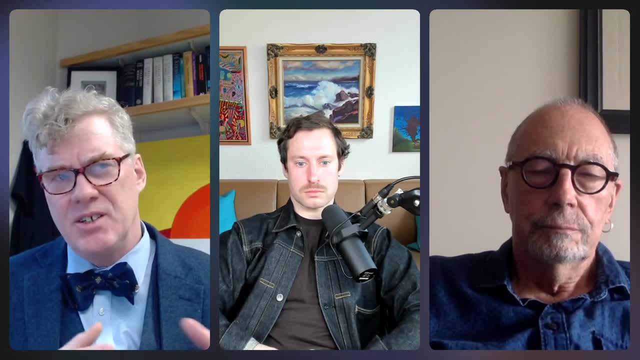 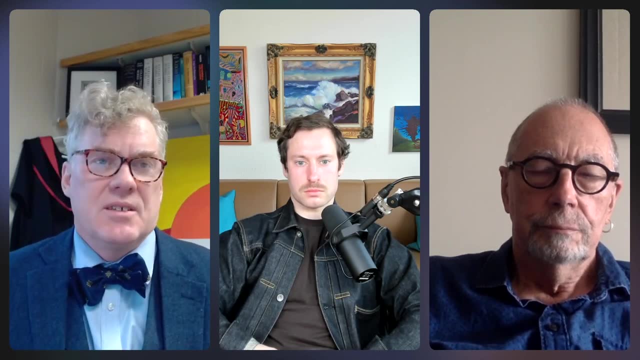 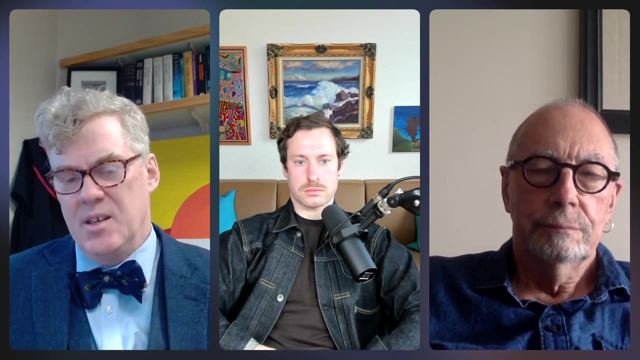 I mean, if I have, say, some kind of model or interpretation of this base language, then to say that phi is true is just to assert phi. I mean one can be completely deflationist about it and accept the T scheme in this way. 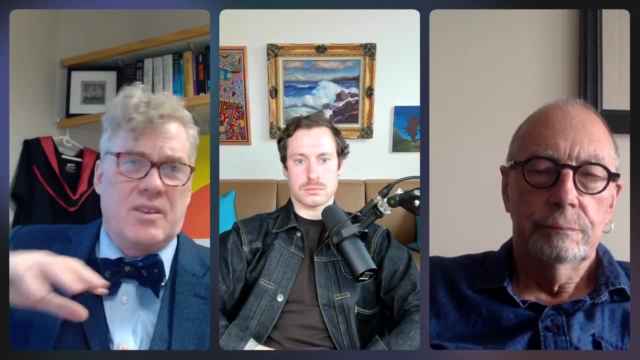 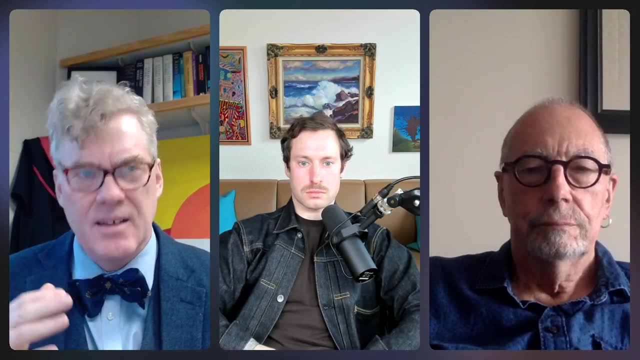 But of course we're only getting truth about the assertions that are sort of at a lower level for the base language. But you know you can iterate it, because once you introduce a truth predicate like that, then you can have another truth predicate for the truth assertions that you were just previously making. 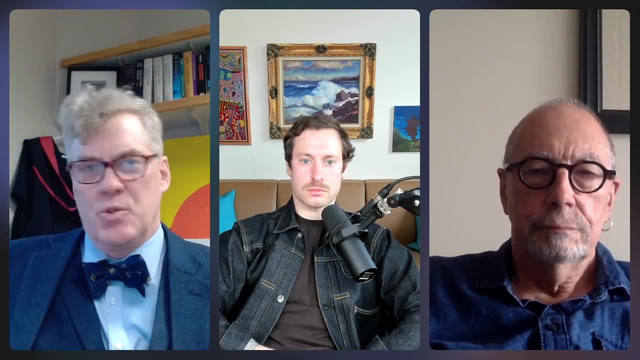 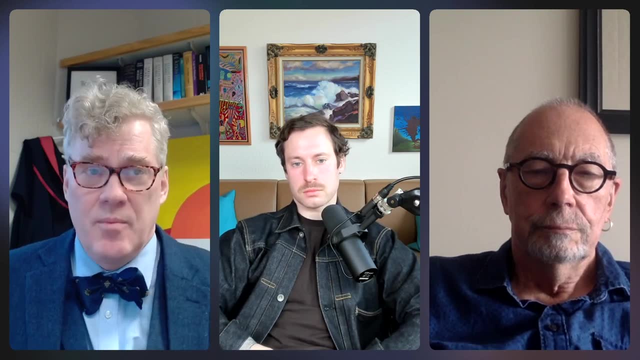 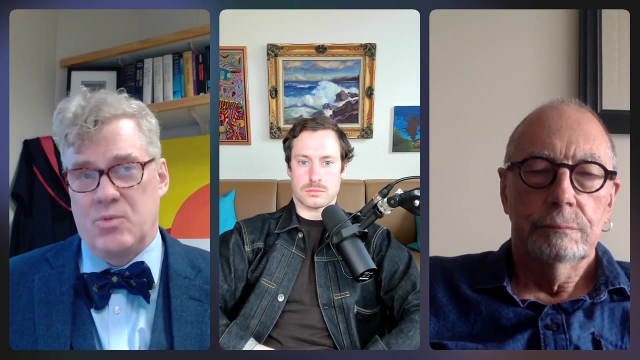 And so you're talking about truth, about truth, and then truth about truth, about truth, and so on, And of course there's a kind of transfinite iterative hierarchy of truth assertions to be made there. And that way of talking about the nature of truth and what it's like to have a truth predicate seems relatively unproblematic. 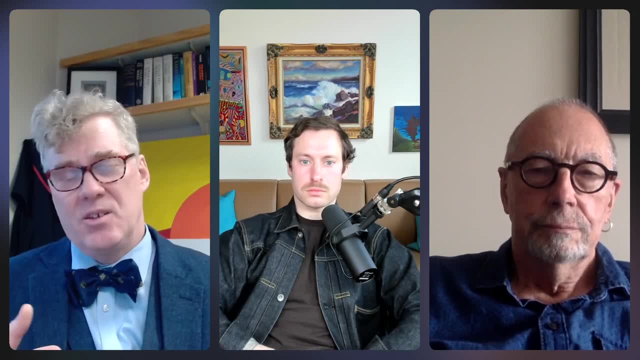 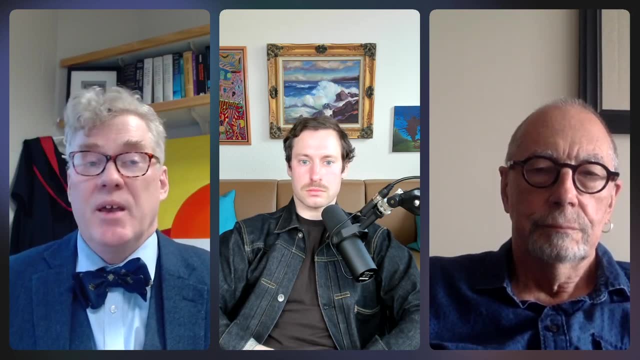 because one can just define any truth assertion by induction on the hierarchy itself, ultimately reducing down to assertions made in the base language. OK, but the liar sentence of course isn't like that, because it's not part of this well-founded hierarchy. 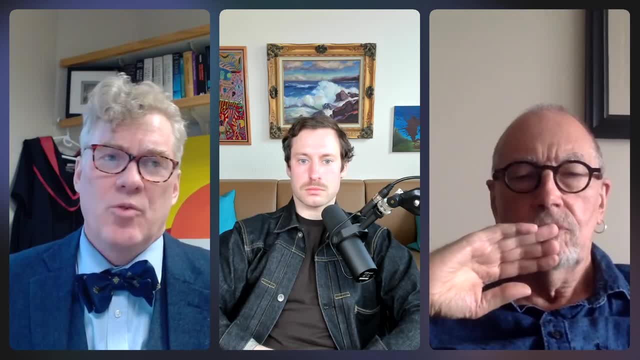 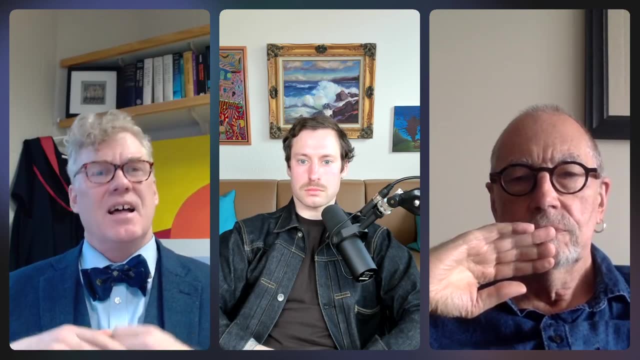 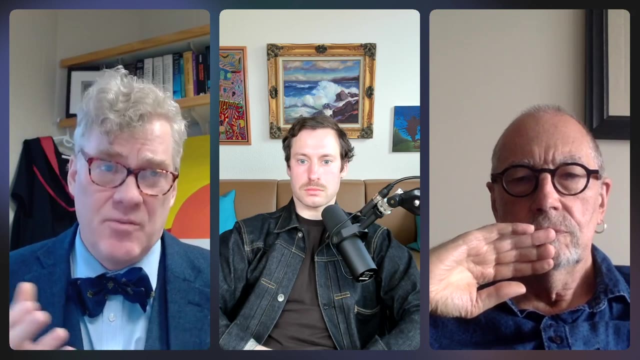 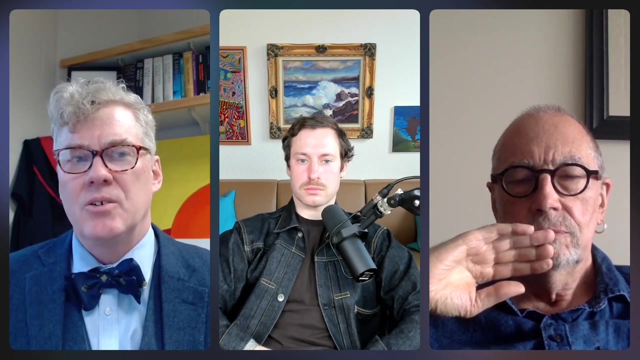 but it's having this kind of self-referential theme, And so it's not so clear to me what the concept of truth is. now. That is, this self-referential kind of truth. I understand very well truth assertions made when they're part of this sort of even very tall, well-founded hierarchy. 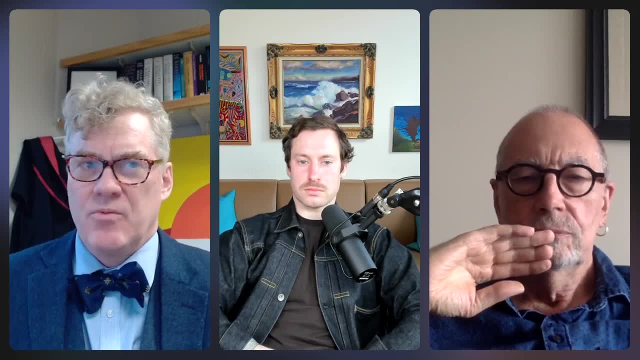 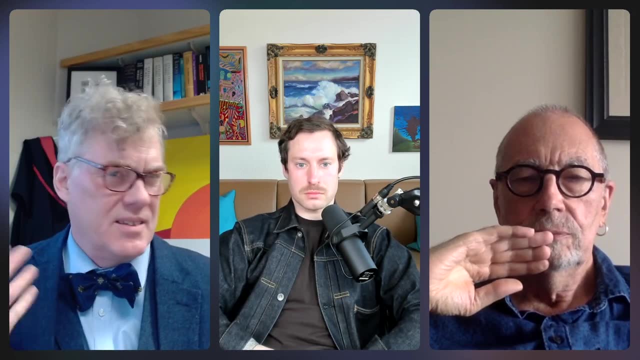 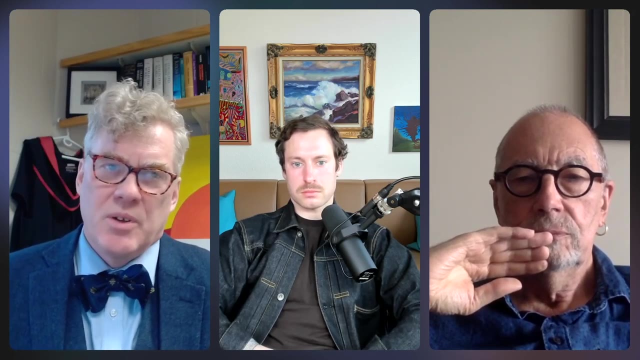 That's what I'm thinking of as my theory of what truth is like, And so I question whether the liar sentence is using a concept of truth that isn't like that, And it seems to be something very like the mistake of the general comprehension principle. 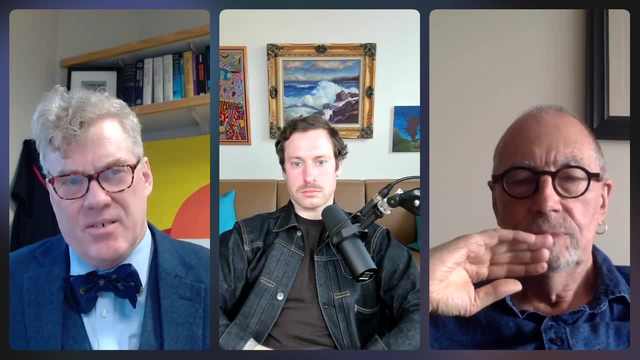 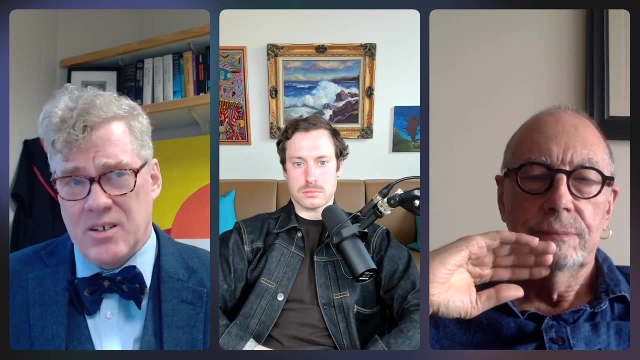 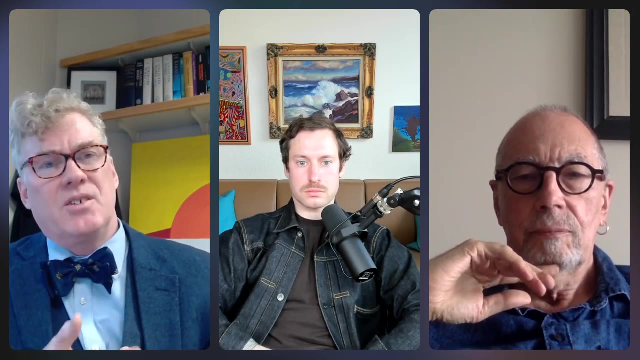 And in both cases they're so easily refuted in one line that it makes me think it's simply a kind of logical error informing the sentence in the first place. So this is the kind of explanation, that the kind of alternative explanation that isn't as radical as changing the underlying logic. 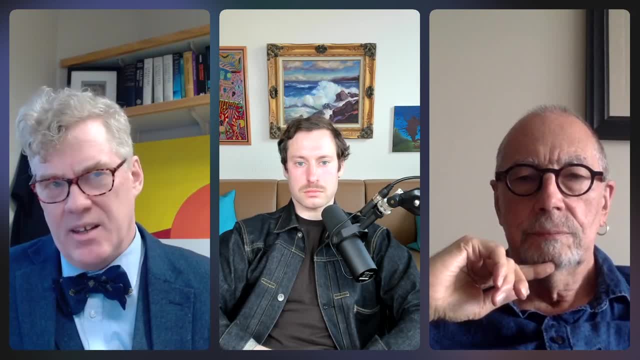 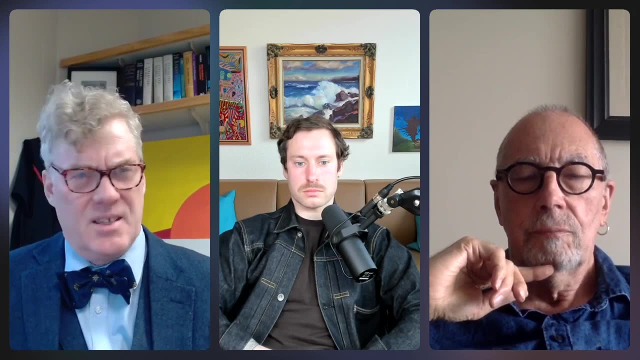 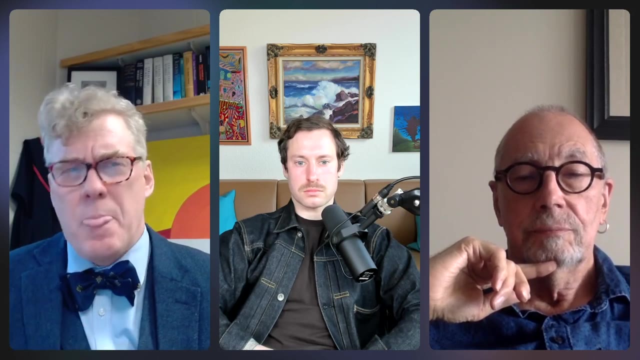 But it does seem to lead to some insight about the nature of truth. You can formulate the Tarski recursion and the discordational criteria and so on, And all of those things seem to be helping us to understand what the nature of truth is like in a way that the paraconsistent solution of the liar paradox doesn't seem to have those features. 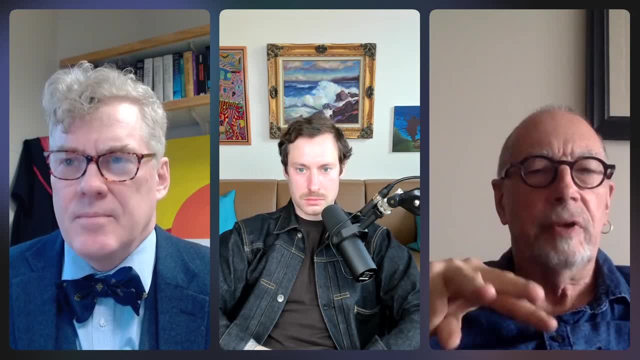 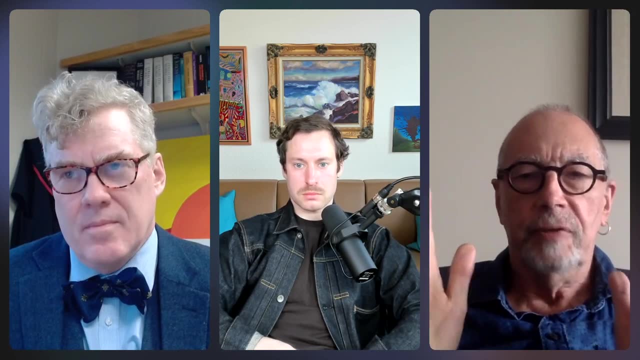 Okay. So there are lots of things there. Let me say three things by way of. The first is: we're now in the domain of different solutions to the liar Okay, And of course there are many, And each of those has to be addressed on its own. 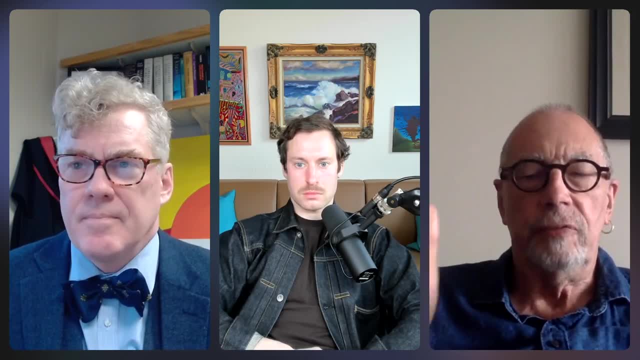 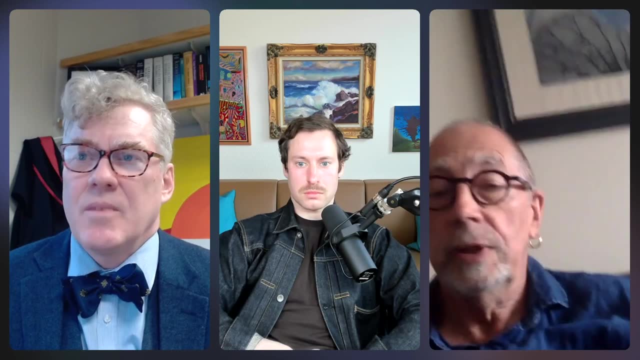 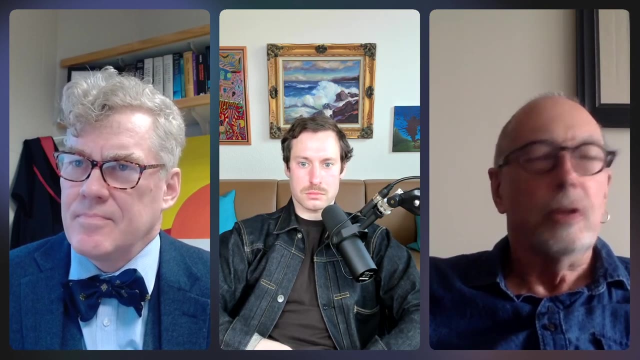 Okay, And we can discuss what you suggested if you want. I mean, I'm not sure how profitable it is to go out on that route over this medium, but we could do that. The second is that, of course, it's not in question that you can construct simple, consistent, formal languages. 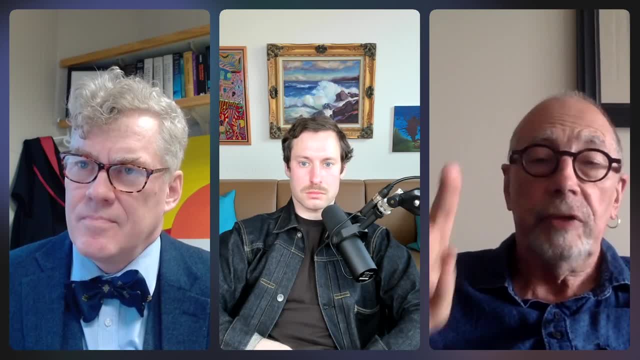 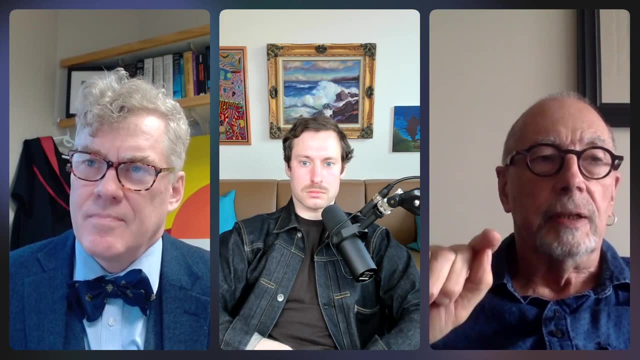 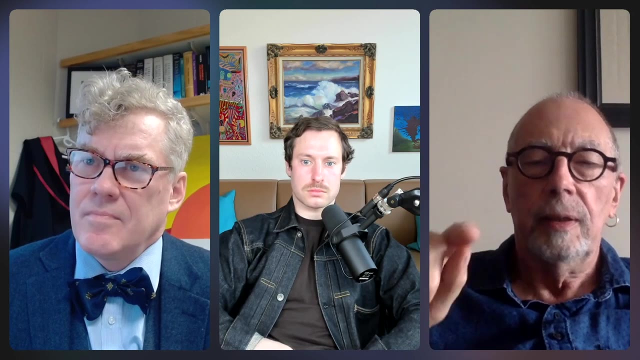 Of course you can, But the question is, as you said, what understanding it gives you of what's going on. Okay, Now the third thing is. The third thing is that you asked me what solution, what explanation comes out of the paraconsistent solution. 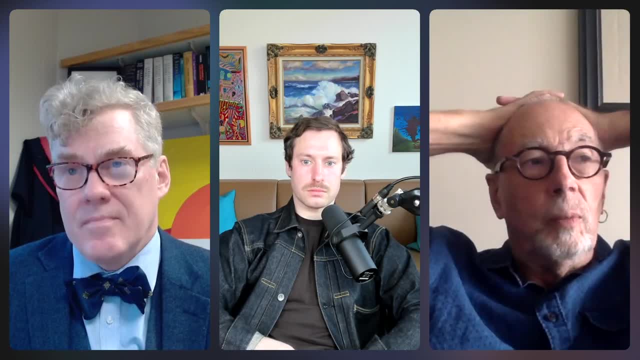 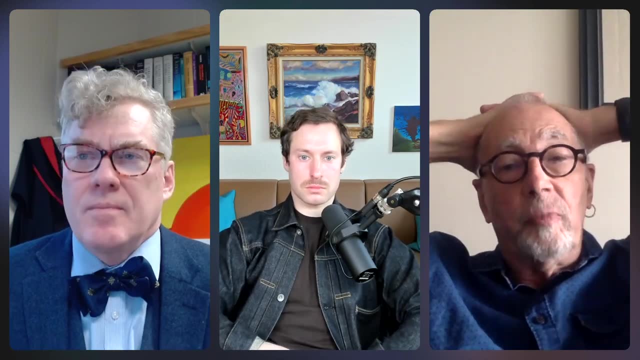 And I was sort of gesturing at a solution I've given elsewhere, which is to do with the enclosure schema. Say it again: Yeah, The enclosure schema, It's a mechanism for explaining why these paradoxes occur at boundary situations. Okay, 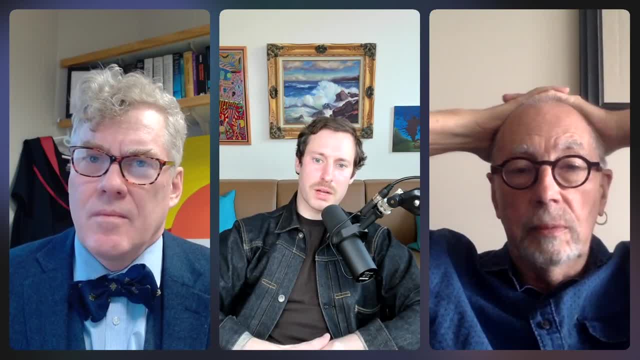 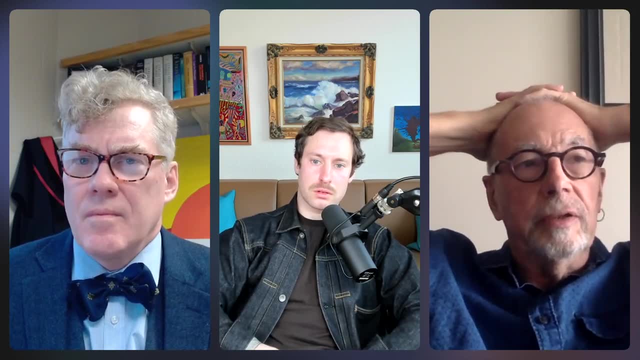 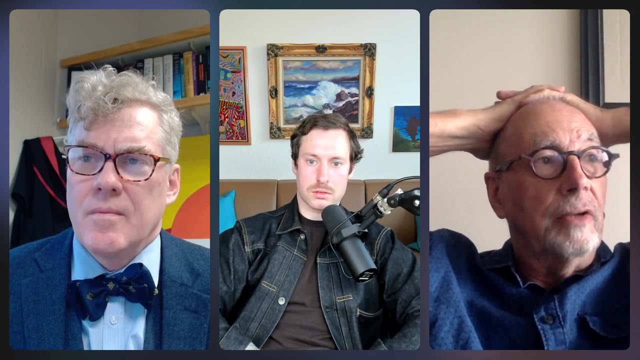 So that's where I would look to answer your question. Sorry, What do you mean by boundary situations? Well, in this context, what I intended was when you've got the totality of all truths, totality of all ordinals, totality of all countable ordinals, a totality of all sets, a totality of all categories, these sort of mega totalities. 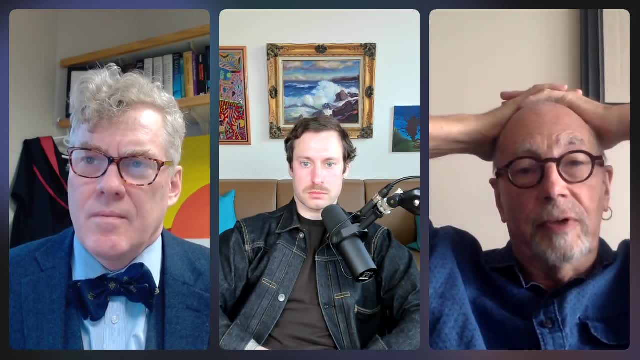 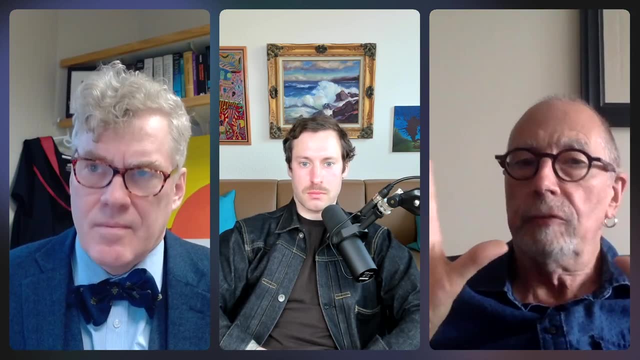 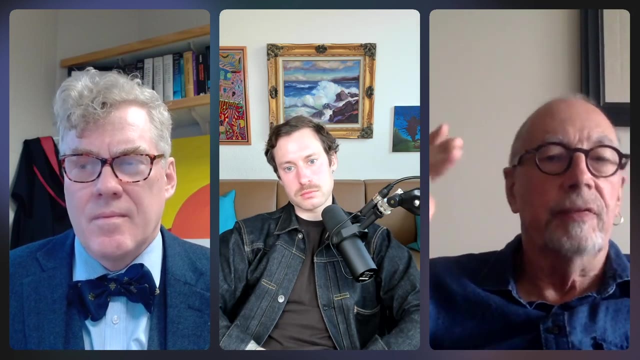 Well, the totality of all countable ordinals, of course, is not a mega totality, But whenever you've got a totality of this kind and a mechanism which does that And a mechanism which tears through boundaries, you're going to get this kind of a contradiction at the limit of the totality. 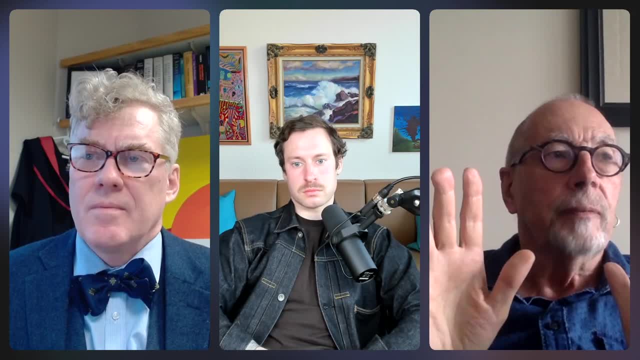 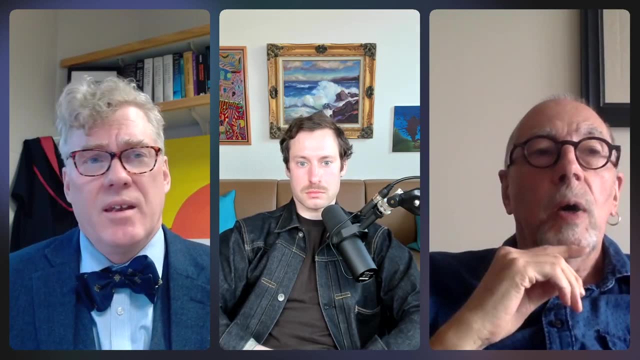 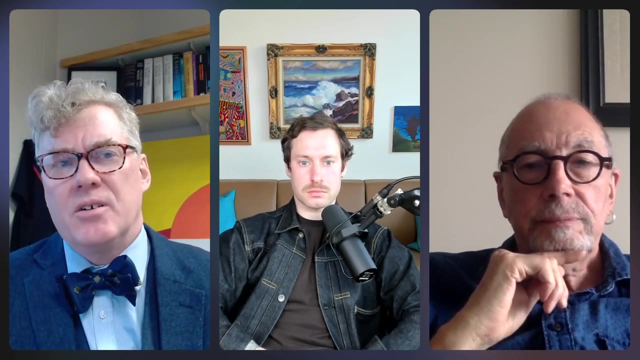 So that's what I had in mind. We can discuss that if you'd like. It's sort of what I was alluding to, actually, I mean, when I was referring to the analog of the general comprehension, which is, of course, about the totality of all sets and forming sets from that totality. 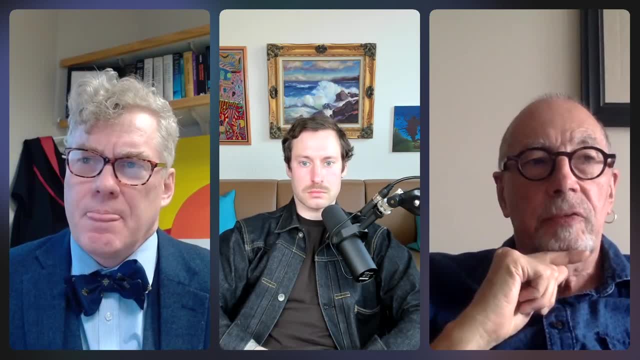 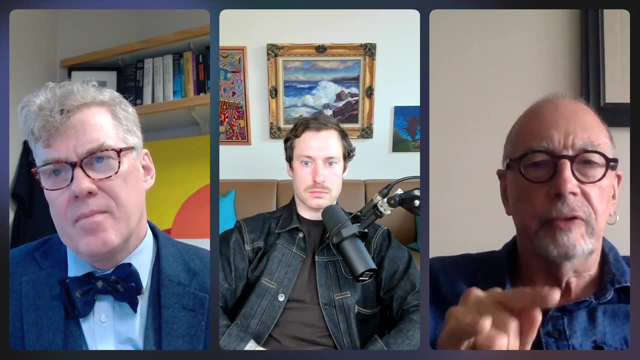 Yeah, Well, OK So, but I mean the solution that you. I mean, you said two things. The first is that the real solution is there's no totality, Right, But then earlier on you gestured at something else. 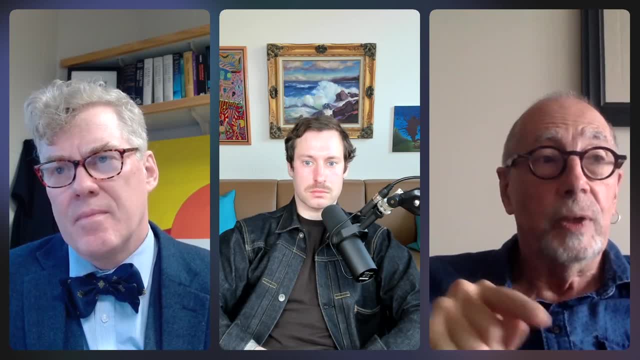 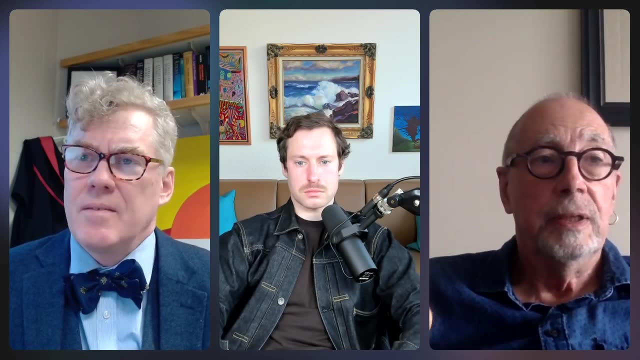 Namely, the notion of truth is vague and we have different ways of articulating it. Now, those two thoughts are different thoughts, And there's a question of which of those you might want to pin your colours to if we pursue this Right. 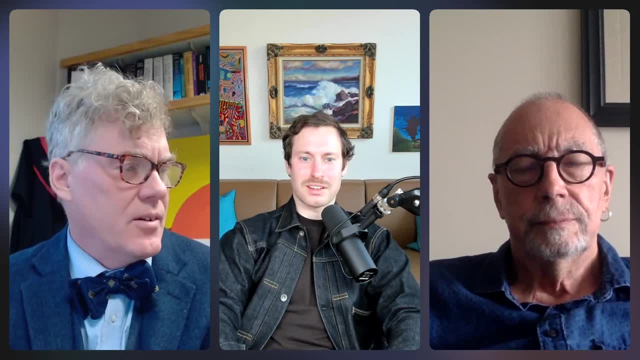 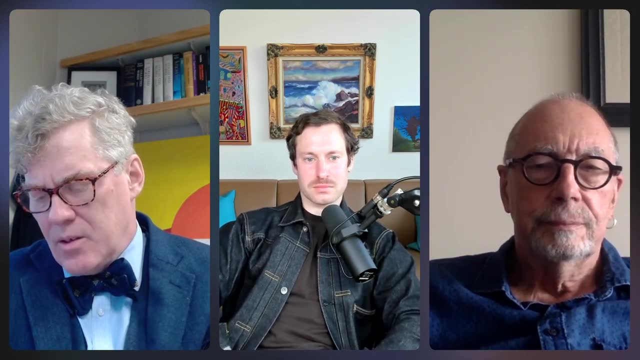 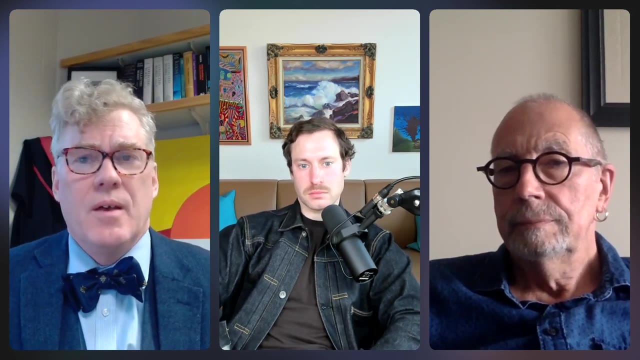 I don't know if I would say truth is vague rather. Yeah, I was curious about that. My view is something like One can try to be clear about. what does it mean to say that a statement phi is true And one way of understanding that? 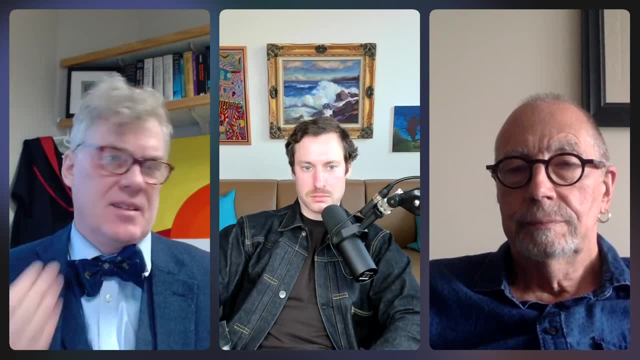 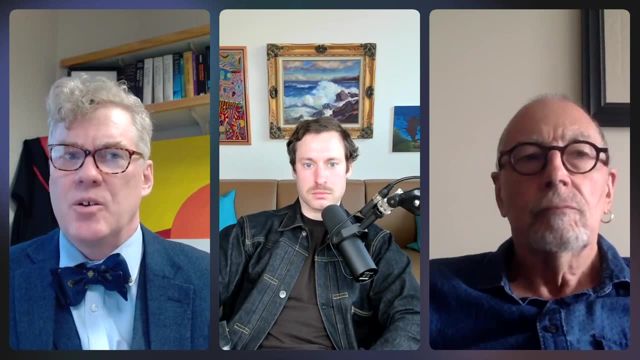 I mean, one can just take the t-scheme of t is, you know, phi is true, And this is the kind of logic that's underlying, I think, your analysis of the logic. Sure, But a different way You know. so maybe I don't know. 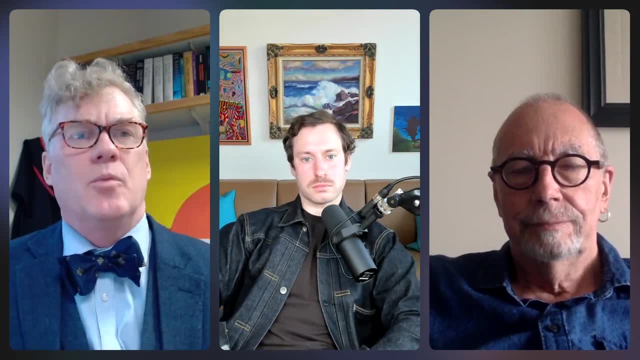 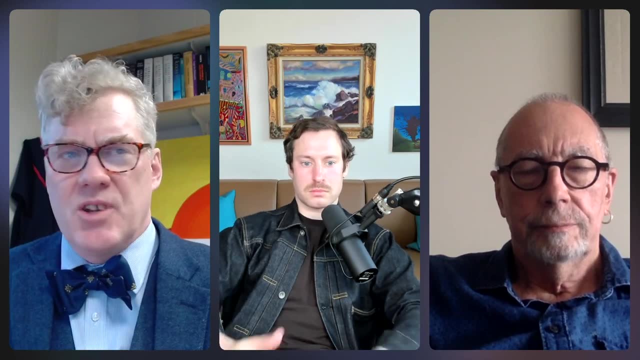 I mean, I would view that kind of interpretation is just completely deflationist, The t-scheme of t phi, if and only a phi. And whenever we make a truth assertion, whenever we say that an assertion is true, what we mean is that that assertion is the case. 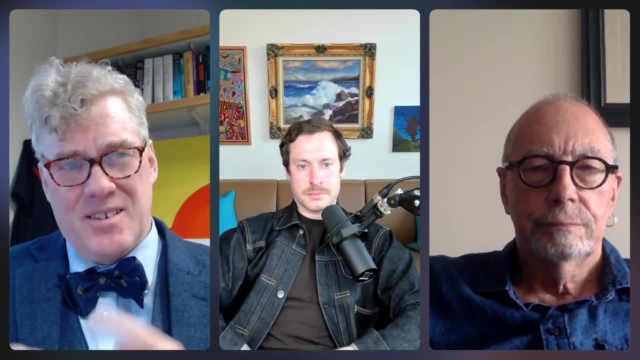 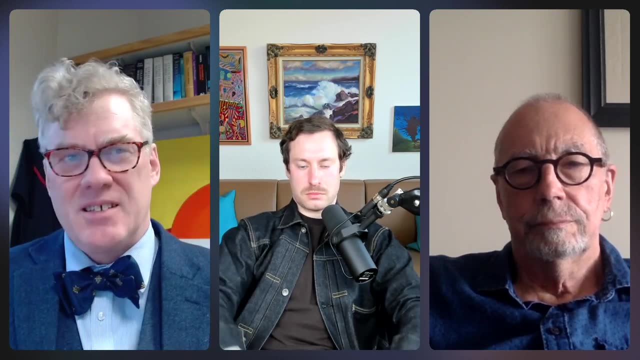 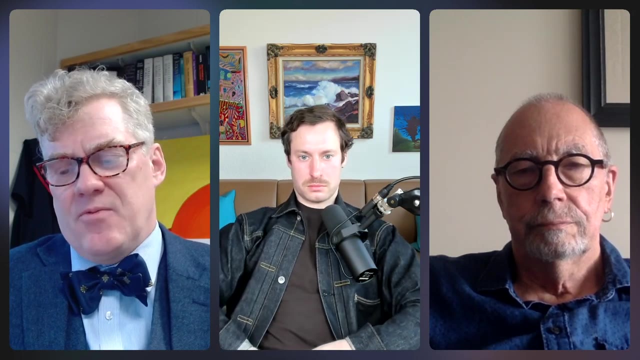 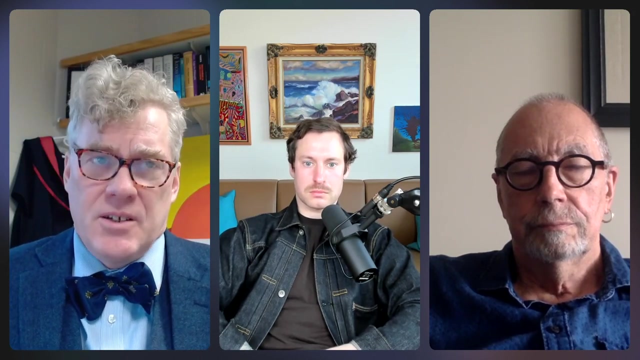 OK, but it's, it's. you know, the liar paradox somehow doesn't The liar sentence doesn't, It is. It is leading to contradiction precisely because of that scheme. Right? But another way I mean to understand what it means to have a truth assertion is to formulate what it means to have a theory of truth and to talk about things like the Tarski discotational schema and the recursive definition of truth. 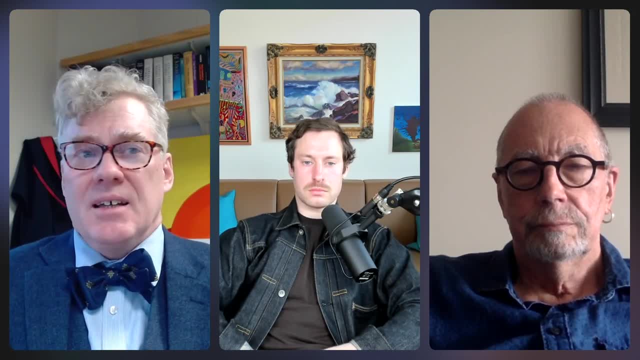 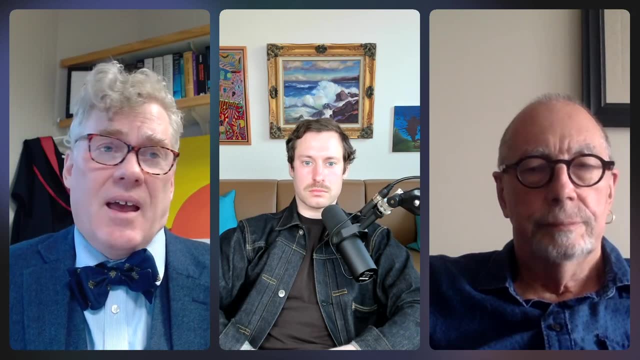 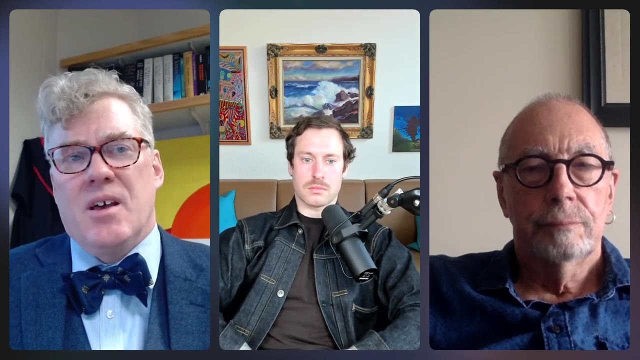 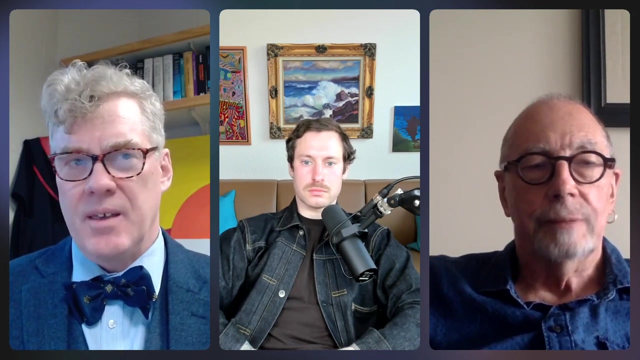 And that understanding of what truth is like is leading to this well-founded hierarchy that I was describing earlier. And and on that concept of truth, there just is no liar sentence. You can't. It's. it's kind of illusion that it's expressing a proposition because it's using this self applicable thing which this well-founded hierarchy doesn't allow. 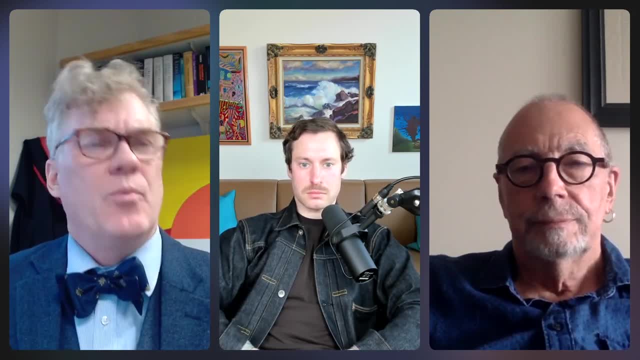 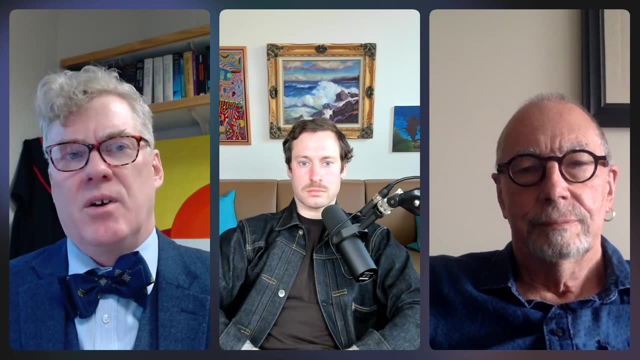 And so one hasn't. I mean, one can say, well, we have a pre reflective concept of truth or something and it's going to obey the T schema. And that's the kind of logic that one is doing when analyzing the liar paradox. 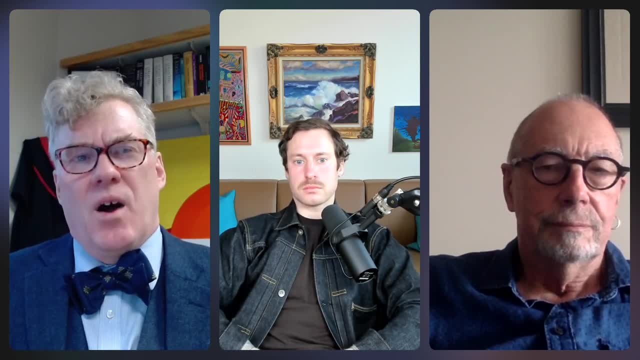 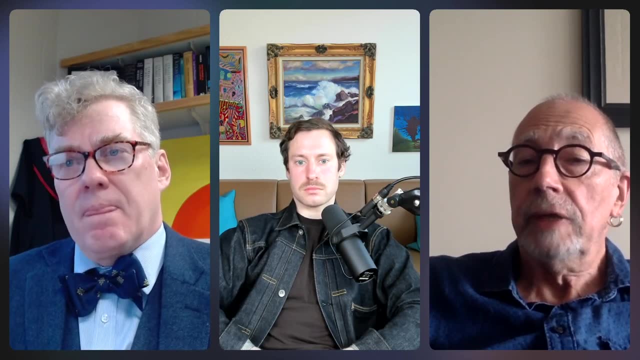 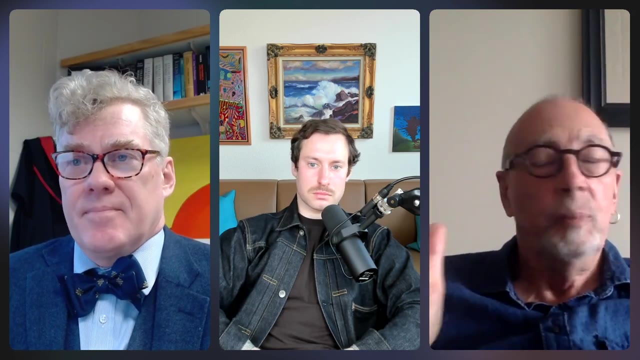 But I would want to have an explanation of what is that kind of truth like, And that's easy. I mean it's, it's a notion of truth that satisfies the T schema. Now that is endorsed, that that you could be a deflationist about that. 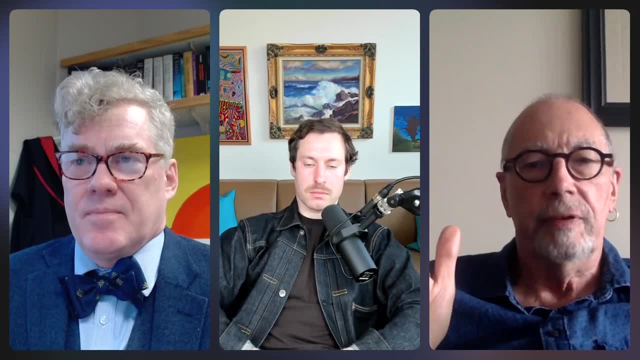 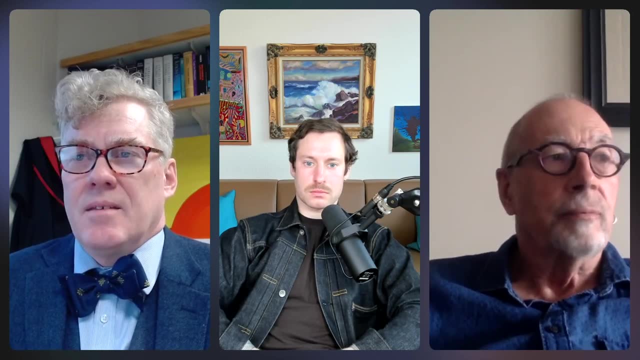 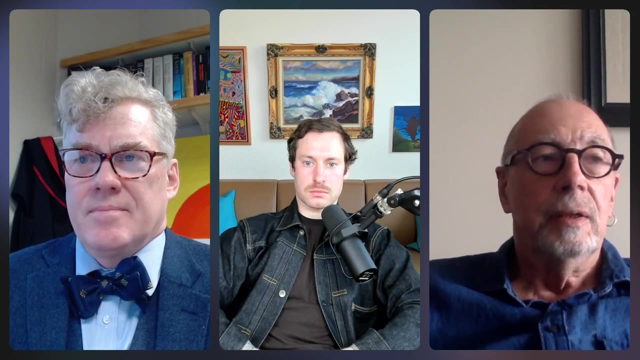 But of course you don't have to be. I mean, a lot of theories of truth will satisfy that condition in the details, as you like, I see. I mean, I mean that the T schema actually goes back to Aristotle. OK, and he's. he's certainly no deflationist about truth. 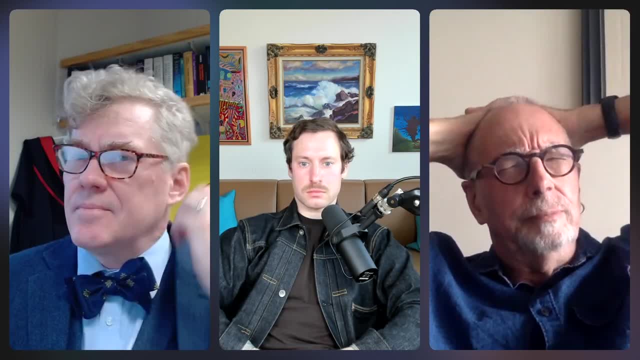 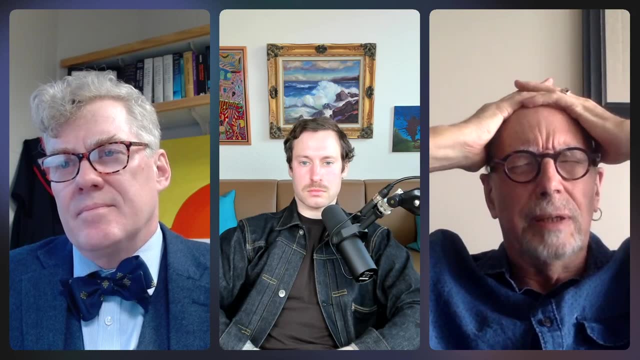 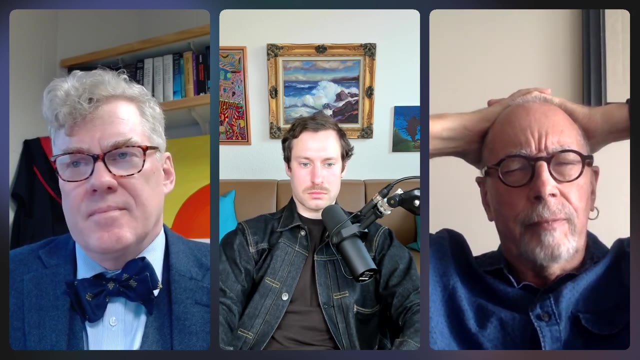 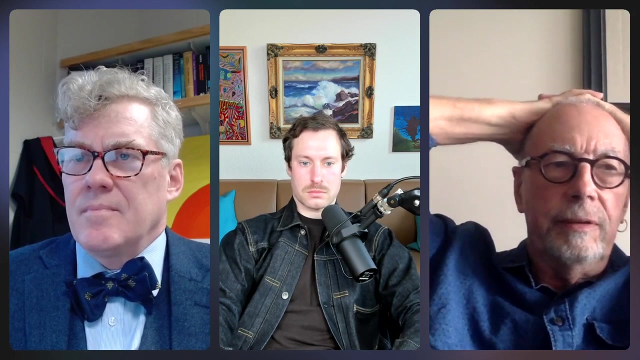 But, but anyway, I mean again. You seem to be to me now with two thoughts here. One is that There are different notions of truth And for some of the theory, some of the parents are going to rise and some it's not. 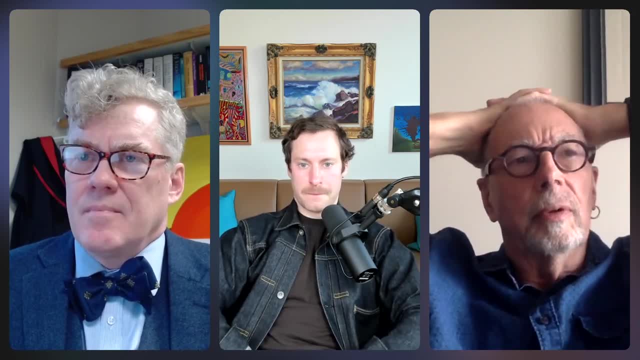 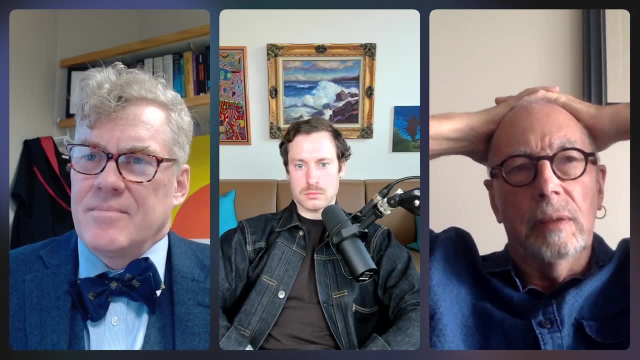 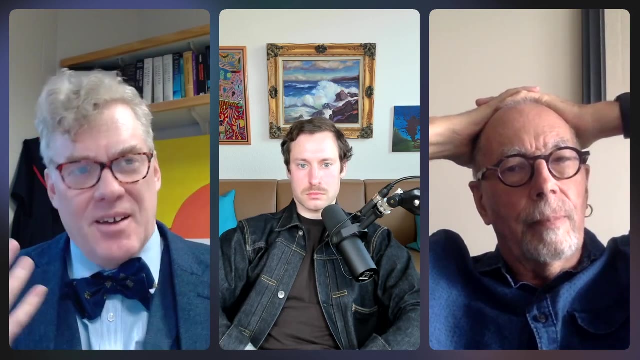 Not. that may be true, OK, but there's another thought, namely that there's no theory of truth according to which the T schema is correct. I mean, one could arguably take the liar paradox as a proof of that. I mean, of course you know, this is in classical logic. 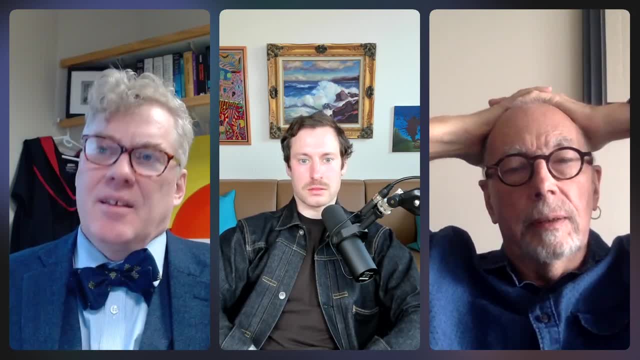 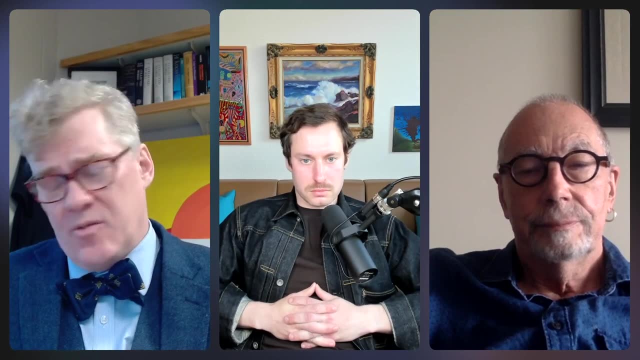 Basically, it's a reductio, right? Yeah Yeah. This is why I mean, if I'm understanding, your approach is that you want the T schema and the liar paradox therefore leads you to these two contradictions, just on its face. 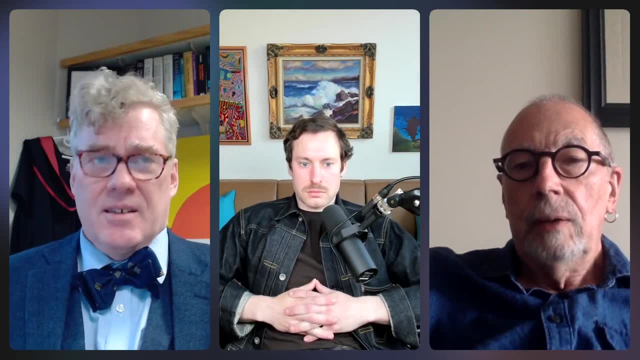 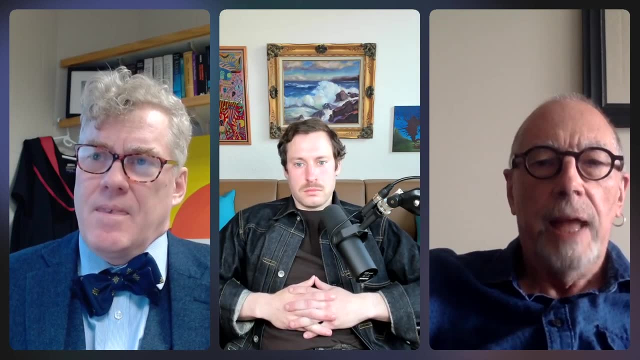 And this is why you have consistency, Is that? Yeah, Look, I mean, it's not just that I want it, I mean it's true, And anyone would endorse it, But were it not for the paradoxes, Right? 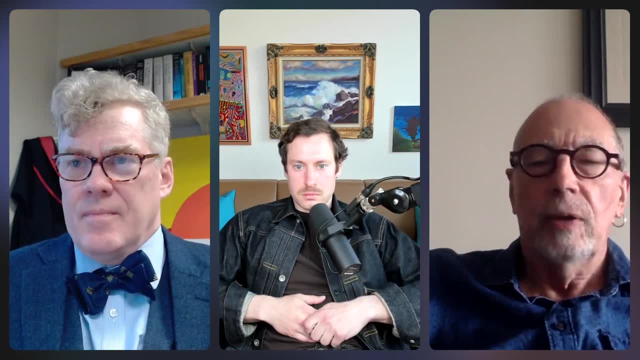 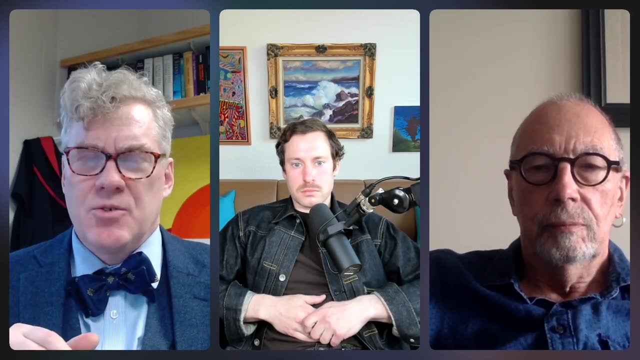 And everybody thinks it's true, Otherwise it wouldn't be a paradox. So when you say it's prima facie true, what do you mean? that the contradiction is true? No, the T schema. Oh, I see, Right, OK. 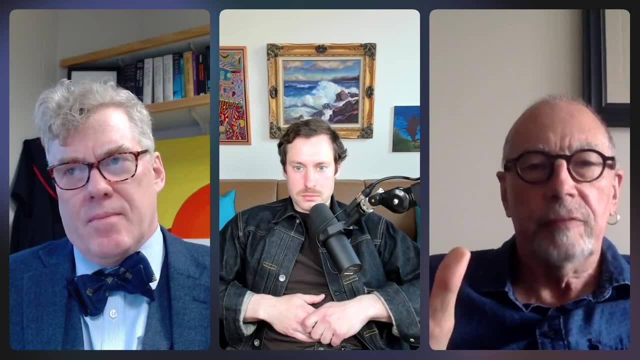 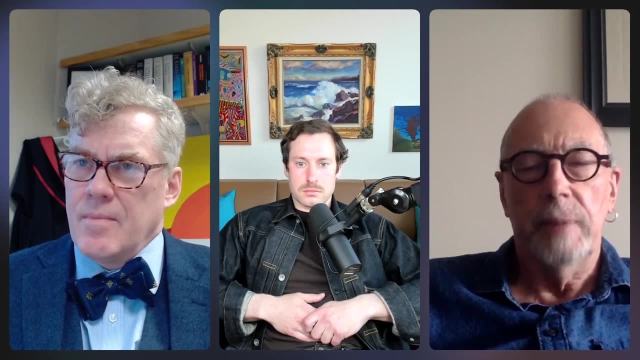 Now you can say that the appearances are not veridical. That's a very standard move, of course, But as you know, if you make that move, then there are other paradoxes that lurk in the wings. I mean, you said that it doesn't express a proposition or it's not worth it. 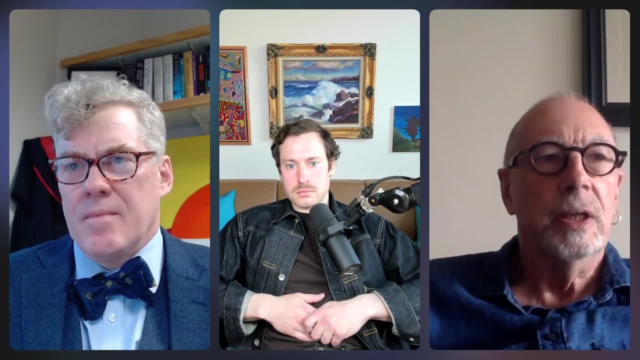 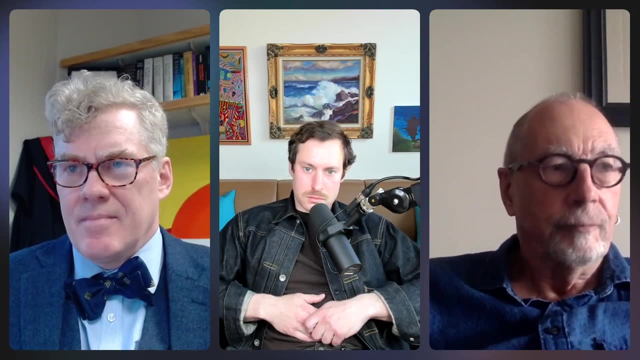 It doesn't express a proposition, or it's not well formed, or et cetera, et cetera. But there are these paradoxes which say: well, consider the sentence, The sentence is either not well formed or false. And then you're back with the contradiction. 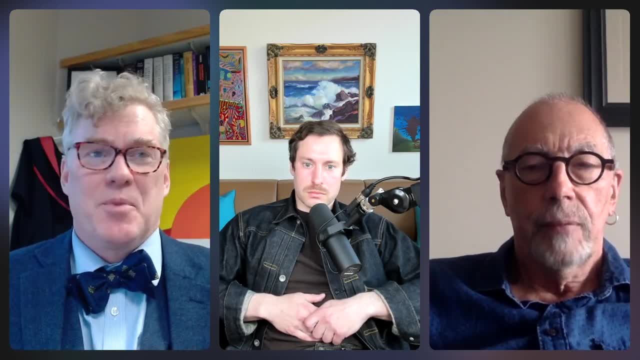 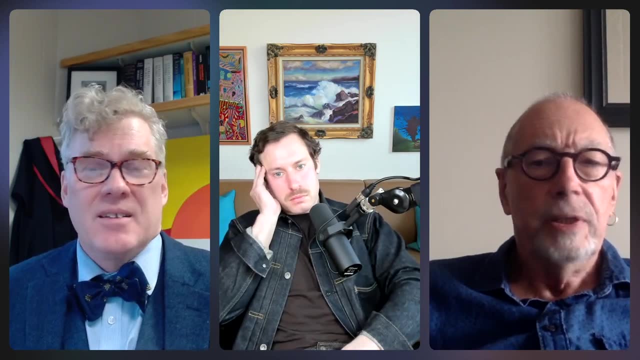 So No, no, Because that one also is not expressing a proposition. I mean because it's predicated in a self-applicable manner, which is: You've just said that it's not true. You said that's not well formed. 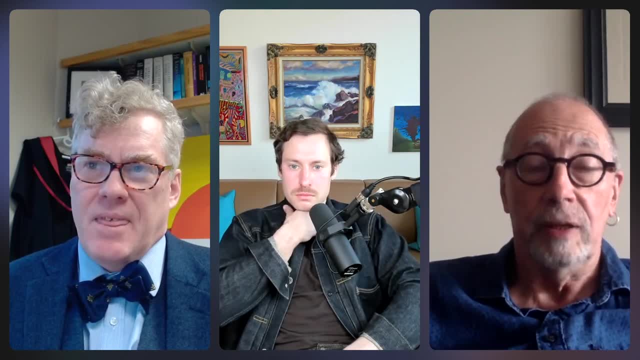 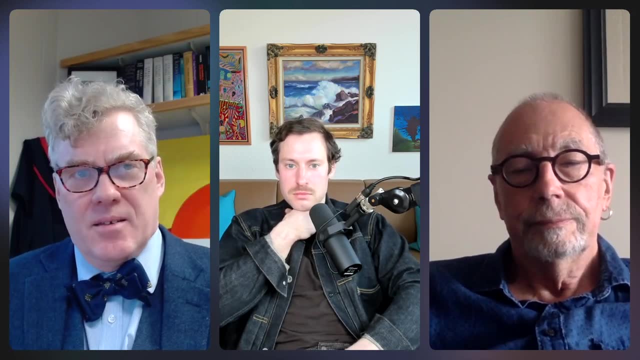 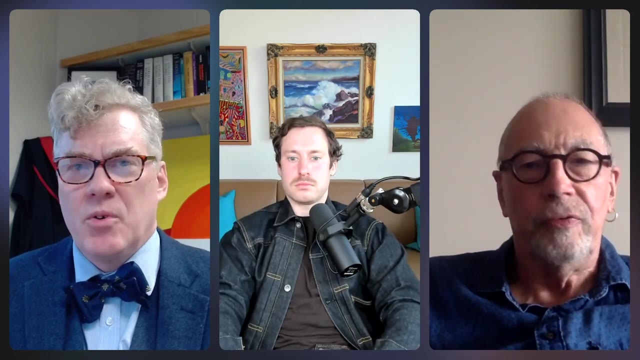 So I presume you think you're saying something true when you say that. I mean the view right is that there is no proposition expressed by the Lara Paradox or any of those revenge ones, And they all separate the same flaw of self-applicable. 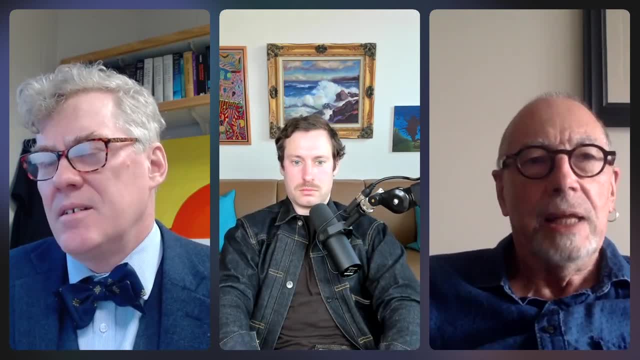 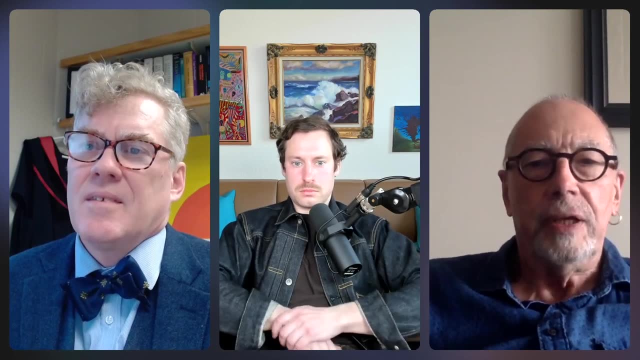 OK. Well, if there's no proposition there, then either it's false or there's no proposition. So if you think it's no proposition, you should think it's false. If you think it's true, I mean this is a bad proposition. 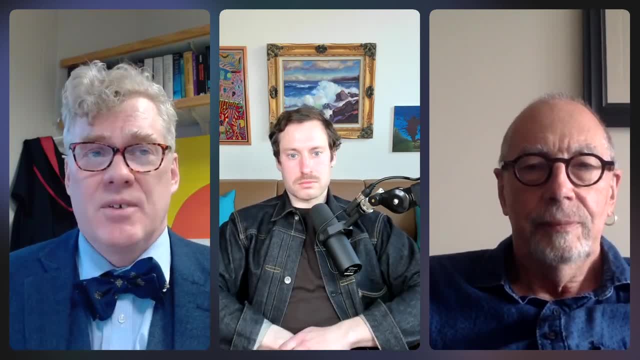 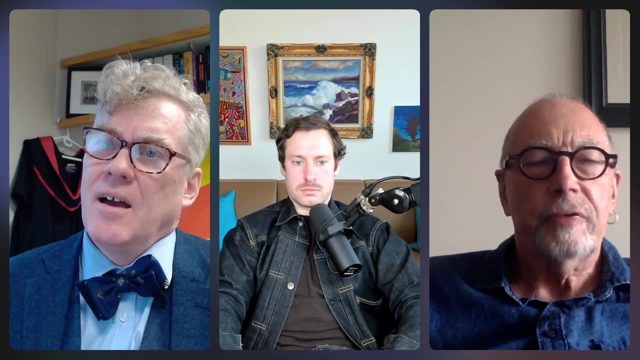 That disjunction, that seeming proposition that was a disjunction is also has the same status, Right? I mean, of course, that's the line that one is going to take. OK, So you just said something that you think is not true. 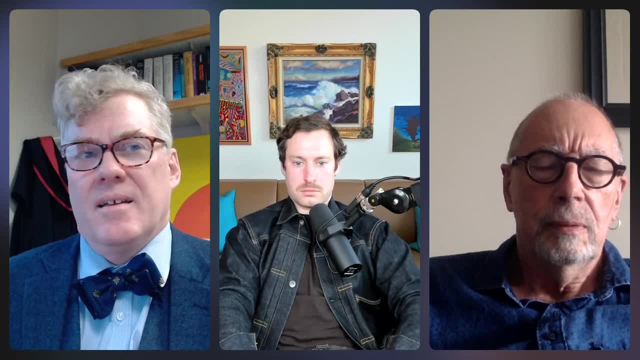 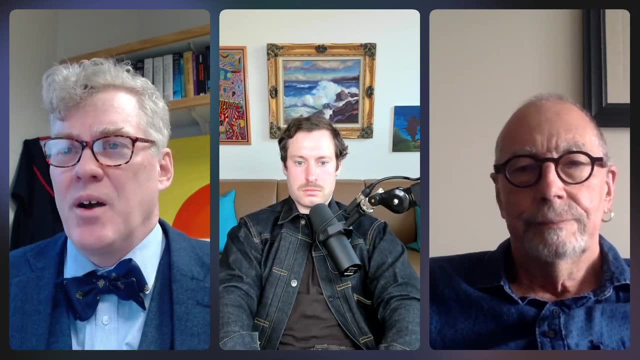 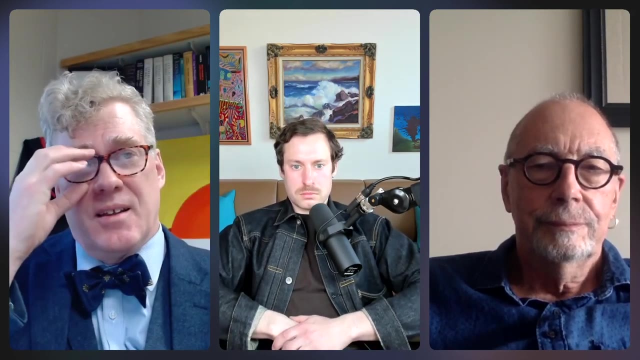 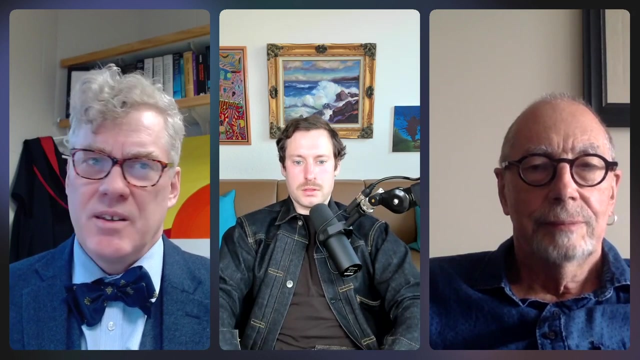 Maybe it expresses no proposition. This assertion- you know, the assertion which I can put quotes around and talk about it as something that to be uttered Right- Is, on this view, not meaningful, And neither are the revenge ones, for the same reason, because they're employing the concept of truth in a self-applicable manner. 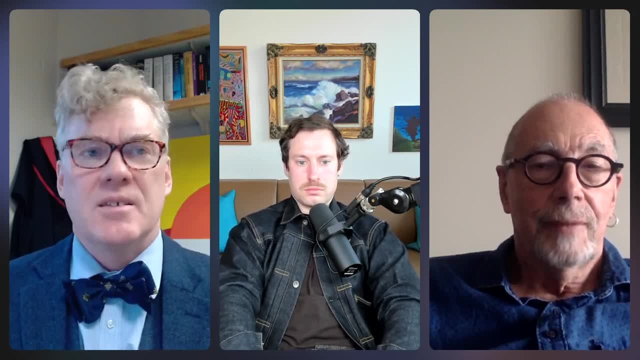 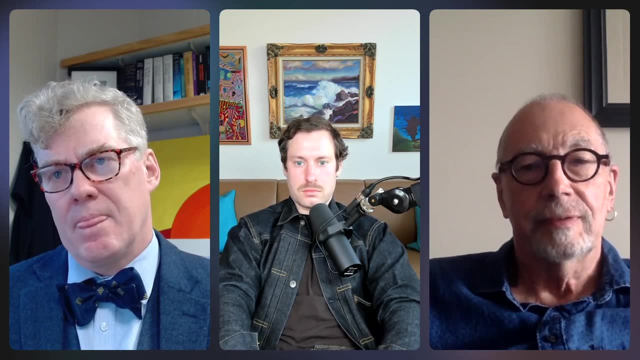 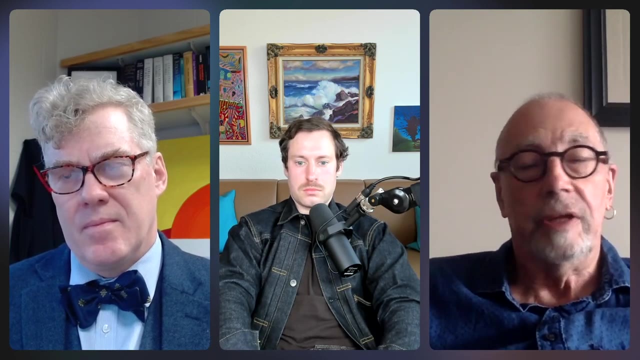 But we don't have any such theory of self-applicable truth. But look, I mean, you said that proposition. that sentence does not express a proposition. OK, And you presumably you think that what you said was true, in which case you seem to be in this extended paradox. 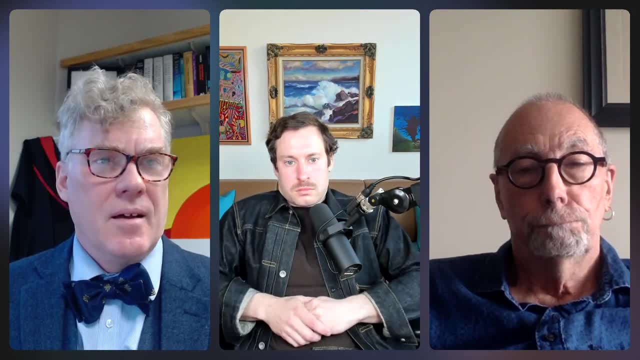 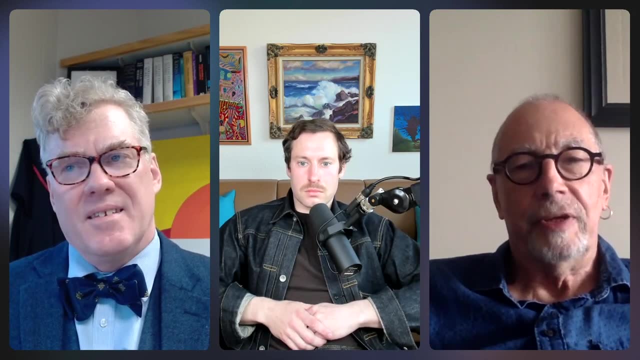 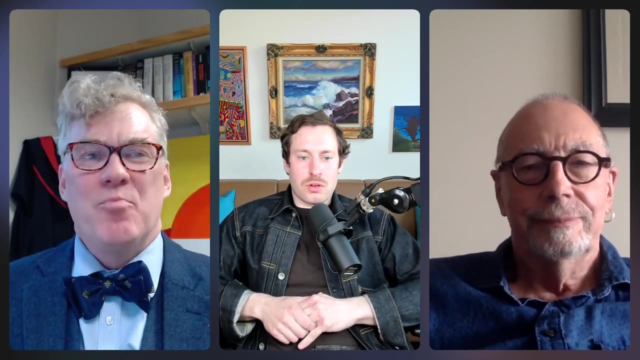 I don't see that I mean: Well, maybe at this stage we need a blackboard. John, let me come back to something, actually, that we mentioned earlier, which is this deflationary to whether one is deflationary about truth. 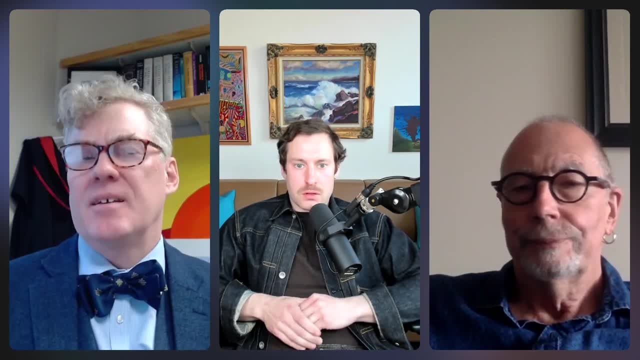 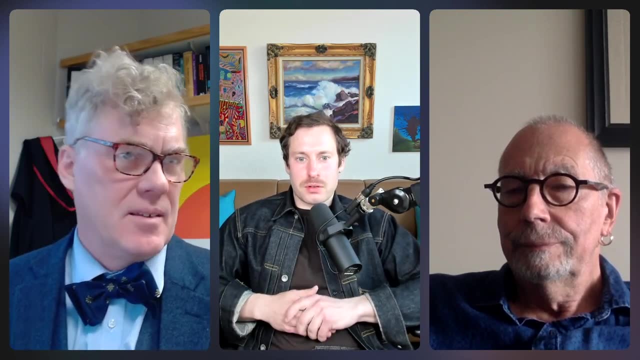 I mean sort of the T schema can be seen, I think sort of John, can you say what it means to be deflationary? Can you say what it means to be deflationary about truth? Oh, I mean just something ordinary. 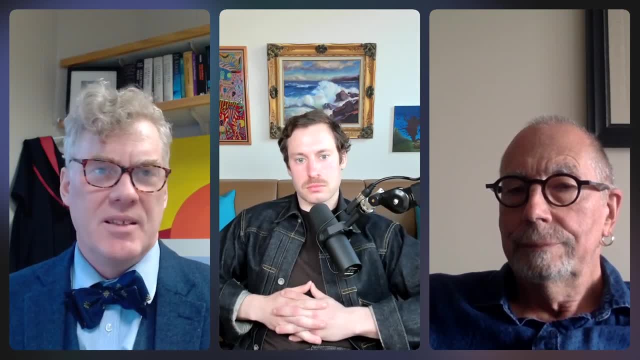 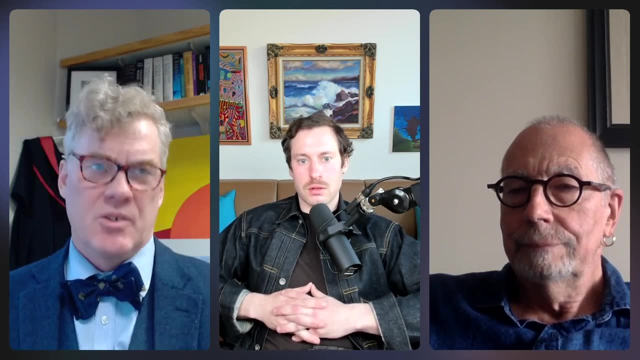 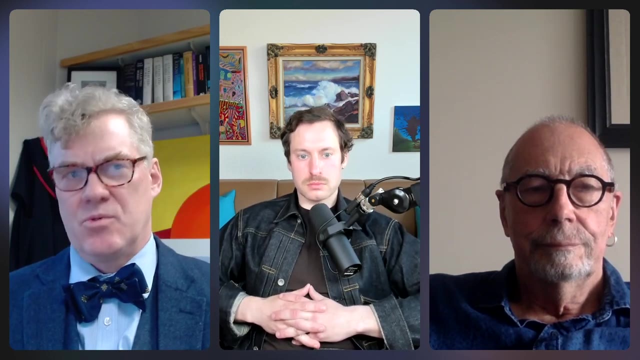 To be deflationary about a topic means to basically explain away instances of those topics in terms of other, possibly more primitive notions or something. So to be deflationary about truth means that truth assertions are just reducing to assertions that don't involve the concept of truth. 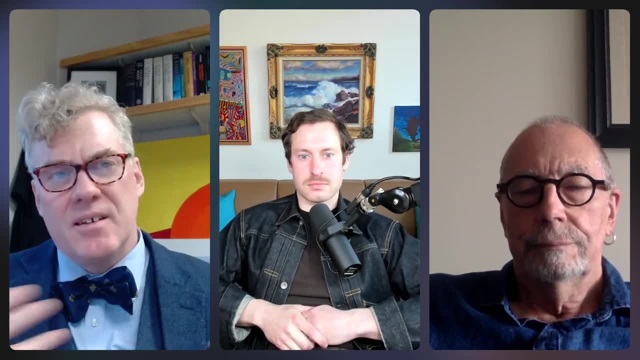 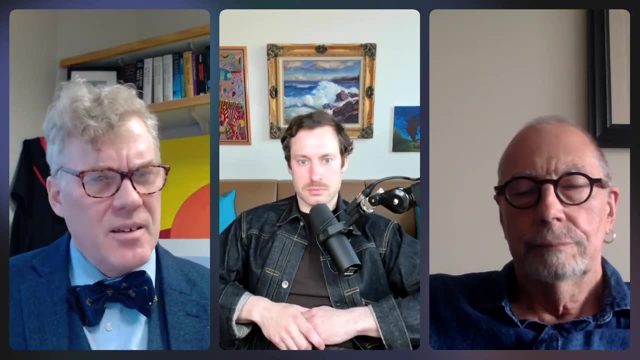 So we've deflated the concept, in a sense, by reducing it to other things, Reducing it to other things that don't involve truth, And the T schema, which is the assertion phi is true if, and only if, phi is sort of explicit. 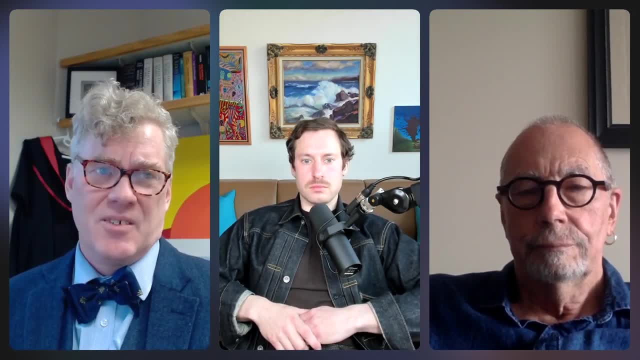 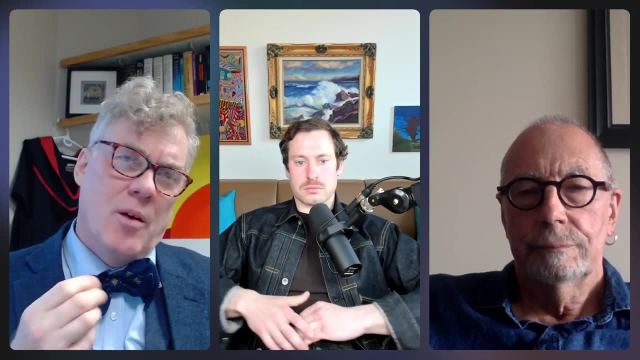 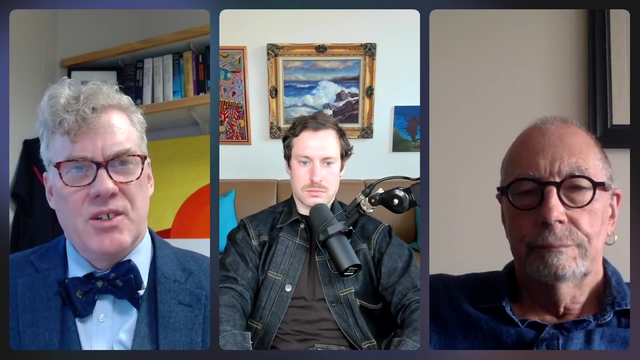 Every instance of the T schema is asserting a deflation. you know an instance of deflationary approach to truth. So my view about this sort of deflationist part of it is that individual truth assertions. One can be deflationist about individual truth assertions. 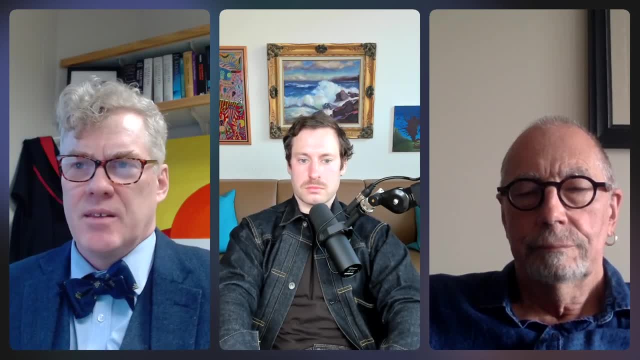 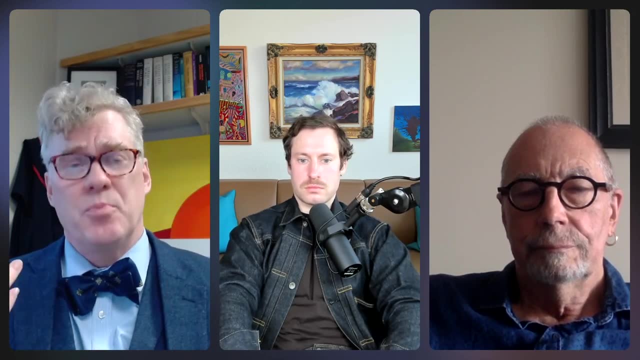 Because they can always be eliminated by the T schema. But that doesn't mean I'm a deflationist about truth altogether, Because to have a truth predicate, we know I mean mathematically, we know it's- the logical complexity is much higher. 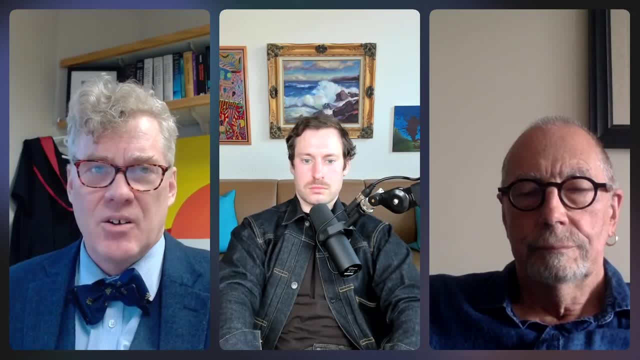 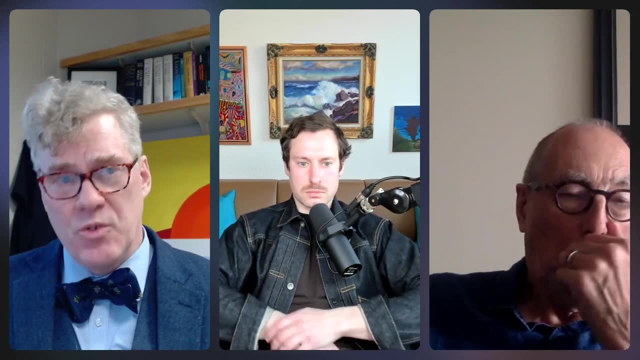 For example, if you have piano arithmetic together with a truth predicate- even this kind of well-founded kind of truth predicate that I was talking about earlier, where we have only truth for the arithmetic assertions and not for assertions involving truth, This implies can't PA. 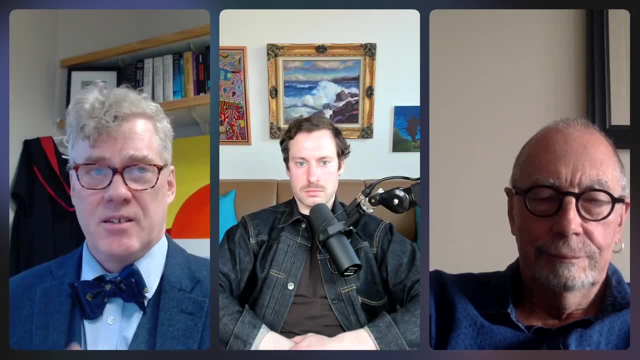 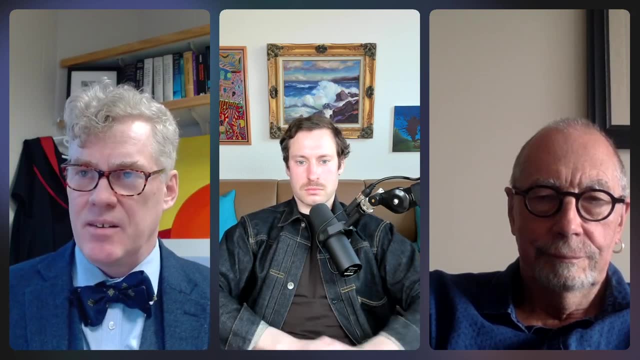 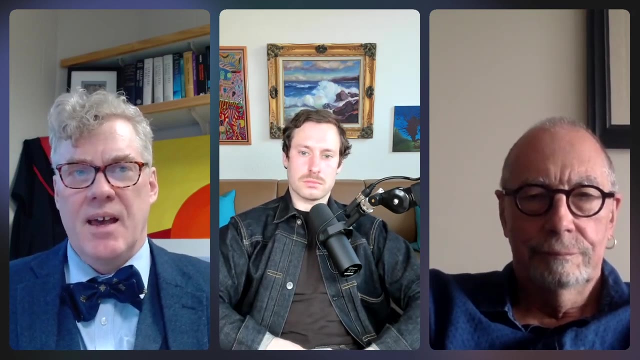 It's strictly stronger in consistency strength if it's an inductive truth predicate And so having a concept of truth- I'm not a deflationist about that- To have the whole predicate as a completed totality and to be able to reason with the concept of truth in that sense is definitely stronger than not having any concept of truth. 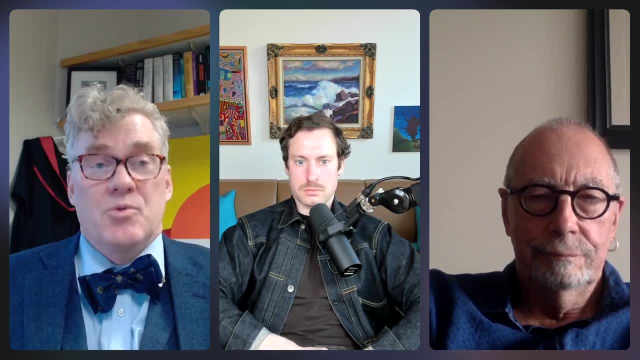 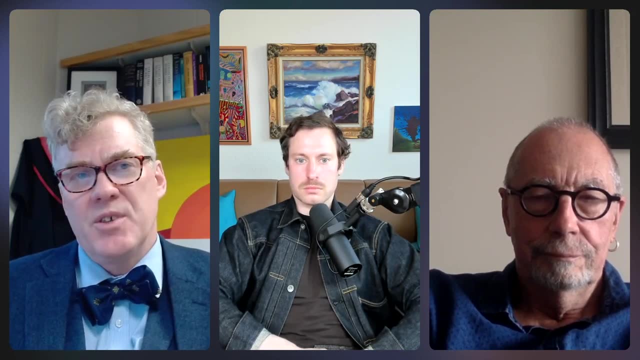 So I'm not a deflationist about truth in that sense, But I am a deflationist about truth. So I'm not a deflationist about is truth assertions made, sort of one-off truth assertions, To say phi is true, it just is to assert phi. 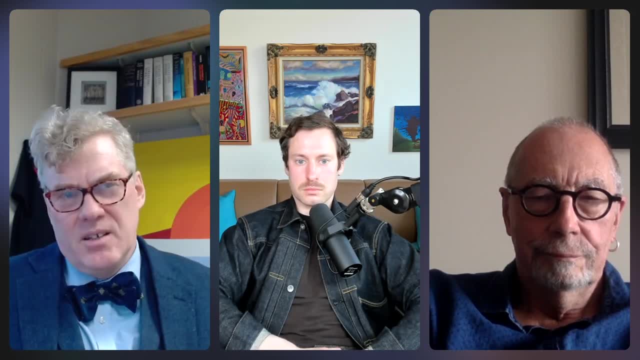 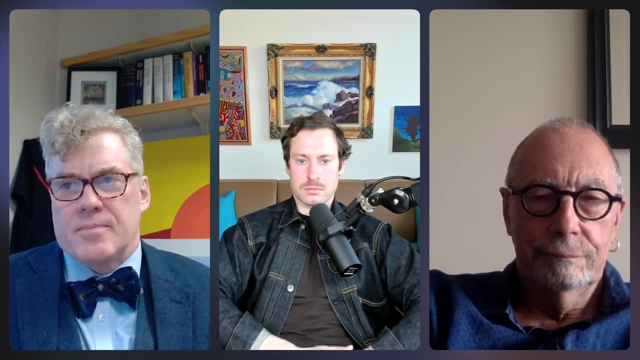 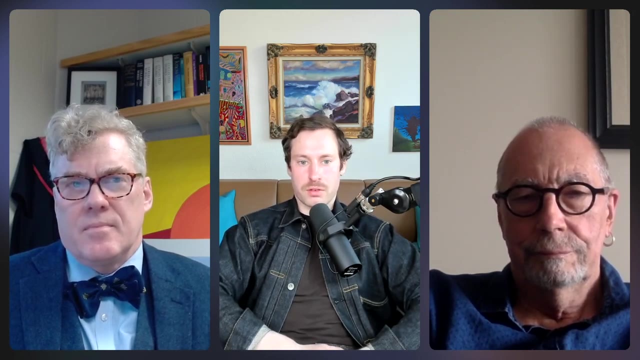 And I can agree that. So I like to distinguish between sort of individual truth assertions and having a truth predicate, which seems a much stronger thing. Now, Joel, is your preferred way of solving the puzzle than just to say, just to dismiss it? 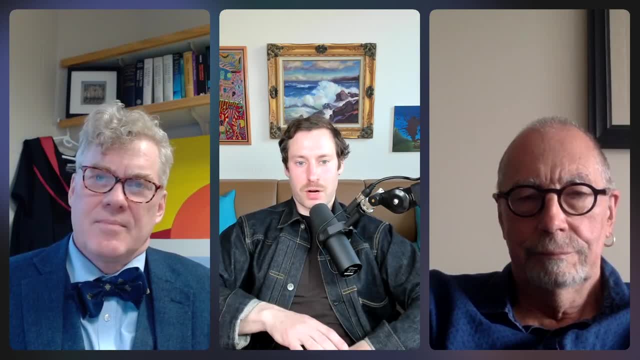 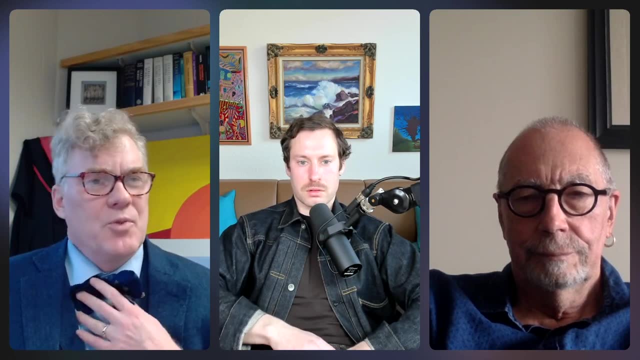 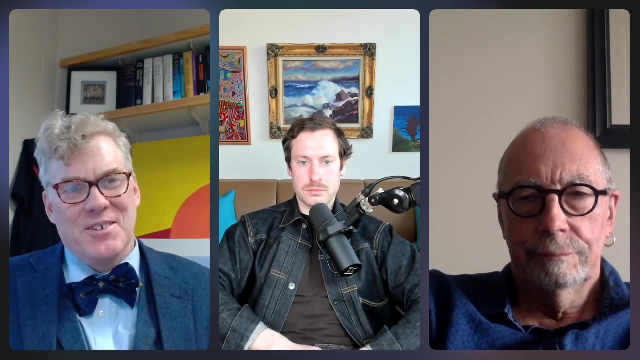 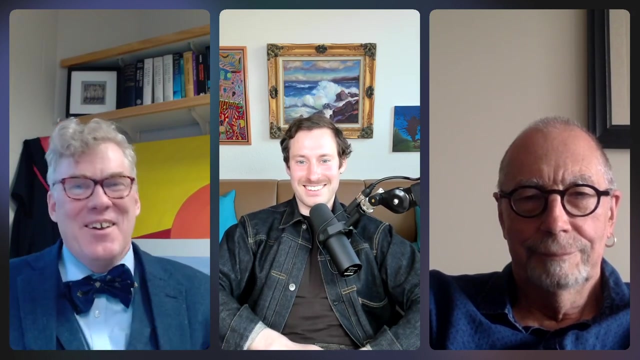 And say that there is no proposition expressed by the liar paradox and just you, just don't let it get off the ground, Right? So I mean, I don't know if I have a preferred way, And actually I've talked with Graham and Hartree and so on, enough that to have the experience of whatever you say about the liar paradox. either Graham or Hartree is going to trap you in some revenge situation. 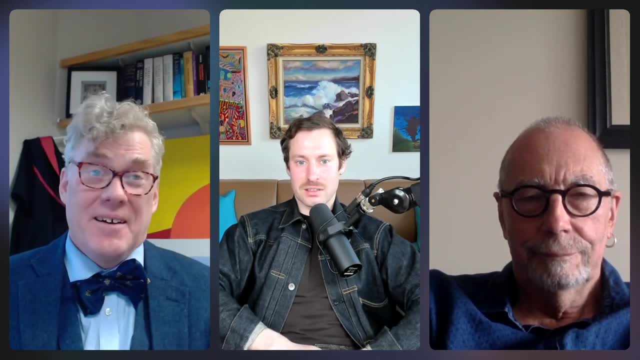 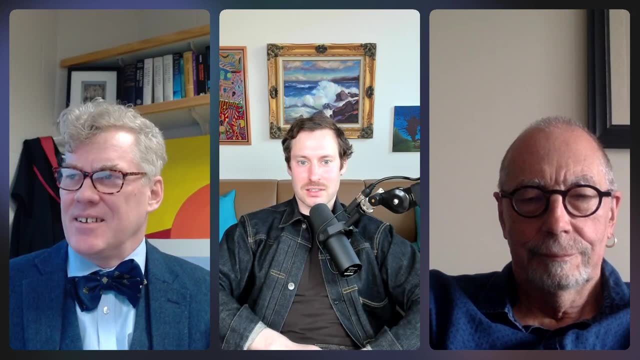 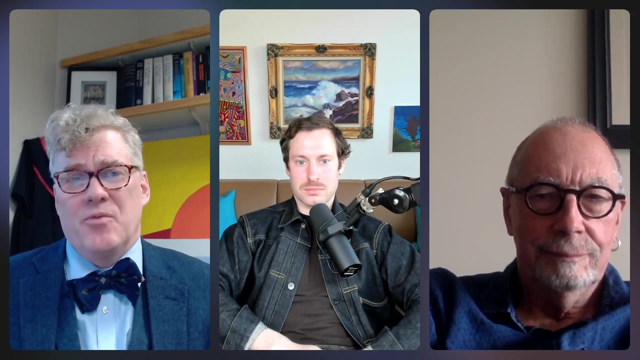 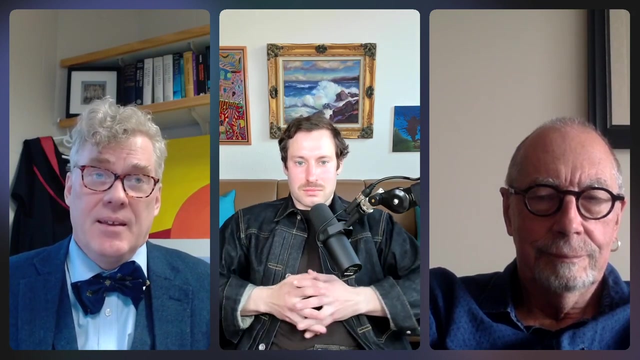 So I really hesitate to To make any definite statement about the liar paradox. Rather, my approach, though, to answer your question is to talk about the nature of truth and what it means to have a truth predicate, And my preferred kind of explanation of that is always to talk about these well-founded cases, which are, after all, the main uses of the concept of truth. 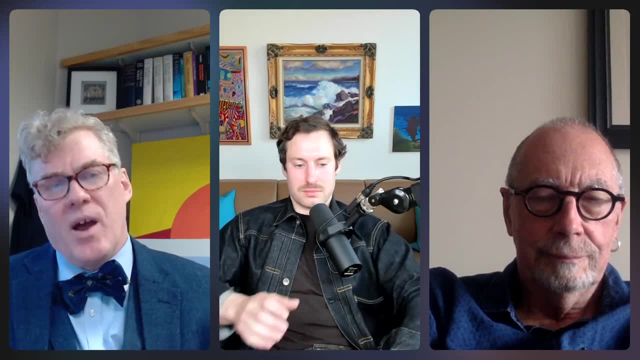 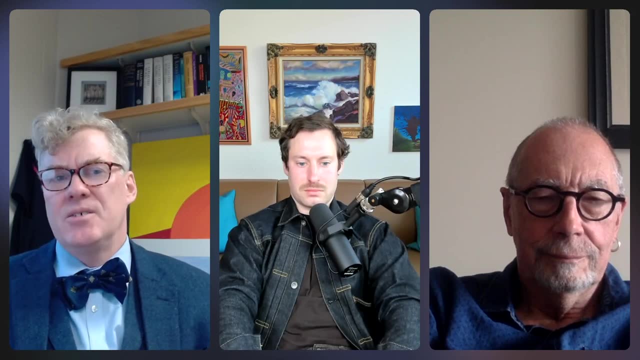 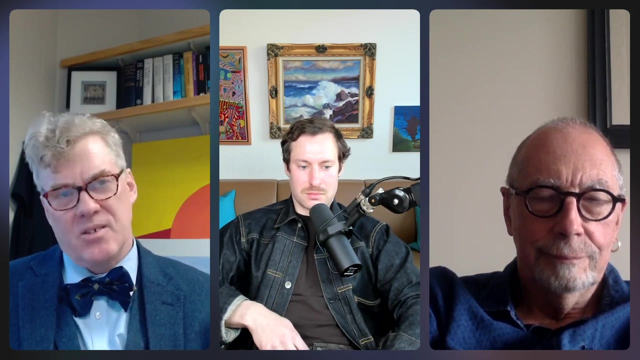 If one looks beyond the liar paradox, when are we making truth assertions? When are we using the concept of truth in mathematics or even in everyday usage? It's almost never in those self-referential, self-applicable situations, But rather it's almost always in this kind of well-founded case. 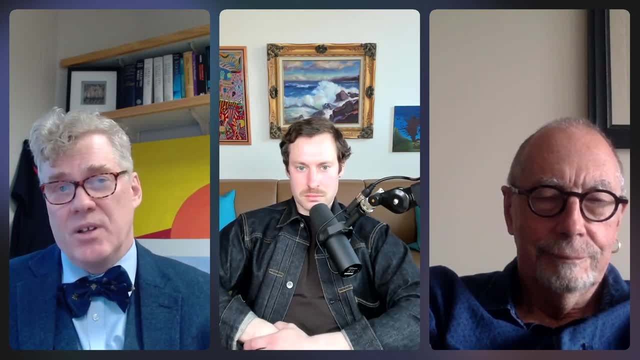 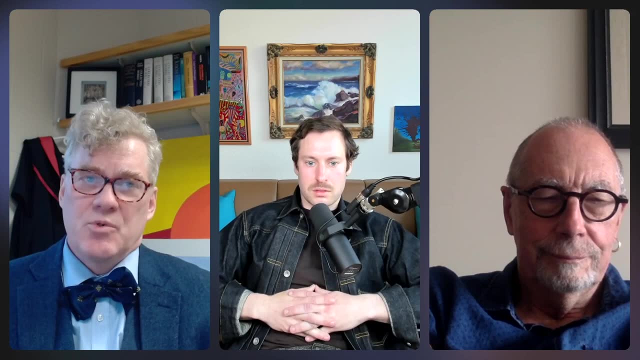 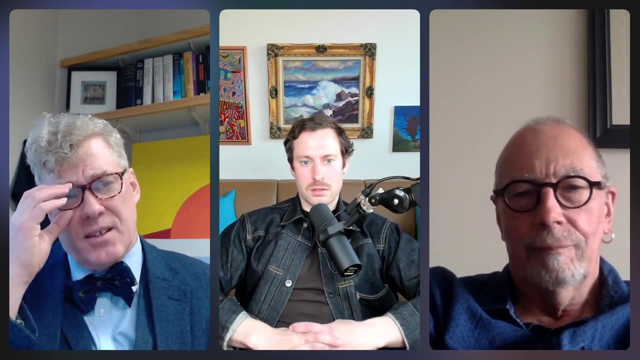 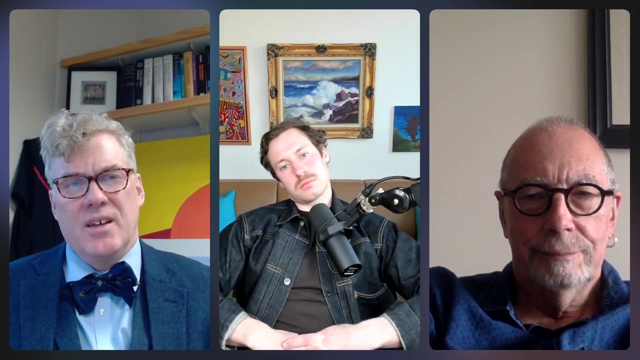 And that's the case of truth that we really need to analyze, And I think we have a very satisfactory analysis of the nature of truth for those kinds of sentences that appear, Sentences that appear in that well-founded, iterated truth predicate situation, And what I think about the liar sentence is that it's something akin to ignoring this underlying, well-founded hierarchy. 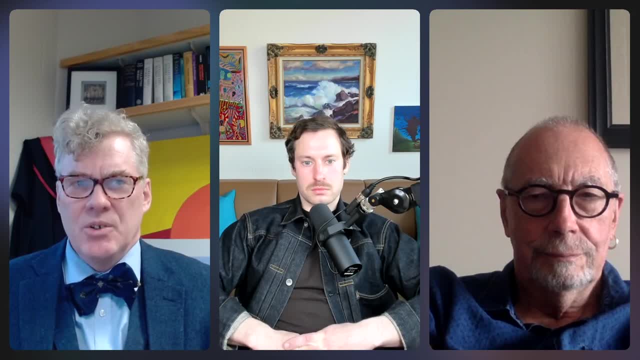 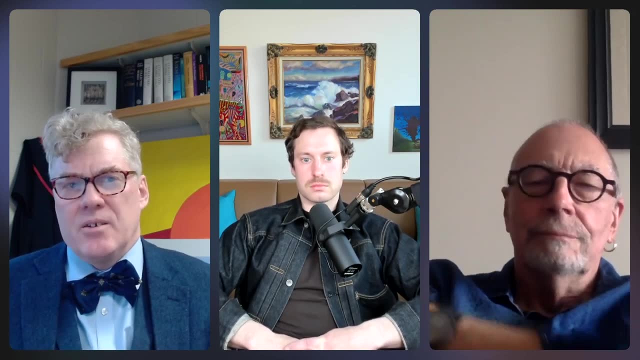 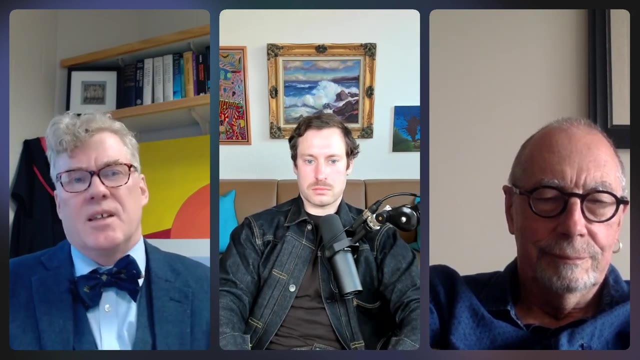 which is exactly similar to the way that the Russell paradox ignores that general comprehension principle, ignores the underlying hierarchy of the hierarchy of truth, The hierarchy of sets, And you know, by presuming that you can form the set of all sets with any given property. 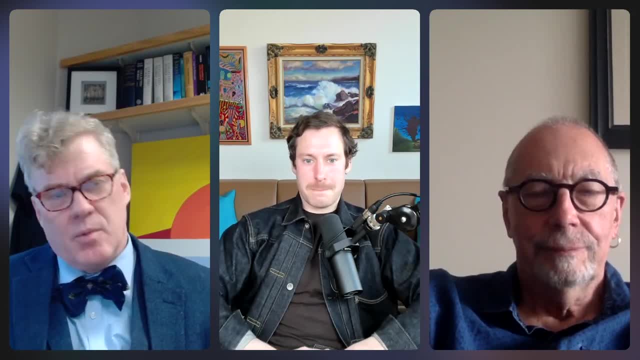 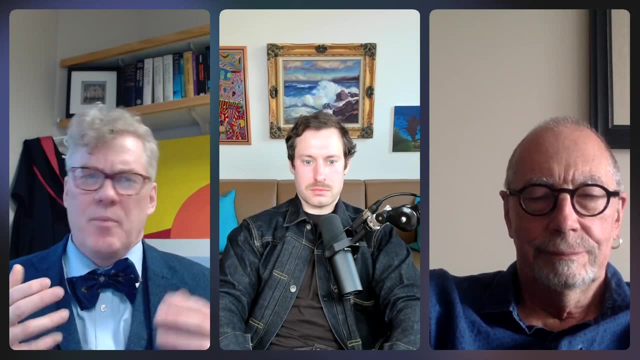 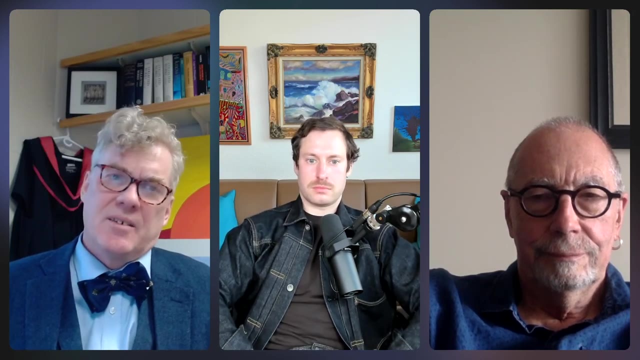 and that the sort of expectation that we should always be able to make truth assertions about any assertion, including ones that are already involved in the concept of truth, And so I'm deeply suspicious of the liar sentence, because I view it as sort of violating what I understand to be an inherent, underlying part of what truth is like. 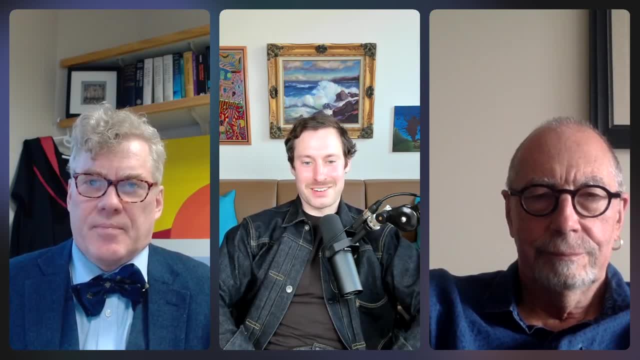 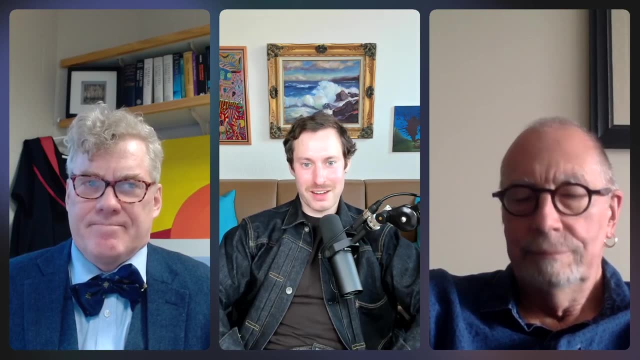 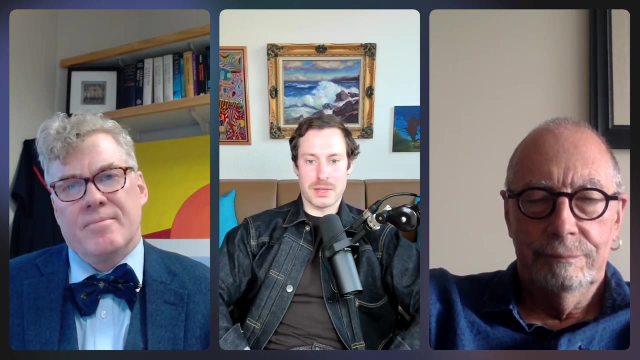 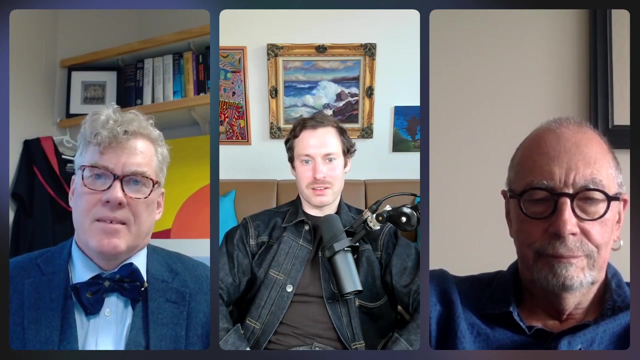 And now, as Graham mentioned, I mean Eubulides came up with this paradox maybe 2500 years ago, and people have been talking about it ever since, and many people like Graham treating it very seriously. So do you then just appeal, maybe, to something about human psychology, like an error in our thinking, that makes it seem so compelling? 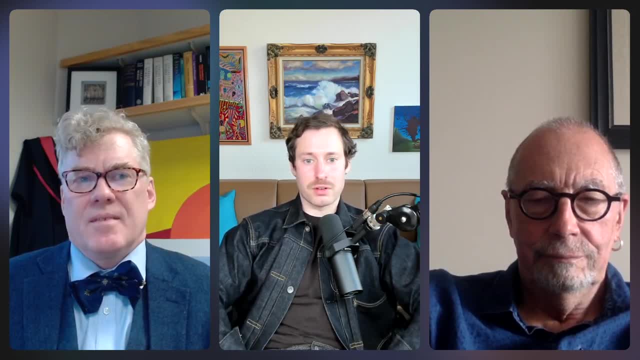 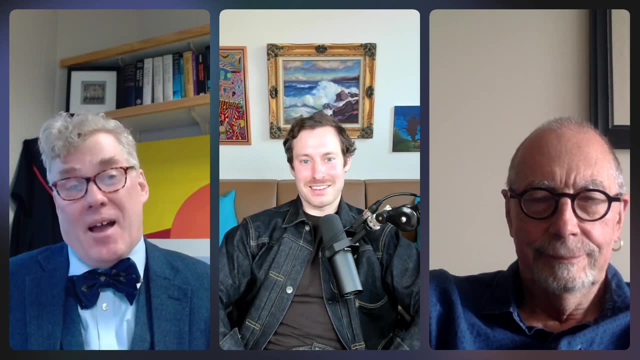 but really it just doesn't get off the ground. It's just the fault of natural language. I see, I don't know, I'm not going to be able to say something definite. I view it as a kind of illusion that whether it's expressing something or not, 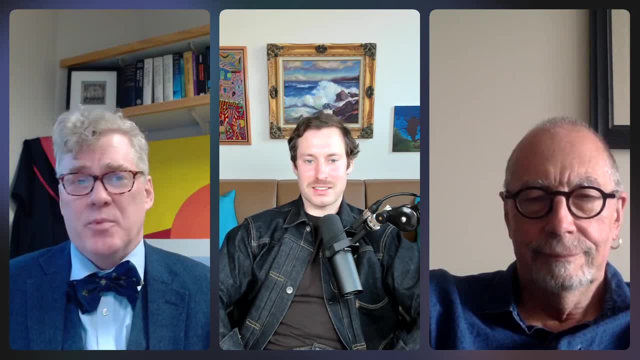 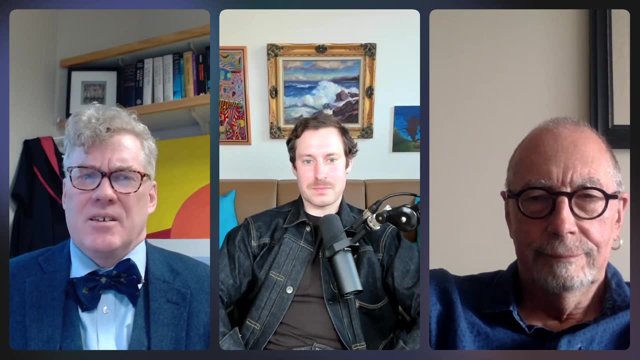 And the proof that it's an illusion is the contradiction that we can prove from it. If you take it at face value, then you're getting this contradiction, And to make the move as Graham does, which I understand, is very tempting and seems quite reasonable. 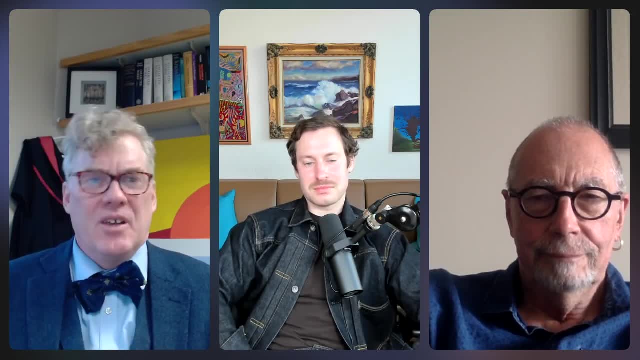 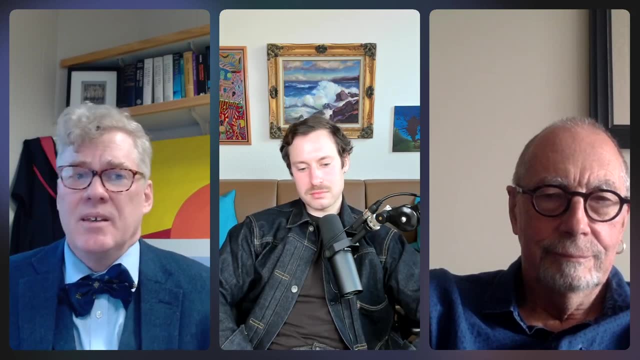 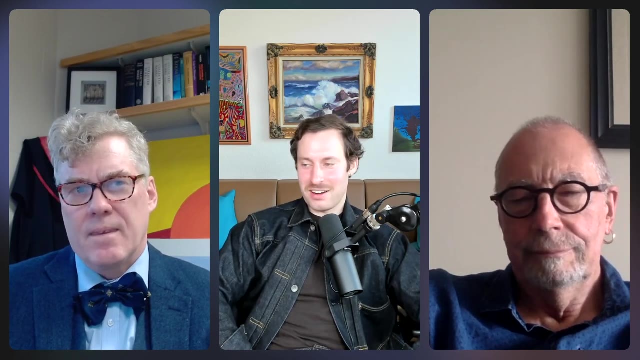 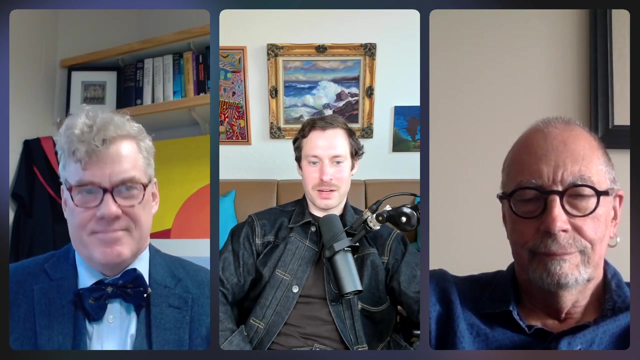 but I I wonder if it has explained the illusion or if it is just accepting the illusion without actually giving me a better understanding of how it could be that there are true contradictions. And I think Hartree is going to be on the show relatively soon, mainly to talk about mathematical fictionalism. 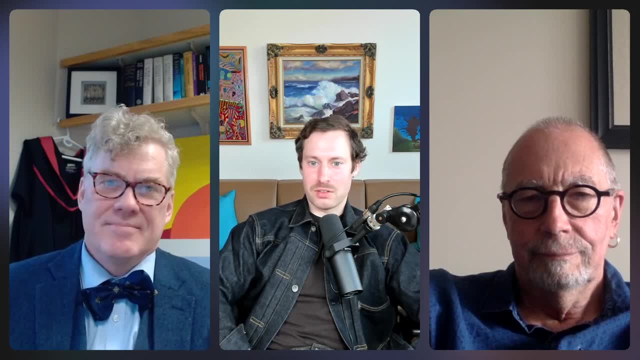 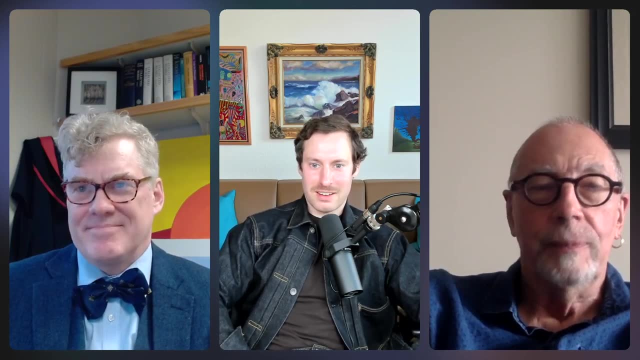 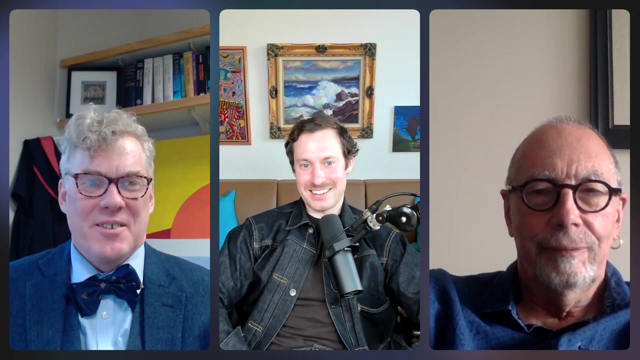 But Graham, does he have the same views as you do on the liar paradox? We both disagree with each other and with Joel. Okay, great, Maybe it should have been a four-way podcast. What is the theorem of philosophy in general that any two philosophers are disagreeing with? 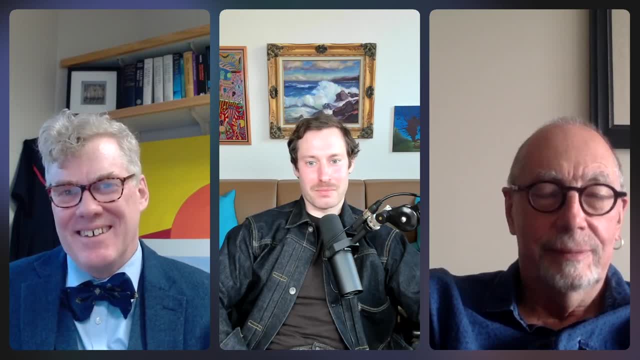 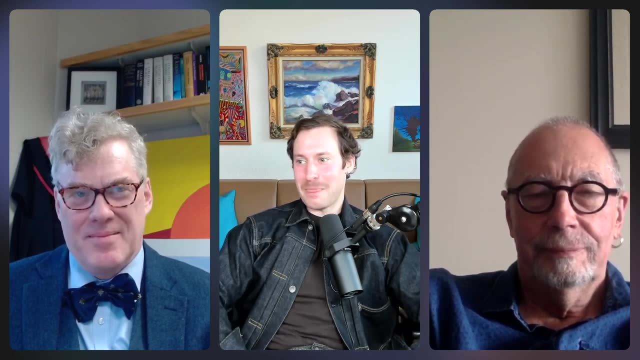 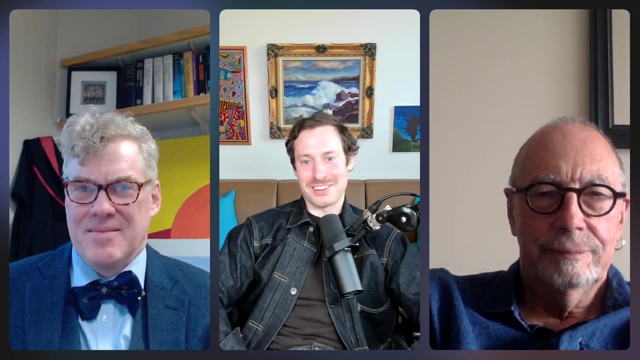 Michael Harris, the number theorist at Columbia, was on one of my first episodes and he said something to the effect of: he understands that philosophy progresses just by force. And I thought: well, he's a philosopher. He's trying to smash each other's work the best he can. 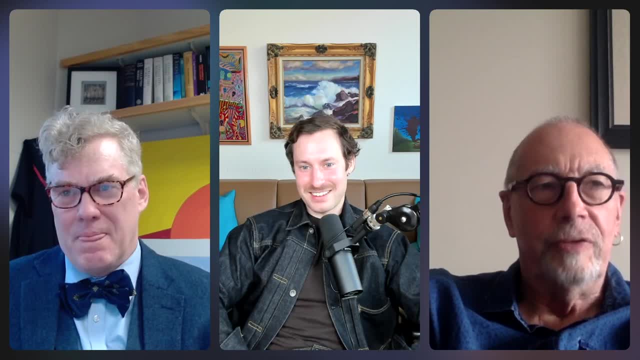 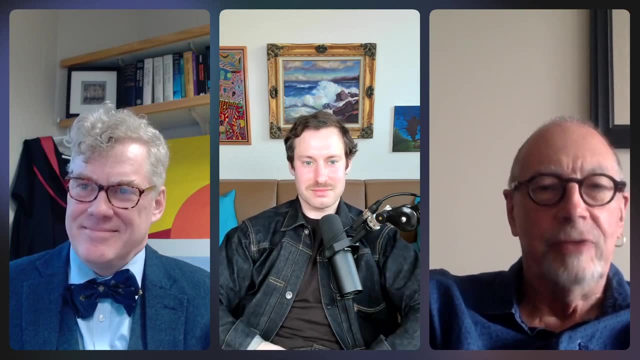 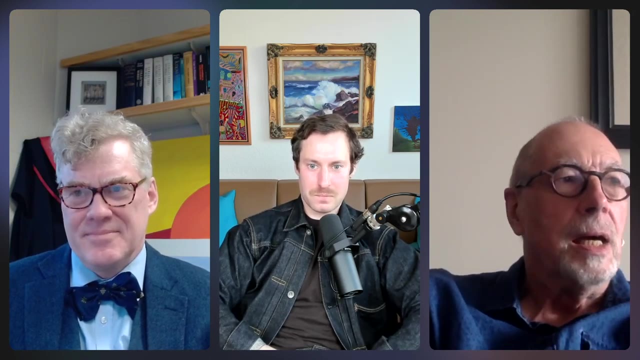 Joel subscribes to classical logic, which is a logic invented by Frege and Russell around the turn of the 20th century. Logical theories have been changing for two and a half thousand years. That happens to be the kind of one which many people subscribe to, and Joel does too. 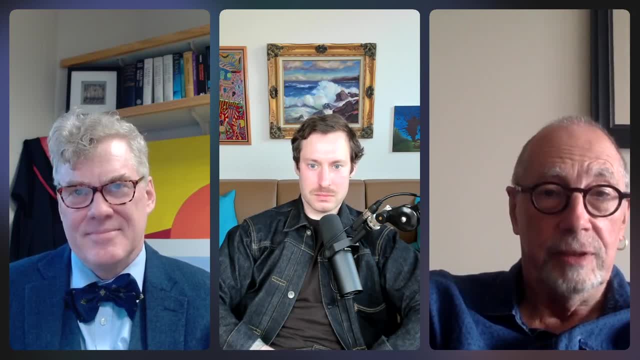 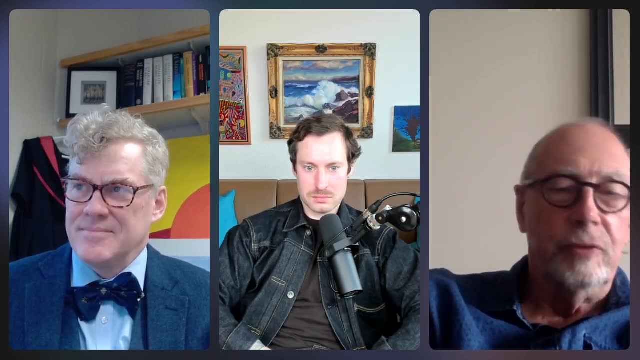 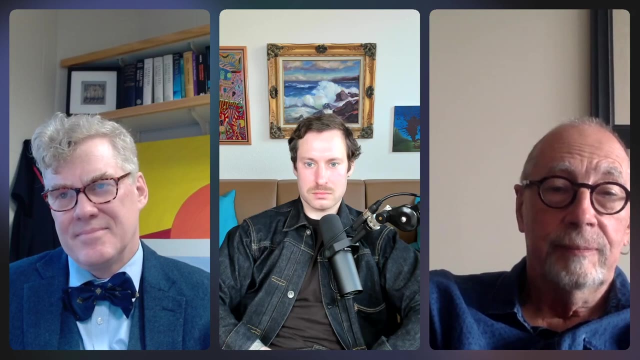 Both Hartree and I do not subscribe to that account of logic. but we don't subscribe to the same kinds of logic. I subscribe to a logic in which the inference from a contradiction to an arbitrary conclusion fails. Hartree subscribes to a logic in which the principle it's good at middle fails. 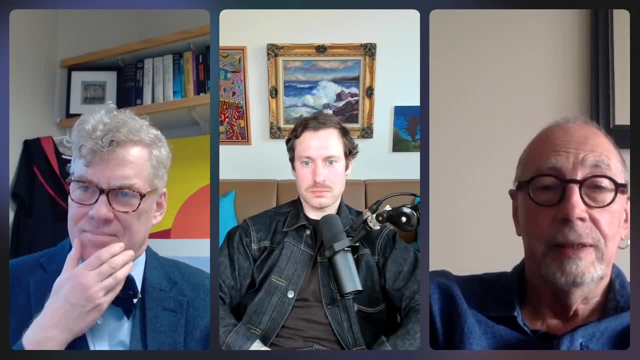 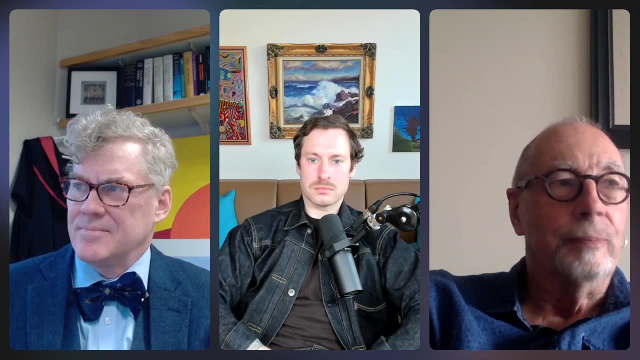 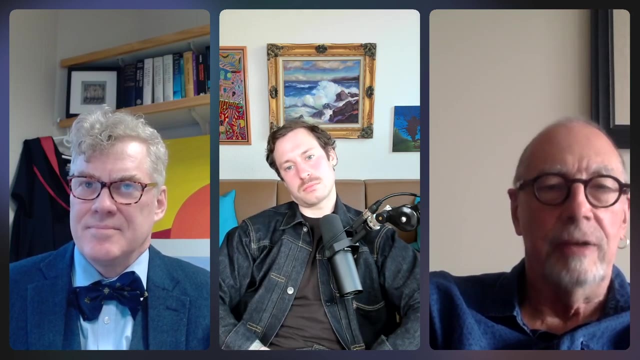 So you've got three possible solutions to the liar here. One is to endorse classical logic and then fiddle around with the notion of truth. One is to accept the T schema and then fiddle around with the logic. Those are three very standard solutions to the paradox. 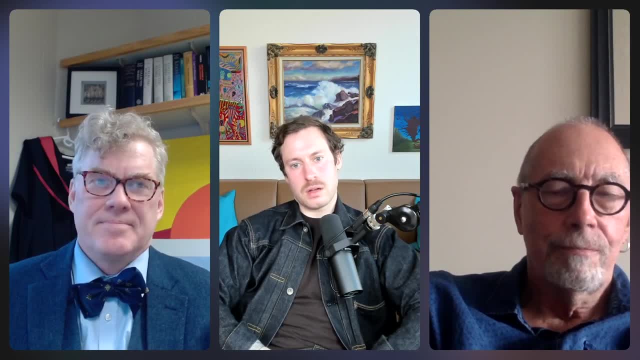 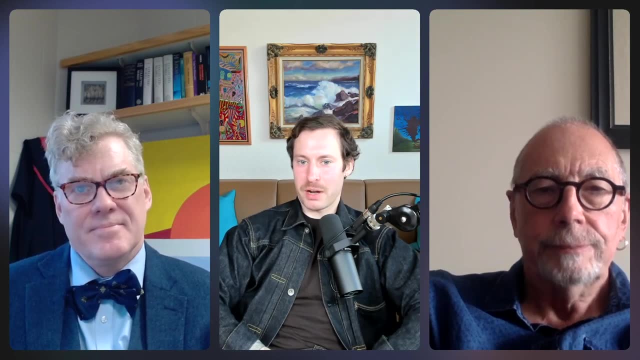 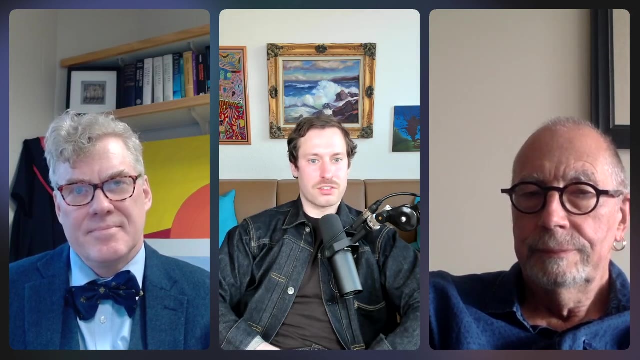 And you'll find a way to do that, sure? And Graham, I am curious because maybe I'll be misquoting or misremembering, But I recall from our last conversation that you said something to the effect of you're sympathetic with there being one true logic. 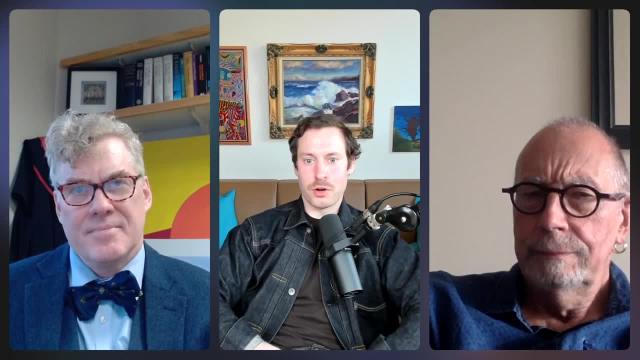 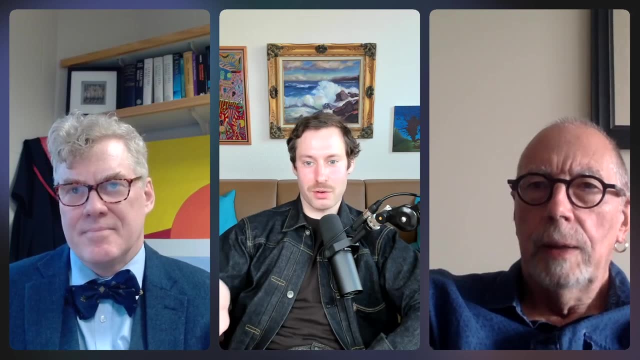 And it is classical logic, It's the logic that is true of the world, And maybe so you're furrowing your brow. So it seems like maybe I am misremembering, Maybe I am misremembering something you said, But I was going to ask if I'm misremembering what you said or if I am remembering what you said. 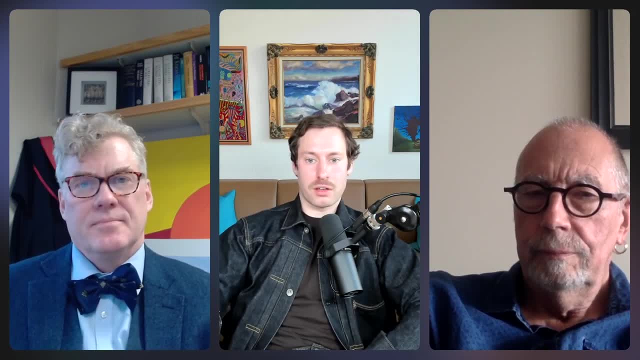 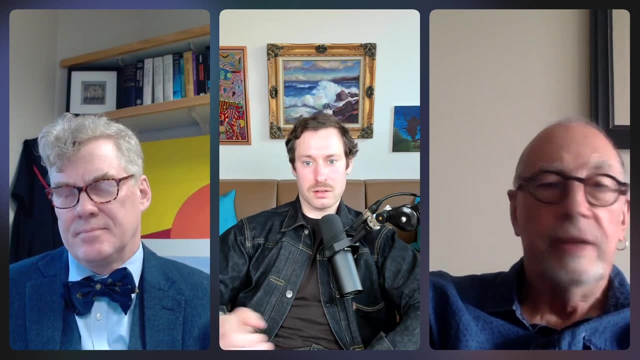 then why does it strike you, in this case, as natural to deal with the liar paradox by reasoning paraconsistently? Look, I may well have said I think there's one true logic. OK, I certainly didn't say it was classical logic. 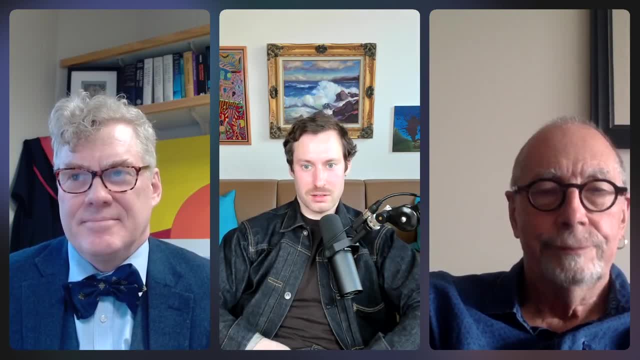 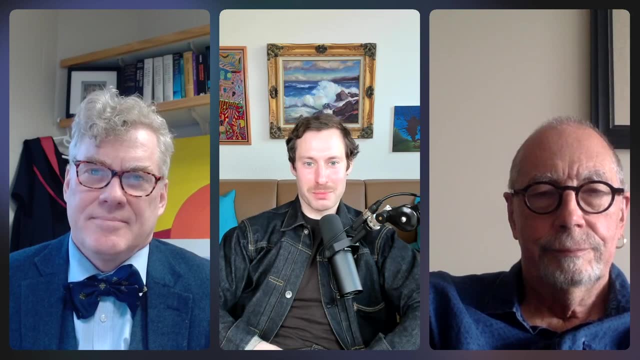 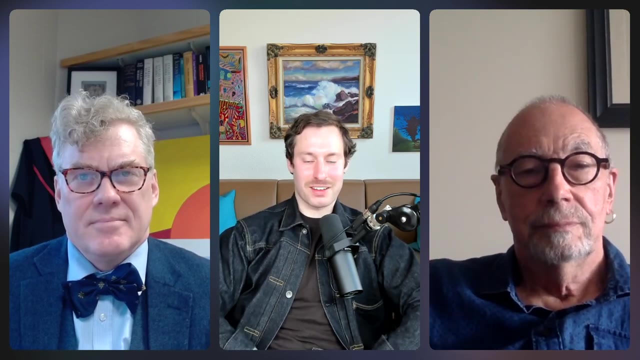 OK, I just said it was a paraconsistent logic. OK, Great. And then, Joel, another question for you. In your upcoming book, The Book of Infinity, which we talked about more in our last episode, there's a chapter, I think, on infinite liars. 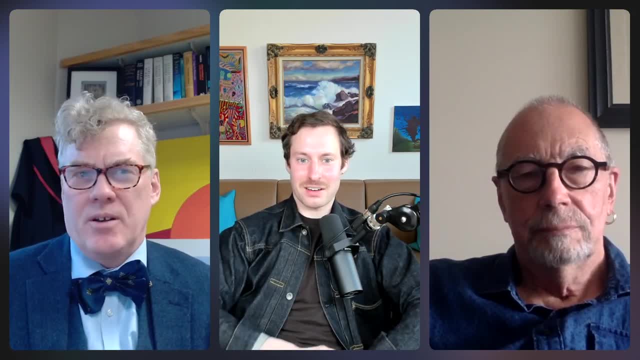 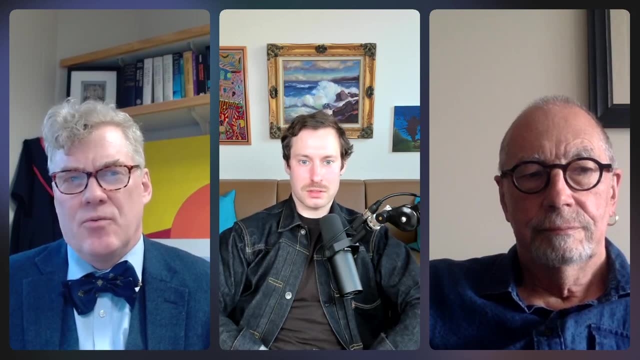 Oh yes, This was a reference to the Yablo paradox, which I'm sure Graham knows very well. It's a kind of approach, I mean, it's a version of the liar paradox that's trying to avoid the use of self-reference. 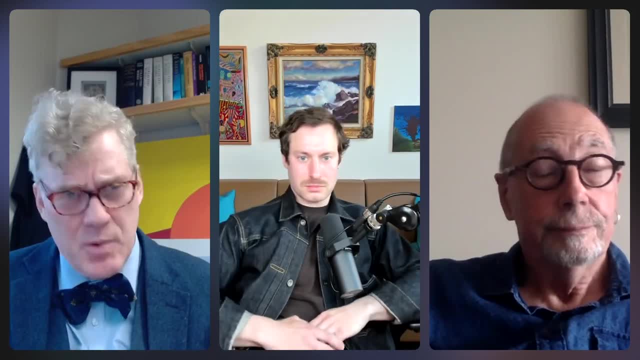 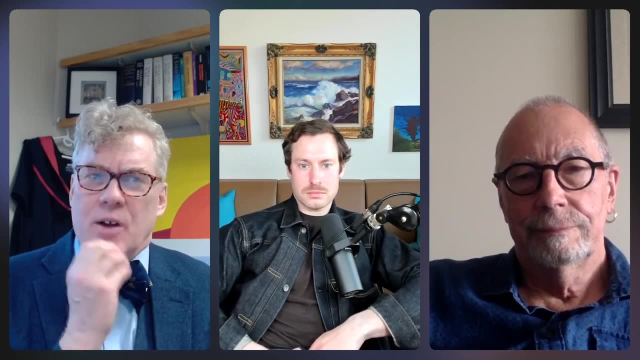 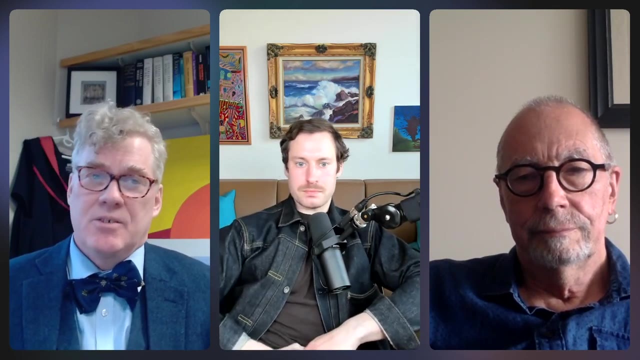 The liar paradox is making this self-referential assertion And sometimes people say: well, maybe that's the source of the difficulty. I mean, my attitude about self-reference is that there's nothing inherently bad about self-referencing. In fact, we can prove, using Gödel's fixed-point lemma idea and Carnot's ideas on those fixed points, that self-reference is inherently a part of all of our mathematical theories. 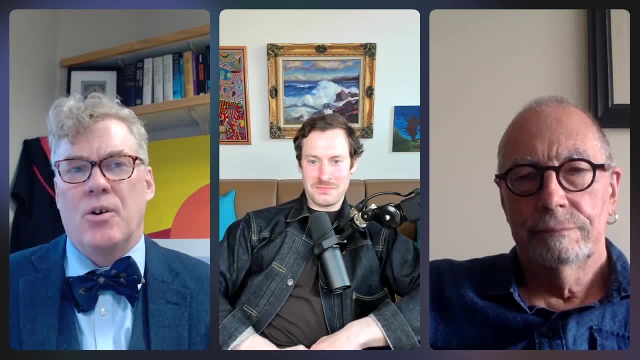 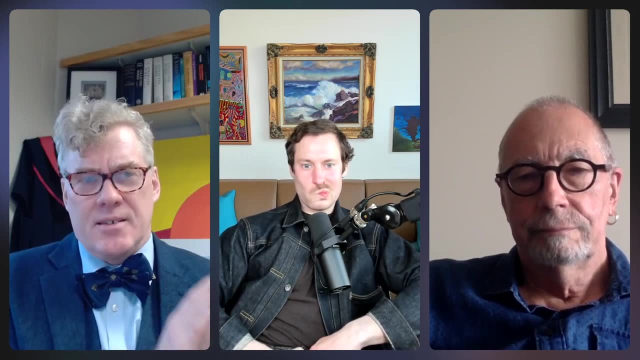 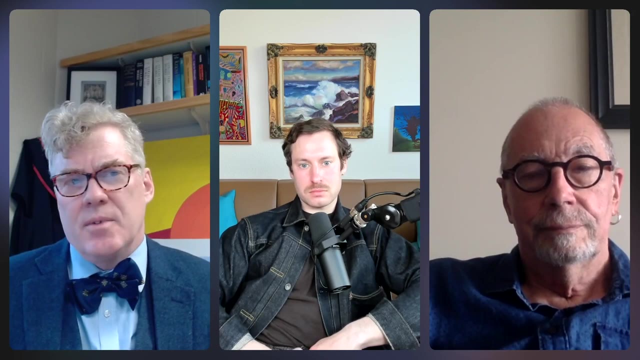 And it's not especially problematic or worrisome. So I don't find anything worrisome about the self-reference part of the liar paradox. But the Yablo paradox goes like this: You have infinitely many statements and each one of them says that all of the later statements are false. 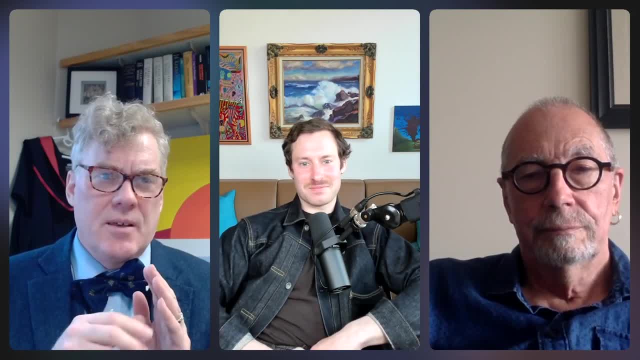 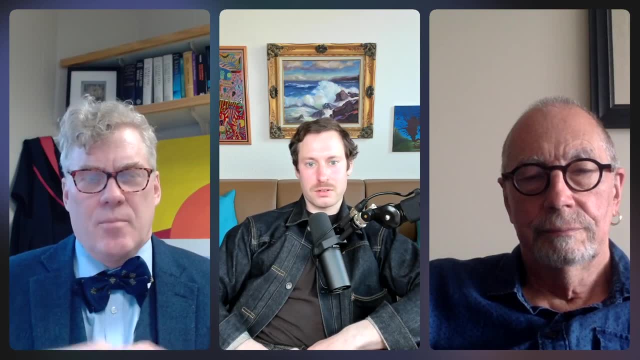 None of them is referring to themselves, right, Because they're only referring to the later ones. So this is avoiding. Nothing refers to the first one, But let's just analyze it. So each statement says: all the later ones are false. All the ones that come after are false. 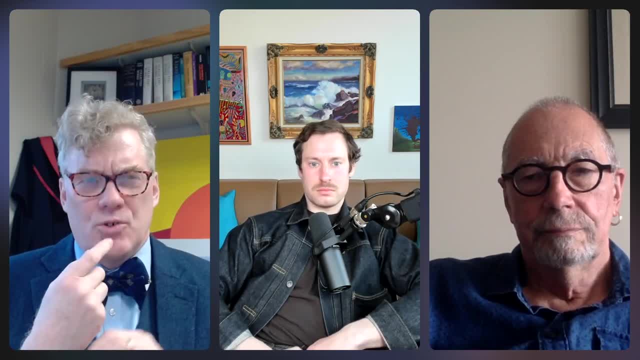 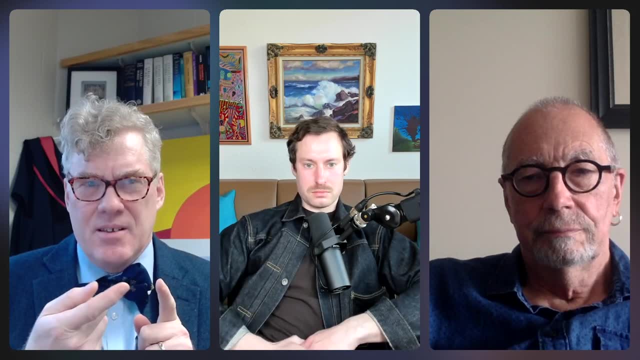 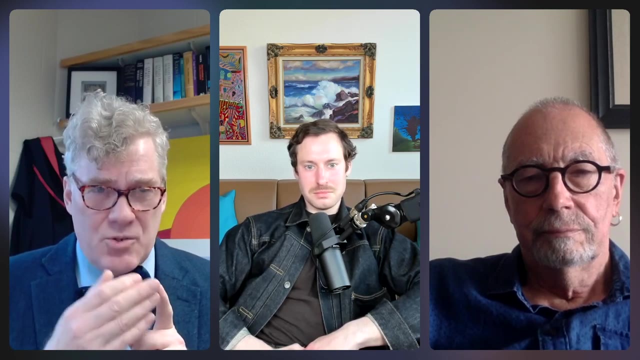 But then if one of them were true, Then the next one, then all the later ones are false, But then the next ones should also be true, because what they assert is the case. So if one of them is true, then all the later ones are false. 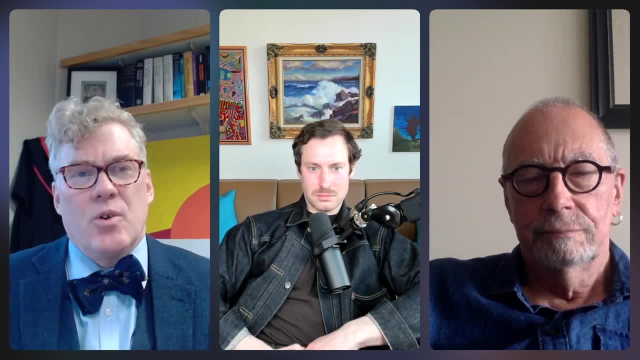 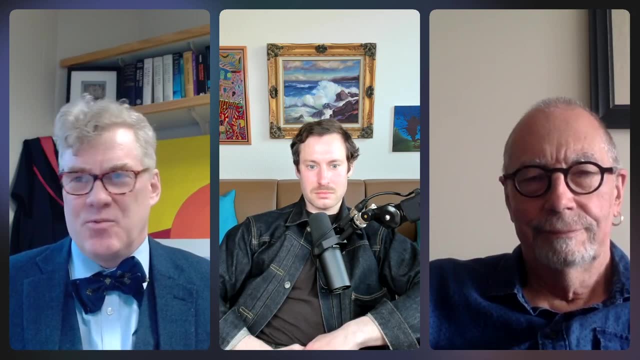 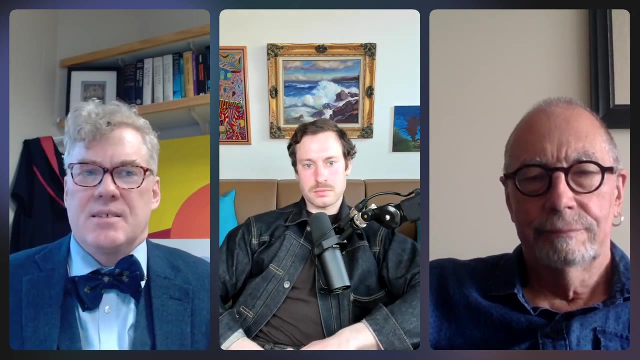 But then they should all be true, right? So therefore none of them can be true, But then they should all be true because of what they assert, And so it's basically the same as the liar paradox Reasoning, But it's with these statements that are in some sense- I mean arguably not self-referential. 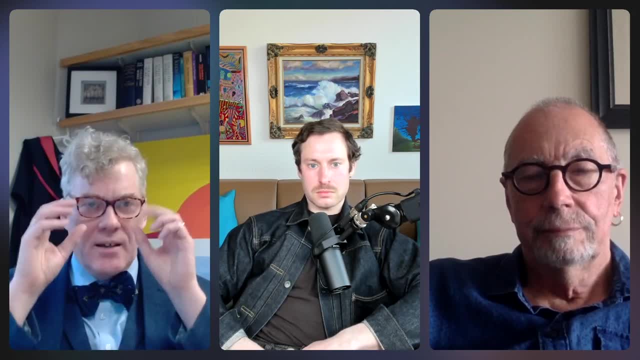 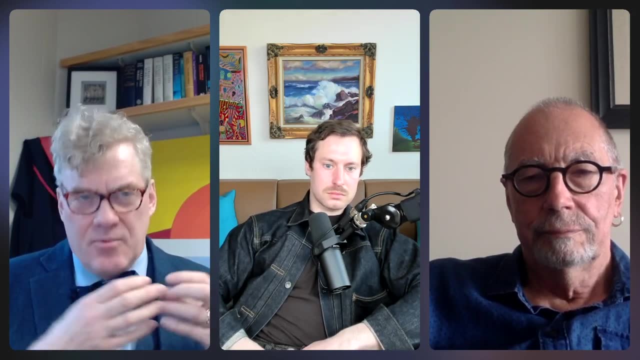 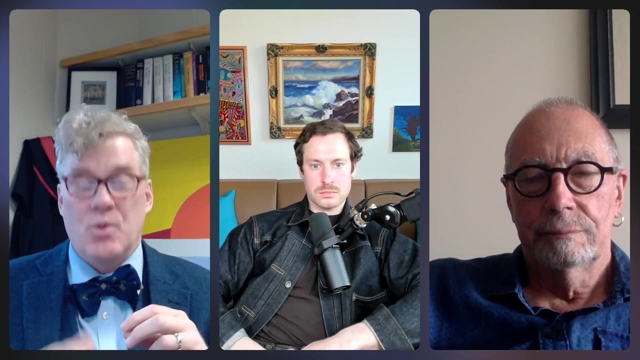 I mean, I would argue actually they are self-referential because each one of them is referring to the other, So each one of them has to have, you know, the capacity of making this reference to the later sentences. So this is really just kind of one sentence with a parameter. you know that's changing as you go. 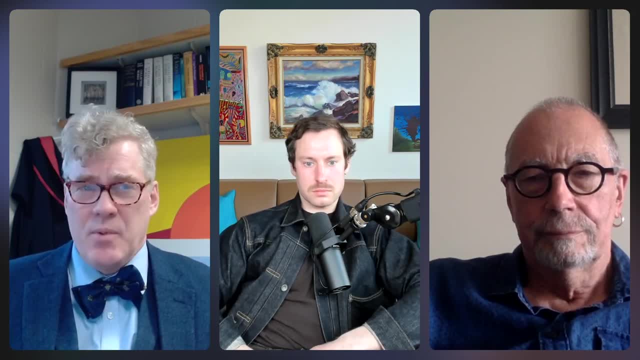 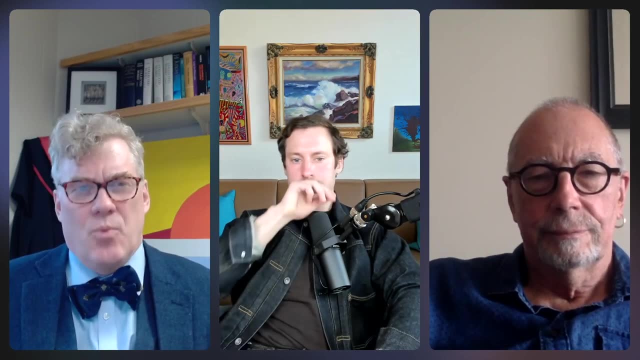 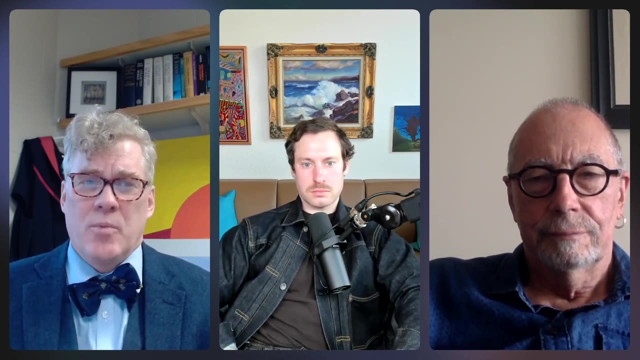 And they're all talking about that sentence- with that parameter and they're changing the parameter. So there's a sense in which it is still self-referential, because there it's just one formula with a variable that's changing And the formula is asserting something about that very same formula again at the later instances of that variable, which is still a kind of self-reference. 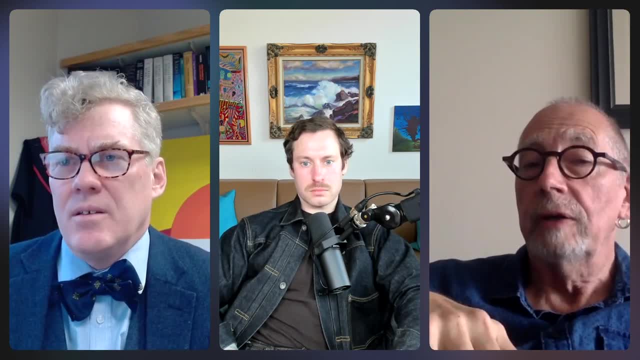 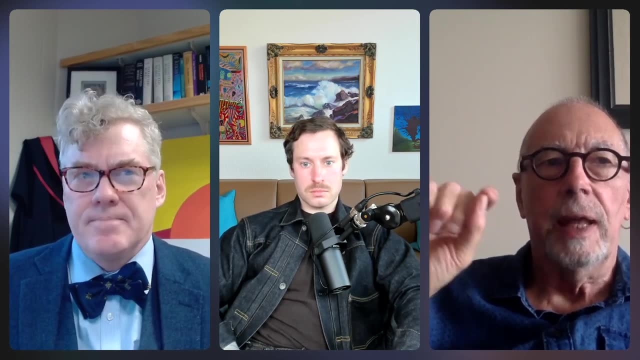 I'm not sure Joel and I are pretty much on the same page about this. Of course. I mean refresh rate doesn't use self-reference. But when you start to look at it carefully and how you actually formulate it, things which are distinctly self-referential start to appear. 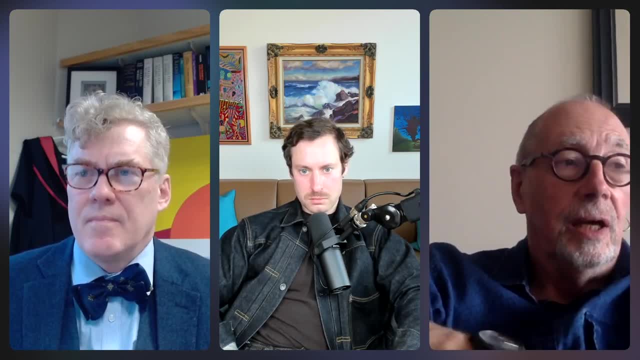 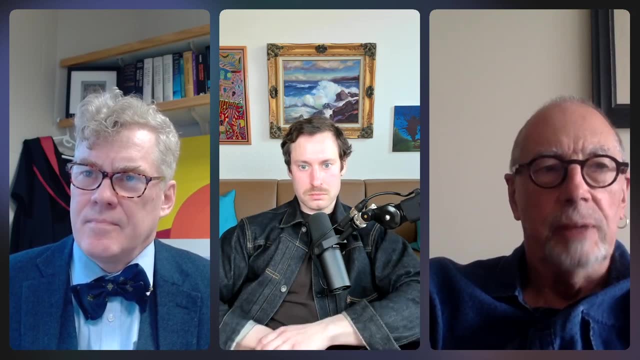 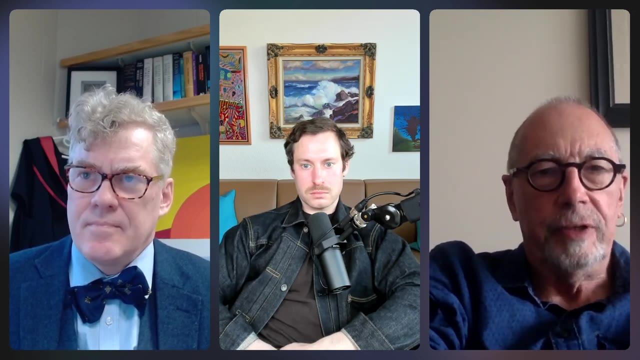 Yeah, So this is a contentious issue in the literature. Sure, What's at issue is exactly how you characterize self-reference, which is anything but obvious. But I mean, I think, when push comes to shove, Joel and I agree on what he's just said- 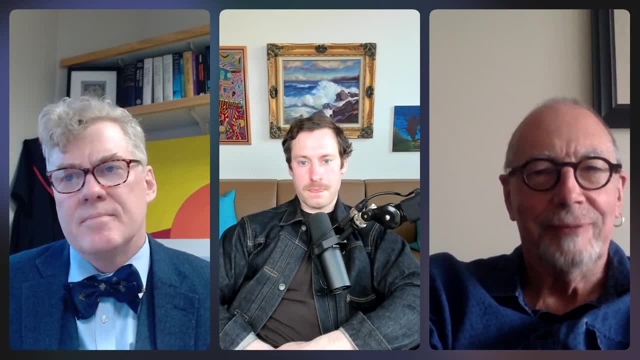 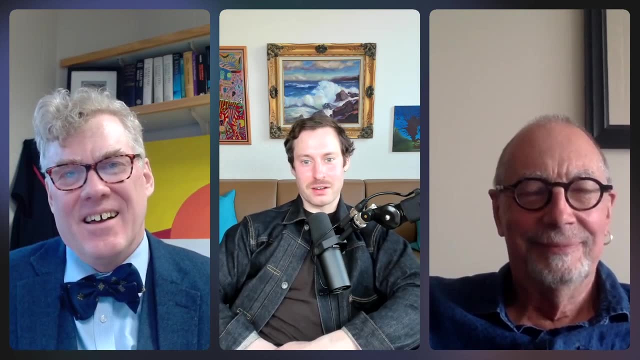 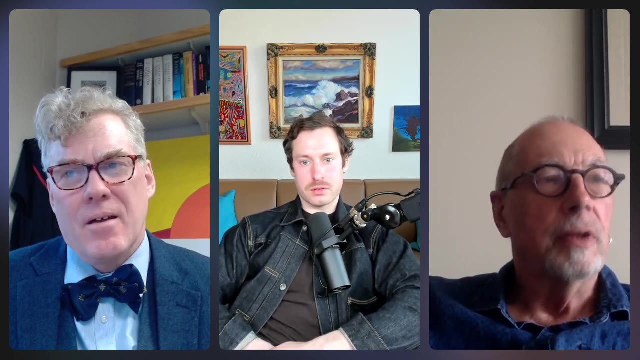 Yeah, I mean, I assume he agrees on what he just said. So Yablo's paradox requires then a different treatment for you, Graeme, than the standard liar paradox? Not exactly, No, Wouldn't you say that each instance is a true contradiction? 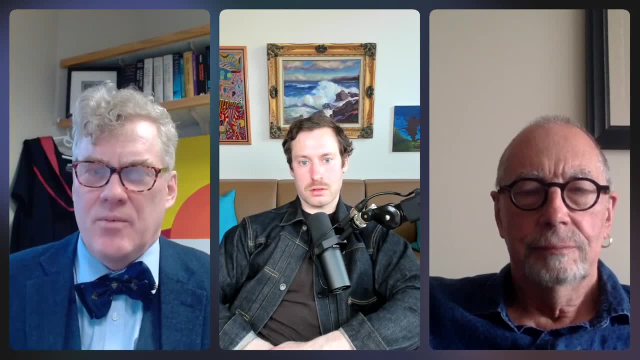 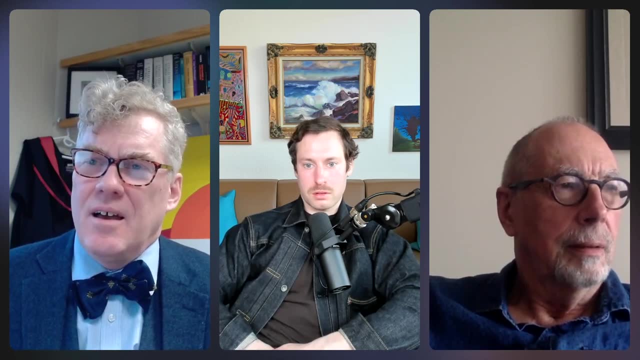 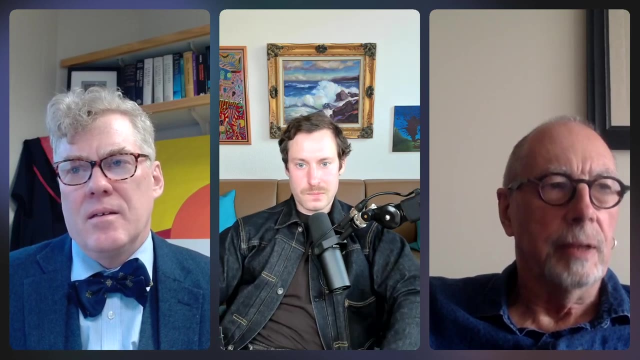 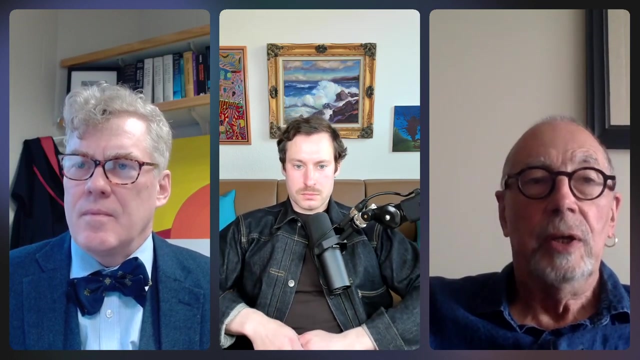 I mean, I would assume that would be your analysis of it, But please tell us So. it may depend on how you set the thing up. OK, But if you set it up in the way you did, essentially you've got an infinite bunch of sentences but only one proposition expressed by all of them. 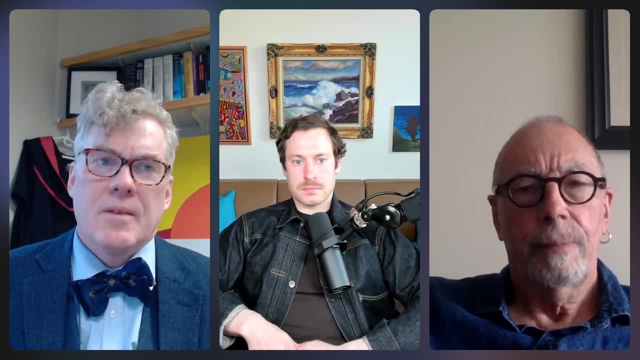 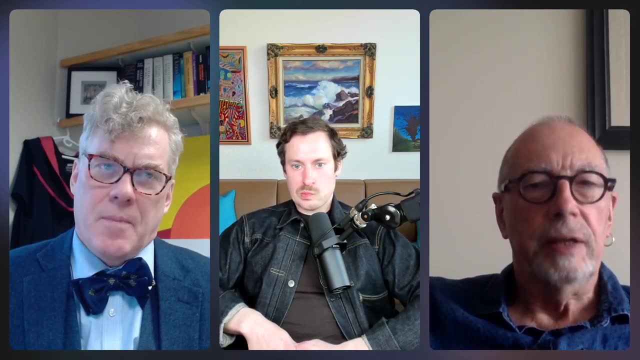 So you're back to the liar. I see Right. So you would say it's somehow equivalent to the liar. Well, I think it might depend on how you set it up. I think there was a math overflow question about this once. 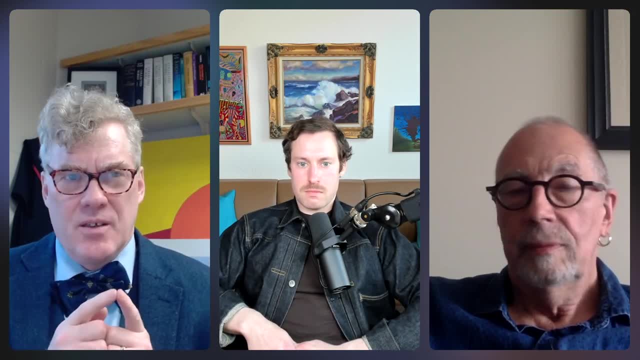 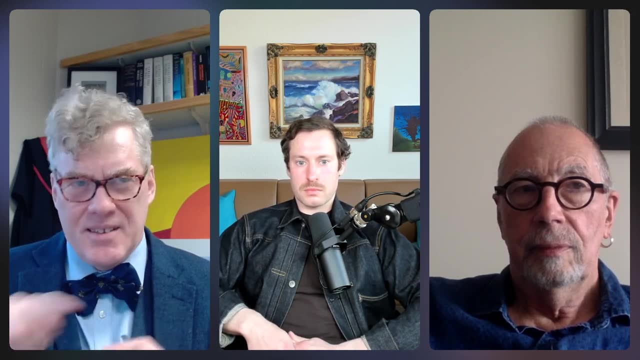 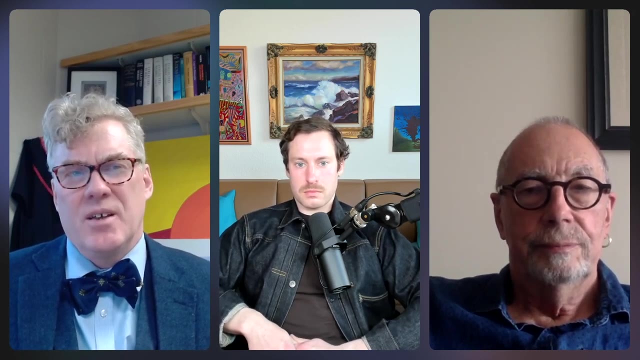 Because you can actually produce sort of instances of using the Carnot fixed point. You can produce a first-order formula with a T predicate that's somehow equivalent. It's expressing this Yablo thing, Yeah, And then in that case you can prove it's just. every single one of them is equivalent. 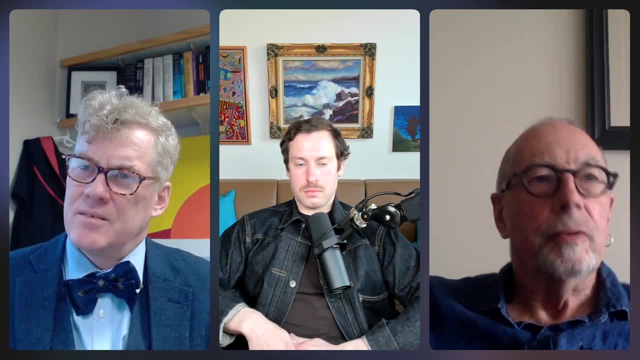 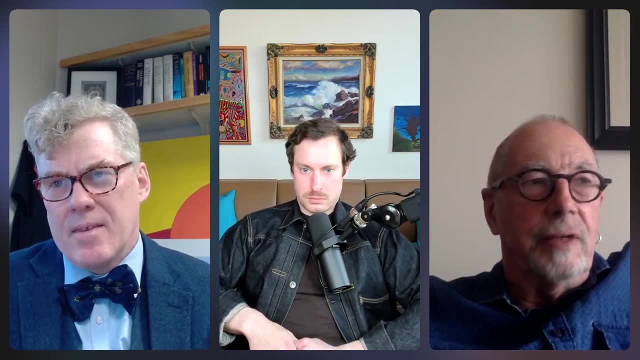 One of them is equivalent to the liar theorem. This is true, But there are different ways of setting it up. I mean, for example, one is by Roy Sorenson, And he says: hey, imagine you've got this infinite line of people right? 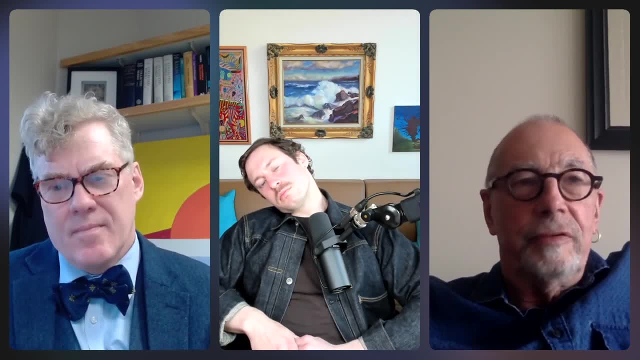 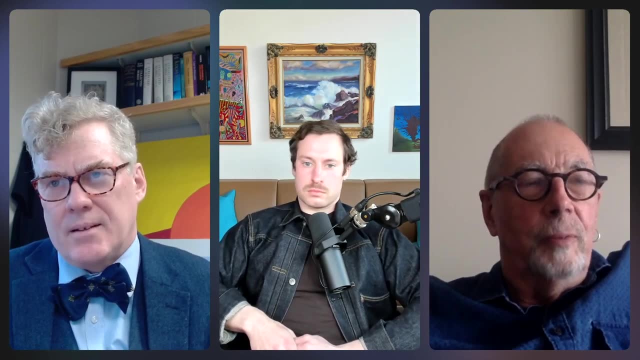 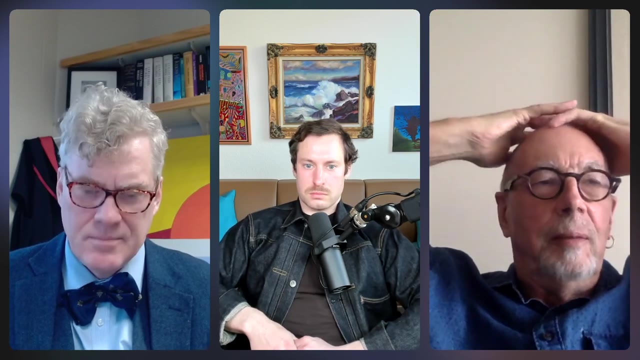 And each person says that is a sentence And each sentence is of a form, So give them all names, right. There's person one, person two, person three And person N says the sentence that person N plus one says is false. 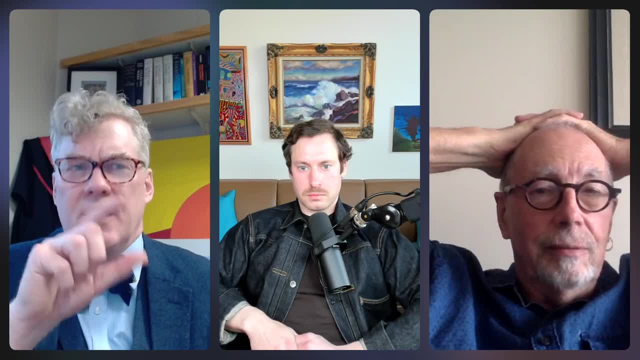 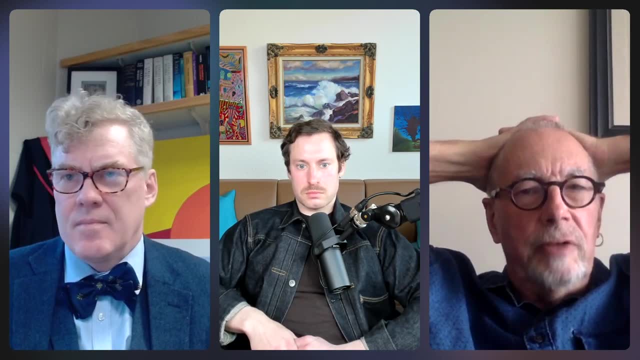 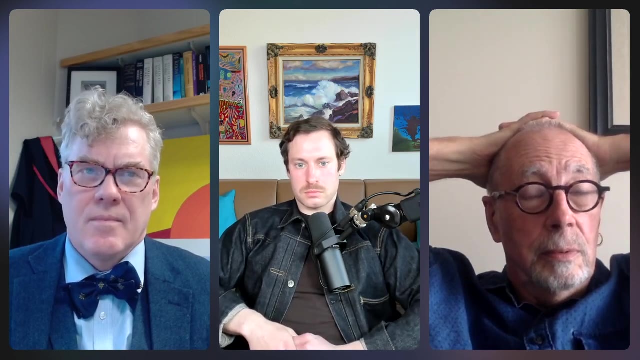 So just making it to the next one, So each of them says the next guy's Correct, Correct, And then it doesn't look like the same sentence or the same proposition because each of them refers to a different person, Right? So, as I say, you can set the thing up in different ways. 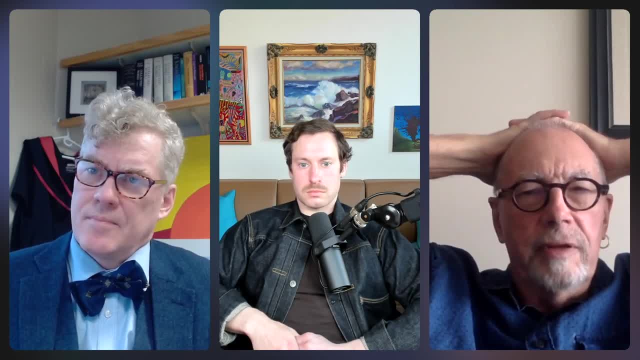 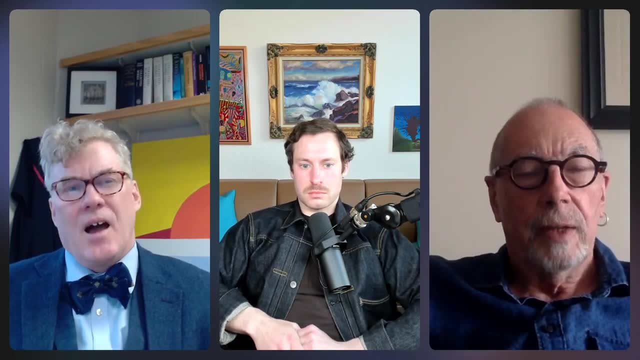 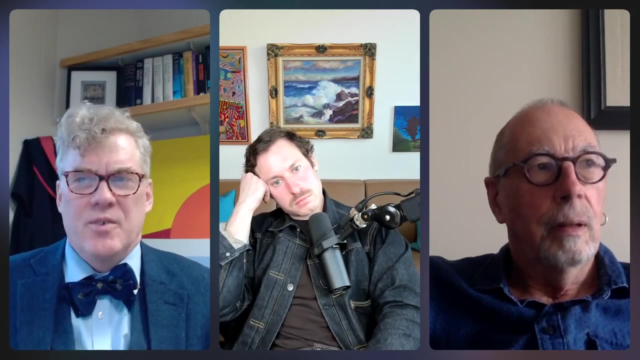 And you may want to say slightly different things about each context, each setting up, as it were. Right, That's interesting. I would want to know, you know, is there a sort of consistent solution of truth assignments to these sentences that is going to fulfill the T schema and so on? 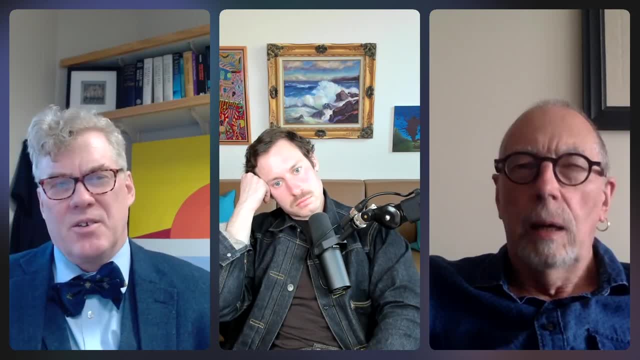 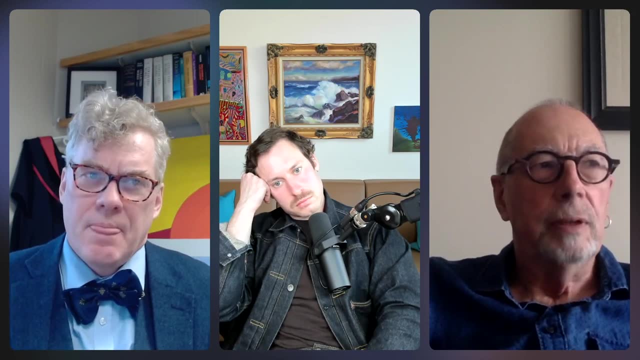 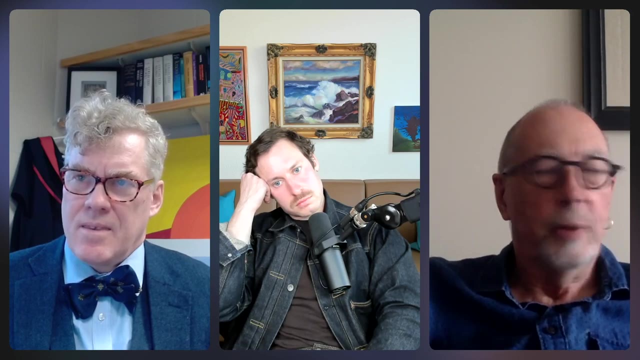 And I guess if it really is paradoxical, then the answer would be: there's no consistent way. I think, any way you lined it up, you're going to hit the possibility of power consistency Right, But of course there are the other ways out of it too. 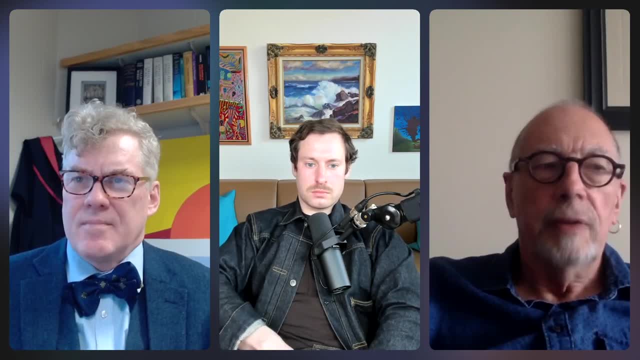 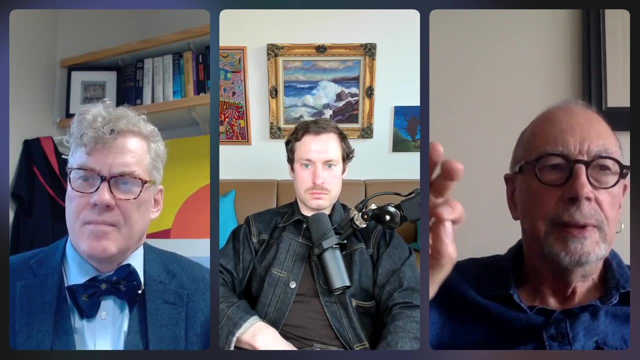 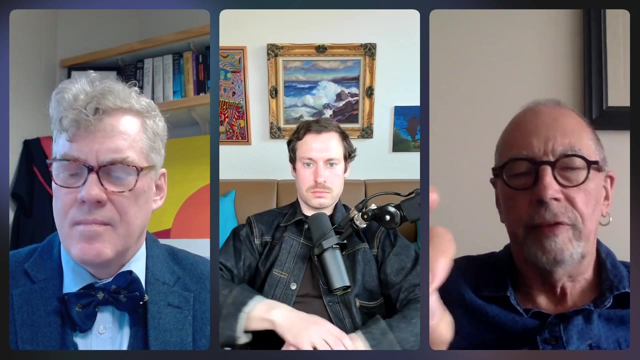 So I mean, I don't think that the Yablo paradox actually brings anything new to the table. It might appear to, But when you start to examine it in detail, I think we're in very familiar territory here, And I guess that's one of the things we agree on. 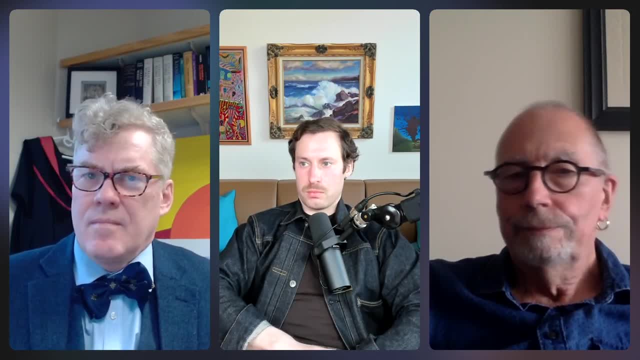 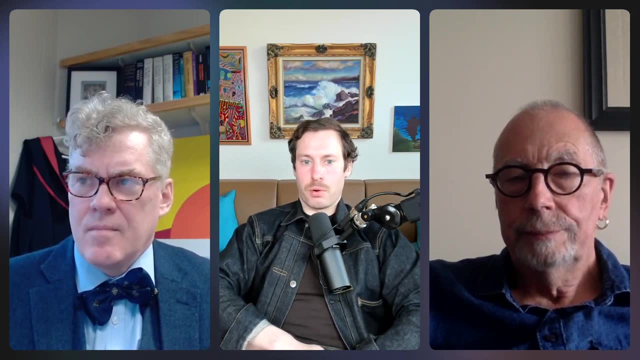 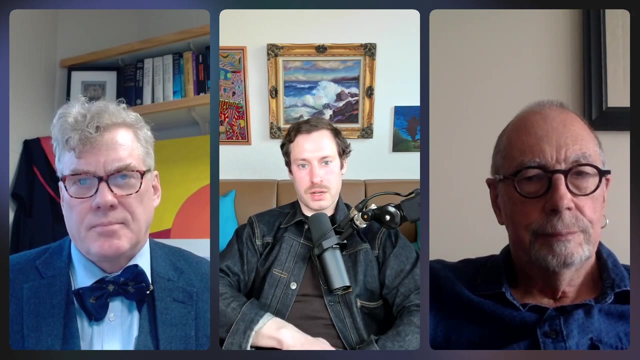 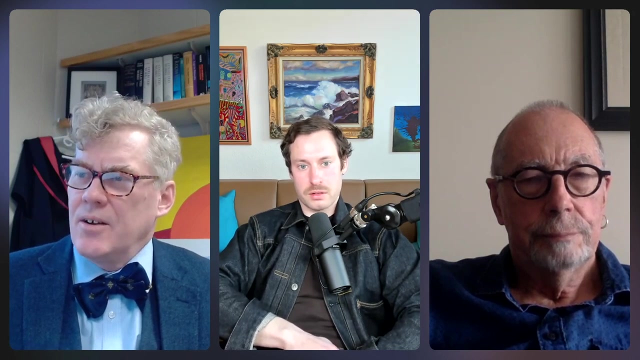 Now stepping back, I guess, to broader questions at issue here, Joel. what, for you, are the important stakes here, surrounding this switch in logic? Why are you so committing, So committed to retaining classical logic and avoiding going to pair consistency? Oh, I see, Right. 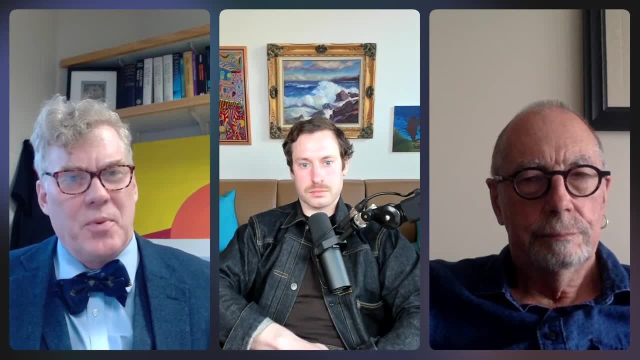 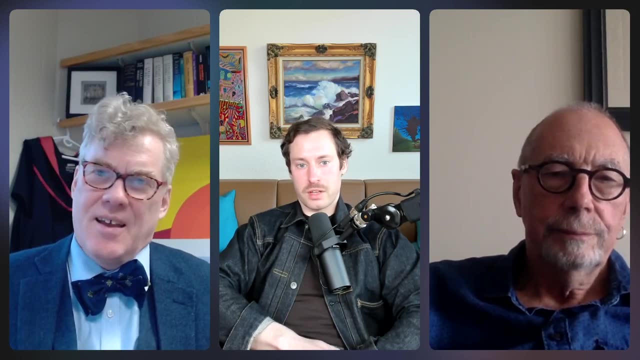 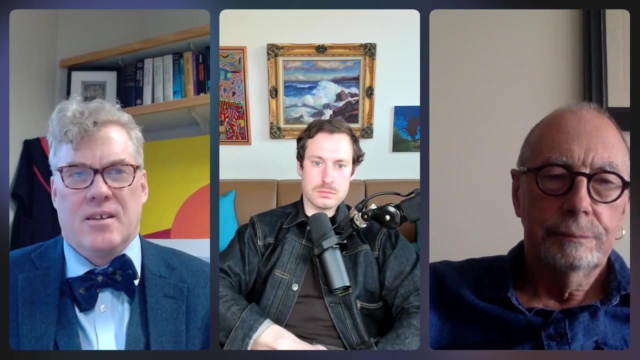 So I'm totally open to changing the logic. I mean, I don't feel that I'm, You just don't think it's the appropriate treatment here. I just haven't been convinced, And I mean, if, if I felt that the new logic was helping me to understand the phenomenon. 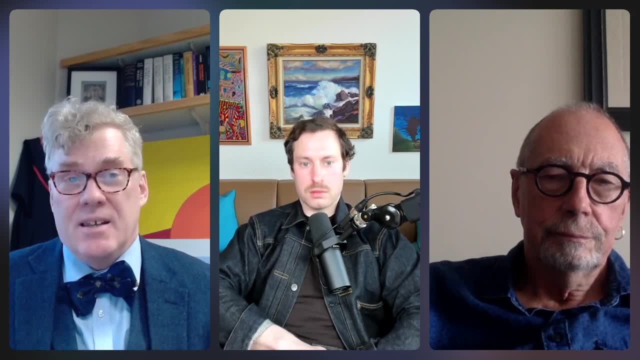 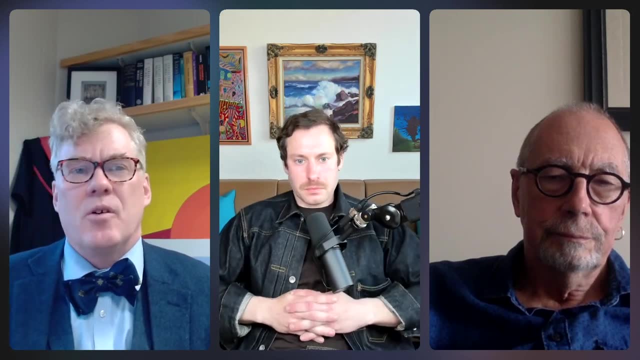 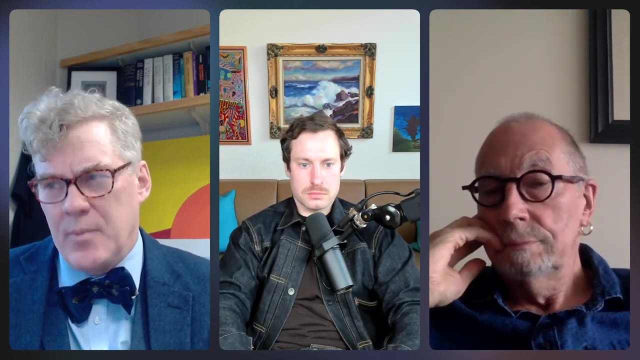 Better. And if I was getting insight From by considering a phenomenon, a mathematical phenomenon or you know, a philosophical phenomenon, in a different logic, then then I would be perfectly willing. And I mean, this is sort of the criteria. You know what is the criteria by which one chooses the logic. 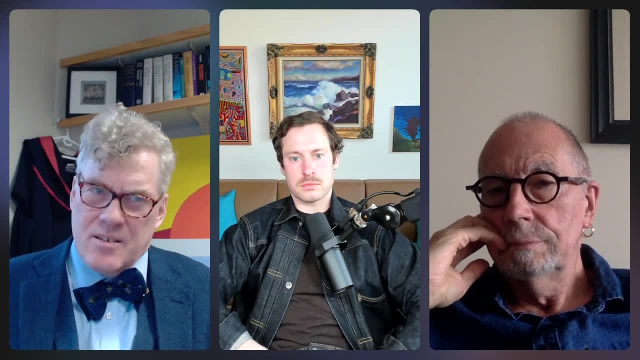 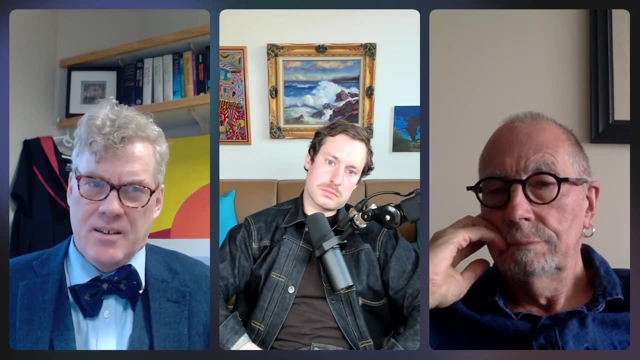 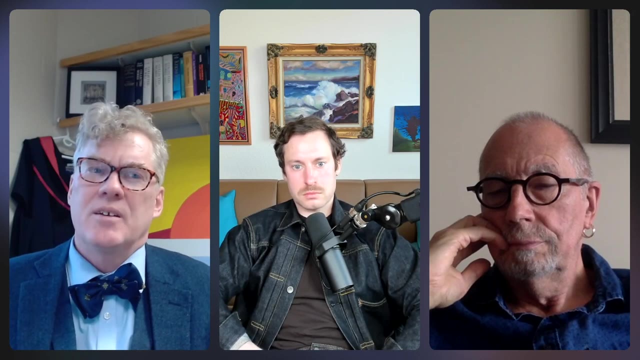 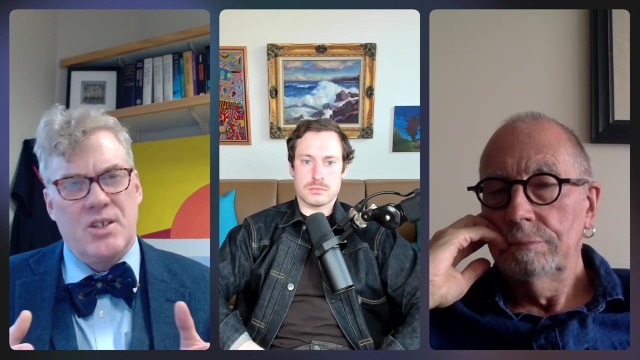 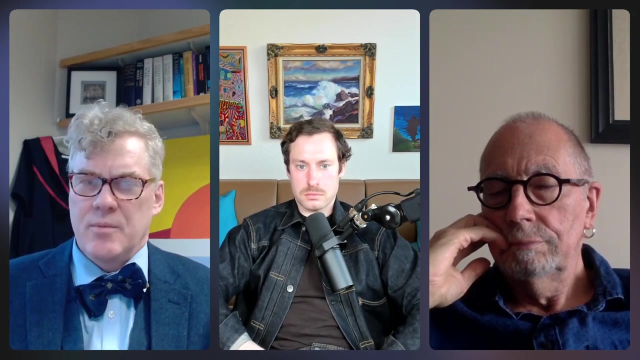 And, in My way of thinking about it, is that classical logic has been so Enormously successful and clarifying in helping us to understand how to reason in, say, mathematical situations- Let me just stick mainly with mathematical kind of situations- And and so then the question would be: well, are there situations where you would want to change the logic, say, to intuitionistic logic, or constructive logic, or consistent logic or something like that? 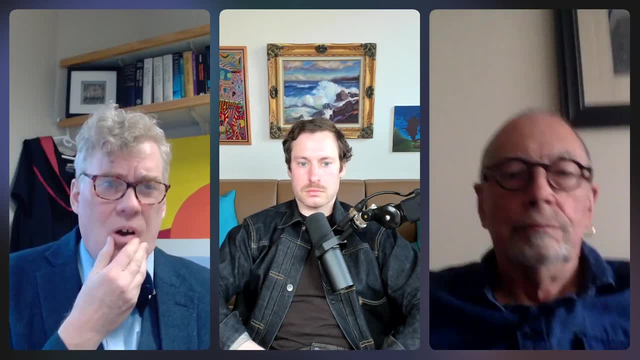 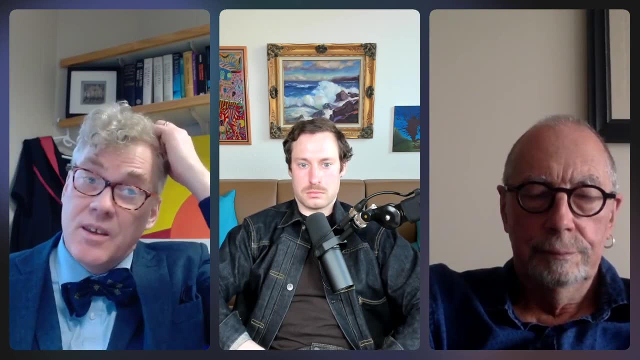 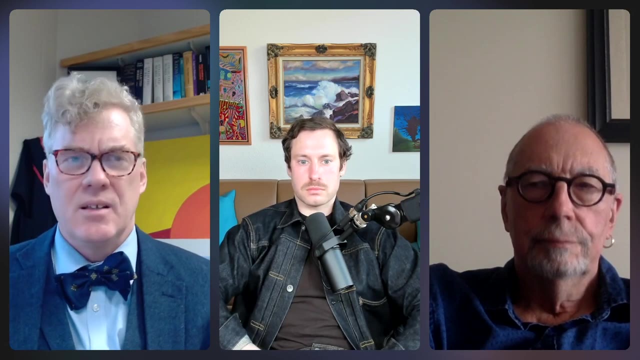 And there are some situations. For example, there are communities Of constructive mathematicians who are looking at topos theory and univalent foundations is a new big thing And you know, in those, some of those topos is the internal logic is not obeying classical logic. 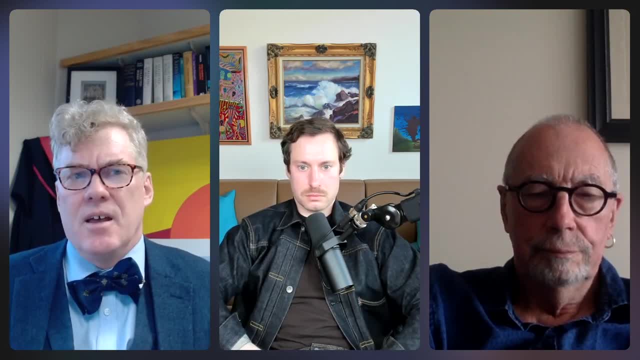 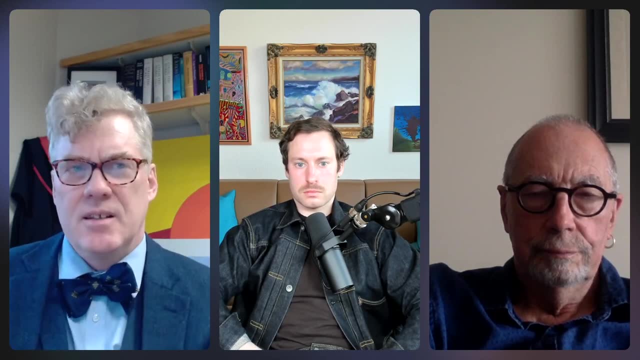 It's, it's obeying intuitionistic logic, And so the the practitioners, the constructive mathematicians who are, who are working and studying these topos is are using an intuitionistic logic and getting quite good at it, And And there are big communities of people doing that- 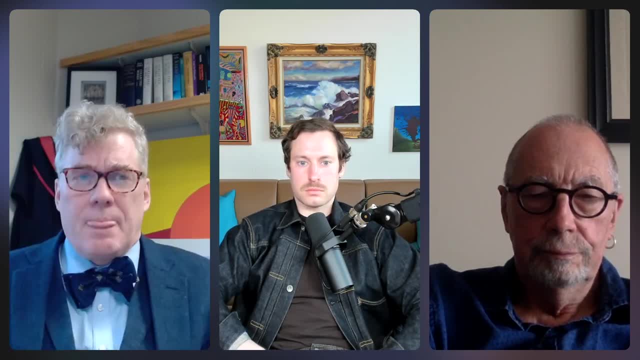 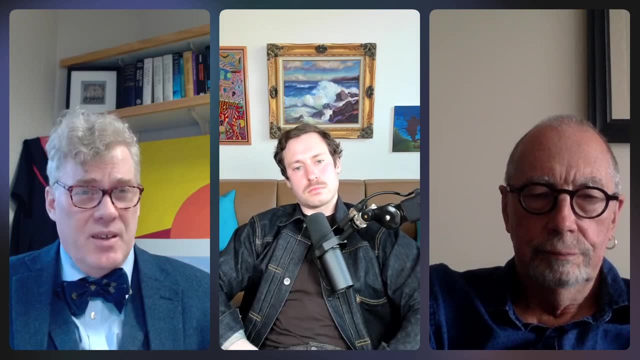 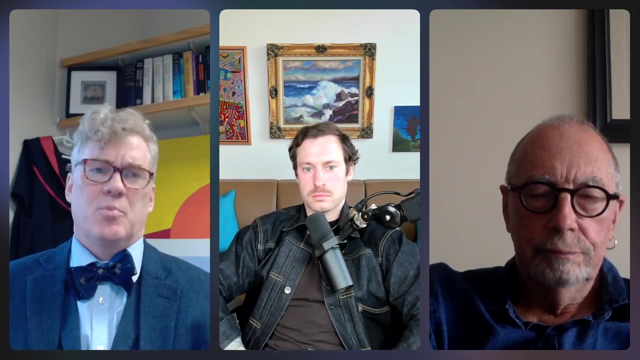 And And so OK, so from that point of view it seems perfectly reasonable to me for them to be working in intuitionistic logic in in those settings, because the intuitionistic logic is leading, is providing insights in how to reason about the truths of those mathematical structures. 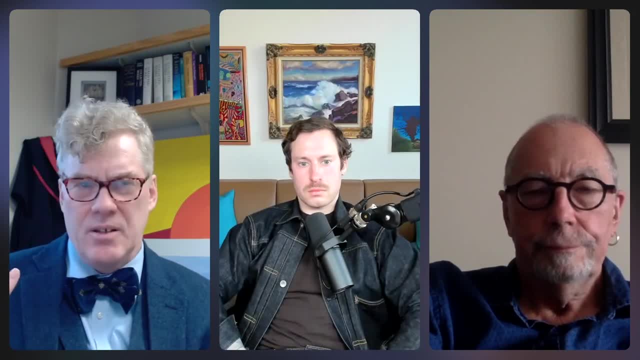 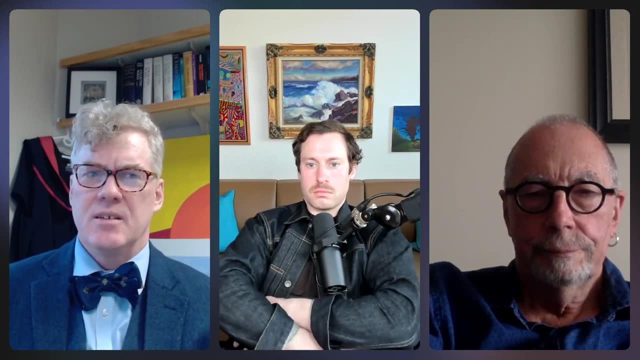 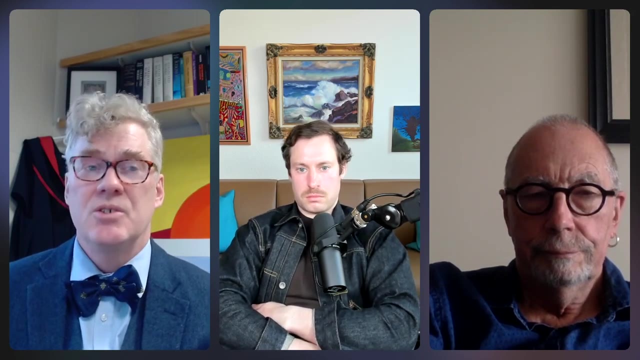 So I don't happen to work with those kind of things. I don't happen to work with those kind of topics is very much, And you know the kinds of mathematical questions that I'm interested in generally don't give rise to those kind of mathematical structures or universes in which the intuitionistic logic is appropriate. 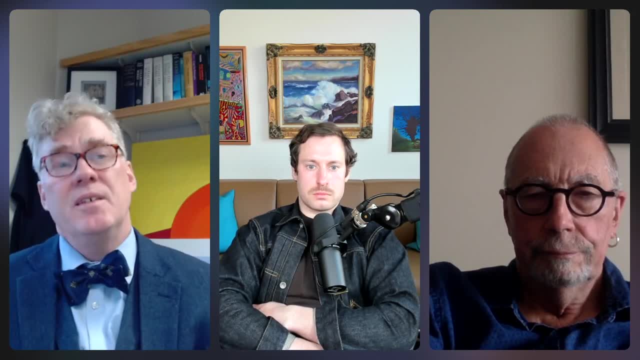 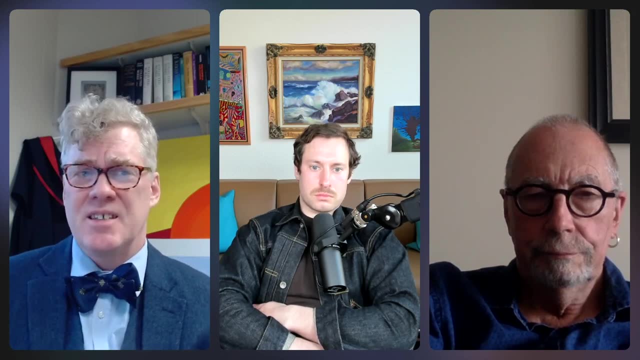 And so so it hasn't happened to me yet that I've come to understand the mathematical phenomenon better by thinking in terms of intuitionistic logic instead of And. but you know, I mean, I'm open minded about it, I think, I hope I am. 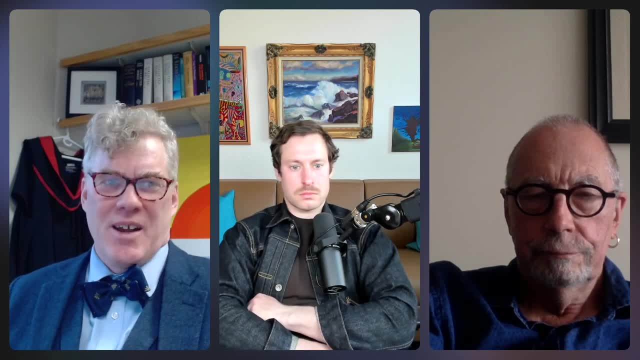 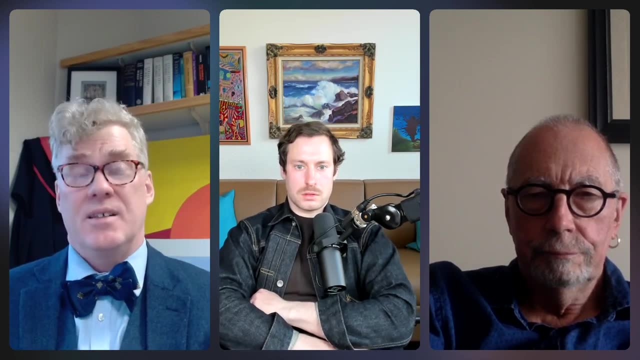 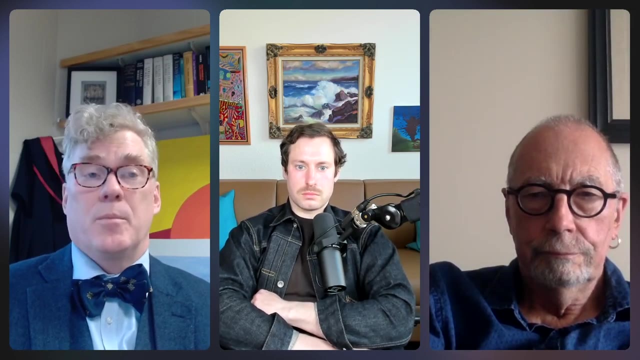 I mean, and, so I try to be, and maybe it will happen, And, and and. I guess I feel similarly about the pair consistent logic. I mean, if I felt that it was, You know, providing new insight of something that I wanted to understand, then that I'm perfectly willing. 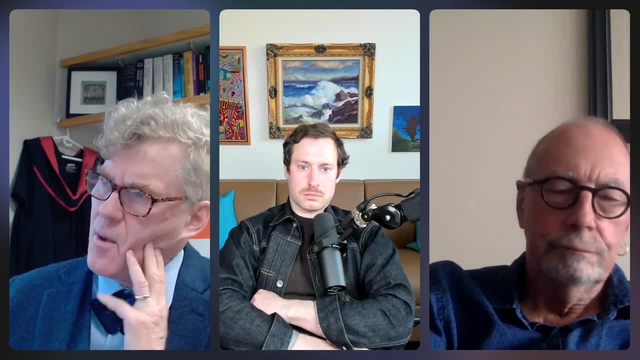 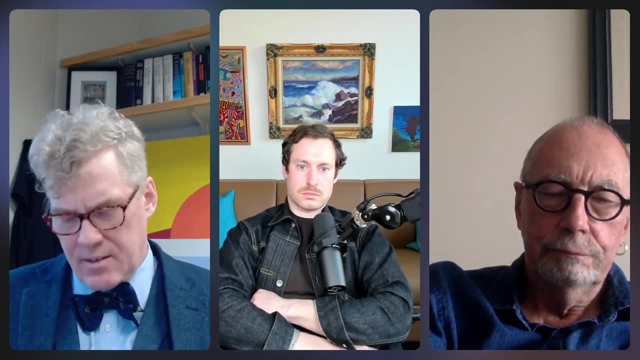 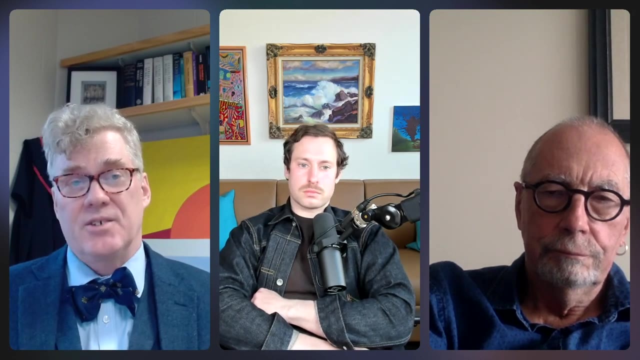 I mean there's another related thing which is OK. The sort of typical view of the comparison between intuitionistic logic and classical logic is that intuitionistic logic is viewed as a, as a part, a sub logic in a sense of classical logic, weaker, strictly weaker, because it's it doesn't have a lot of excluded middle, for example. 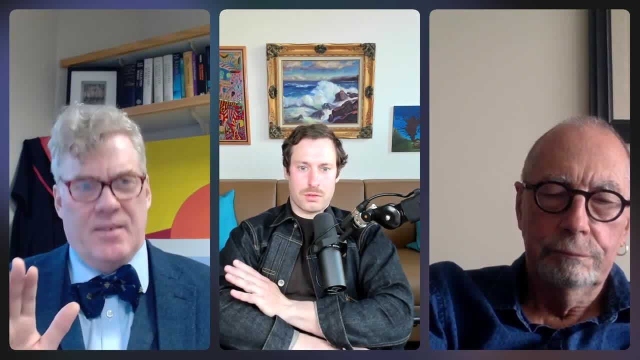 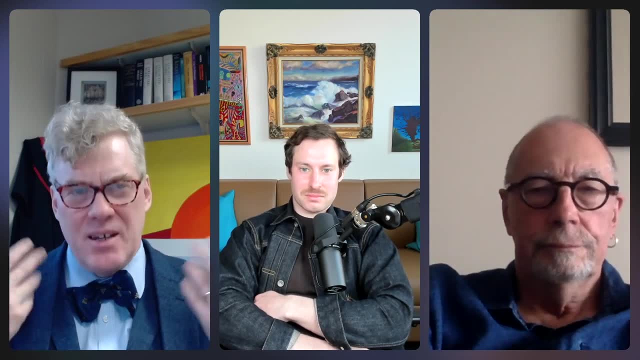 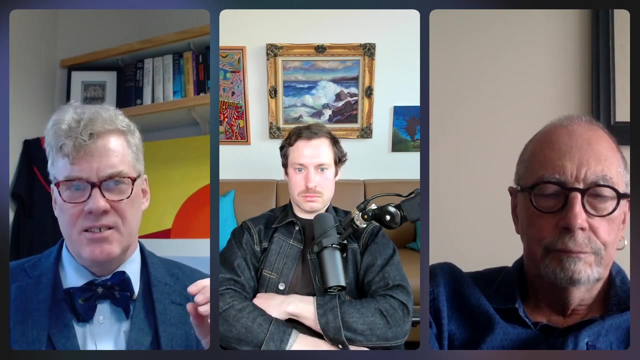 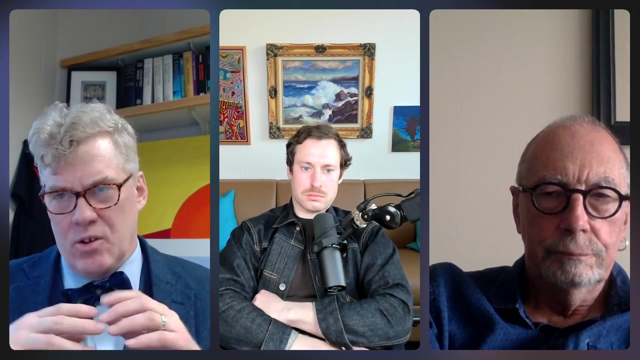 And? but isn't that not true? Hang on, Let me just get to this point, which is exactly that Classical logic is embeddable into intuitionistic logic by, for example, the double negation translation. So any assertion in classical logic, we can make a kind of translation of it by putting in, not knots at every level hereditarily into the statement. 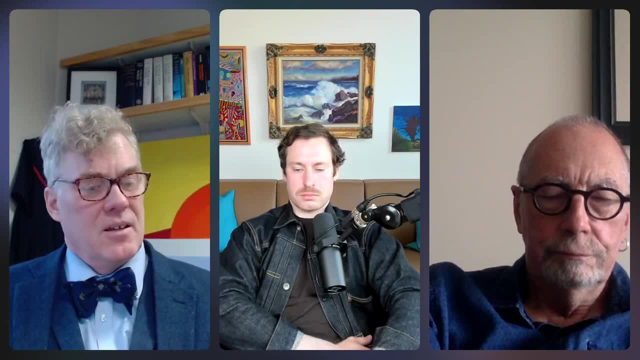 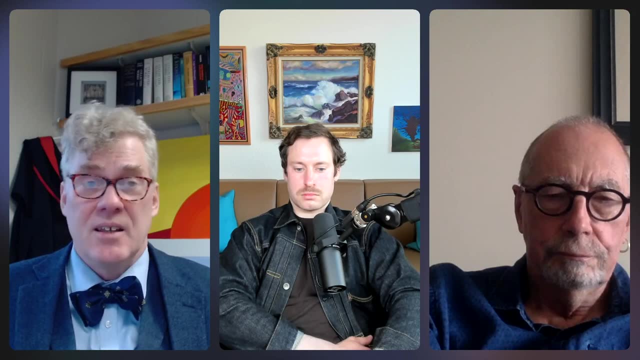 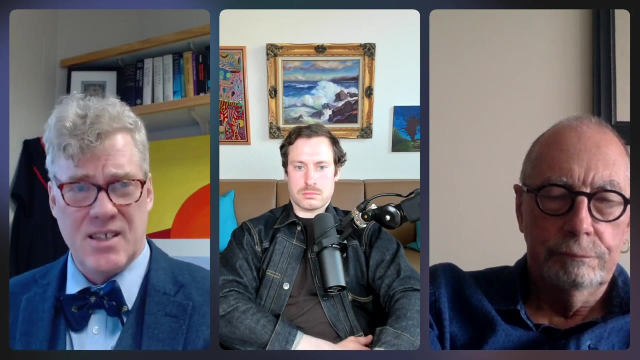 And then the the. the corresponding classical reasoning translates into something that's intuitionistically valid. But it's not. It's not with the same statement, It's with this translated statement. So for a memory statement fee you can make this double negation translation. 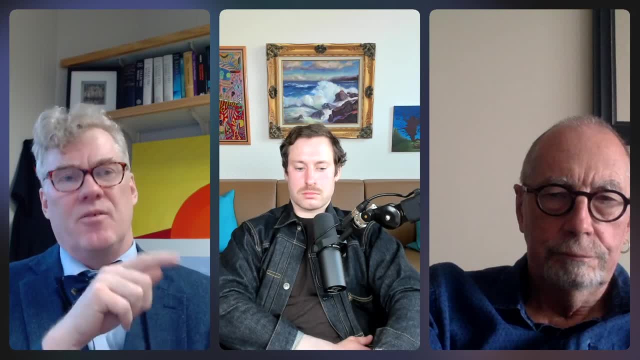 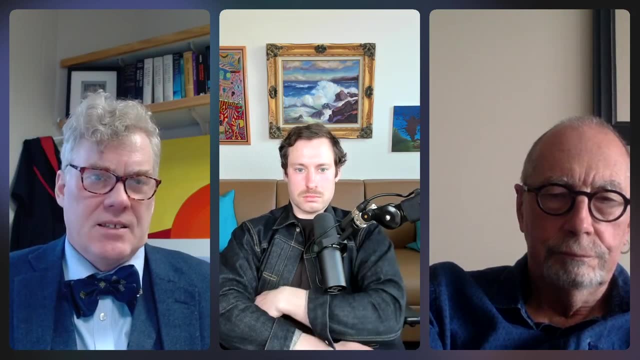 Let's call it: It's not just not, not fee, but it's not not fee and then not not stuck also hereditarily inside fee at every level. Right, That's the translation, And it's a translation that the classical logician thinks is totally fine. 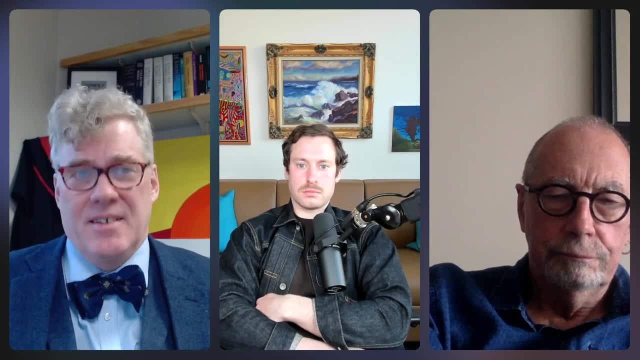 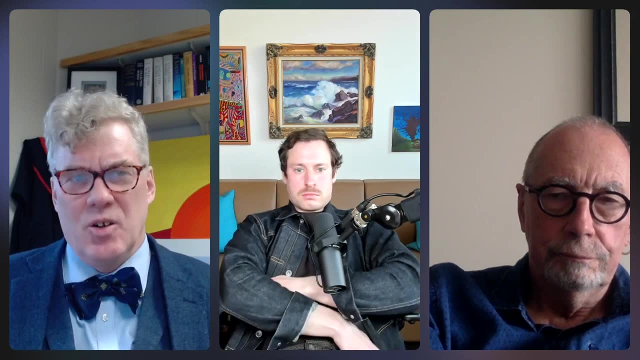 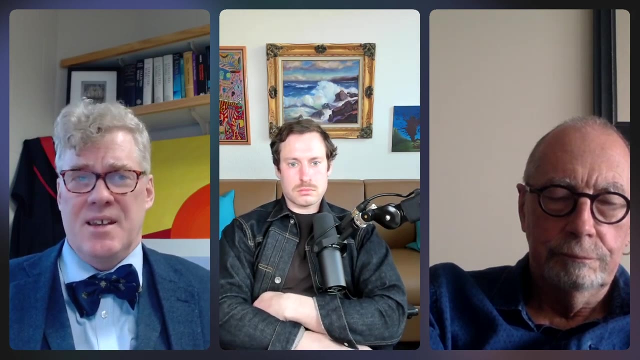 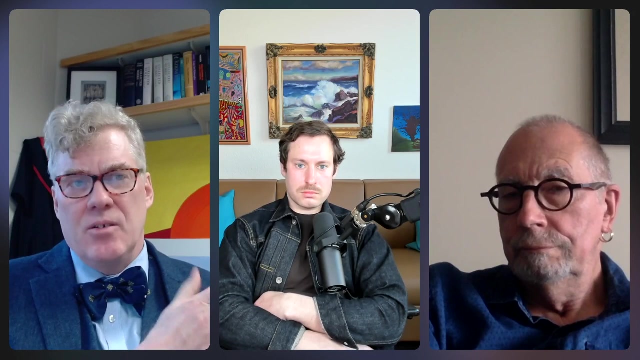 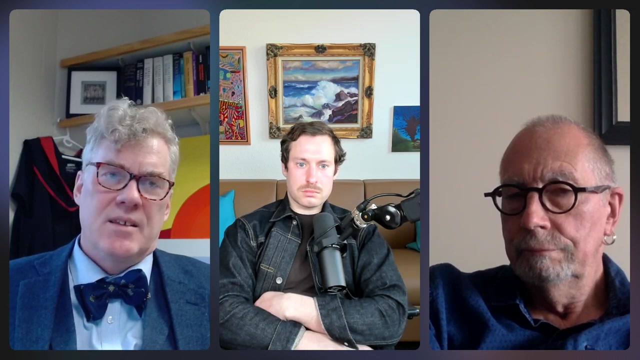 Right, Because saying not, not for a classical logic is, is to not do anything. And and so so the classical person, the classical logic person, agrees that the translated version is expressing the same content, the same semantic meaning. And yet, because of the double negation translation, then when reasoning about those translated statements, the intuitionistic logic can prove exactly the same things about those translated statements. 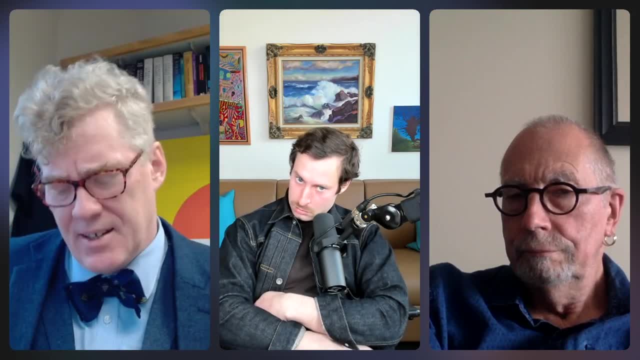 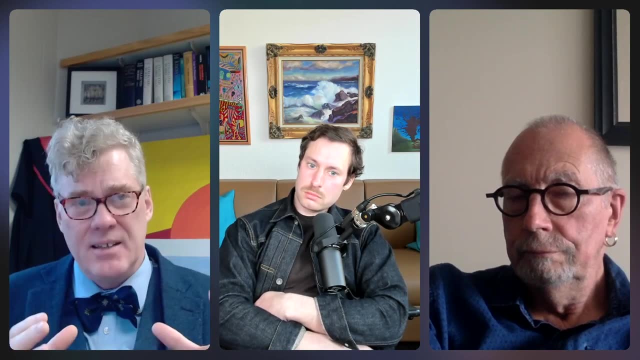 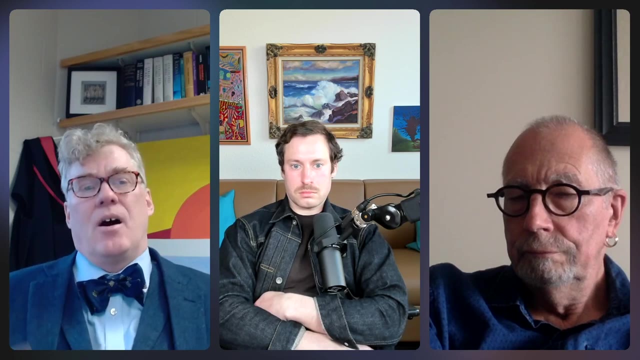 And therefore what I'm trying to say. What I'm trying to say is is that one can view intuitionistic logic as an enlargement of classical logic, because it contains this perfect interpreted copy of classical logic by the double negation translation, And yet it also has more. 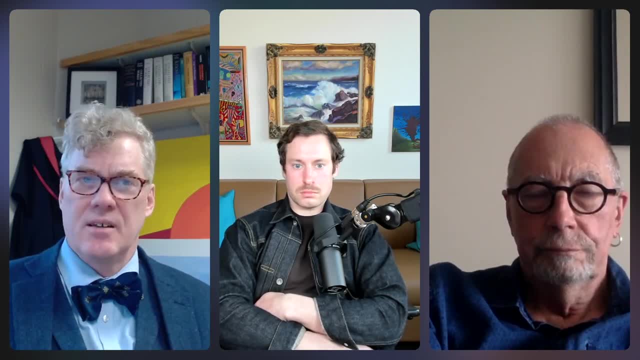 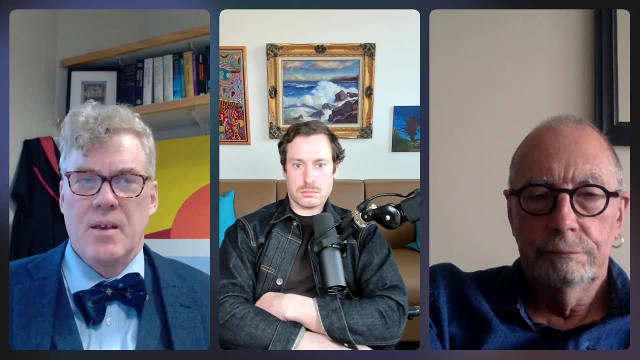 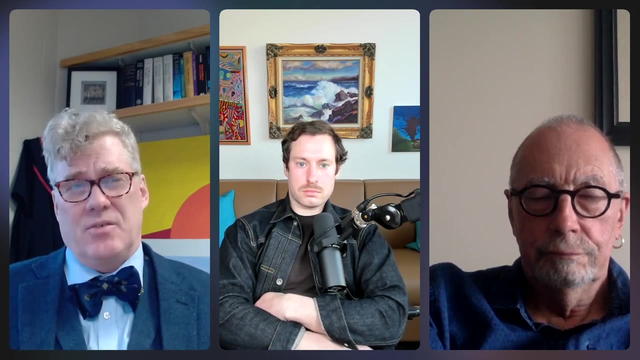 And so the point is that the assertions of intuitionistic logic- not all of them- are translations of classical logic, because not every assertion has this double negation form, And so it's a way of thinking. So it's a way of thinking about intuitionistic logic as an extension of classical logic rather than as a reduction of classical logic. 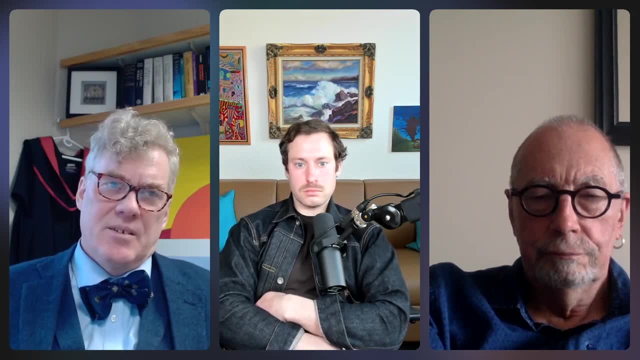 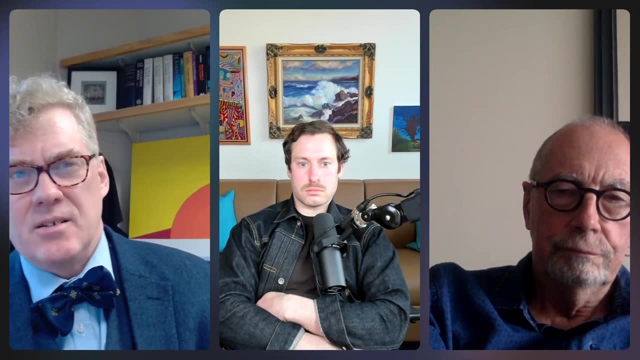 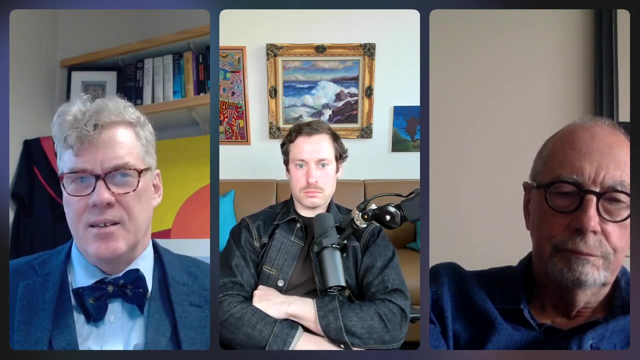 And I find that perspective extremely interesting because, In a sense, intuitionistic logic is more powerful than classical logic. because of that- And you can't translate the other way- I think this is true. There's no way of translating from intuitionistic logic to classical logic. 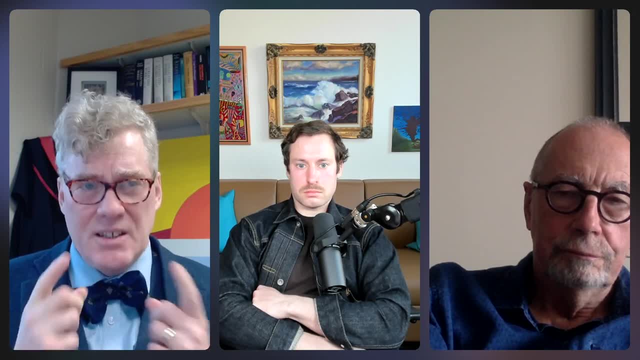 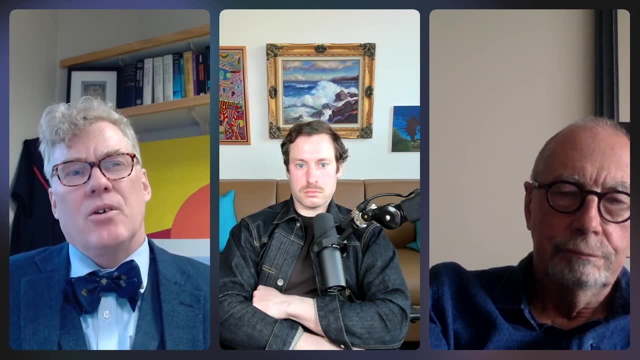 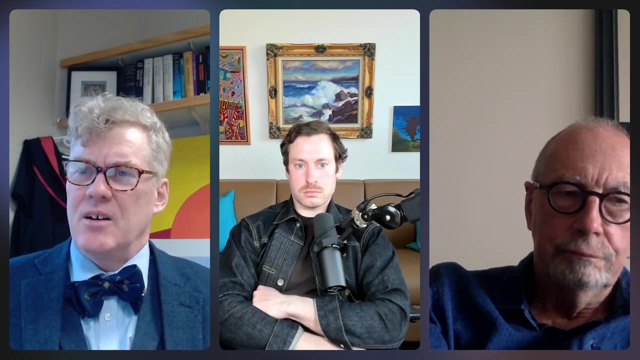 And so, in that sense, intuitionistic logic is strictly, Strictly, stronger than classical logic. If you are willing to make these translations, And I wonder, Graham, do you know anything about whether there's such a similar phenomenon for pair consistent logic, or can we? 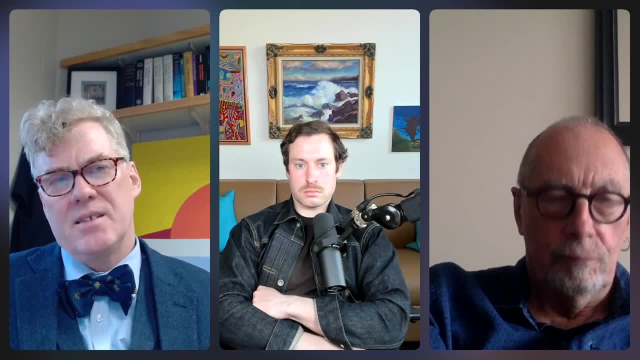 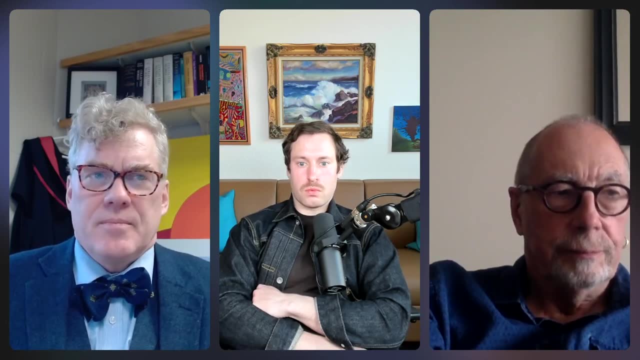 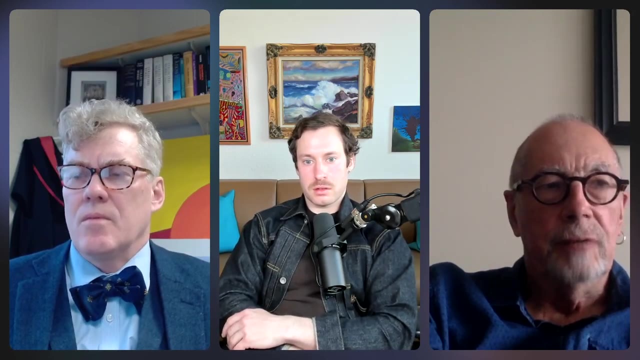 I'm not quite sure how to think about the pair consistent case in that respect, I mean, with respect to that phenomenon. Do you know anything like that? Well, Let's distinguish between pair consistent logic and pair consistent nothing others. Well then let me just say, of course, once you've got any logic, there are millions of ways of translating it into other logics. 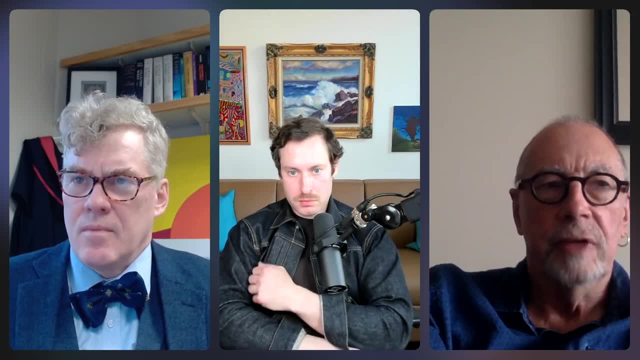 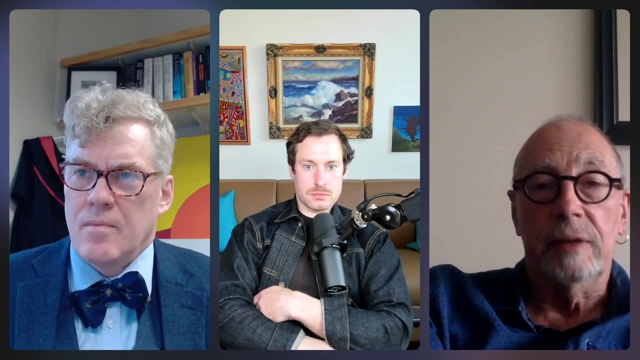 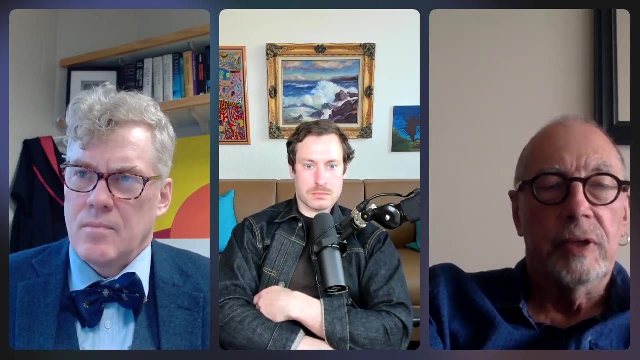 There are all kinds of translation results at the level of first order logic And you can certainly find these translations. The situation is messier when it comes to pair consistent nothing others, And We know that there are lots of inconsistent theories which require 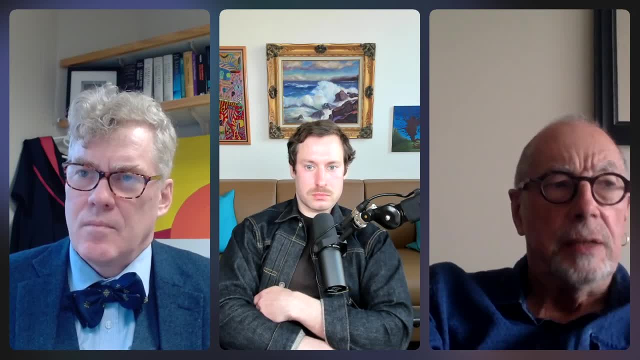 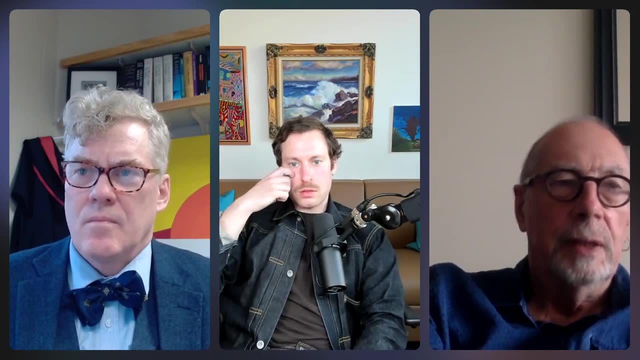 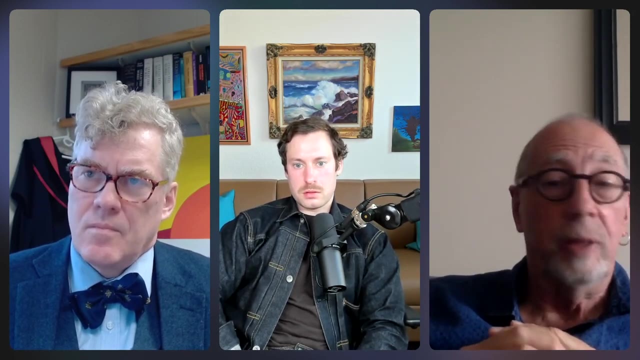 A pair consistent logic, otherwise all hell breaks loose. And it's not so clear that those can be translated into something that's classically kosher. Again we hit the problem that you've kind of alluded to of what is a legitimate translation and what's just playing the cymbals. 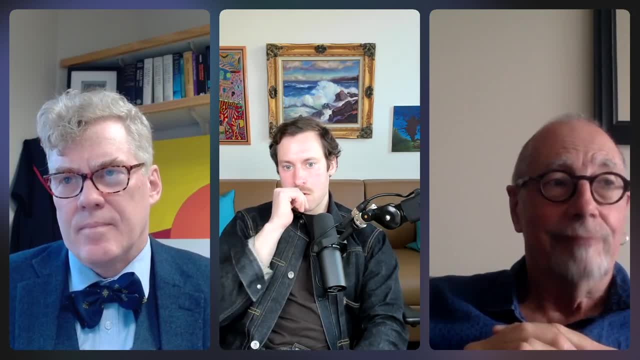 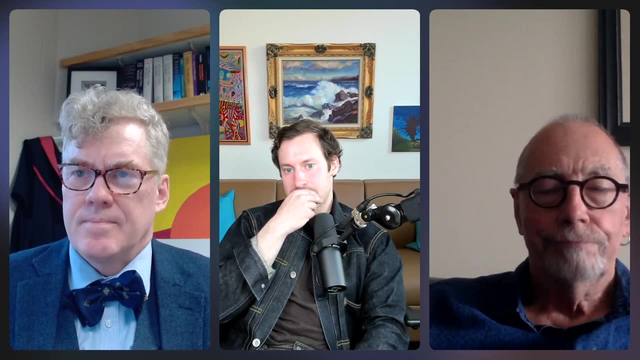 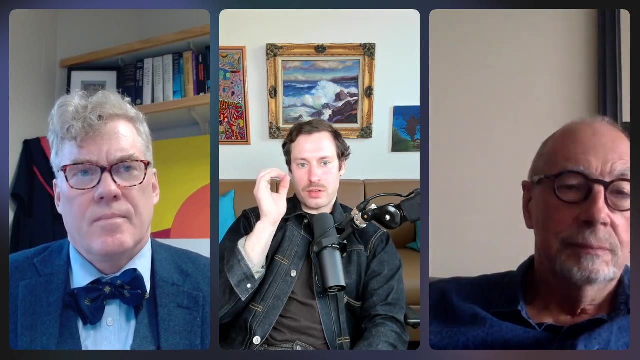 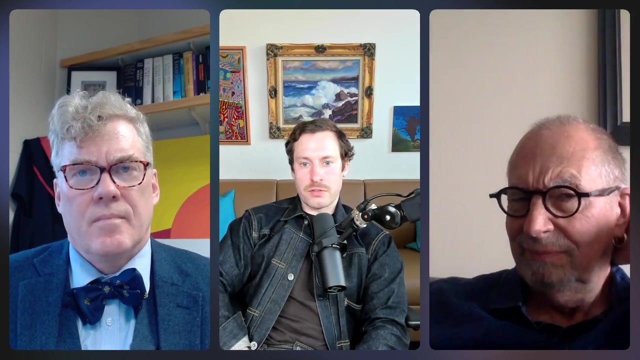 And that's something that's A feature of some of the literature in philosophical logic in the last 20 years. So, Joel, what you just said with regard to switching logics I found very helpful, And I'm wondering if it's pointing to a salient difference between your two views on logic. 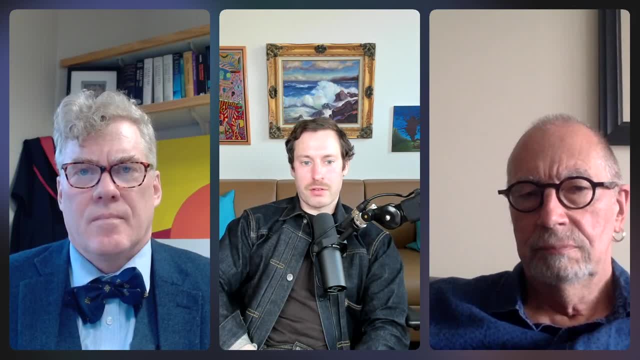 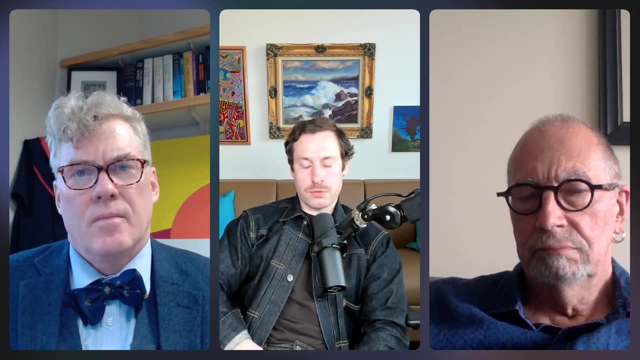 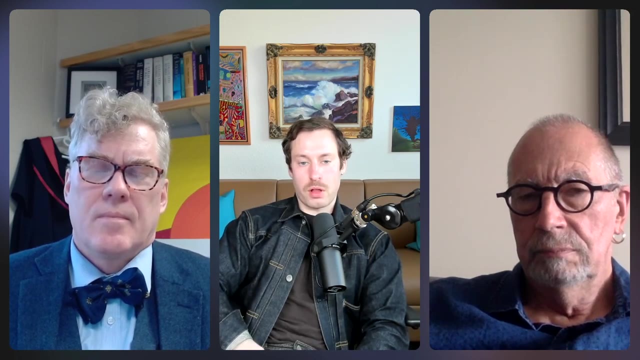 And I just want to make sure that I have it right. So, on the one hand, Joel, you pointed To insight and fruit and fruitfulness as criteria maybe for selecting which logic to work with, whether it will help with, say, mathematical reasoning or whether it will shed light on 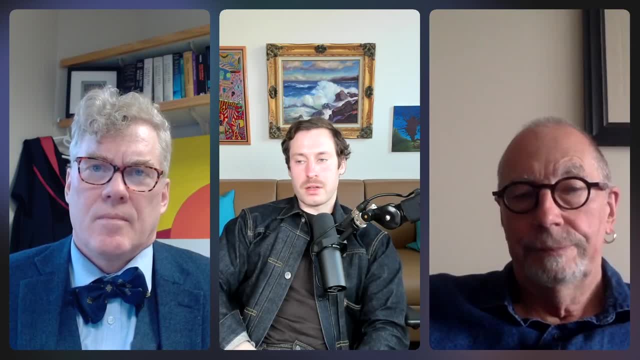 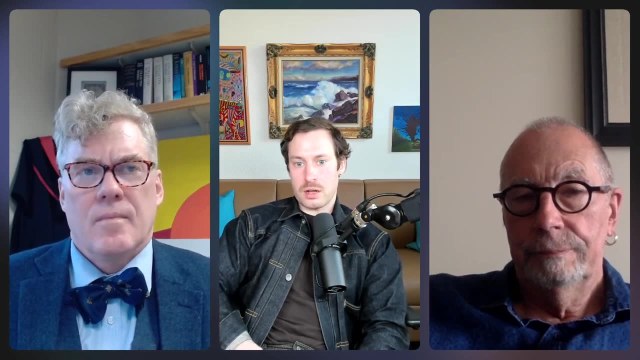 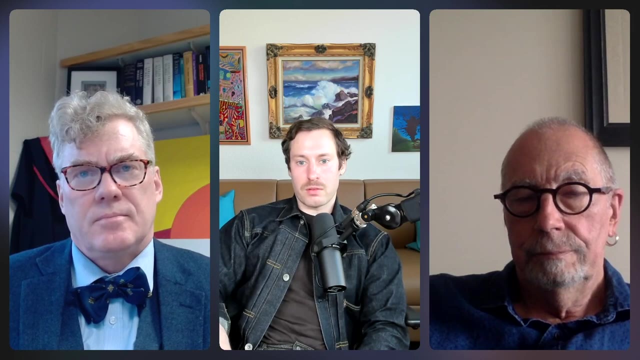 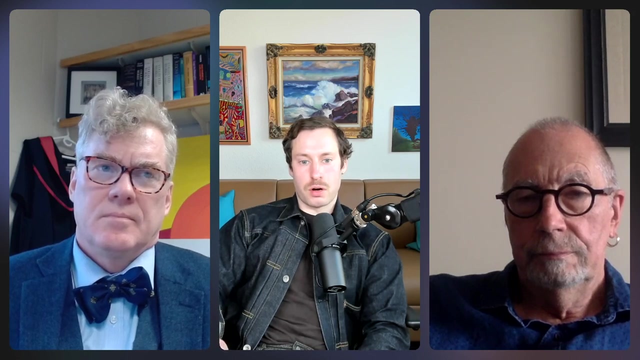 The liar paradox. But Graham, in Expressing sympathy for the view that there's one true logic pair, consistent logic, That strikes Me as Some sort of- Maybe even like a metaphysical thesis about logic, whereas Joel's view is more. 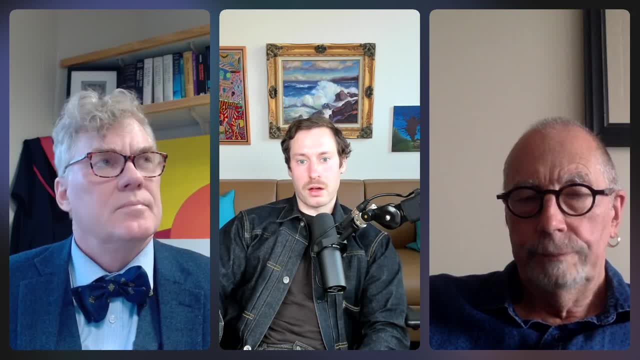 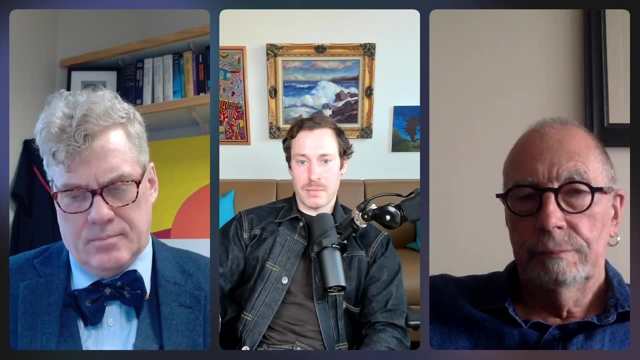 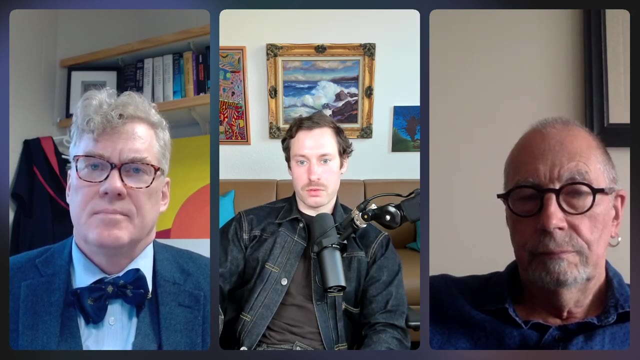 Instrumental. I mean. logic is a, is a way of reasoning, And maybe it's it's deflationary in a way, about what logic is. And I wonder if- if I'm making sort of An apt observation or if I'm misconstruing either of your views here. 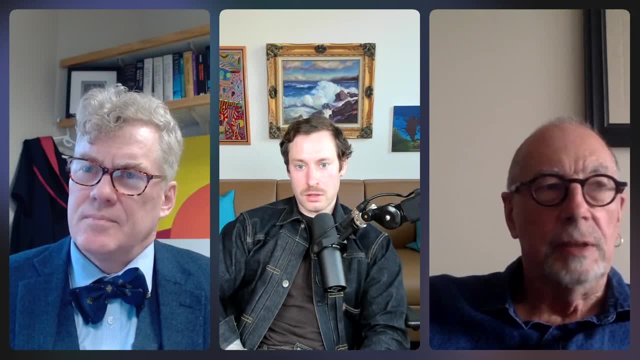 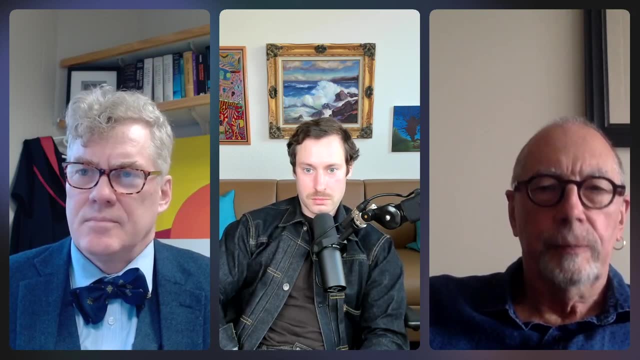 Well, I'm not entirely sure what your view is about these things, Joel, And what I thought I heard- but maybe I'm wrong- is some kind of clueless position. You know, there are lots of good logics and you just 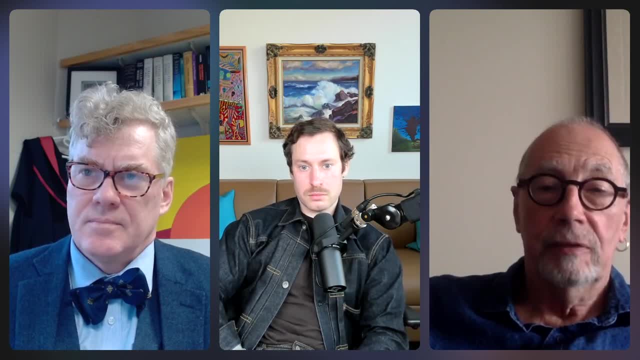 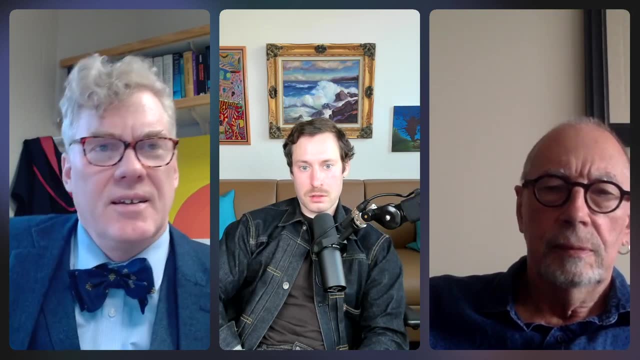 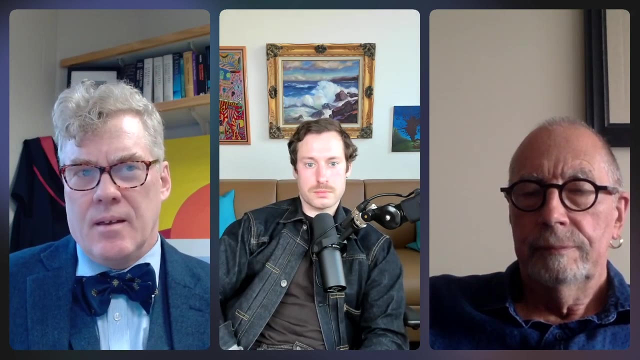 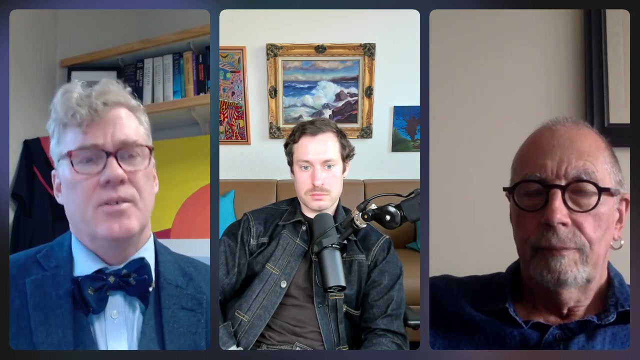 Do whatever you want, which you feel is correct. But am I mishearing? No, I mean, of course I am a pluralist about these things, But what I was expressing before is that There are communities of mathematicians who are using constructive mathematics and intuitionistic mathematics and so on, and even some very consistent mathematics. 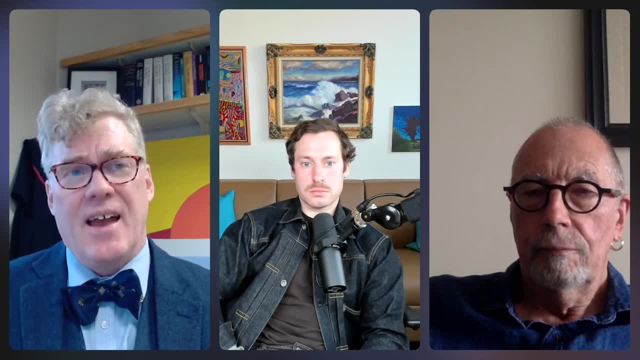 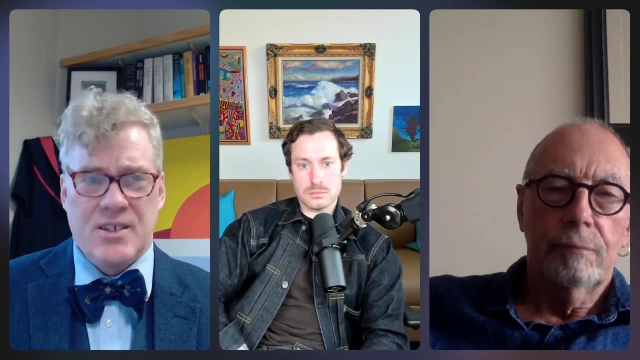 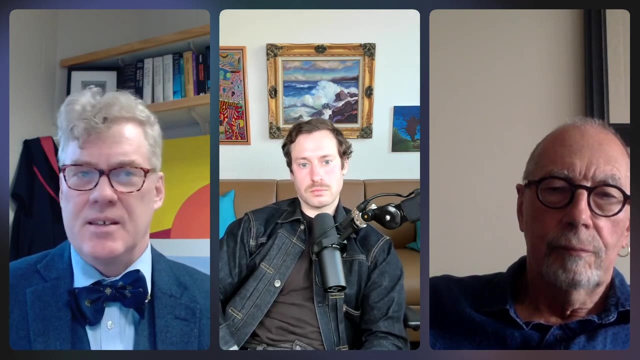 And- and personally I haven't had the experience of coming to some mathematical insight by by weakening my logic, And the questions in which I have been interested don't seem to be benefiting from this kind of change in the logic, And so I don't know if that makes me a pluralist or a singularist. 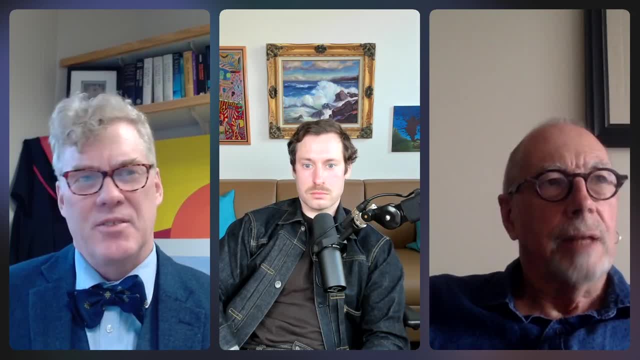 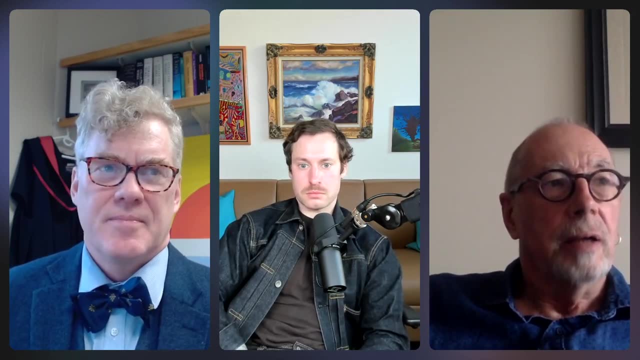 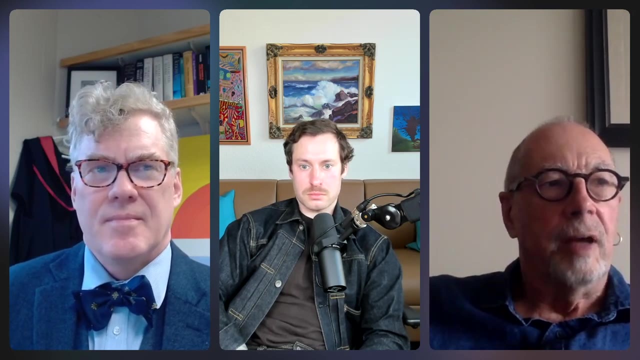 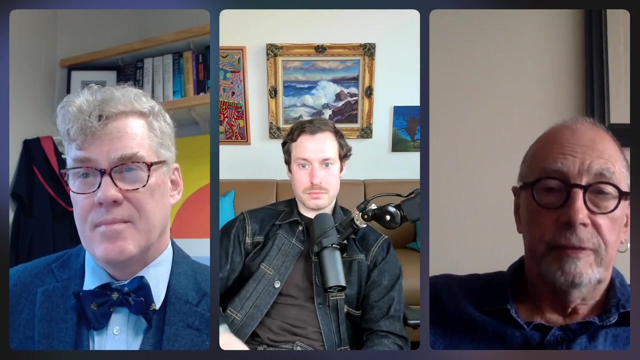 I'm not sure About the logic. Well, in one sense, yes, In another sense not necessarily. I mean, I mean, this takes us to the question of mathematical pluralism, Right, And I'm inclined to think. they're intrusionist structures, paraconsistent structures, classical structures, which all have mathematical interest. 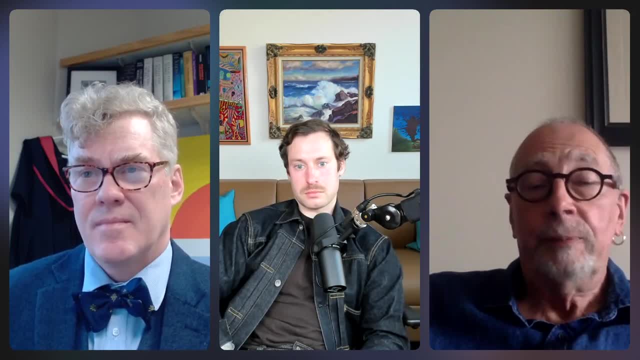 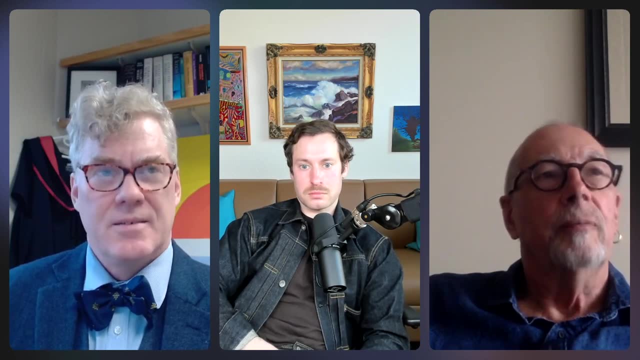 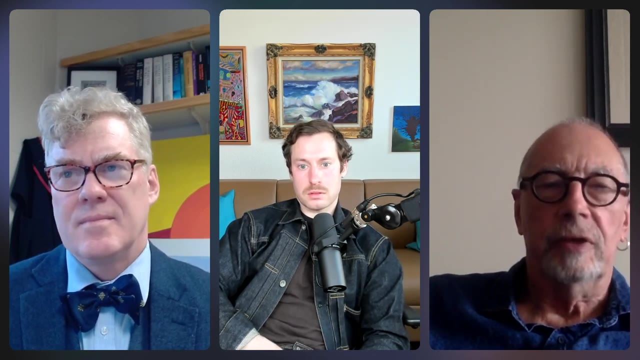 And, of course, if you're reasoning about an intrusionist structure, use intrusionist logic and so on. So I think we're on the same page there. Yes, But reasoning about truth in a structure or what preserves truth in a structure is, of course, not the same as reasoning about what preserves truth, simply. 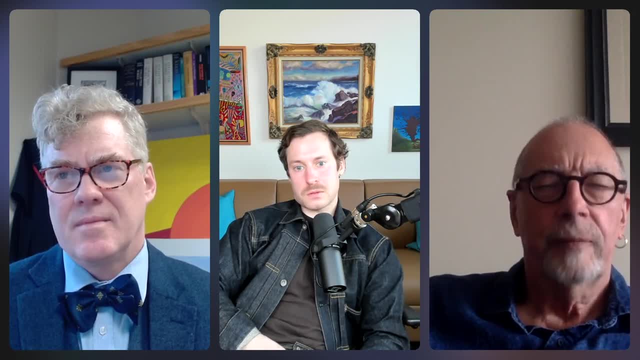 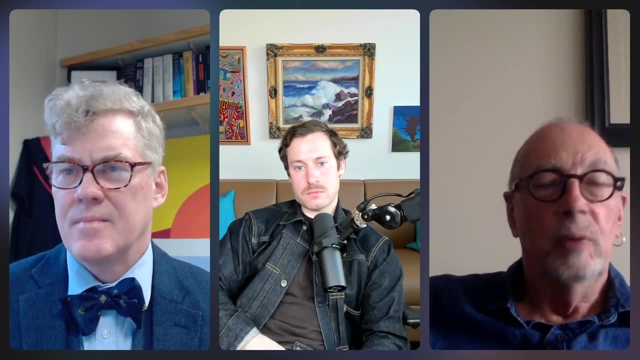 That's not a rather clumsy way of putting it. Let me rephrase that If you're reasoning about a structure, You want to use a kind of inference that preserves truth in that structure. But normally when we reason we're not reasoning about truth in a structure in any obvious sense. 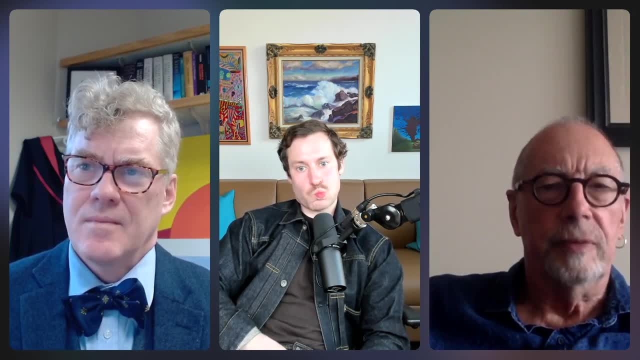 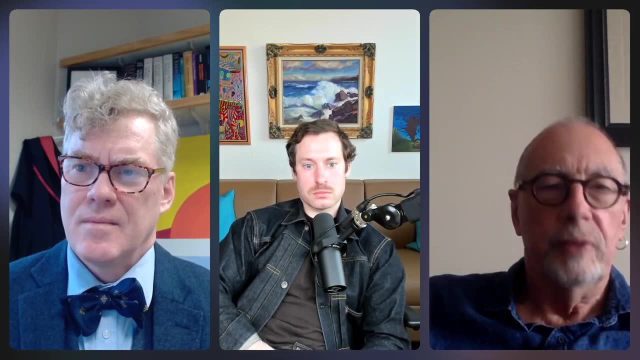 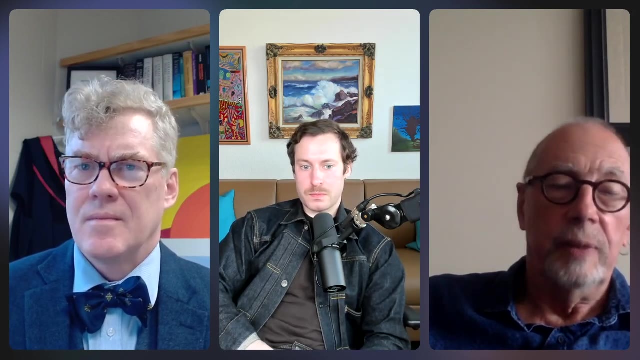 And then we're reasoning about what preserves truth, simply. Now, some people have problematized this distinction, like Stuart Shapiro, But I think it's a pretty good distinction. So I think you can be a mathematical pluralist without being a logical pluralist. 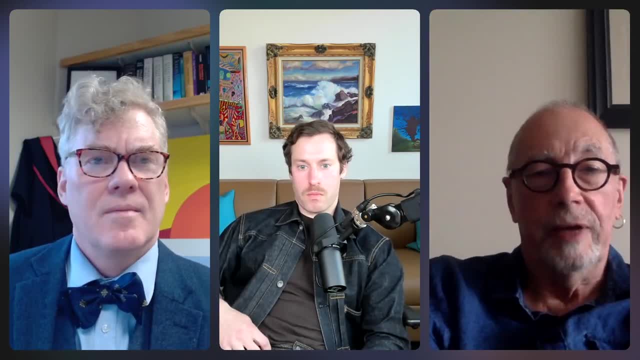 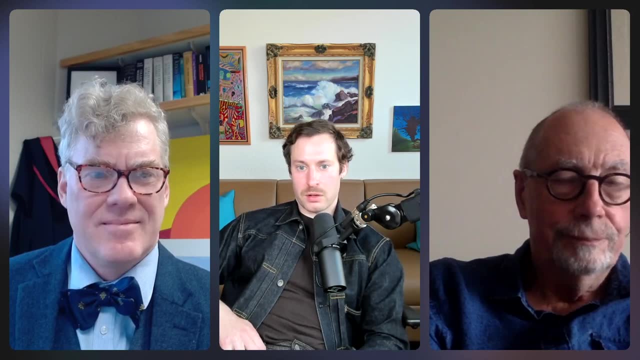 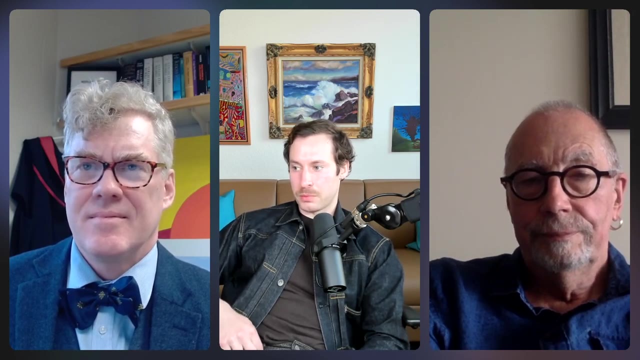 But I mean, this puts mathematical pluralism, I guess, squarely on our agenda today. Yeah, And that's where I would like to go after this, But I want to clarify then for you, Graham. So I guess this is bringing metaphysics into the picture. 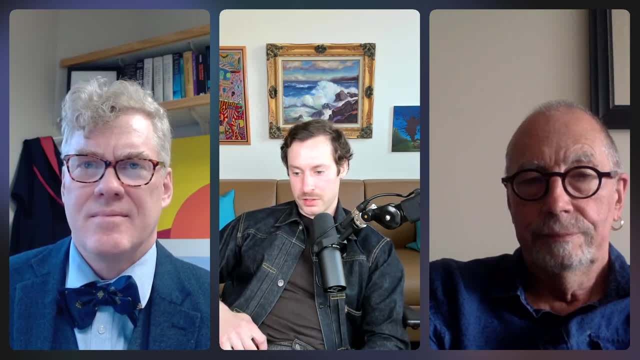 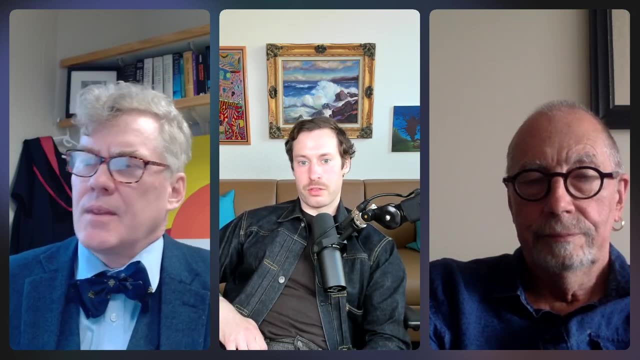 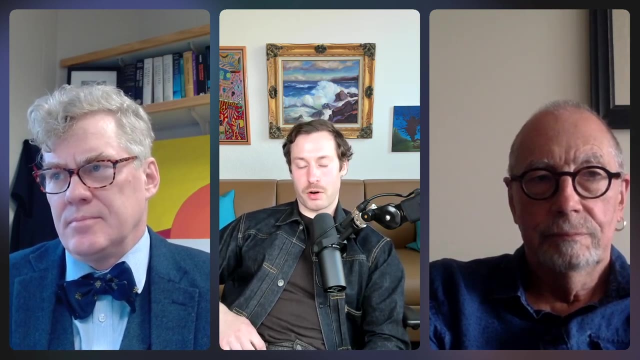 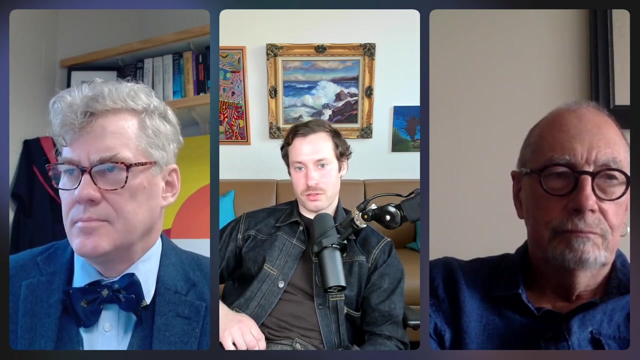 But is this a correct interpretation of your views? That paraconsistent logic is the logic, The logic of our world, But we should be reasoning about other possible worlds perhaps, Or we have license to reason about other possible worlds, Say, if we want to construe mathematical structures as worlds or something like that with other logics. 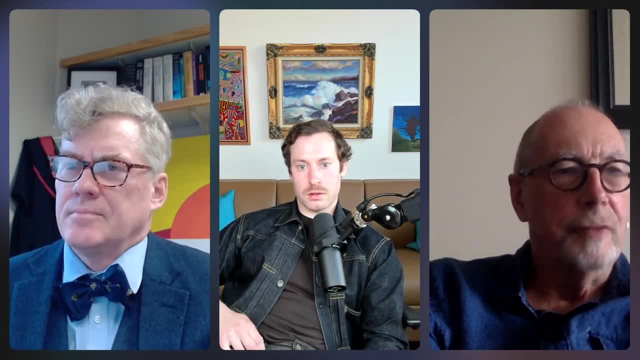 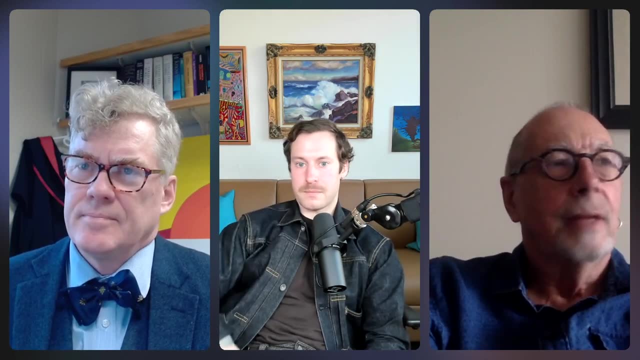 You can put it that way if you like. I mean, it's sort of that makes it really heavy duty metaphysics And talk about worlds and so on. Yeah, Yeah, Look, generally speaking, I'm happy to go along with that. 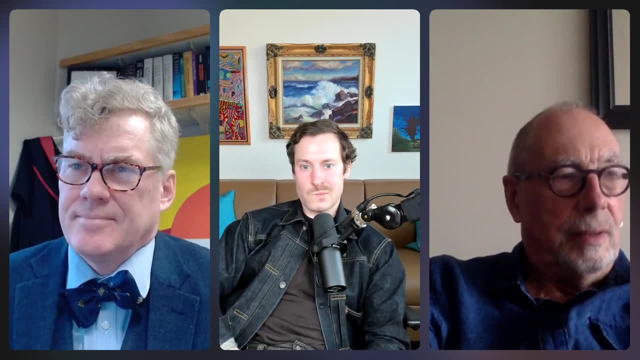 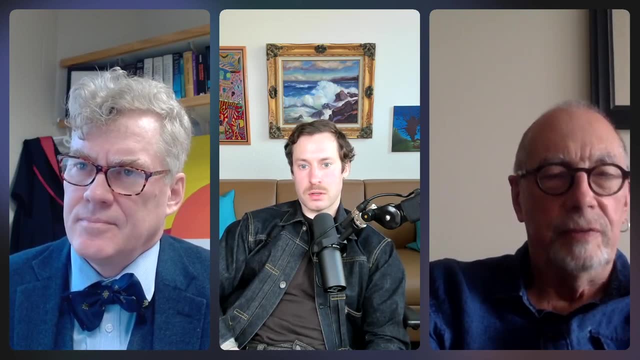 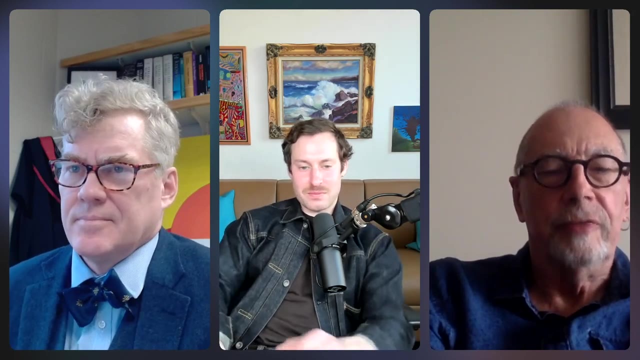 But I don't think a logical monist is essentially committed to this heavy duty metaphysical stuff. I think that's a different part of the story. I mean, I think Frager was obviously a logical monist, right, He had a very different. 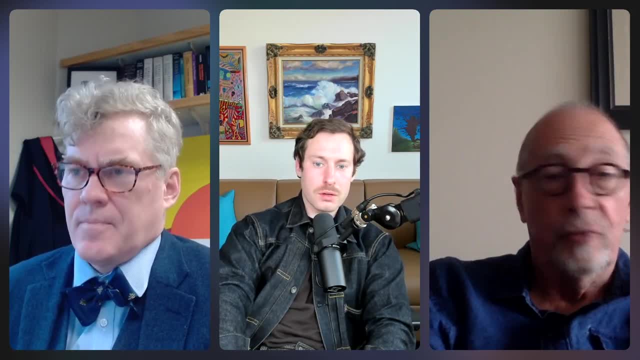 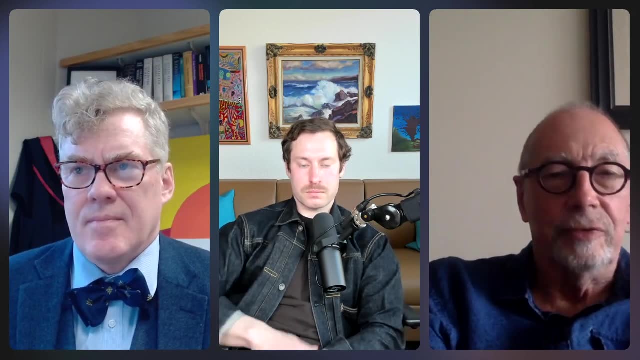 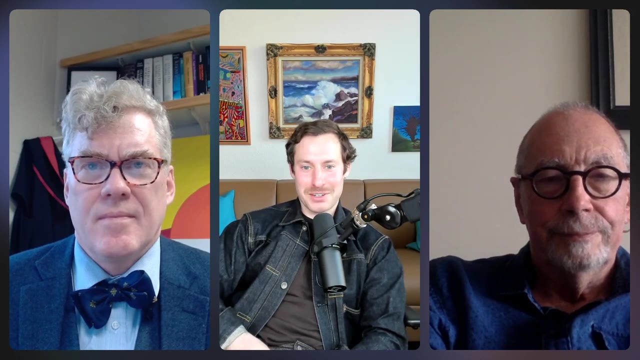 Who did you say Frager was a logical monist, And I don't think he thought into this sort of the kind of metaphysical story you're telling. He had his own metaphysical story, Okay Well, maybe it would be a good time then to turn to Joel's 2012 paper, The Set Theoretic Multiverse. 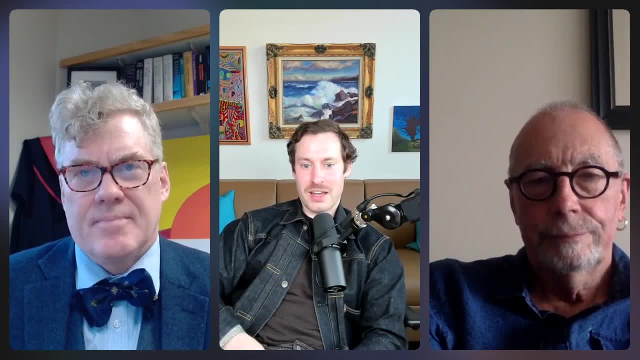 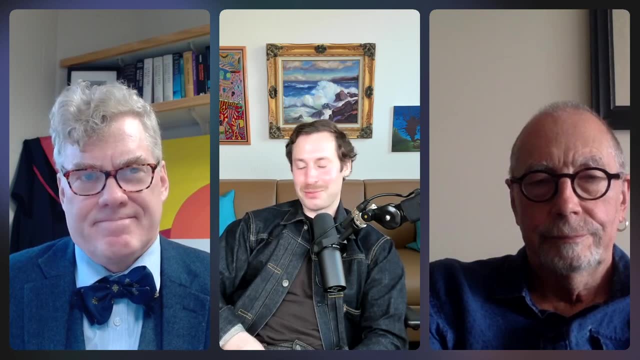 In which you introduced the multiverse view of set theory. And I'm not alone, even in this conversation, in thinking of this as a groundbreaking paper, Because when I was thinking about PhD programs a few years ago And I talked to Graham about what I should write about, 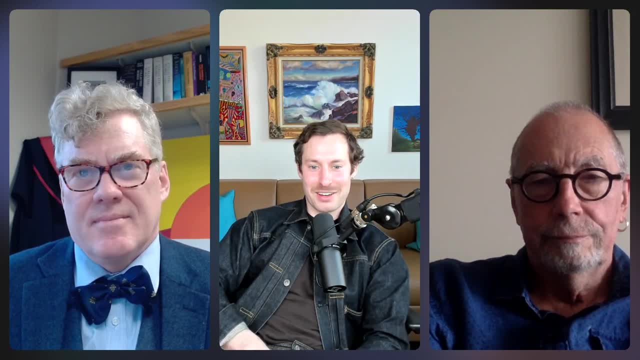 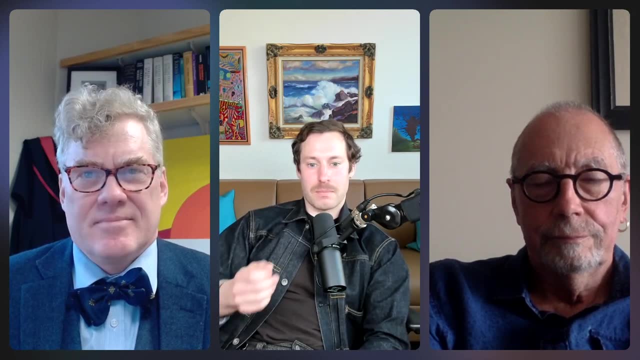 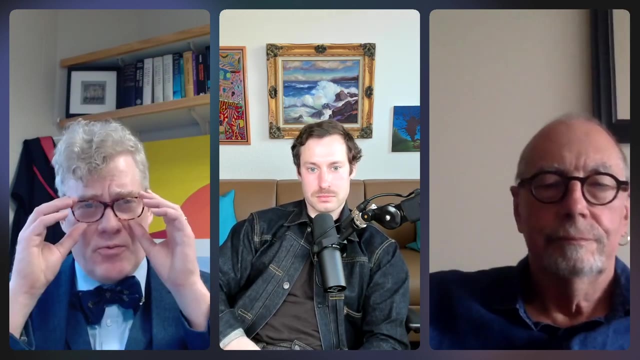 I mean, his immediate suggestion was that I take a look at your paper. Oh, yeah, Yeah. And so what, at first blush, is the multiverse view of set theory Right? So the multiverse view of set theory- I want to distinguish it sharply- you know, sort of set theoretic pluralism. 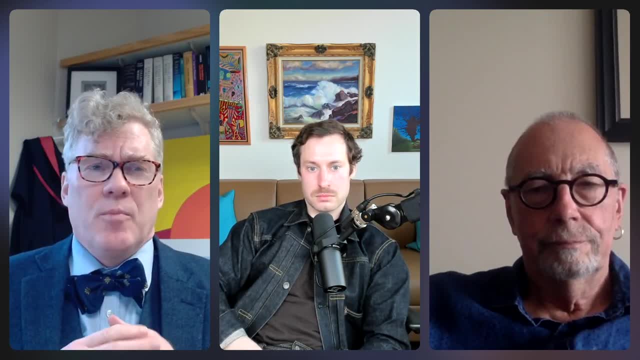 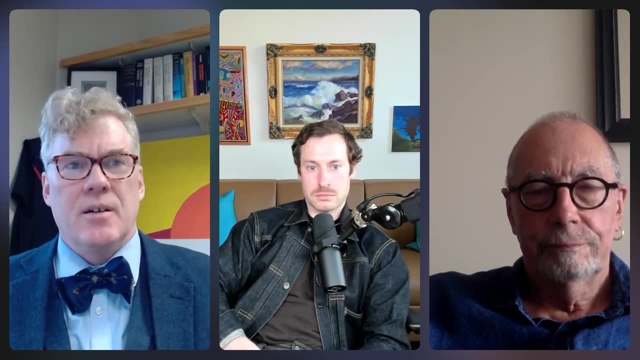 Which is what the paper is about, From logical pluralism, Which is a topic that is much more the kind of thing that we're talking about, More the kind of thing that Graham is working on And JC Beale And many others. 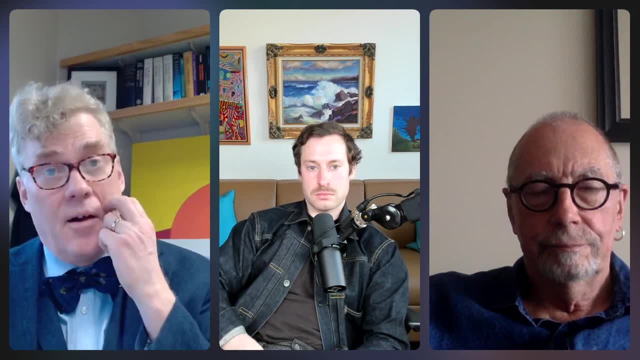 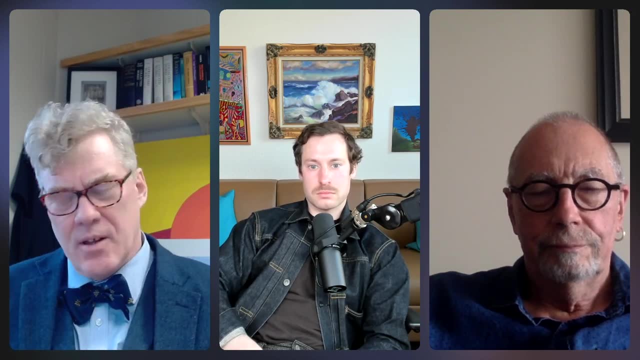 Greg Restle And so on. So it's not really the same thing And it has its origins in different places. So as far as set theoretic pluralism is concerned, It arose for me when I was a graduate student in Berkeley. 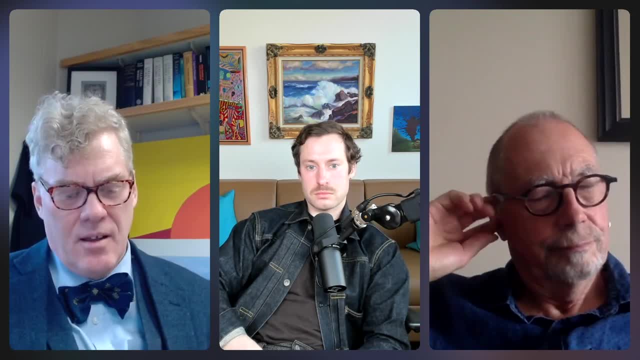 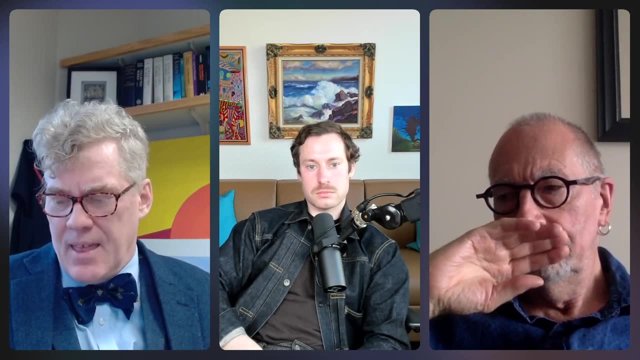 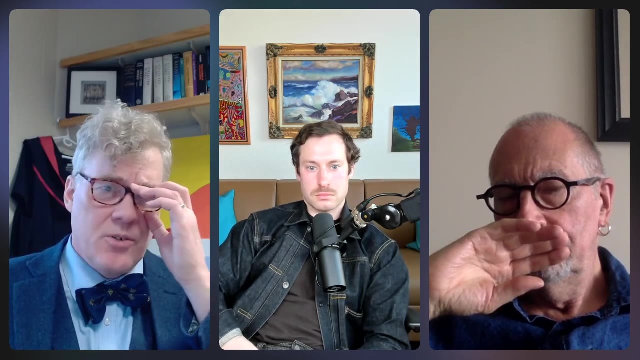 I worked with Hugh Wooden And Solovey was there And so on. You know big logic group in Berkeley And set theorists working there And the sort of overriding philosophical view held by those researchers was very strongly monist, Platonism. 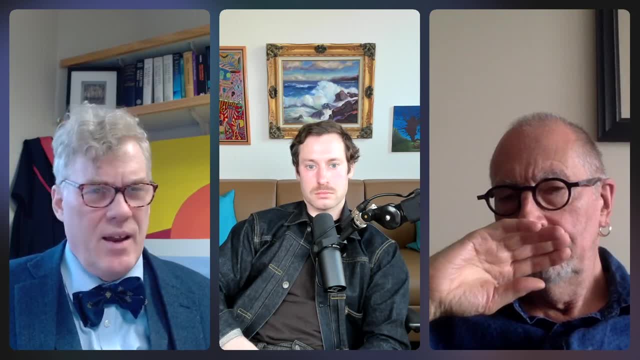 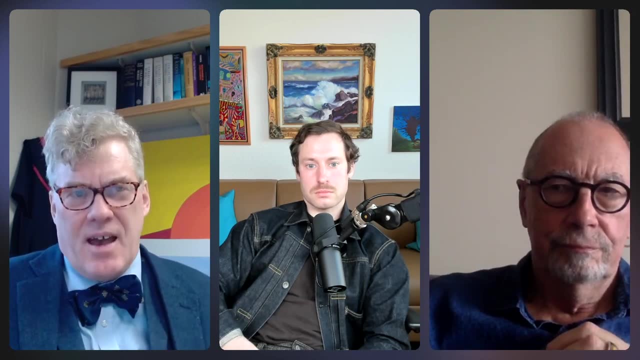 And, for example, when you know, the continuum hypothesis is known to be independent, And it was known by them to be independent, of course, But the attitude was that. well, nevertheless, there's an answer to the question Of whether the continuum hypothesis is true or not. 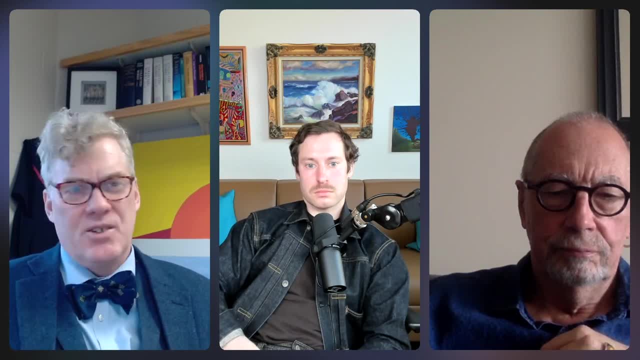 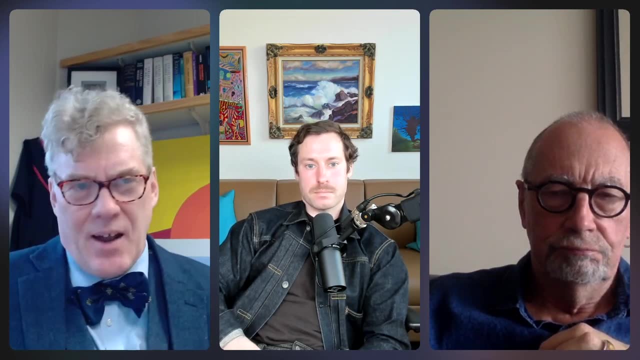 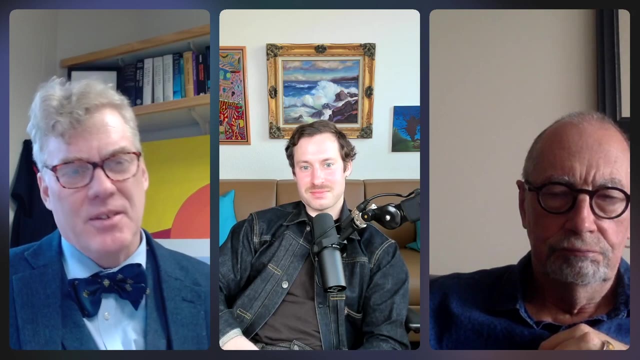 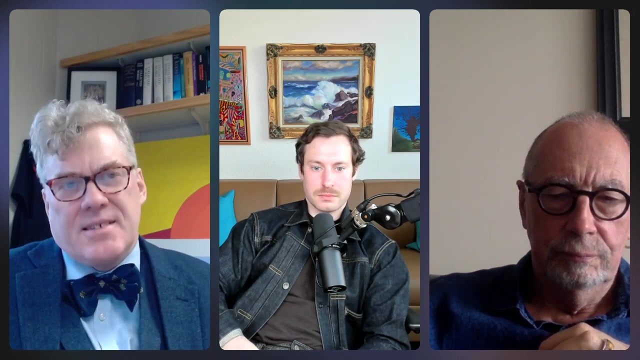 And we're going to try to figure out which it is And to so okay. So that was when I was young in Berkeley, But somehow I was always kind of unhappy with that attitude about it Because meanwhile the tools that set theory has developed, had developed over the years. 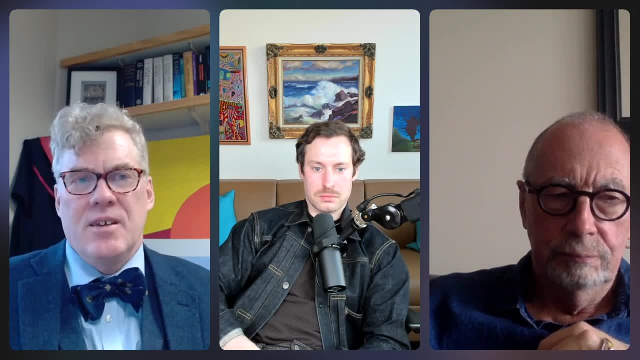 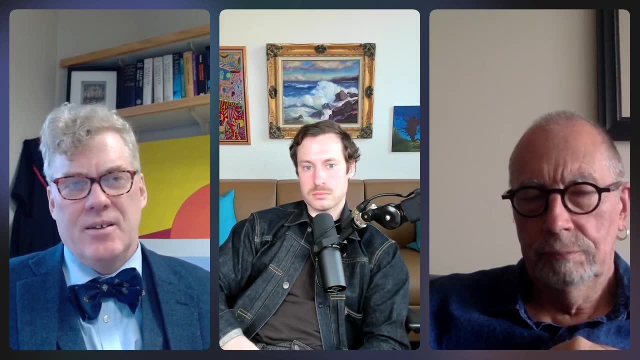 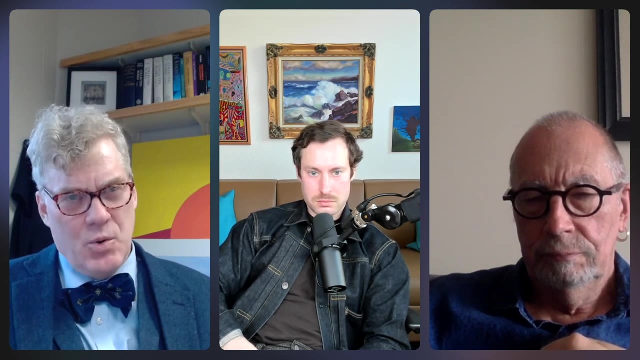 Had developed over the, you know, last 50 years of the 20th century Were all about building various set theoretic worlds, Basically forcing inner models, ultra powers, definable inner models and so on. We had all these tools basically for building models of set theory. 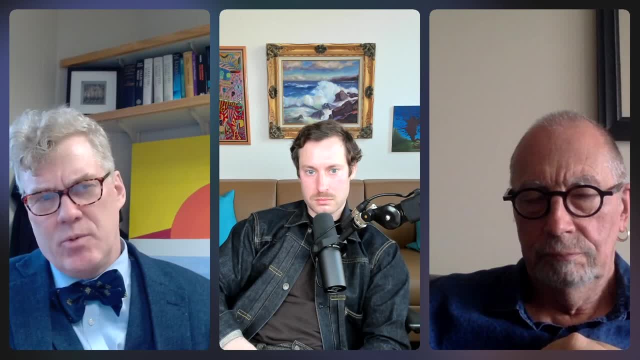 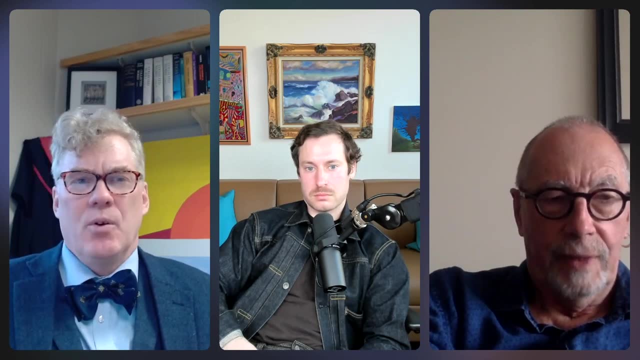 Alternative models of set theory In which the continuum hypothesis was true or false, Or where it was false But some other things happened, and so on, And basically almost every paper in set theory, Almost every published paper, is building a model of set theory. 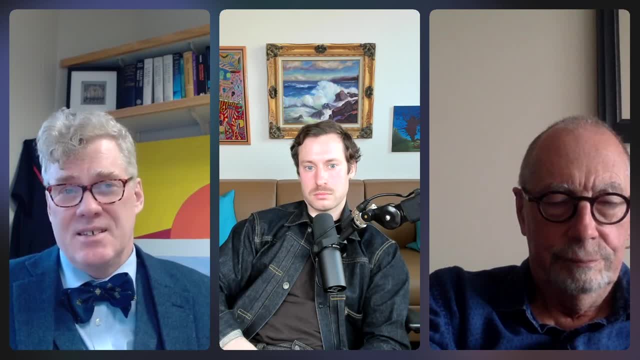 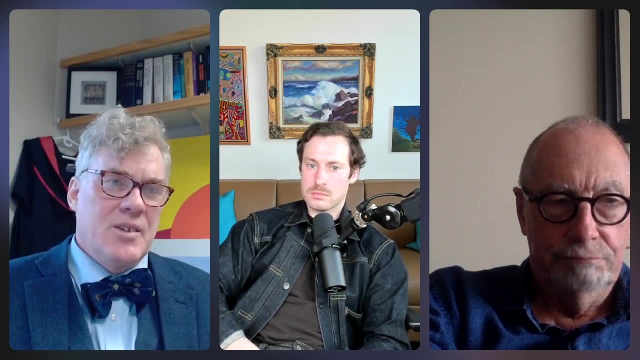 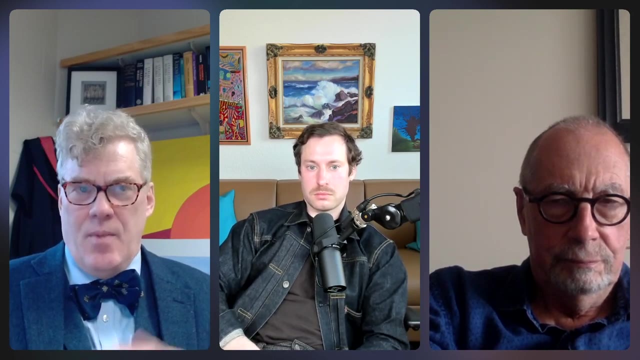 In order to show that a certain combination of statements is consistent Or could be the case, Which is another way of describing what they were doing, And so it seemed like the most natural way to understand what the tools were doing Is model building. 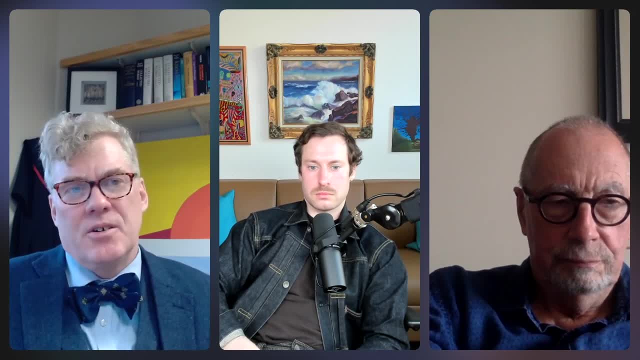 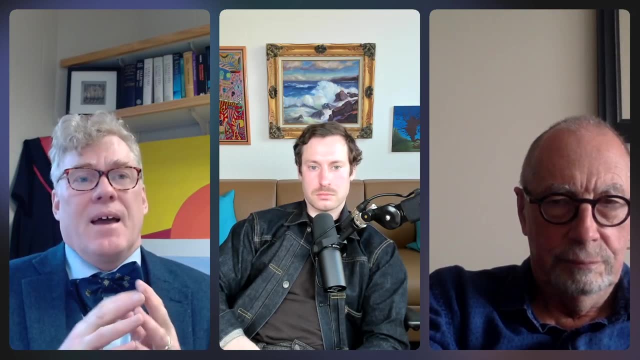 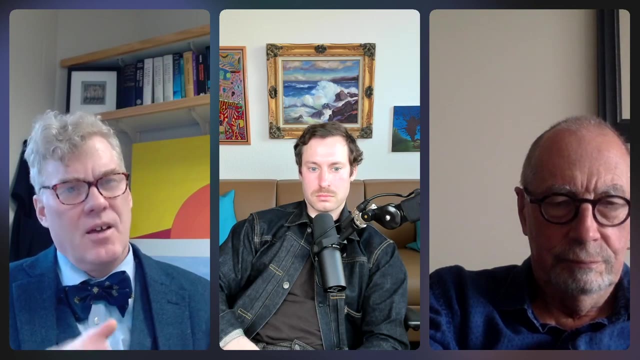 Universe building, Showing us these alternatives, Showing us how set theory could be different than we thought. And furthermore, I mean when you study forcing models At first you know you have this sort of countable transitive model understanding of set theory. 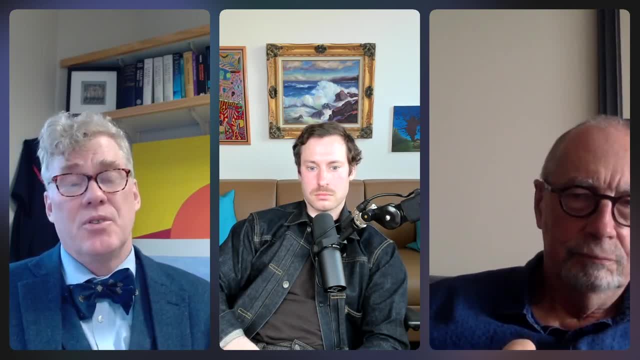 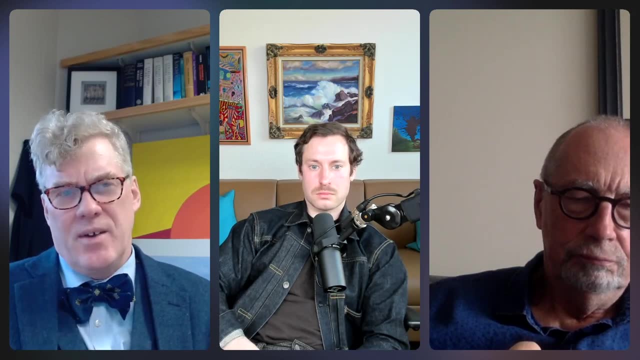 And it's easier to be a kind of Platonist about set theoretic truth If you think that the forcing technique is only about building these sort of fake models. But at a certain point you realize, You recognize that it makes sense to formalize the theory. 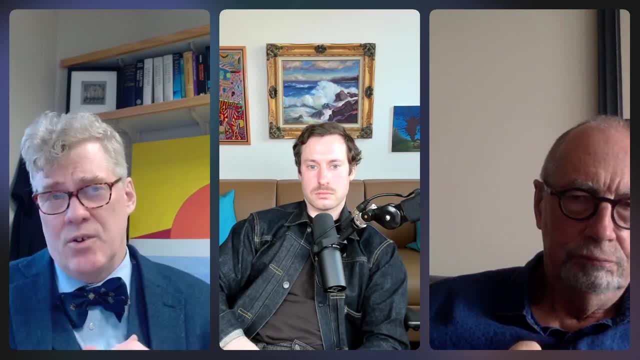 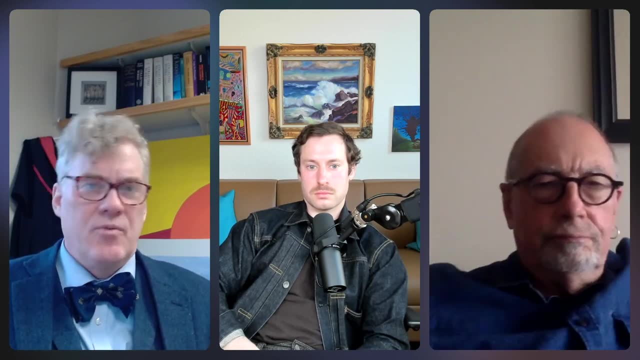 As forcing over V, The universe, The whole universe, And talking about forcing extensions of V, And people started writing this explicitly in papers, Talking about V of G and so on, V of G of H. You know there's a forcing extension of the universe with certain features and so on. 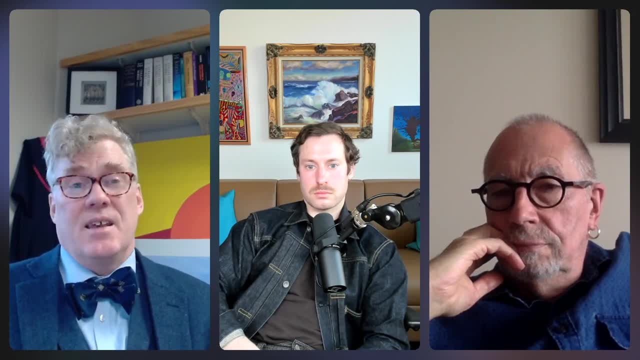 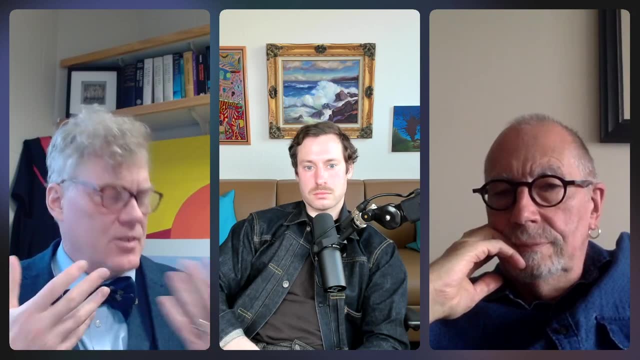 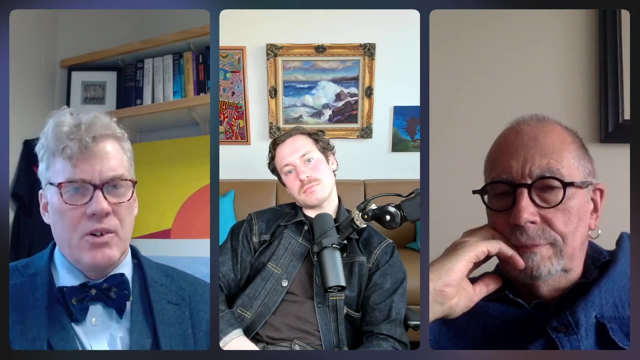 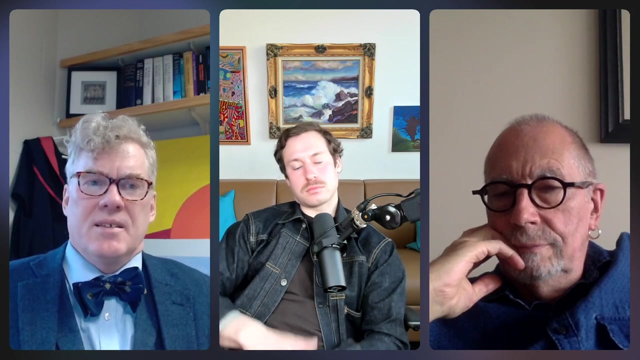 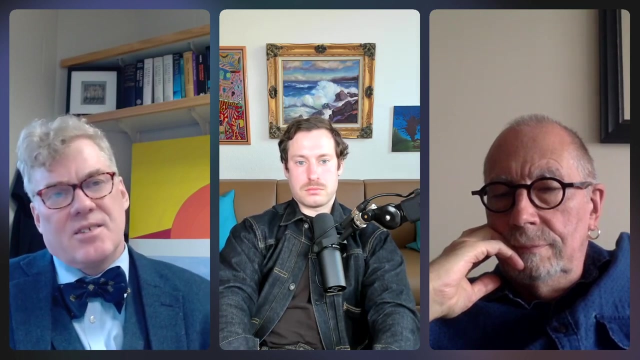 And that way of talking just invites explicitly this multiverse way of thinking And, to my way of viewing the matter, It seemed like What we were doing was exploring this space of set theoretic possibility Which was explicitly pluralist, And that we shouldn't expect to get an answer to C, H. 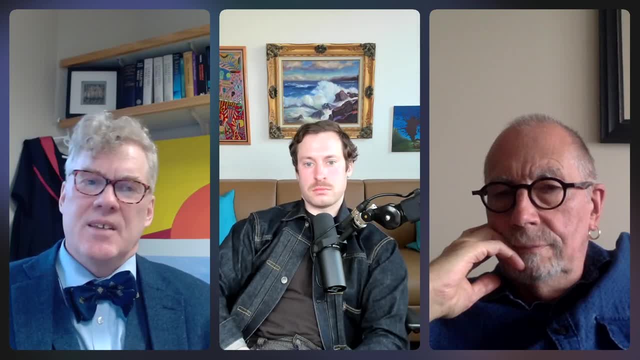 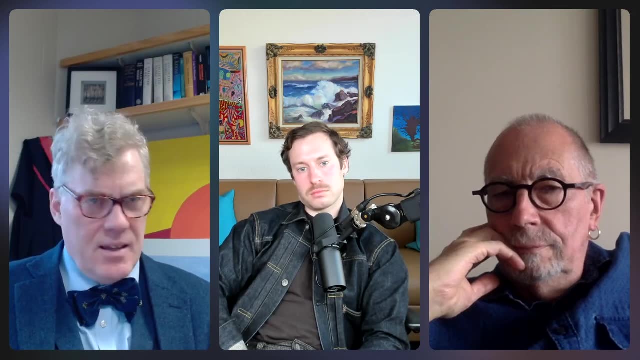 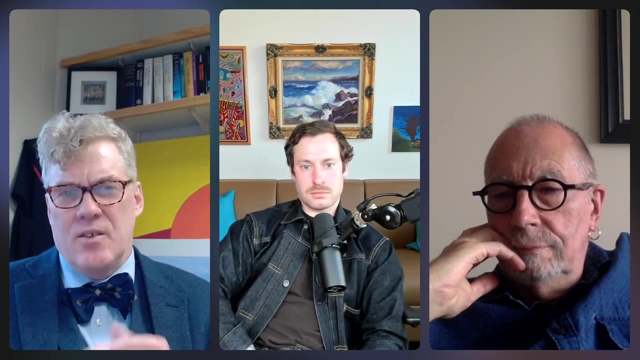 To the continuum of what was this question, A single definite answer, But rather we already understand in a quite deep way How it could be That C H fails, Or that it's true, And furthermore, Because our understanding of the forcing extensions is so strong and deep. 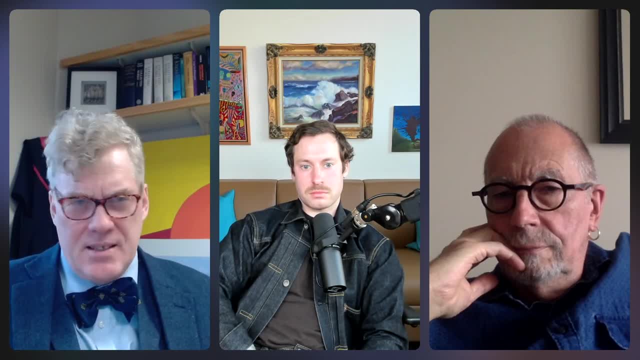 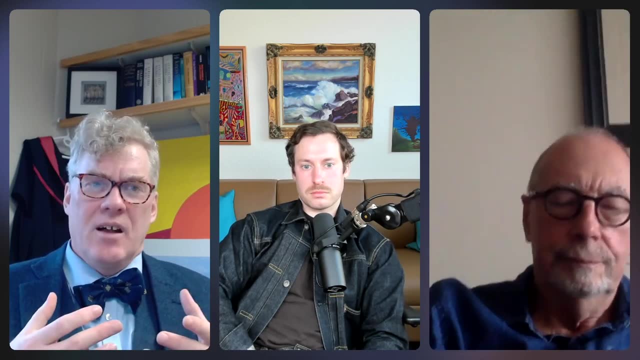 It's not just that we know the continuum hypothesis is logically independent And there's no proof either way. That's not what the nature of our knowledge is like. The nature of our knowledge is like You give me any set theoretic world. 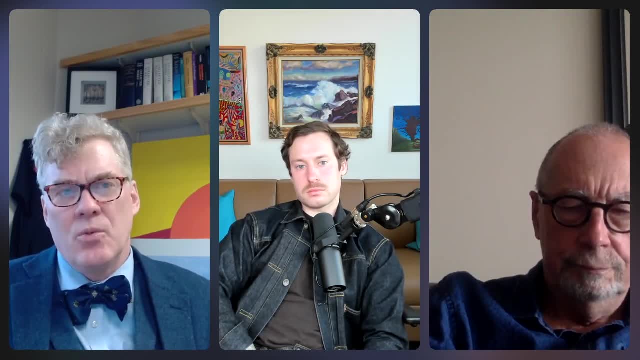 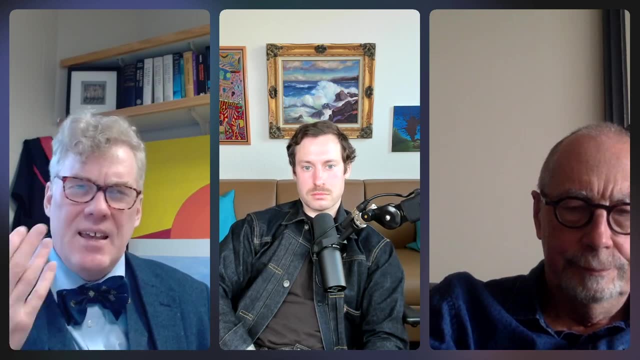 Then I can, from that world, construct another world Which has a different answer To the C H question. And it's to say: Well, there's a single definite answer to C H, I think in my book Or in my paper. 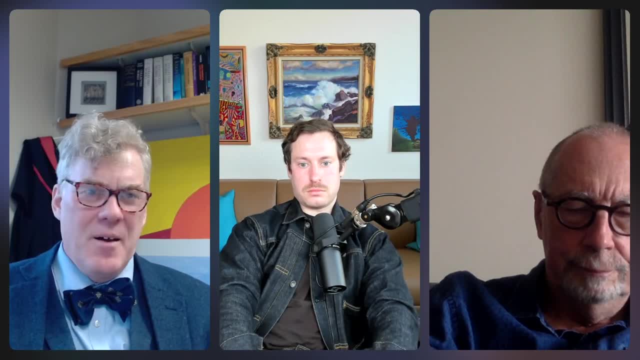 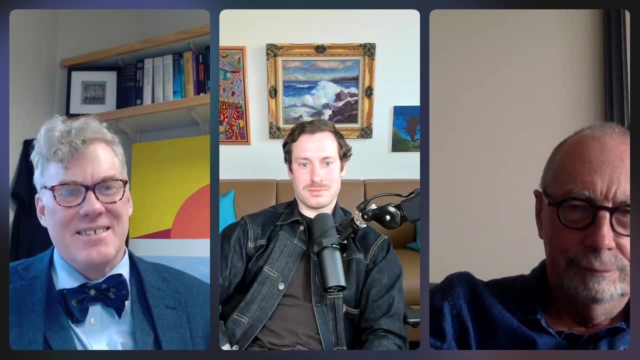 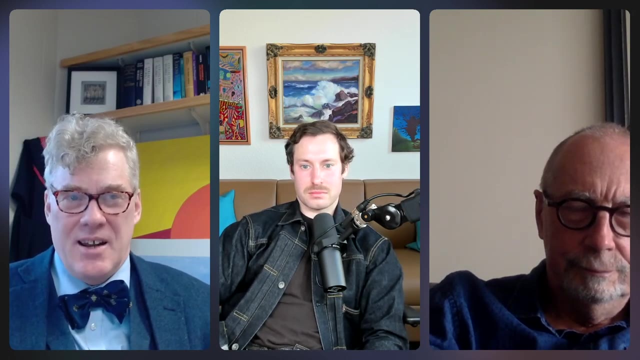 I say it's like someone saying Only Brooklyn exists, But I already know about Manhattan and Queens, And so I've been to these other universes In which C H fails And I understand That, actually the universes in which C H fails. 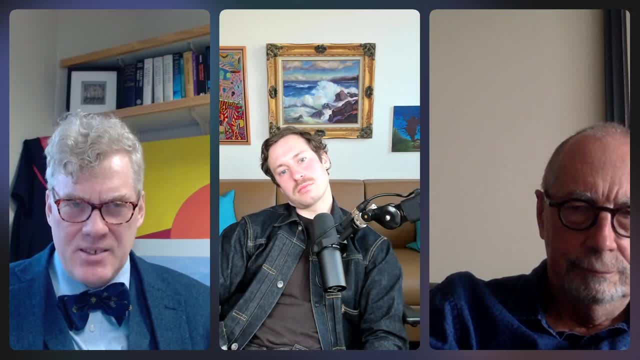 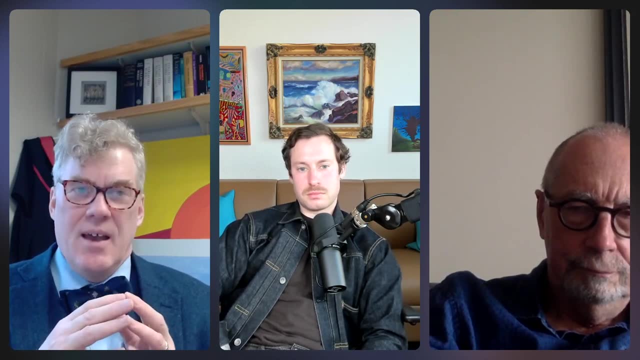 Are kind of dense In the space of all universes. Because of this forcing connection You can move from one to the other In a way where the former one has kind of access, By means of the forcing relation, to those other worlds. 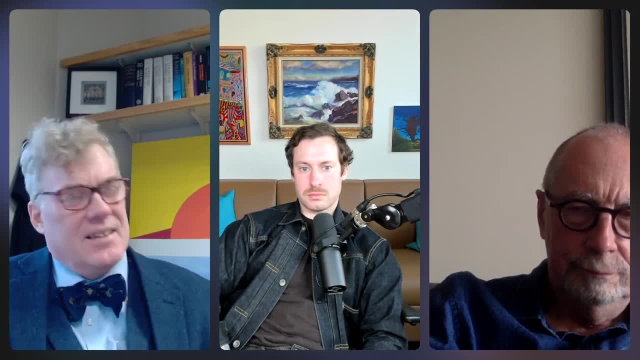 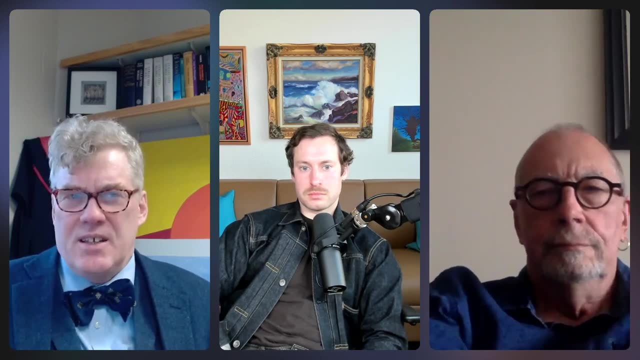 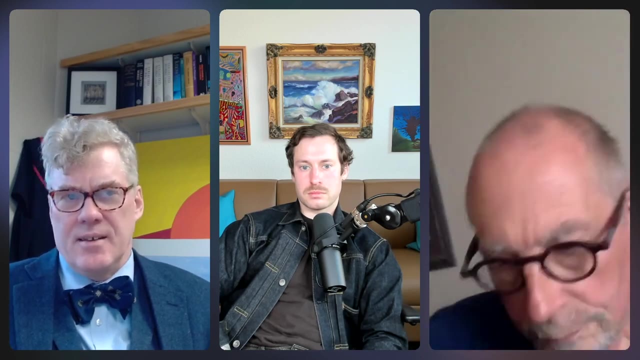 And so, So it seems, It seems to me much more natural To discuss the. The forcing extension seemed perfectly set, theoretic And acceptable, And so. So this is explicitly- And I had a really hard time, though I think I mentioned this in my last- 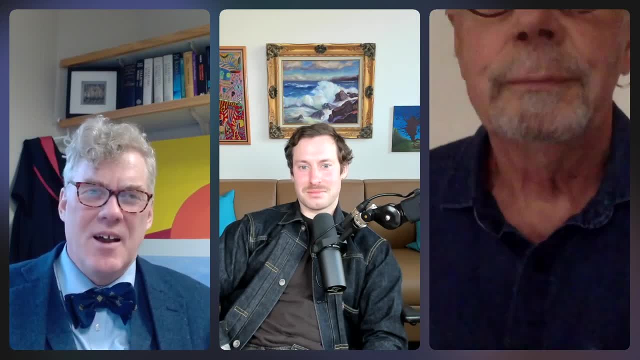 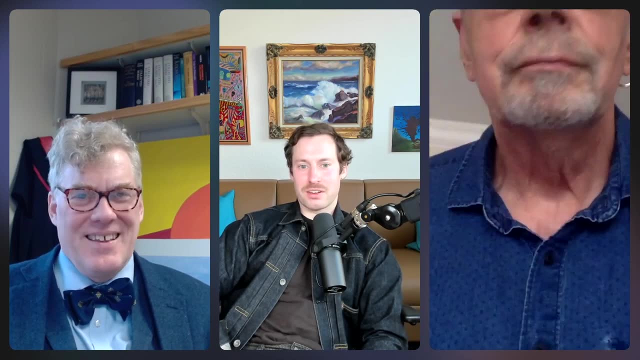 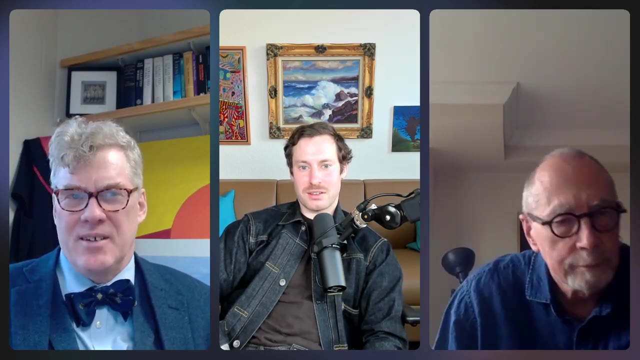 Discussion with you And I had a really hard time Sort of coming out to You. I remember you you mentioned giving this. Was it at NYU? There was a conference organized at NYU about mathematical pluralism And so 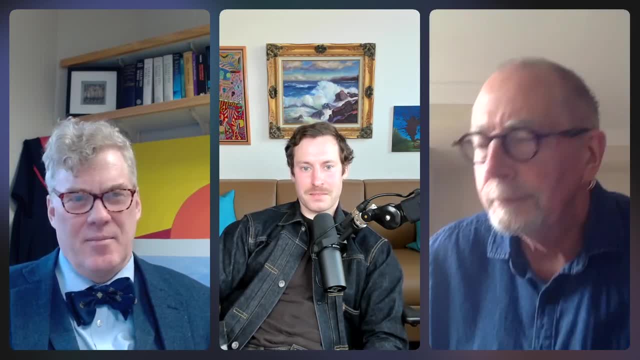 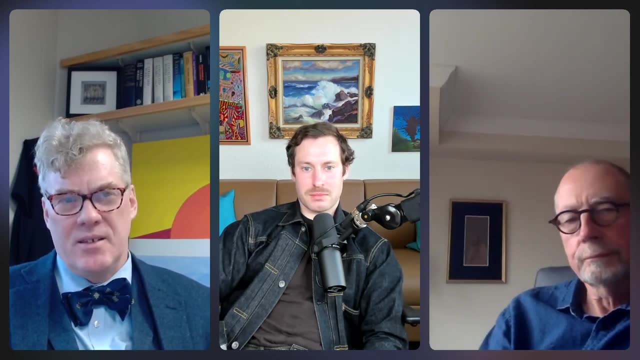 And it was about this issue. So wooden was there, And Any philosophers of mathematics for there, And and I I gave my that's when I first started speaking publicly about this sort of pluralist conception, And and I was so 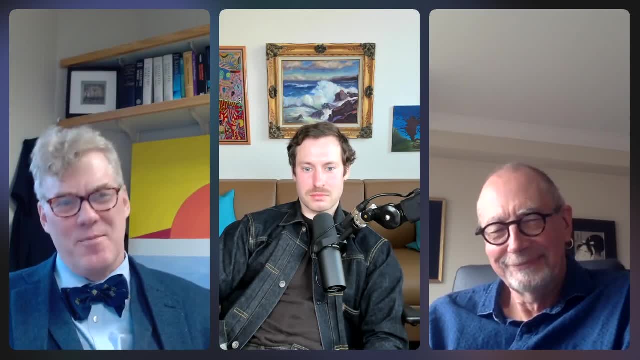 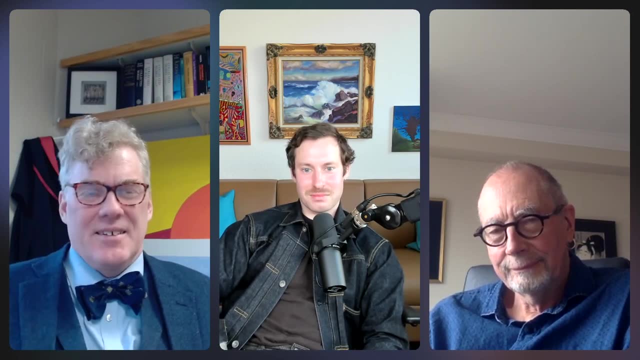 I was a nervous wreck before that, but everything went fine, And so from that time- No, I've been talking about 20 years or whatever it's been- And so I'm glad I I'm glad I did it. So 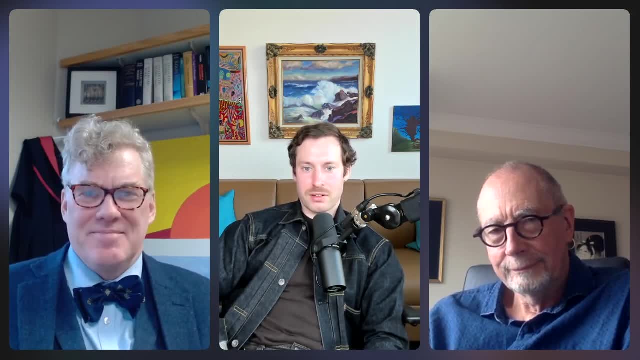 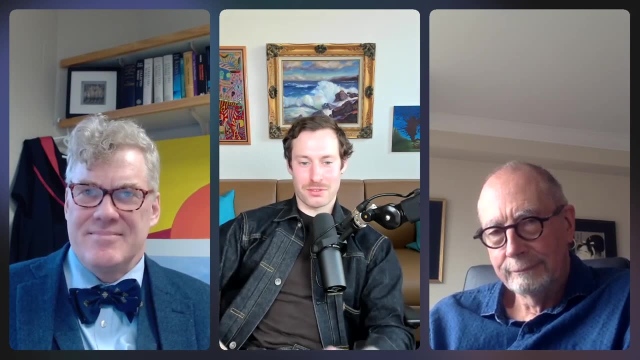 I don't know if that answers your question or not. Oh, it certainly does. And, Graham, I'm going to come to X- you know Polaris in a couple of minutes, but of course Always feel free to jump in. but 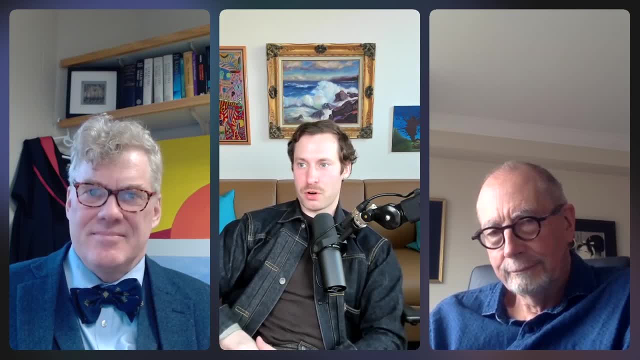 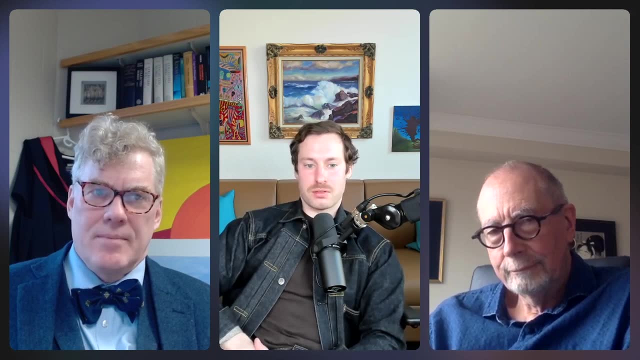 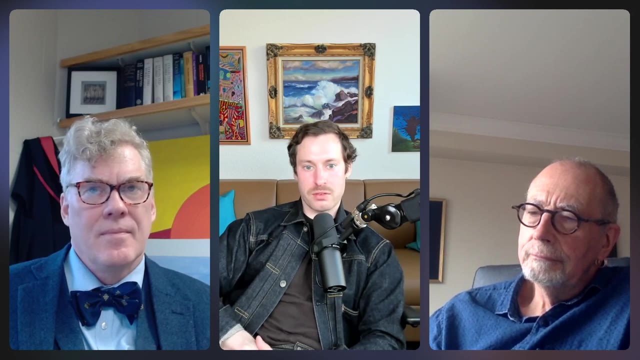 Joel, Just before we, I guess, Talk about the view in more detail, It's been almost 11 years since the paper came out. Has Your view changed in any substantive ways since then? Well, I'm still Strongly committed to this pluralist conception. 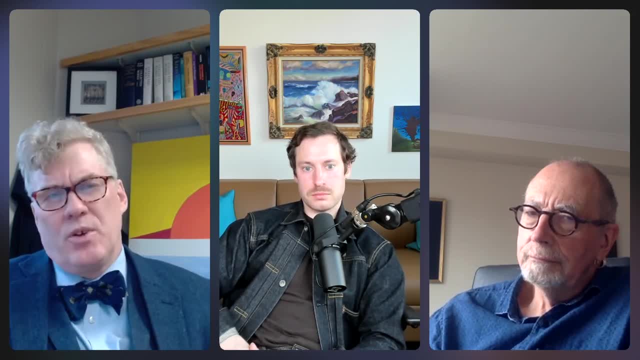 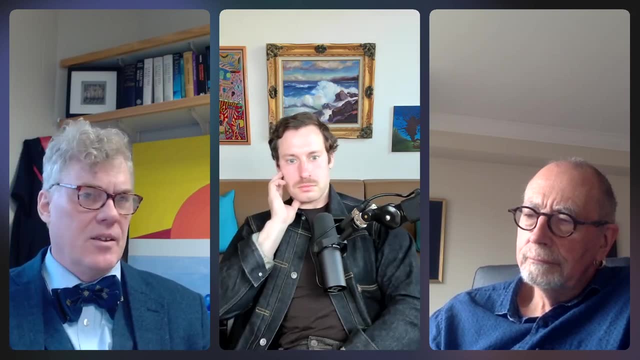 And I guess my view has become more refined a little bit, because I recognize that actually Well, there's different kinds of pluralism, even in the philosophy of set theory, for example, one can be a monist sort of all the way up, you know. 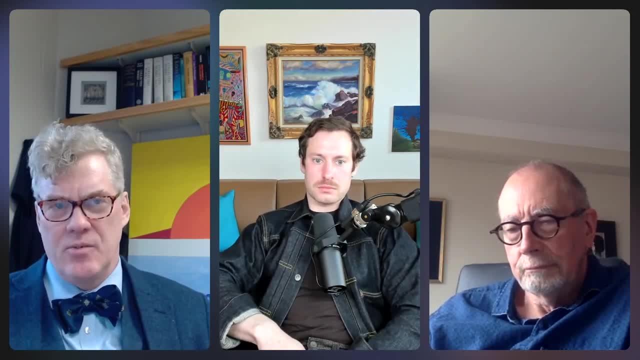 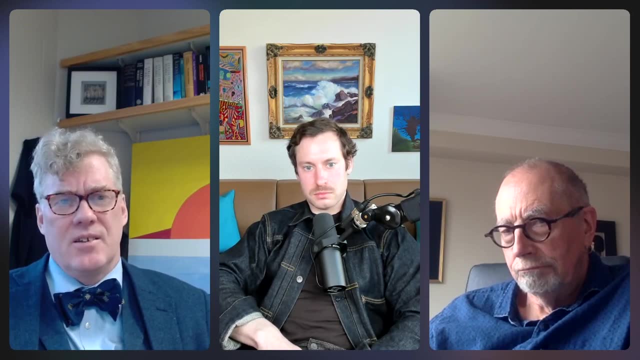 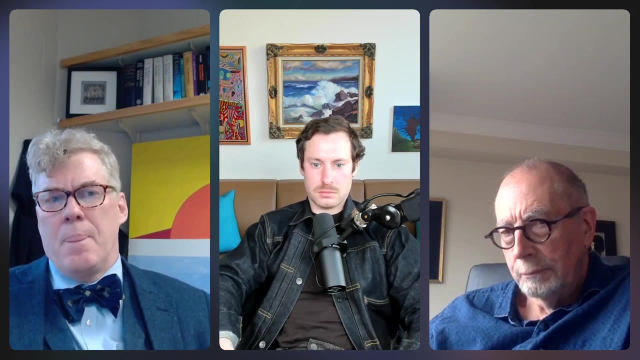 about all mathematical truth, about the entire set theoretic universe. There's one true set theoretic universe in which all set theoretic questions are Have a definitive truth value. This is the view of the Sort of Hardcore monist view And therefore, if mathematics is interpreted in set theory, 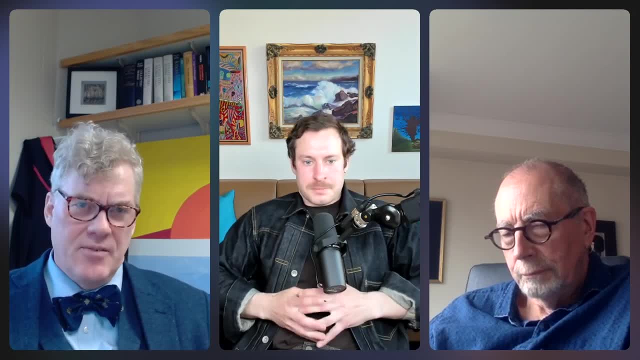 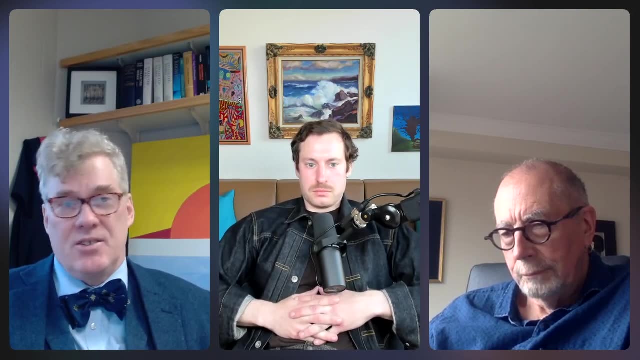 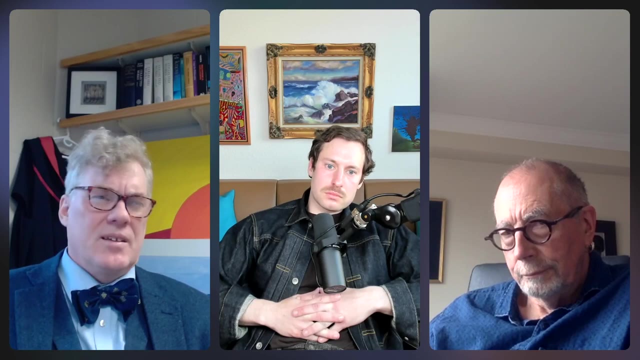 which is the consequence of set theoretic foundationalism. Then one can sort of extrapolate this perspective also to mathematics. Generally, There would be correct answers to any given mathematical question. Okay, So then there's a little bit softer view, which is something like Fefferman's view. 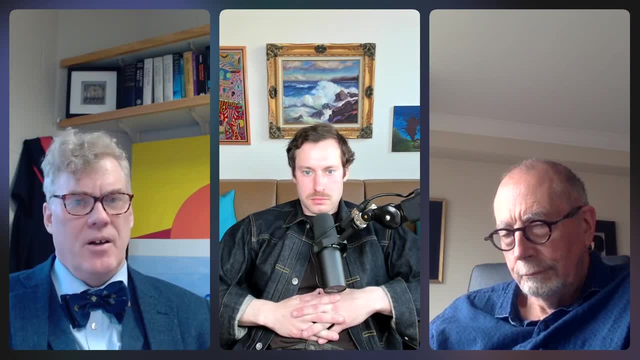 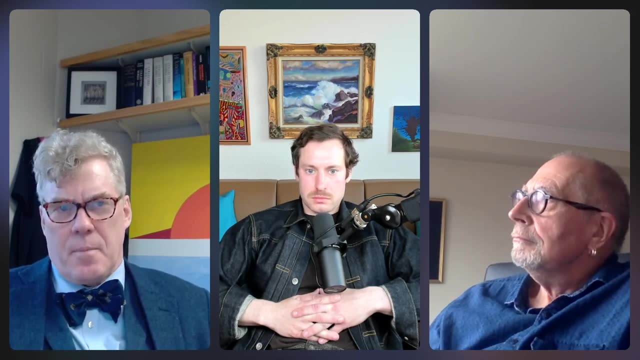 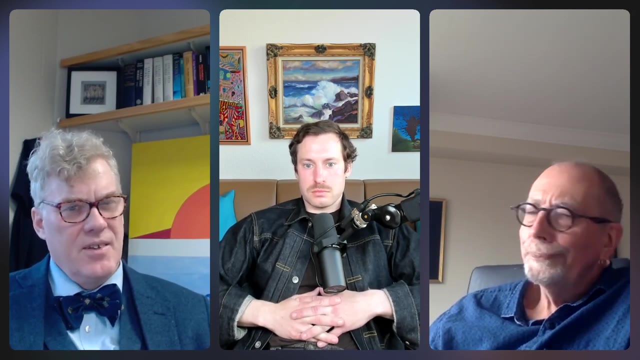 Where he's a monist about arithmetic. He thinks arithmetic statements have definitive answers, But he's suspicious. Once you go up, Sort of you know, you take the power. sets of integers- Okay, Sets of sets of integers is definitely in. 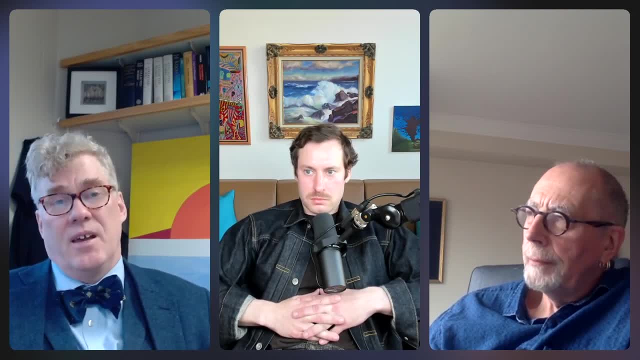 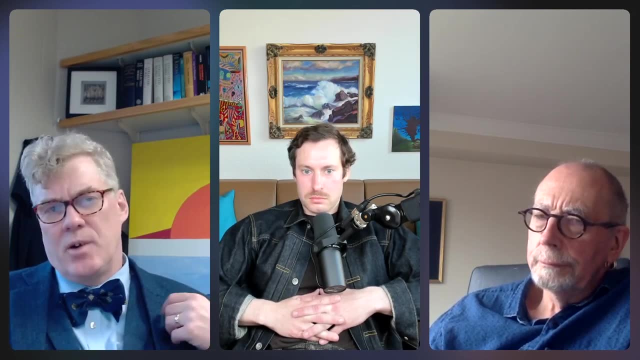 This sort of vaguer realm, And that's where questions like the continuum hypothesis are. And so he wants to say the continuum hypothesis is a vague assertion Because we don't have a good enough understanding of it. We don't have a good enough understanding of what it would mean to have 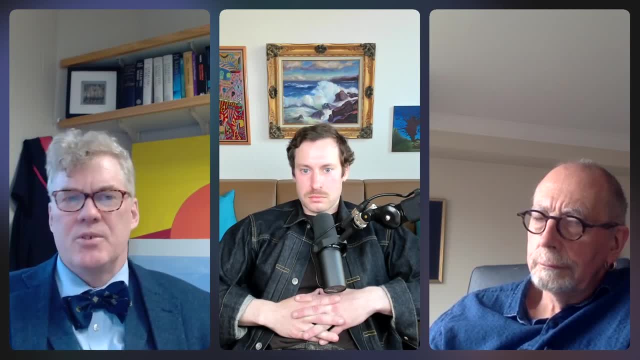 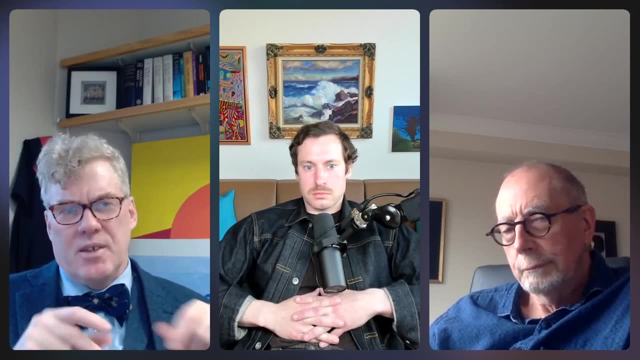 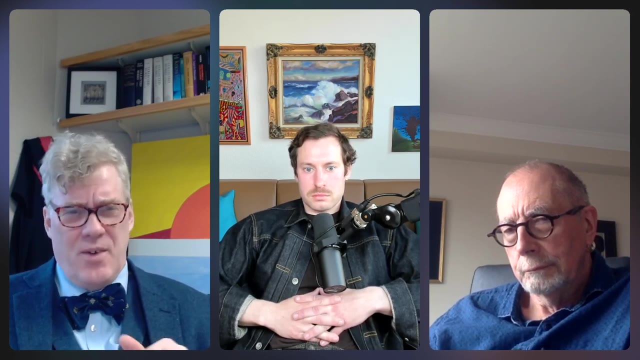 The set of all sets of natural numbers. Okay, So it's this sort of hybrid of pluralism and monism. It's sort of Monist about arithmetic and pluralist about higher set theory. And then there's what Peter Kohler calls the radical pluralist view. 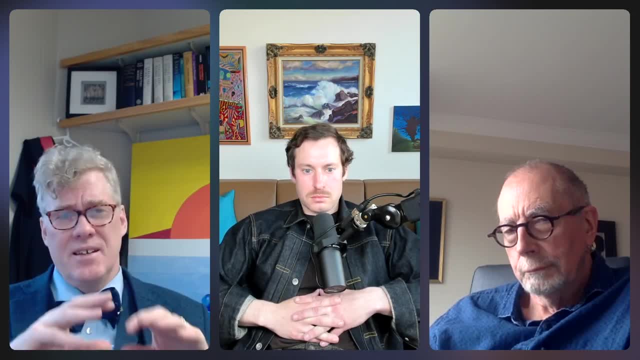 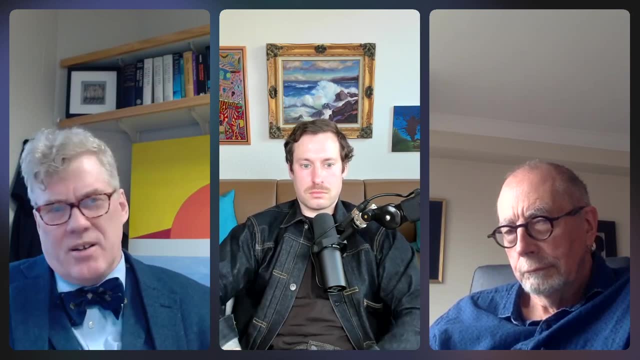 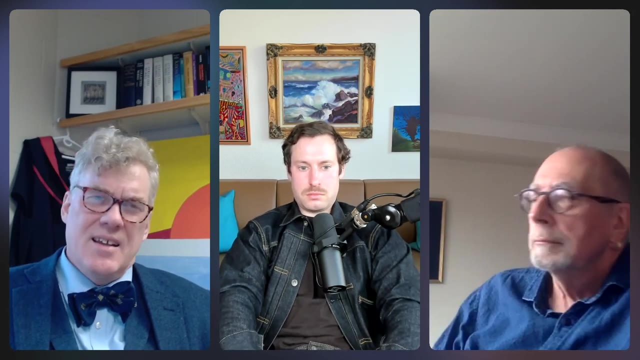 which is what my view basically is. I'm a pluralist, also about arithmetic. I think that When we, You know, it's very strong intuition that people have about the Definiteness of arithmetic truth, Because I guess the idea is: well, look, we can say the natural numbers. 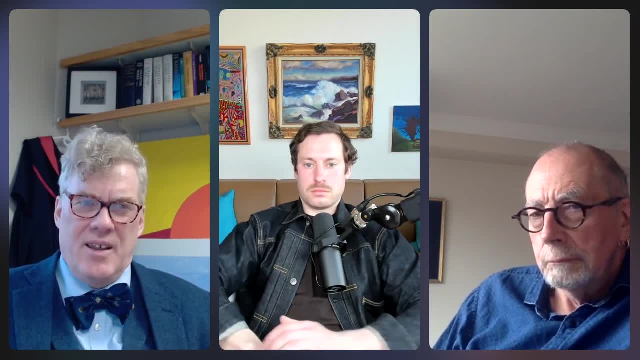 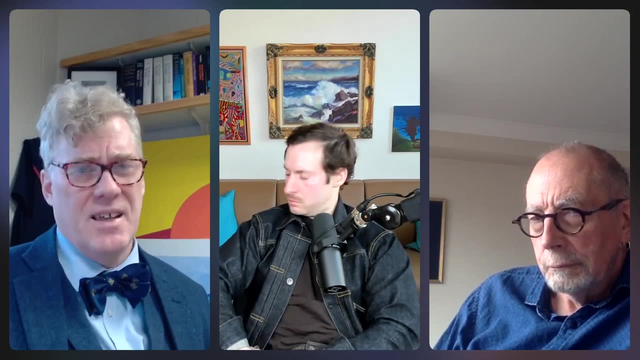 you know, 0,, 1,, 2,, 3, and so on, And we think that that's meaningful And that it's describing a definite mathematical structure. But my view is that Maybe we're making a mistake about that. I think we are. 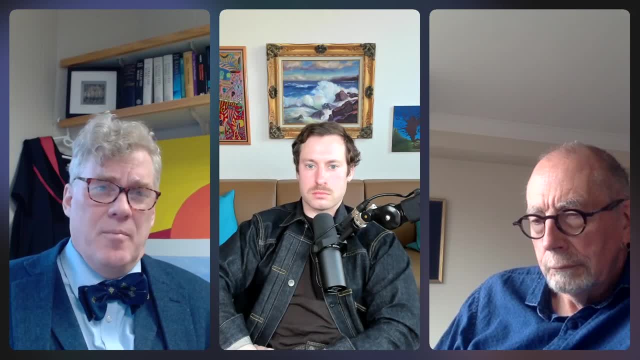 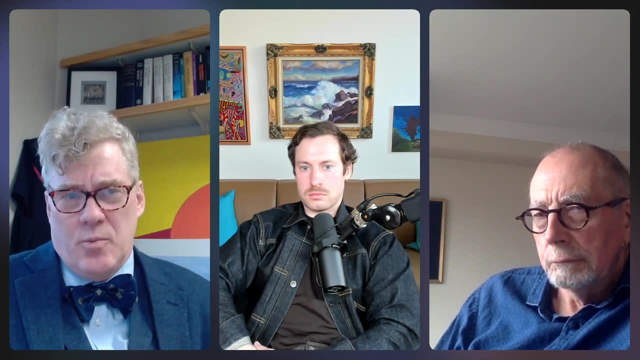 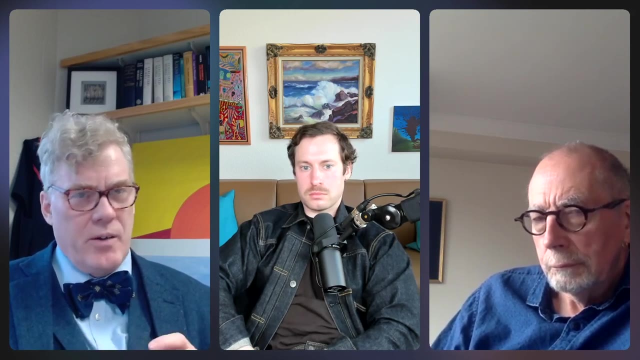 And and that The main reason, the best argument for the Definiteness of arithmetic Truth Is coming from Categoricity argument. The axioms of data can arithmetic. So we have a zero and we have a successor. and he says: 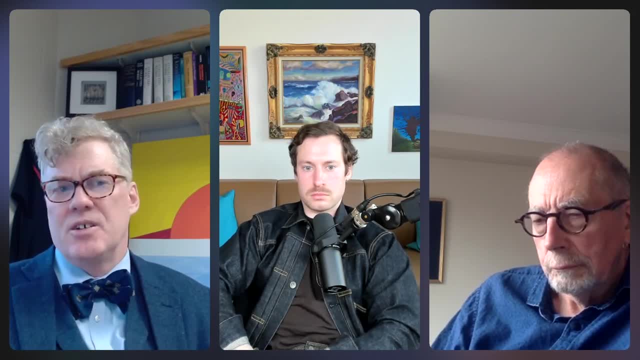 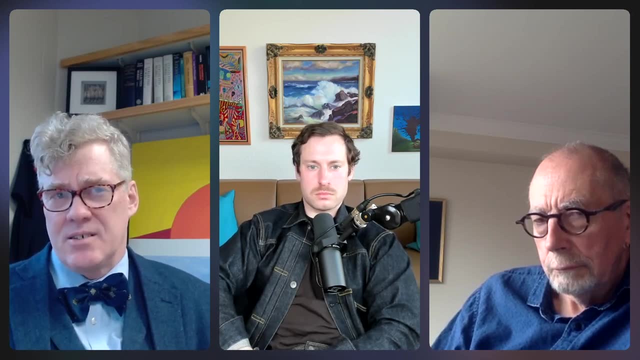 zero is not a successor and the successor function is one to one And we have Induction. So any set of numbers that contains zero and it's closed under successor has every number And, and then I can prove you know- a hundred and whatever. it was, 30 years. 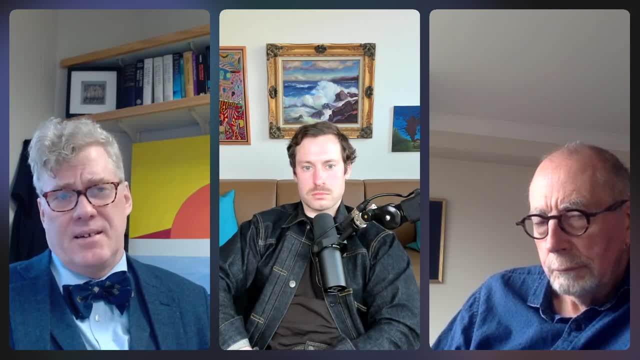 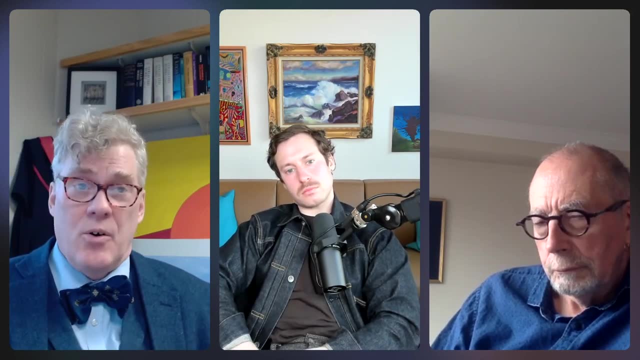 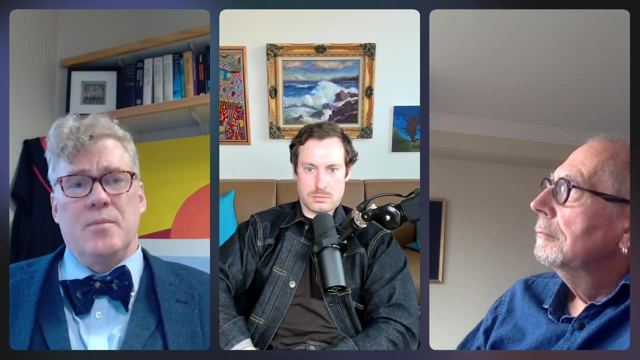 ago That That all structures obeying his axioms are So. it's categorical. It's a categorical theory, Which is to say that there's a single mathematical structure underlying his axioms, And that's why we think that there's only one concept of natural numbers. 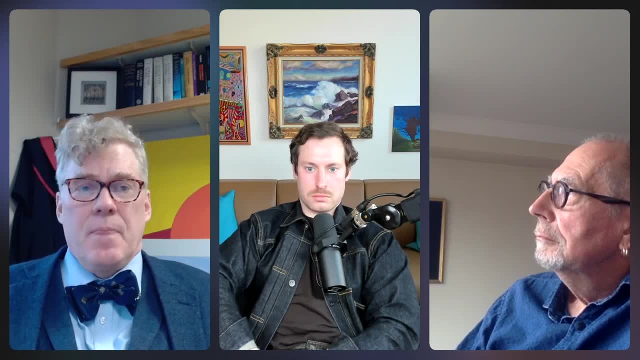 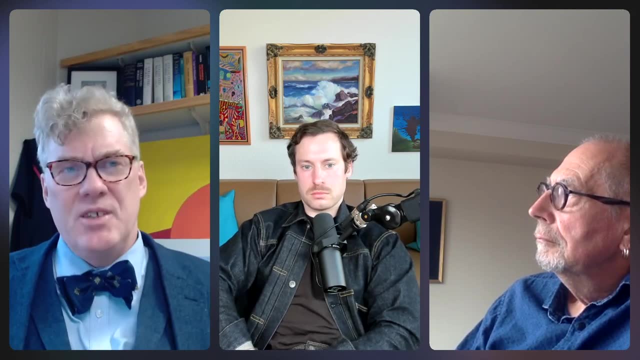 because we have this Categorical account of it. Okay, But I say: wait a minute, because, look, you were trying. you know the. the person who's defending Definiteness of arithmetic truth is Is trying to say: we know what we mean by definite arithmetic truth. 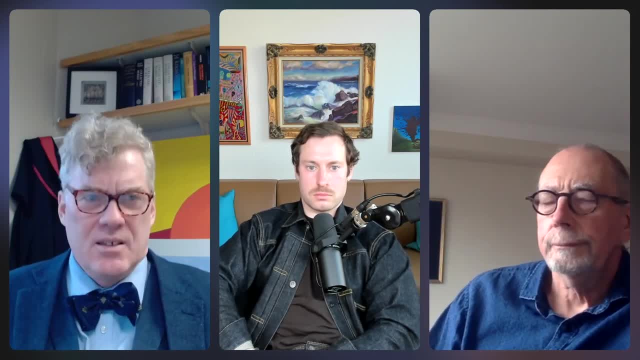 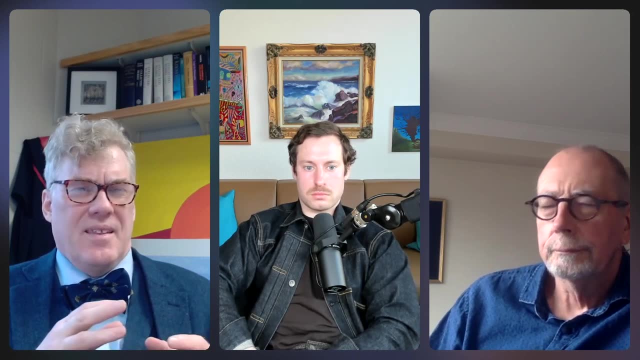 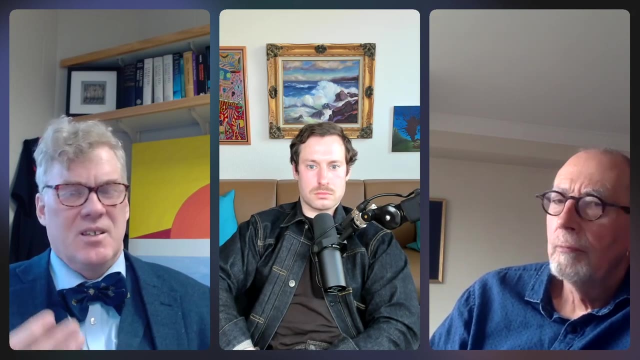 because we have this, This single arithmetic structure of the natural numbers That data can prove is categorical. But that's telling me what it means to be finite on the basis of his second order induction axiom, which is basically appealing. So this infinitary, 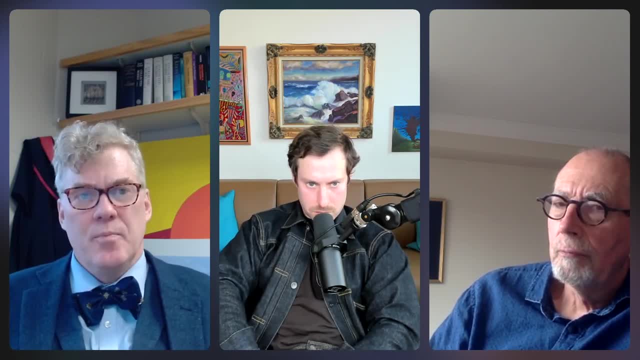 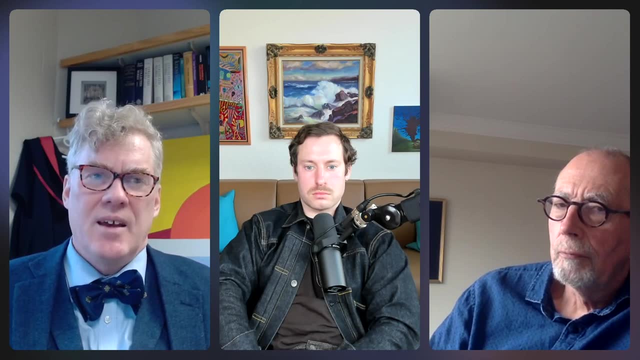 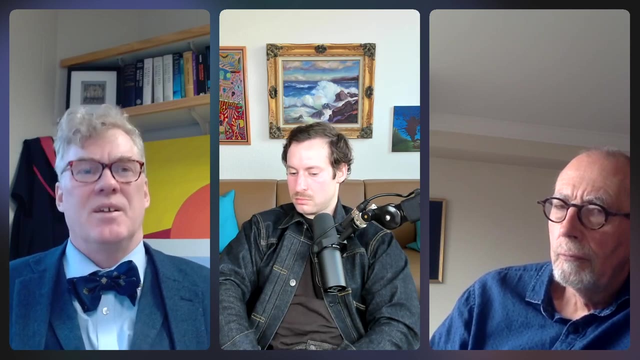 This vague infinitary realm. How can it possibly be satisfactory to, to secure our definiteness of the concept of finite on the basis Of this higher order Concept of arbitrary set of natural number? It's, it seems to just fail on its face. 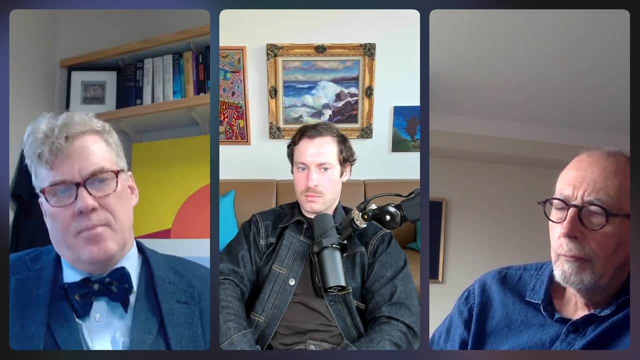 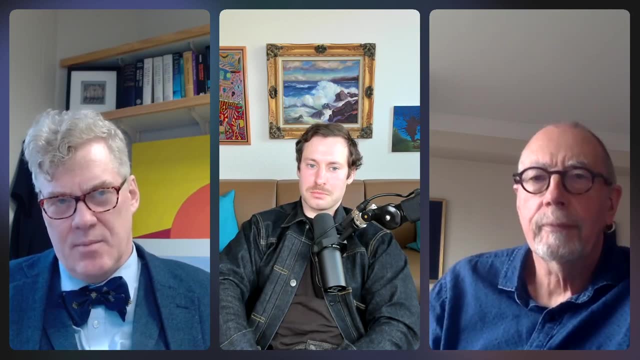 And- and that's the- The worry that I have is that actually, we're mistaken and there isn't A single definite concept of finite, and it's going to splinter and there are going to be, There are going to be mathematical developments. 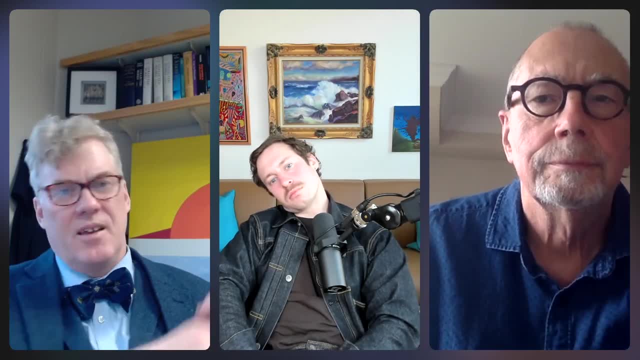 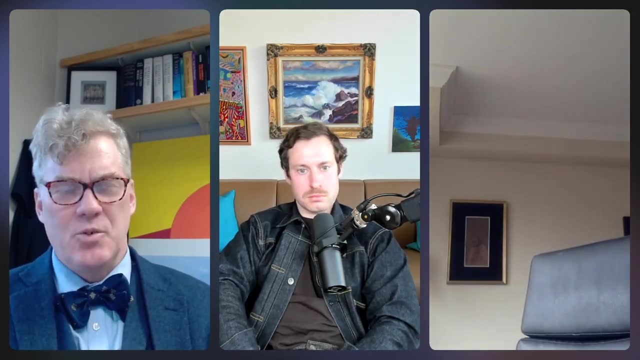 That continue. the progression of, say, Non-Euclidean geometry is sort of splintering. you know, before, Before the discovery of non-Euclidean geometry, the geometry was about the ones you know, the one true geometry. But then we realized: wait a minute. 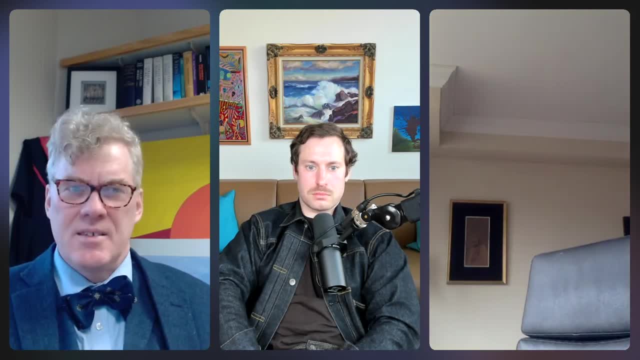 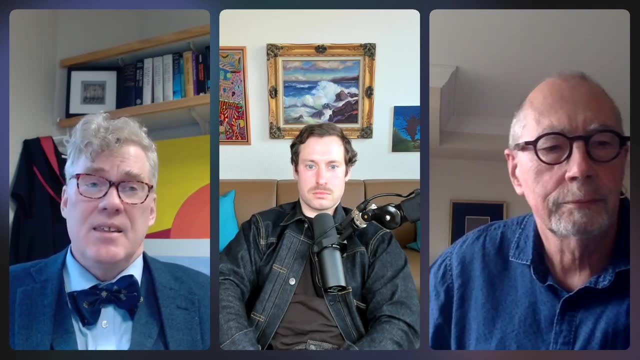 actually there's several concepts and they're not the same and they have different truths. Okay Then with forcing, we had a similar kind of thing happen In in set theory. We're leading to this indefiniteness of set theoretic truth in the 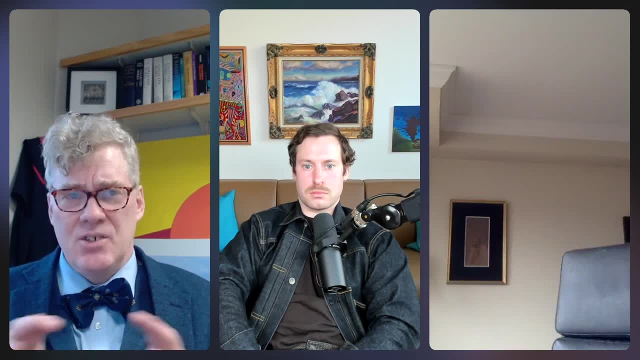 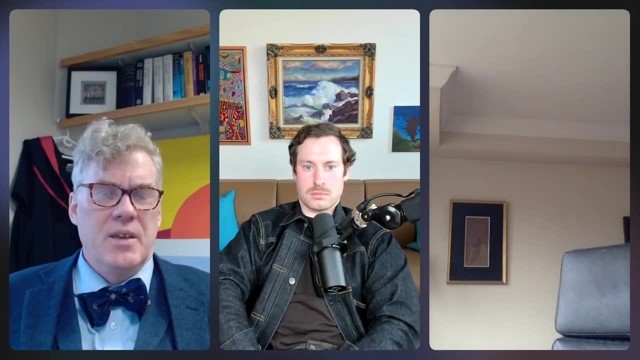 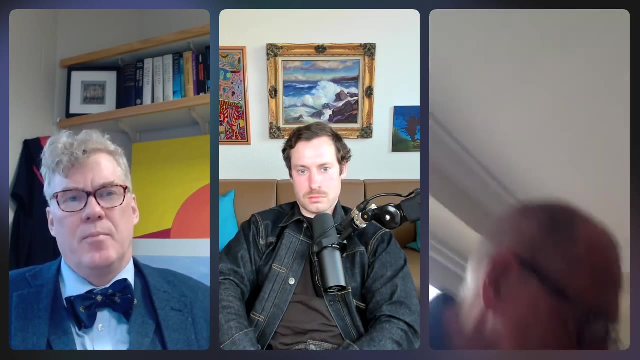 higher realm. Forcing can't change arithmetic truth, But I think that eventually we're going to realize that There will be Methods for Modifying arithmetic truth that will be just as satisfactory as the forcing method is, And and we'll change our view about the definiteness of finite numbers. 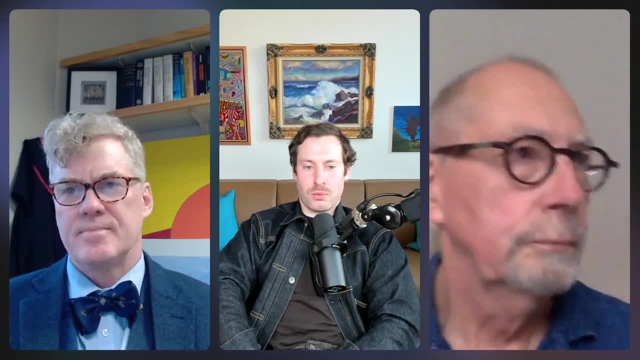 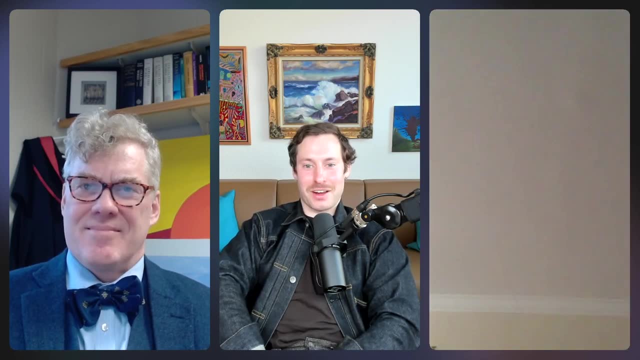 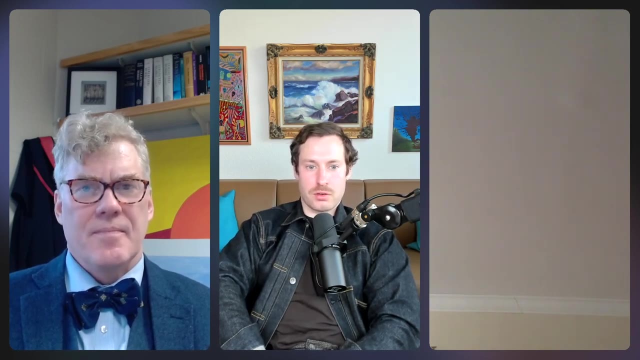 And so, Well before We To use, To use your phrase- Explore the space, Set theoretic possibility and take it for granted. You mentioned Kolnar Peter News, Who is another student and colleague of what And who you also mentioned. 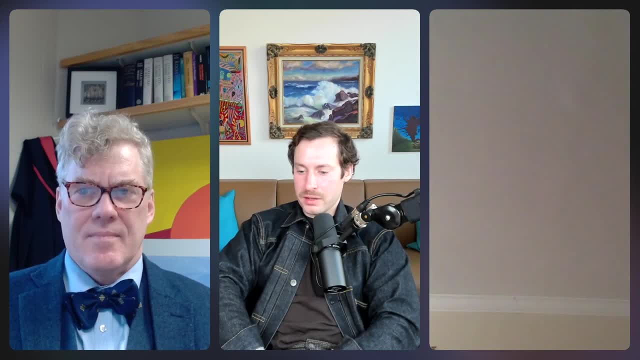 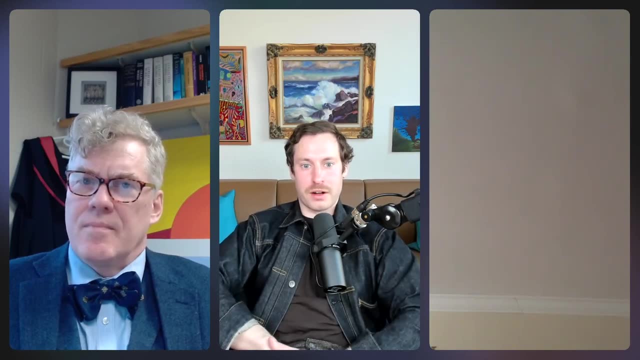 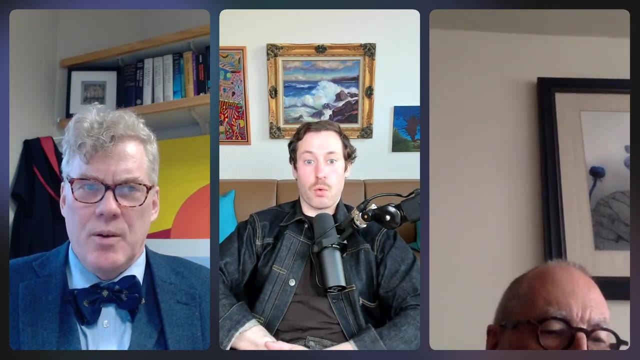 They're both at Harvard And I know that to Haim Gaifman: uh, Colner was at least one point, uh very devout sort of realist and singularist about the set theoretic universe, You said at one point, but that's what I was. 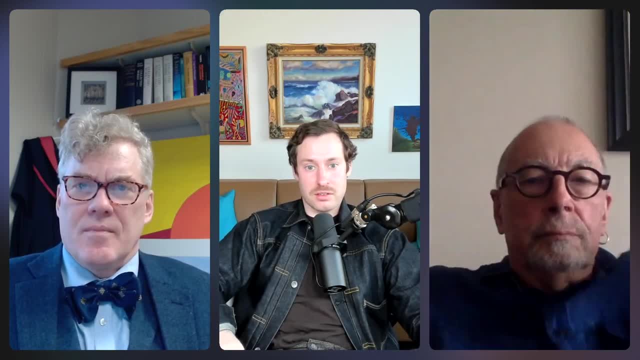 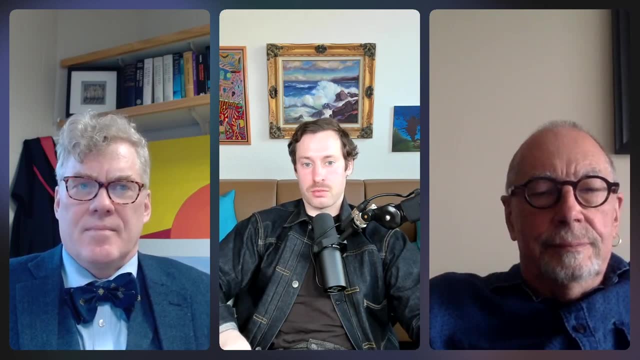 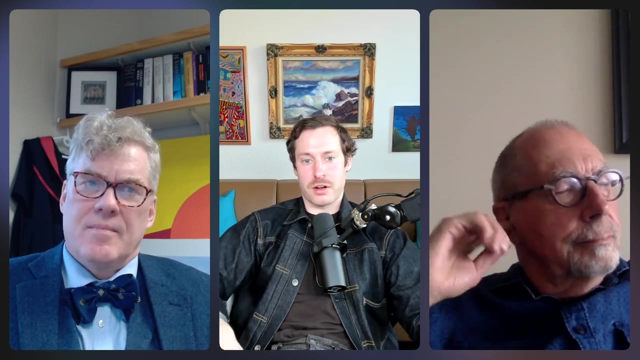 going to ask. I was going to ask if he still is And if I mean, in the same way that you tried to be open-minded when discussing the liar paradox with Graham, if you try to be open-minded with regard to the singularist picture of the set theoretic universe and 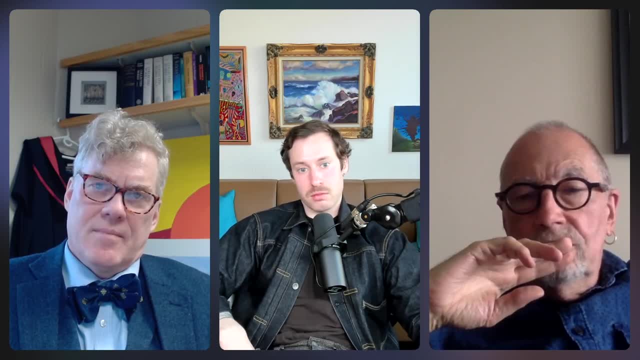 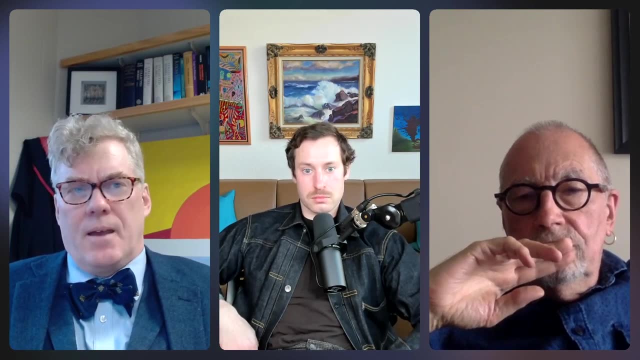 how they have argued against you, Right? So so I, I, I don't know that. I think of Colner as one of the- um, uh, monists all the way up. I mean, that's usually defended and I don't know that. 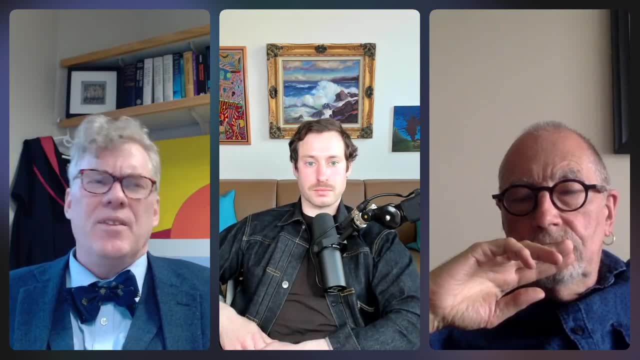 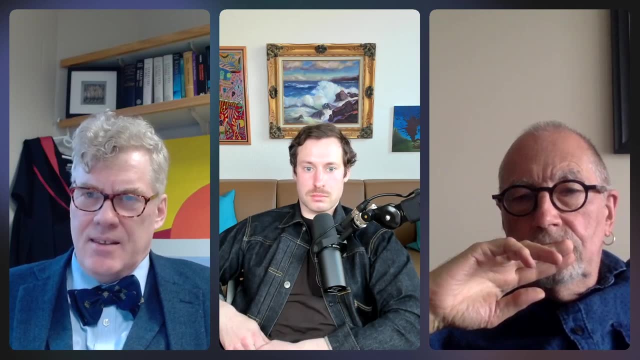 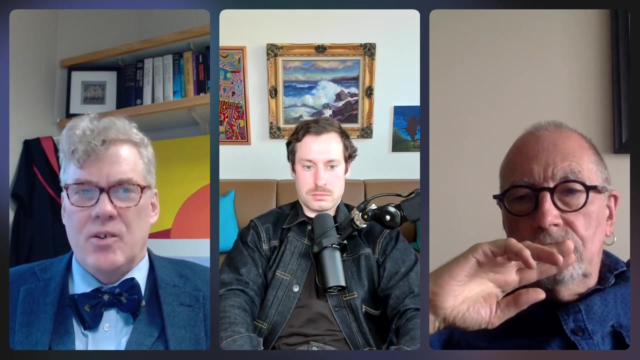 he's ever changed his mind about that. Yeah, I think so, Right. So one thing is that of course, everybody agrees on all of the mathematics and in that, in that sense, there's nothing at stake mathematically in the philosophical debate. 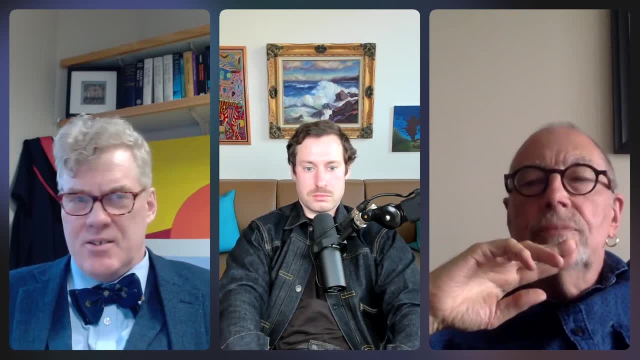 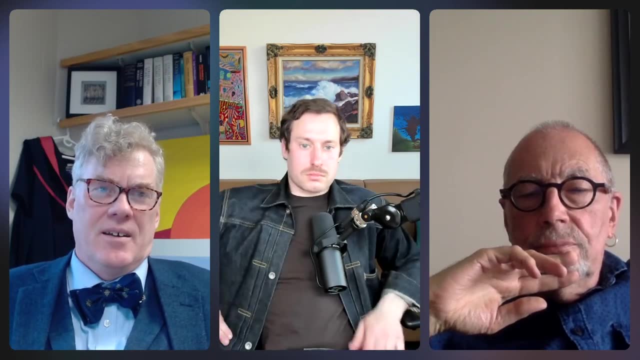 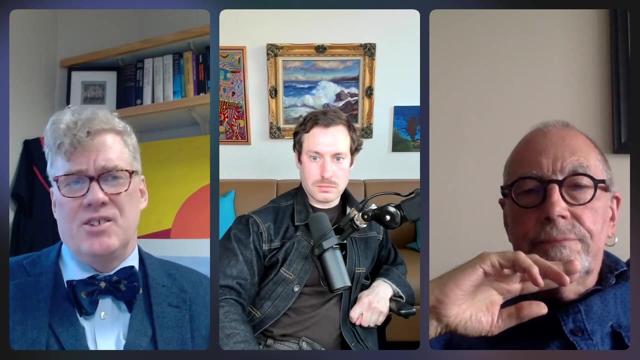 Right. So it doesn't matter if you're a pluralist or a monist or whatever, as far as you know whether your proof is correct or not. We all agree on the sort of validity of the proofs, which is different, a different situation, I guess, than if we were sort of changing the 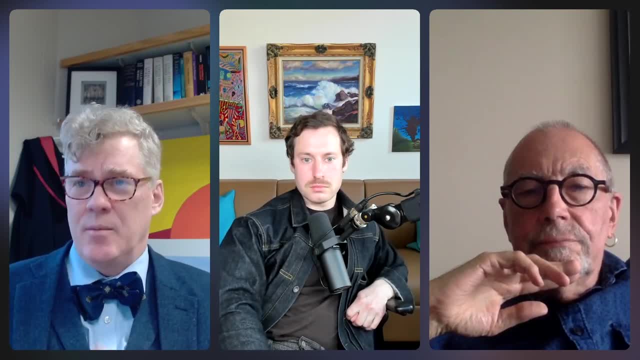 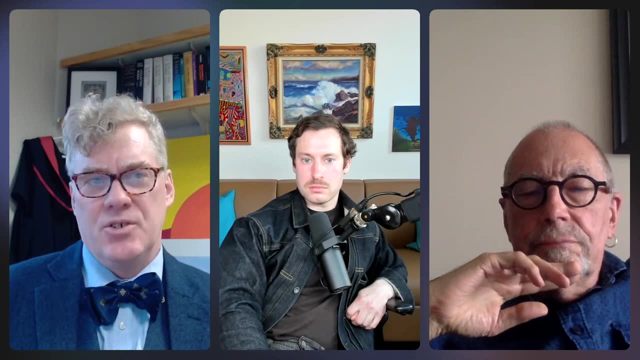 logic or something, then maybe we wouldn't agree on that, Because if one person is is working in a different logic than another, then, um, you know, the validity of proofs, the validity judgments of the proofs would change Right. So in the set theoretic case, 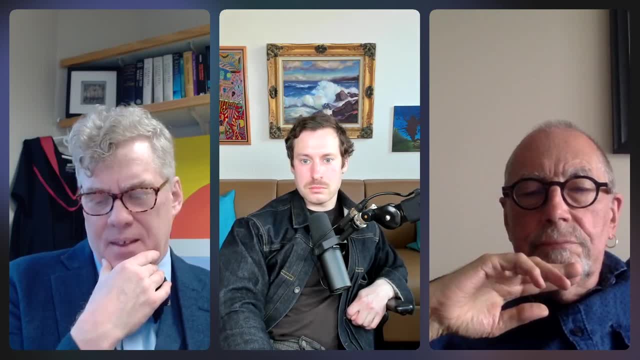 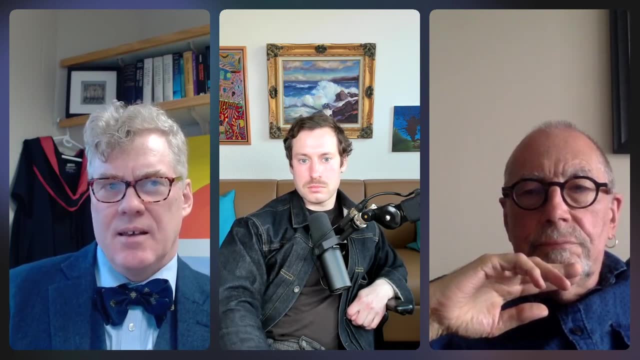 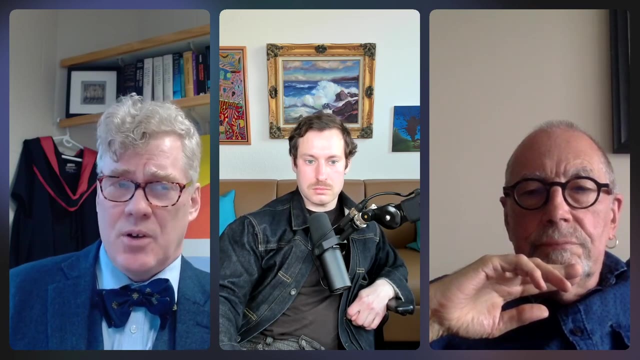 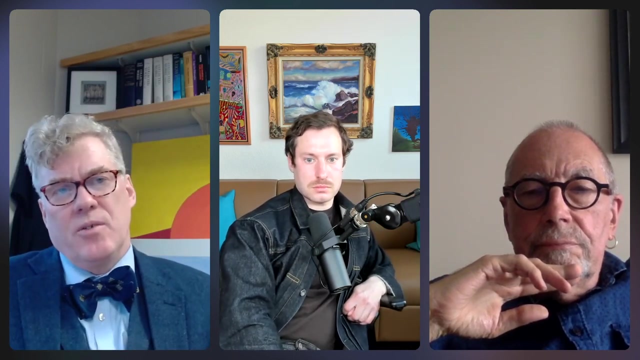 I mean with set theoretic pluralism. um, what the debate is really about, I think, is a kind of proxy. The philosophical debate is about where we should go. which projects, which set theoretic projects should we find Interesting or fruitful? And, of course, if you are, have the monist point of view. 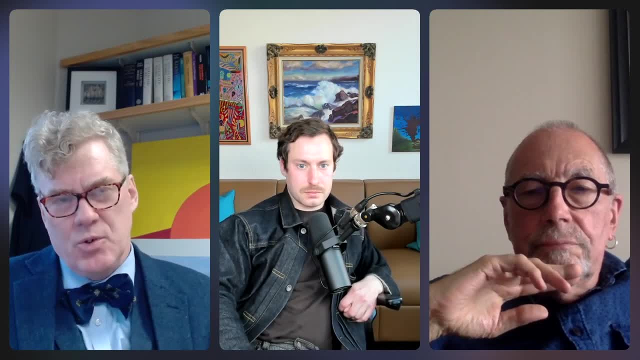 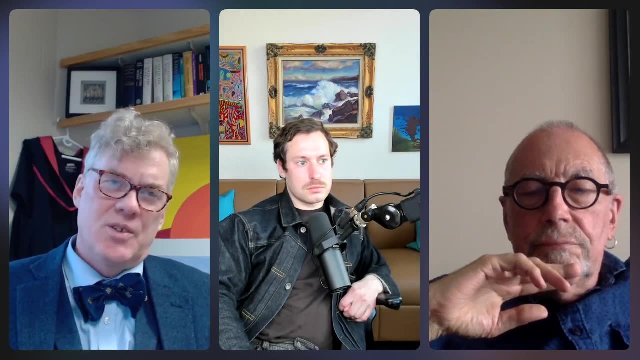 then you're going to be led to find out what's really true in the one true universe, And so you're going to be led to try to formulate what. what does it mean? How will we recognize the truths of the one true universe? You know by what, by what criteria will we judge something? 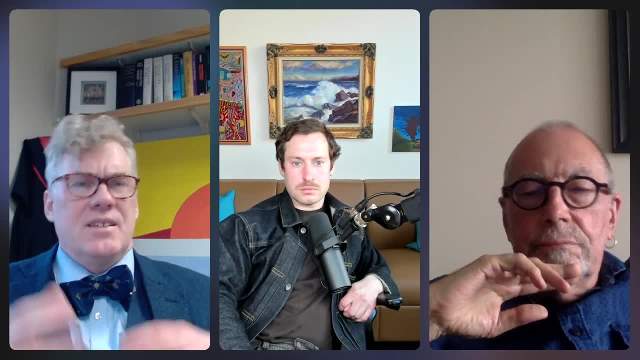 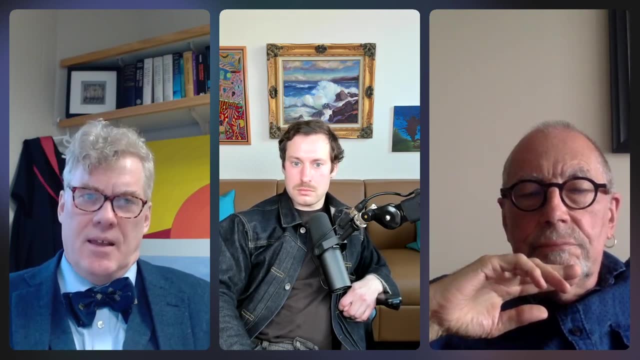 is, is you know fit, And so this has led to um, uh Woodin's work on the, um, ultimate L and, and this kind of thing is sort of candidates for uh, for this uh, you know. 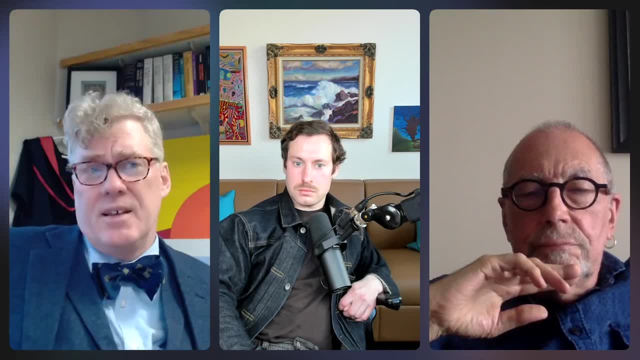 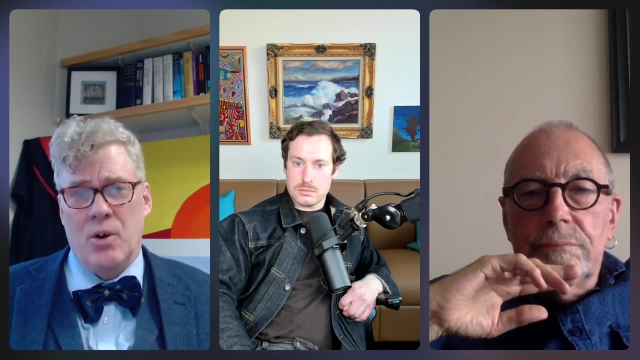 this definite truth and so on, Whereas if you're a pluralist about set theoretic truth, then naturally you would want to be kind of exploring the multiverse and so on, which is what my work on the mode of logical forcing has done, And my work on set theoretic geology is about that kind. 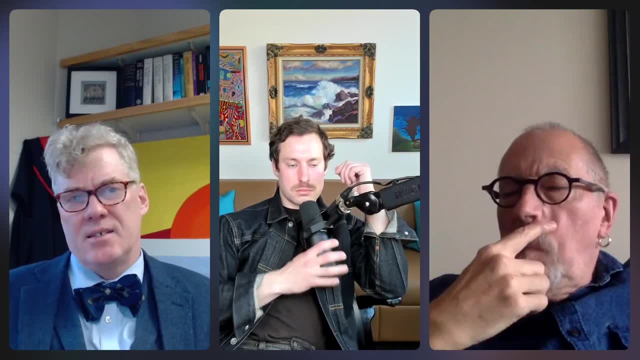 of thing, And and the sort of potentialist analysis of different different potentialist accounts of set theory is also, you know, important. So, um, I think that's, I think that's very, very important- can be seen in that light. 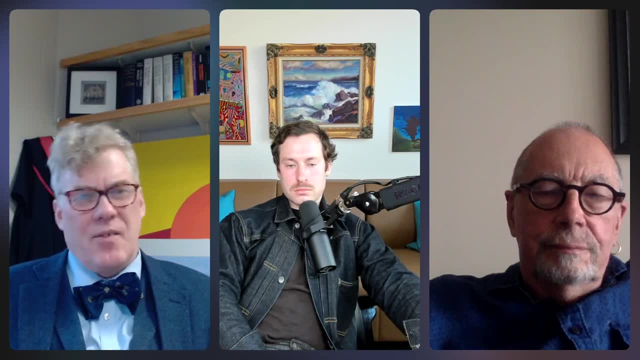 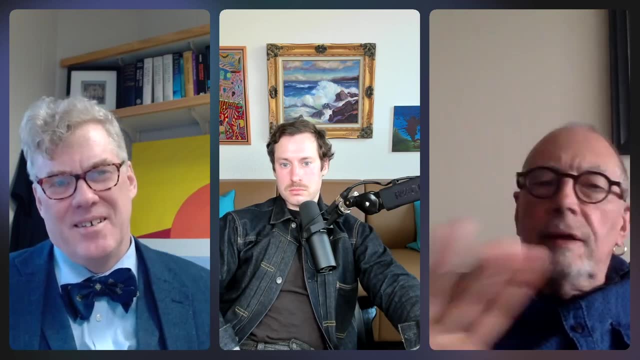 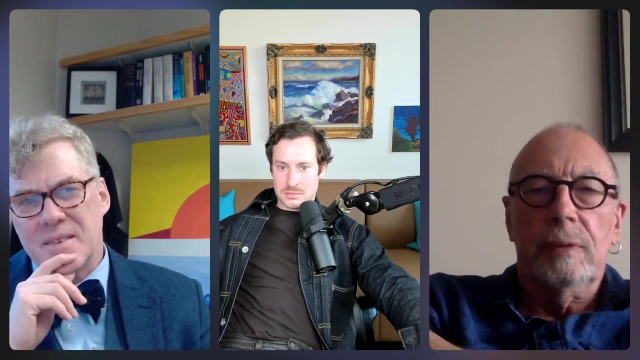 And so maybe the philosophical dispute doesn't actually have any consequence. for I'm not sure. Graham, can you say something about how that kind of issue plays out in logical pluralism? Yeah, well, it's not to. Let's leave logical pluralism aside. 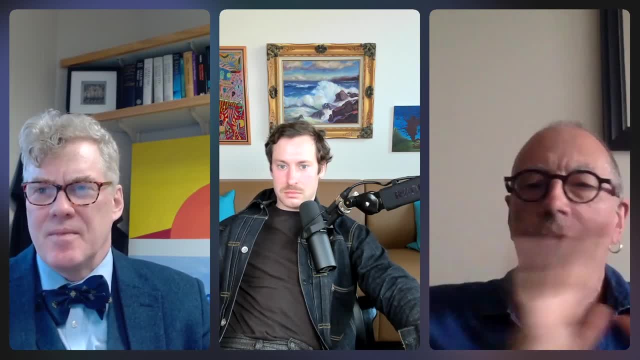 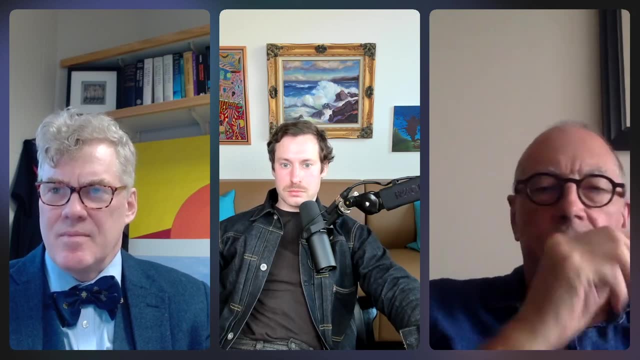 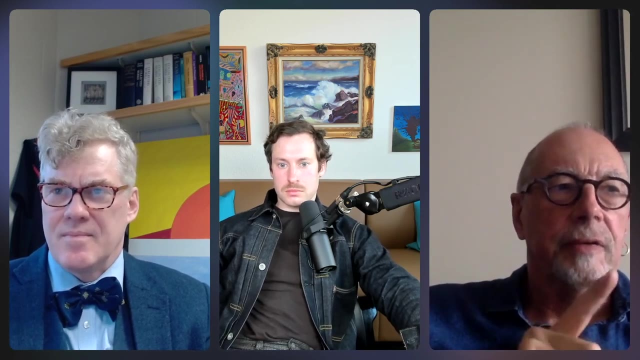 and mathematical pluralism aside, because I agree with you that those are separate issues. Okay, And let me return to the philosophical. Let me return to the question that Robson raised about the philosophical problem of the view, But let me prefix this by saying that 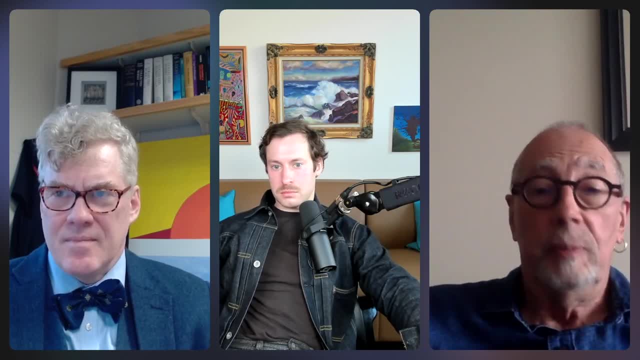 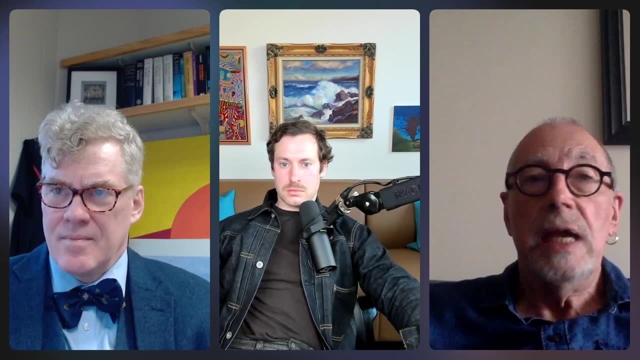 I'm very sympathetic to your view about the secularity of the pluralists. okay, The more I've thought about it, the more plausible it seems to me. Is there a reason you used the word pluriverse instead of multiverse, though? 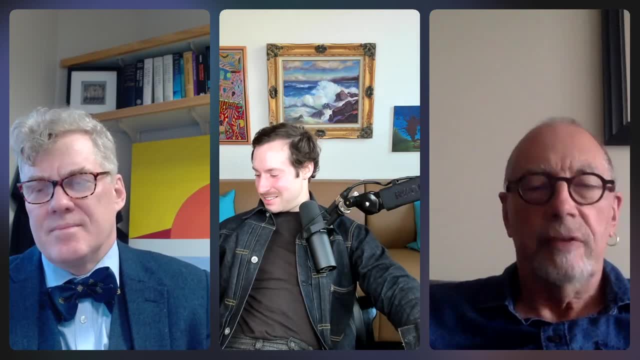 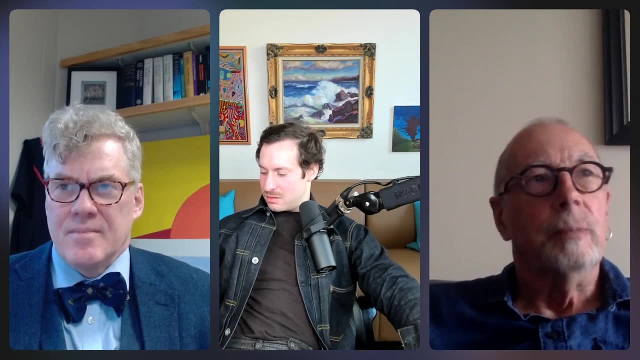 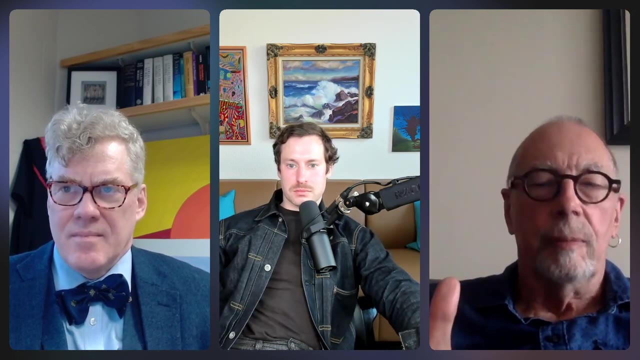 Okay, Just kidding. Even to the extent of the arithmetic stuff, I mean, once the determinacy of the past operation goes, all bets are off right. So, um, I'm still uncertain about some things, but I'm generally very. 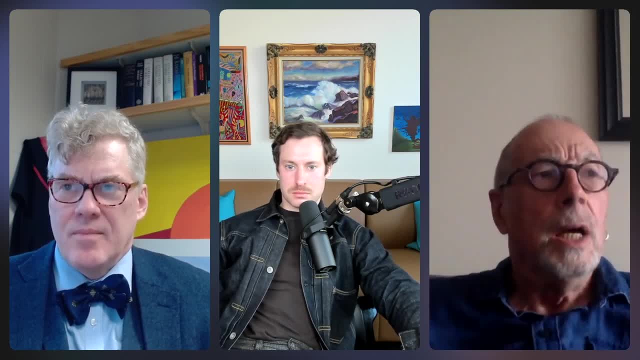 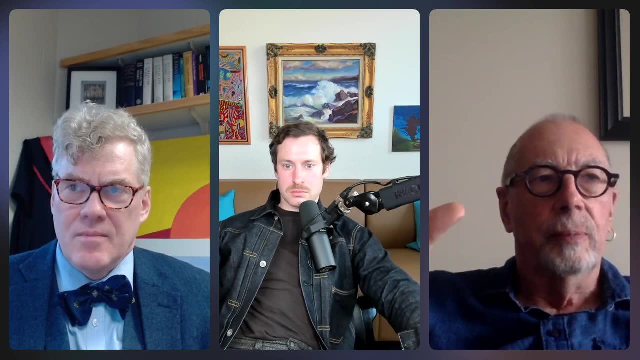 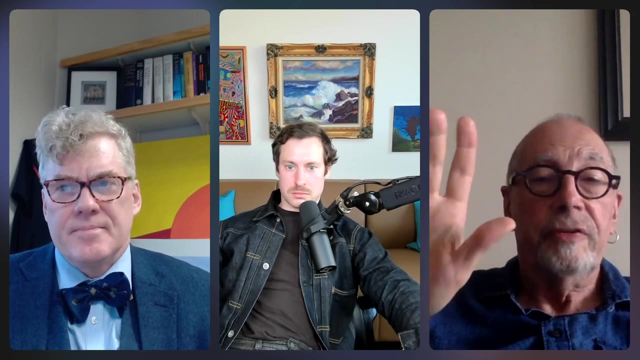 I'd like to be on board with the view, completely right. So Robinson asked why people have problems with the view, And these are philosophical problems. They're not mathematical problems, as you pointed out. But there is a very standard objection which you're well aware of. 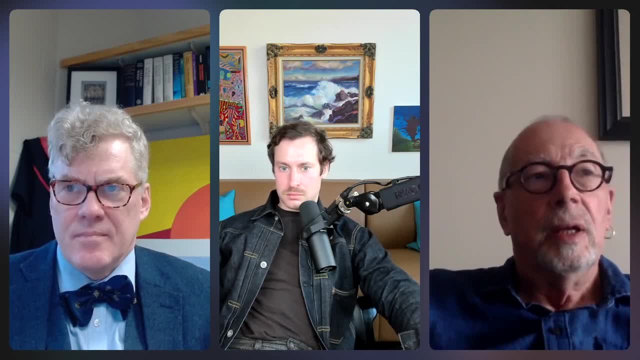 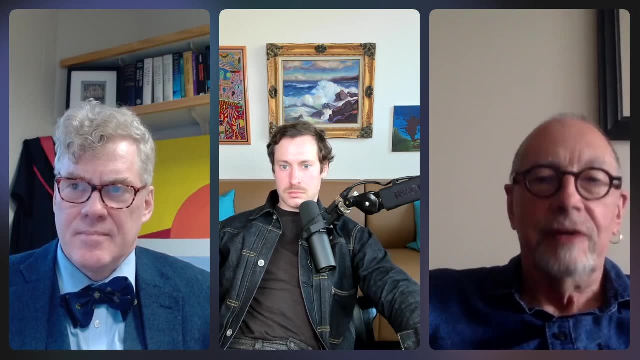 because we've talked about it before, And that is this: When you're investigating the multiverse of the pluriverse, or whatever you want to call it, where are you investigating it from? So it looks as though there's some kind of hyper-pluriverse. 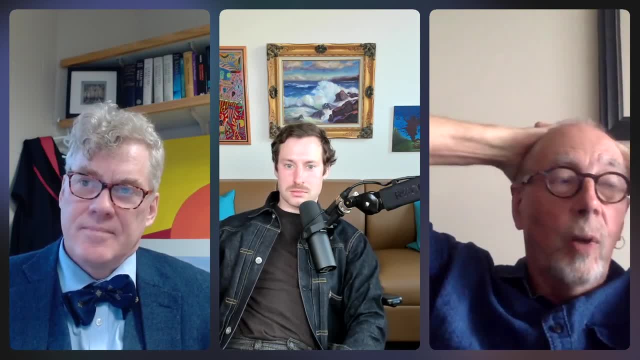 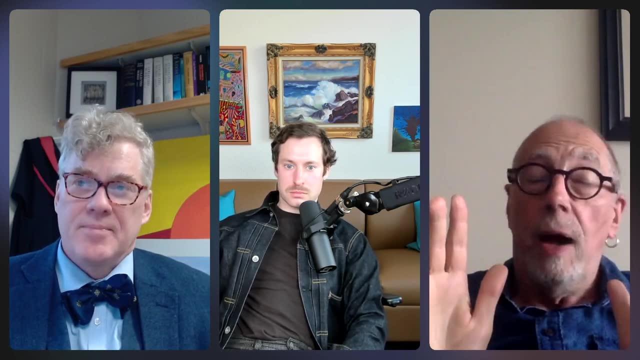 which contains all the plurality, And you're working within that, okay. So that's an objection that I'm sure you must have heard many times. Sure, sure, yeah. Now I actually think that there are ways of getting around this objection. 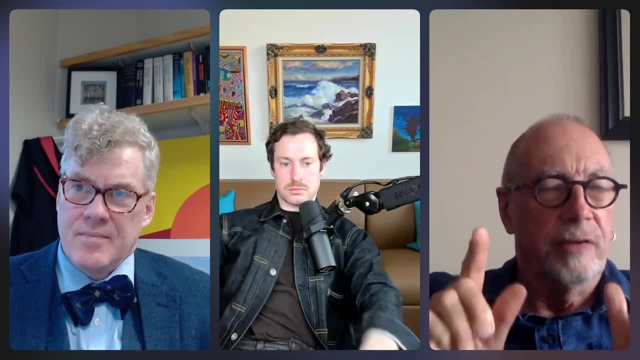 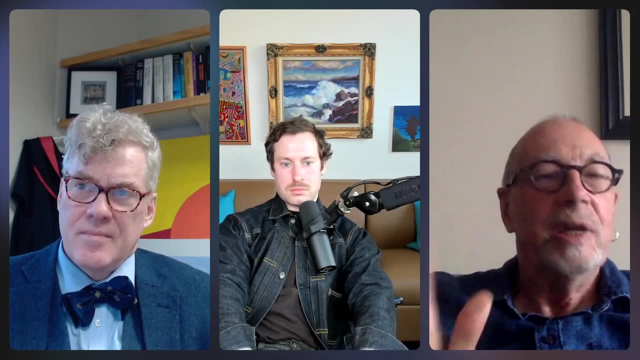 We can expose that as well, but I suspect we're kind of on a similar page there. But there is one version of this problem which worries me And I'd be happy to be told it's a confusion, but since I've got you here, let me put it to you. 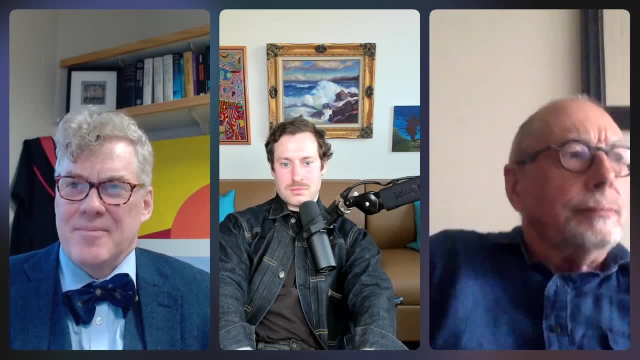 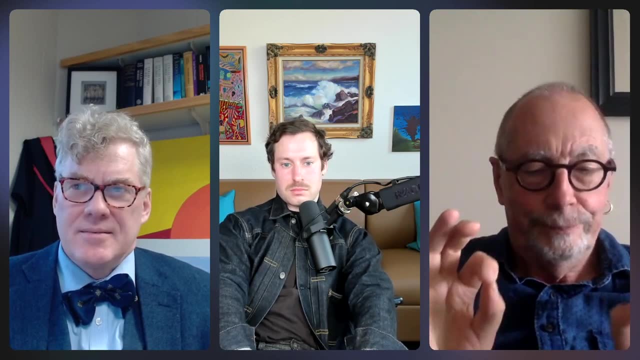 and see what you think. Okay, And you'll see why. it's a facet of this problem, but it's a very specific facet And it goes like this: Take some set theoretic member of the pluriverse, some structure, right. 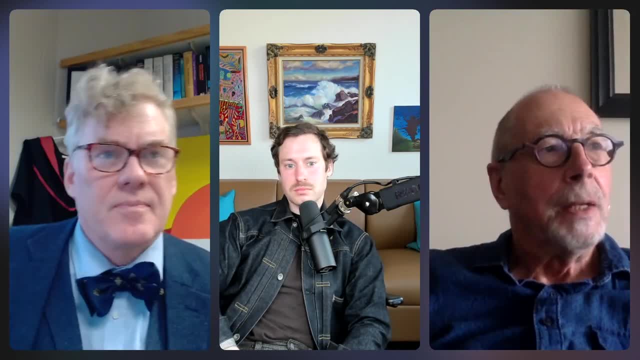 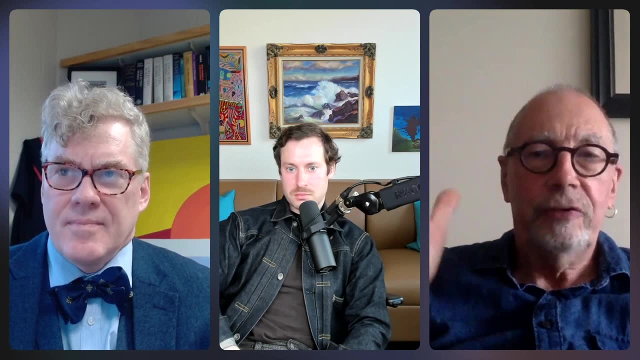 Take some set of it, Ask whether it's countable or not. Well, of course, from a pluriverse perspective, that doesn't make much sense, Because this structure is going to be in two different structures. Let's call them M1 and M2.. 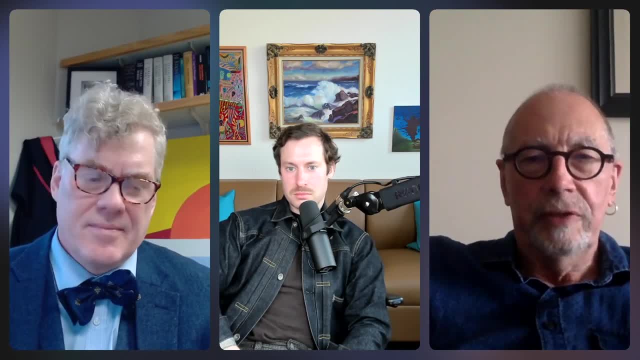 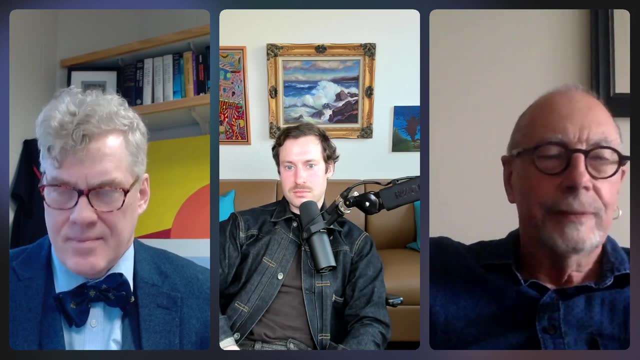 And according to M1,, X is countable. According to M2, it isn't Okay. So it looks like you've solved the problem. The truth is relative to whichever of these structures you're in. Okay, Fine, as far as it goes. 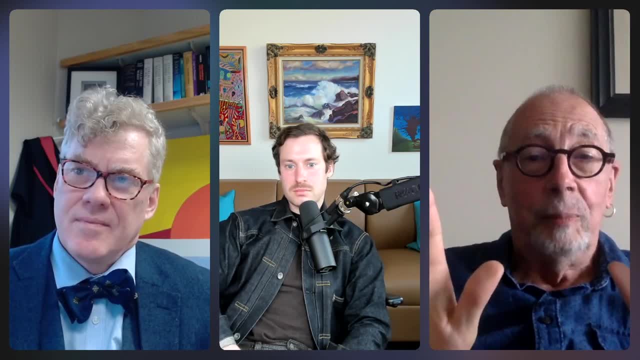 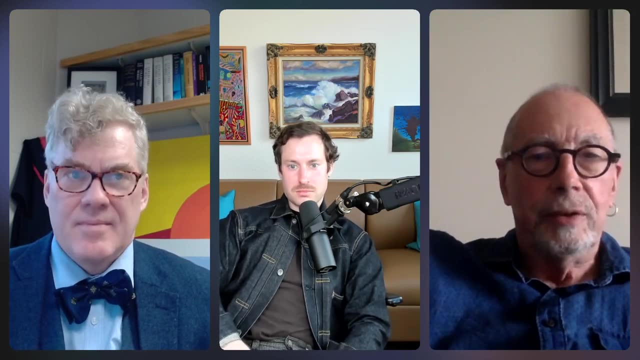 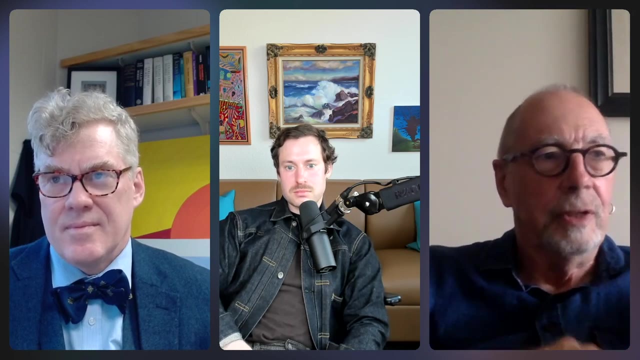 The trouble is that it don't stop there, Because M1 can be in different structures itself, Let's say M3 and M4. And according to M3, X will be countable in M1. And according to M4, X won't be countable. 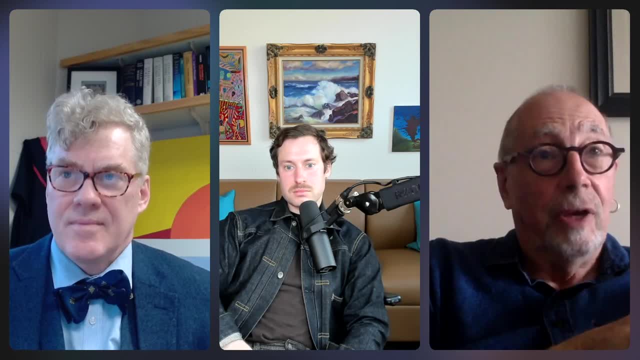 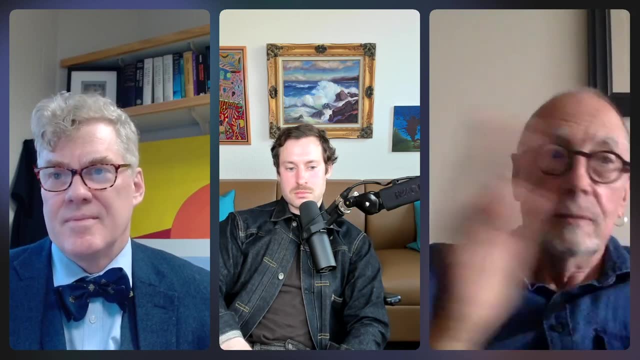 with respect to M1.. So you're going to get different answers depending on whether you think of M1 while a member of M3 or M4.. Okay, Fine, But of course the problem iterates Because you can go all the way up, whatever up. 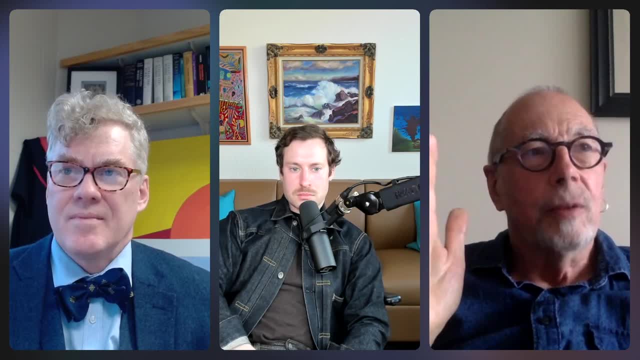 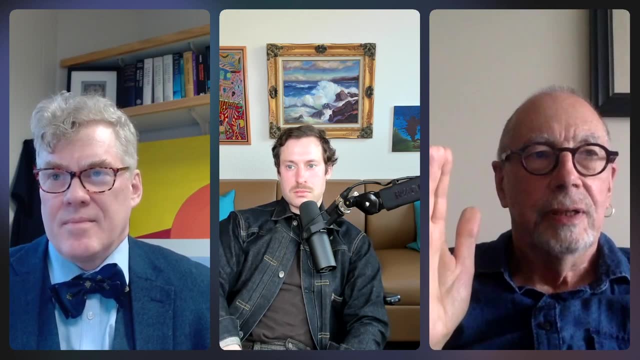 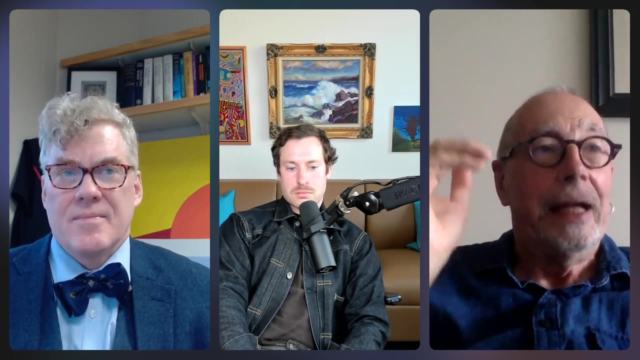 means in this context, And the worry is that you've traded in truth for truth in Australia, But now truth in a structure has become truth in a structure, in a structure, which has become truth in a structure, in a structure, in a structure, And truth's implicator. 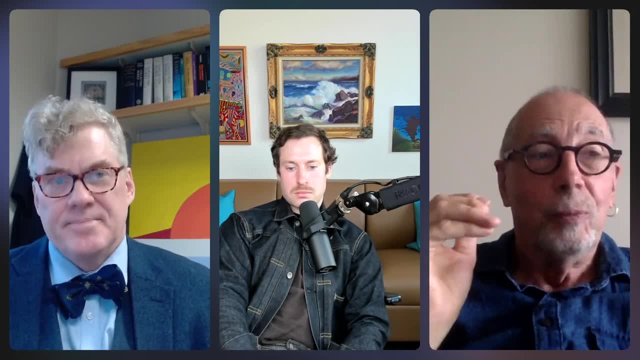 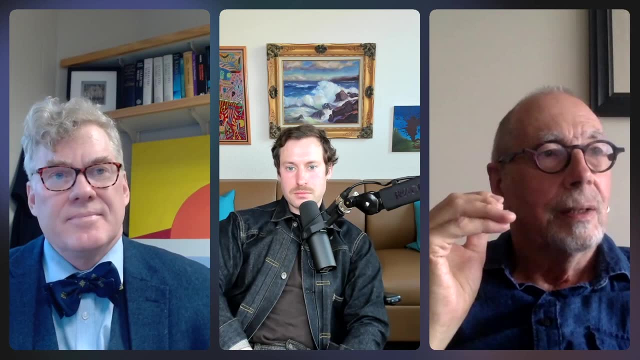 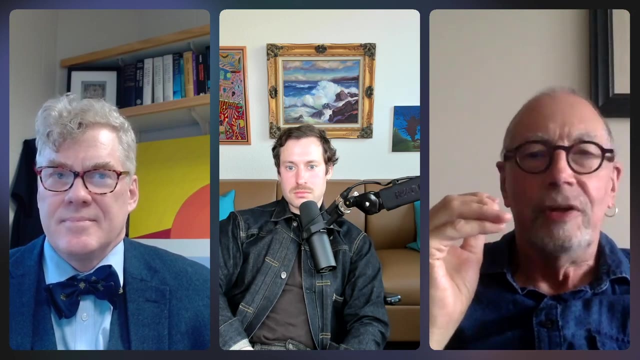 has just disappeared from the picture. So what the hell is one doing when one examines these things? I mean, the notion of truth in a structure has now become unstable And it's not clear what you're doing when you ask the question. Is it true in the structure? 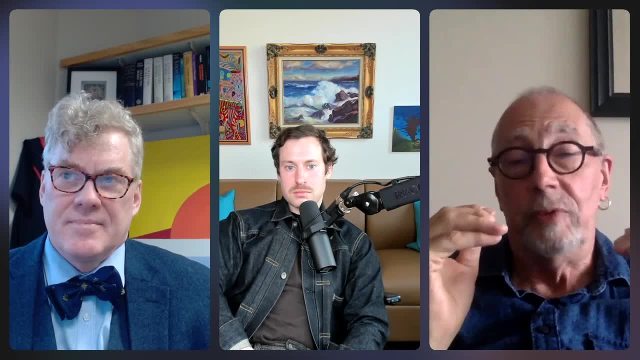 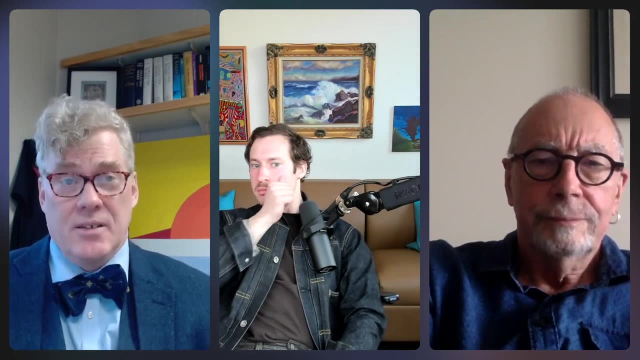 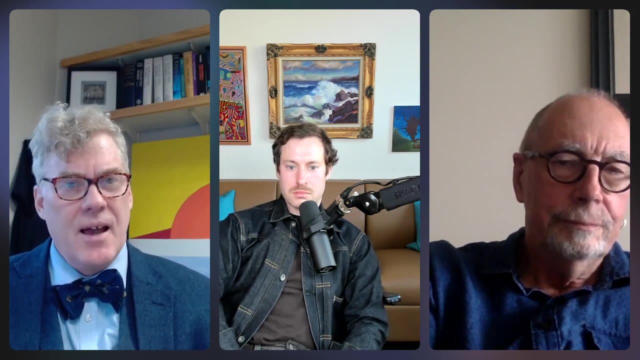 I mean, that's the version that sort of worries me about this objection, now I see. So let me respond, because I definitely have heard this and thought about it a lot actually, And my view of the matter is that I just bite down. 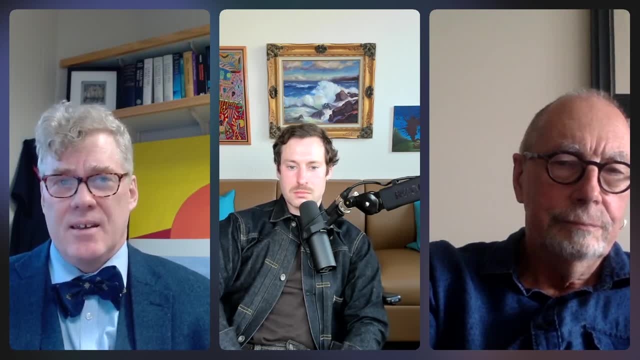 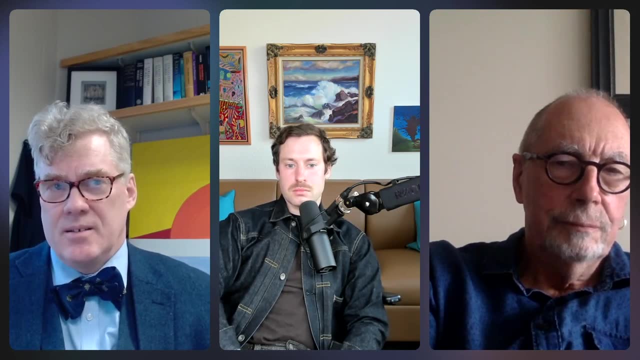 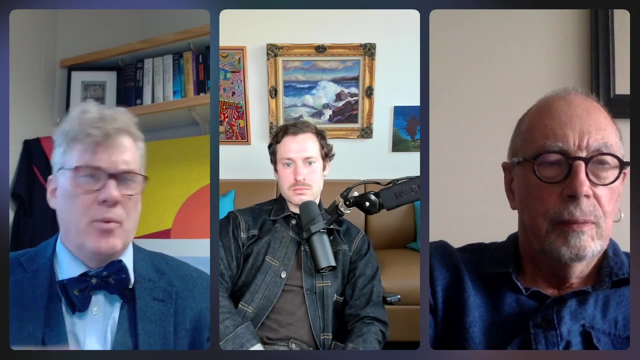 hard on everything that you just said and say that that's the nature of the metatheory-object theory. distinction is that there isn't just two round every set theoretic context, or maybe we call it a model of set theory or a universe or whatever. 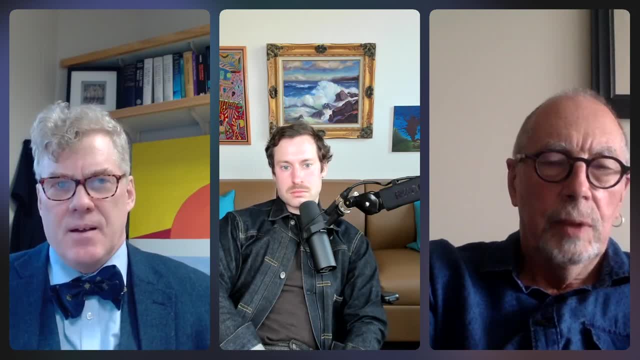 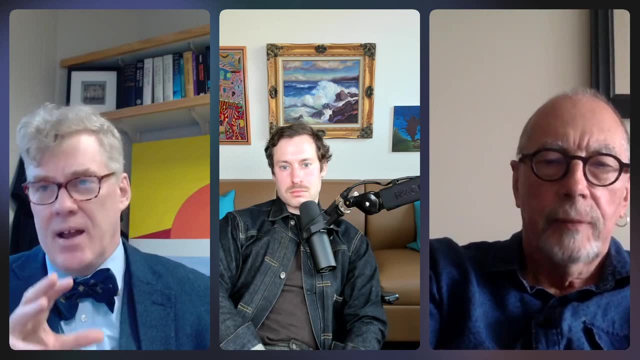 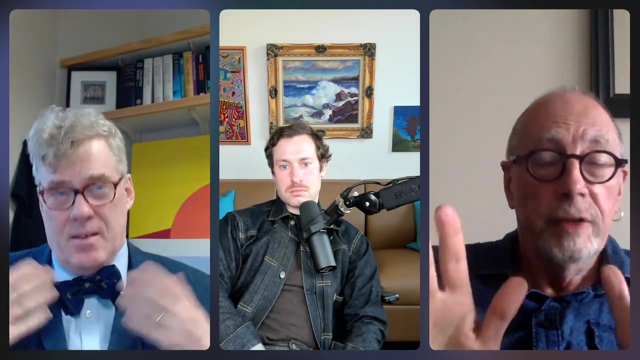 Any realm in which you can do, say, set theory provides a metatheoretic context for the objects that are available there and it itself might be an object theoretic realm in a higher one, and so on. I understand that view, but I'm worried. 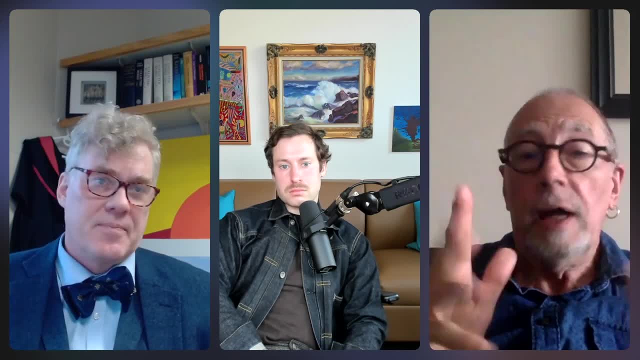 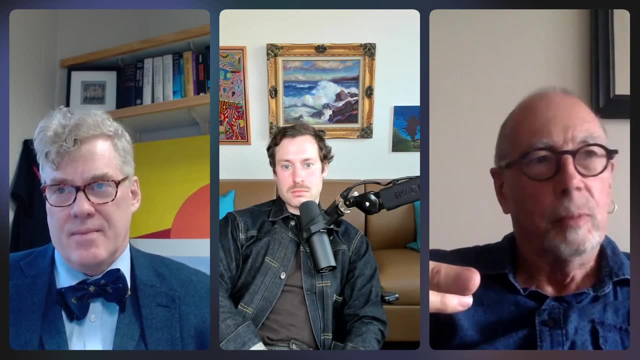 that there's a vicious regress there. So if I ask you: there's this set, let's call it X, is it countable? And you say: well, it is in this structure, but it's in that structure, That's fine. 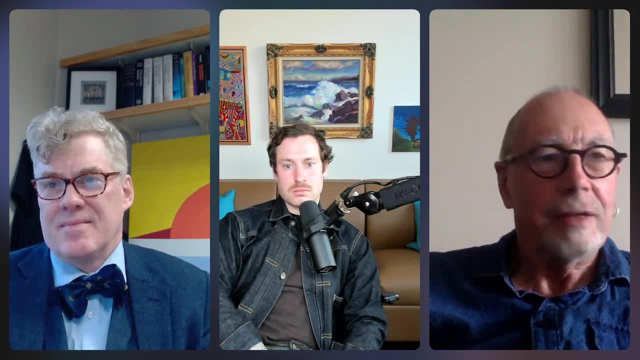 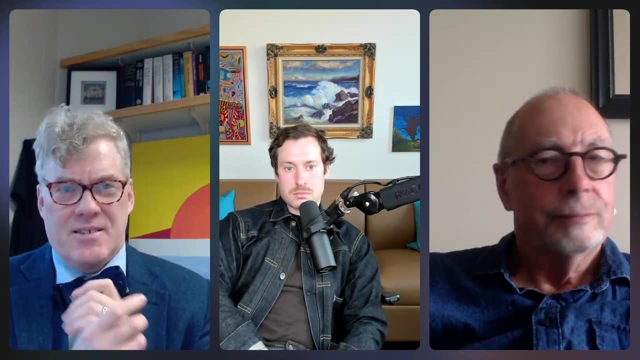 And I say yeah, according to which structure? Because that answer is going to vary. I mean, you can make, for example- it's like Skolem's paradox on steroids or something. You can have three models: M1,, M2, M3,. 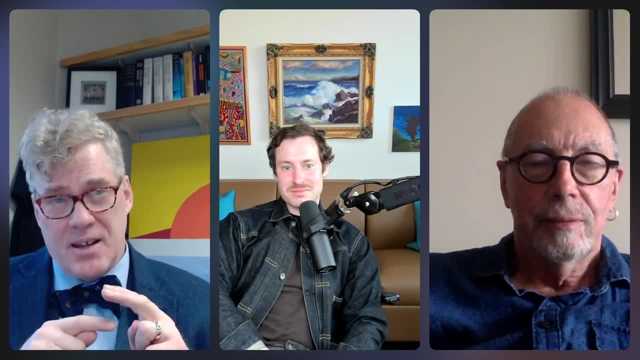 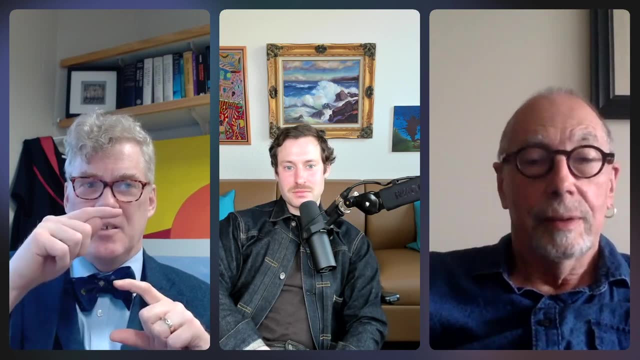 and they're contained, and you have an object in the bottom one and it's thought to be finite in the smaller model and it's thought to be uncountable in the middle one and countable in the top one. I mean so even so. 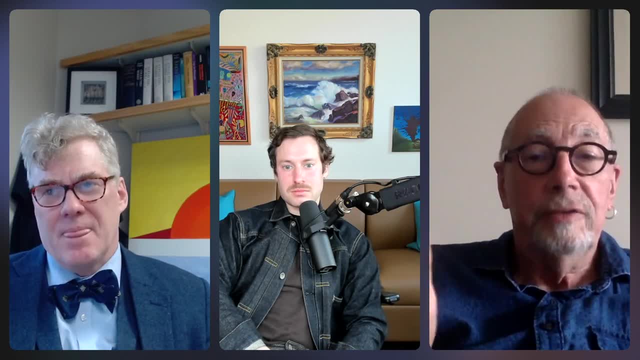 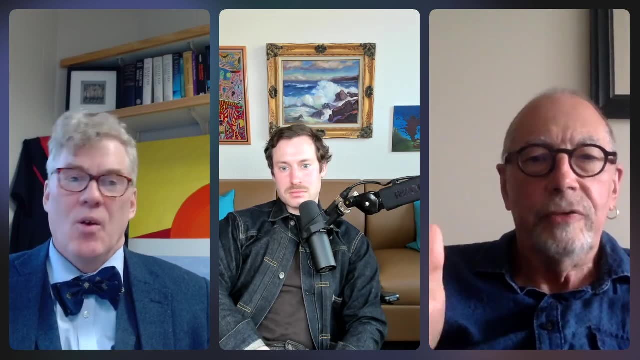 you can make this happen. So when I say to you: is this set countable or not? Right, How can you get a coherent answer? Because it is in this structure but not in that structure. But that's not determinate, because that depends on which structure. 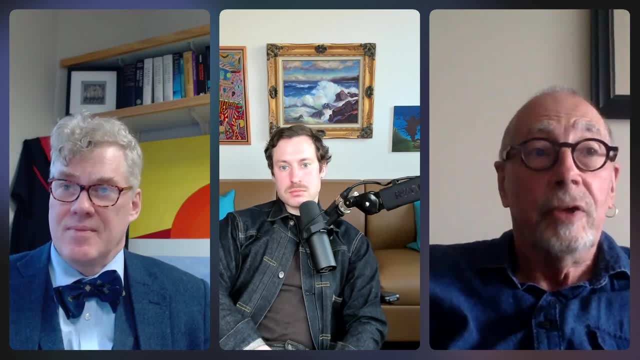 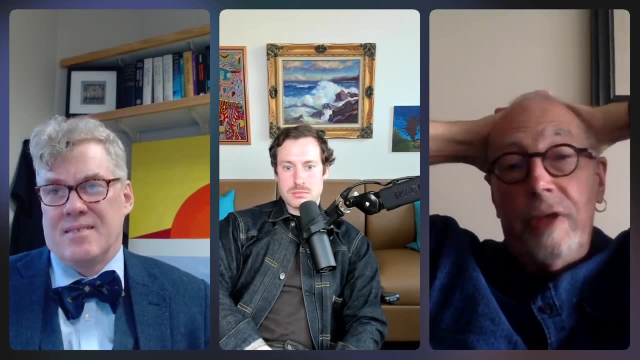 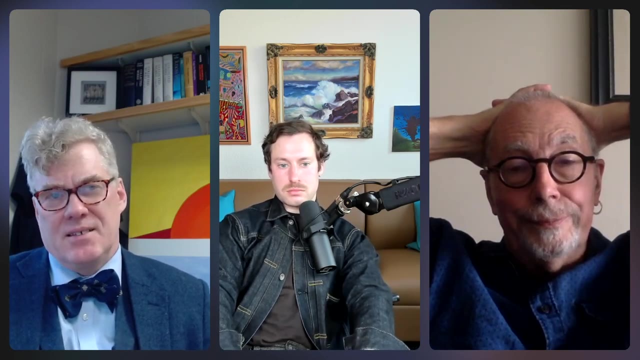 those structures are structures in, So there's, there's a regress here, and the worry is that you've just the regress voids any answer you give of determinacy. Well, I mean, it's sort of like the it's de re. 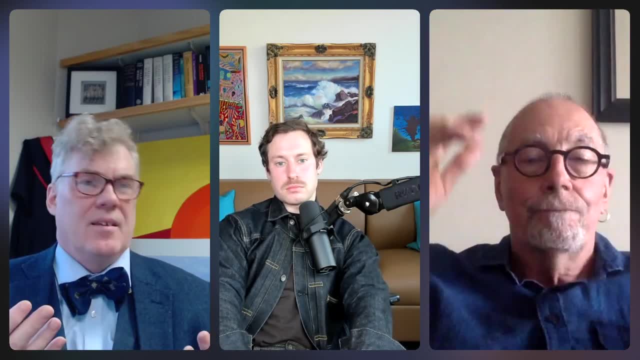 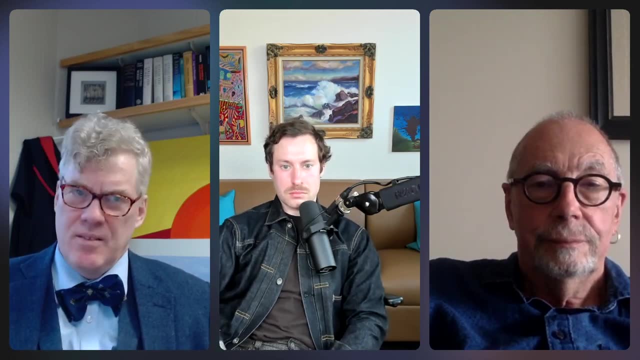 de dicto issue, isn't it? Because the I mean, why can't one just answer? look, if I'm making a mathematical assertion, then these are always relative to the. you know, the current set theoretic universe, which is set by 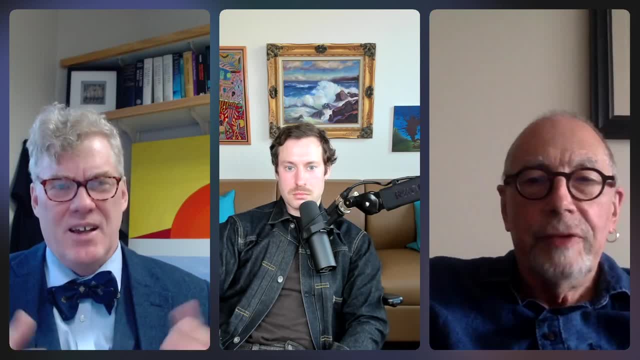 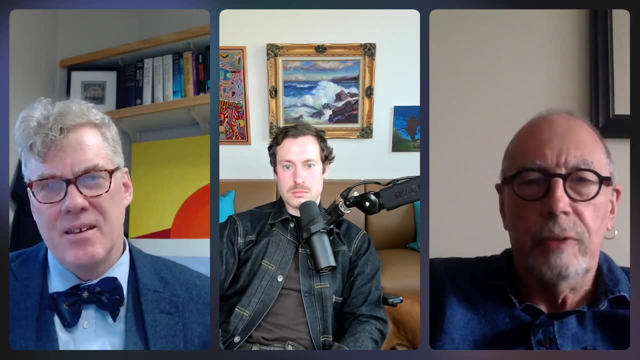 context and often not stated explicitly, and so on. If I say the reals are uncountable, I'm sorry what? There isn't a unique set theoretic universe. No, no, I'm not saying a unique one, but 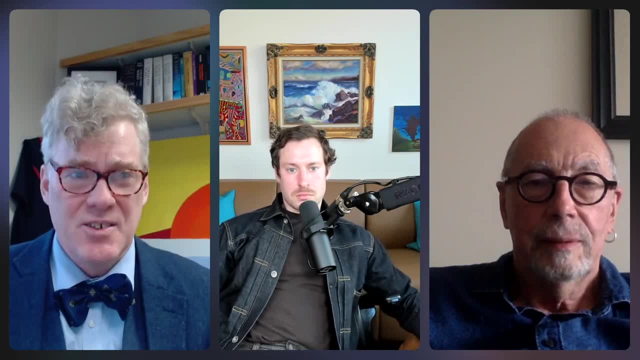 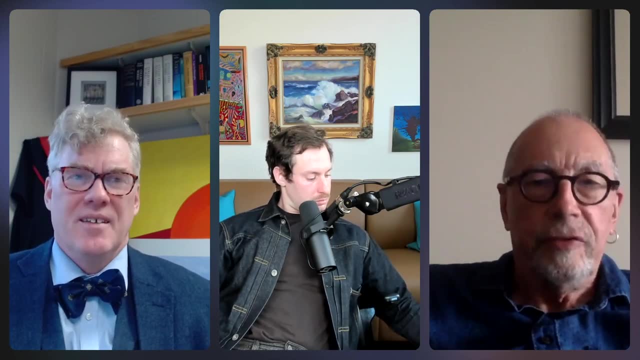 any such mathematical statement is always to be understood as sort of relative to perhaps unstated universe. right? If I say the reals are uncountable, It's self-relative. No, but we can use for example to say the reals are uncountable. 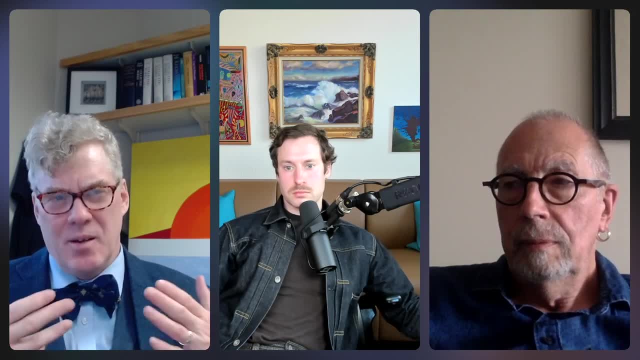 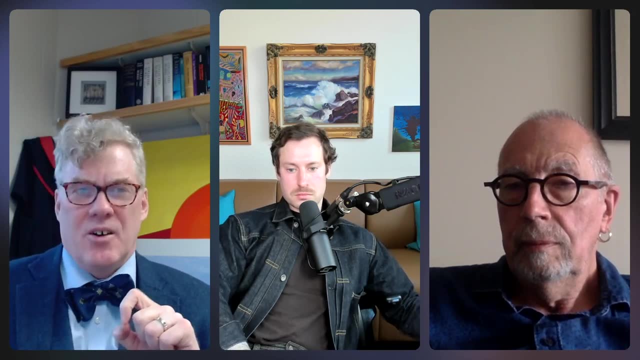 is a kind of de dicto assertion I'm not talking about, you know, that set of reals which I recognize can be countable in the forcing extension in which you collapse, that cardinal. but rather I'm understanding the reference de dicto to be the reals. 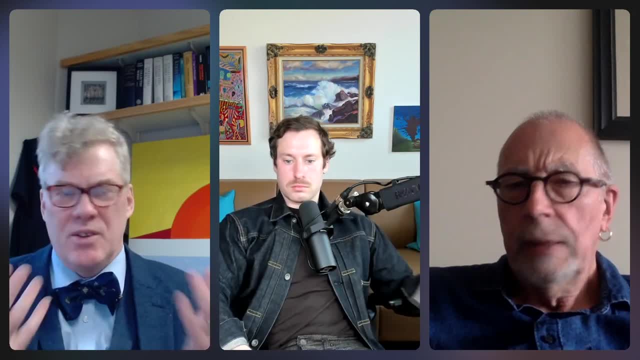 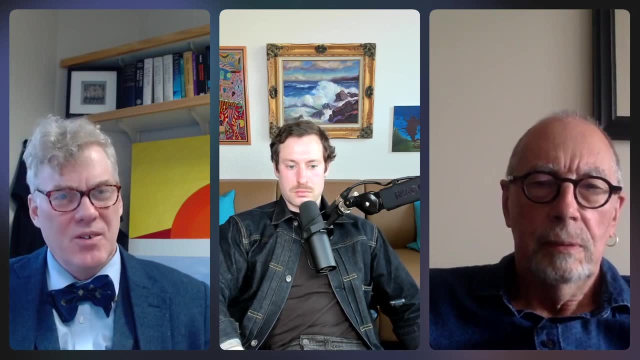 of the current set theoretic universe, and if CFC is true there, then we can do Cantor's argument. What's the current set theoretic universe? Well, whichever in any of them, you can go in there and take the reals. 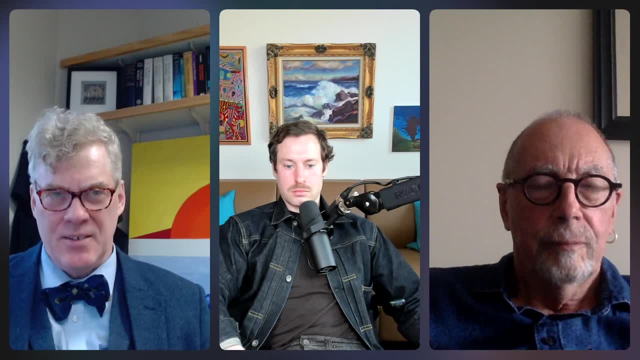 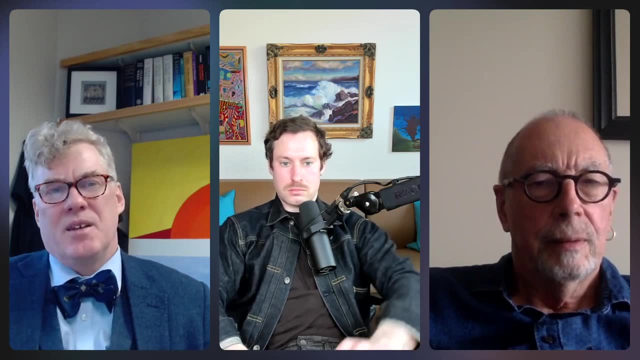 that are available there and they will be uncountable in that one. And that's just the de dicto reading of the statement, right? So I'm not making the statement about the object that you thought it was, I'm making the statement, you know, by reference. 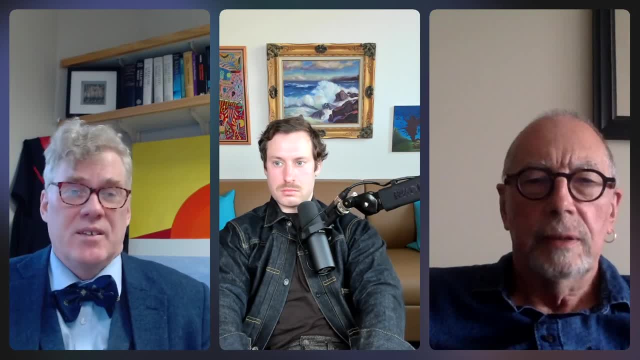 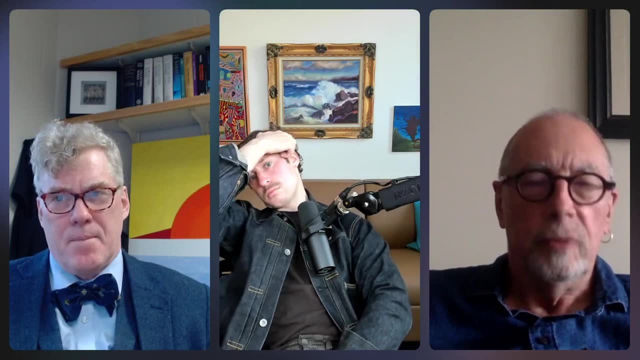 to a certain description, the set of real numbers, And Look, I'd be very happy to be proved wrong. okay, but I don't see that going de dicto helps, because what holds de dicto in a model may well depend on which. 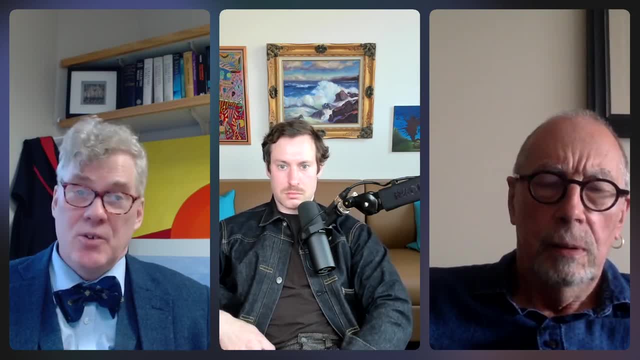 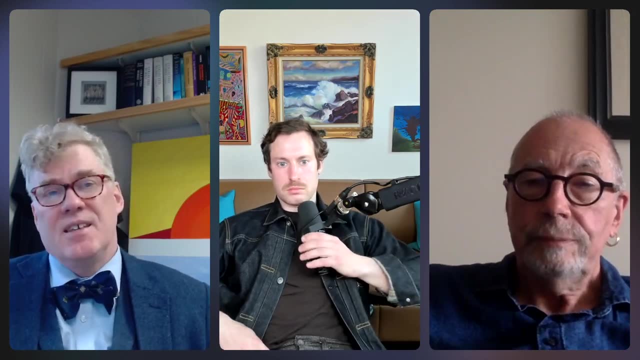 model. that model is in, I agree, but it's harder to make instances of that. I mean, just take the claim. the reals are uncountable. You know, we can prove this in CFC. It's going to be true. 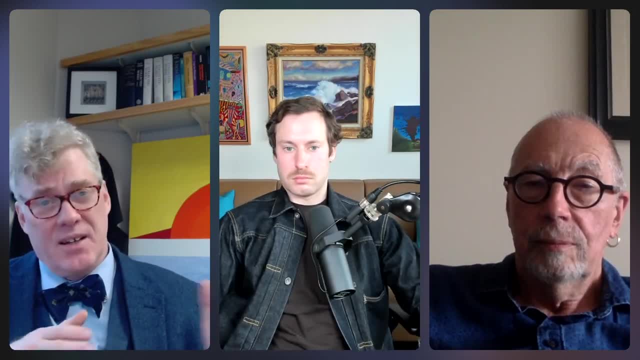 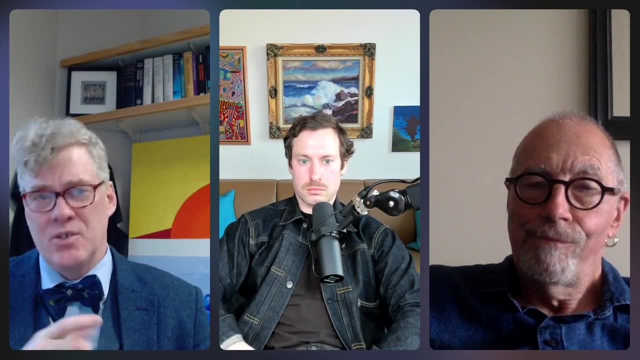 in every set theoretic universe when it's interpreted as being uncountable in that universe. and that set of real numbers in that universe is uncountable in that universe means that that universe doesn't happen to have a collapsing function, even if some other universe. 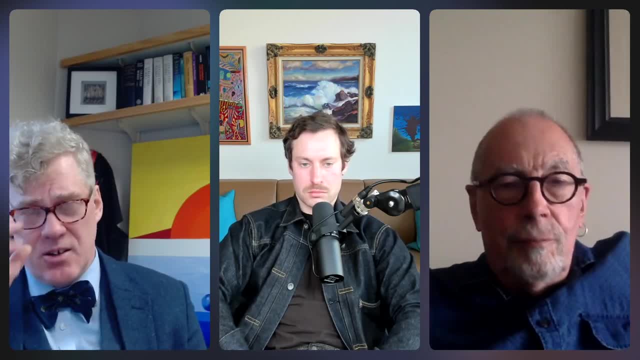 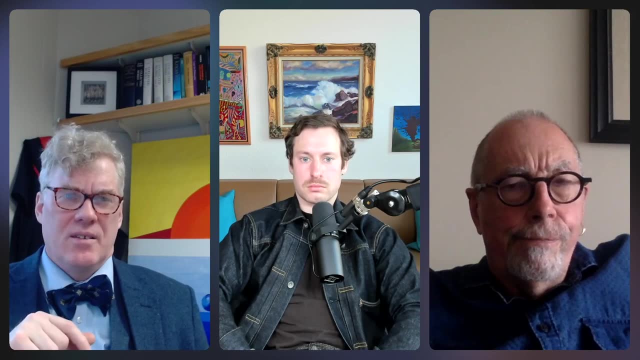 will think differently. This other kind of situation that you're describing- which is fascinating, by the way- I think they're much harder to produce, instances where the satisfaction relation itself is the thing that's changing. No, but there's a paper of yours where you 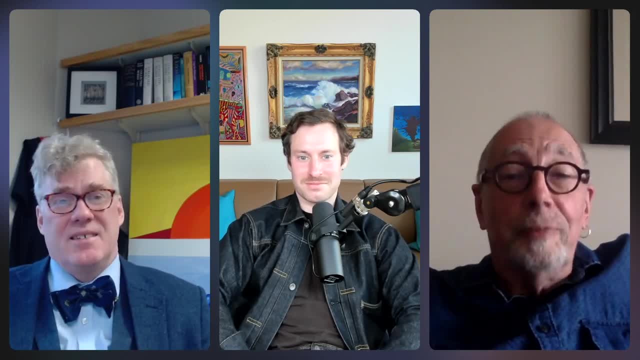 do that? Yeah, I do it, but it's. That was a god-lacking paper. when I read that, Oh good, I'm so glad you like it. What's the title? I think you're referring to my paper with 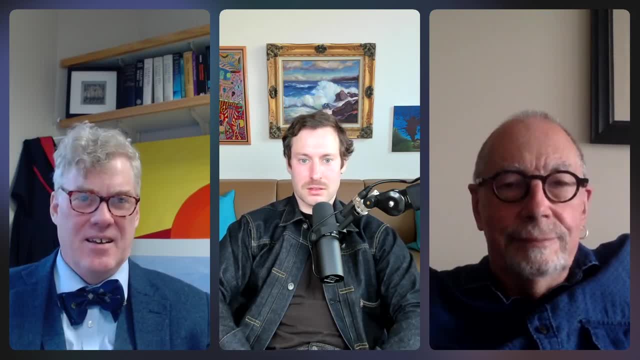 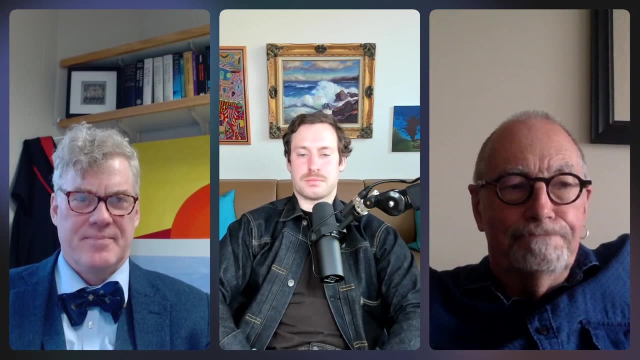 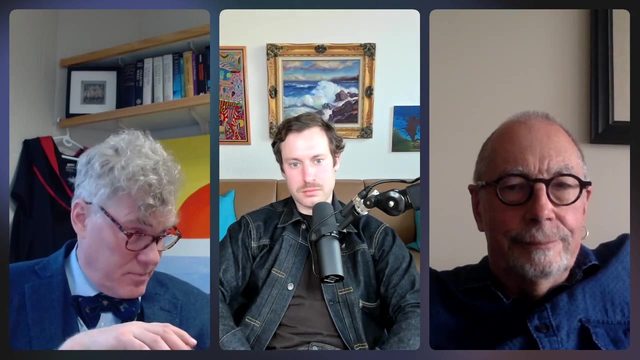 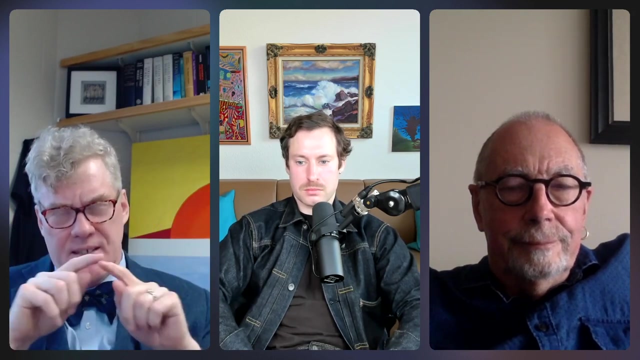 Ruji Yang. right, It's on the archive and it's called: Satisfaction is Not Absolute. Yeah, So the main theorem there is that we produce a model. Let's see: We produce a model, two models of set theory that have exactly the same arithmetic. 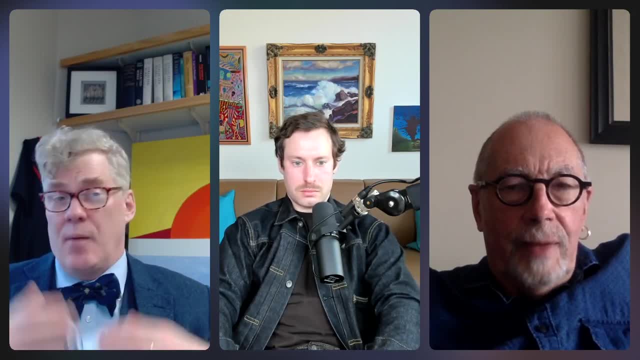 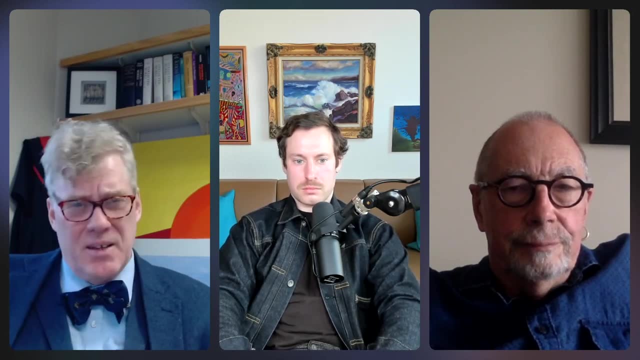 structure So they have the same natural numbers. I mean, in general, different models of set theory can have different omegas, different natural numbers. This is known because they can be non-standard or whatever, and this is completely understood. But sometimes two models of 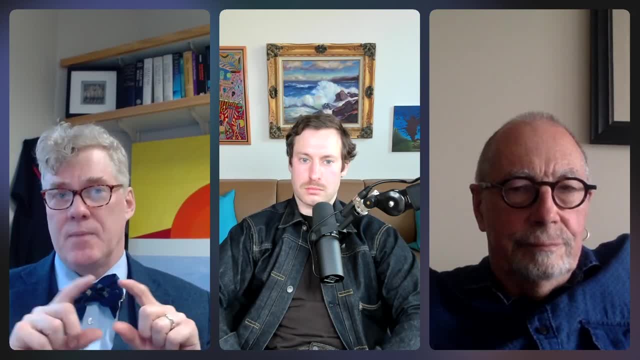 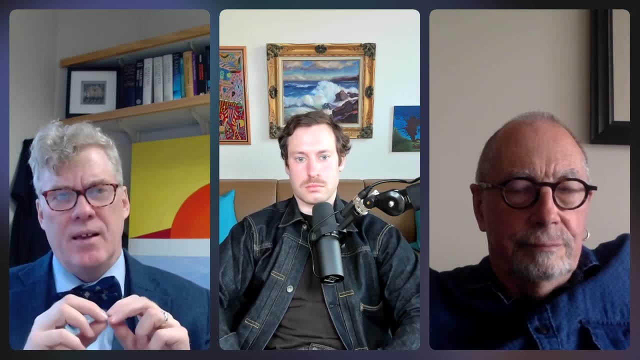 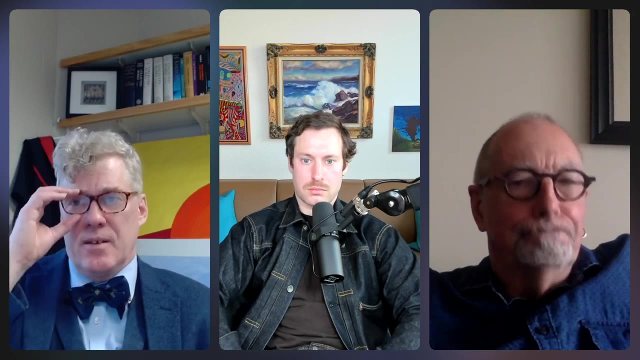 set theory might happen to have the same omega. I mean isomorphic or maybe literally identical. So we produce two models of set theory that have the same omega, but they don't agree on which sentences are true in that structure. And so there's a sentence that 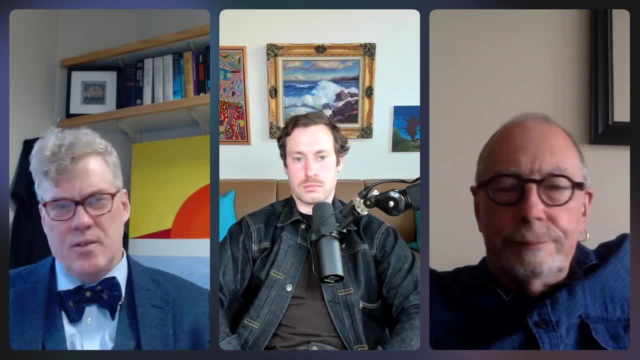 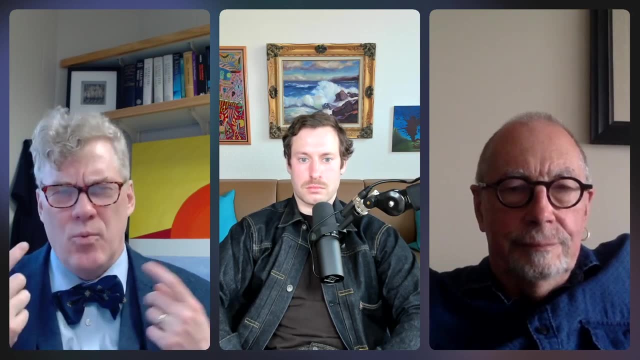 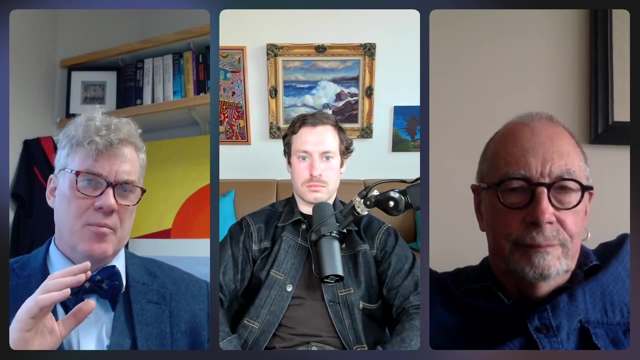 they both think it's a sentence, and one of the models thinks that this sentence sigma is true in the arithmetic structure and the other one thinks that it's not true. so what? the way i interpret this and what we were trying to do with this example was to, was to criticize the move that, if you're definite about the structure, 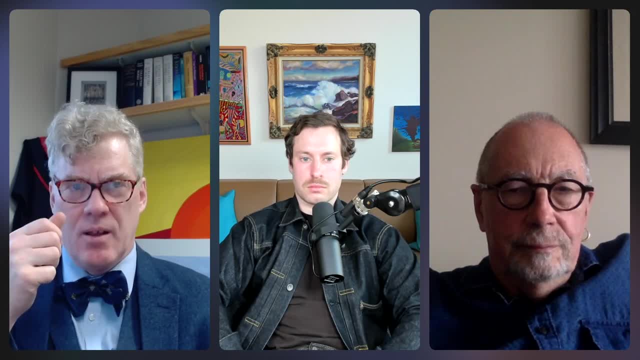 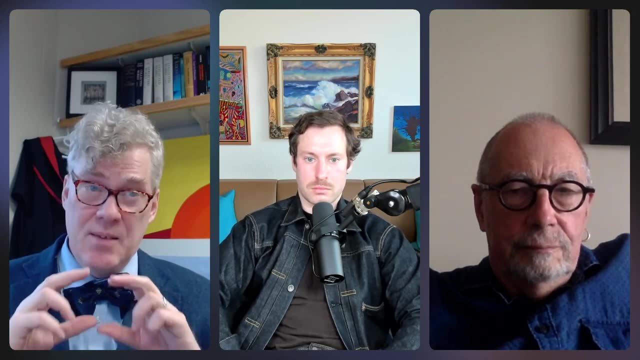 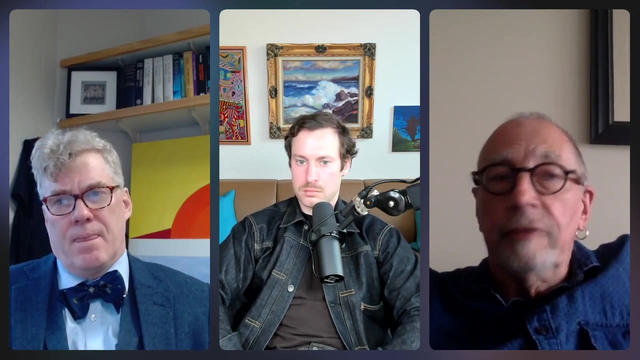 that you should also be definite about truth in the structure, because this situation is exactly a situation where the two models have the same structure, but they, the truth, is somehow indefinite. yeah, and the reason, if i understand it right, joel, is this: how you characterize the domain is a. 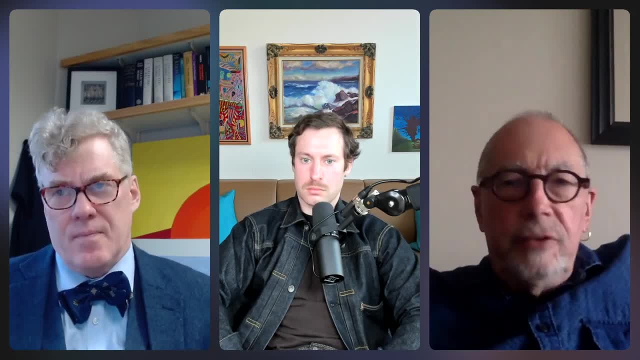 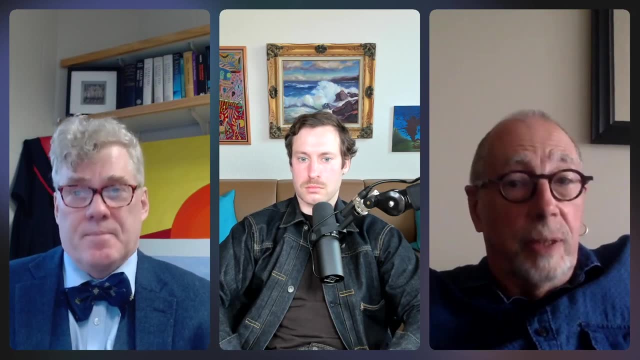 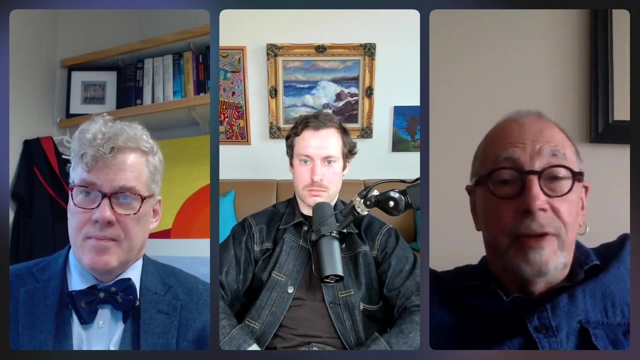 second-order matter. but even setting that aside, how you define satisfaction in that domain is a second-order matter, and so once the pattern is right around all over the place, then the determinacy of satisfaction is going to disappear as well. um, but that had never occurred to me. so i read your paper. um, oh good, i'm glad so i have a student. 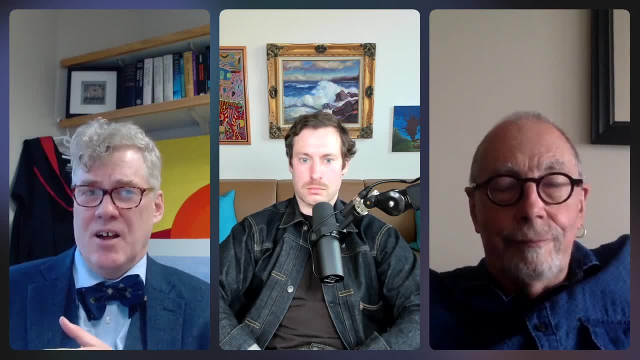 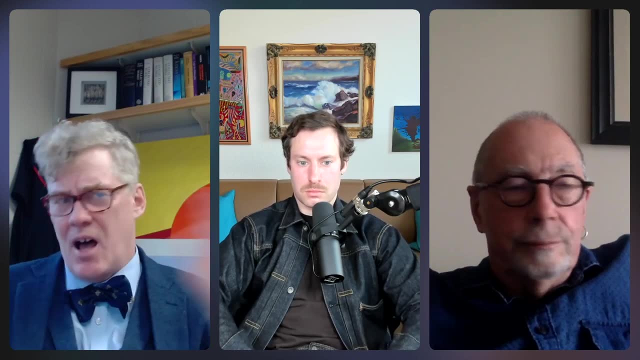 now in oxford, who's working on paraconsistent logics and some of your ideas, but using this theorem, namely because the theorem is this situation: there's not just two models, there's actually lots of models and it's following from krajewski's work, his old work of krajewski. 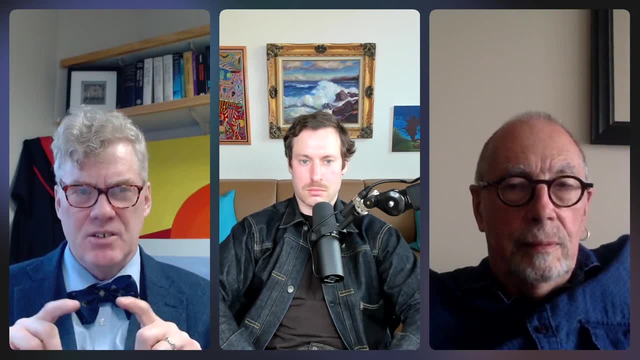 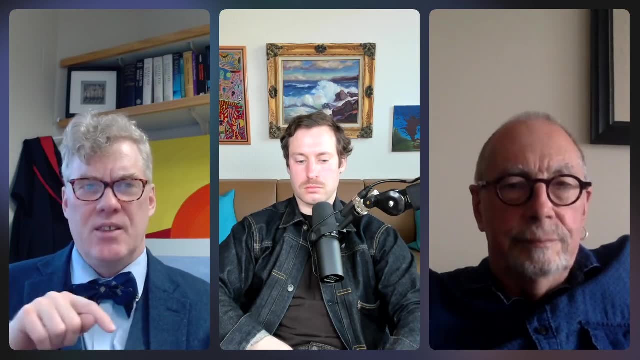 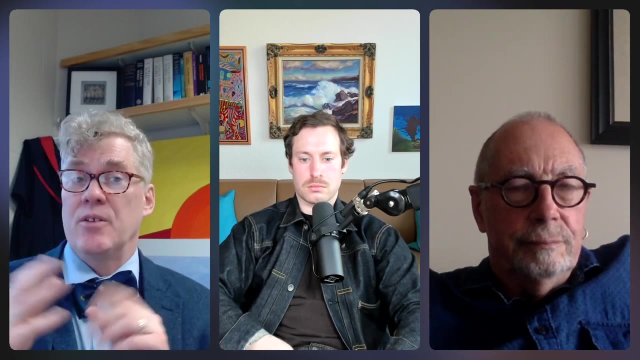 but the situation is that you can have a structure that has many, many different truth predicates for the same structure. so so we can have a model of set theory and we can put a truth predicate on there, different ones, many different ones. they disagree with one another, and so it's about. it's about the situation where you have sort of multiple 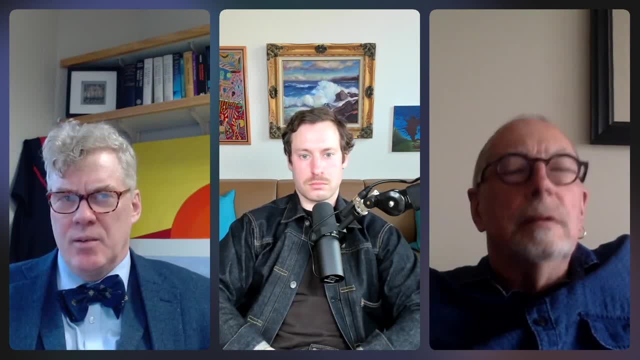 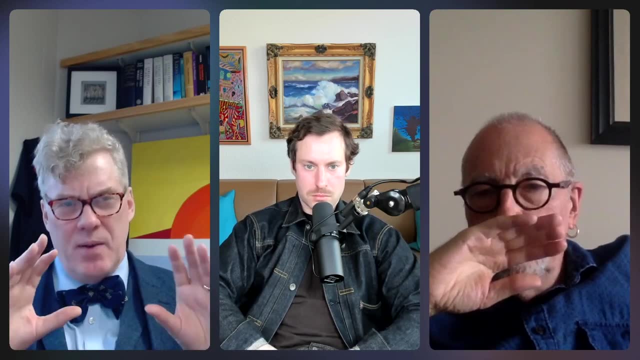 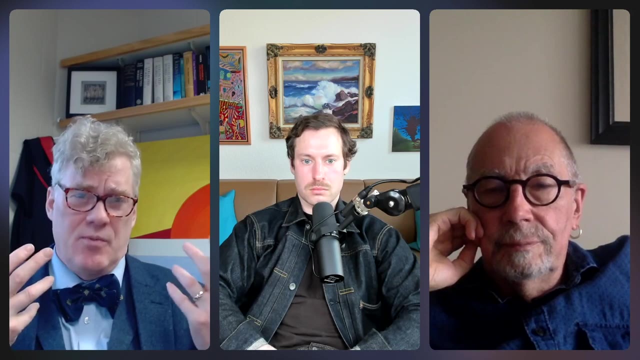 concepts of truth for the same realm of objects, and go on. sorry, yeah, so there's a little. there's a. the parakonsistent angle on it is that, well, look, we could, we could. from this situation, we can have a concept of truth which just means 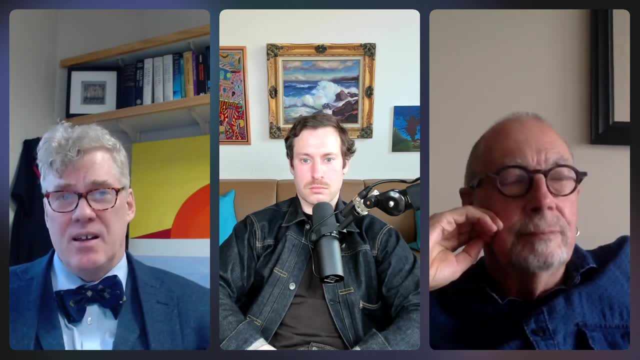 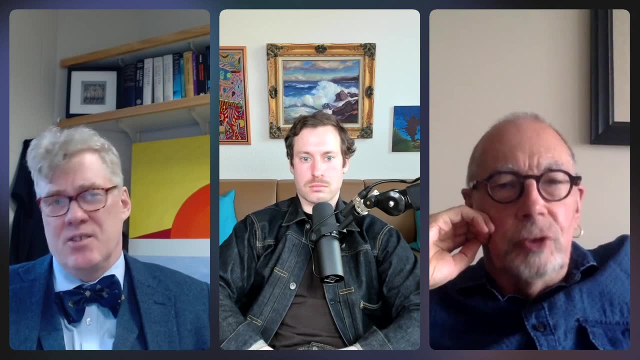 it's true for at least one of them. oh, that's a paraconsistent concept of truth, because, because they disagree, there are some statements that are true for one of them and the negation is also true for one of them, So this is actually subvaluationism. Look, I didn't know about that. that's interesting, but just. 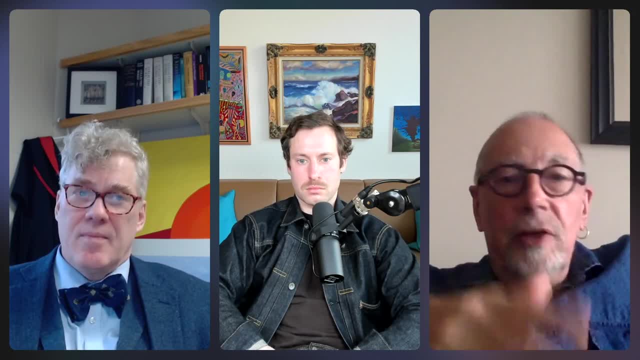 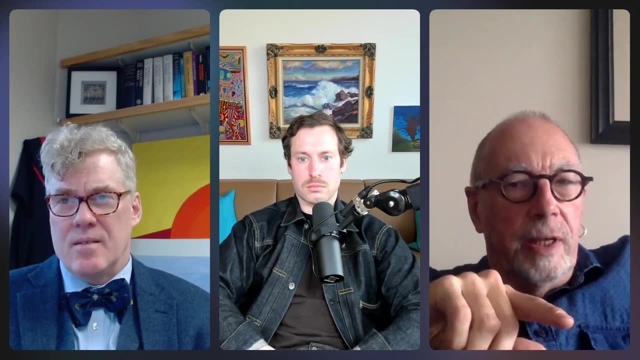 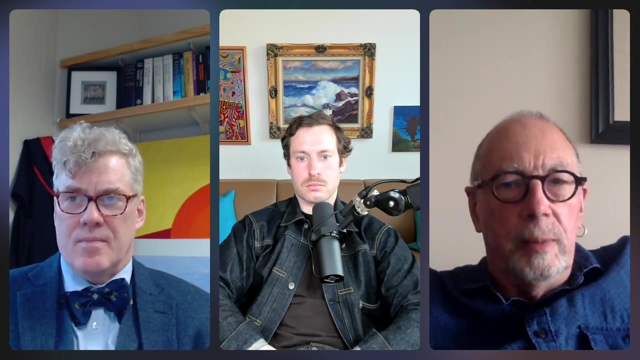 coming back to what my initial problem was, I don't think that moving from de re to de dicto is going to help, just because the de dicto stuff is going to be subject to the same kind of indeterminacy all the way up. 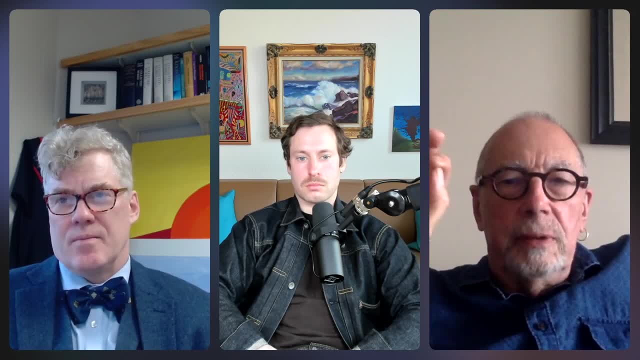 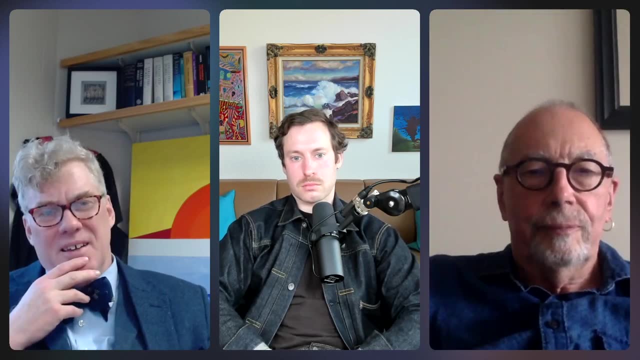 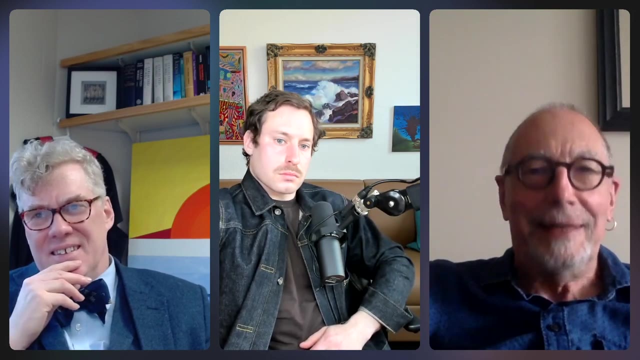 And this objection worries me More than where the hell are you coming from when you investigate the four evils? I mean it doesn't worry me because that's just how it is. that's how I look at it. I mean, the problem is exactly that's how it is, just because that's how it is seems to. 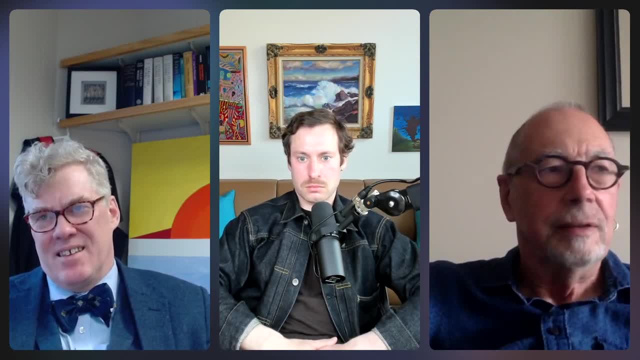 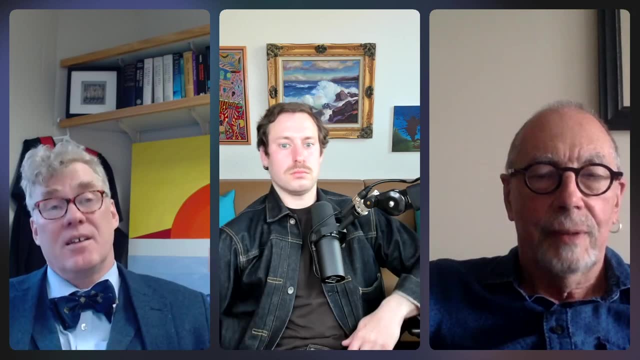 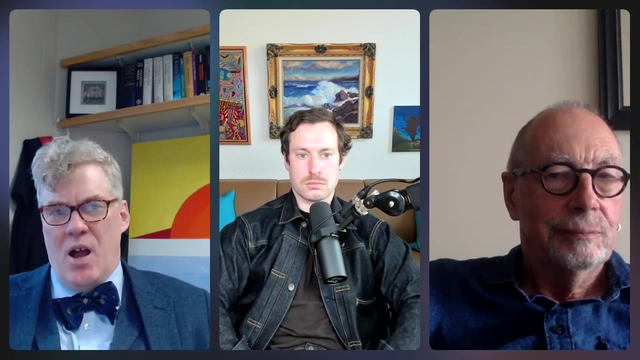 render the deterministic any answer to any question. no, no, because not, it's not like anything goes, because we can still prove that like regardless. you know certain things are going to be the case and you know that there is going to be some kind of common ground because you know, we, we have. 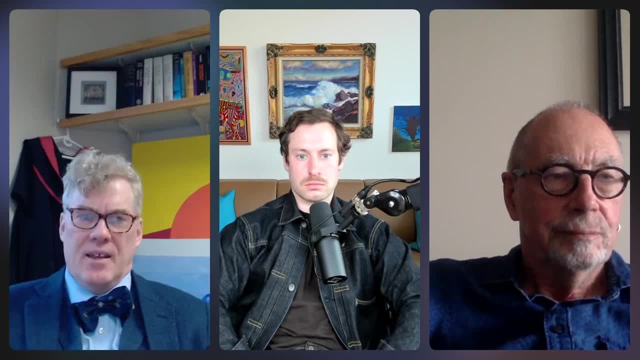 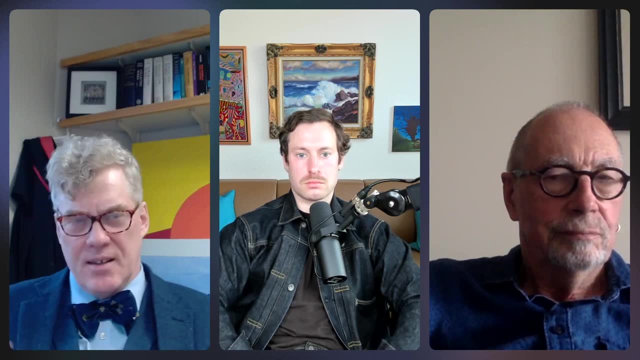 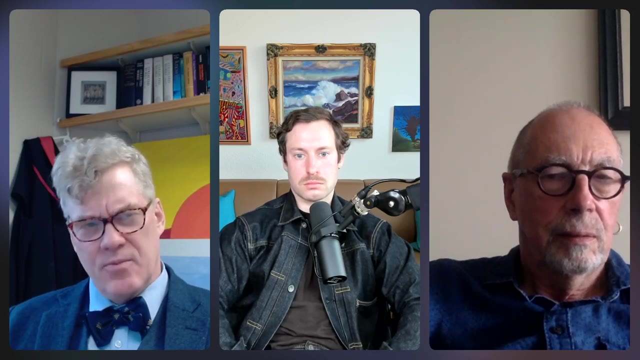 we can prove theorems from a theory, and if you know, if this sort of pluralist conception has it, has the property that they're agreeing on on these axioms, then they're going to agree on the conclusions too, because of the proof. and so it's not like: look, you can make any statement. 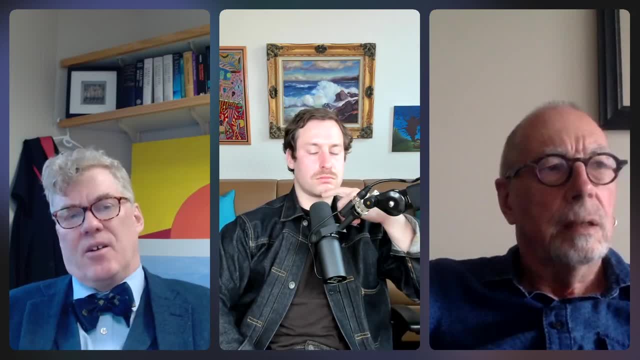 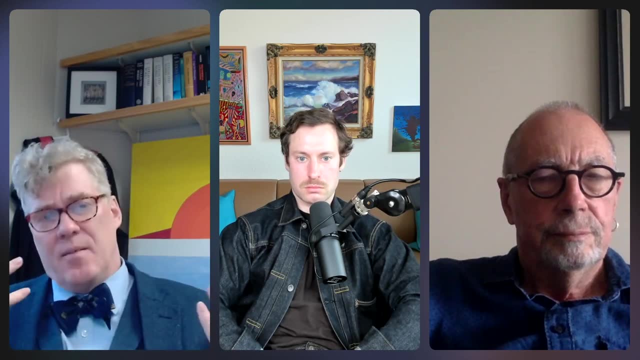 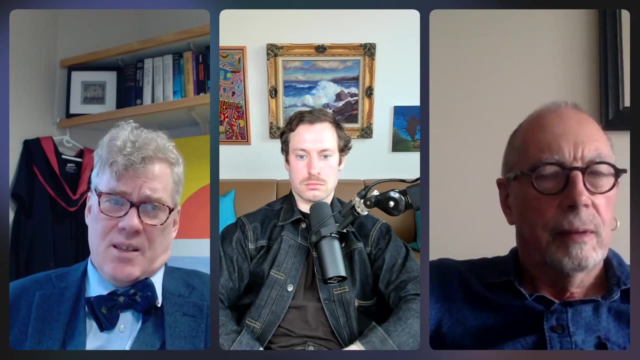 true or false if you just go somewhere else, there are, you know, there's limits, but meanwhile, these weird situations that you're describing, which are, i find, extremely fascinating, that's what when i say that's how it is, that's what i mean is that, yeah, so we have to have a larger concept of 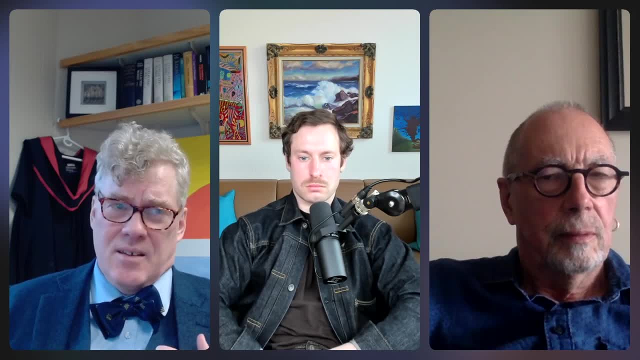 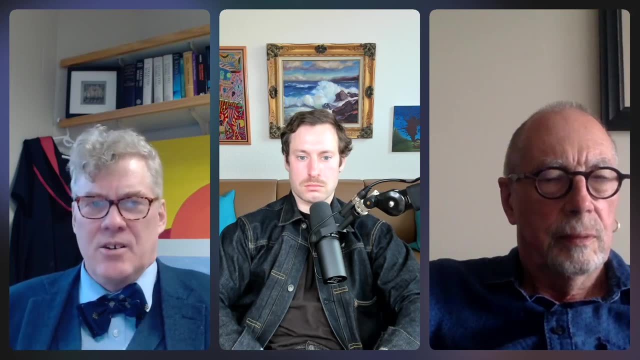 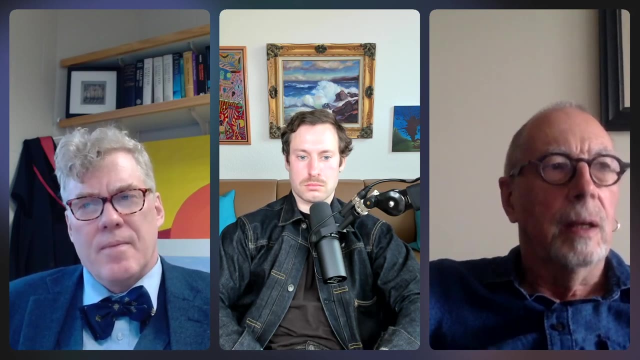 metamathematics and this and the, the object theory, metatheory distinction is just too crude. it has to be encompassing of this enormous hierarchy that you're describing. i wasn't suggesting that anything goes. um, the worry is not quite that. the worry is that, um, if all truth is relative to a. 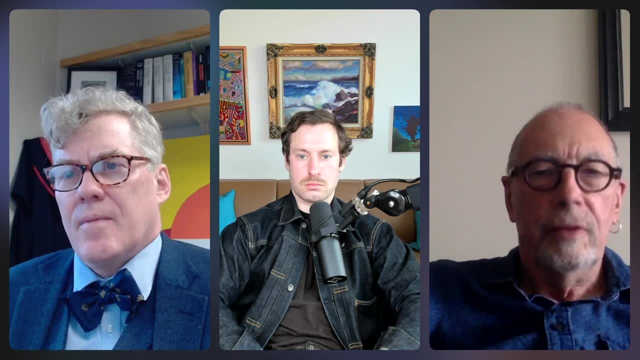 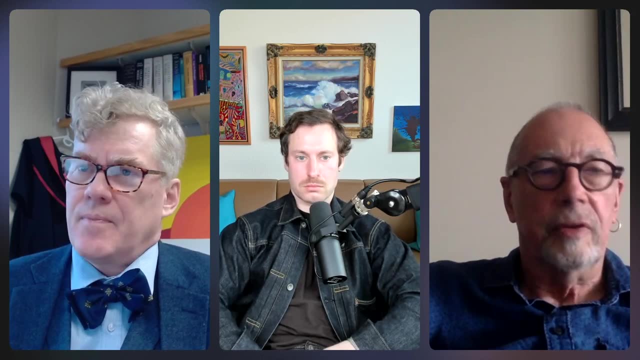 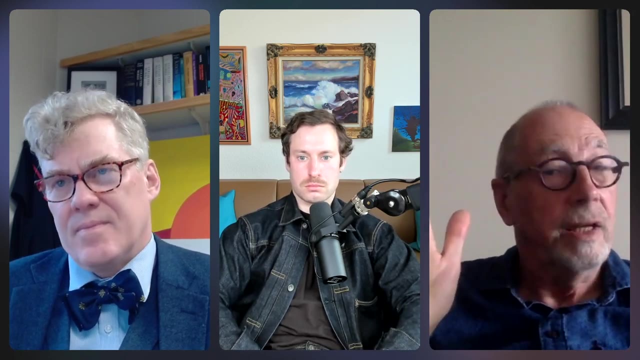 structure, then that something is true in a structure is also relative to the structure. sure, yeah, so there's no determined answer to the question of whether something is true in a structure, in a structure and a structure, and so the kind of determinacy of any answer. the question is just as it is now. maybe you can construct some kind. 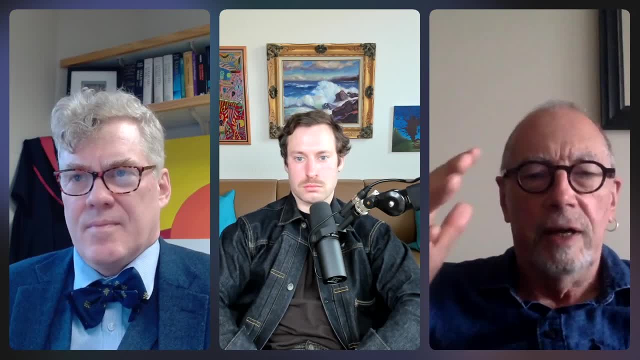 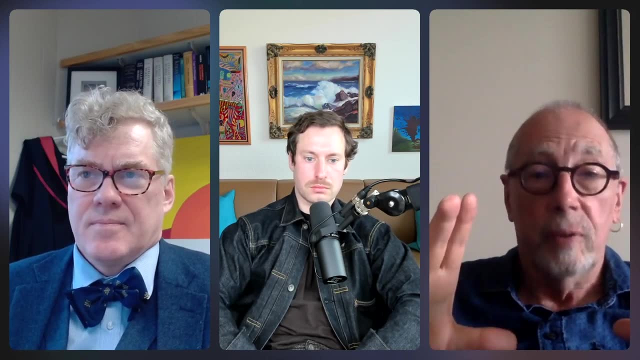 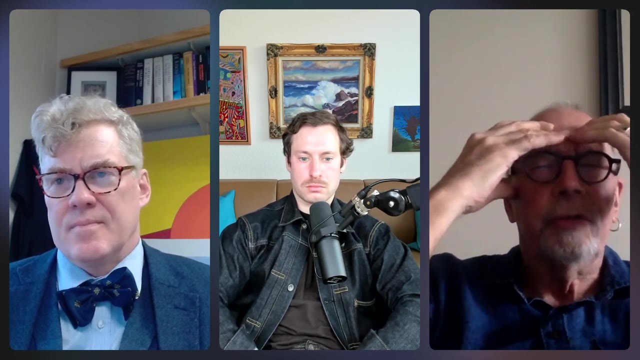 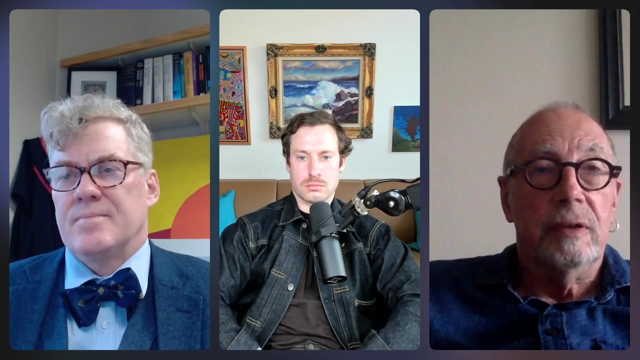 of absoluteness in the way you suggest and say, well, yeah, but there's a kind of a nucleus of stuff which is absolute. um, that, that will be a good answer to the question, if you can get it right. um, uh, then. but i mean, we need to understand what constitutes this notion of absoluteness. um, okay, maybe there's a good answer. 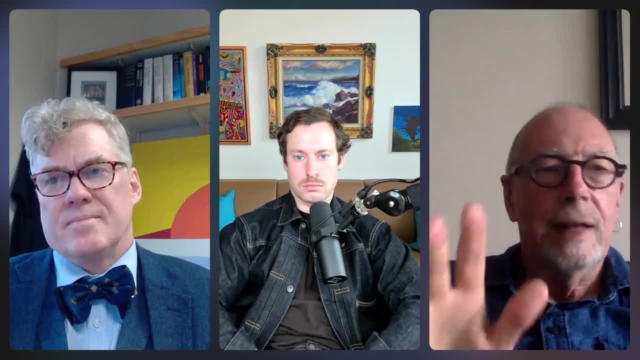 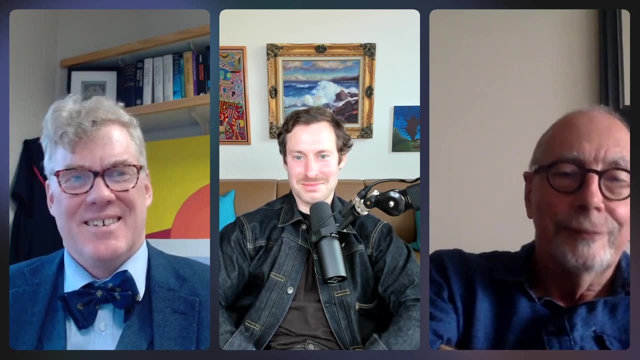 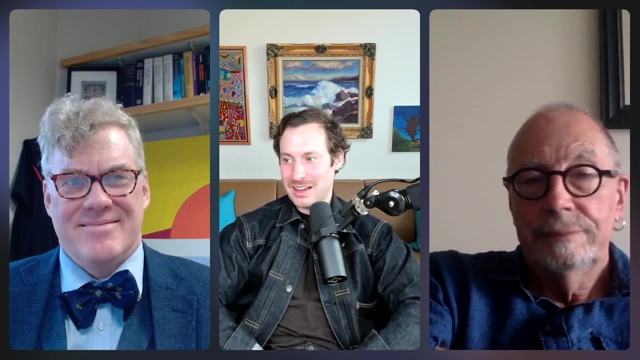 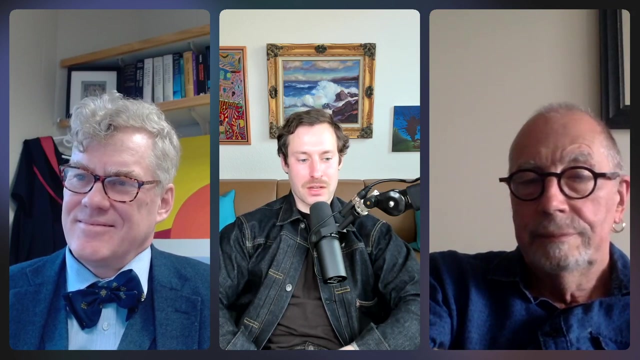 uh, now it's going to get technical. maybe we'll we'll talk about this by email, um, okay, yeah, okay, well, well, uh, since we're, i guess, for the moment, steering away for a technical material, maybe it's a good time to take a step back just a little bit. and so, joel, you explained the mathematical motivations behind. 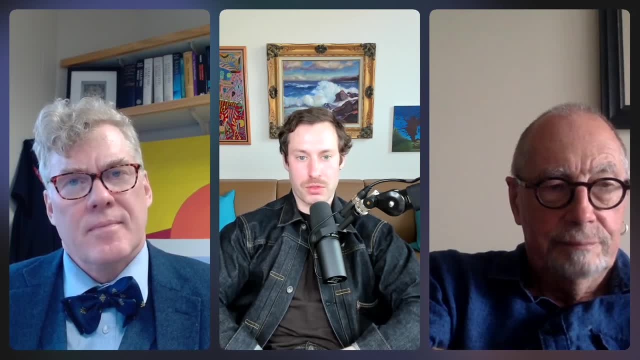 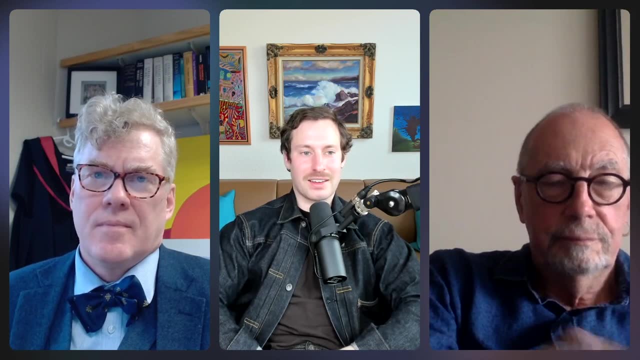 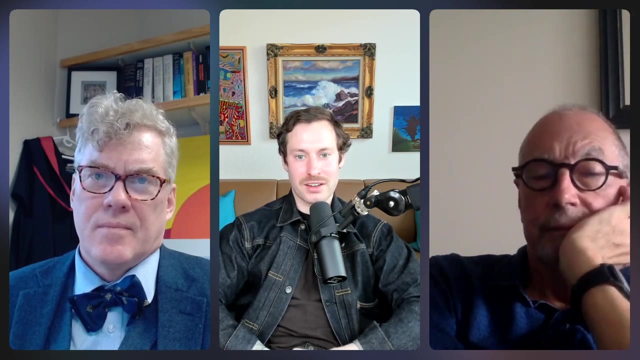 how you came up with the, the multiverse view, but i'm also curious about whether ideas in sort of the, the philosophical zeitgeist, uh- contributed to your idea, and graham in particular. i wonder how you feel about this and how it relates to your idea of the multiverse. 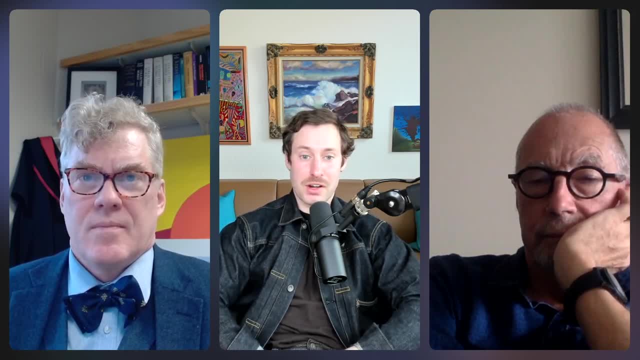 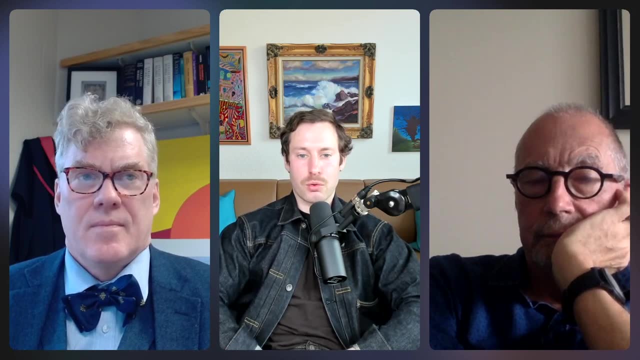 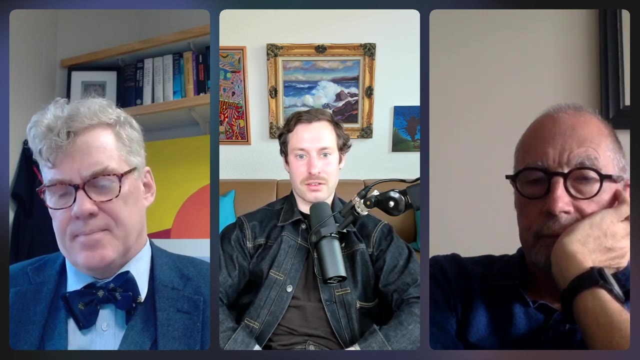 to your thinking about the multiverse, because what i have in mind- i mean particularly when you use phrases like exploring the space of set theoretic possibility- is whether you were at all influenced by something like lewisian possible worlds. i mean this idea that there is this multiplicity of 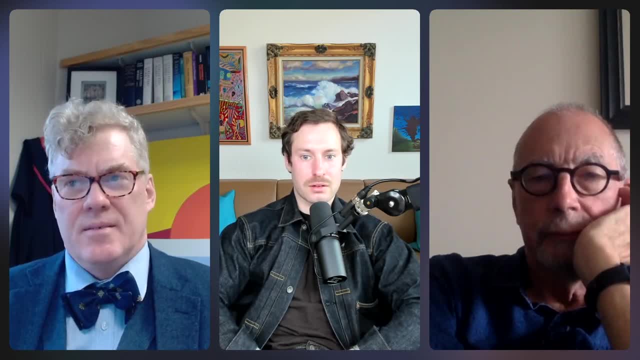 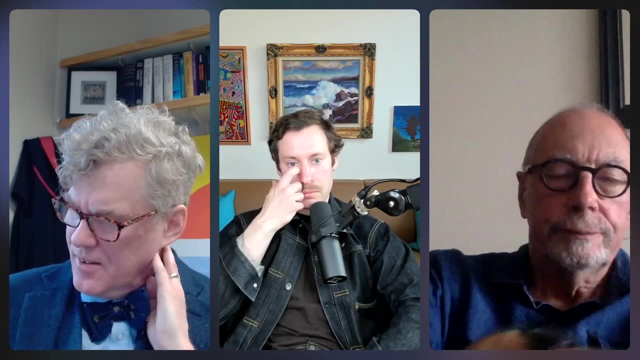 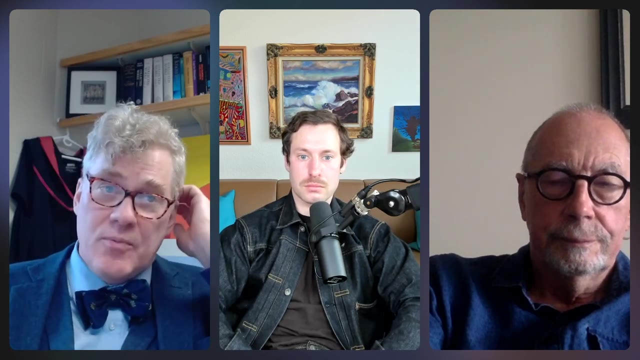 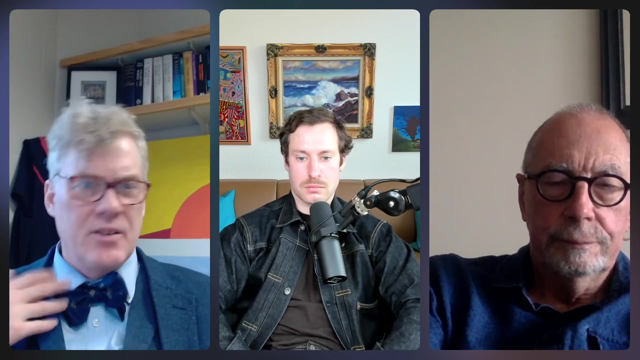 spaces out there, right? not at all. not at all for you, graham, not sure, i mean, i wasn't really either, because when, uh, you know the origin of these uh views was, uh, i mean i, i learned after, after working on the concepts and producing the paper and so on, about you know, people like uh balaguer has quite a lot. 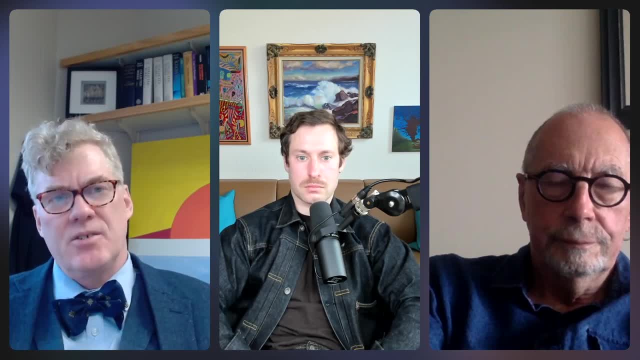 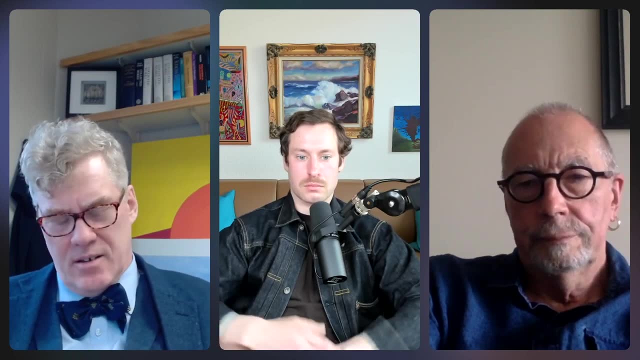 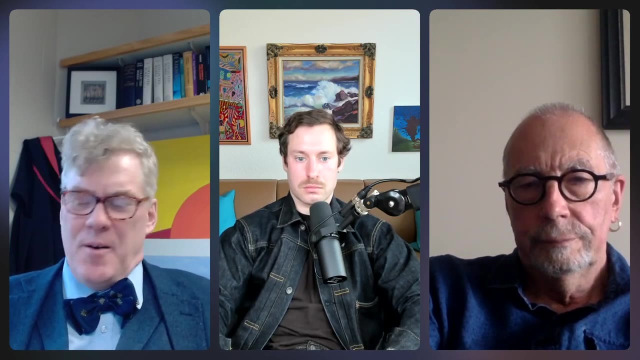 of work on this plenitudinous platonist idea which has a very strong affinity for my kind of pluralism in the set theoretic universe and and of course the the um, lewis's, uh, um, huge spectrum of worlds and so on and um, it wasn't really the origin of of my views, but of course there are. 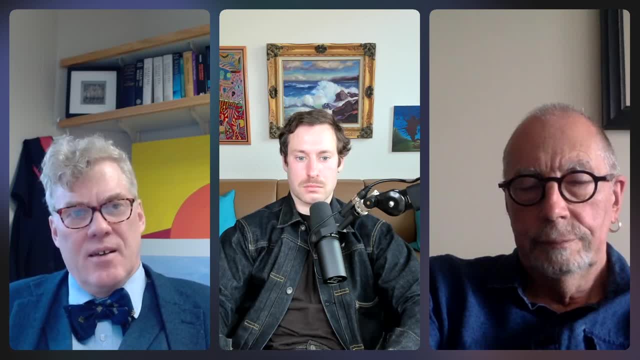 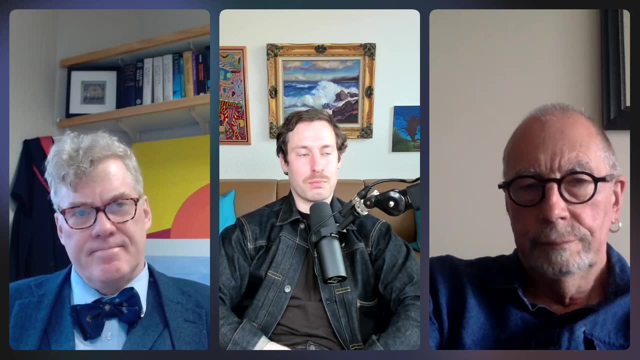 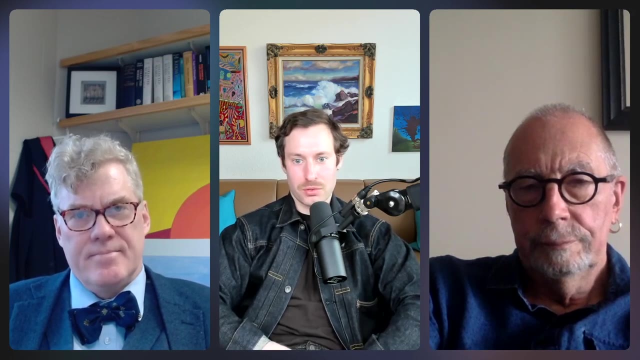 very strong connections there that i subsequently came to realize. and then you mentioned another thing you mentioned earlier is that everyone agrees on the mathematics. like you, colner, graham wooden, you all agree on the mathematics, but then parenthetically- parenthetically, i mean, it's quite. 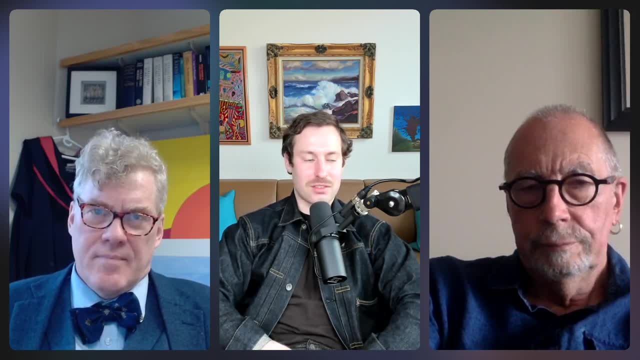 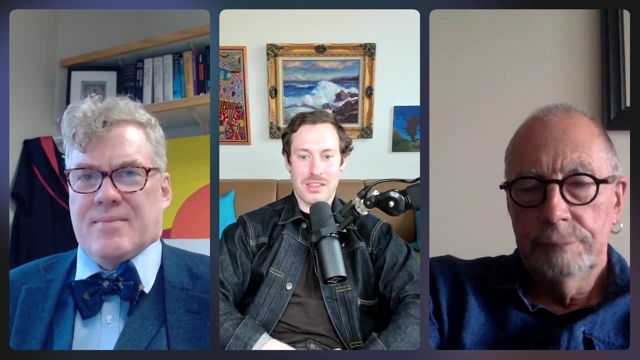 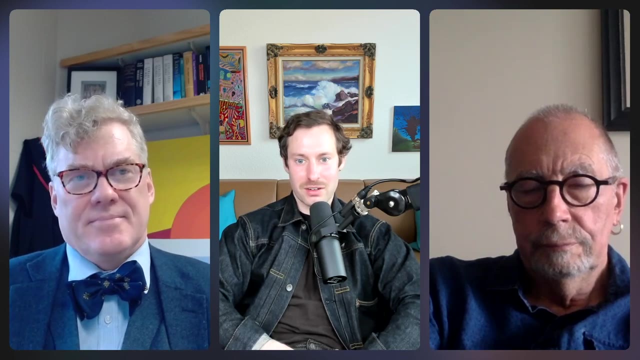 fascinating that mathematics, which i mean we think of as the objective, natural science par excellence, can have problems that may be thought of as solved or not solved, uh, depending on philosophical considerations. so i mean, the continuum problem was hilbert's first problem, right and a hundred and 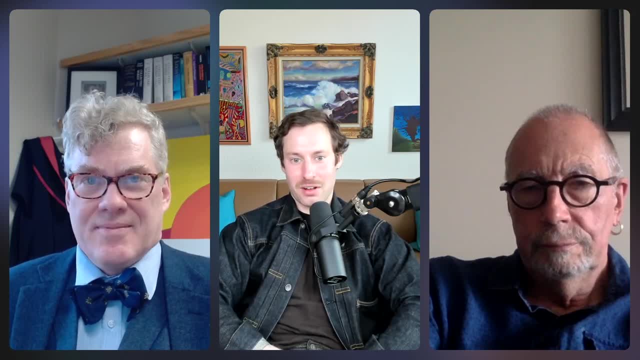 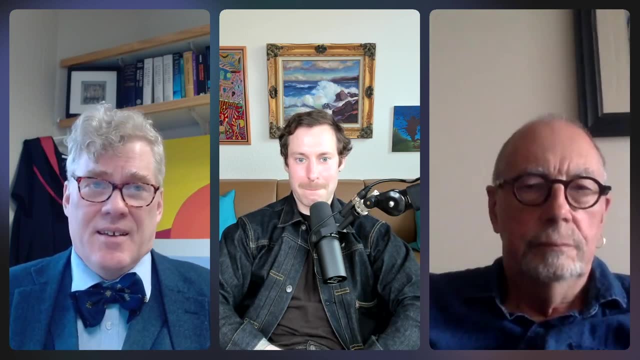 some years later there's dispute over whether or not it's been solved exactly. i mean sort of answering that question, but i guess i think the point is that we should become a more distant meaning of both. you know- and of course i think that's part of the monist view- that that ch is an 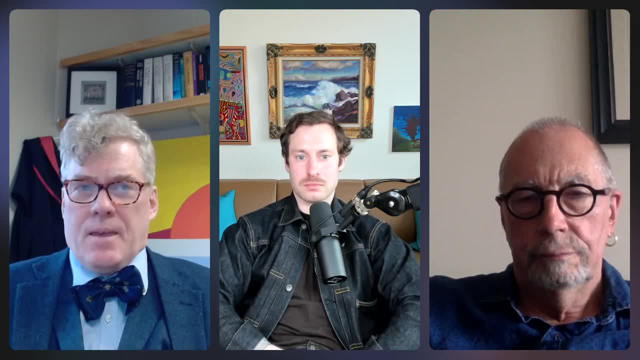 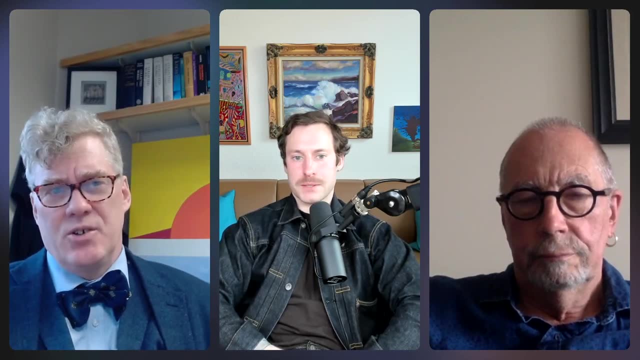 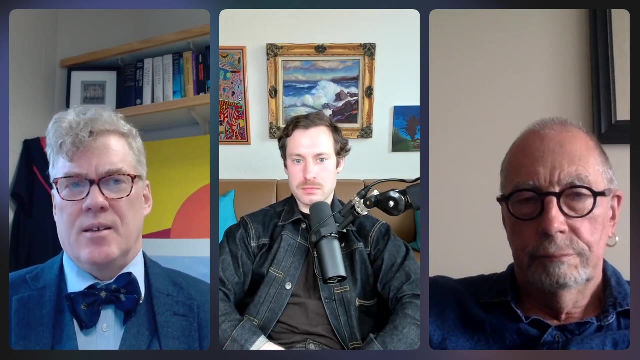 open question, um, but i've argued explicitly that we should think of it as as a settled question, because we understand very deeply what's going on with it. we we know, of course. we know it's independent and we know that, given any set theoretic universe, you can make a porcelain extension where you achieve either value, either true or false. there's two porcelain extensions realizing those possibilities. 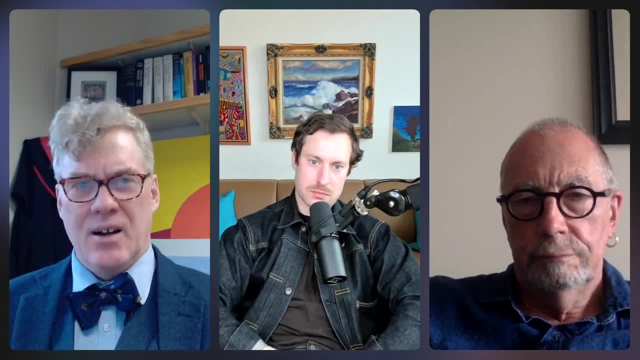 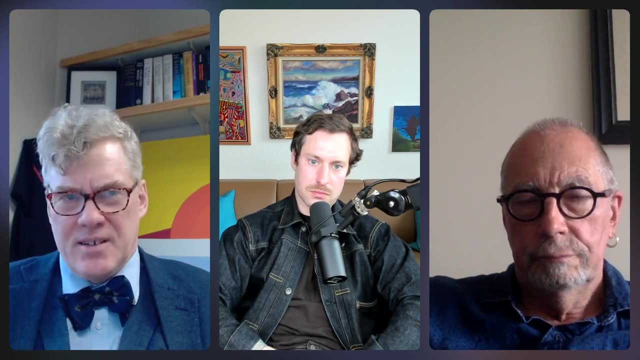 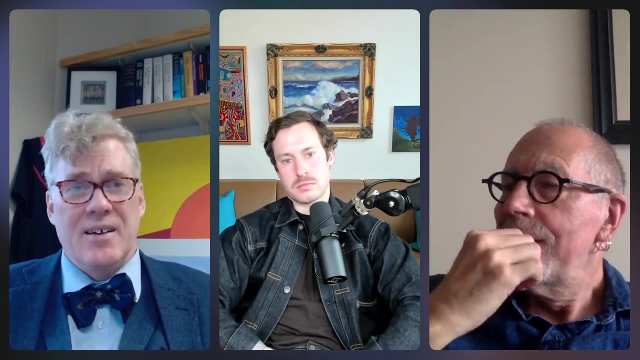 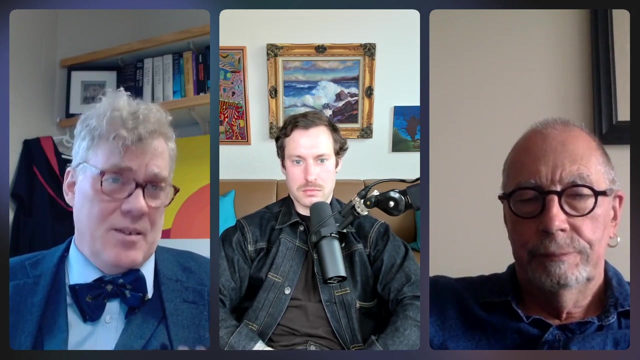 and and furthermore we understand very deeply how we can have not ch with various other kinds of statements about, say, cardinal characteristics, the bounding number and the dominating number and all those technical things that we can. we understand in a quite deep way what's going on with ch in the multiverse? and- and that's the answer to the ch question, to my way of thinking, 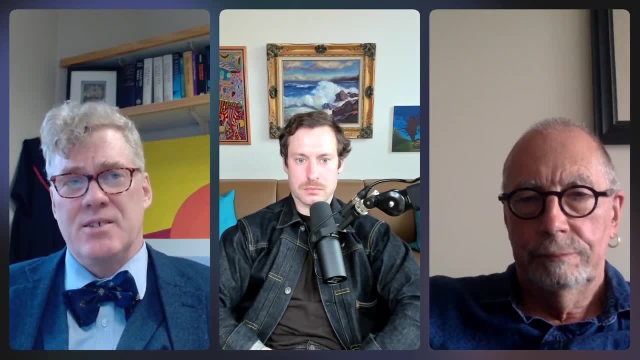 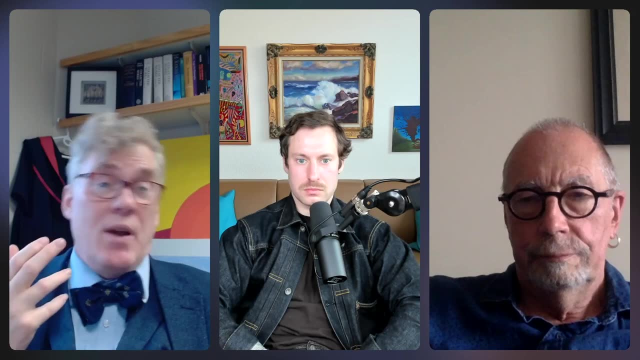 that is the answer, and we should think of it as a settled question. so you're right, there isn't agreement about this, because a lot of people talk about the continuum hypothesis as an open question that we're still trying to figure out the answer to, and- and that's the point, i guess, where we don't- 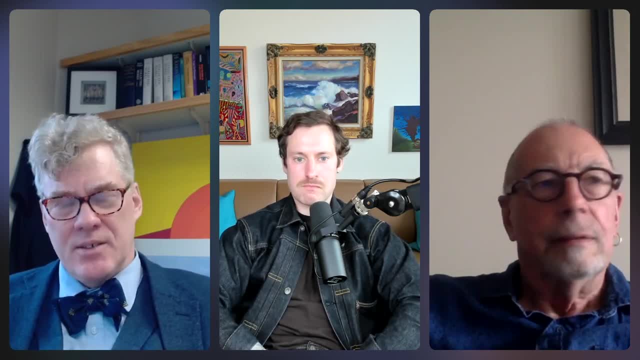 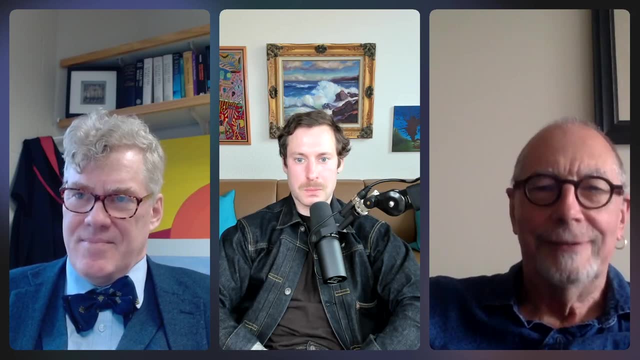 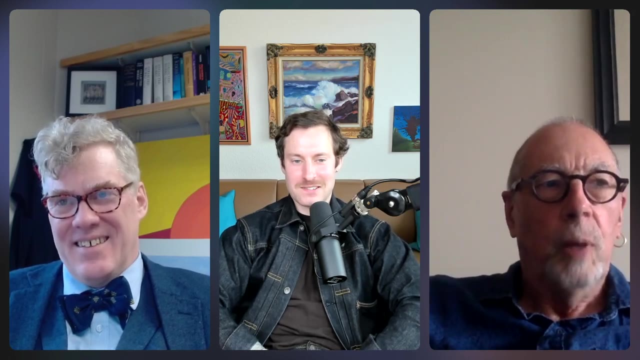 agree, because i think that's not a correct way of understanding what's going on. yeah, let me just say that whenever someone says we, my next question is always: who's the we? and i'm not going to say what you think. i'm going to say: okay, um, but when you say we, you talk about. 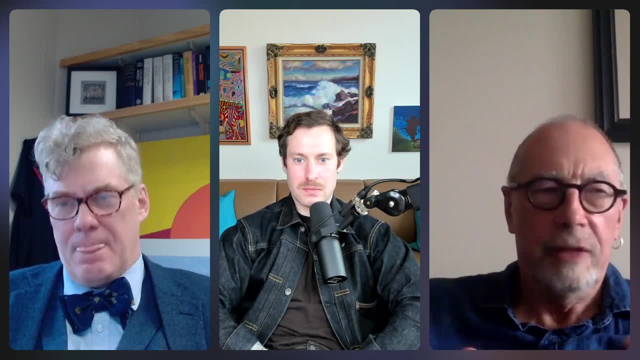 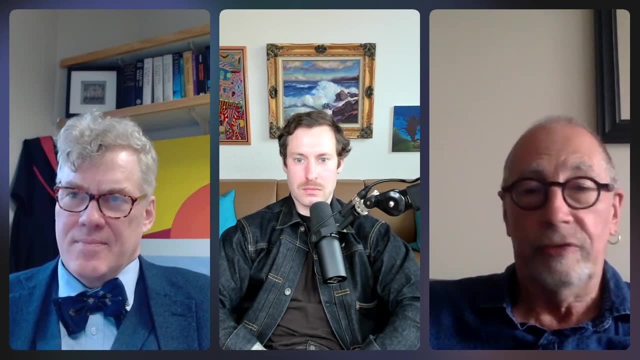 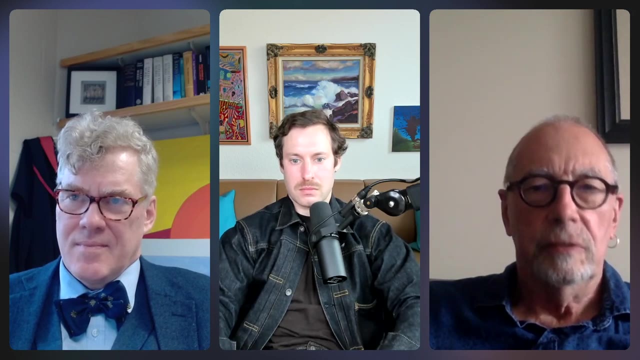 sort of generally speaking, contemporary magnitudes, and that's fine, um, but of course mathematics has been changing for two and a half thousand years, just in the west, let alone the rest of the world. um and uh, i've absolutely no doubt it's going to continue to change, and sometimes 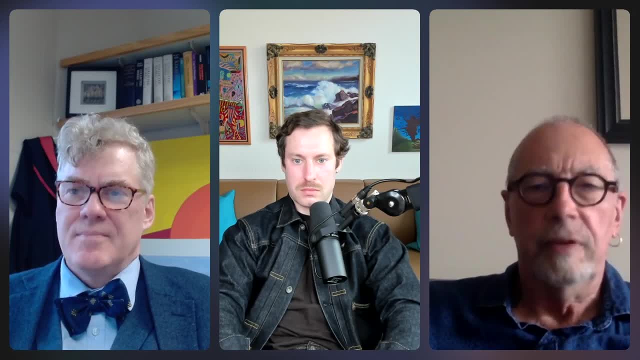 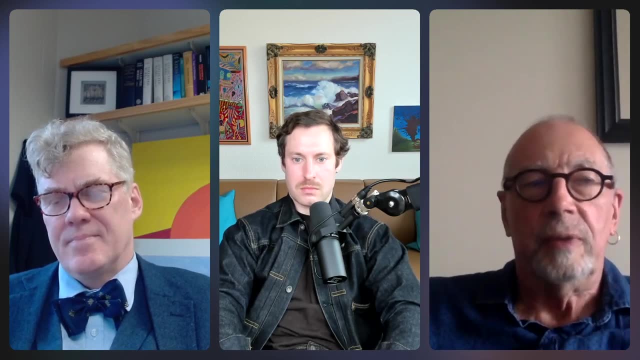 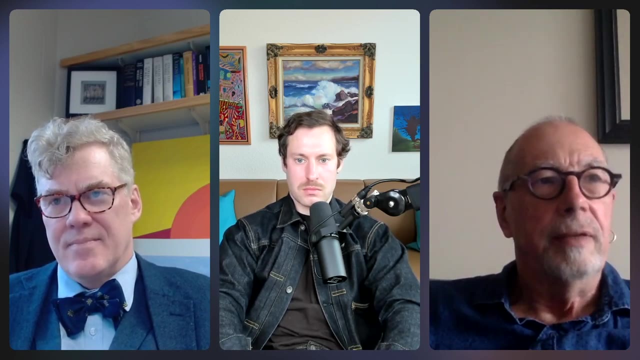 as mathematics changes, we overturn some exceptional things, and that that happens too, um, of course it's hard to predict what's going to happen, because it's. it's impossible, in fact. but i would be gobsmacked if mathematics in the year 3000 were anything like the mathematics 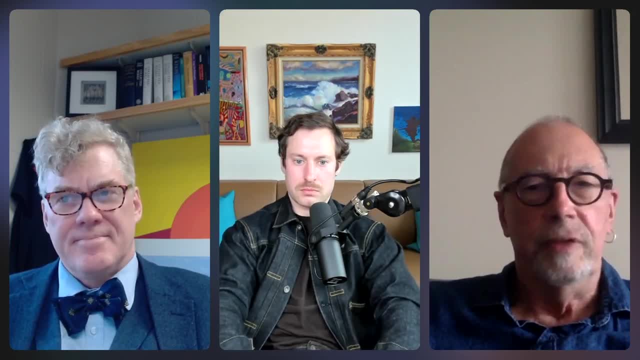 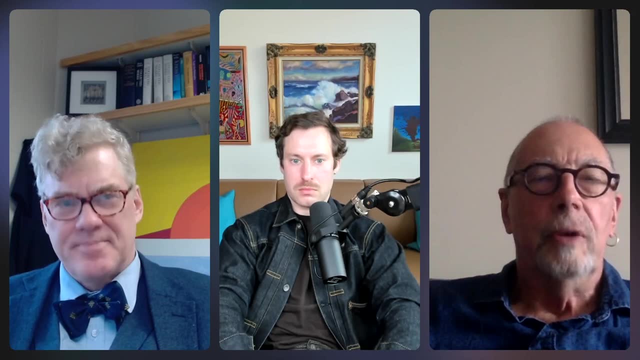 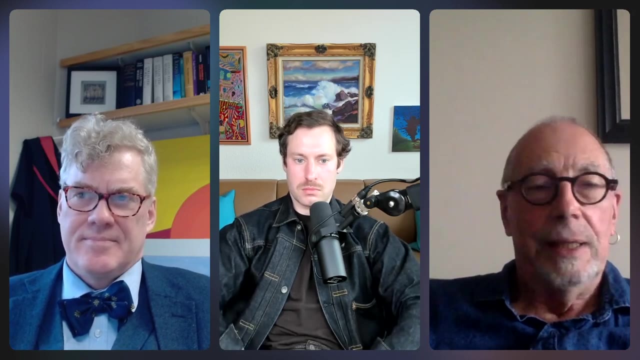 in the year 2000, any more than mathematics in the year 2000 is like mathematics in the year 1000. i can agree with all that, yeah. so um i, i think all these views about what we know, what we don't know, even in even in mathematics, are going to have to be subject to revise. oh well, 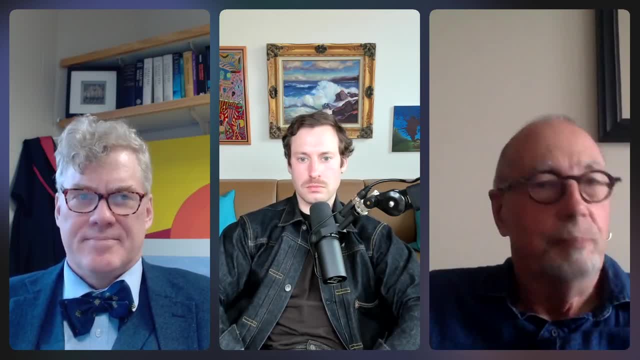 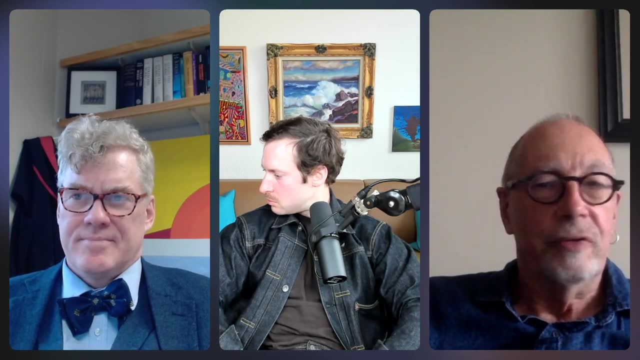 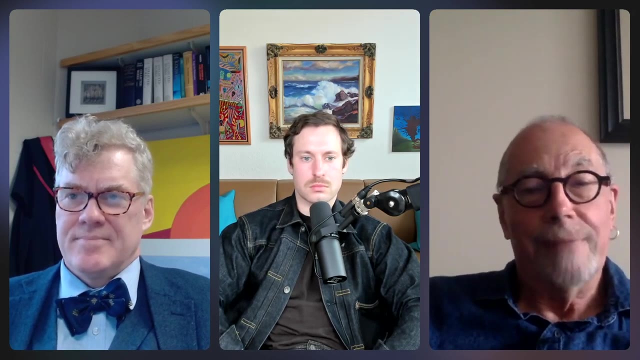 that's how it seems to us at the moment and maybe it will remain, maybe it won't, but i i do think that that that is worth bearing in mind. the we in the community of mathematicians in 3000 may have a very different view from the we of the mathematicians in 2000. i think that seems almost perfectly right. 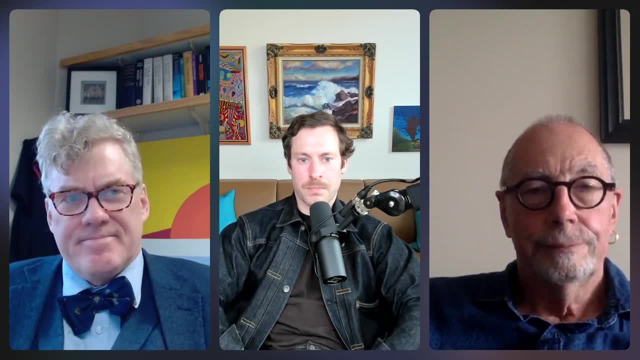 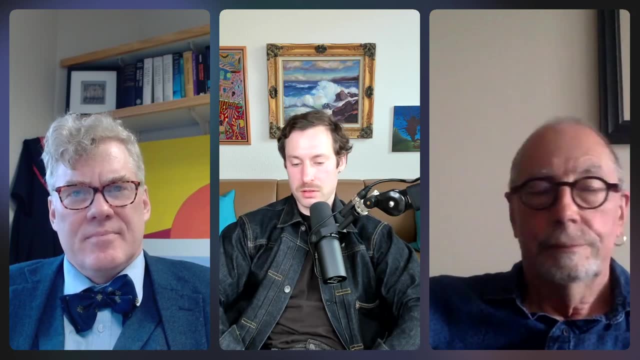 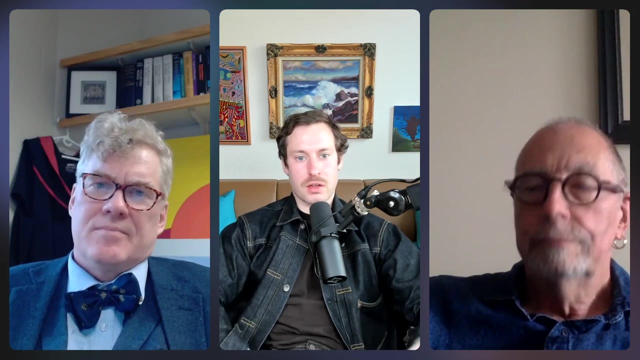 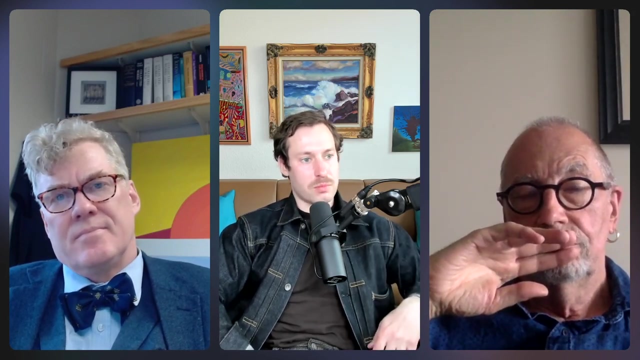 i think that's that's got to be right. so, in light of your view, though, of the continuum hypothesis or the continuum problem being settled, how do you view sort of woodens and colner's program, which i view as something like a continuation of girdle's program, search for new axioms? so if the continuum 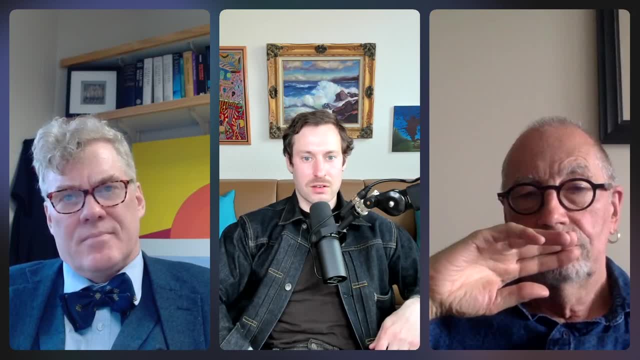 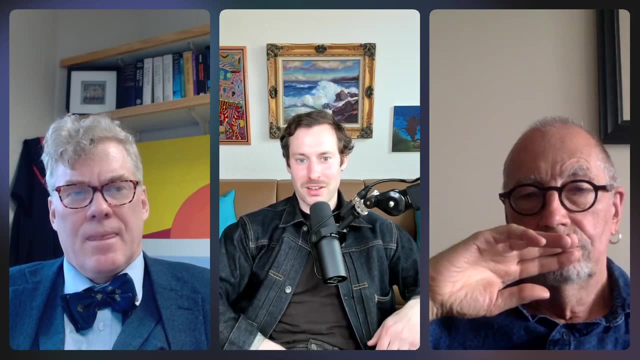 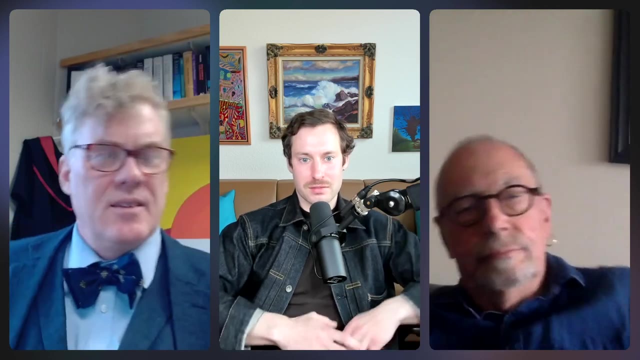 hypothesis is um settled, is it just? you just view them as exploring deeper into one realm of the, the multiverse, and exploring the continuum hypothesis behavior there. yeah, i guess. so i mean of course the, the, even the philosophical views aren't incompatible. right for it. from the 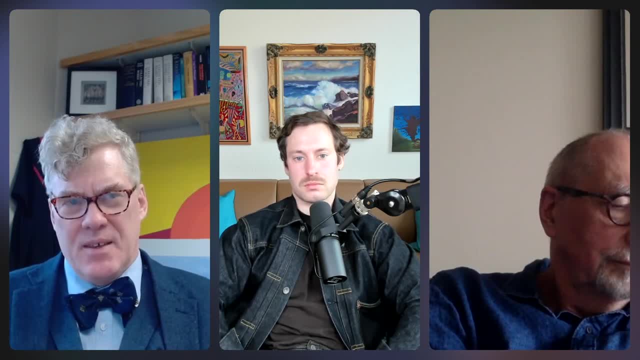 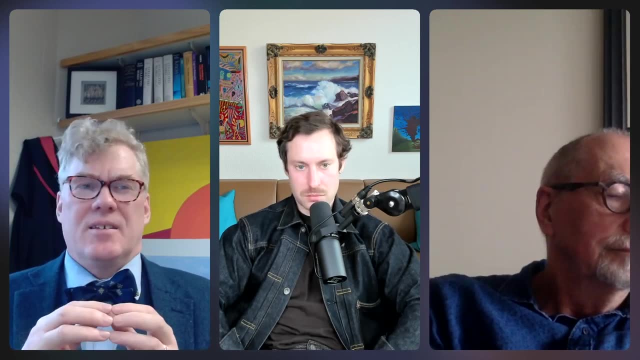 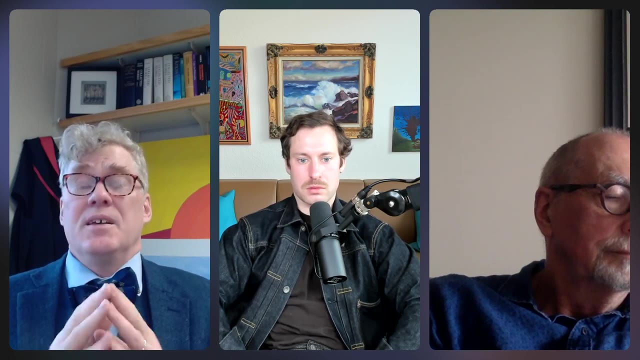 pluralist point of view. the monist project is trying to find the, what, which one is v, right, and and and to, to articulate the criteria by which we would recognize it or judge it and so on, to be the right answer and because it's of course. it's not a math, it's not a mathematical. 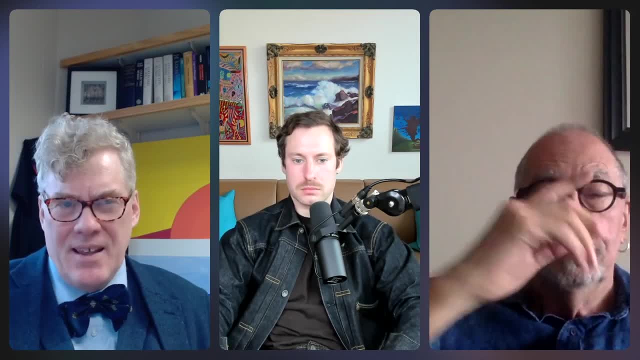 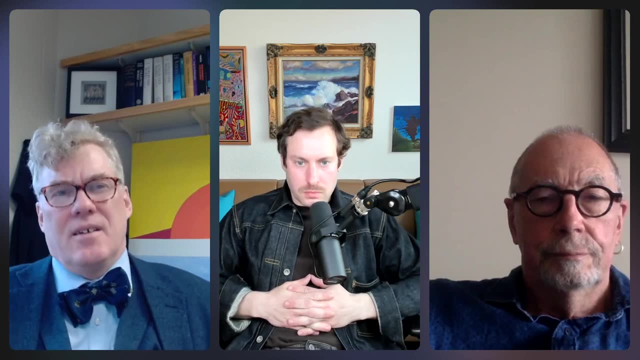 problem right to find out which way it goes. we know it's independent, we can't settle it. and even with large cardinals we know we can't settle it because of the levy solvay theorem, and so so the the continuum problem is is is much harder to find a reason for why we would settle. 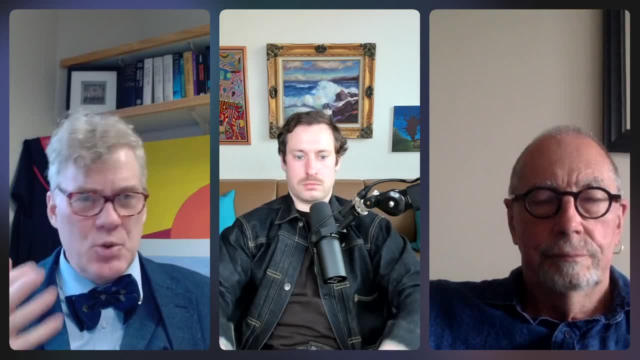 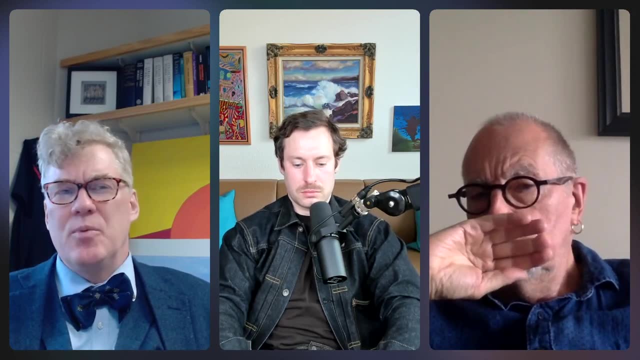 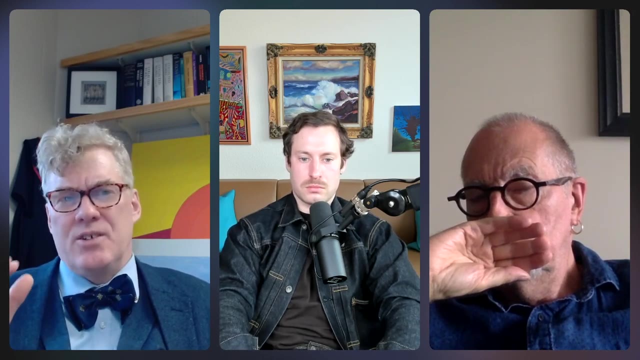 it one way. i mean the, the kind of dream solution. what i've called the dream solution would be that we would find a principle that everyone agreed expressed something fundamental about the concept of set and which also happened to settle this ch question right. so the missing axiom in a 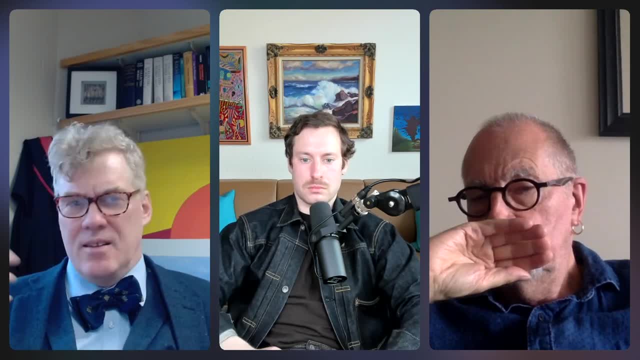 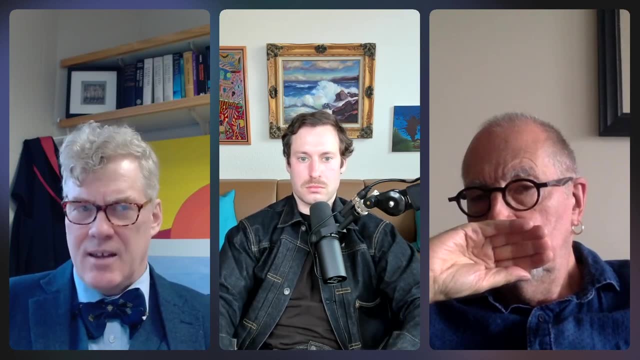 sense. this is the dream solution. this is what. this is what girdle wanted with large cardinals, but he wasn't able to have it because of the levy solvay theorem. large cardinals can't settle ch either way. um and, but maybe there's some other missing principle. it's something like what happened. 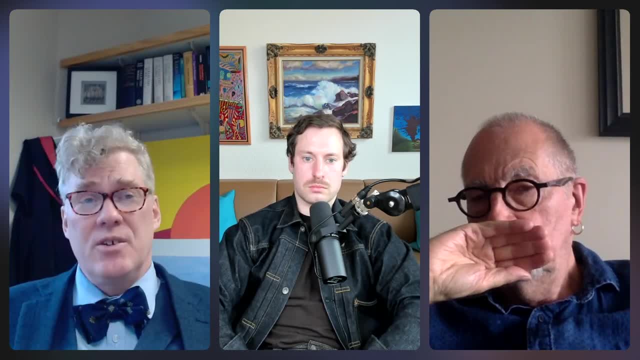 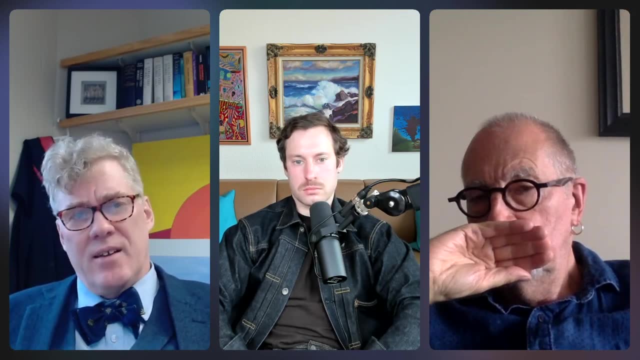 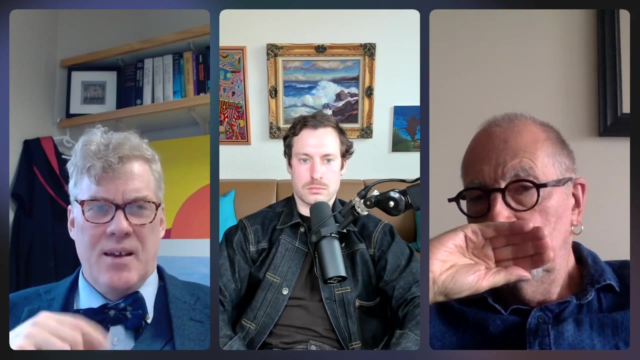 for example, with replacement. when zermelo first introduced his axioms of set theory, he didn't have the replacement axiom. it wasn't on the list, but as soon as frankel mentioned it. basically look, if you have for each number n, you can define a set, a sub n, and you want to form this: 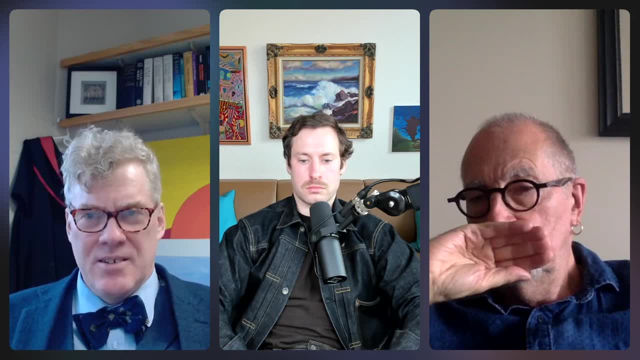 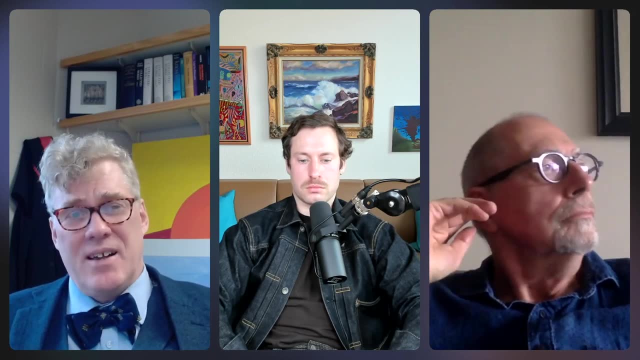 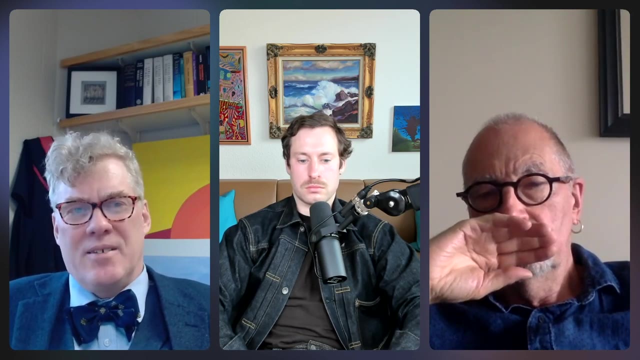 set of all you know, the set that has a 0, a 1, a, 2 and so on, that countable set, and without replacement it might not be a set, And so everyone recognized that. look, replacement is expressing something that we already thought was true about sets, and that's why it was accepted. 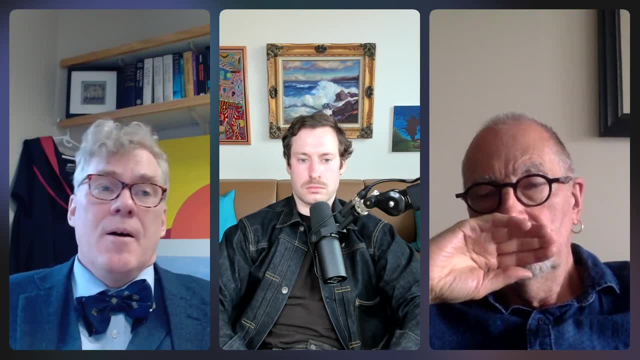 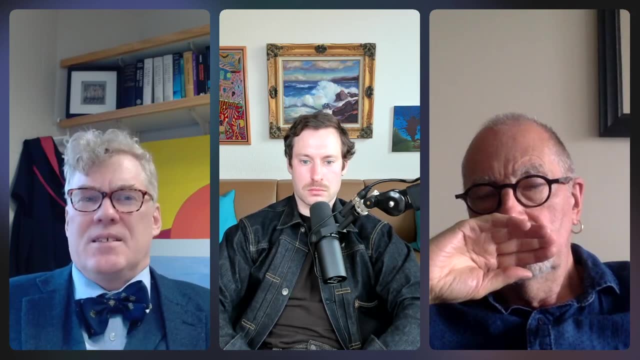 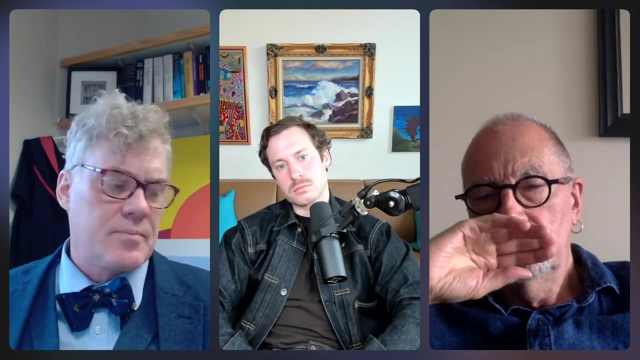 so readily onto the list to make ZFC right, And so maybe we would find an axiom like that that would also settle CH. That's the hope, the dream. But I've argued that this dream solution is impossible now because if you give me some axiom and initially maybe it looks really great. 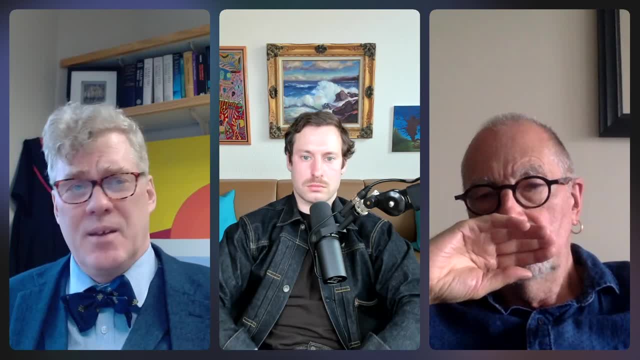 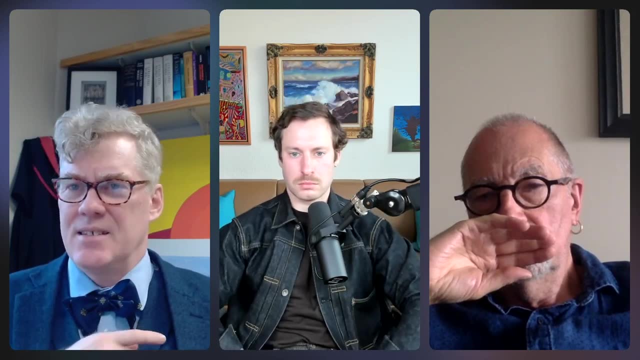 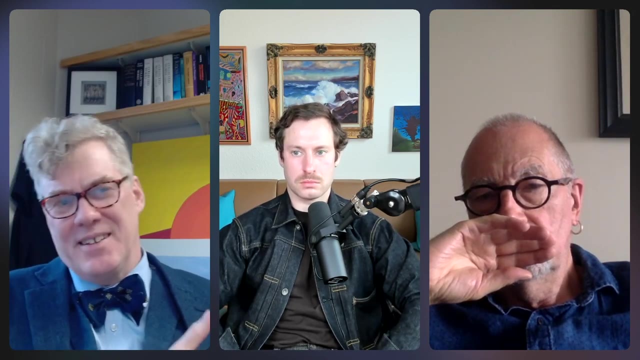 and natural and so on, but then you prove that it implies not CH, then it's immediately contradicting my experience in these not CH worlds. It's like you're saying only Brooklyn exists, right, But I know about Manhattan and Queens and I know how it could be that CH holds. 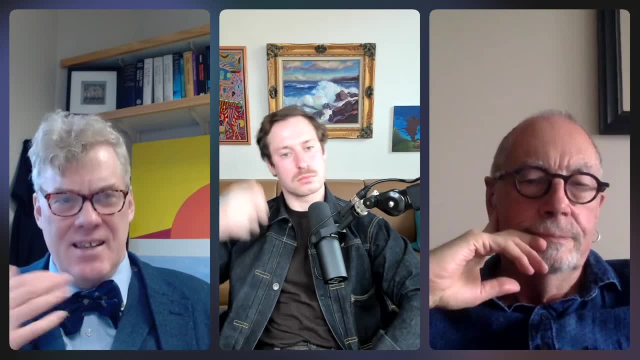 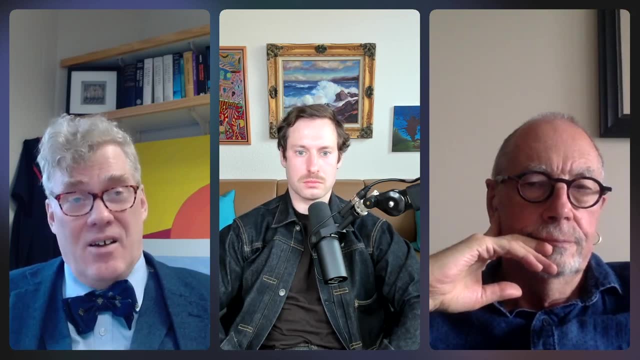 and I know how it could be that CH holds, and I know how it could be that CH holds. I know how it could be that CH fails. So any statement that provably, you know, implies one of those I know is not necessarily true of the concept of set. 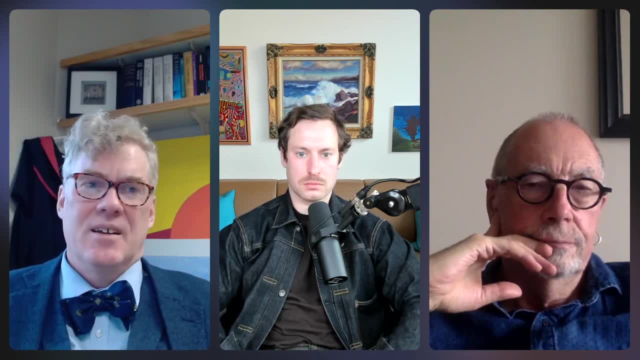 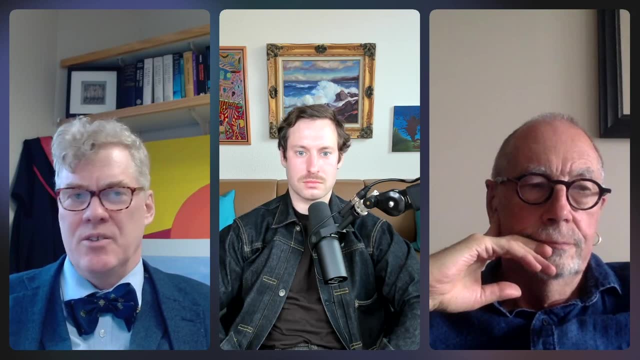 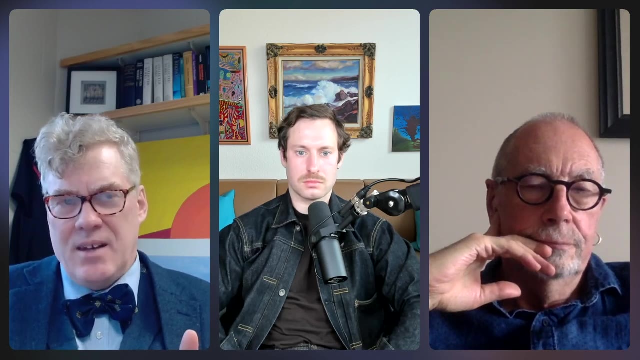 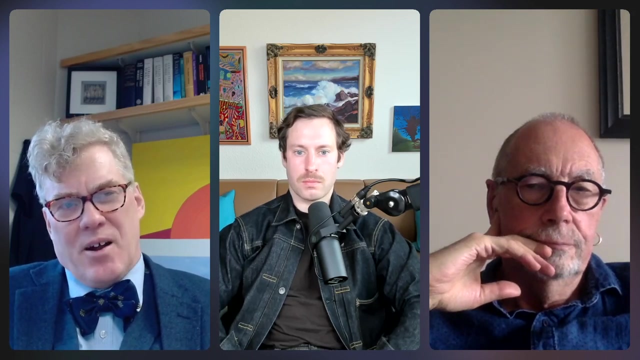 Because I know there's these perfectly set, theoretically acceptable realms in which CH is true and in which CH is false other ones, And so I can't accept the new axiom as manifestly true for sets. because of that experience I don't know how convincing that is, but this is my argument against the dream solution. 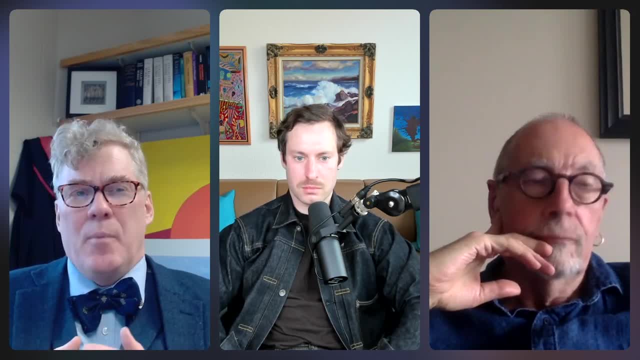 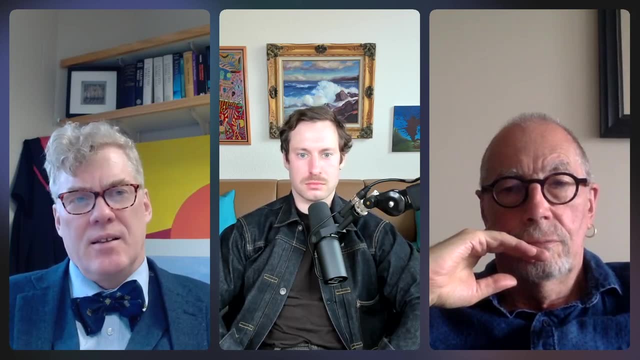 I think as a phenomenon it won't happen ever. I mean, there was an attempt. Freiling's axiom- I don't know if you know Freiling's axiom of symmetry. Chris Freiling considered the statement: Okay, it goes like this: 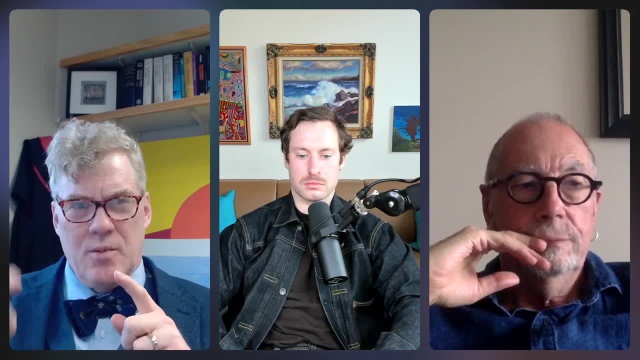 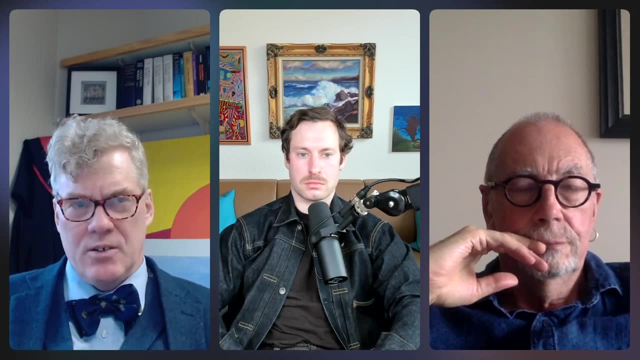 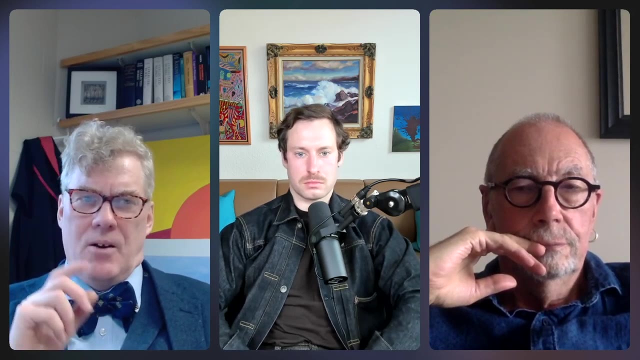 We attach to every real number a countable set of real numbers. A function maps reals to countable sets. Suppose we have such a function. And now Chris Freiling says: throw two darts at the real line. Okay, so the first one lands at X and the second one lands at Y. 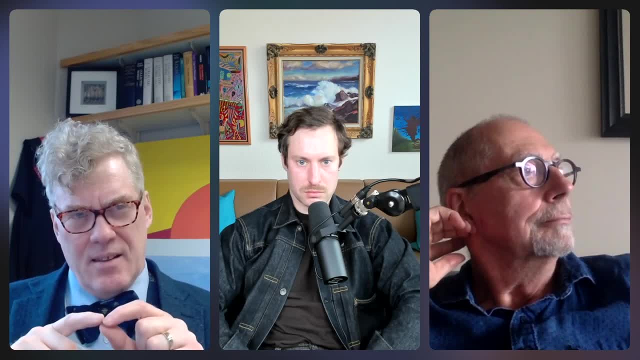 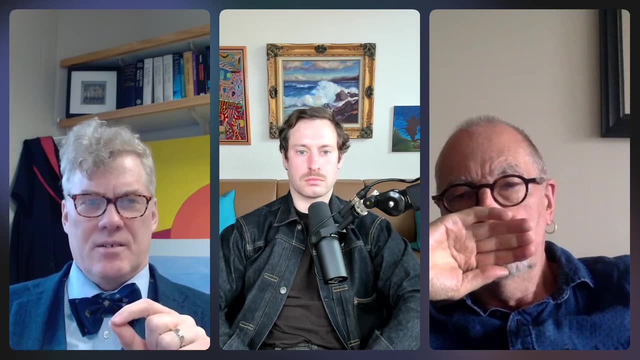 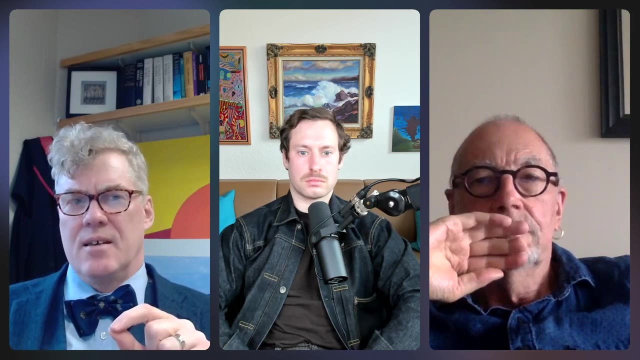 Now, if once X is there, then the set attached to X is some countable set. So almost surely Y, The other dart isn't, isn't hitting that set. So almost surely Y is not in this set F of X. But then, by symmetry, because it doesn't matter which one I think of as the first one, I could have looked at Y first. 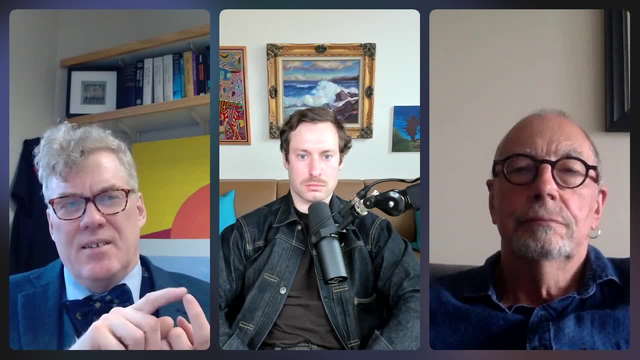 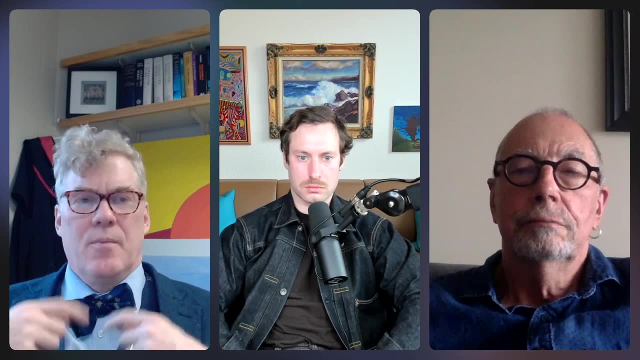 Then almost surely X is not in F of Y. So the axiom says for any function, F, from reals to countable sets of reals, there are at least two points, X and Y, so that neither of them is in the set attached to the other one. 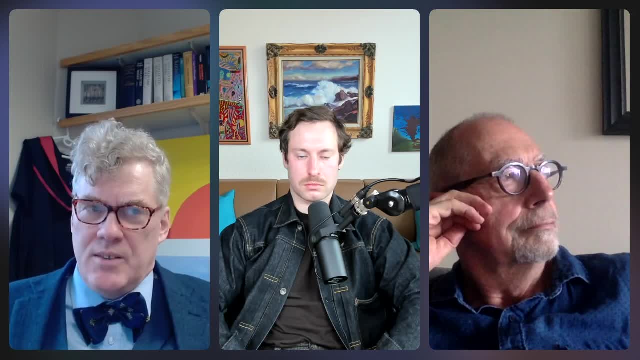 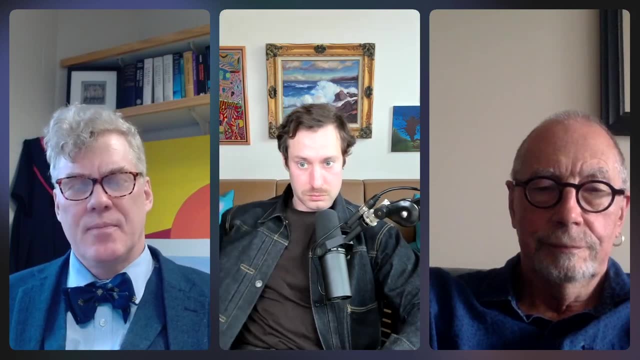 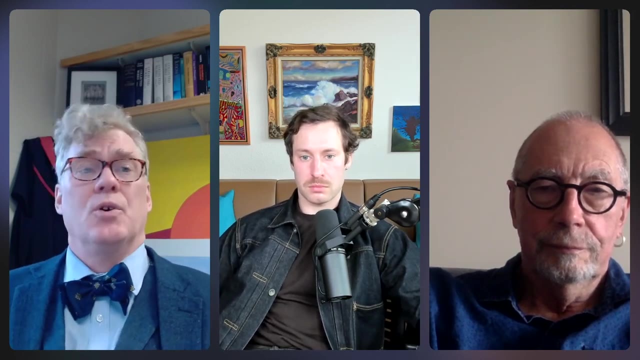 And so he gives this philosophical argument for why we should think it's true, involving these darts. So okay, so Freiling proposed this axiom, which he argued for by thinking about darts, throwing darts at the real line, And then he proved. well, actually it was proved earlier. 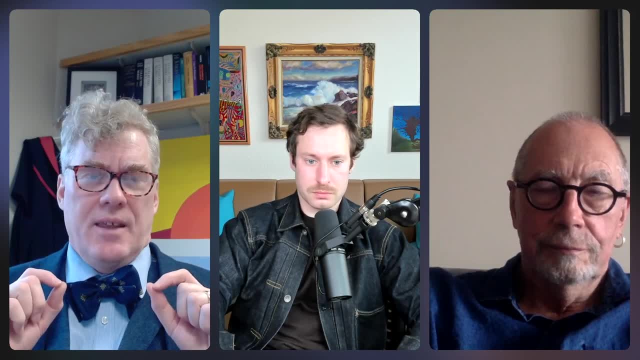 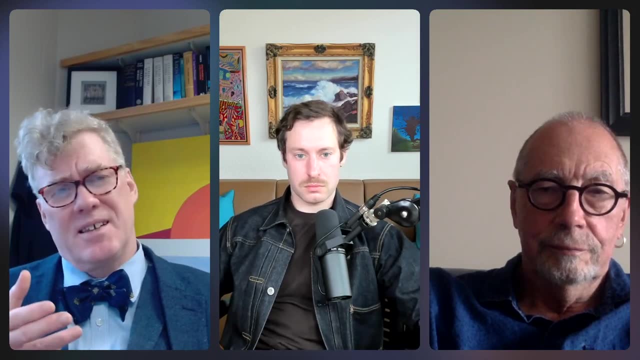 by Sierpinski, I think it was, that this principle implies not CH, It's equivalent to not CH, And so okay? so what's the response? Because it's an instance of the dream solution, if you like his axiom. 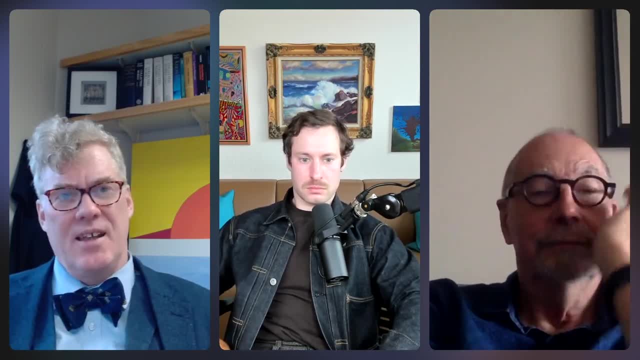 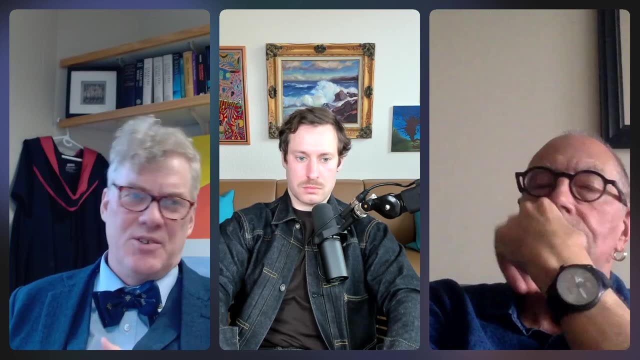 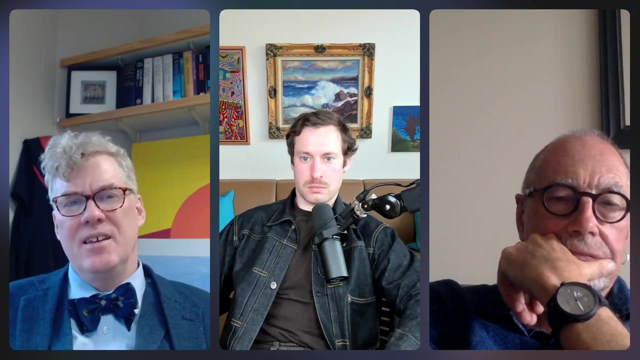 And then you discover it's equivalent to not CH, then that's a reason to think. not CH maybe. But the response of the Satheretic community was almost universal rejection of his argument And to say: look, the argument is naive, It's based on. 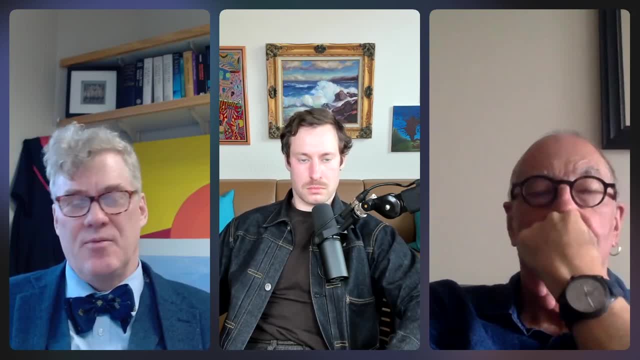 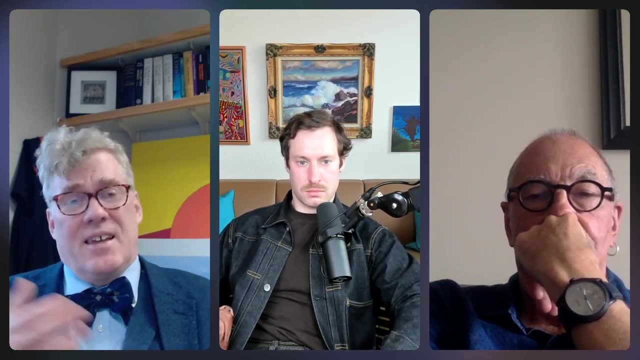 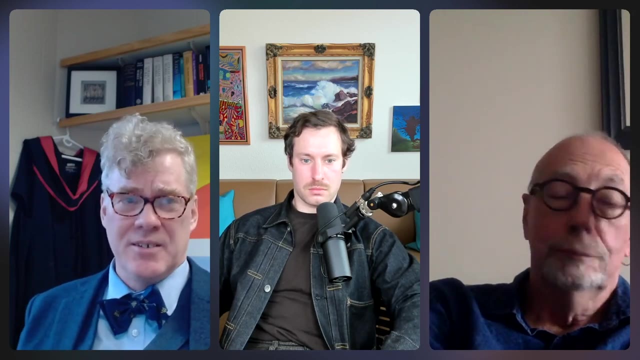 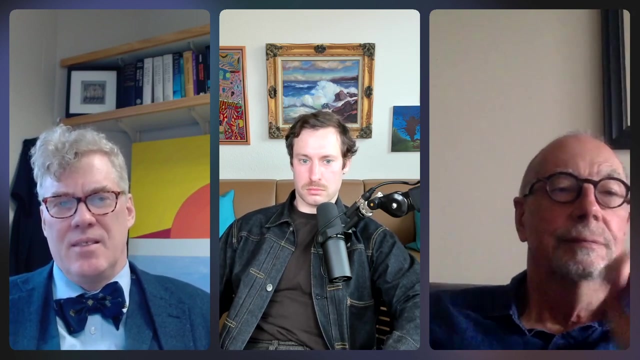 misguided conceptions of measure and the Fubini theorem and so on, And so they gave these. basically, it completely conforms with my prediction about how the dream solution candidates will be handled, Which is that once we know that the statement implies the axiom or the negation of the axiom, then we will reject the naturality of the statement. 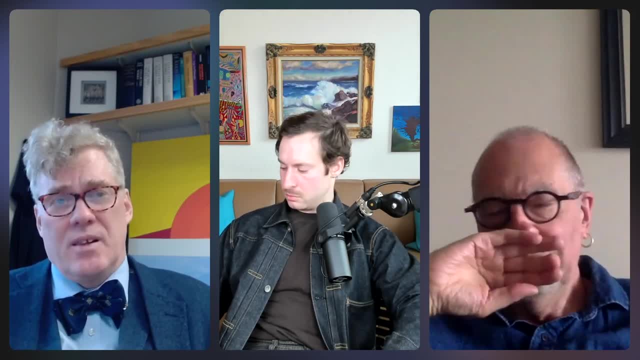 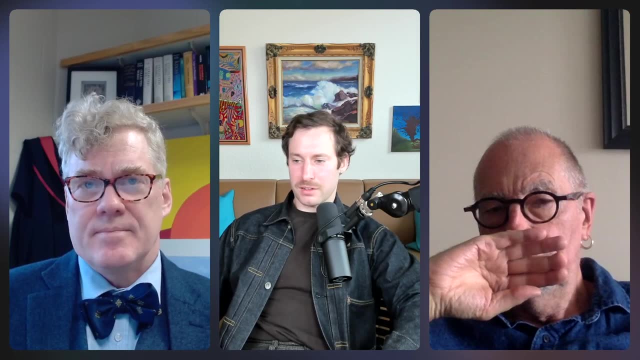 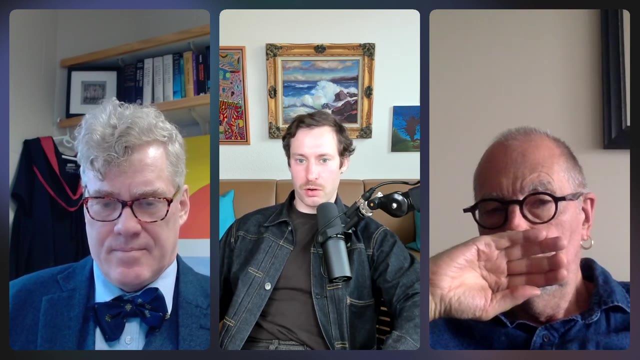 because of this deep, deep, deep, deep, deep familiarity with the way things that can go wrong. so i'd like to turn now to graham's conception of the multiverse. so i know that a couple of years ago you were working on a text called x uno. 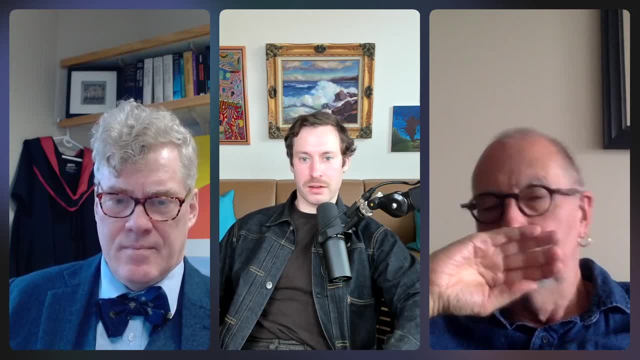 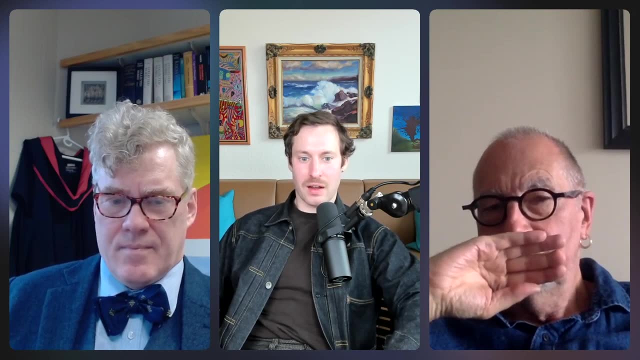 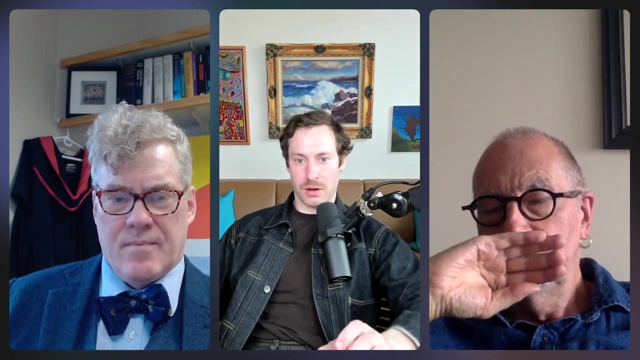 flores, from one many, but i couldn't find it when i was uh preparing for this. so one, i guess. what is the status of that work? and maybe you could say, i guess, what, what it is? that seems to be a natural question, but my understanding, at least from what i recall, since i didn't have it in front. 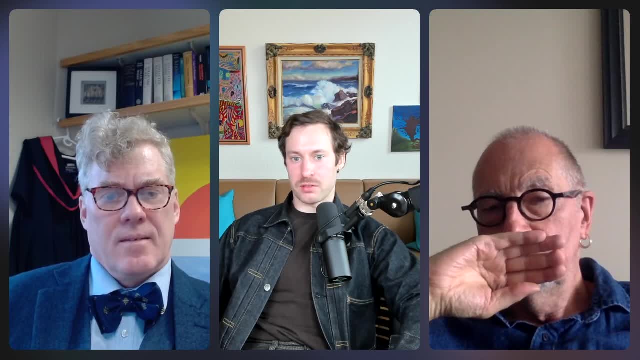 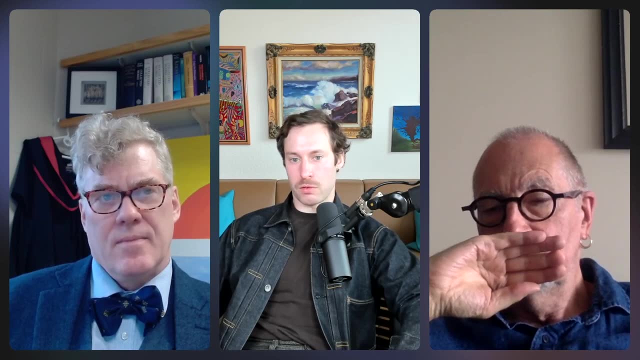 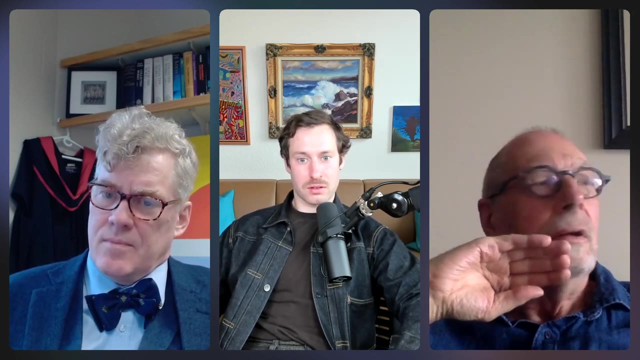 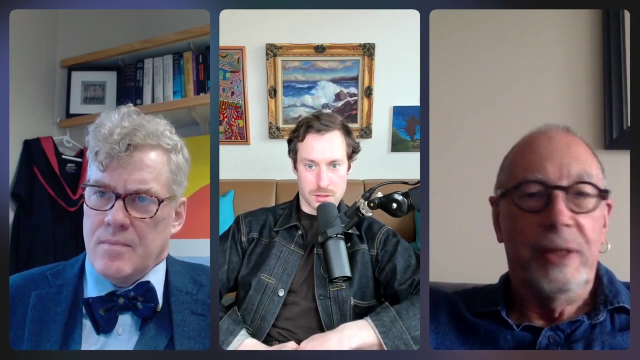 of me was that your conception of the multiverse differs, i mean, sort of drastically from joel's, in the sense that joel's revolves more around axioms, whereas yours revolves more around different logics. okay, so, um, the first question. first, i sent the manuscript off to cup nine months ago. 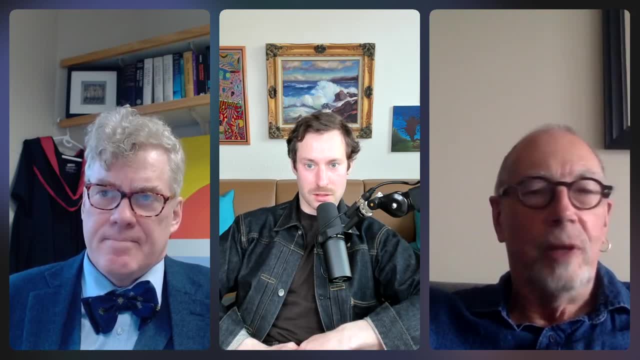 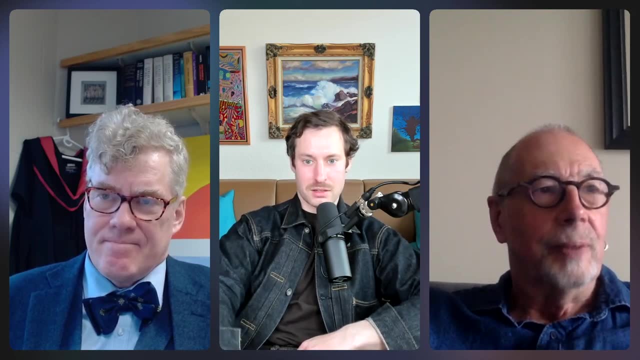 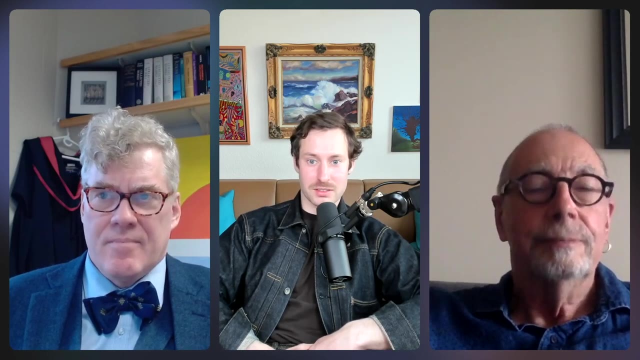 uh and um, i'm still waiting for referees reports. okay, there is action on that front slowly, but, um, when i get the referees reports, it's going to require some polishing and so it'll be a book. oh, and now i don't know when i'm going to find. 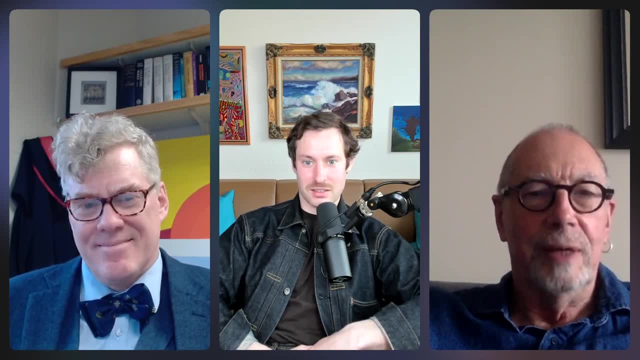 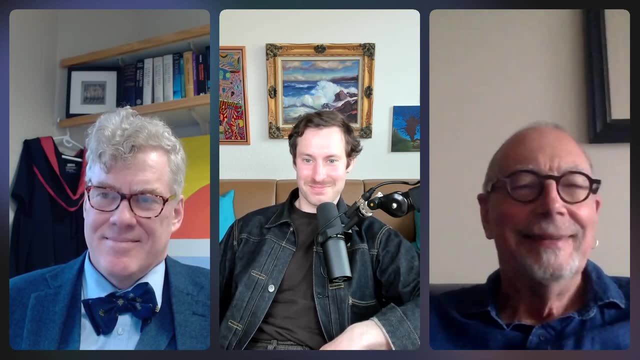 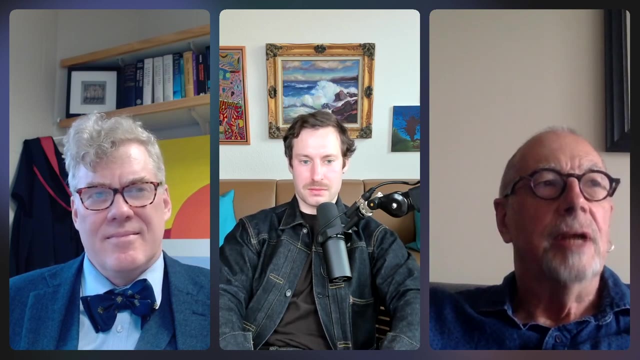 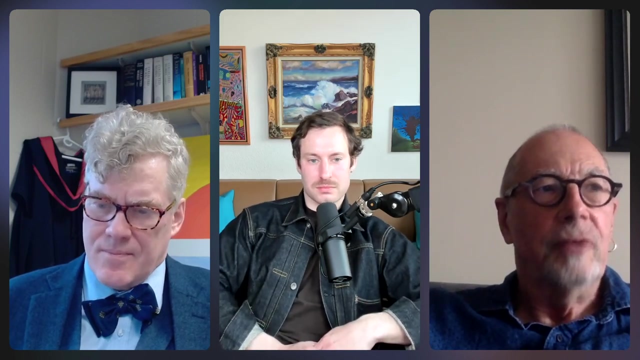 time to do it, so i'm not going to predict when it's going to come out. okay, okay, um, well, i love the name. thank you, um so, um, the thought is this: uh- and it touches on what we talked about a little bit earlier on- there are mathematical structures which have an internal 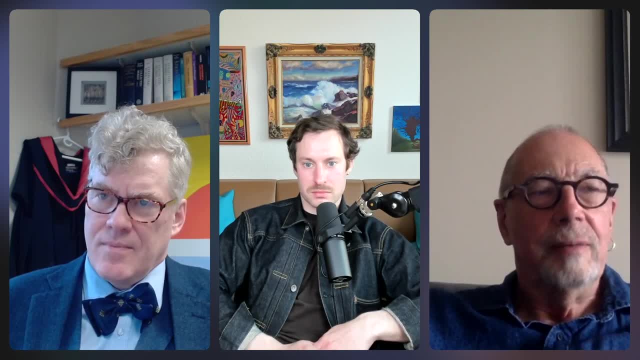 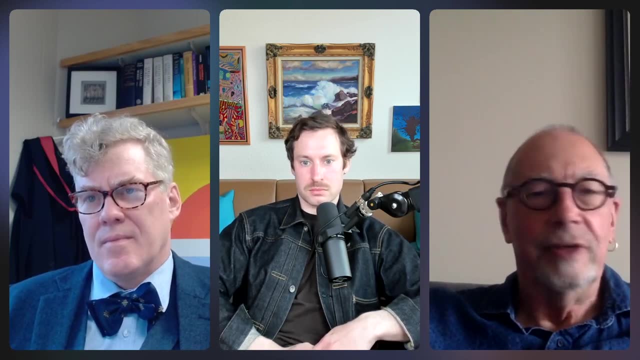 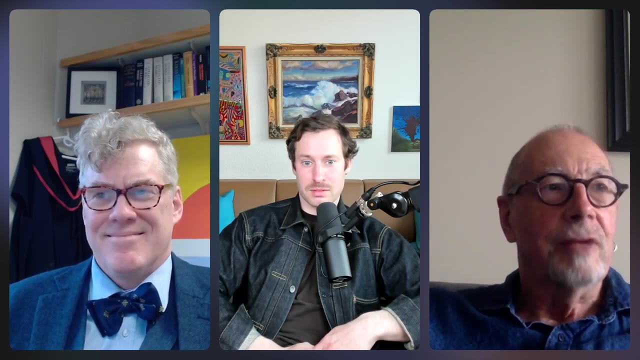 logic, of intuitionistic logic. there are mathematical structures which have an internal logic of a paraconsistent logic, and i kind of suspect that for the rest of the world there's only interesting logic. you're going to be able to say something similar, right and uninteresting logics, i would guess. well, if there are any interesting logics, there are unlike to be the. 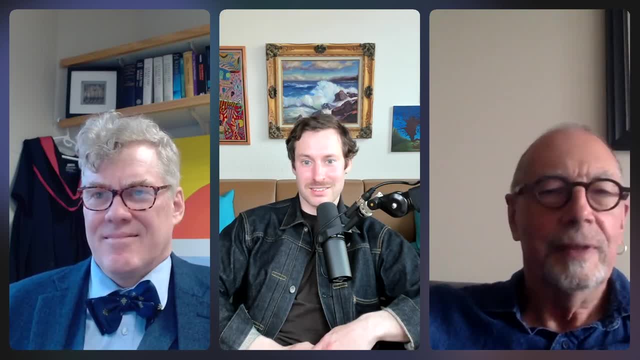 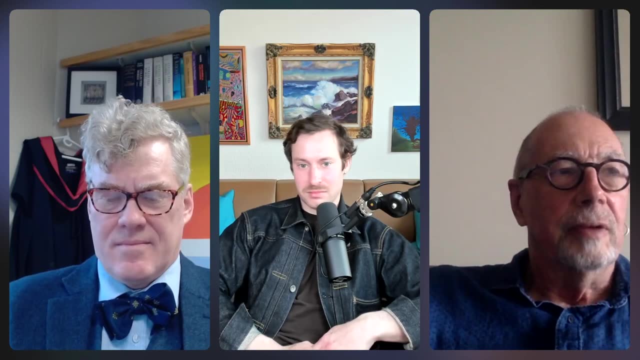 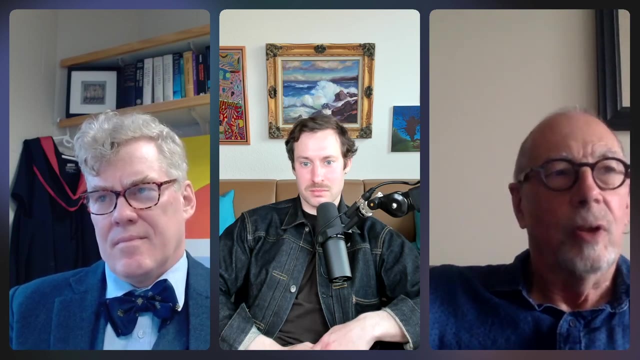 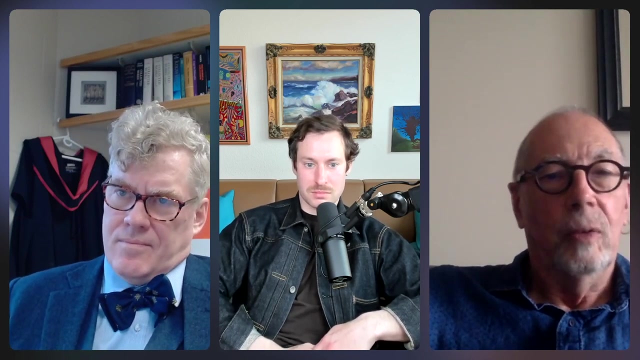 basis of interesting mathematical theories. but who knows um? and the sort of prime thought of mathematical pluralism is that mathematical interest does not, is not restricted to any particular logic. these, all these structures have a interest in, are interesting mathematically and you can investigate all of them. you probably won't. 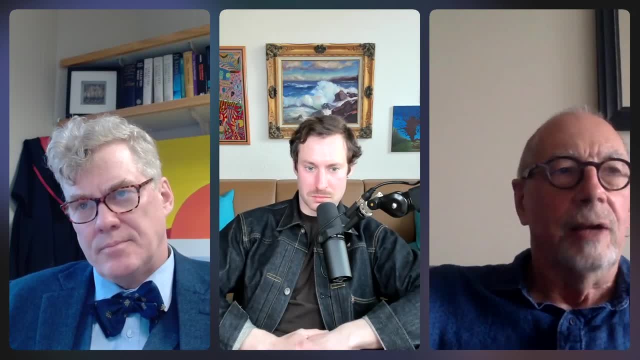 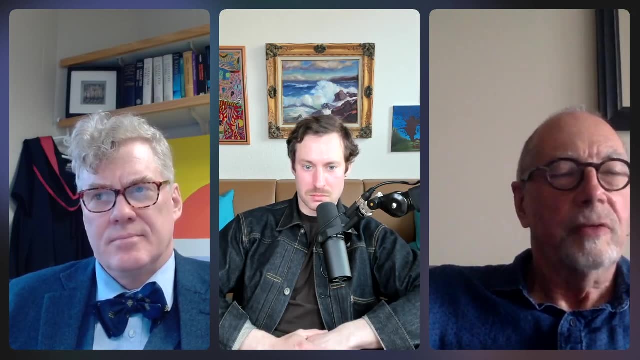 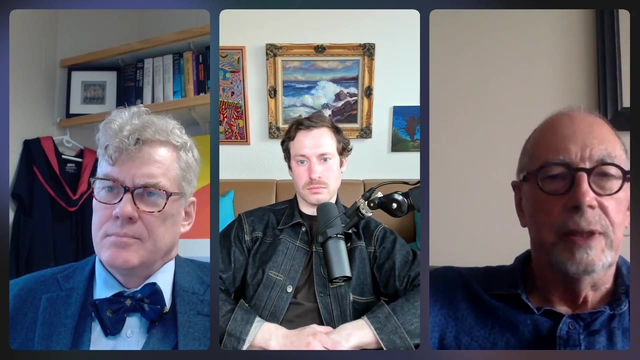 be interested in all of them, but that doesn't mean there aren't? they aren't all equally legitimate, um and so, uh, the view of mathematical realism is: there's all these mathematical theories or structures based on different logics, and in some sense they're all equally good. qua pure mathematics. 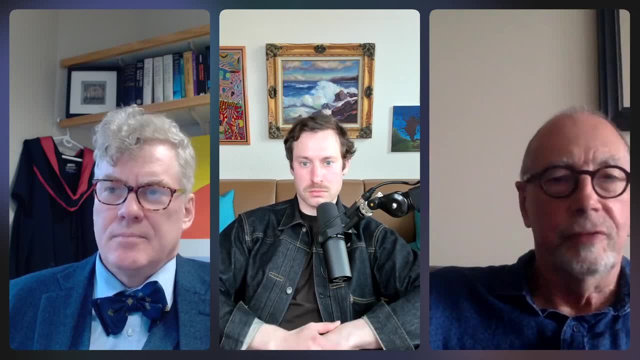 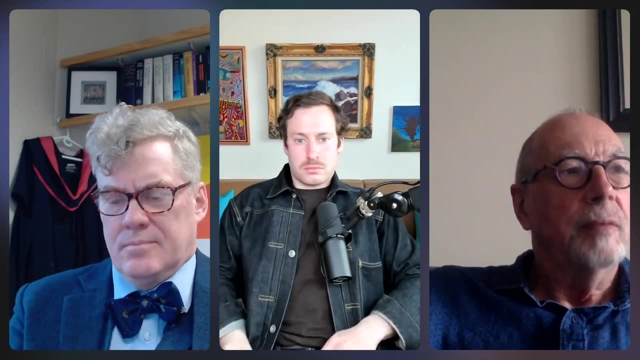 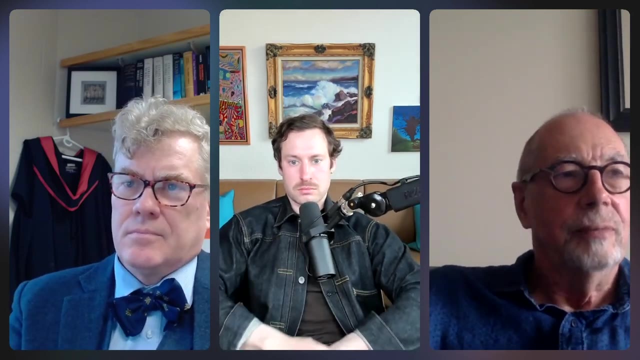 and in terms of applied mathematics, is a different story. but quite human, um and uh, i've never been quite sure what joel's view is on this, but, uh, from what he said earlier, and well, what you say earlier, joel, um, you're not unsympathetic with this view. 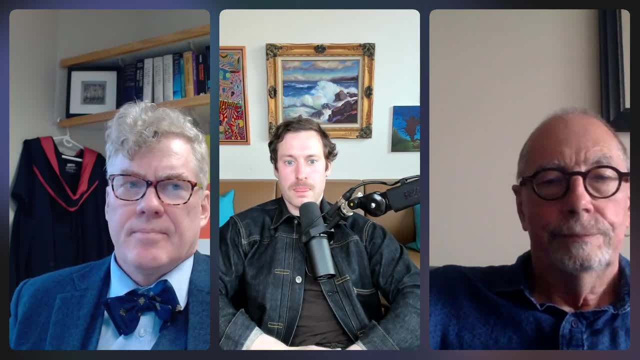 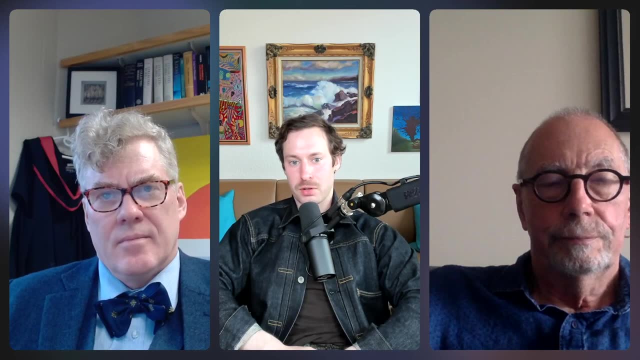 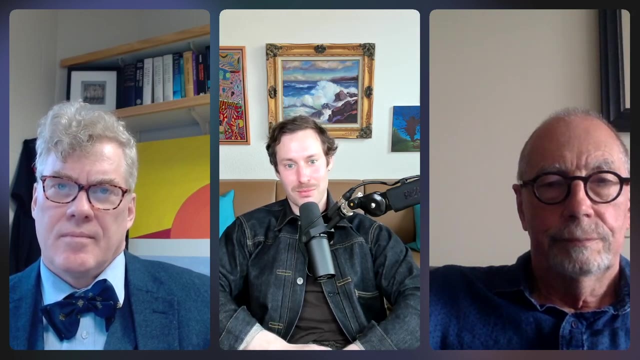 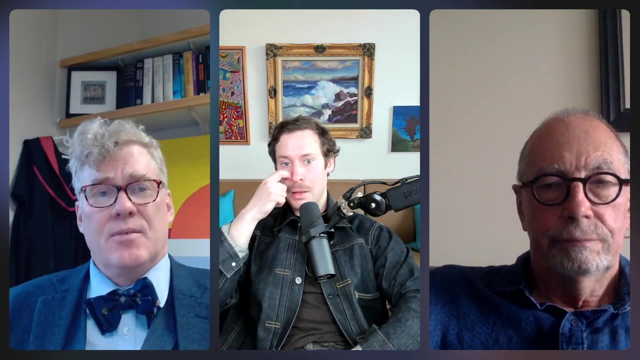 that's the sense that i got. but i was wondering, joel, if i mean in your set theoretic multiverse there is a number of realms for intuitionistic, um logic based set theories. is that the case? i mean, of course? uh, one can have a conception of. 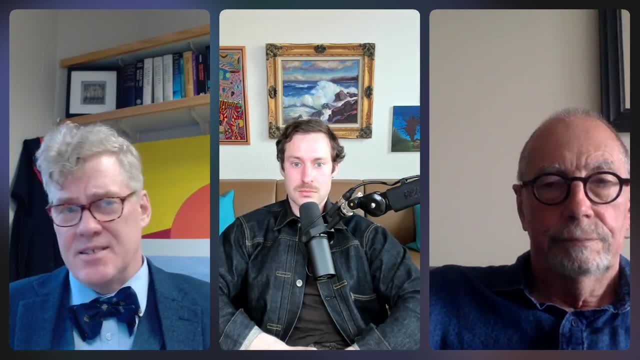 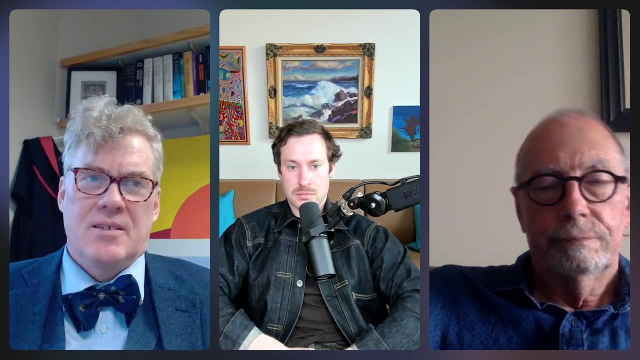 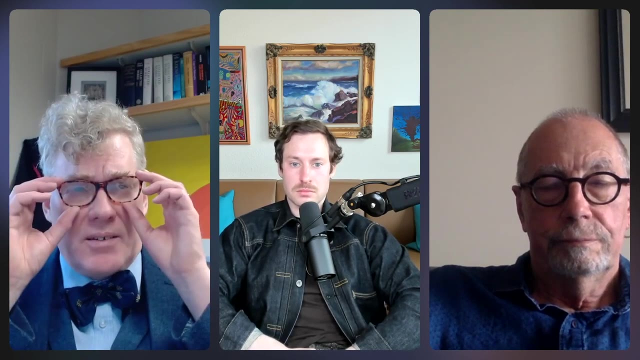 set theoretic pluralism which is accommodating the intuitionistic uh set theory, or even very consistent set theory, and i would view that as sort of you know, partaking of the similar ideas um to to, you know, uh, to what i had in mind, but um, i mean, as i said earlier, i 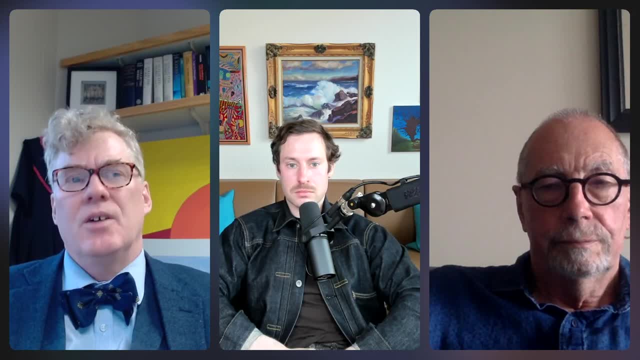 i myself have a lot of experience with the theory of set theoretic pluralism and i think that's a. i have a lot of experience with set theoretic pluralism and i think that's a happen to look at those very much, although i've done a little bit of work. i mean, as graham knows, 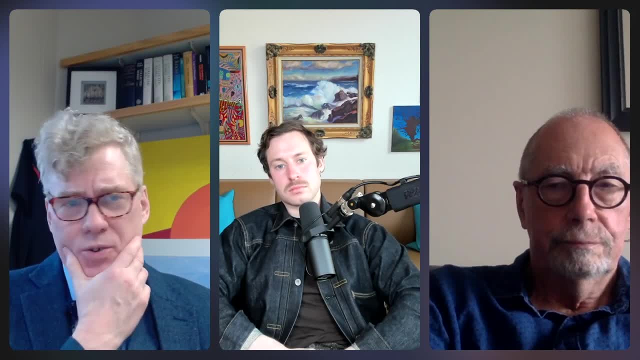 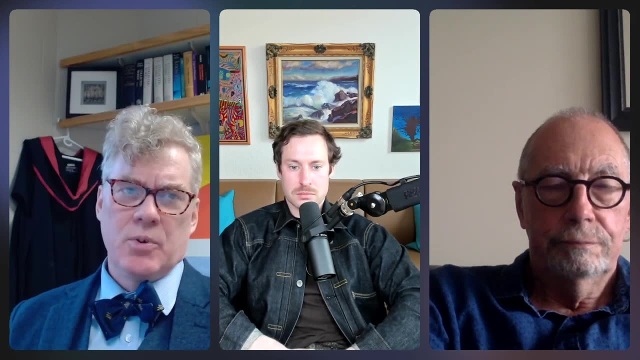 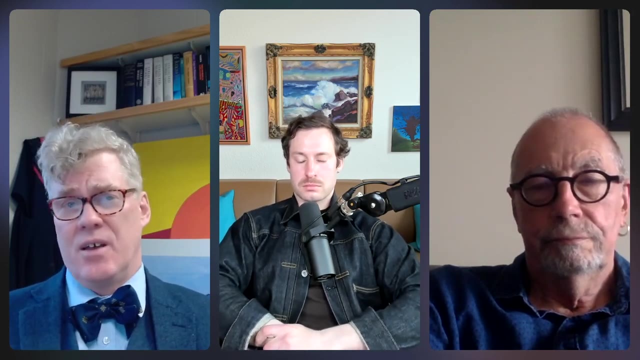 i uh had an approach to pair consistent set theory, based on the sort of green value model approach, but using pair consistent algebras instead of green algebras, um, and and this gives a very robust- what i view as a very robust- collection of set theoretic conceptions that 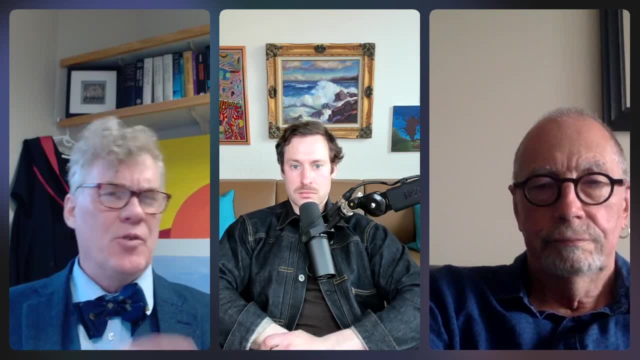 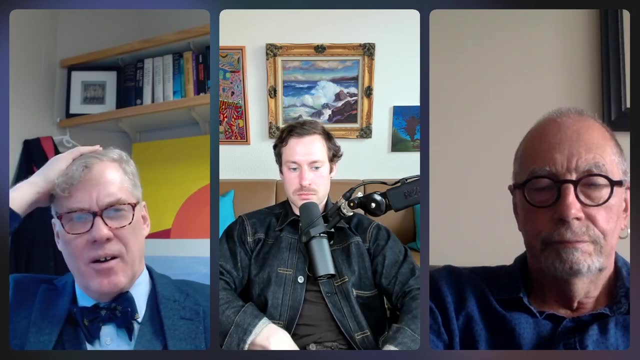 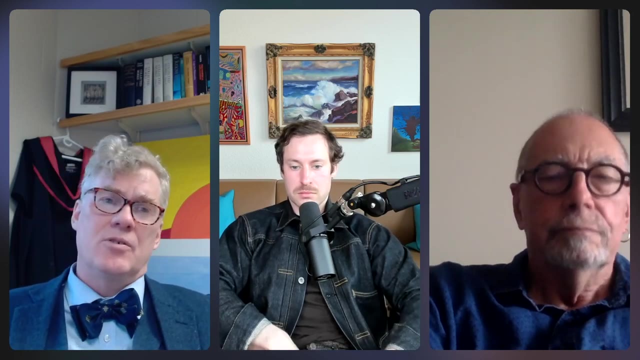 would have pair consistent logic happening. you know, after i did that, uh, benedict lover wrote this really great paper. he had a co-author, whose name is escaping me now, um, in which he did it much better than me, uh, and developed this sort of theory of these structures quite a lot, and 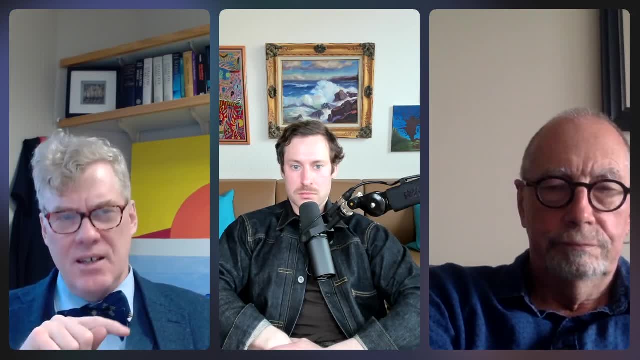 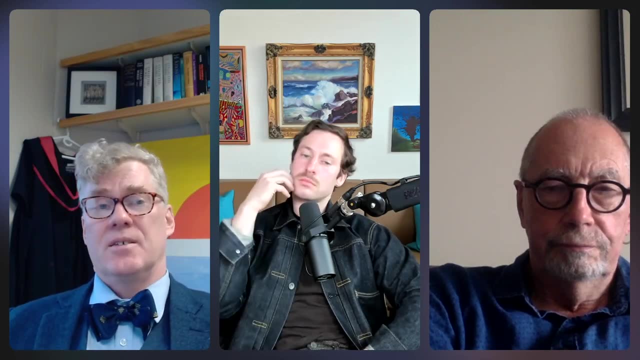 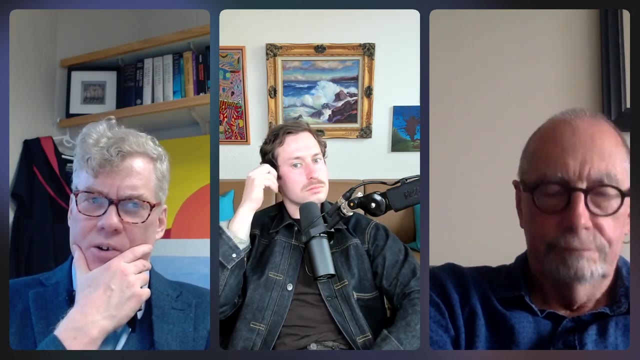 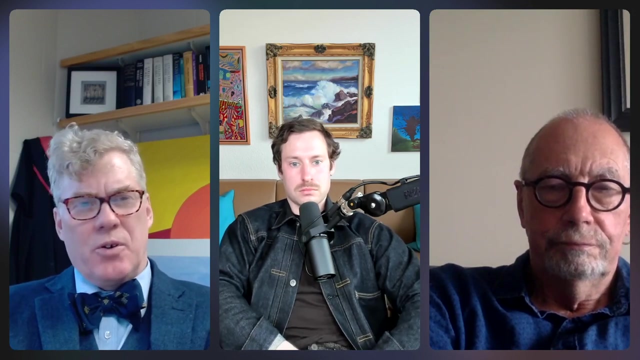 and analyzed exactly what you need in the algebra, in the pair consistent algebra, in order to achieve certain things um in the resulting set theoretic model. but i had the sense at the time it was at this meeting in connecticut, if you recall, and you were there and jcpo was there and, uh, some of the other logical pluralists were there, i think. 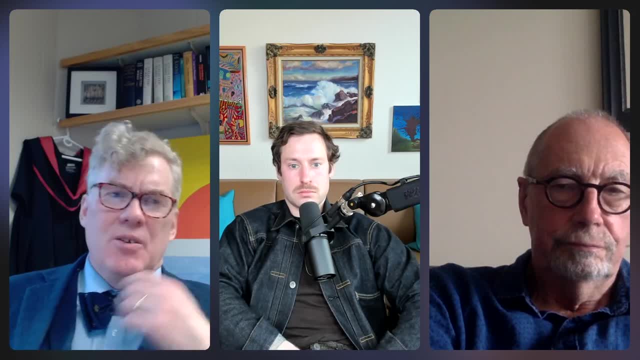 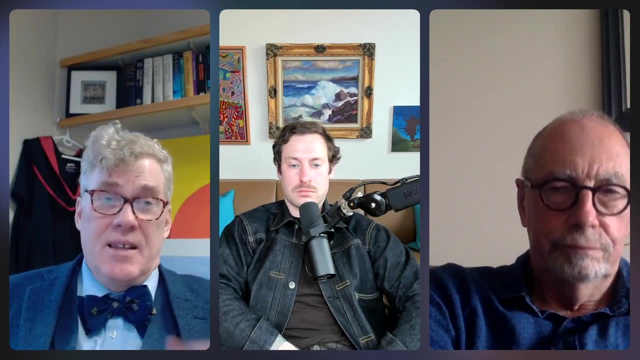 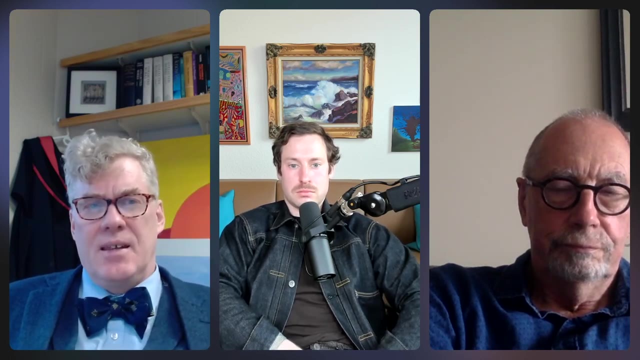 and um, but there was a view that that those kind of models weren't really what was wanted from pair consistent set theory. at least that was my sense of the reaction, because part of the view was to get was specifically aimed at getting models of pair consistent set theory in which the general comprehension principle comes out. 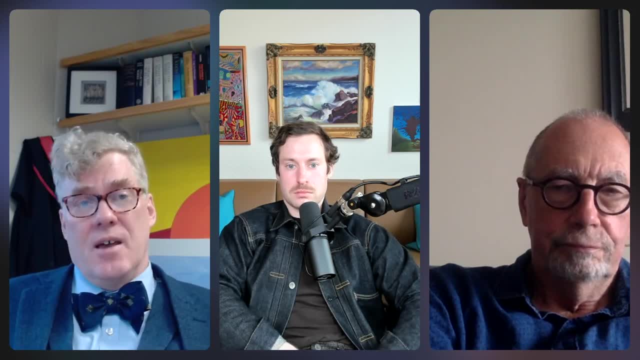 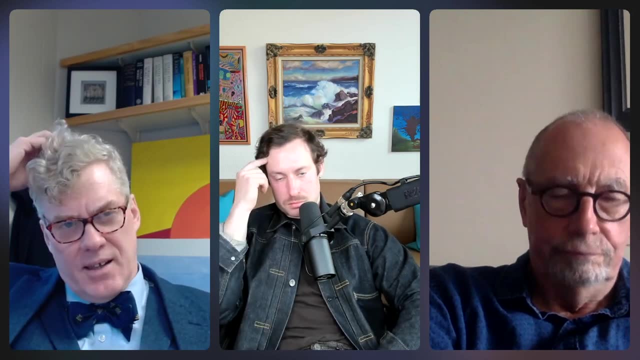 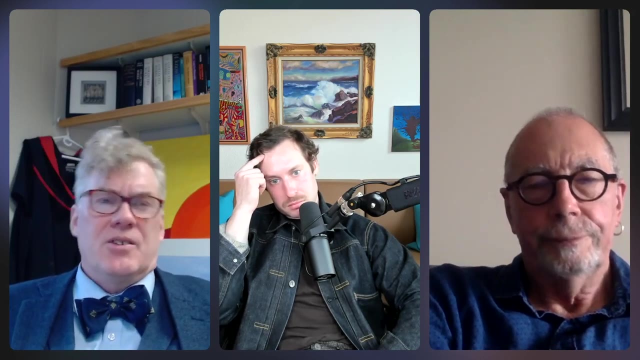 true and also false. i mean, necessarily it would also be false, but you wanted it also to be true and none of these models were like that, because the general comprehension principle was just false and not true at all. um and so, uh, so yeah, i mean, i guess i view all that as sort of part. 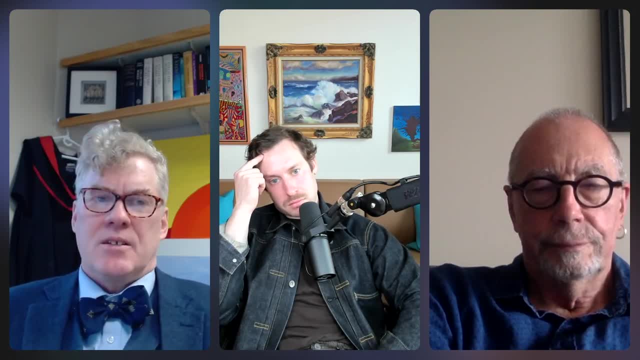 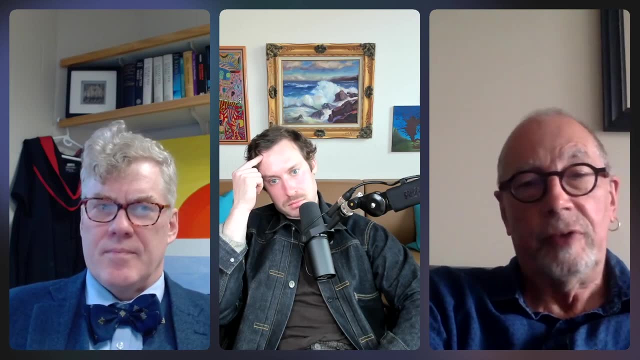 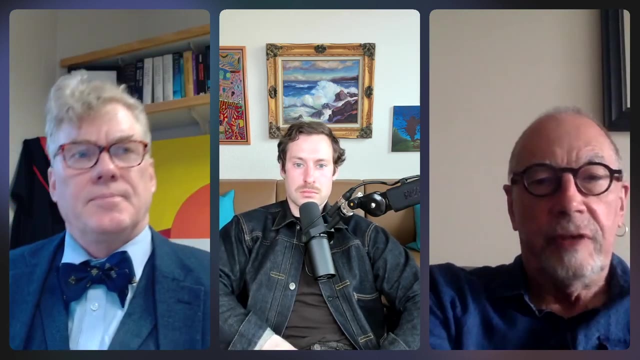 of set theoretic pluralism, even if it isn't the main part that i was looking for. well, with respect to what you say and that particular meeting, which was very fruitful, your suggestions were particularly fruitful. i thought um the situation is this, um, since the kind of 70s. 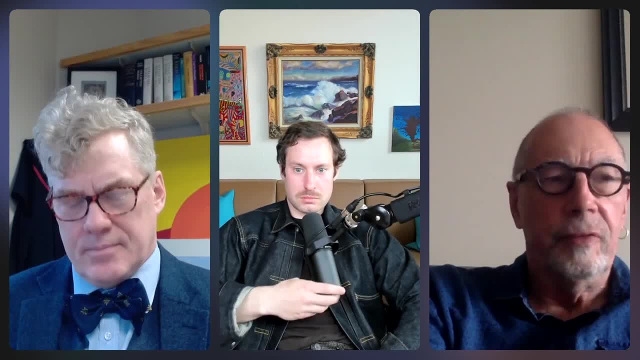 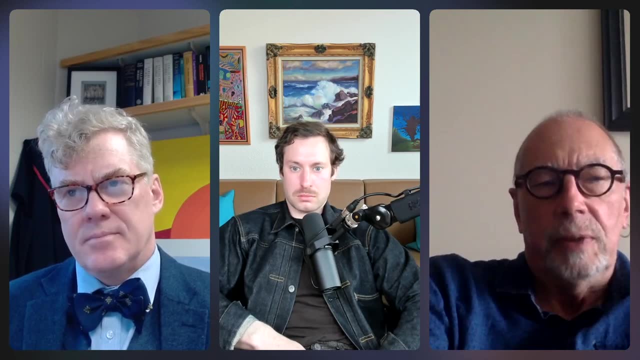 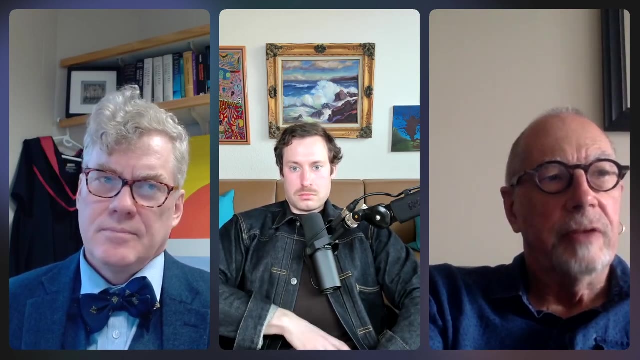 uh, the thought is that the naive theory of truth and the naive theory of sets um could and should be formulated with a pair of consistent logic. i mean, this takes us back to, you know, the solutions, the liar paradox and so on. and it must be said that, as far as the 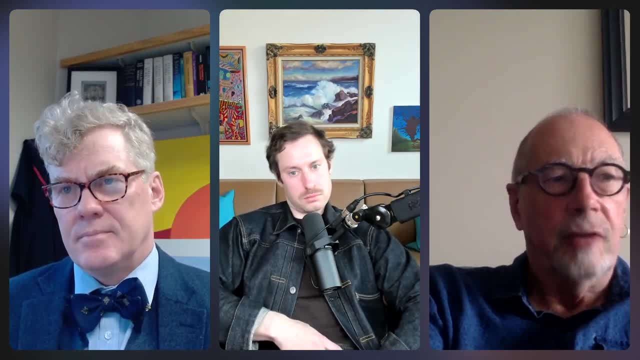 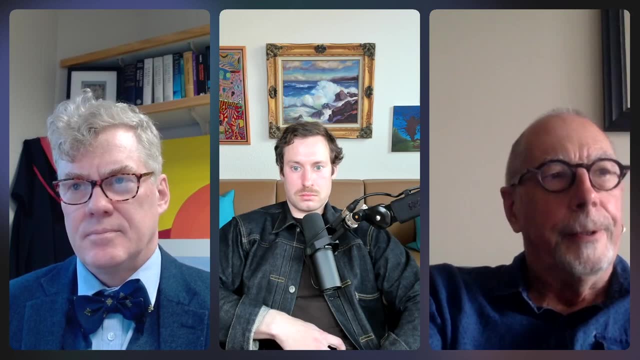 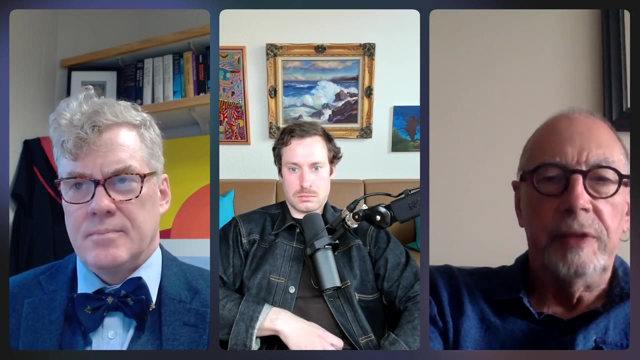 theory of truth goes: um. that's pretty well tied down there. we know what our consistent theory of truth is like. we know its properties and so on. um, the power consistent theory of sex has turned out to be a much more problematic beast. um, and for a long time it wasn't even clear that you could prove. 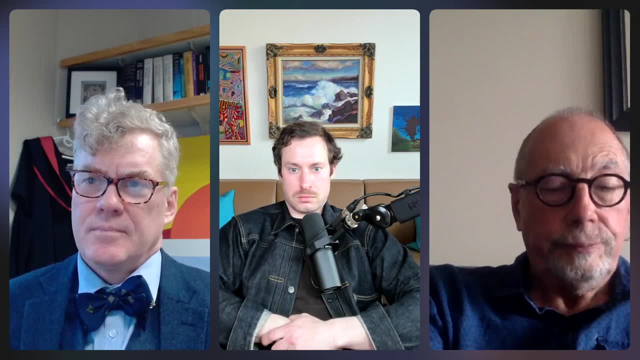 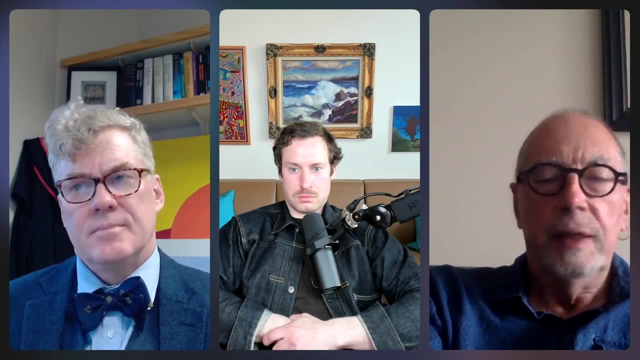 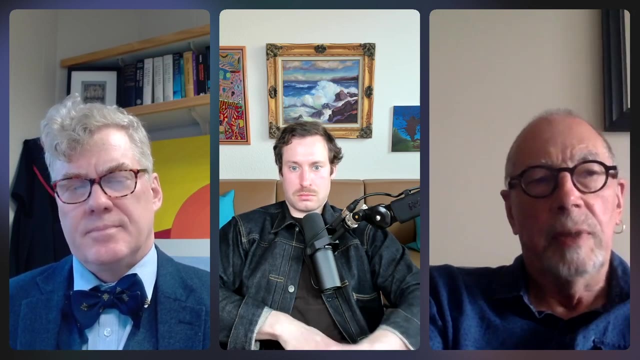 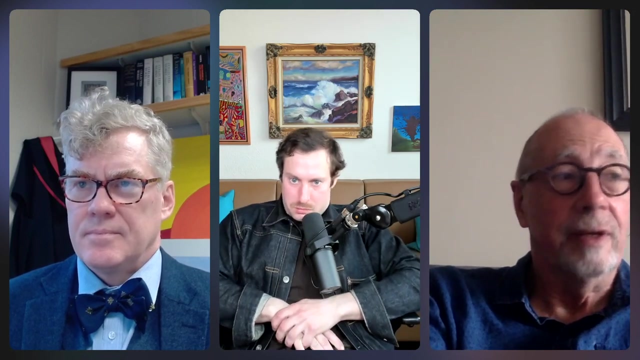 standard results of um ordinal theory, cardinal theory, in in such a theory um presumably any of decent power. consistent set theory should do that. in that way, i mean, the set theory differs from the truth theory because the naive theory of truth doesn't have to answer too much, whereas the naive theory of sets. 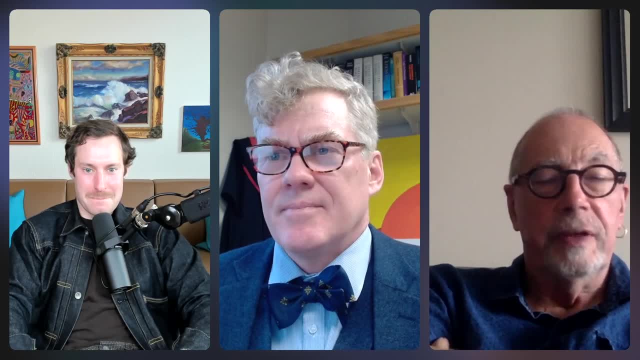 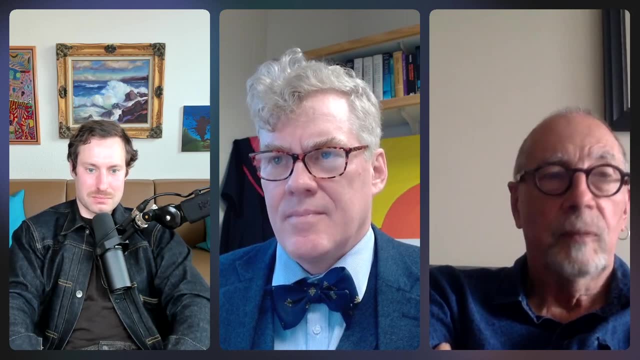 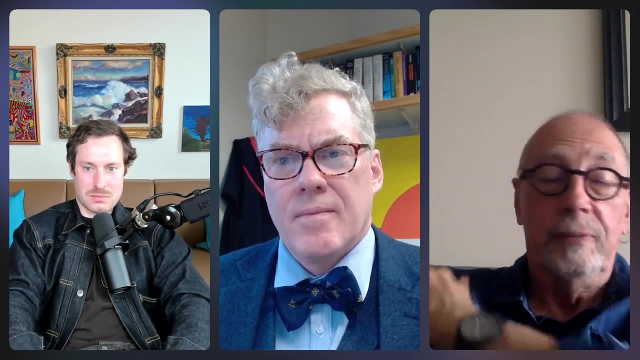 has to answer to a lot. so the problem of finding um proofs of the standard results of transfer over with it was solved by zack weber about 10 years ago, um, and it is a very nice solution. before, people who attacked the problem, such as me, have been trying to reconstruct the old proofs. but what that turns out to be, 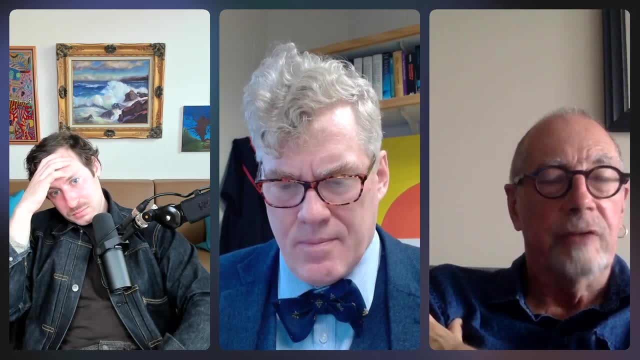 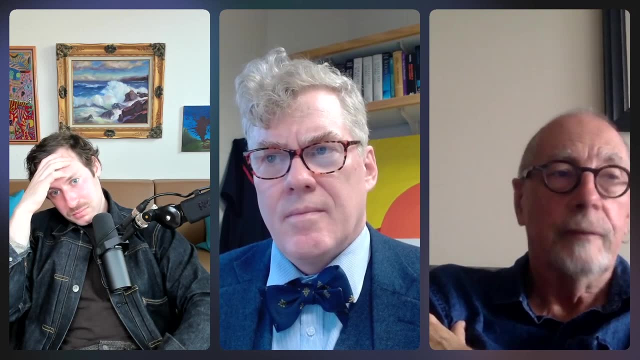 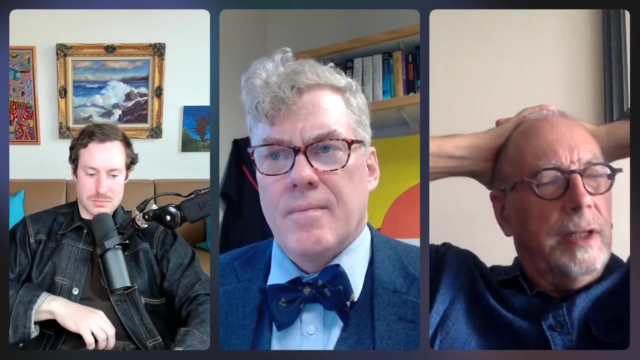 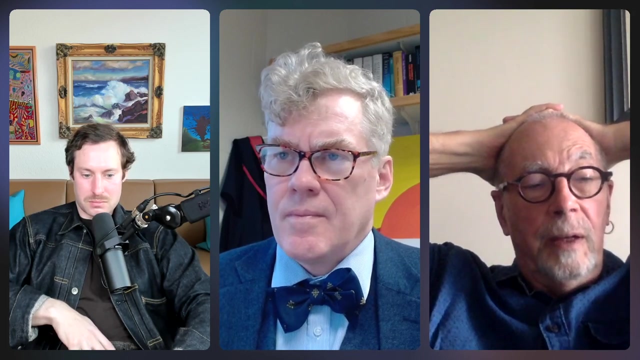 pretty helpless, um, and so what zack did was construct very different proofs which use the properties of inconsistent sets, essentially, um. okay, so that that was really nice work, but it doesn't really solve everything. because it showed that you can use paraconsistent set theory to do trans finite arithmetic. that's fine, but of. 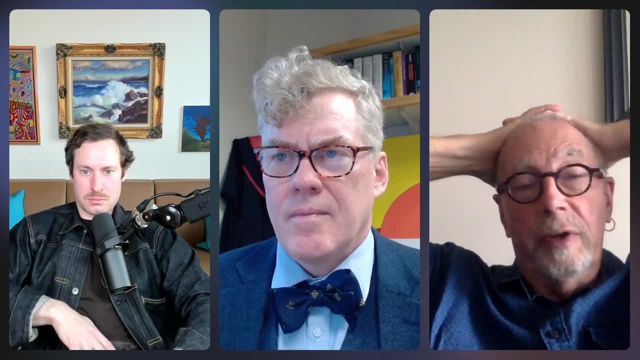 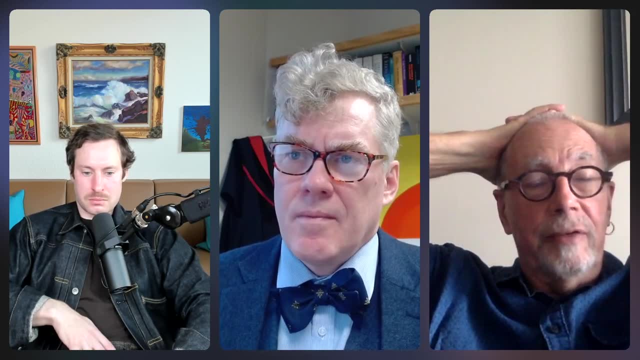 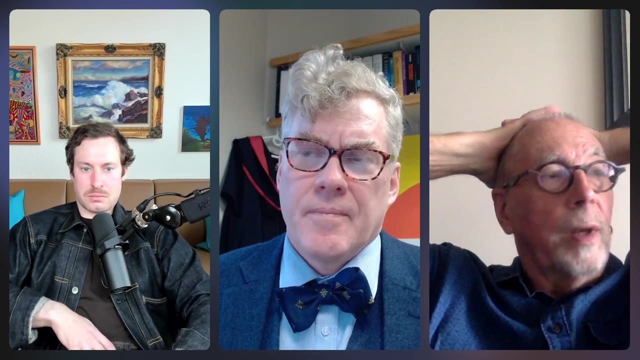 course we use set theory to do a lot of other things. We don't use it for model theory, for example, and it still isn't clear whether you can get a paraconsistent set theory if we do that. That's still an open question. Now, when I talk, 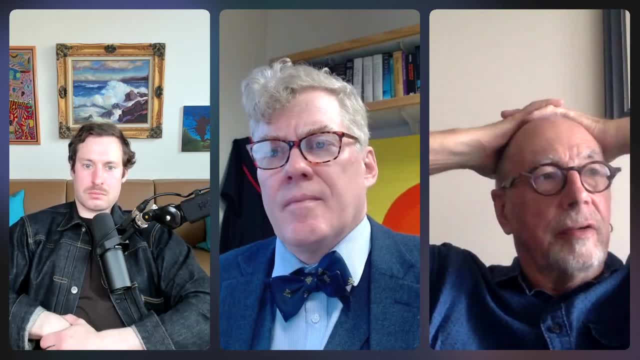 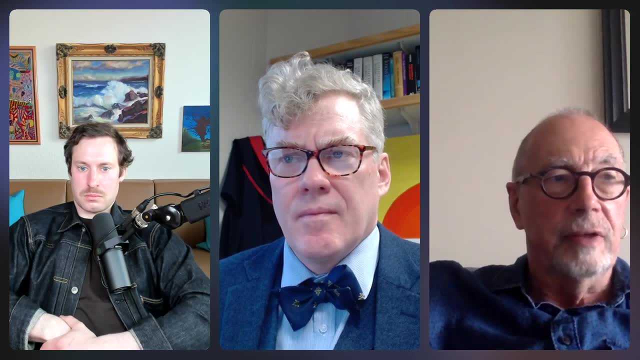 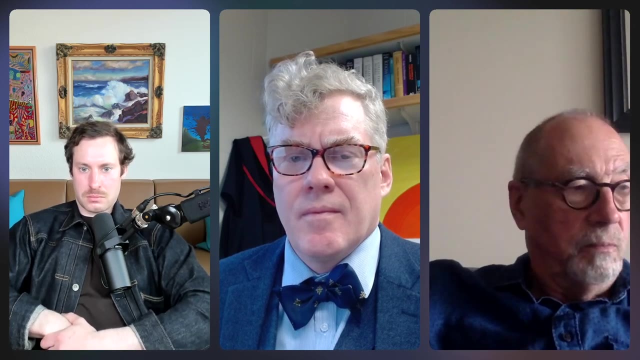 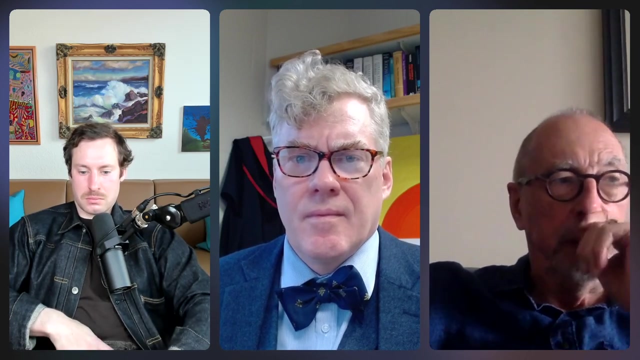 about paraconsistent set theory. in this context, there is an assumption I've been making, which is that you formulate your paraconsistent set theory with a detachable conditional, usually a conditional for which most moments work, Probably a relevant conditional. that's where most of the work has been done And 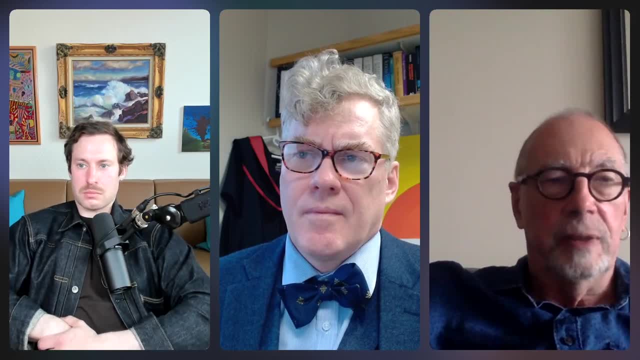 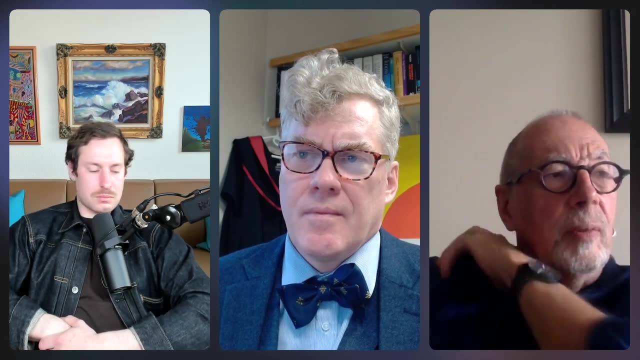 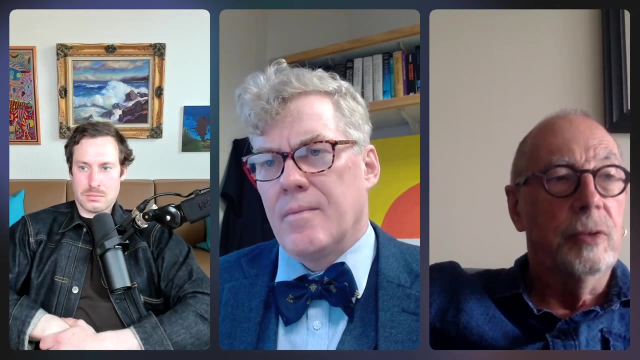 that's the question I've just been talking about. but because it seemed rather clear, I'm not going to go into that. Okay, and then there's the grim possibility. I thought about a rather different way of approaching things 20 years ago, which is this: You don't talk about a mono-verse. 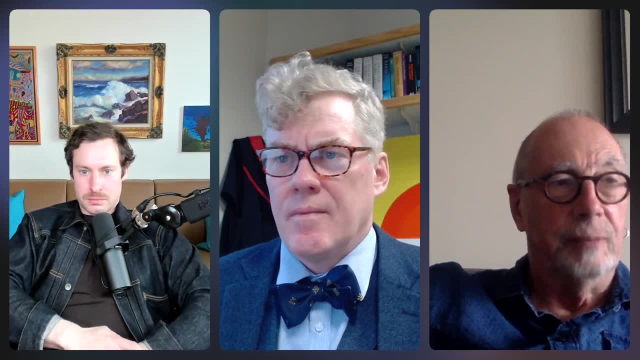 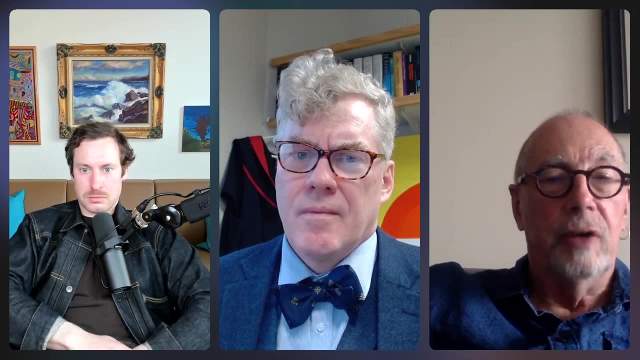 you talk essentially about a pluriverse. So it sort of links with Joel's view here. And there are lots of paraconsistent set theories and there are lots of monoverses. and there are lots of paraconsistent set theories and there are lots of monoverses and there are lots of. 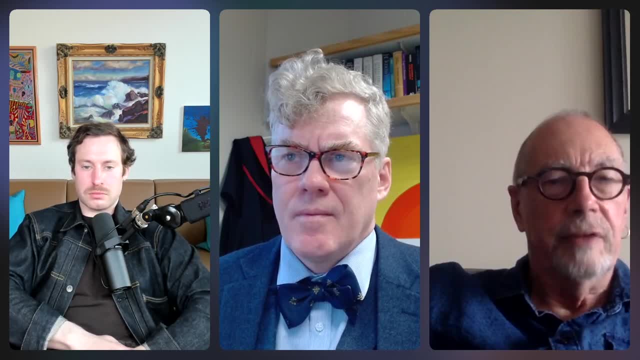 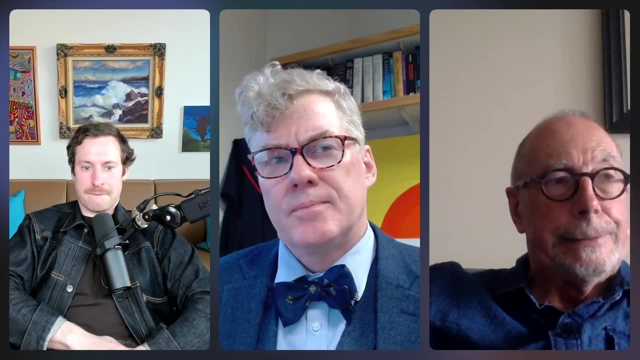 paraconsistent set theories and there are lots of monoverses and there are lots of for reverses. You can think of these as models. It won't do any harm. for the moment. Some of these are classical, some of these are non-classical and some of 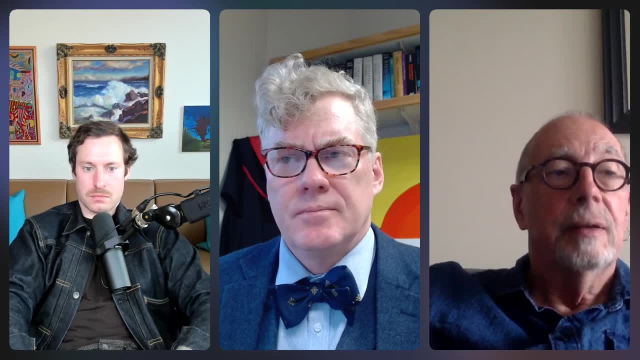 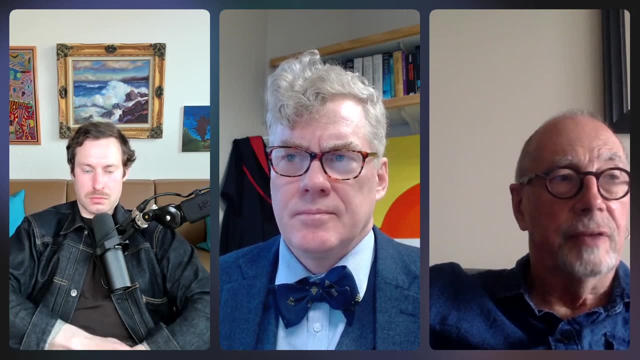 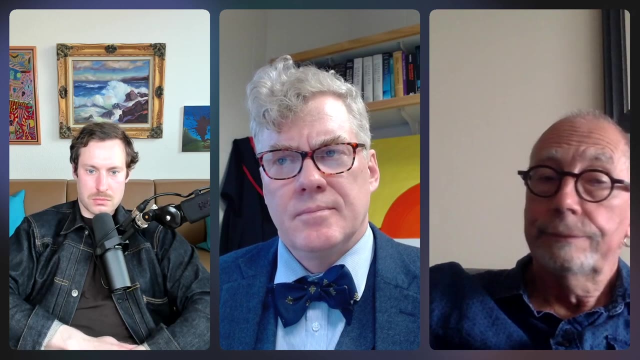 them are going to satisfy naive comprehension, at least in the form of a material biconditional Some of them are going to have, some are going to verify that, and all the theorems of ZF. That's kind of surprising. So there are some. 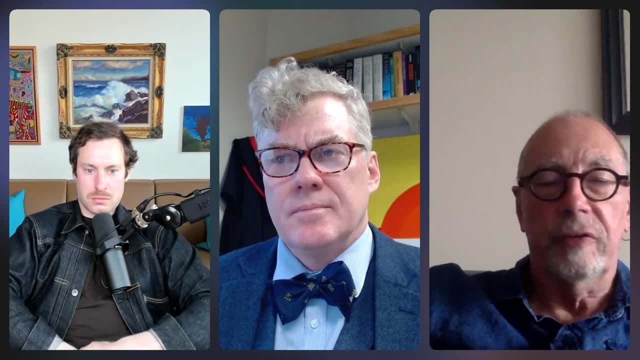 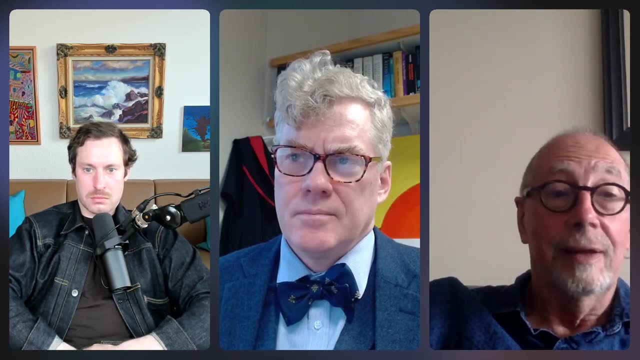 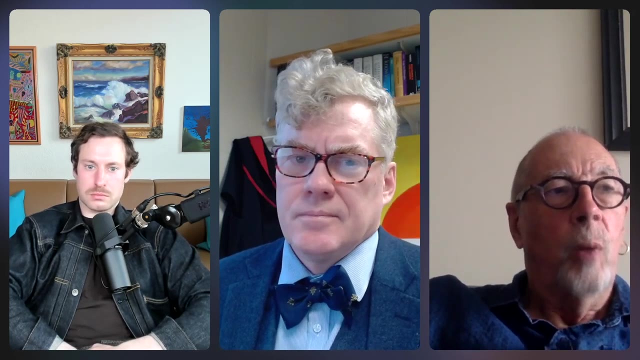 interesting model theoretic constructions- some of these were discussed in the STORS meeting- which allow you to construct members of the pluriverse that are like that. So the thought is: hey, what we're doing when we're doing? power-consistency theory. 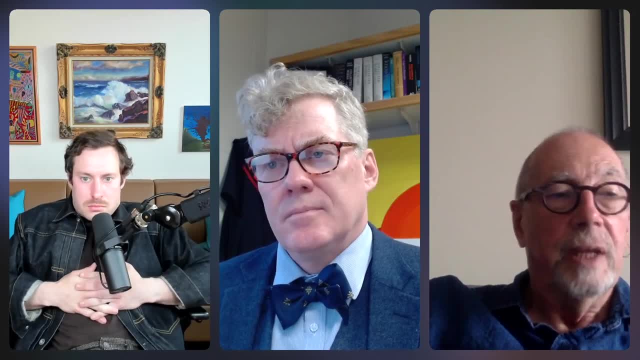 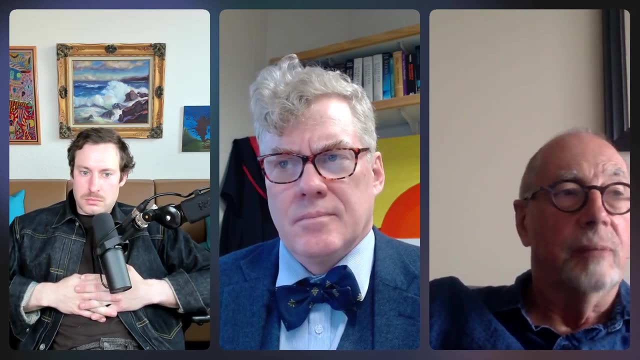 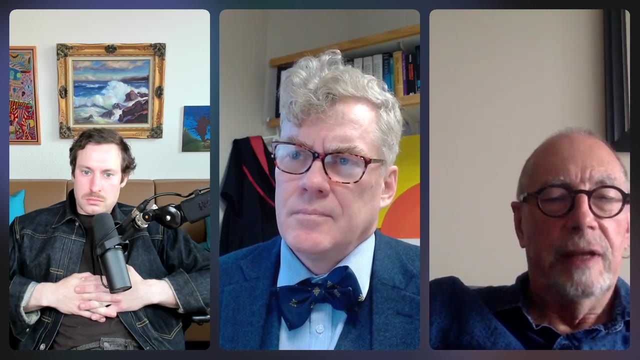 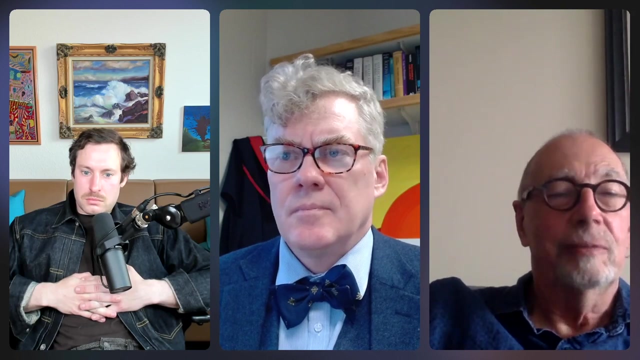 on naive set theory, rather, is working in these models, which model ZF or the theorems of ZF, and also naive comprehension, And I guess, unless and until a version of power-consistency set theory with a robust conditional turns up. that's what I kind of like, So it's a bit complicated, but that is in. 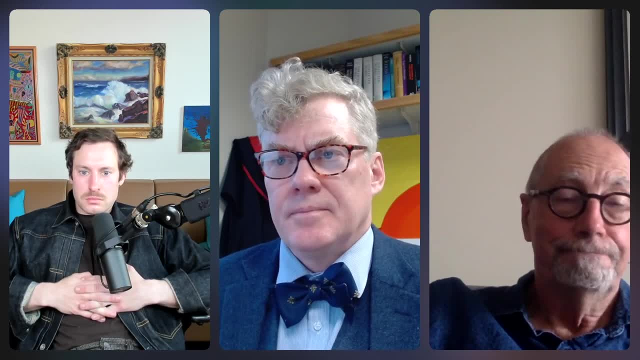 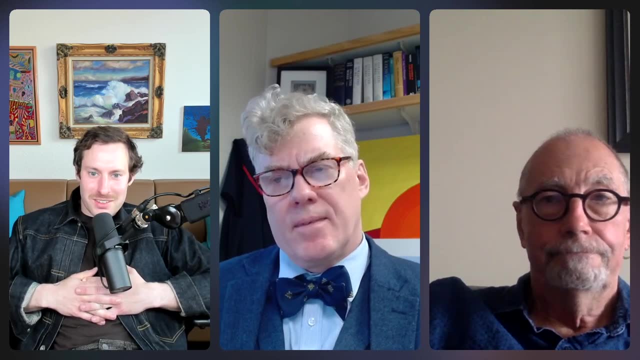 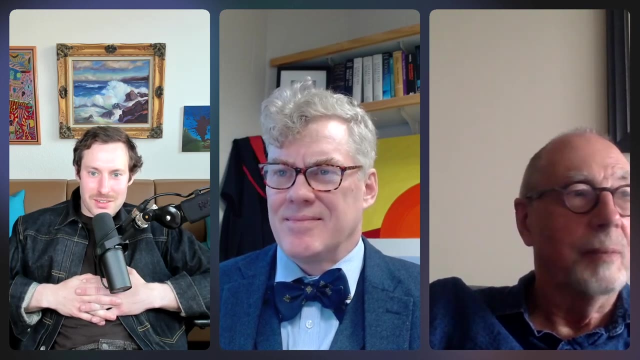 as far as I can summarize it in a nutshell, is it Graham? I'm just curious. where does the UNO come from in the title? Where does it come from, Yeah, or what does it correspond to American? what do you call it? 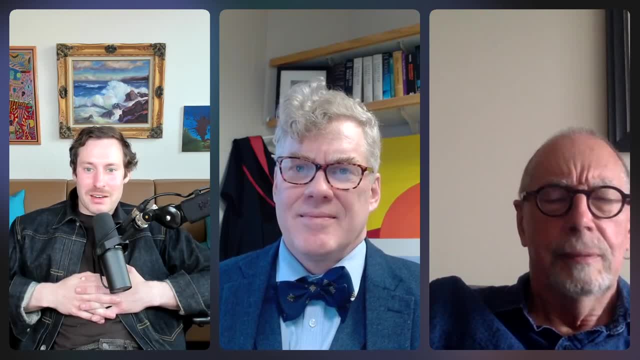 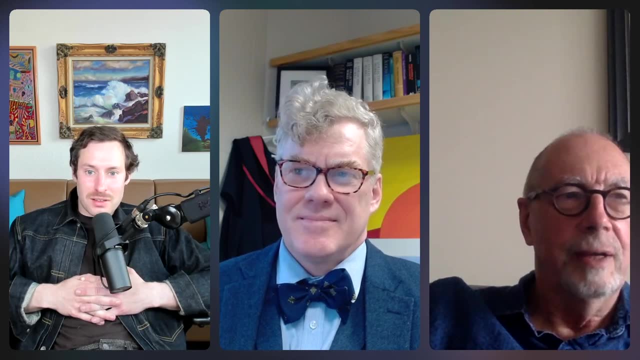 No, no, no, I mean pluribus unum, No, but I mean. what does it? why is that the title of your book? I don't know. No, I don't know, Because it bends the American. what do you call these things? 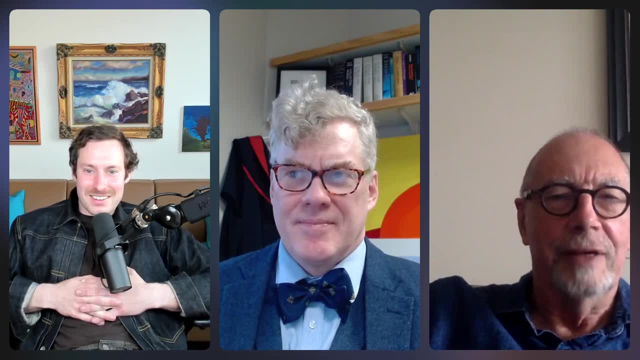 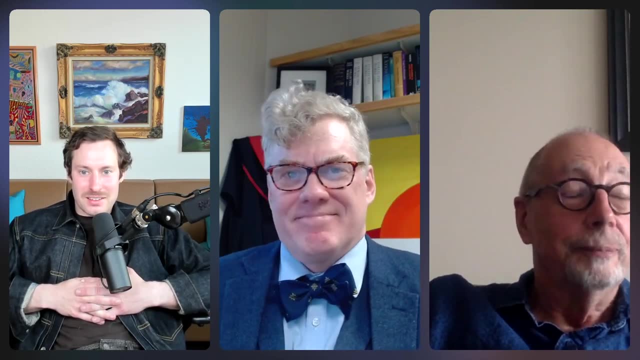 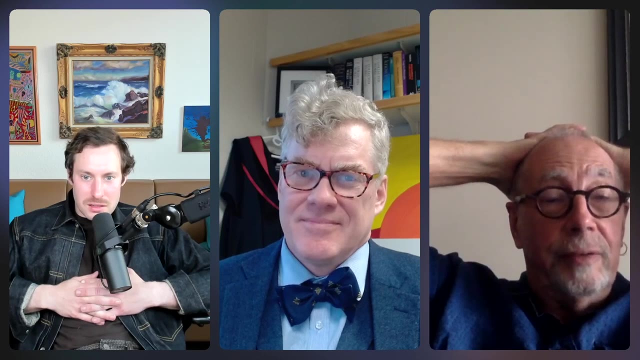 It has more status than that right. It's the official slogan of the United States: Pluribus unum. Okay, But the first chapter of that book explains how studies and foundations actually led us, which is based on some kind of mathematical monism. traditionally, that's been the great. 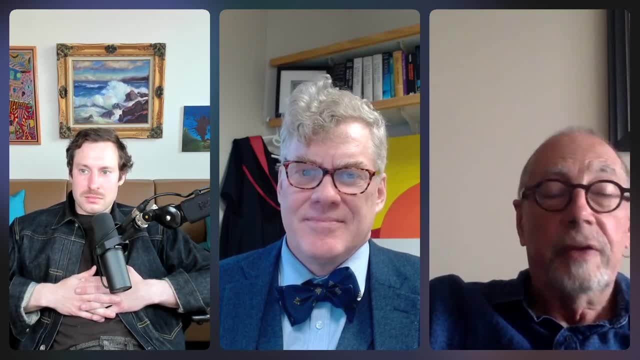 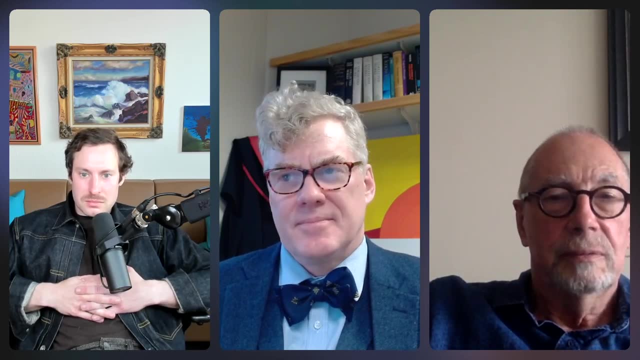 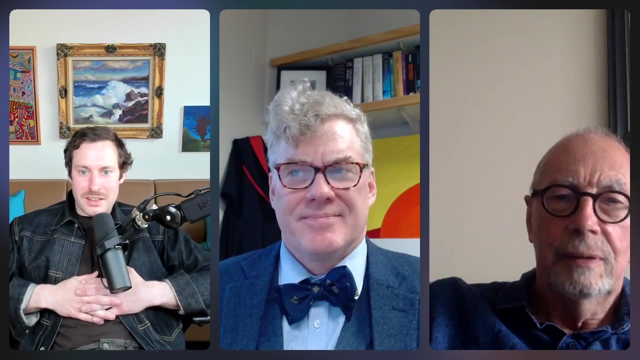 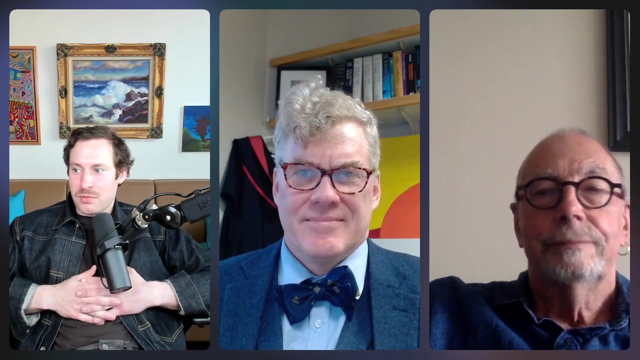 view Um 12.88 trailers. foundational studies have led us to this plurality. um, so, actually no pluralism from one in foundational studies, we got to a many. is that what you're asking? yeah, yeah, yeah, that's what i'm asking. okay, and now i i'd like to talk a bit about, i mean, some philosophers. 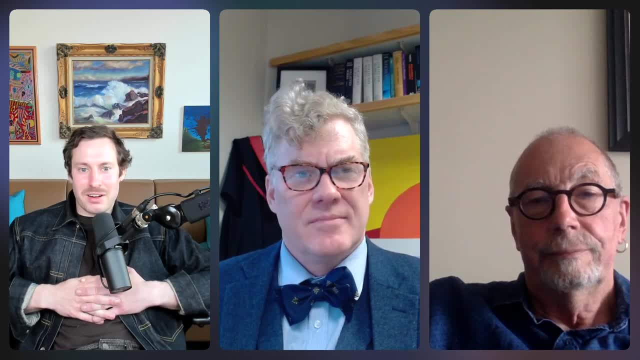 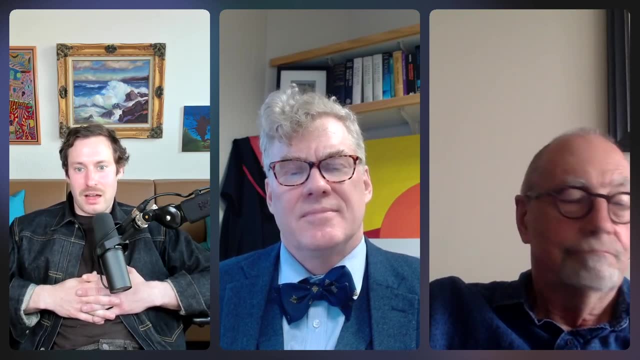 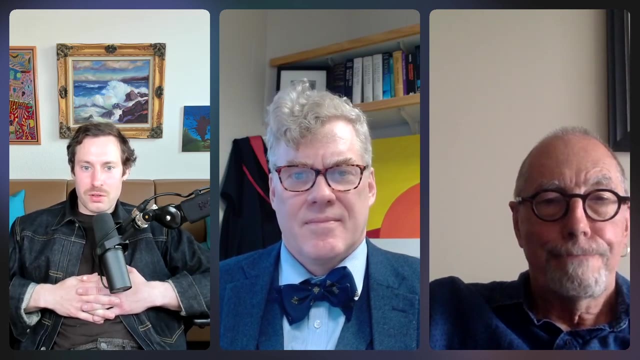 mathematics. uh, heim, for one really doesn't think that there's any place for talking about metaphysics at all in talking about the philosophy of math. but i think the questions are still really important and because they're natural questions to ask, and i also wonder if you two have different 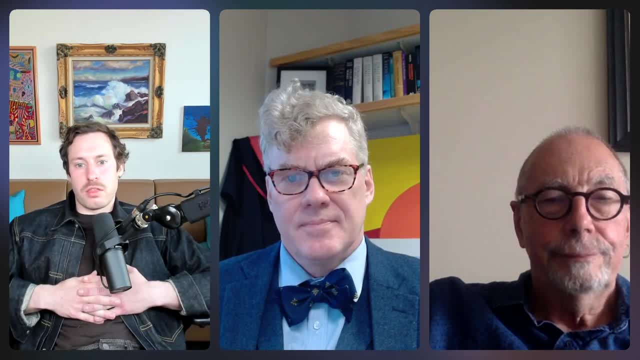 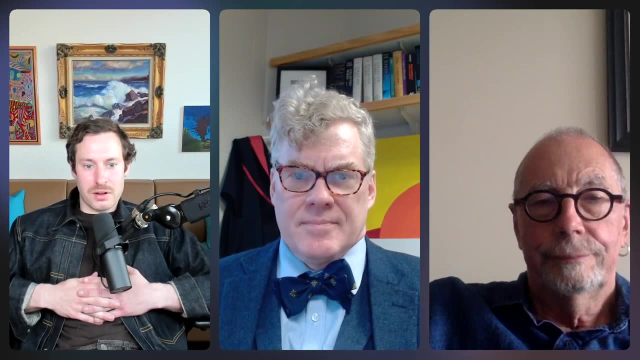 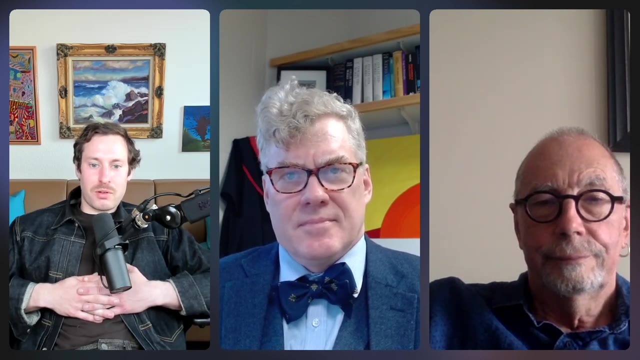 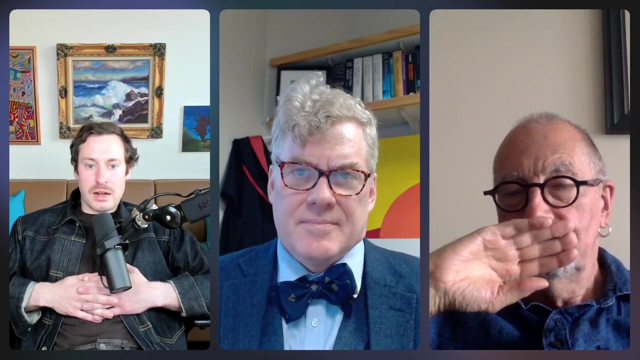 metaphysical conceptions of what the multiverse view amounts to. and one reason why i have this guess or hunch, is that joel in in the paper, in the set theoretic multiverse, you write. i'll quote you: the multiverse view is one of higher order realism, platonism about universes, and i defend it as a 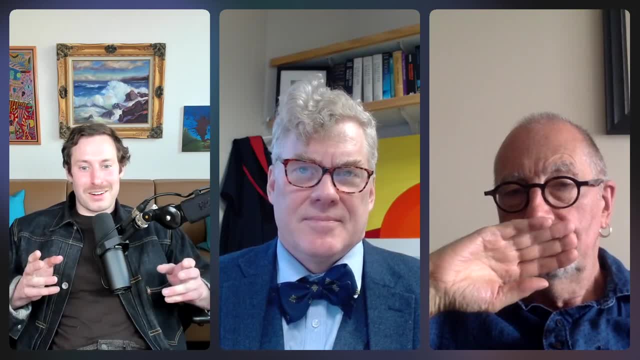 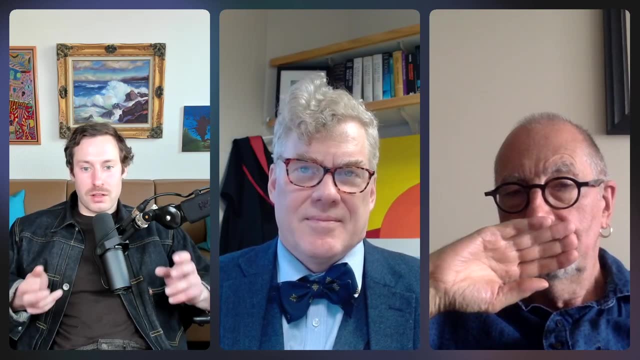 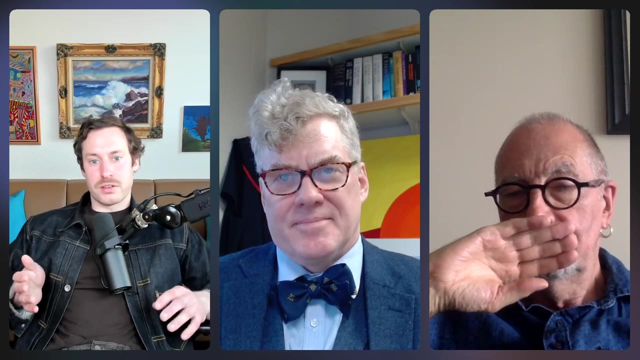 realist position, asserting- and this is the key phrase here- actual existence of the alternative set theoretic universes into which our mathematical tools have allowed us to glimpse, and i mean. the reason that i'm expecting there to be some divergence on your views here is that graham has 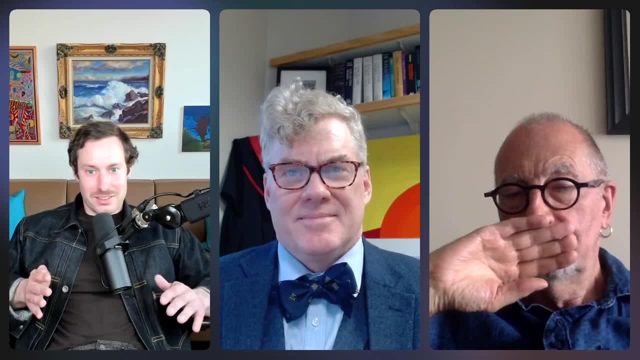 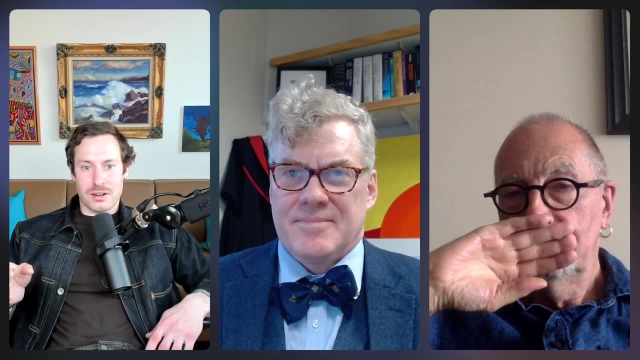 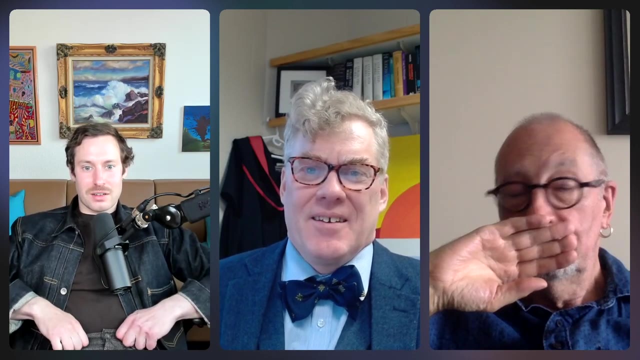 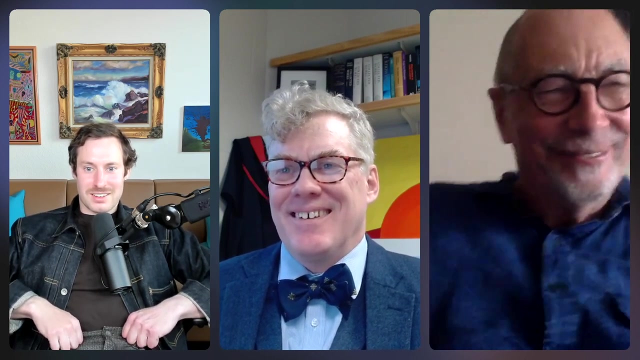 been very clear on this, so it might just be a verbal issue here, but i wonder if there's something deeper than that. and uh, yeah, do you want to go first, graham? um, i don't mind, joel, do you want to go first? i'm happy either way. yeah, whatever you want, all right. so i mean a question. i. 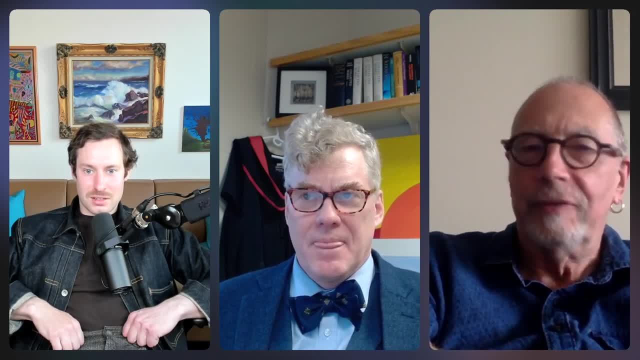 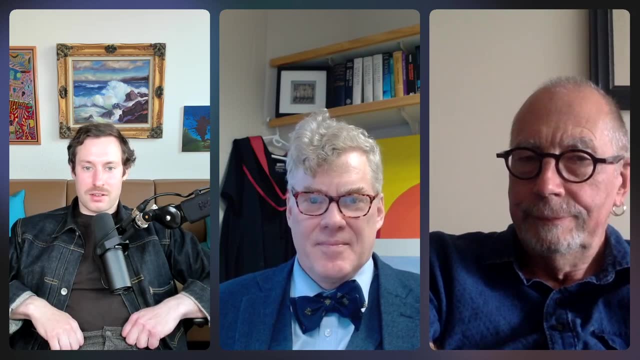 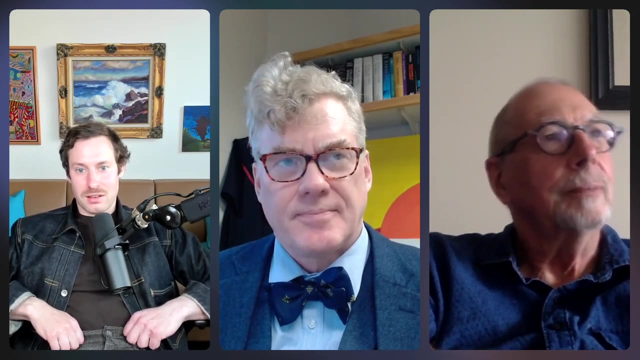 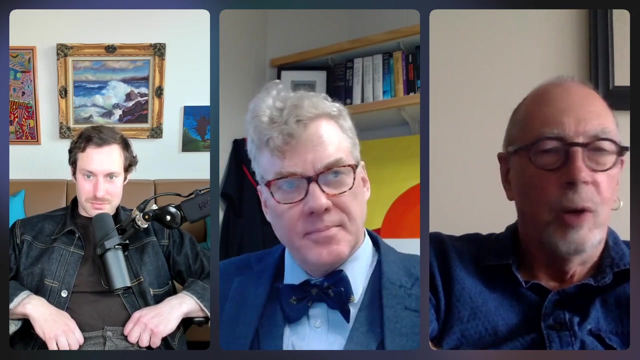 would ask you: uh, robinson, uh is what you mean by metaphysics to begin with? sure, i- i suppose i have ontology in mind- just what exists, what it means to exist, how things exist, yeah, okay, um, so you're, by ontology, you mean what exists and you don't necessarily mean what objects. 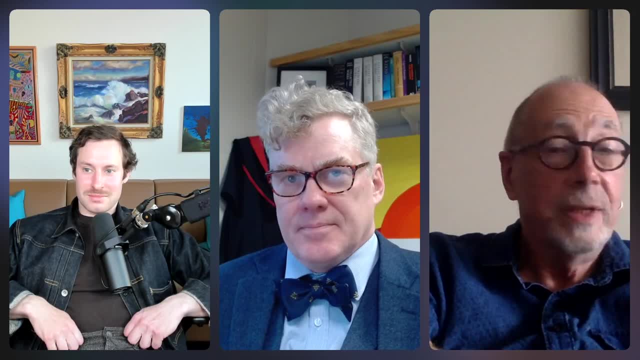 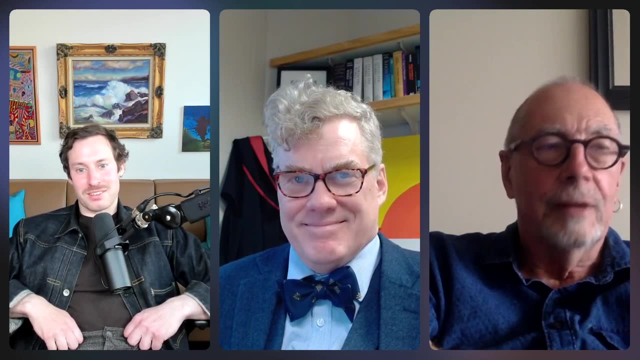 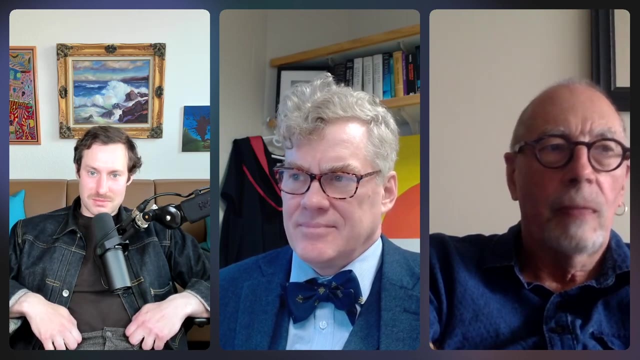 are there. these don't mean the same thing. yeah, i know that you've stressed that, but maybe i mean both, both aspects of the question. well, look, there's a prime question here about what you mean by existence, um, and you can use the word in different ways, of course, but there's an obvious sense in which 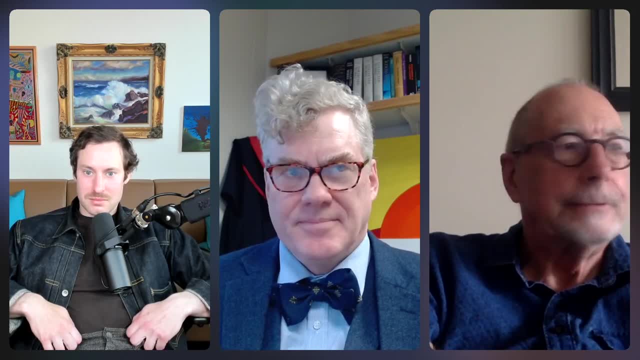 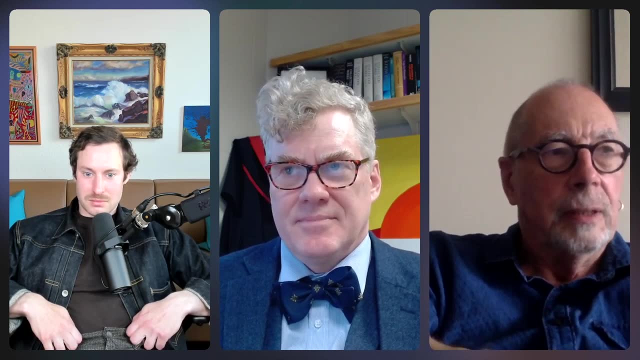 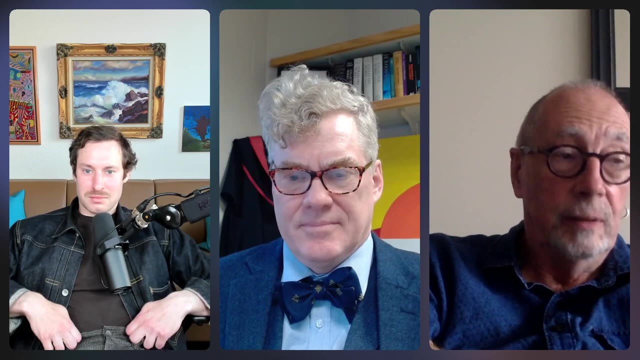 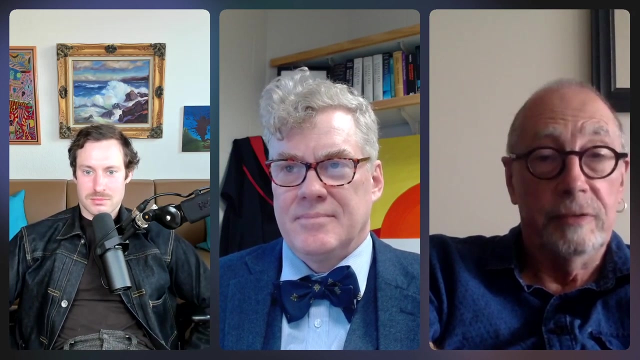 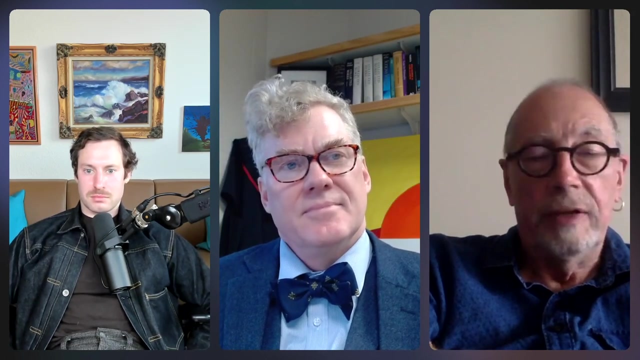 charlotte combs does not exist. okay, whatever that sense of existence is, i think that some things don't exist. um, there is a question that actually goes back a long way in philosophy as to whether mathematical, pure mathematical structures exist or not. um, and people, especially under the influence of quine, have assumed that anything that you quantify over 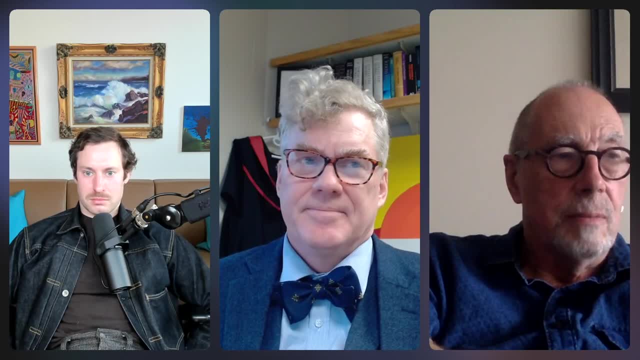 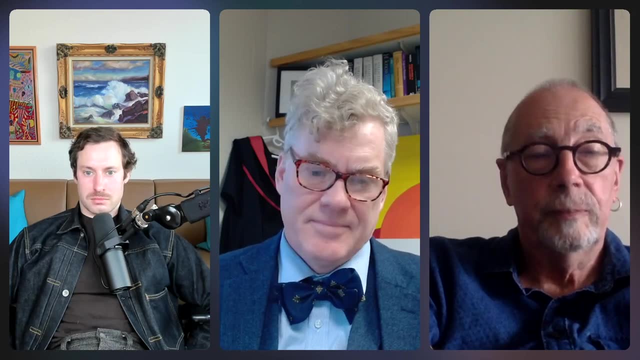 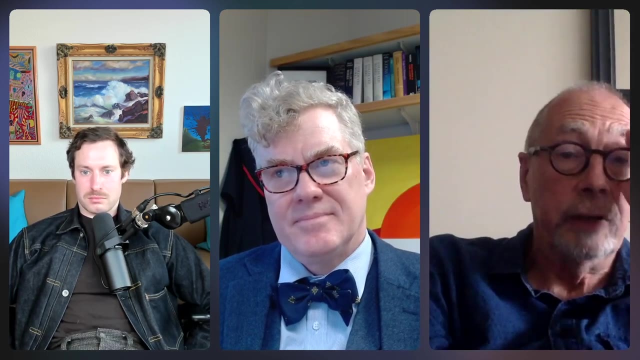 exists. um, i don't subscribe to that view. i think that some things you can quantify over don't exist, such as charlotte combs. um, even if you accept that distinction that some things don't exist, there's a second question of whether you take pure mathematical entities to exist or to be non-existent objects. this ain't. 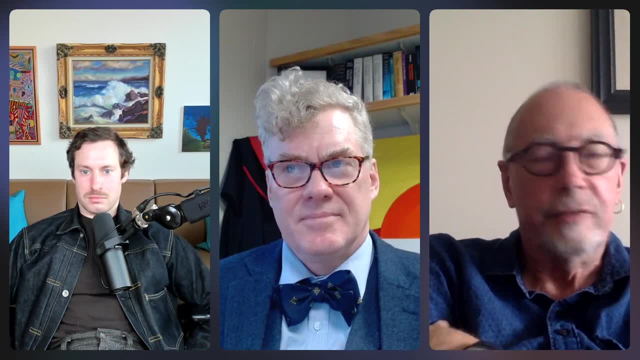 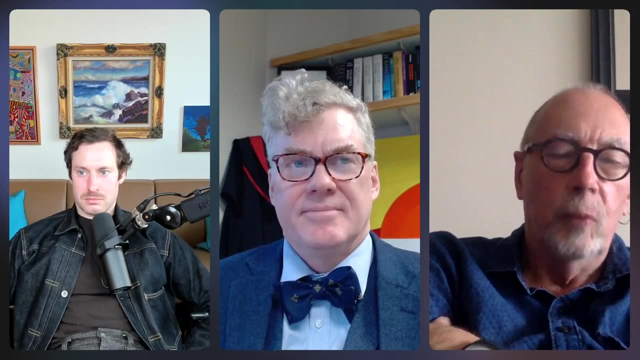 going to make any idea of difference to the mathematics right. it's a philosophical spin you put on the subject matter you're investigating. but for what it's worth, i'm inclined to think of existence in the form of a mathematical entity and i'm inclined to think of existence in the form of. 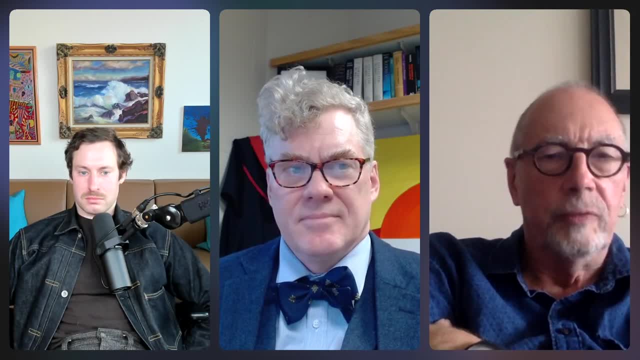 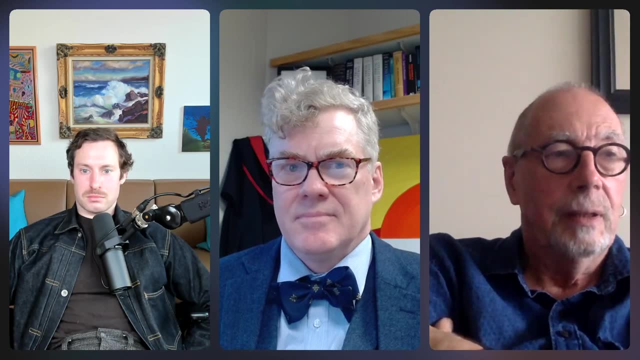 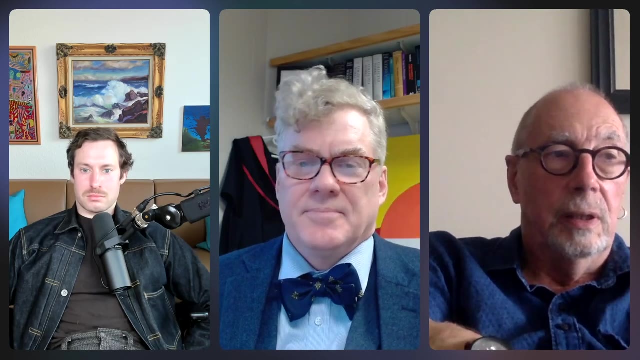 the sense that i'm talking about as being in the causal domain, being in space and time and being able to enter into causal chains, that kind of thing. um- and in that sense i take abstract mathematical objects between non-existent objects- um, i think joel normally expresses himself in terms 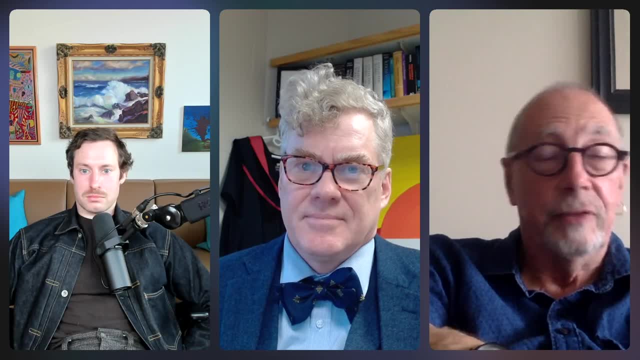 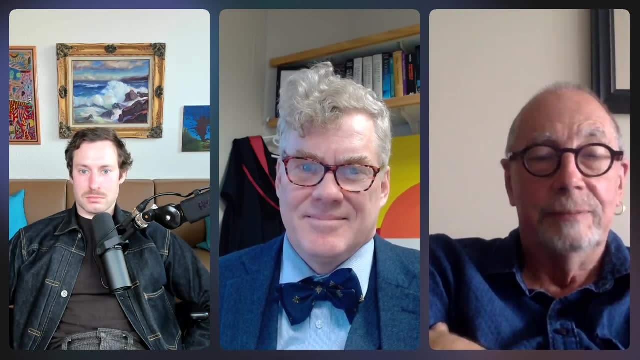 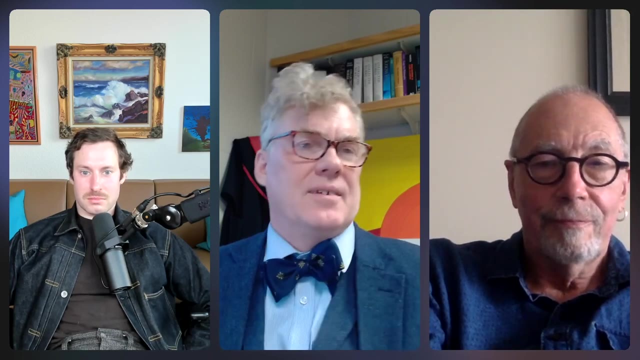 of their will exist. but i don't know whether it's because he has a line on existence or whether he just takes over the standard, you know way of expressing himself in mathematics, philosophy. but okay, over to you, joel. you can say: right, so i have. i think we, we have a, maybe a big disagreement here. 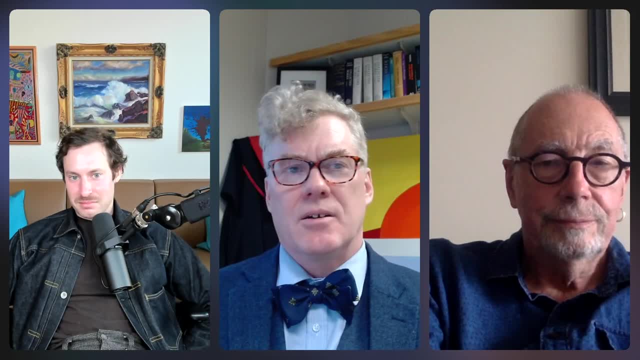 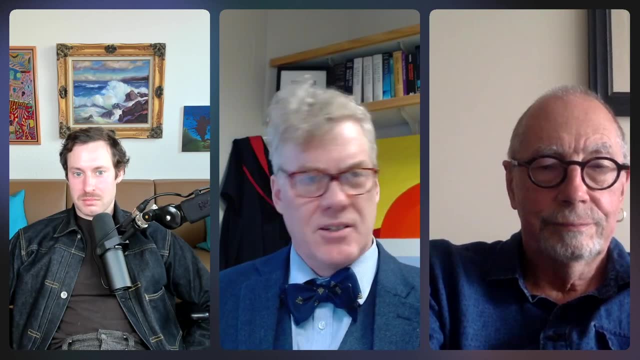 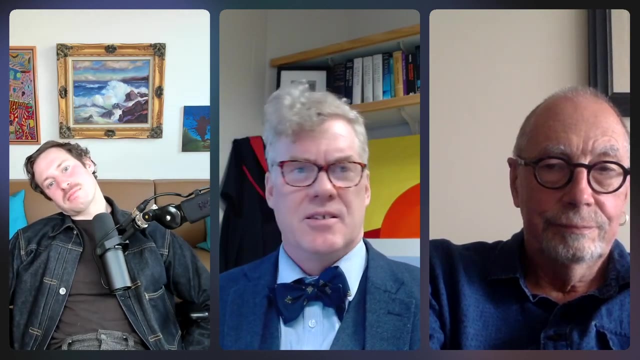 right, my views on abstract existence are complicated, but let me relate a story. last a few weeks ago, here at notre dame, we had a philosophy lunch and the discussion proceeded with um somebody talking about the way they talk about santa claus to their children and so on. you know, based on the sort of santa claus as a fictional character. so they 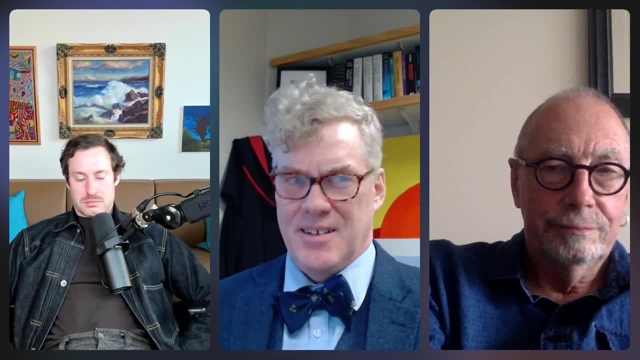 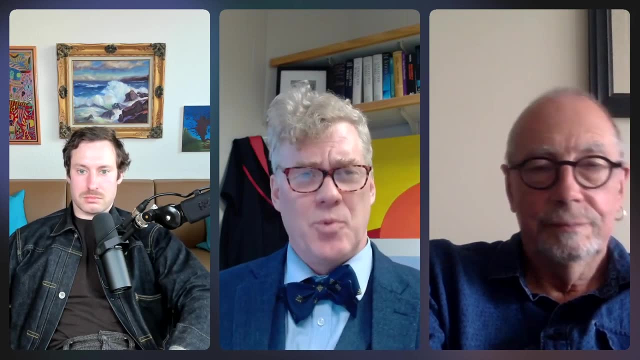 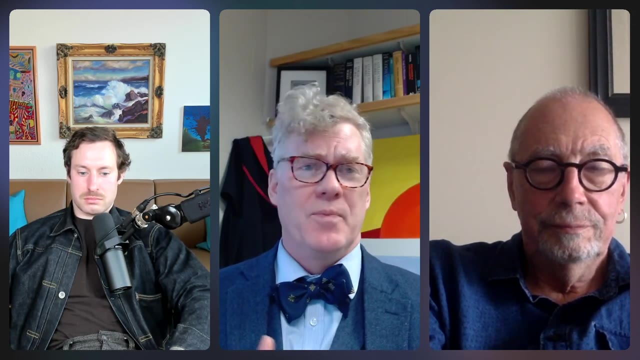 answer all questions, with the idea of answering questions about santa claus based on the story that's surrounding him and then someone else brought up. well, suppose we want to make assertions about not santa claus but santa bear, who, according to the person who brought this up, uh, isn't even a fictional character. 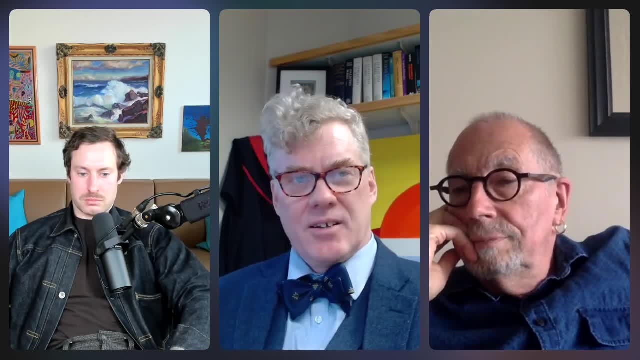 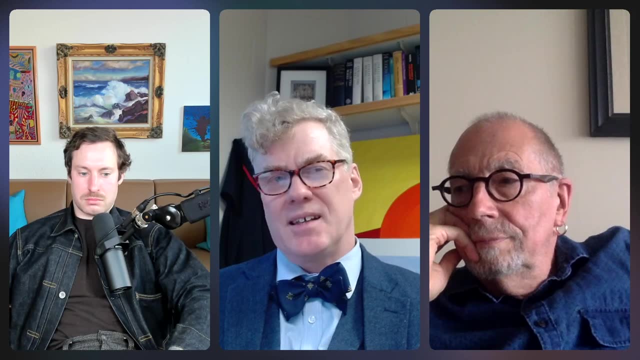 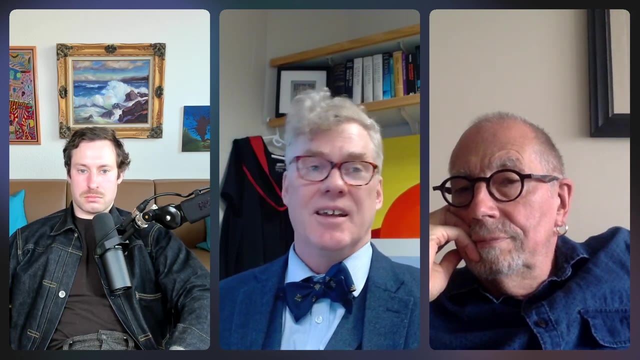 um, and so doesn't even exist, you know, on the grounds of fictionalism, um. and i immediately objected and said: look the the abstract existence, the status of existence of santa bear and santa claus is really not that different at all. and furthermore, beethoven's 10th symphony and his 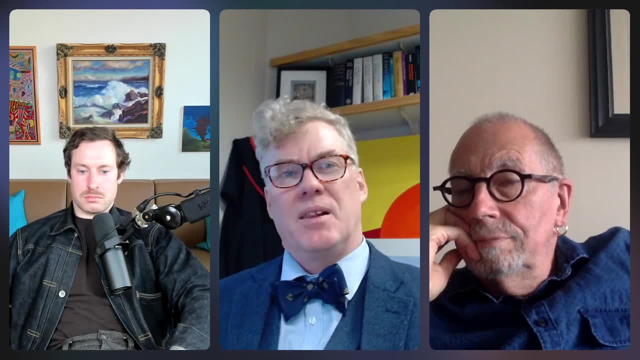 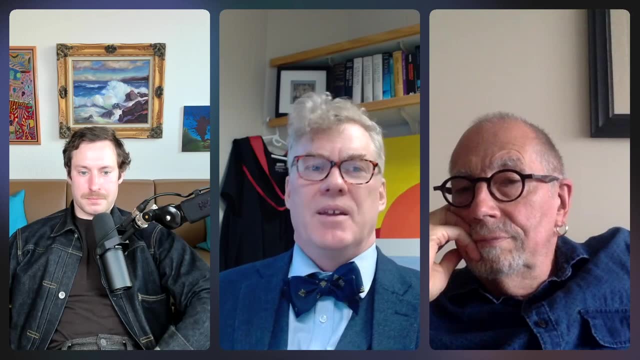 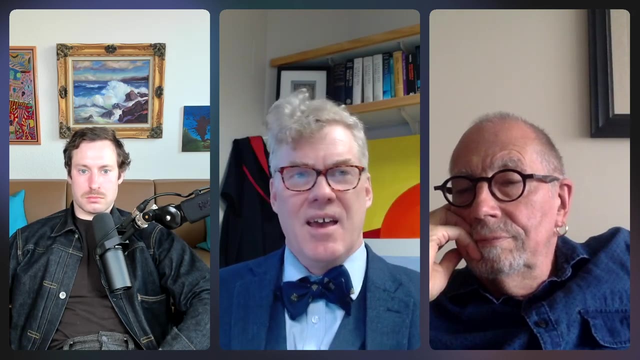 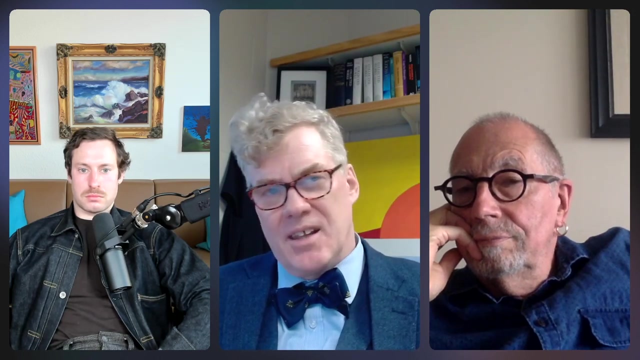 27th symphony and philip burghardt's 20th symphony. and again, you know, here in the exam he's not just a personal character. you know he's got some kind of storyline that he can have meaning, and yet he has no real kind of driving force. Hes a very straightforward. 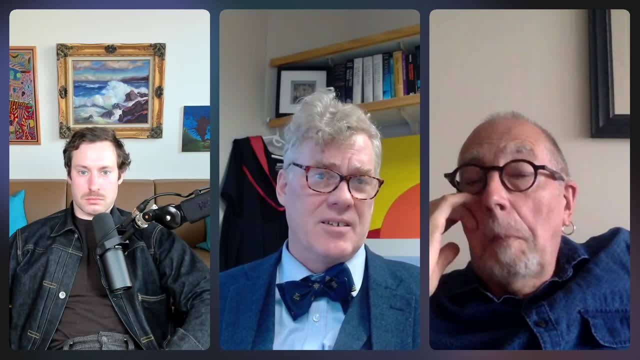 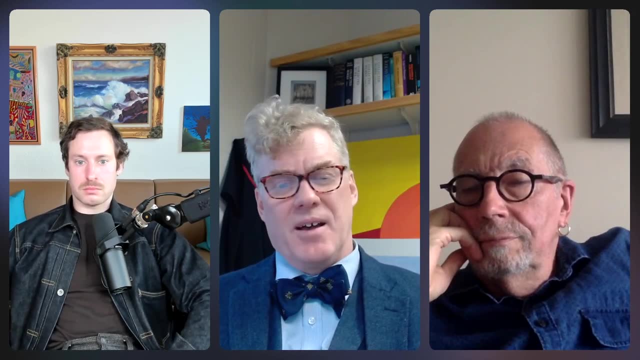 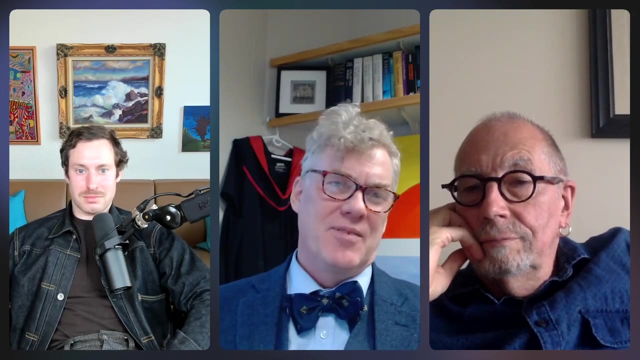 as an abstract object, or Santa bear and Santa Claus and so on, and this is this view. is so I was. I was sort of criticized by um Sam Newlands who said: look, I didn't know that you had such. he accused me of having radical metaphysical views about this kind of existence. but I think 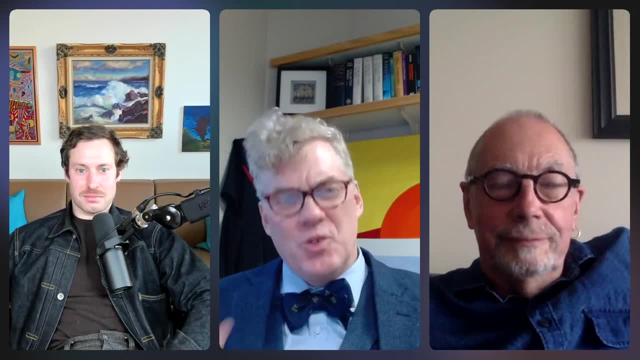 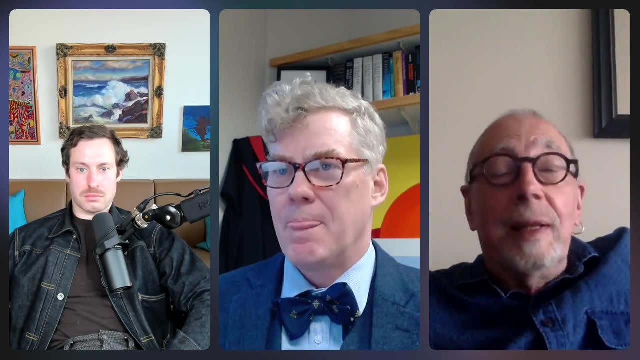 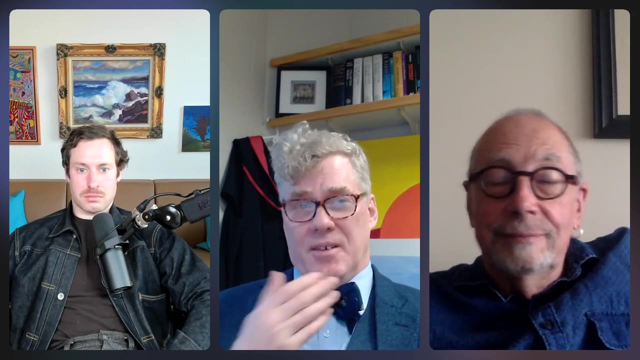 of it as kind of ordinary, I mean, and and furthermore, though, I want to make the main point, which is that, in my view, let me just say that, before you do that, let me just say that we're on the same page here, I agree, okay, great, so the the. the next point, though, I think, is where we're. 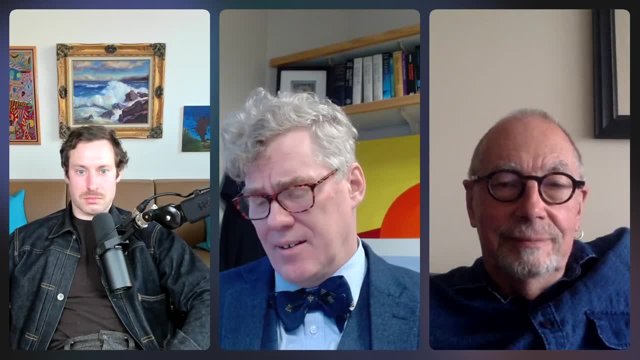 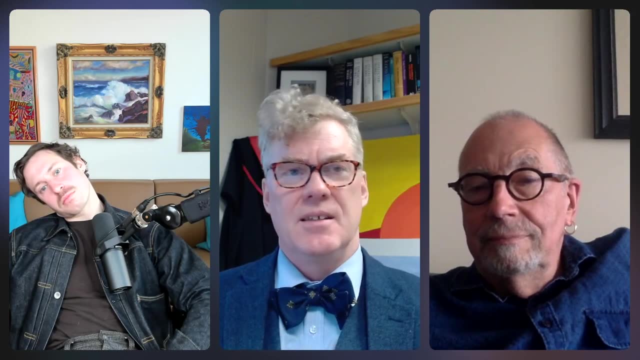 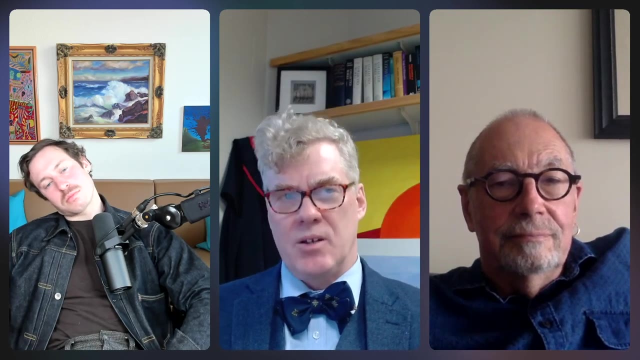 going to maybe disagree, um, which is that, um, people often talk about, you know, existence in space and time and so on, in physical existence, in a manner that suggests that that's the one that we really have to exist in, is the problematic one, and my view is that this is exactly backwards. that 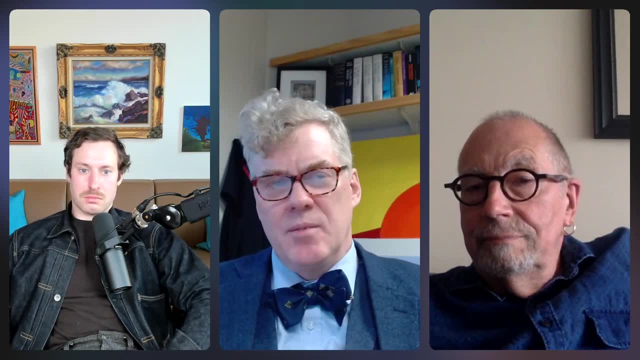 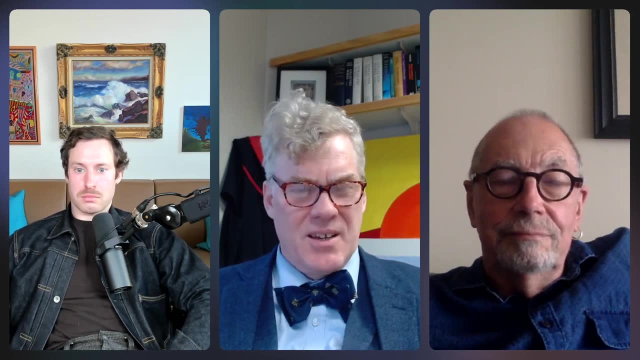 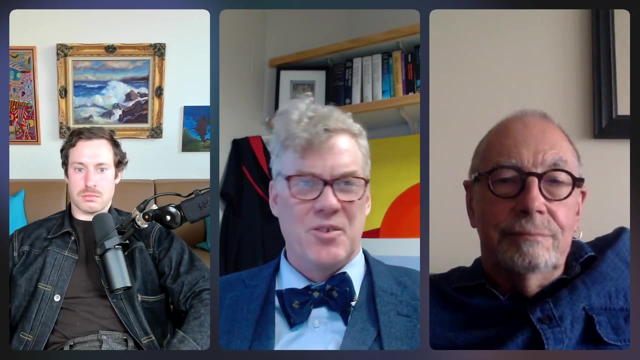 actually physical existence is the one that's deeply mysterious. I mean, the more physics we learn, the more the more strange physical objects are. they, you know, started out as hard balls or something, or infinitely divisible things for the Greeks, or something. but then and now, what, what, what? 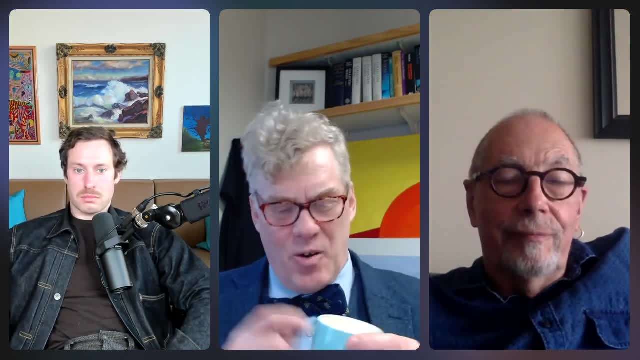 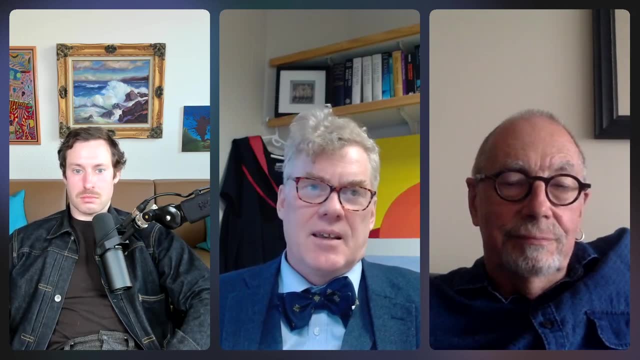 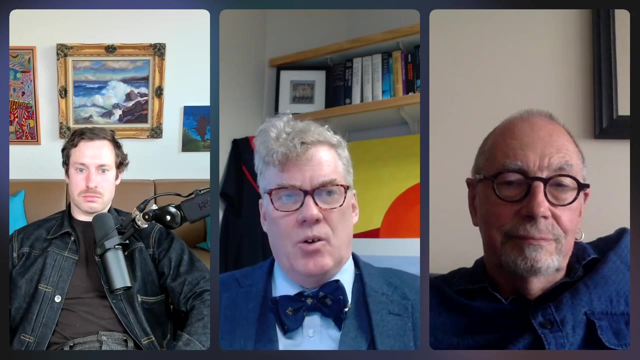 are they? well, even things like this cup right, or you know, clouds of electrons and wave functions and so on, and it's just deeply mysterious what it means to physically exist. in fact, I'm not even sure, actually, one can give any kind of sensible account of what it means to say that a particular thing exists physically. I mean in reality that it 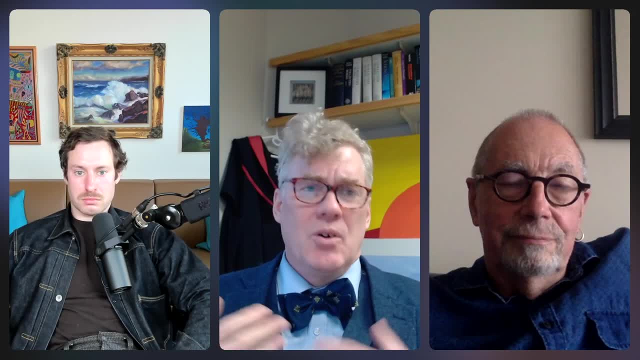 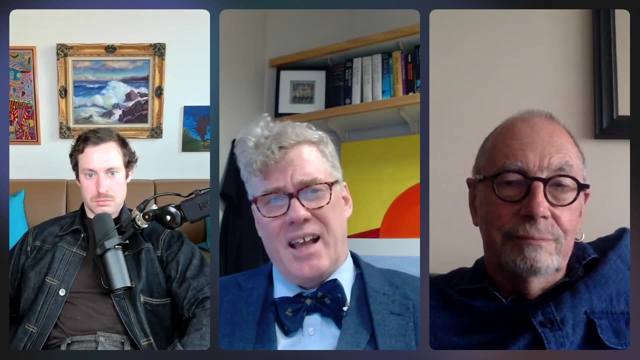 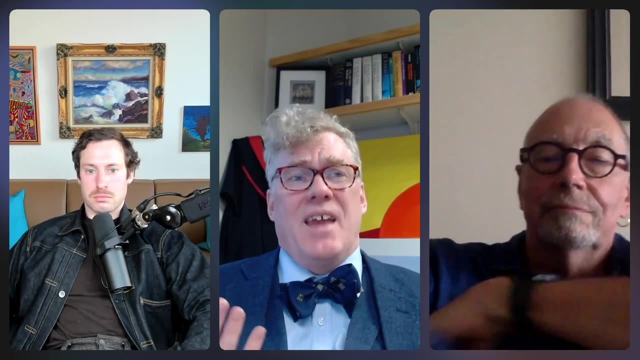 physically exists. I mean, I have a lot of experience. of course I can pound on the table and and, and you know I exist in space and time and I've interacted with many, many things. but that's not really an explanation of what it means to exist in space and time, and I don't think that I can't imagine what. 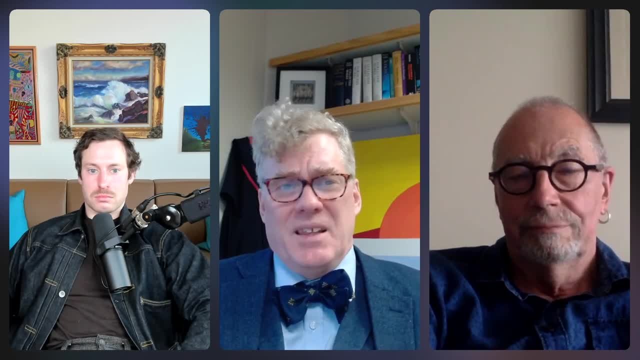 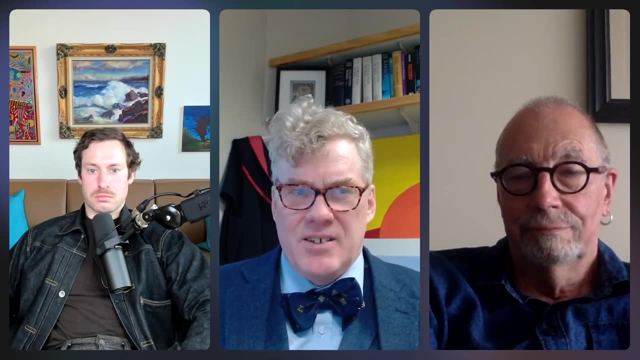 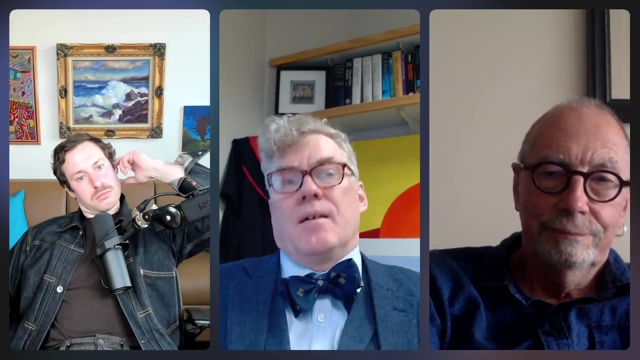 an explanation of the meaning of that would even be like, because, um, it's such a kind of primitive, it's a it's a kind of knowledge situation that we have only this kind of extremely primitive course access to, whereas the existence of the empty set is something that we can seem to. 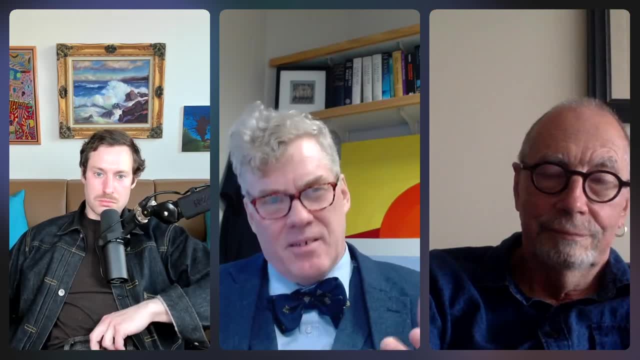 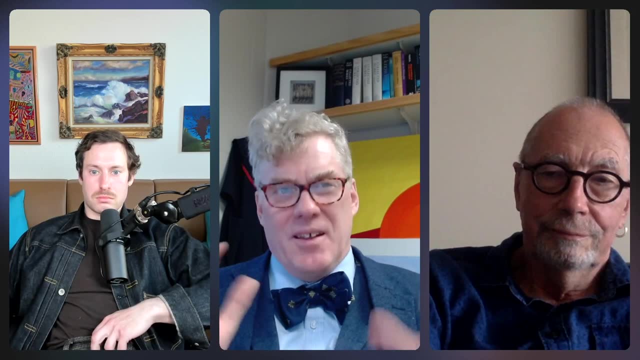 say something about what it means for such a thing to exist, so I can talk about, you know, the instances of contradictory properties, and it's the set of instances of contradictory you know. I mean, you can, of course, argue with me about how successful such an explanation might be, but 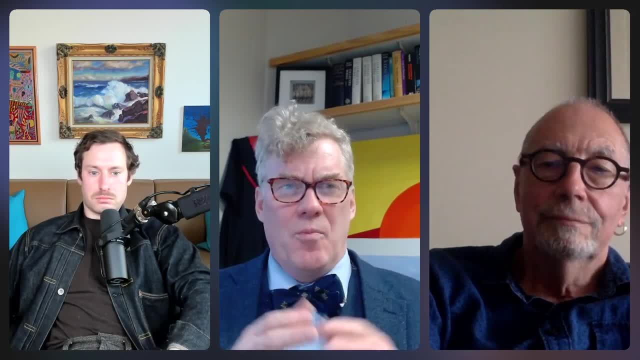 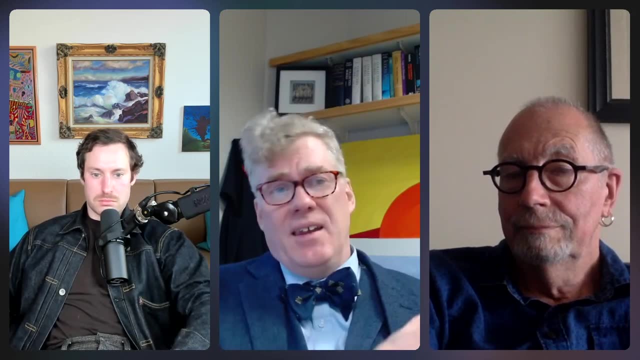 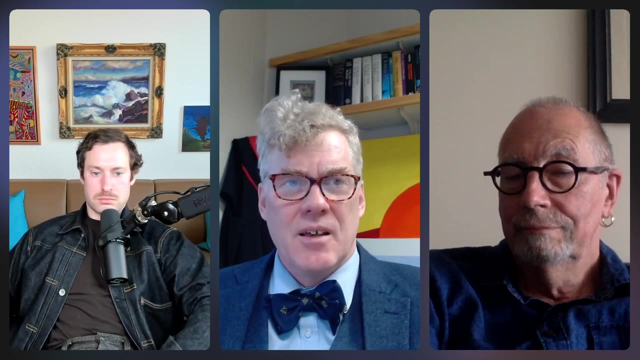 the point I'm trying to make is that that explanation is just far more thorough in giving an account of what it would mean to say that the empty set exists than any kind of corresponding assertion or explanation of what it means say that this cup is a physical object. um, and, and so that's why i think, uh, this, this sort of 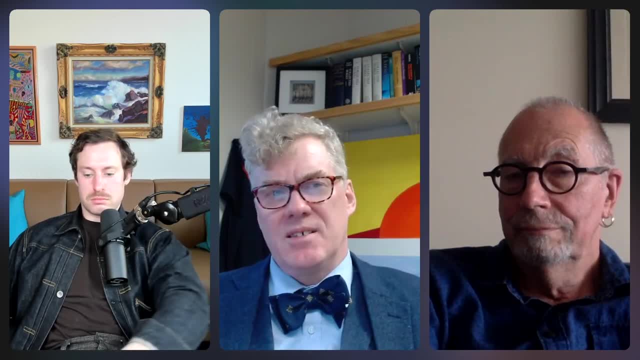 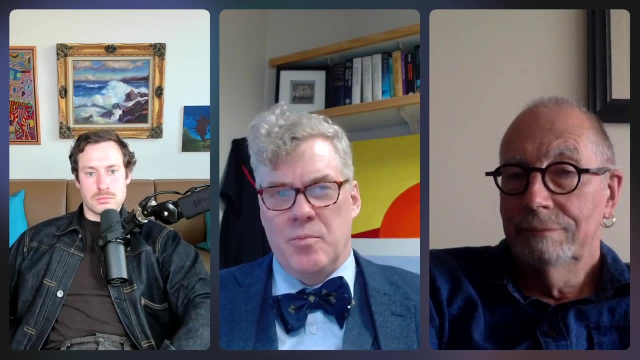 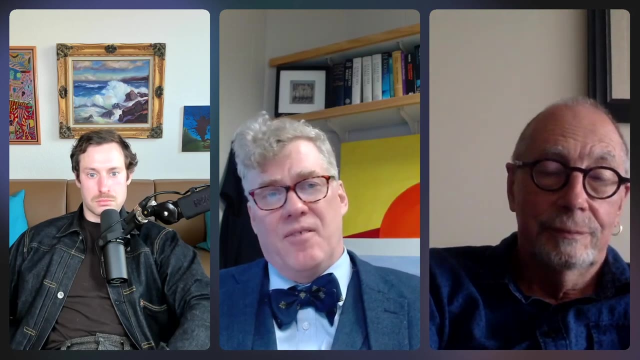 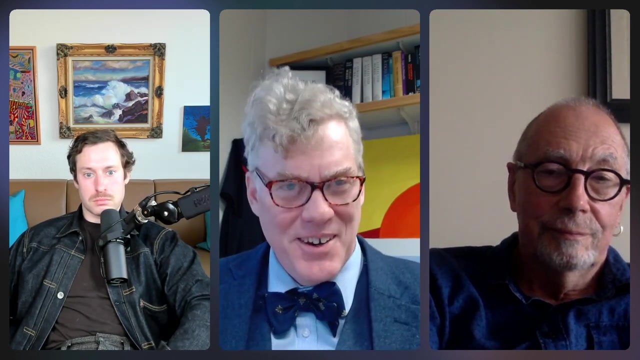 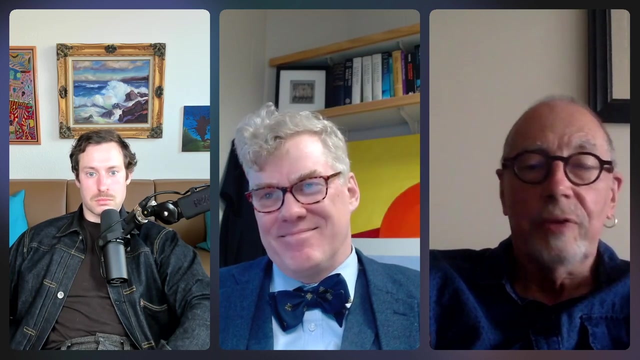 ordinary contrast between physical existence, which is supposedly easy and well understood, versus abstract existence, which is problematic. it's just totally backwards, i think, um, and, and so i'm really willing to have you know, my ontology of, or metaphysics of, abstract objects is quite rich, as i mean my understanding of the nature of it is extremely rich, and so i? i wasn't. my view is: 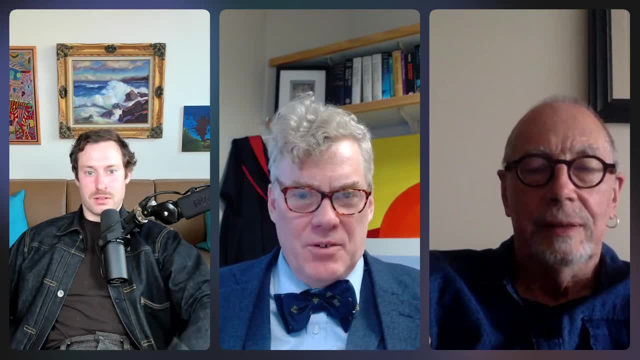 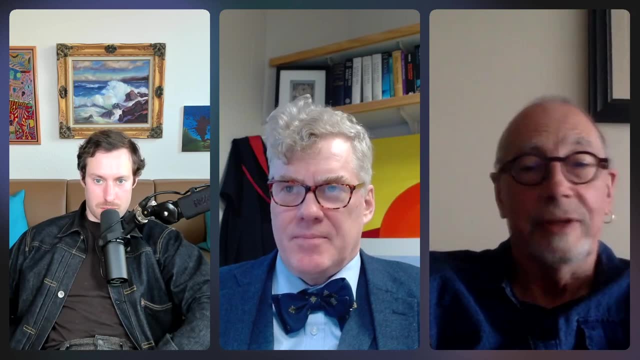 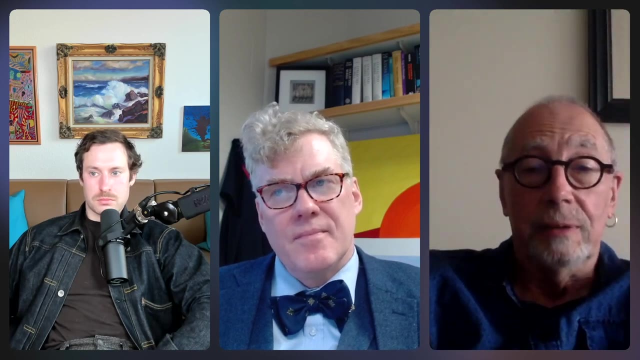 not coming from the thought that existence in space and time is unproblematic. um, i mean, you can use the word exist. i mean anything you like. you know it's something you don't think, so there's a nice knockdown argument for you. um, all i want to know is: well, what do you mean? and i've told you what i mean. um, um, you tell me. 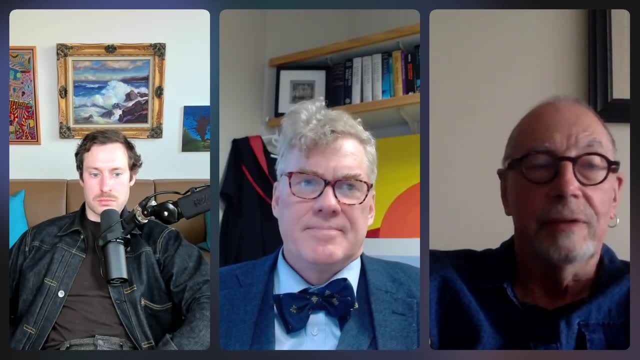 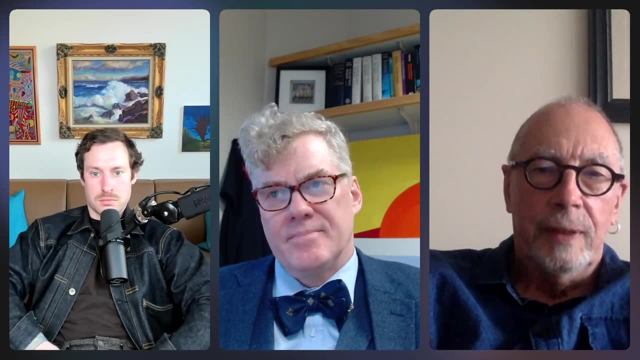 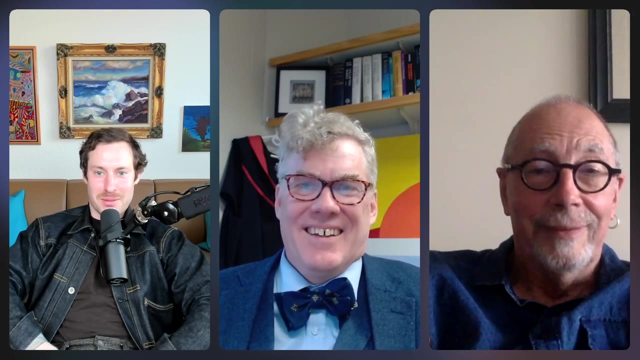 what you mean and we can. if it's different, we can agree to differ about that, um, but there is some sense in which we both agree that show it comes doesn't exist. thank god, now, look, everybody's an atheist right about some. well, joel can't say that he's at notre dame now. well, look, even even the 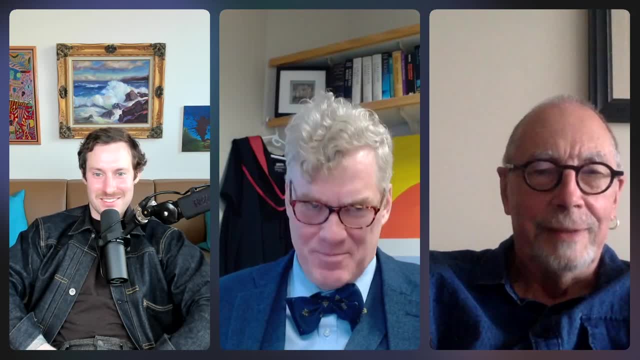 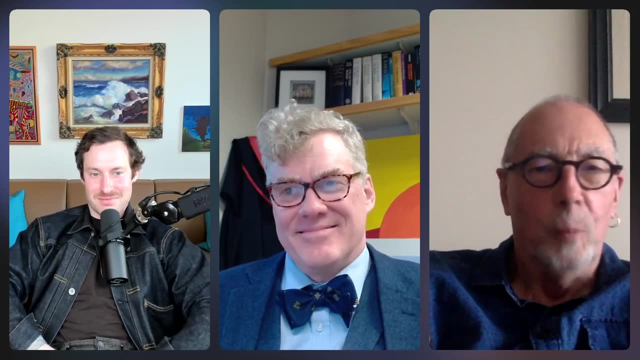 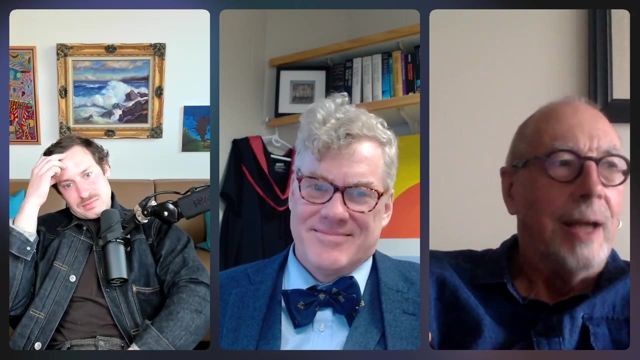 good bishops are not ashamed or atheists about some gods. none of them believes in um ramen, for example. okay, so they might believe that some one particular god exists, but they all think that others don't. all right, so everyone's an atheist about some gods, right, and whatever sense that those gods don't exist in. that's the sense of existence i want to. 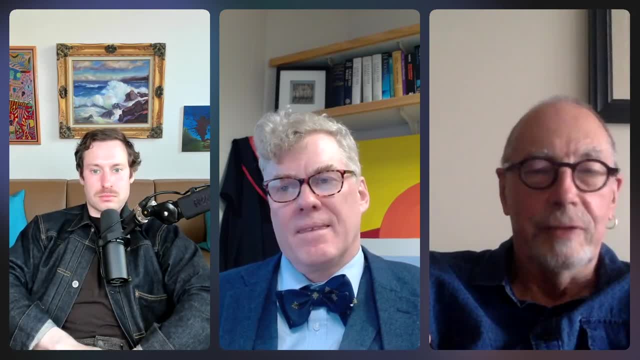 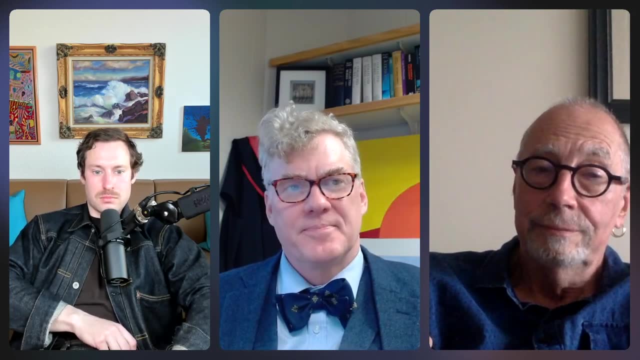 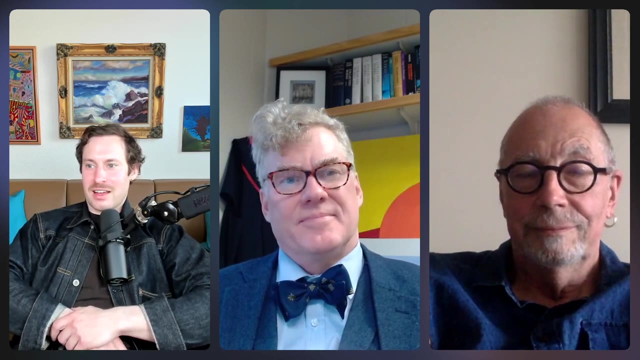 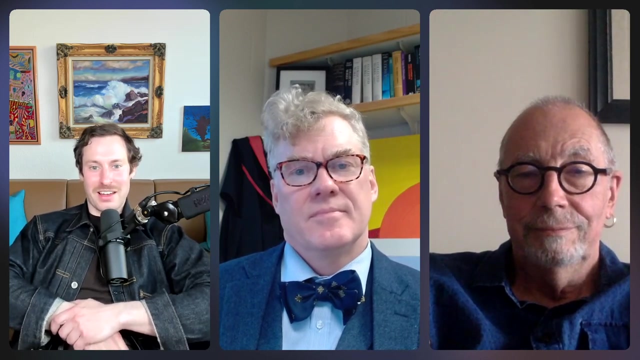 talk about, okay, and i don't see any particular reason to suppose that abstract mathematical objects exist in that sense. now, this is a a question that i think you don't. you don't have to be philosophically initiated into mathematical philosophy to ask. it's a question that i- i mean, i was curious about even in high school. 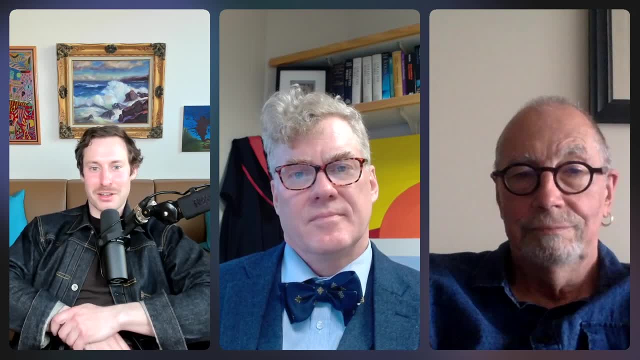 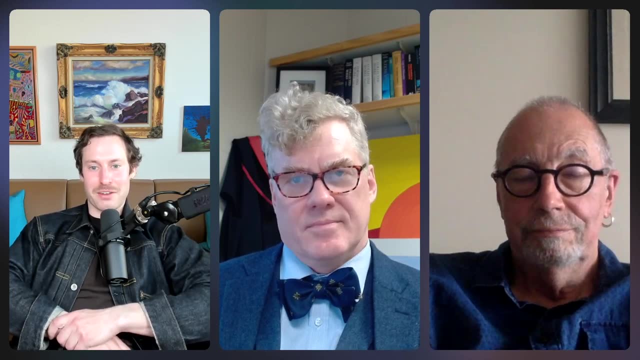 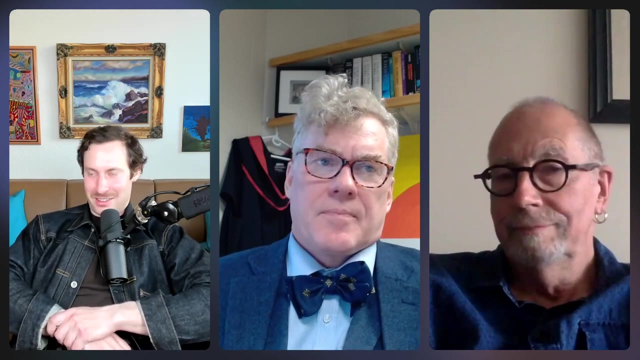 and perhaps you guys will think it's silly. a silly question, uh, but just as uh, graham, you disambiguated my question about metaphysics and i think it's a silly question, uh, but just as i'm sure you two can disambiguate this question, but i would just uh like to ask this classic. 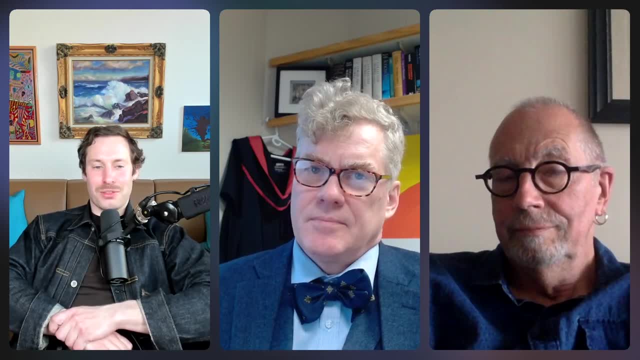 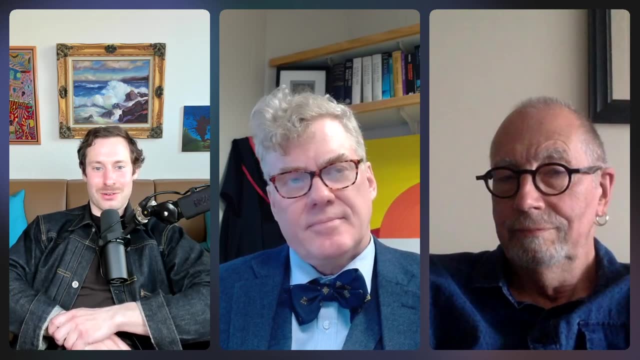 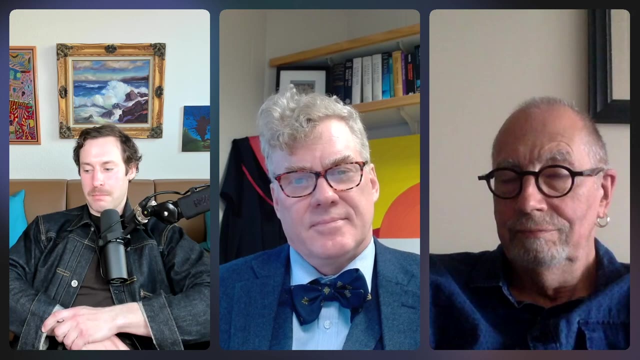 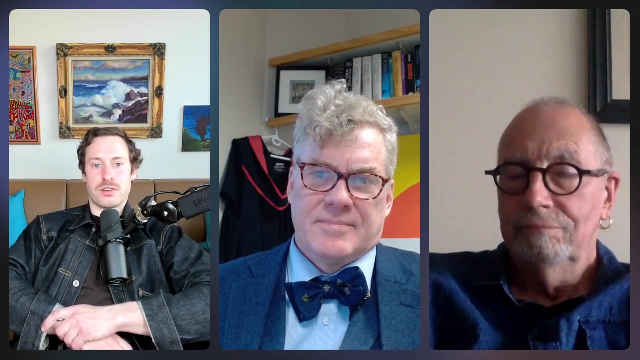 question whether you think of mathematics as created or discovered, because on on joel's case, i mean with his rich ontology of abstract objects, i have to assume that he thinks mathematics is discovered, or at least we discover properties of the set theoretic multiverse. i mean, our tools are things that humans do, so i don't know if it. 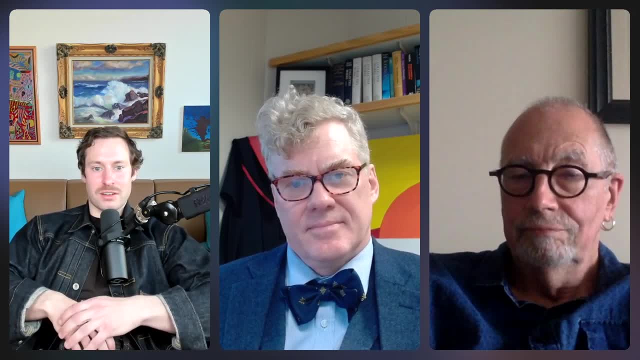 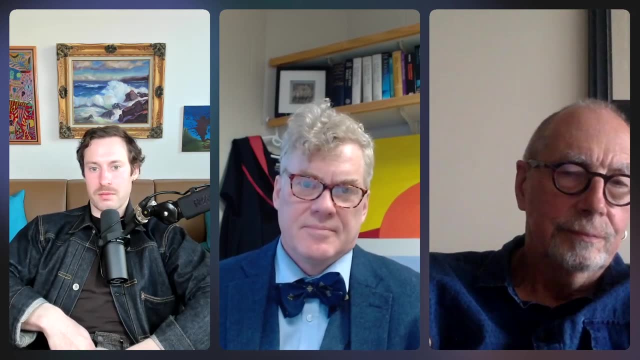 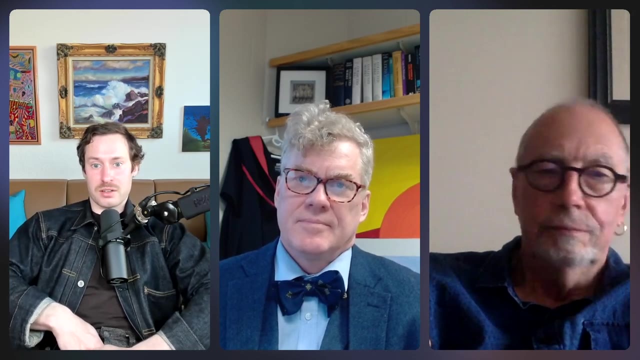 might be a category mistake to say that it's in invented or discovered, but then you, on the other hand, graham likened, you already brought in the analogy of sherlock holmes, and sherlock holmes is is as a non-existent object, is, i think you would like to say that he's created, uh, and if, oh, so you. 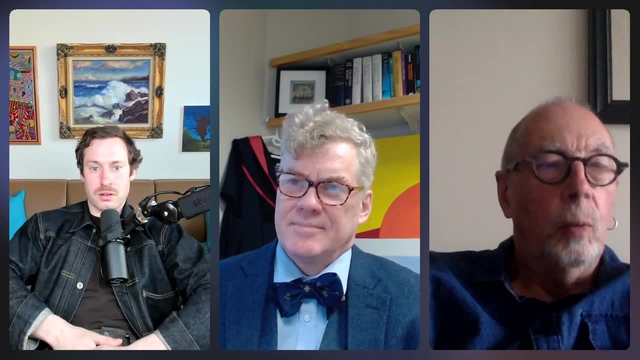 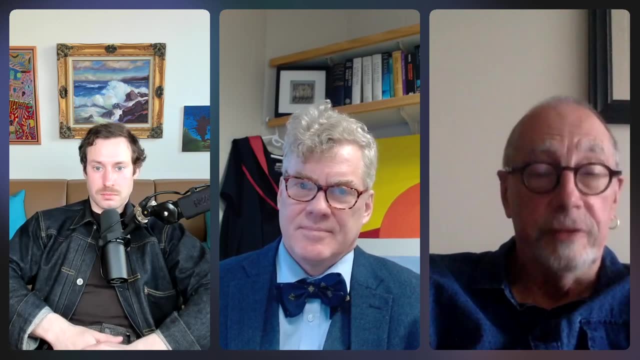 don't okay. so yeah, i'd love to hear how you two think about this question. well look, if you think that some things don't exist, there are two lines. you can run a realist line or an anti-realist line, and you can think that um abstract objects. 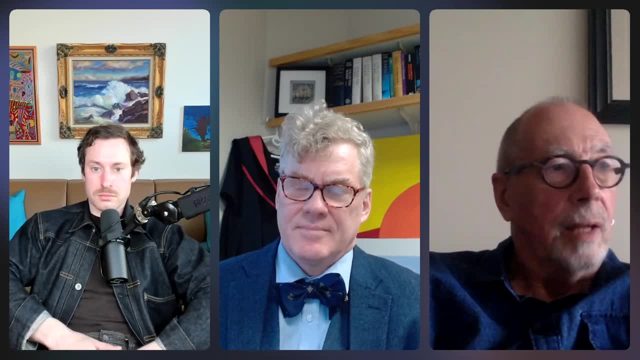 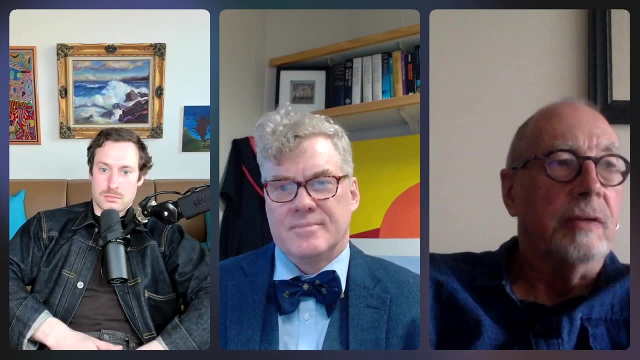 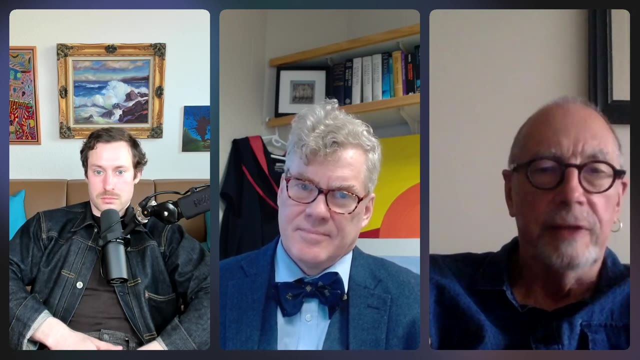 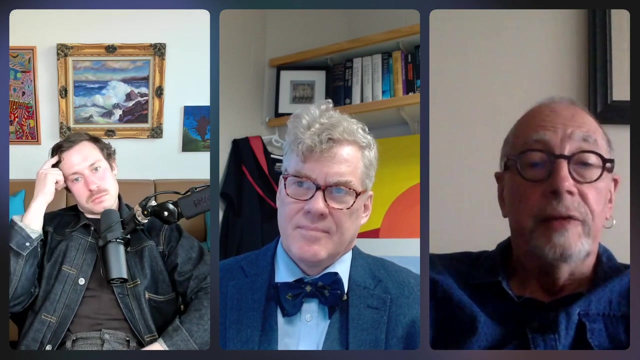 um are there to be quantified over, so to speak. um, or what abstract objects are actually quantified over, depends on the activity of sentient creatures. in that sense, you're an anti-realist. a lot of people are anti-realist about things like sherlock holmes or something. that's one possible view. another possible view is to be a realist. 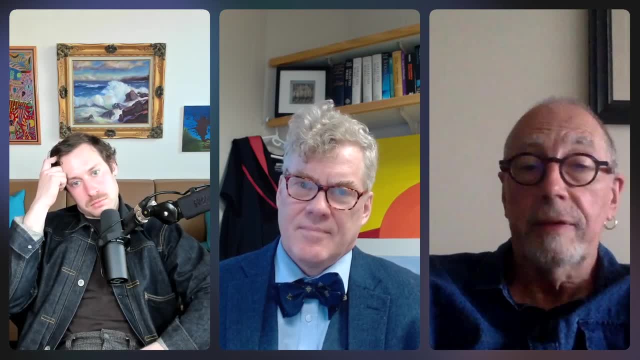 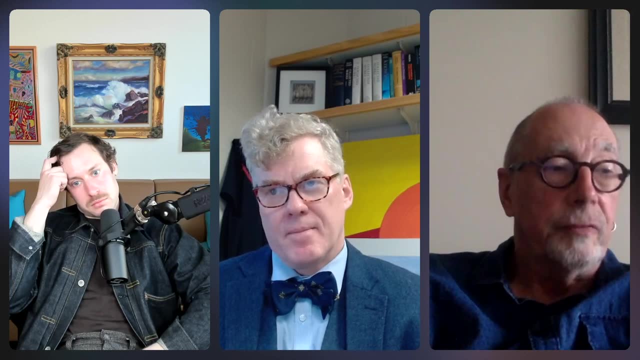 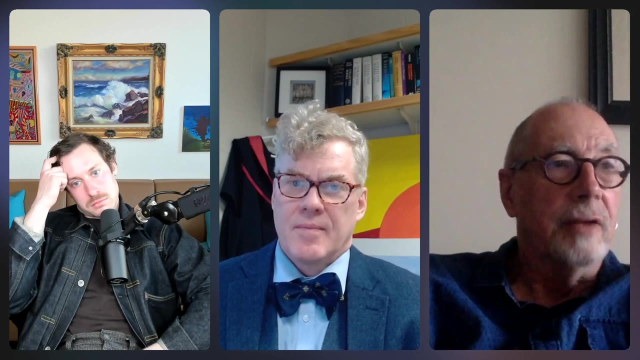 about them. they're there just as much as any other kind of object. um, and in that sense, when conan doyle wrote the sherlock holmes stories, he wasn't creating anything in the sense of bringing the object to the real world, and he wasn't creating anything. 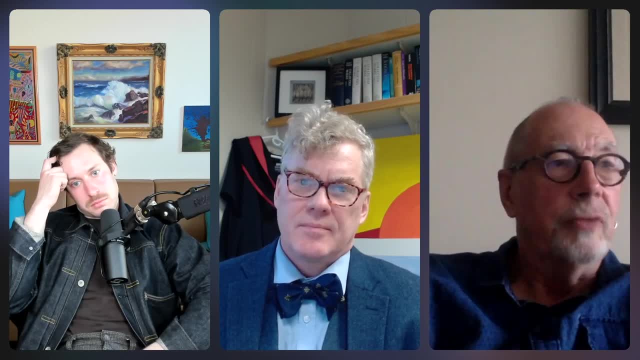 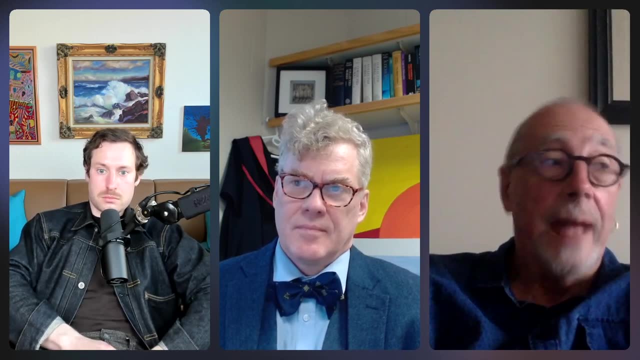 there in whatever sense of there is. rather, he was just singling out one of his objects and giving them a name. now i think you can tell the story either way, but actually i'm more sympathetic towards the realist view, for reasons we can go into a few. 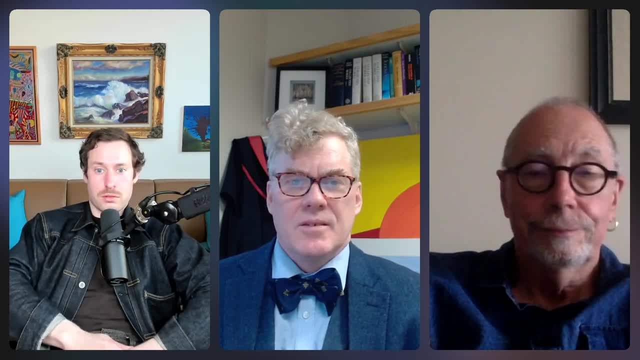 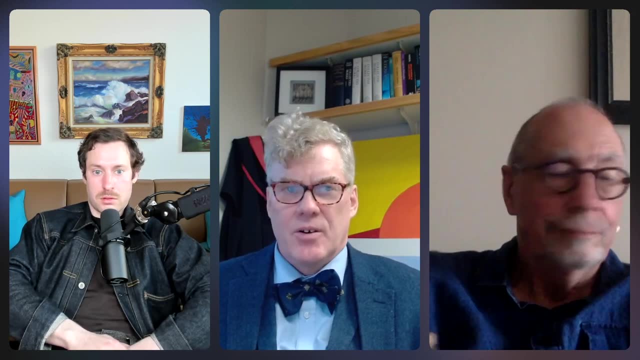 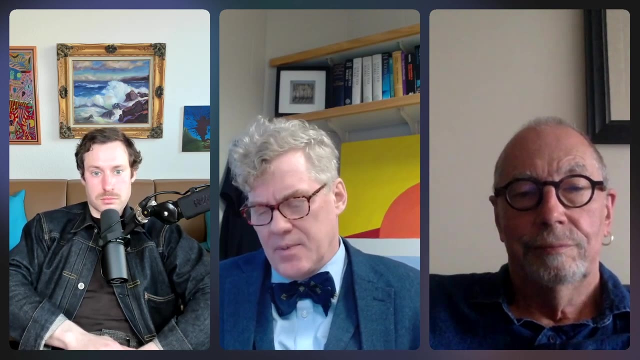 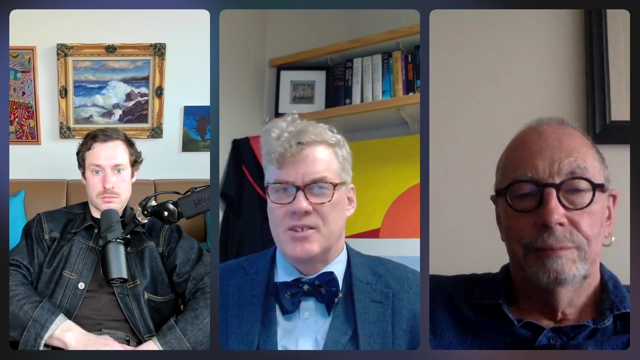 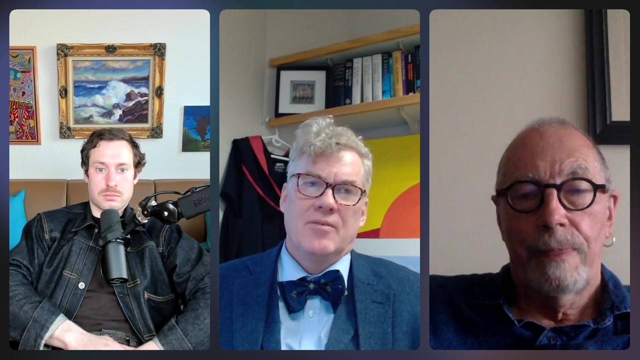 but yeah, go ahead, joe. so so let me respond to what you said about um. i mean, the question is, is mathematics discovered or invented? And my reaction to this question is: of course mathematics isn't so homogeneous to have one answer to this question. I mean, it happens, you know, if one is doing mathematics then very often it has the feeling of discovery. 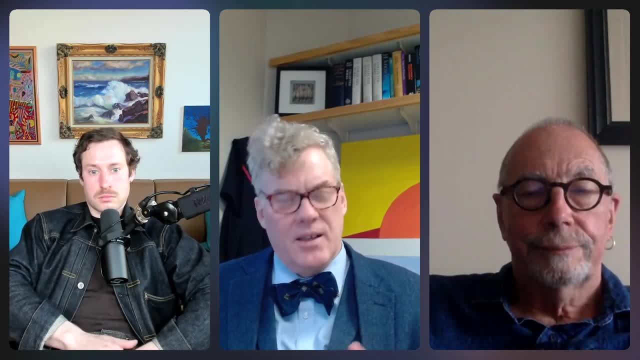 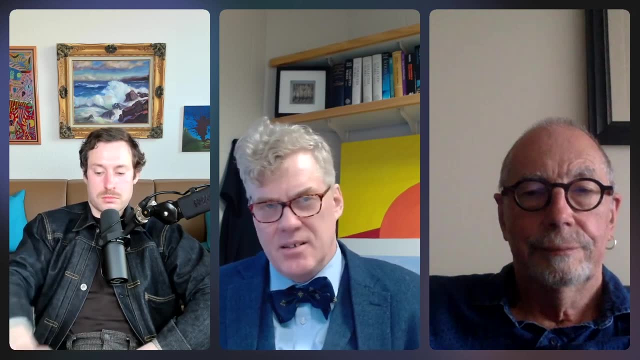 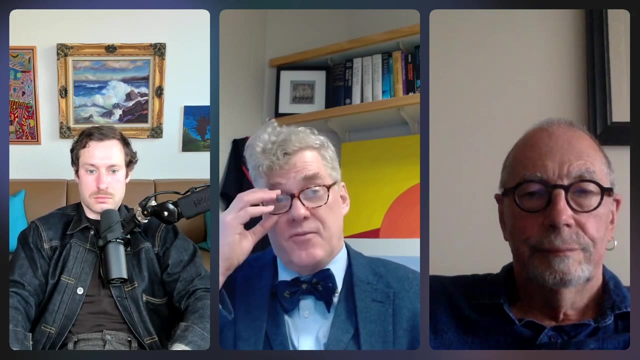 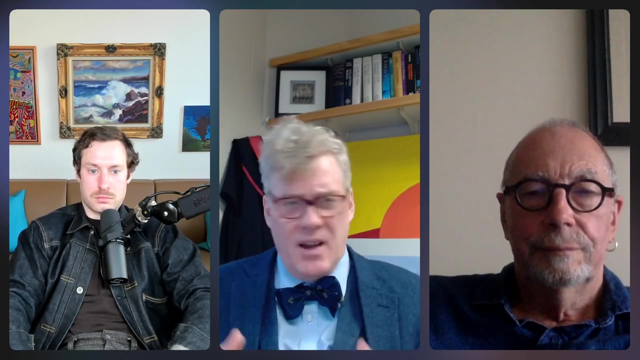 You know, if you're looking at some well-established field of mathematics, you know you're doing number theory and you're doing some finite combinatorics and you're trying to figure out some number theoretic conjecture, then this is the kind of situation where it has the flavor of discovery, you know, because you think that the mathematical structure you're investigating was already defined and well studied by other people and it's part of the community. 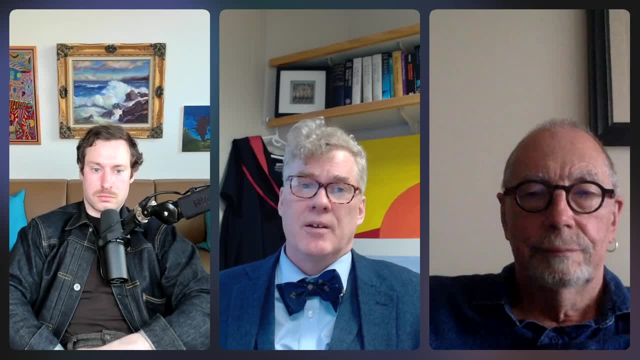 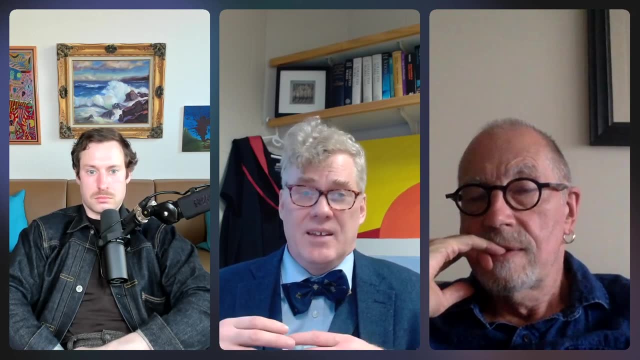 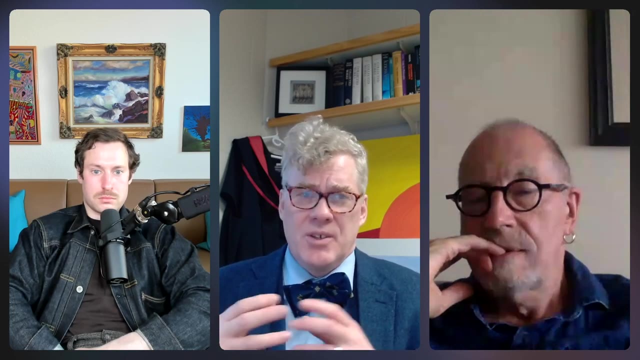 And you're realizing something, And so this is an instance of discovery. But in other cases, in mathematical practice, you're inventing new concepts, new properties that hadn't ever been expressed before, and using them to construct new mathematical structures that hadn't ever yet been defined yet. 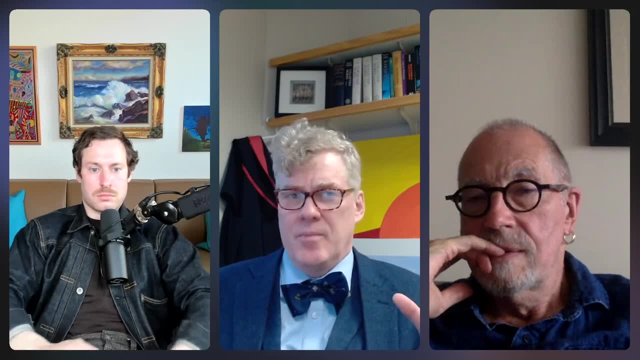 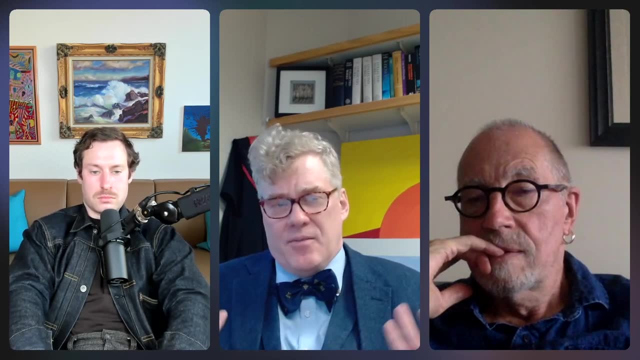 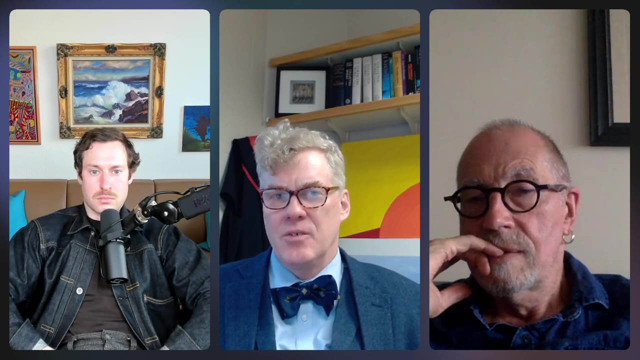 And you're using them and making statements about them. And this almost always has the feeling of invention, Because everything about it is new and you're exploring and it's like what you know, what it's like to encounter something totally new of your own invention. 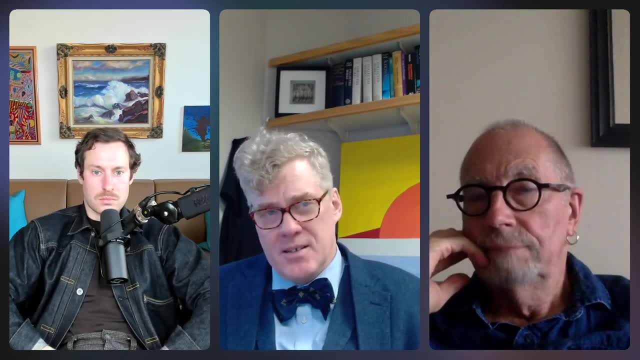 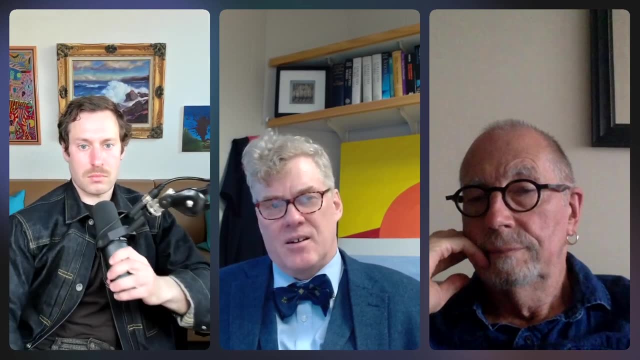 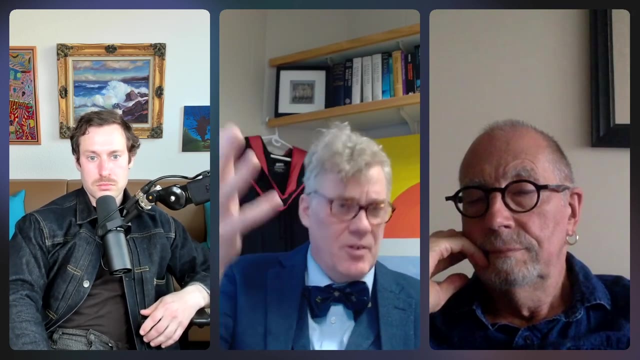 And so I think both of these kind of experiences are quite commonly occurring in mathematics, And therefore I think some mathematics has the character of discovery and some mathematics has the character of invention. Now, but to respond to your sort of suggestion that I should be committed, 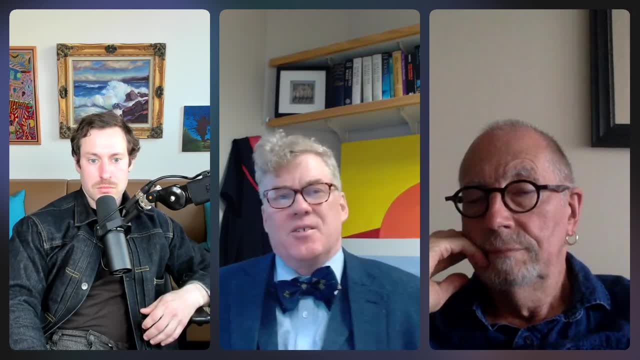 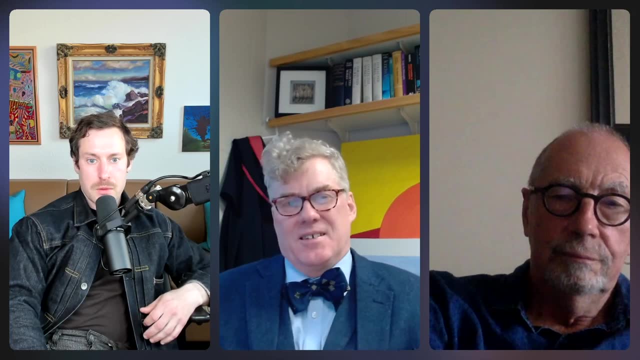 To discovery only because these universes already existed, and so on. And then, yeah, I don't know if I, because I like this sort of inhomogeneous way of talking about it much better, But there's something appealing about what you said. 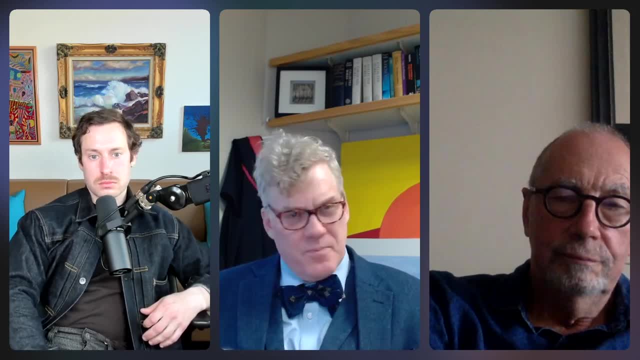 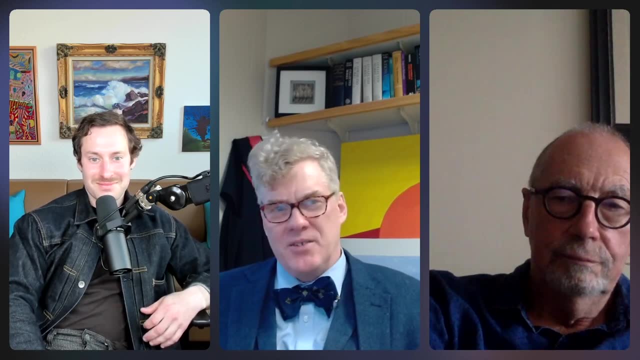 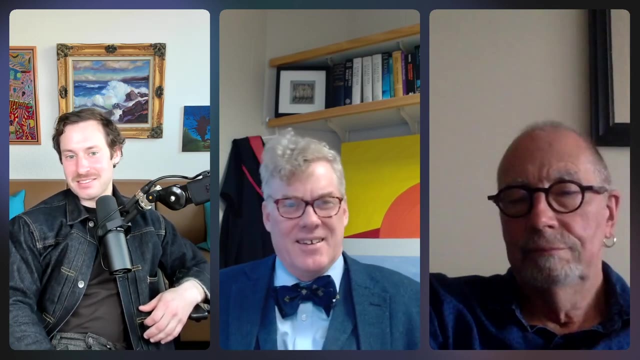 Except I think: look, if I invent a new mathematical thing, you know it's a foobar and it's got two slim gums on it or whatever- Giddy-giddy-bing-bings, Right. So I've been looking at the Google stack, bang, plex hierarchy and someone suggested that the word giddy should be in there. 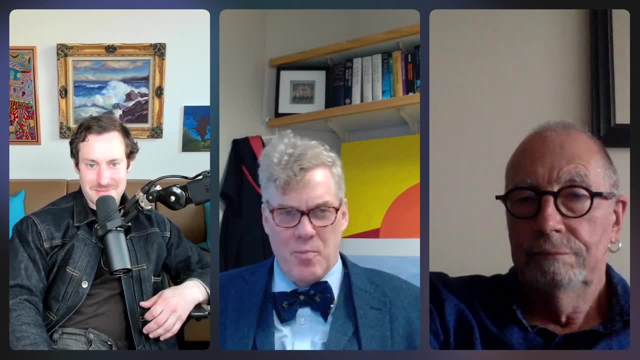 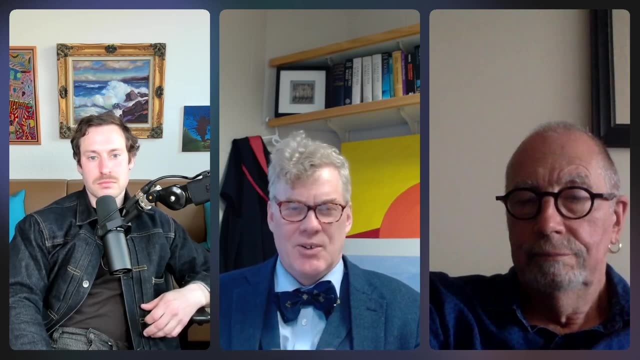 Because I'm looking at which is bigger: a Google plex bang or a Google bang plex plex, or whatever. And so I invented the giddy, And so a Google giddy means Google to the Google, And so now I can form these big numbers called Google giddy-giddy-bang-bang. 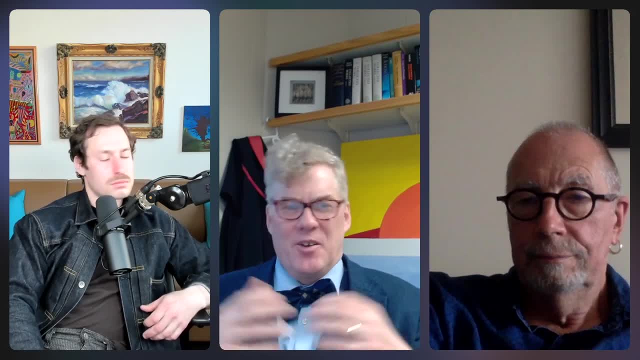 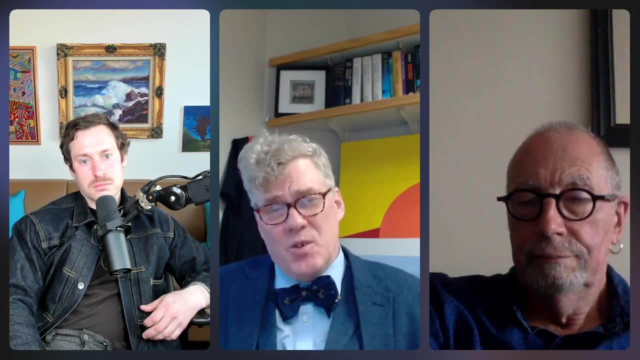 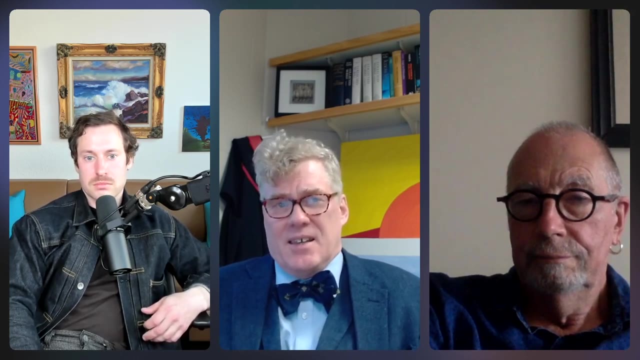 And okay, so this is a kind of invention situation, Although it's really It's just a mathematical operation which already was existing, So maybe it's not a great example. But if I invent some new mathematical concepts and then I study it, then that's exactly the kind of situation where math has the character of invention. 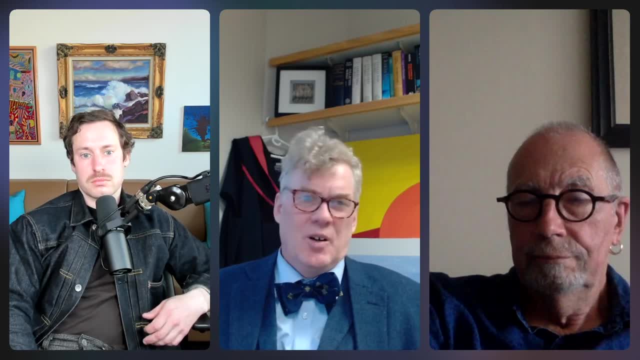 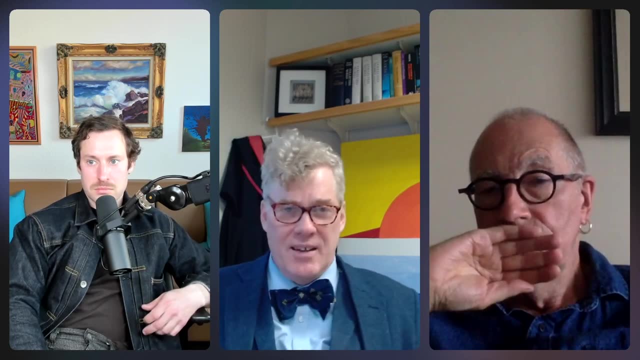 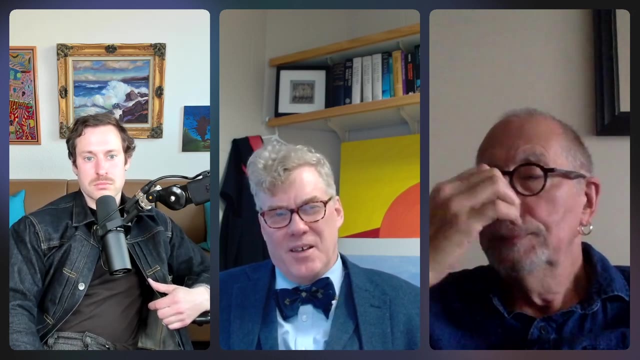 But arguably the structure you know in the platonic realm was there all along, in the same way that Beethoven's 10th symphony was there all along, even though he hadn't ever written it yet, or forever. And so okay, if you really force me, I'll say it already existed, but still it has the character of invention rather than discovery. 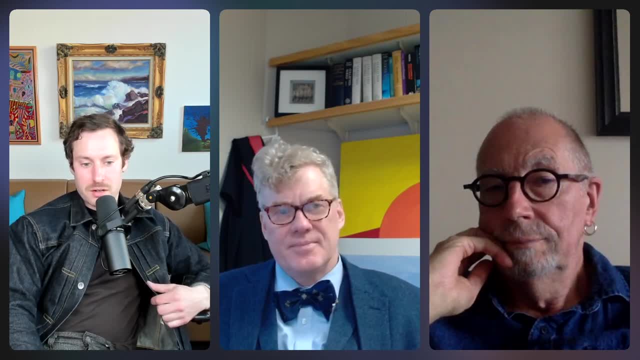 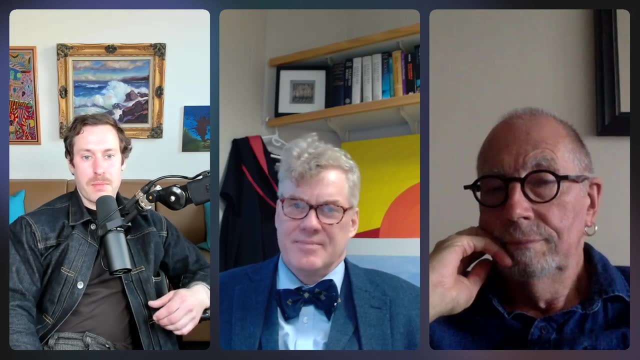 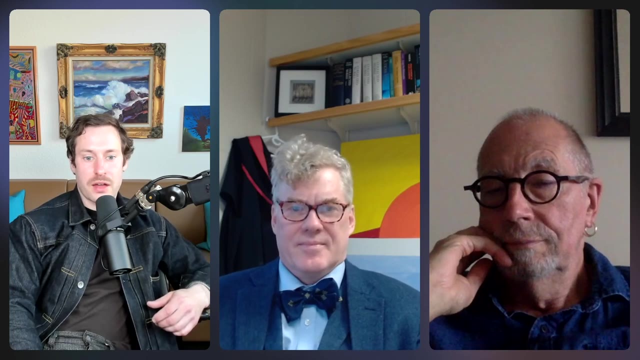 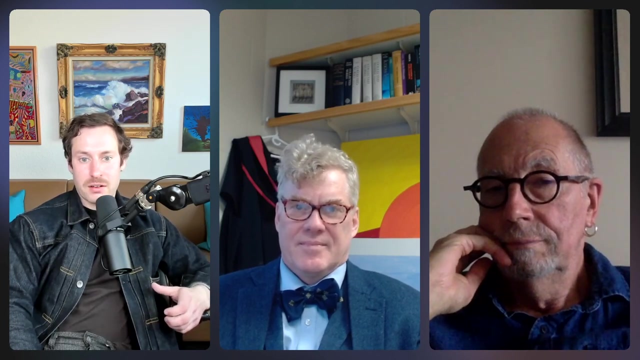 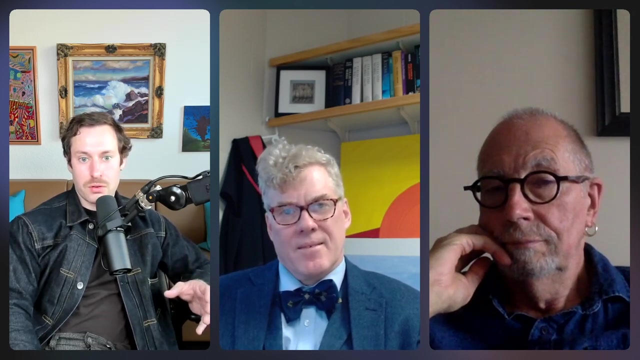 Well, I mean, what it sounds like to me is that you're willing or happy to point out that mathematics has a very creative and inventive element to the practice. But when I hear you say that a mathematician constructs A mathematical structure that hasn't been defined yet, that seems to me to go completely against the sort of ontological picture that you suggested earlier, where you have this very rich ontology of abstract objects and the set theoretic multiverse is already out there. 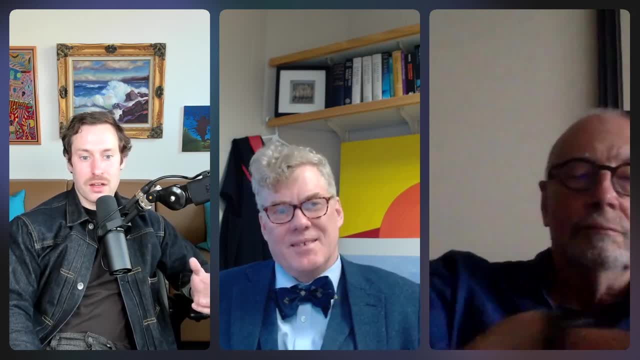 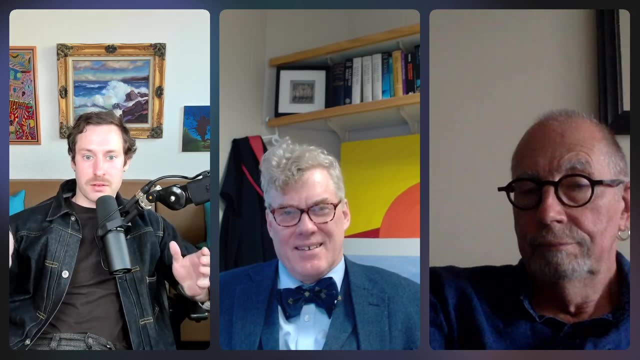 So I don't think you can have it both ways, that a mathematician constructs a mathematical structure, but that structure is already there And there seems to be a Yeah. no, I agree, Yeah, Yeah, I have to think more about it. 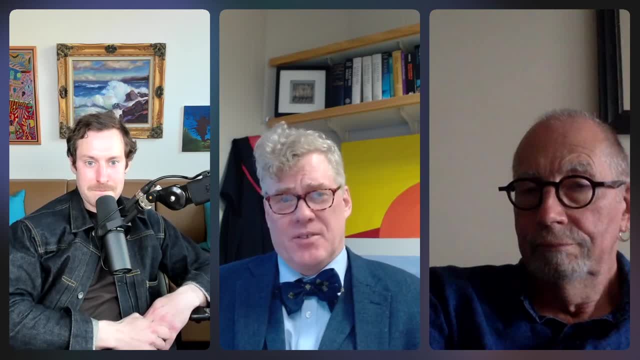 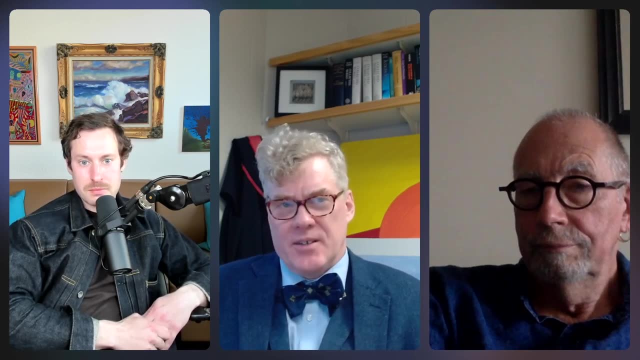 From the personal experience point of view, definitely both situations happen. Okay, So what is the status of these objects? When you invent a new mathematical structure that no one has invented before, then is it more properly said to be a discovery? That's really the heart of the matter. 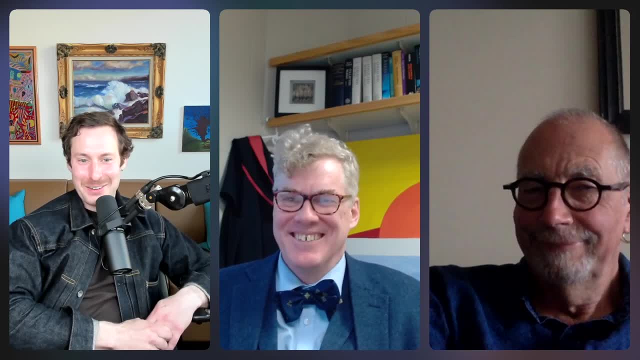 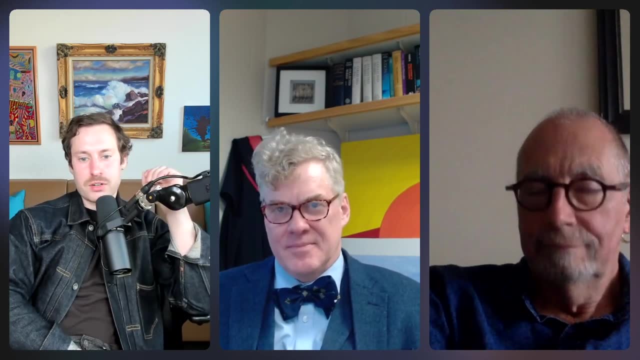 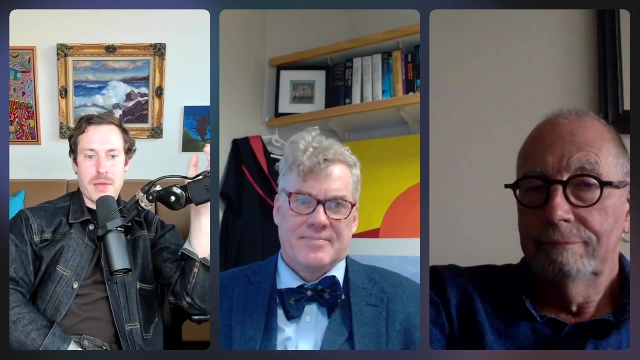 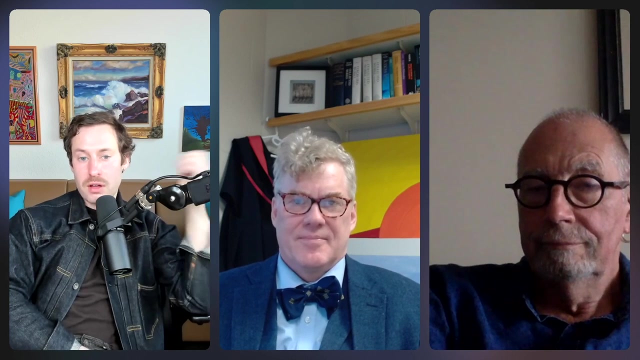 I'm not going to give an answer. No, that's fine. Graham, you mentioned earlier, just sort of offhandedly, that mathematics has been changing for two and a half thousand years, And I wonder if the two of you still think, however, that mathematics is fundamentally the same discipline as it was 2,500 years ago, even though right now- I mean Grant Joel Graham- we're talking about mathematical objects, as 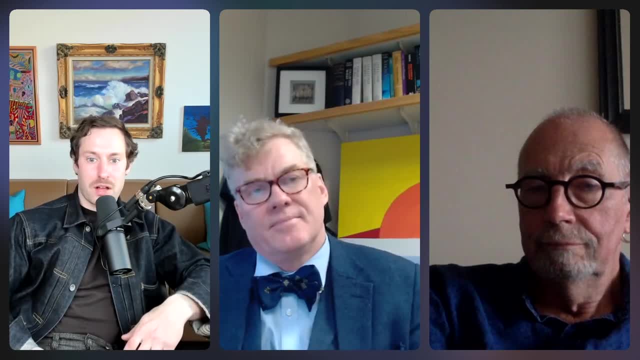 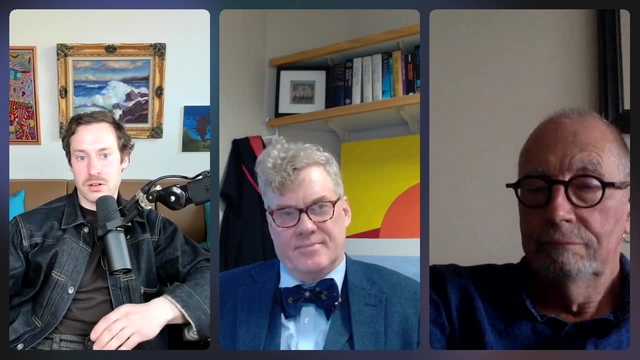 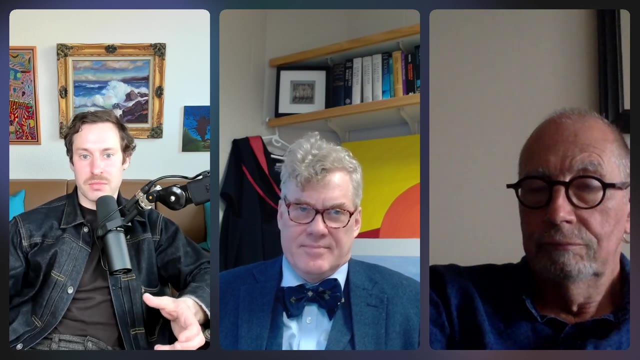 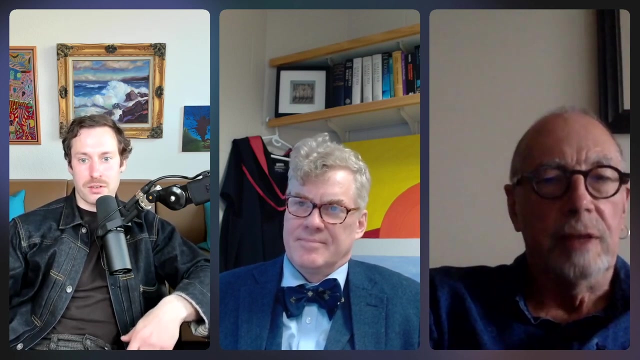 Yeah, Sets, whereas they thought of mathematical objects or numbers like they represented them, as segments. And we have completely different tools. Mathematical culture is completely different. Our notions of rigor and proof are completely different. Are they still the same discipline, or is this again just maybe an issue of language or a category of language? 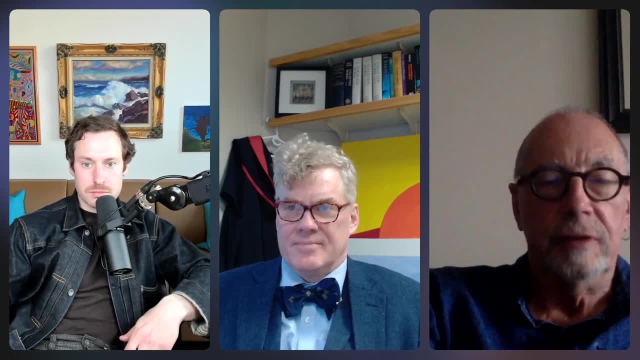 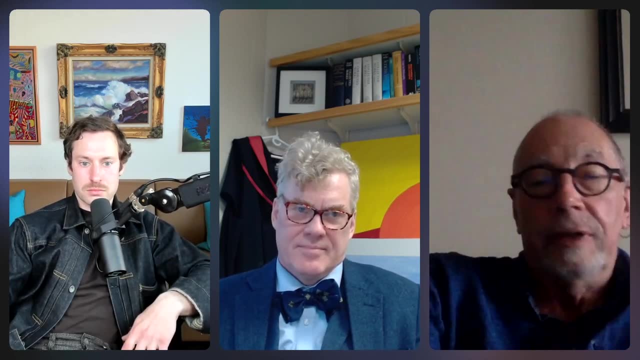 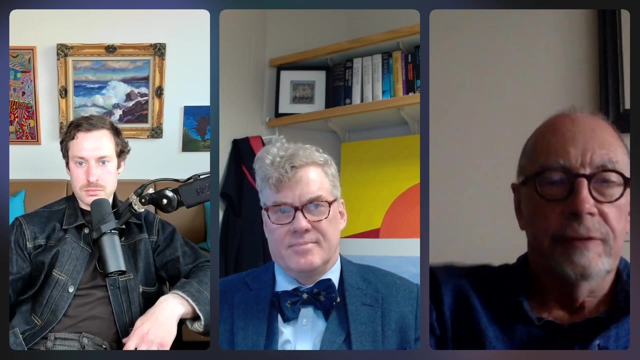 I mean, the same question arises to any intellectual endeavor. right, They all change over time. And what makes an endeavor the same thing over time? You know you can ask the same about any kind of thing. Obviously some kind of continuity is involved and the lines of continuity are very clear in mathematics. 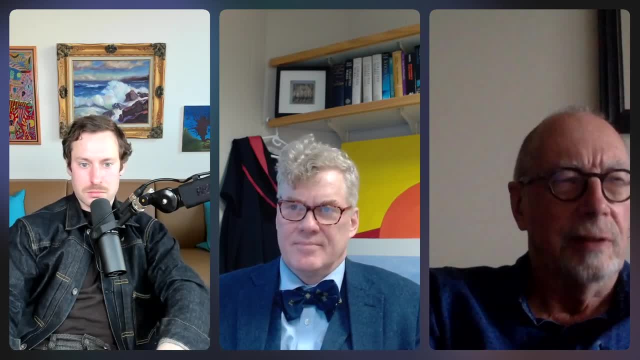 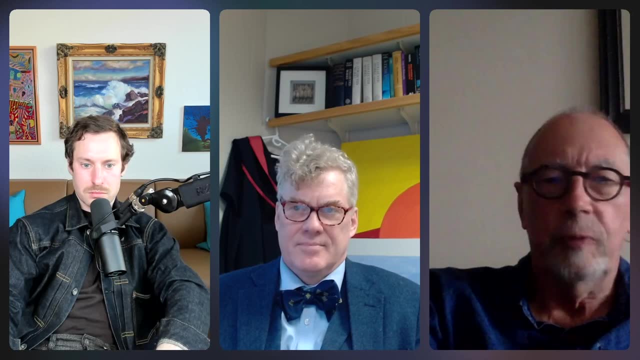 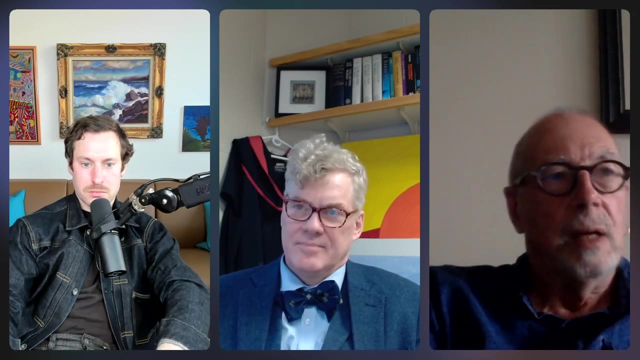 Well, they're not always, because mathematics crosses continents and epochs And then the causal connections become less clear. But you know, set that aside. Generally speaking, there are fairly clear lines of continuity, And that's you know. it's natural to give an identity of those as providing the identity conditions over time. 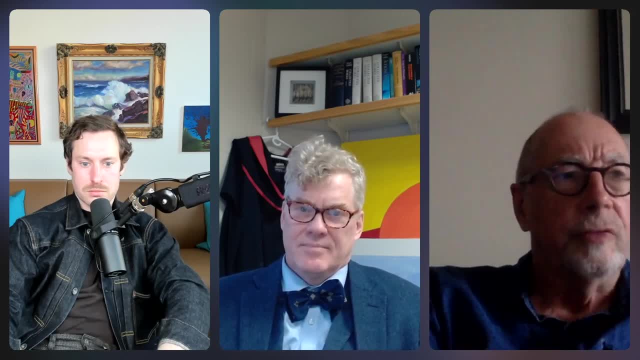 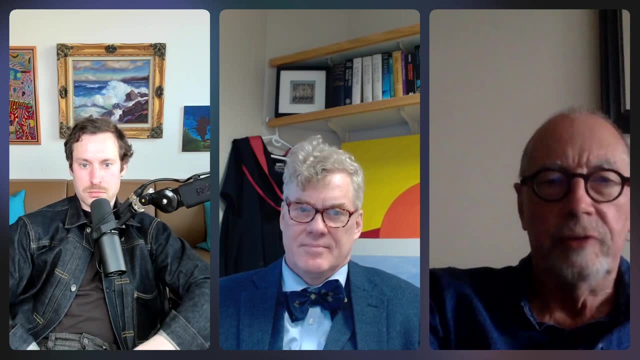 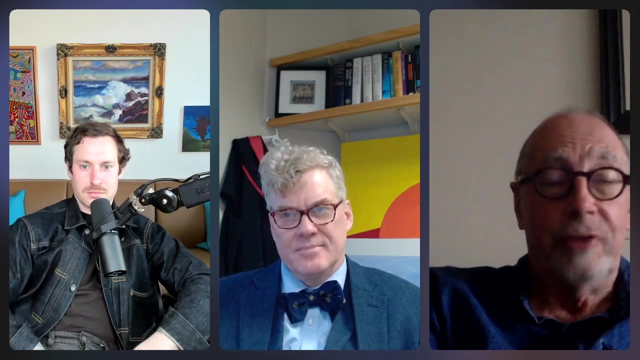 But it's conventional in a certain sense. I mean, was didn't science come into existence at the scientific revolution or before? There are elements of continuity, elements of distinct change. I think You could say yes, it was the same before and after. 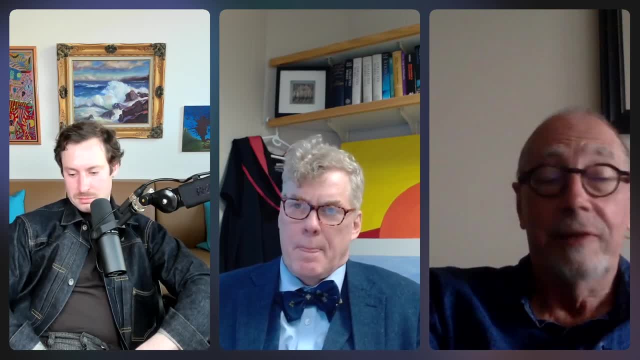 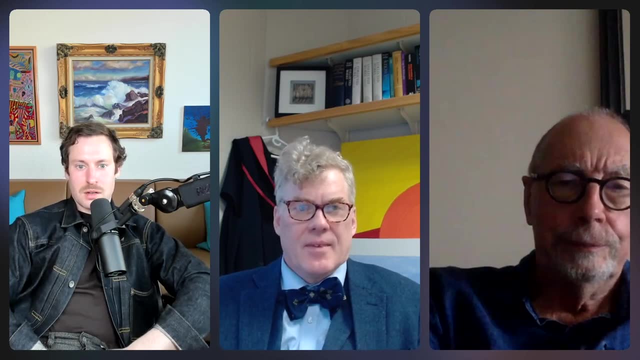 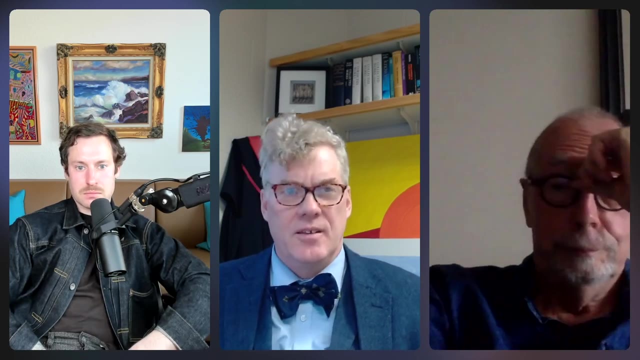 It was science, natural science, or it was different, And I really think that's just a matter of how you, that's a conventional matter. And Joel, what do you think? Yeah, let me mention. So last week I'm teaching a course on infinity, this semester for undergraduates. 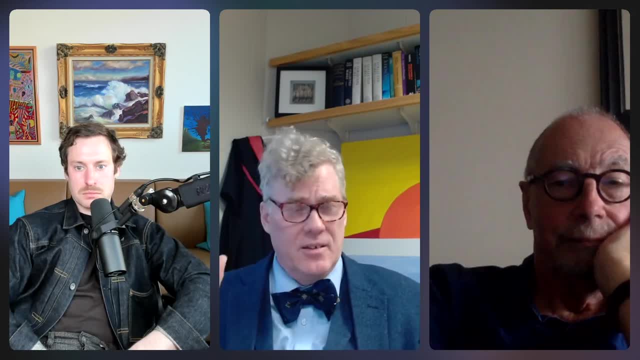 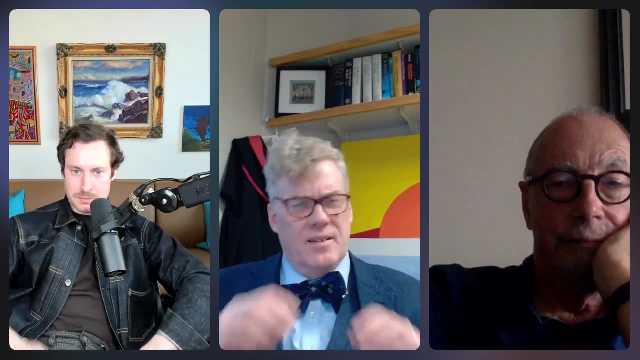 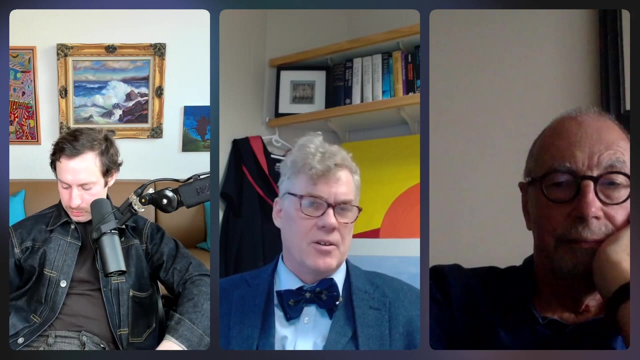 It's like first and second year students and we're doing all about infinity. And I gave a lecture. It's a lecture on Archimedes' method of exhaustion, where he calculates the area of a parabolic segment by filling it with triangles and analyzing the total area and exhausting it. 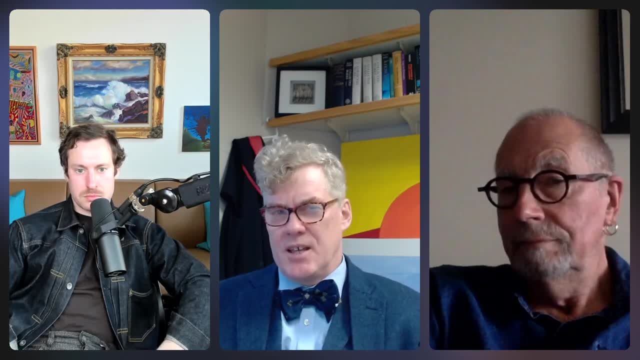 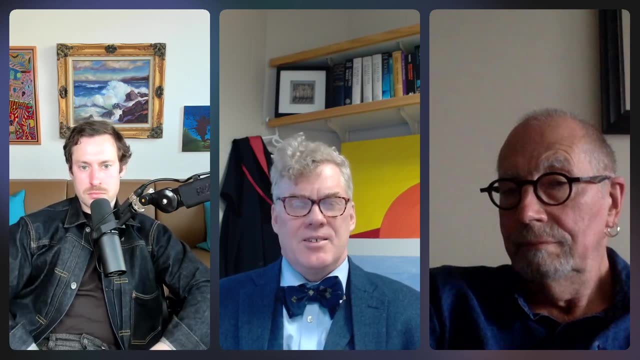 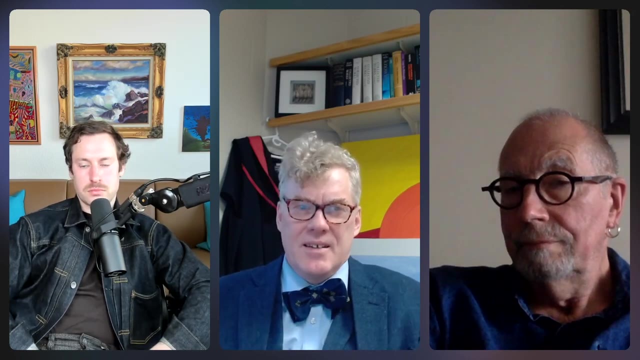 And that work was published in the third century BC, you know, two millennia ago, And it's just amazing to me that there is this kind of continuity And we've been studying that argument for 2,000 years, more than 2,000 years. 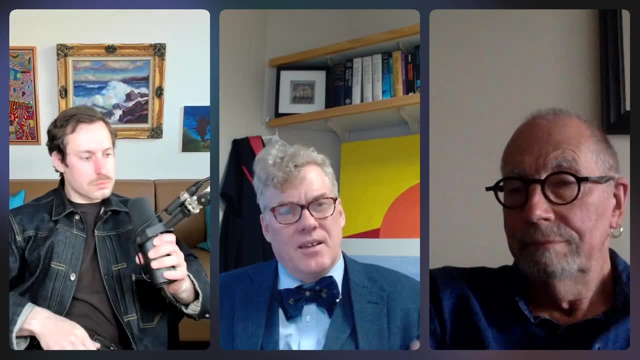 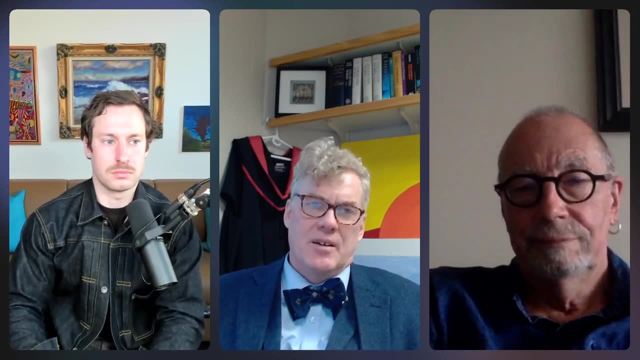 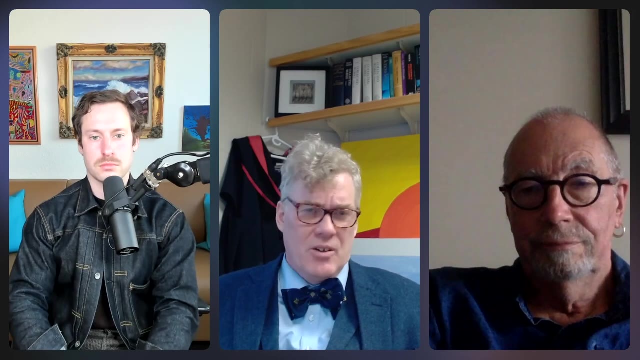 And isn't that incredible? I mean, I think of mathematics as maybe more so than any other subject, I mean, but philosophy is perhaps a close competitor, But mathematics has spanned human cultures, you know, in a way that's sort of invariant between them. 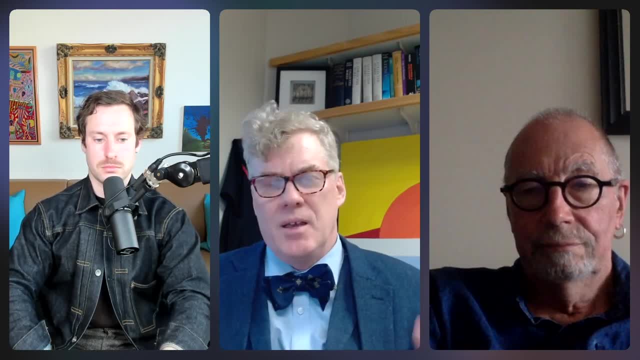 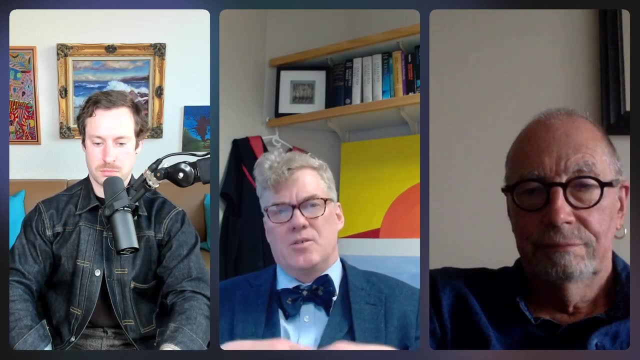 It's not perfectly invariant. If Archimedes was here now, maybe he wouldn't even understand exactly our account of what he was doing. But I think I mean, if one could get over the language barrier, then I think actually we could have a meaningful conversation with him about his argument. 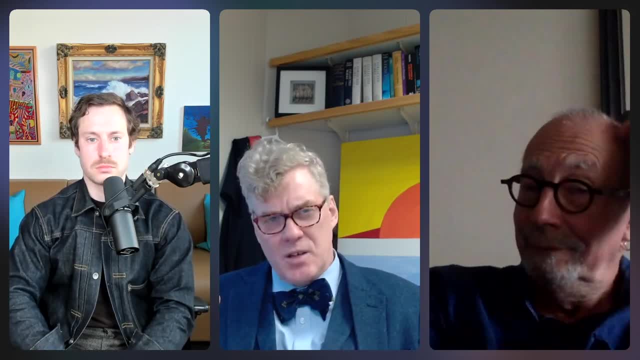 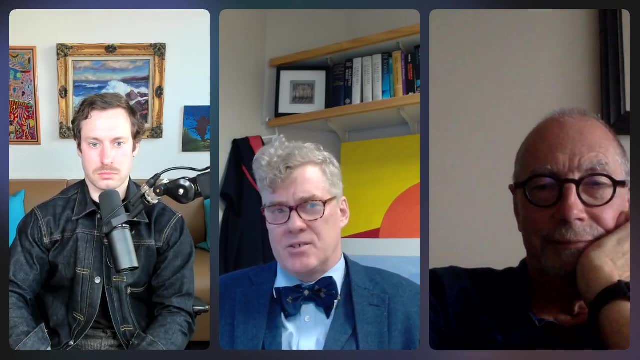 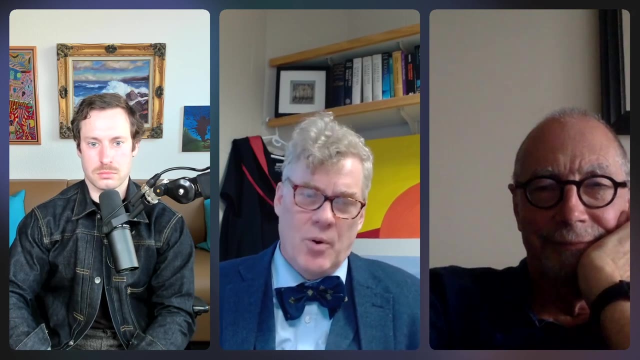 And there's this infinite sum involved, And his treatment of it is very much grounded in potentialist conceptions of infinity rather than actualist. But we would still be able to talk about his argument And in a way I think that would be meaningful on both sides. 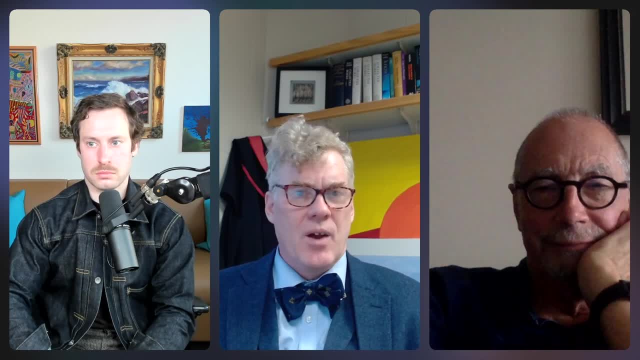 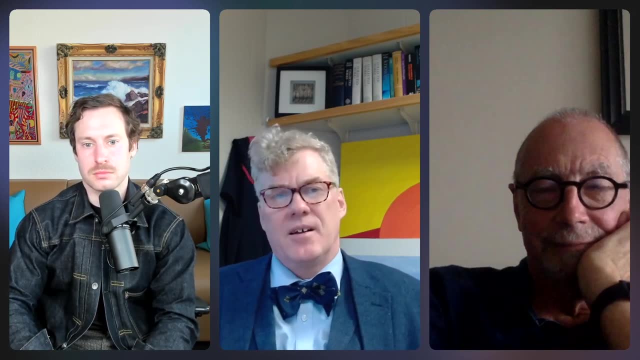 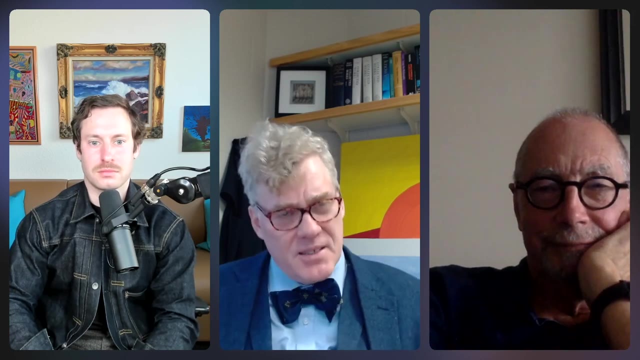 And I just find that incredible, that situation where a mathematical idea has been transmitted from culture to culture to culture, you know, continent to continent, and is now appreciated and understood by people all over the world. And this happens again and again and again in mathematics.